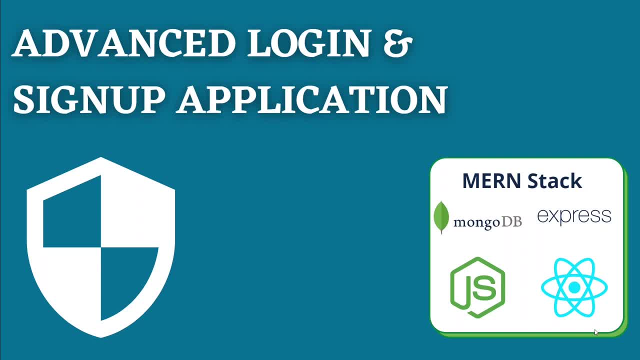 wanted to learn the authentication and authorization techniques, So this course is for you as well, and I will teach you how to build the complete, secure backend. So let's see The demo of this application. So this is the application which we are building. So we have a. 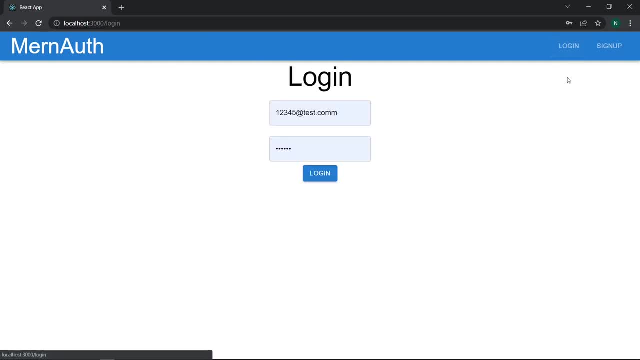 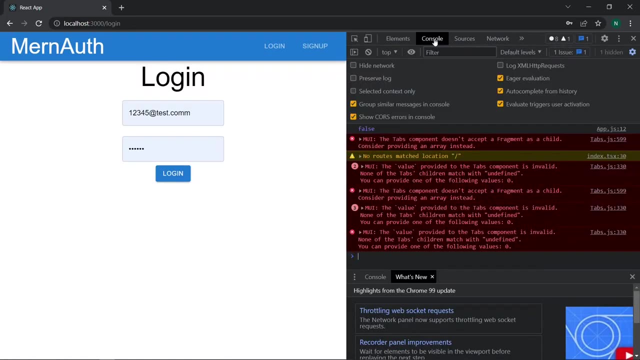 screen and then we have a navigation bar and once I will click on the login now you can see the login tab will appear and then we have some text boxes inside that and once I will go to the inspect to check the console and then you will see the initial state of the redux is false. Once I will click on 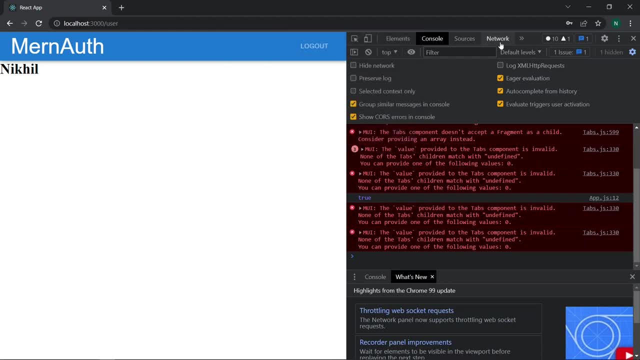 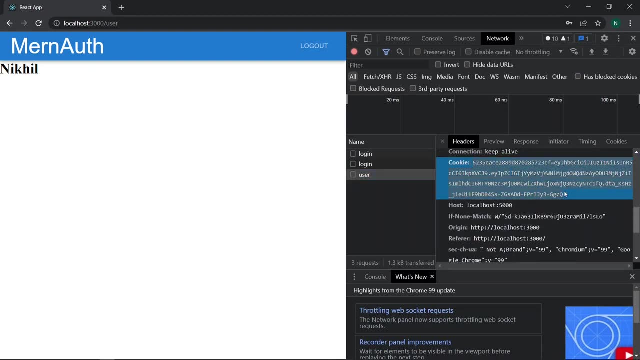 the login. now you can see we have my details and now once I will click on the network tab. now you can see we have the user details and it is now getting the details. and now you can see we have a unique key which is not accessible on the front end. So if you will access on the front end as the 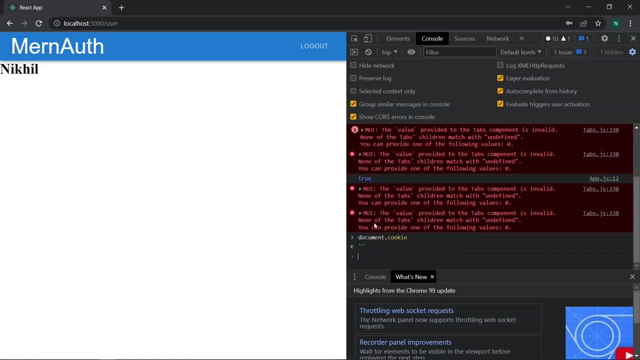 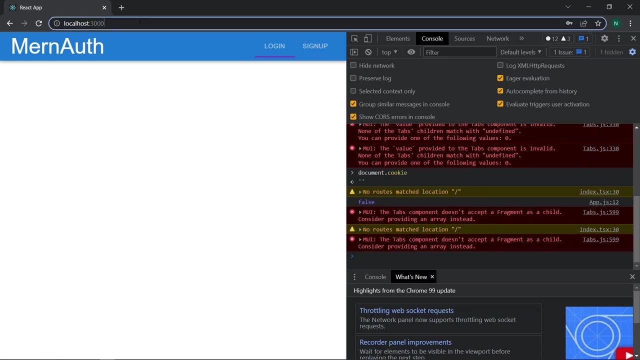 documentcookie. So then you will see we have empty string because we cannot access the cookie in the front end. and then we have the logout screen as well. Once I will click on the logout and then you will see now we are logged out, and once I will go to the users page again, so to see my details again. 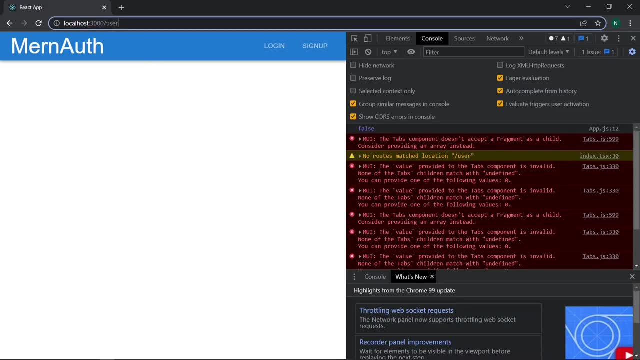 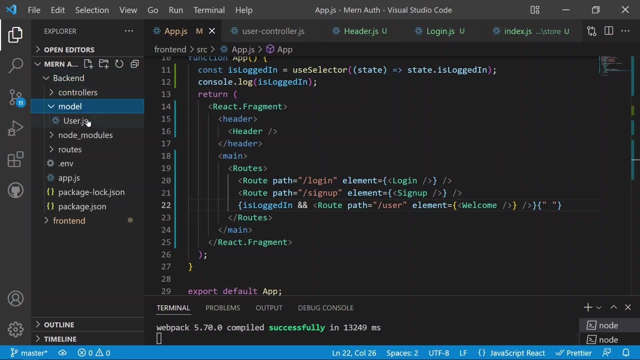 now, you will see, it will show us that the no route match to the location as the user, because these all are the protected routes. and then we have here the back end running on, and then we have the front end running on, and then we have the models of the user and then we have the controllers of the users. we have some. 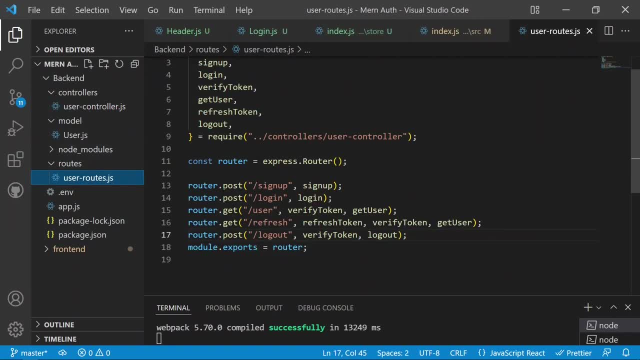 controller functions. and then we have the advanced routing here as we have the post request of the signup and the login and then to get the user, first we will verify the token and then we will get the user, and then, after the users token will expire, so we will generate a refresh token, so the 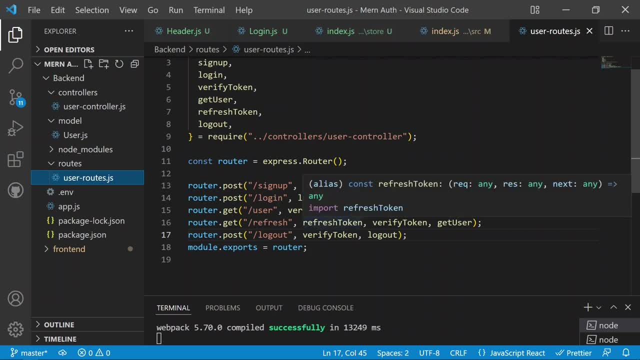 token will be refreshed from this token and then we will just get the refresh token and then we will verify the token again and then we will show the user their details of the get user routes and then we have a logout as well to verify the token and then we will remove the token from the. 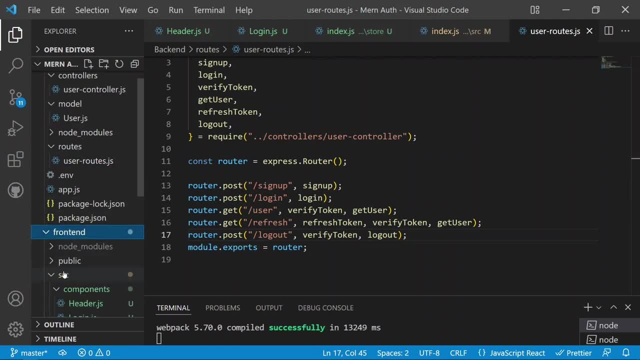 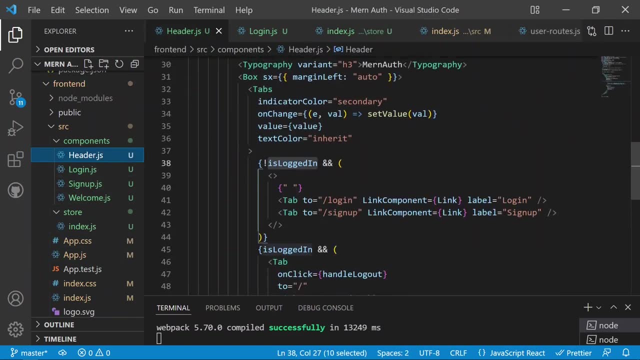 cookies. so these are about the back end, and in the front end we have the material ui, we have the redux, so here we have the redux slice, we have a comma and then we have a header, we have a navigation bar. there we have some routes and then we have the appjs, where we are rendering some routes, like the. 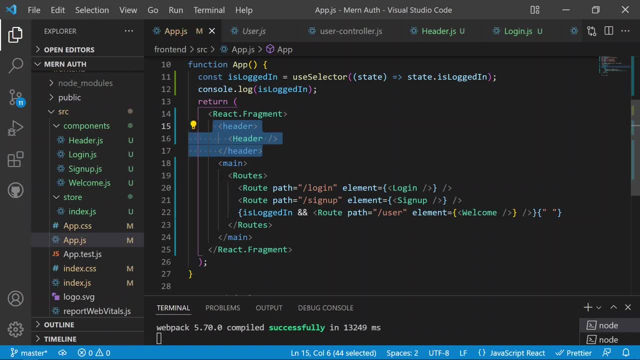 header. we are rendering the header for every route and then we are handling all of the routes there and then these are the protected routes. so if the user is not logged in, so we can't see the user route, and then we have everything working fine. so this is our application. so let's start building the 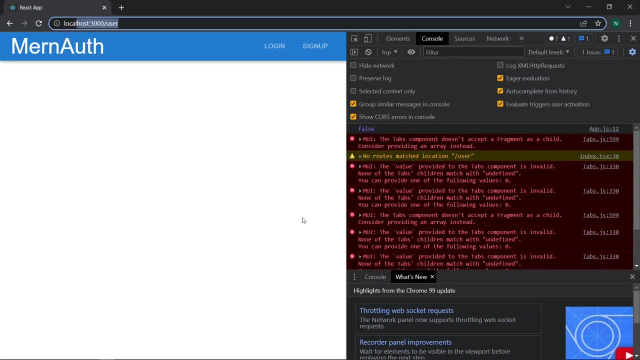 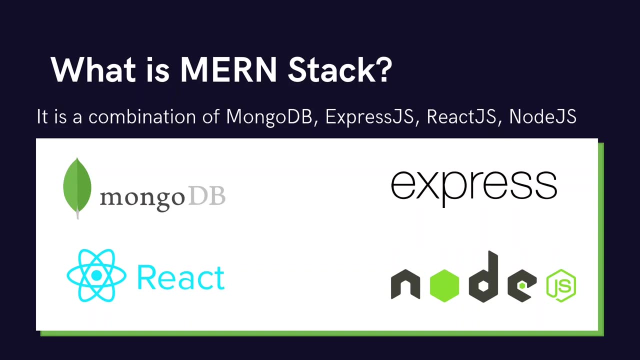 application, and for that we have an introduction video as well. so let's start with the introduction. so, before moving ahead, let's see some introduction about some topics which we are going to use in the application. so the mern stack. so mern stack is the combination of the mongodb express, js, react js and 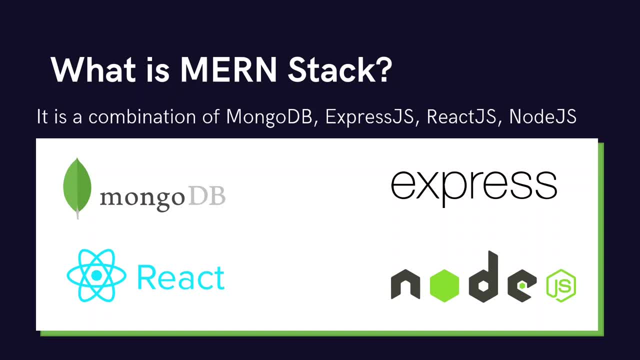 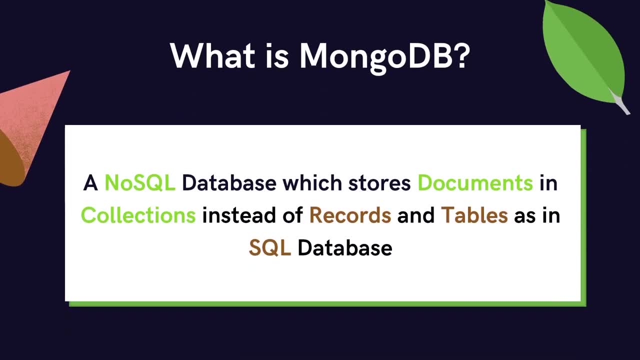 the node js. mongodb handles the database operations and node and the express js handles the server side task and the react js handles the front-end tasks. so what is the mongodb actually? so mongodb is a no sql database which stores the documents in the collections instead of the records and 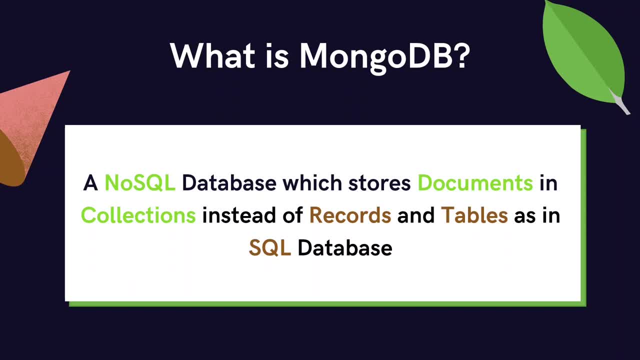 the tables in the sql. so about a collection? so collection is like a collection of multiple documents inside that and a document is a record inside a collection and if you are coming from this collection, you are going to have a collection of multiple documents inside that. and if you are, 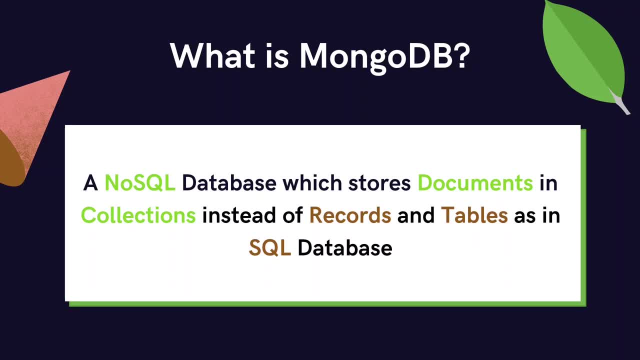 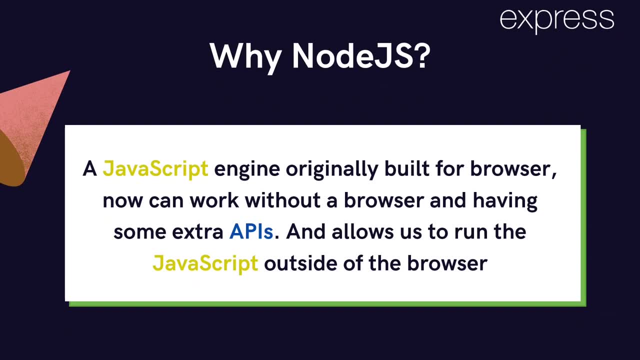 coming from the sql database. then you can relate to the table as a collection and the record on the table as a document. so about the node js? so it is a javascript engine which was originally built for the browser but now can work without a browser as well and having some extra apis inside that. 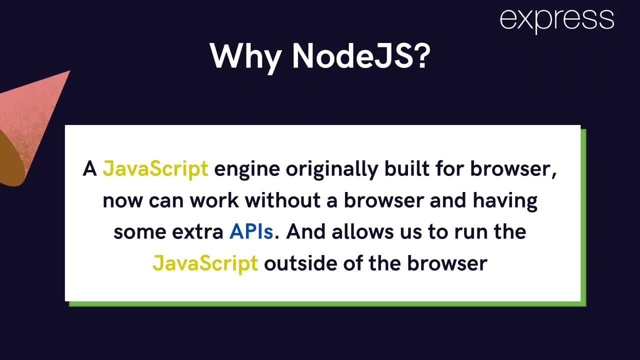 and now it is known as the node js and it allows us to run the javascript outside of the browser now. so initially it was just built for the browsers only and we can see about the chrome's v8 engine, so it was like the chrome's v8 engine that we use, but now it is being maintained as a 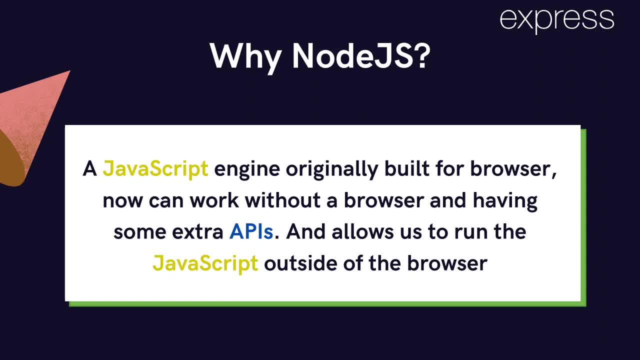 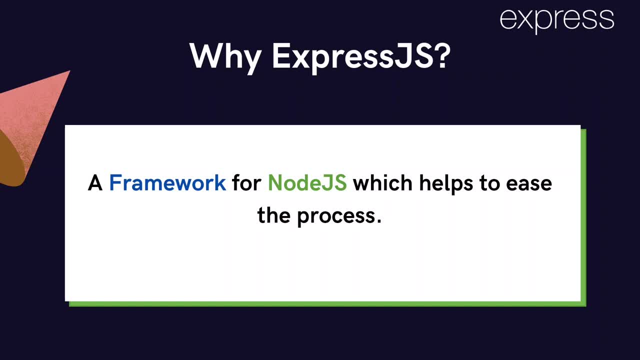 standalone project called the node, and then it have some extra apis as well to use the javascript outside of the browser as well. and now about the express js. so it is just a framework for handling the server-side task that helps the node js to ease the process, and then it contains some controller. 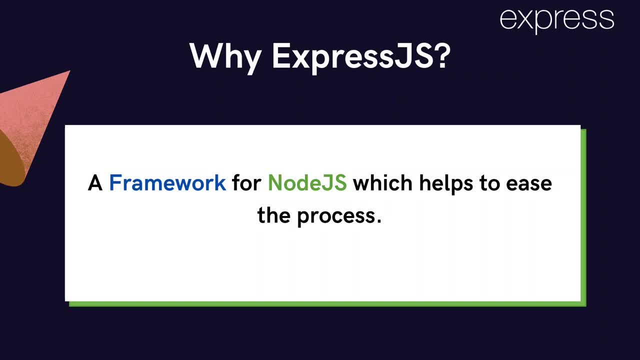 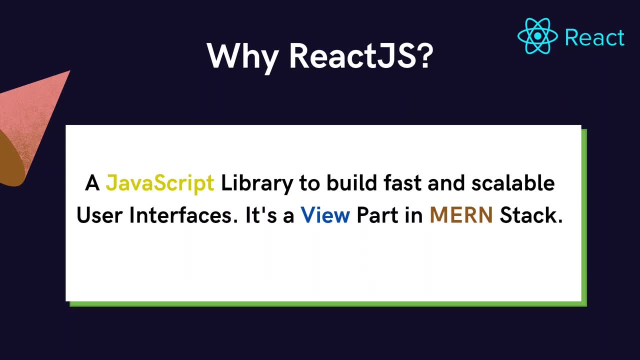 functions as well. it contains the routing, so like it contains all of the http part as well. so now about the real javascript engine. so it was like the chrome's v8 engine. so it was like the chrome's react js. so the react js is just a javascript library to build up fast and the scalable user. 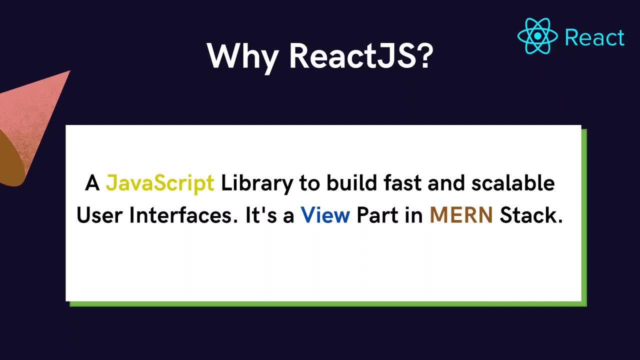 interfaces and it is a view part in the mon stack and the models and the controllers comes in the backend parts and it also combines to the mbc, which is a model view controller application, and it is then combined to the mongodb. and now the main topic of this project, which is the 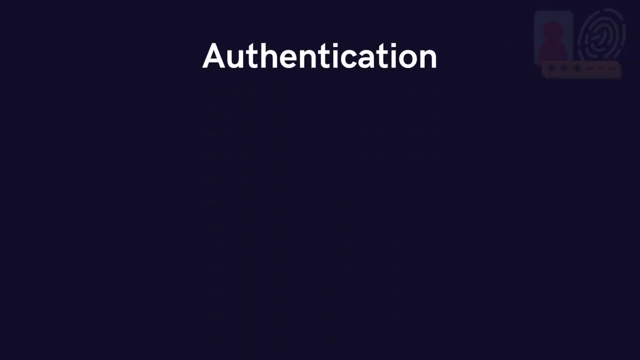 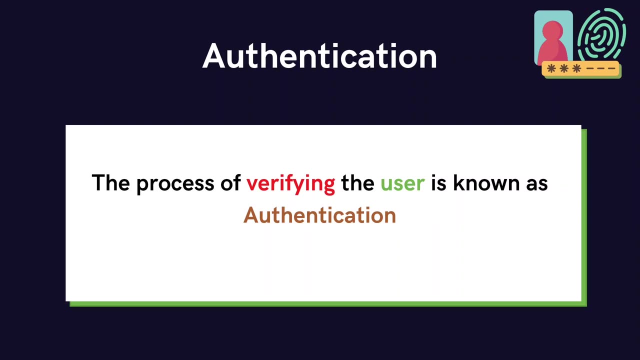 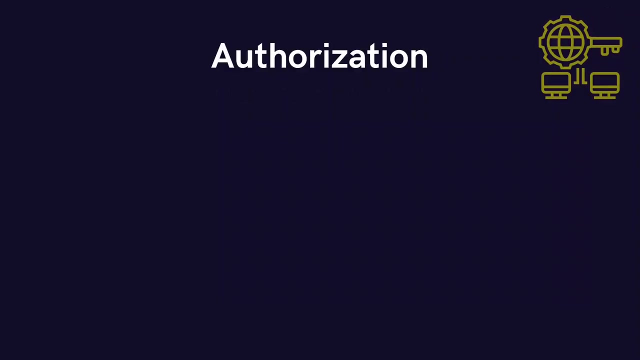 authentication and authorization in the mon stack. so about the authentication? so it is the process of verifying the user. like we verified the user, buy its credentials, like its email and the password, and if the credentials are correct, then we just authenticate the user and then we have the 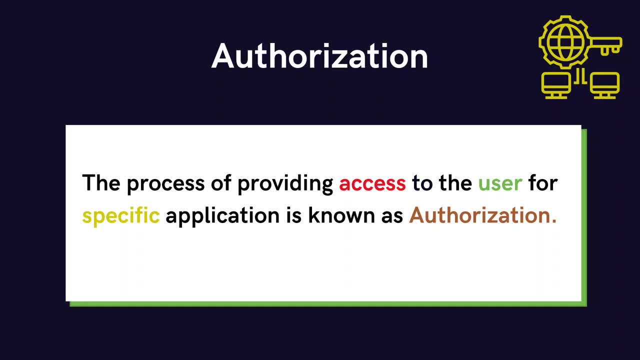 authorization, so it is the process of providing the access to the user or some specific application after the authentication. so, in simple words, authentication is the process of verifying that who the user is, and while the authorization is just a process of verifying for what they have access to in our application, like we can just provide the access to the user. 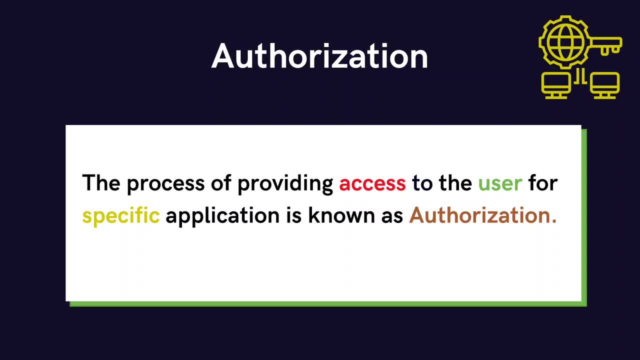 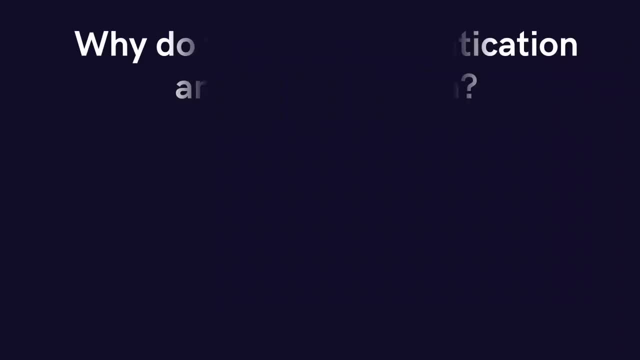 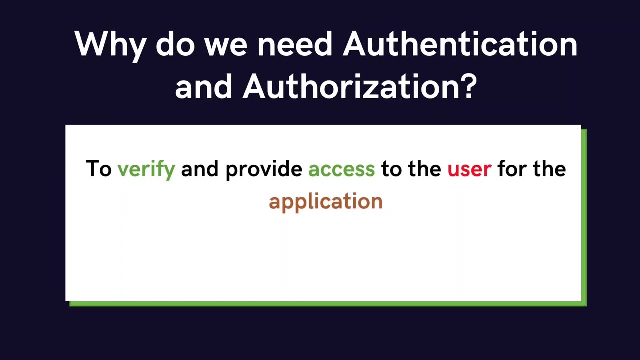 to see just the details of it, but not to modify it. so we have some authorization part, like for what part of application we provide the access to the user. so now why do we need the authentication and the authorization? so we need the authentication and authorization to verify and provide the access. 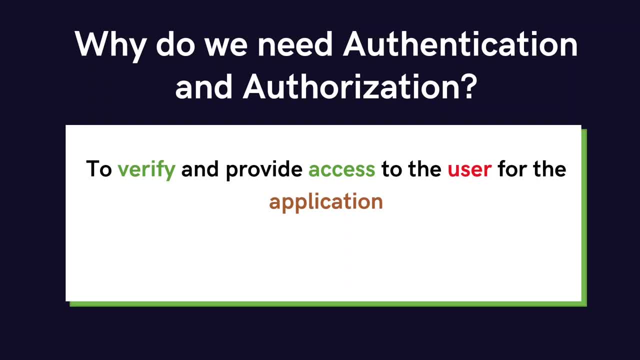 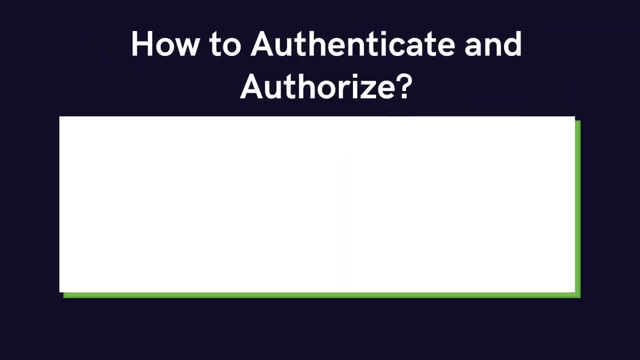 to the user for the application. like we cannot provide the access directly by knowing the password and the email, we just do the authorization as well to provide them the access. so now how to authenticate and authorize the user? this is a very big part. so first we verify the user's credentials. 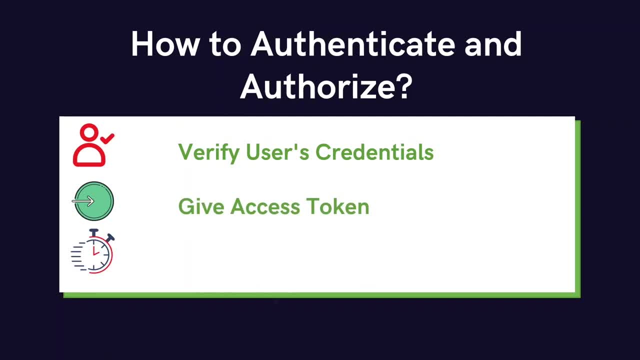 and then we give them an access and then we set the token expiration time. so first we will verify the user's credentials and then, after the credentials are correct, then we will provide the access token to the user and then, after the access token is granted, then we can just set. 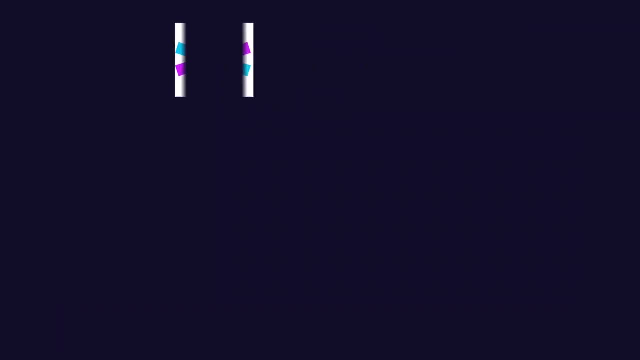 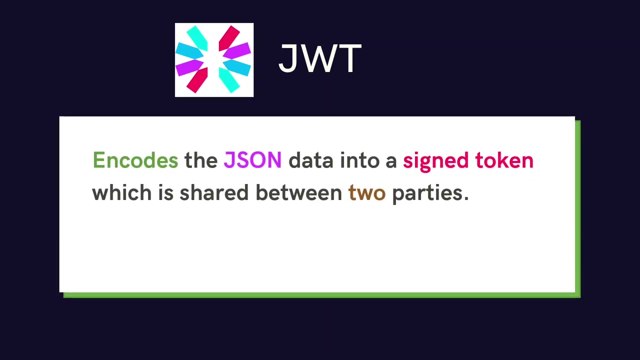 the expiration time for a specific token. but wait, what is a token? so tokens are used to provide some access and in this project we will use the JWT, which is a JSON web token, which is a library to use, and it encodes the JSON data into a 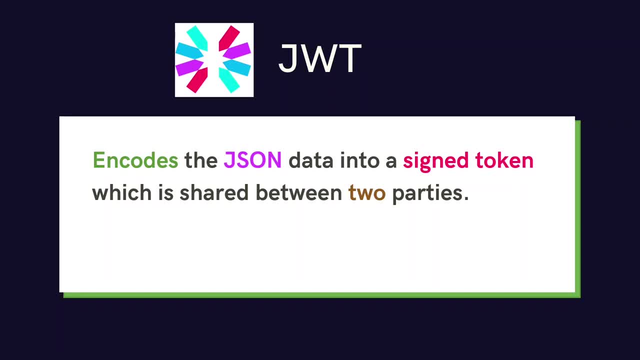 signed token which is shared between the two parties, which are the back-end and the front-end. so it creates an encoded data of the JSON which will be providing, like we can provide the ID of the user, the name of the user inside the JWT and send it encodes that data and it provides the user that token that it. 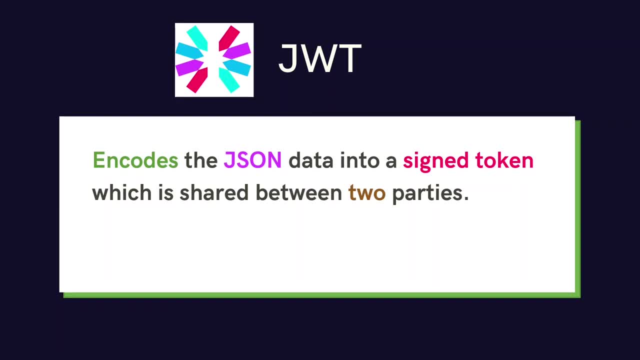 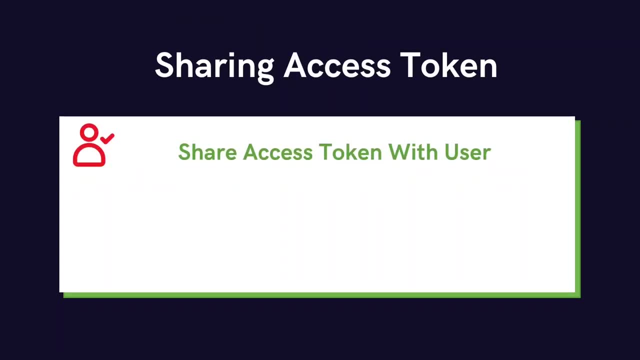 contains your crucial information and don't give it to anyone. so this is about the token, and then we will be using these tokens. and now we need to share the access token. so we share the access token with user after the credentials are true and then we need the token back from the user again. so once we will, 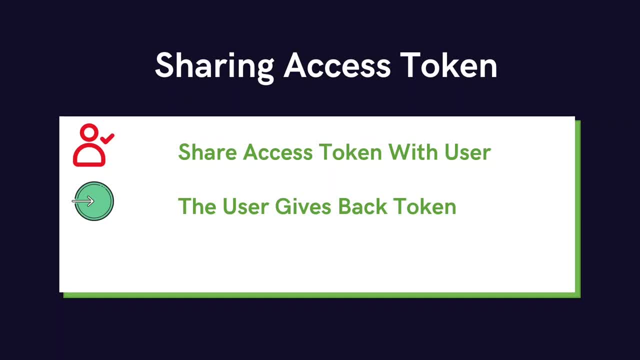 share the token with the user. now we need the token back from the user to verify the details and then to send them the details. so after we will get back the token and when we will verify the token, so then the verification completes and then we will provide the access to the user. so about the access? 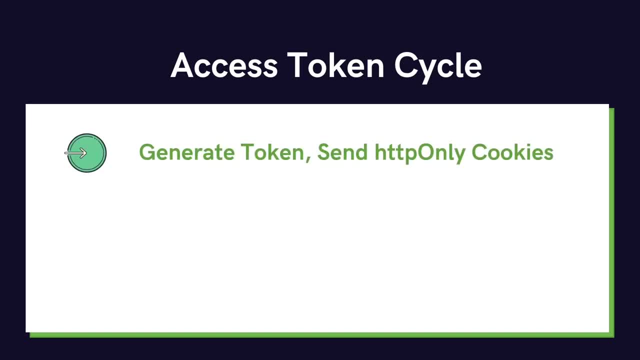 token cycle. so we will generate the token and then we will send the token inside the HTTP only cookie. so, after the verification is completed, we generate a token and then we will send the token inside the HTTP only cookie, and these are the cookies which will be set. it from the back-end, not from the front-end. 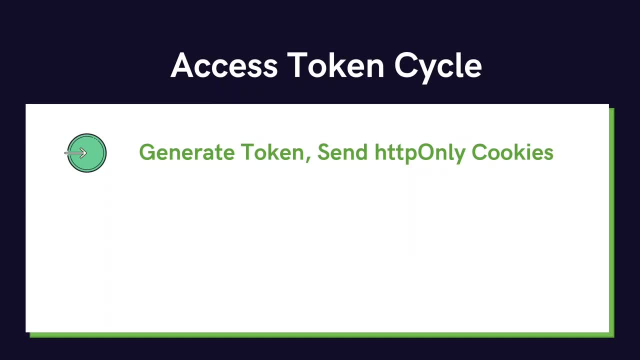 and then it will be added to the request headers which will not be accessible to the front-end. so any front-end user cannot access that cookies and we are using the HTTP only cookies because of knowing the accesses attacks nowadays, which is the cross-site scripting attacks, where the attacker 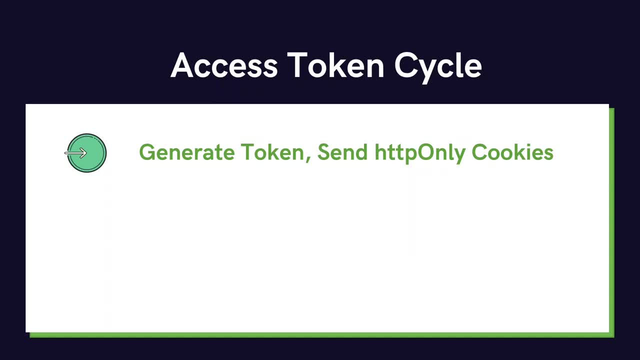 adds some malicious code to our website and the attacker can steal your token as well and then it pretend to be you and it can do any harm to the application and for your data as well. so we don't share the token with the front-end and we just add it to the request and then we will just get back. 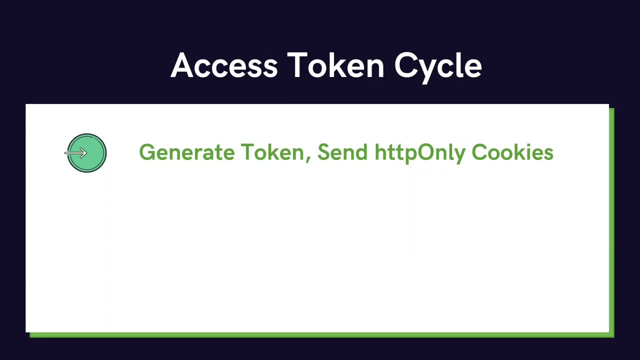 the request from the user via the server side only, so it is not accessible to the front-end overall. so the front-end cannot access the HTTP, only cookies, and then the browser sends back the cookies to the back-end. so this is possible just because of the xos. so exos allows us to send the credentials which we will. 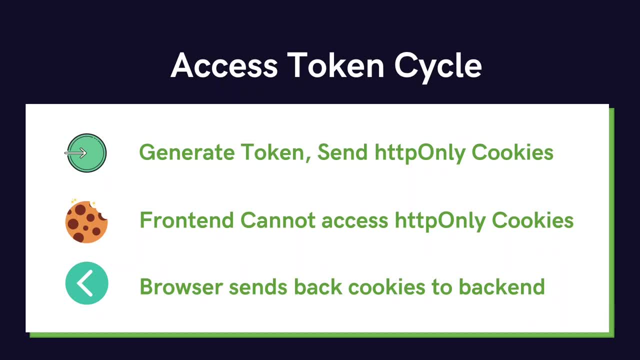 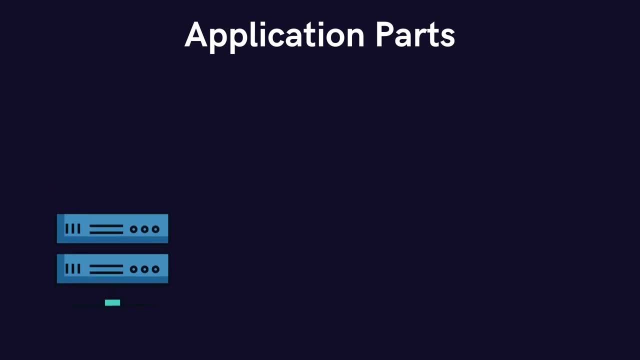 receive from the back-end to the back-end again. so it will be done from with the help of the xos. so we will use the xos to do that, and then the we have the application parts. so first what we have, the backend, and then we have 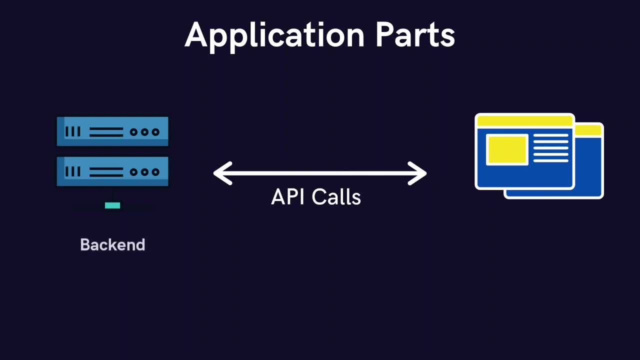 some front end and then we are connected with the api calls and the backend is built with the node js, the mongodb express js, and with the jwt, which will send the tokens, and with the bcrypt js, where we will hash the password and we will just encrypt the password of the user, and then we are using the. 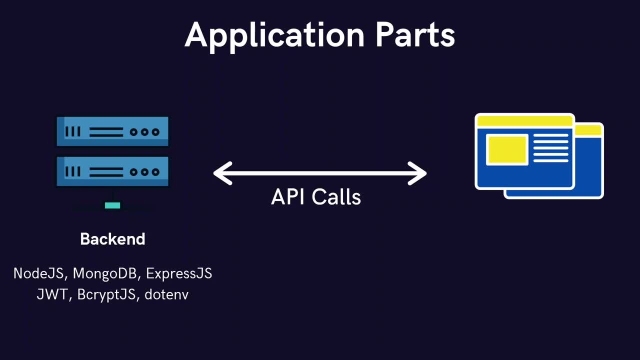 env as well to protect some variables, some key variables, from the code. and we will add to the environment variable sonv, which will be only accessible by the processenv. and then we have a front end application and then it is built with the react js and it is built with the redux. we 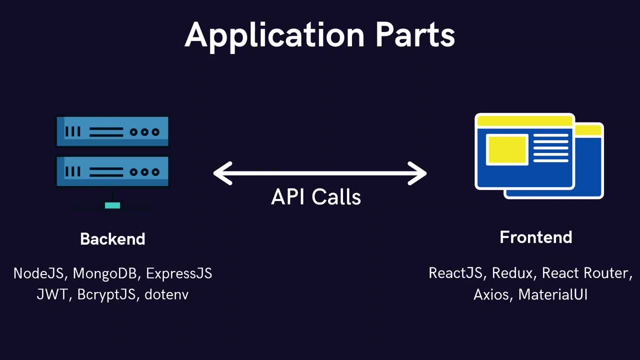 will add the redux for the authentication states, and then we will add the react router and it will handle some routes and we have some protected routes as well, and then we are using the xios to send the request to the backend and then we are using material ui, some components of the material ui, to make some stylings in the application. 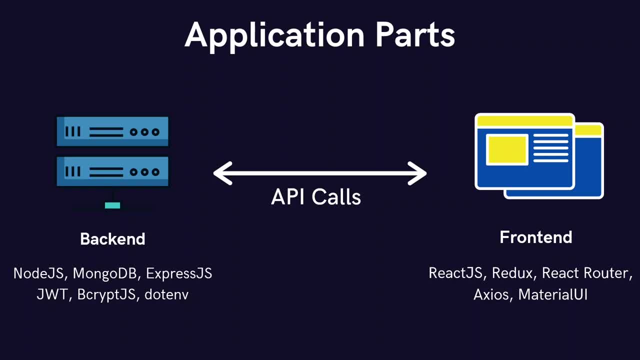 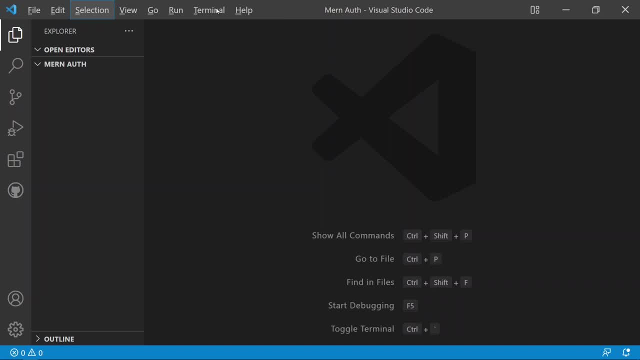 so this is all about the introduction, so let's start building the application. so now, after all that discussion, now we can start building the application. so now we will create the backend application first. so i have opened a folder in the visual studio code and now we have. 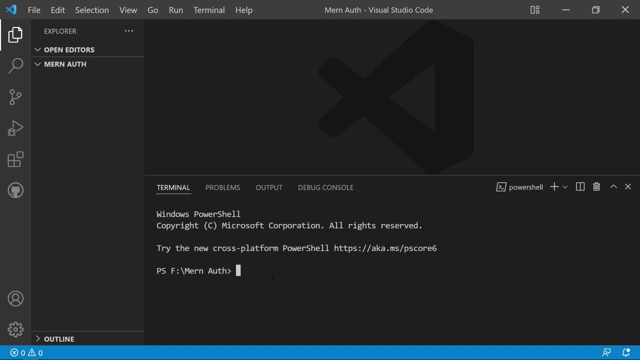 to go to the terminal and then we need to select the new terminal from there and then we need to install the nodejs application, and to install that we have to enter here the command as the npm init. so after entering this command, then you will see, there will be some questions, like the package. 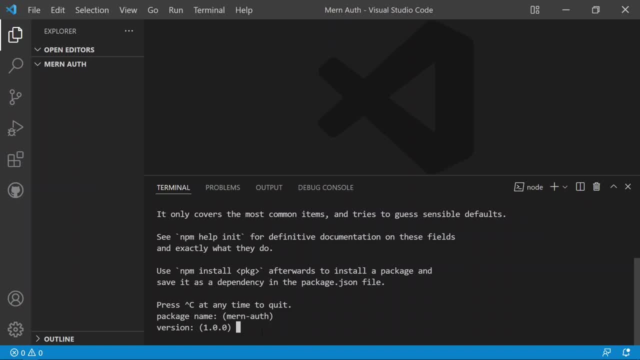 name of our application. so you have to press enter and then you will see we have the version. so initially we will be having the version as the 1.0.0. so we have to press enter again and then the description. we can provide the description as well, but i will not provide here. press enter. 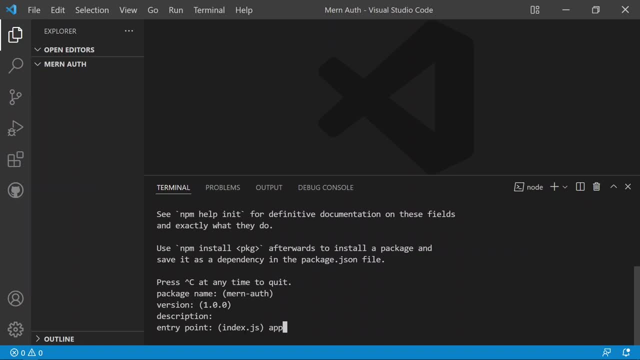 so then you will see. now we have the entry point, so we can change the entry point to the appjs, and then we have a test command. but we can skip all that. so you have to press enter, enter again and again and then license here, and then you can just press enter again. so after this you will see. 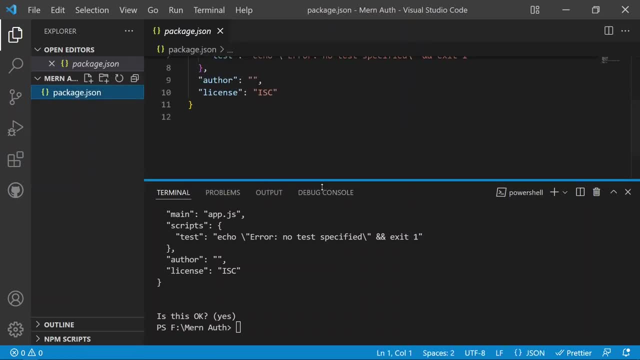 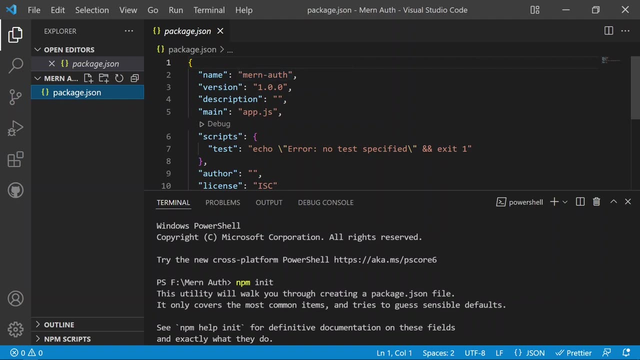 there will be a packagejson file into your directory. so the npm init command creates a packagejson file which have all of the information about your application, like the package name. we have the month auth. we have the initial version of the 1.0.0 description. for now it is the empty. 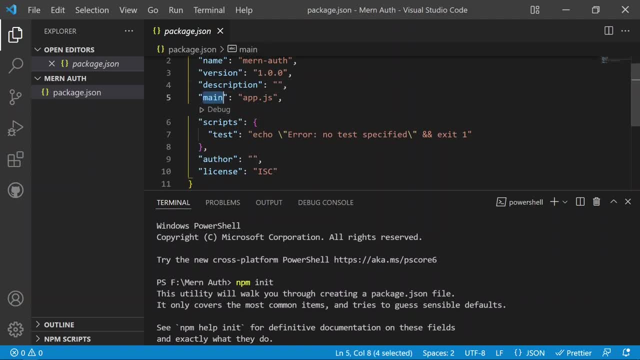 string, but we have the main file as the appjs and we have the scripts as the test, and then we have the author and the license. so we have all of the details of our application. so now we can just create a new file as the appjs to create just a hello world application. so first, 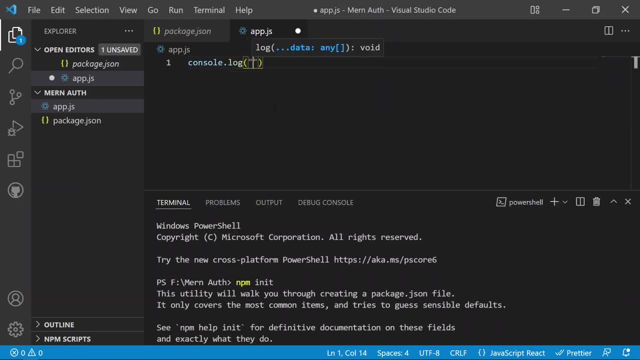 we need to get the as the console dot lock and it will be the hello world. so if i would now save, now we need to run the application, but now how we can run the application? so as of now, we don't have any service installed like the node bone which will automatically. 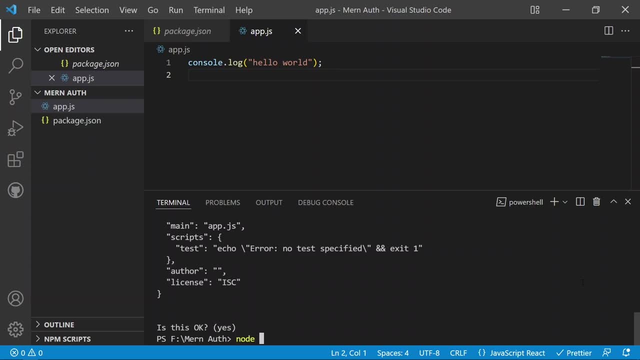 identify the file changes. so we can just run the appjs with the node appjs command. so you have to enter this, then you will see. now there will be the hello world on the terminal. but now we can just create some commands, like there will be the start command and for the start command we have 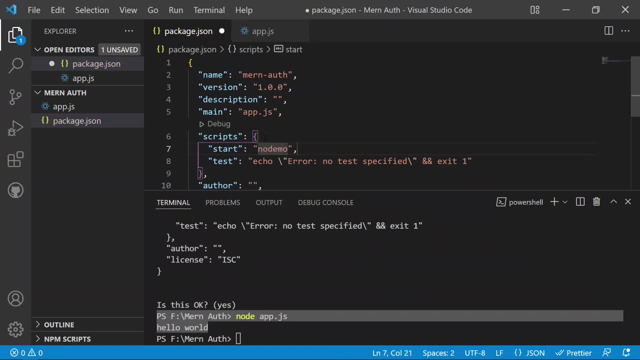 to write the node mon. so as we have discussed in the introduction video that what is the node mon? so we have to use here the node one and then we have to install the node one as well. so now i have entered the command as the node one, as the appjs, so it will automatically detect. 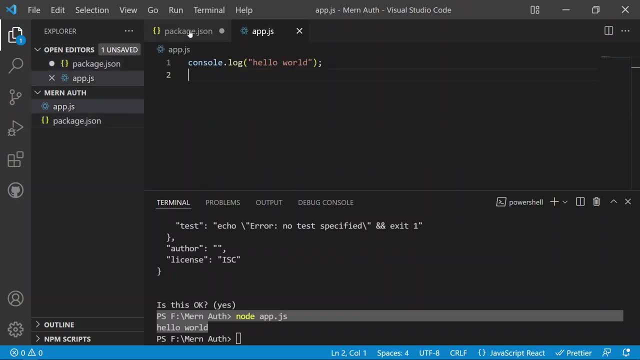 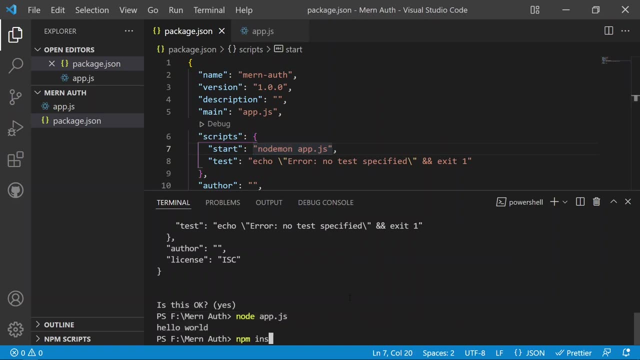 all of the file changes via the node mon in the appjs directory, in the appjs file. so we have to just save and then we have to install the node one as well. so it will be npm install as the node mon. so we have to wait now till it installs in our application. so now the node one has been installed. 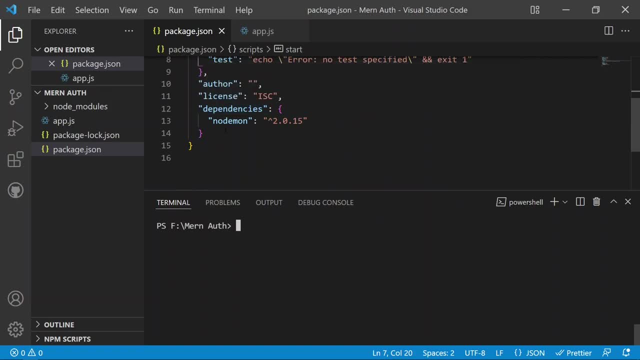 and to verify that. then you can go to the dependencies and you can check the dependency as the node one. so we have installed the node one and now we have the start command as the node one as the appjs. so now we can just run the appjs with the node one. so we have already created a. 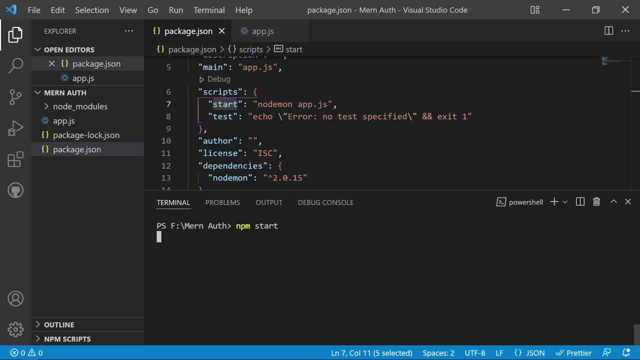 so we can just write the command as the npm start, so it will automatically start the node one here. so this is a command which will start the application from now on. now you will see, now we have the hello world and then you can see there is a newer console log, that clean exit waiting for. 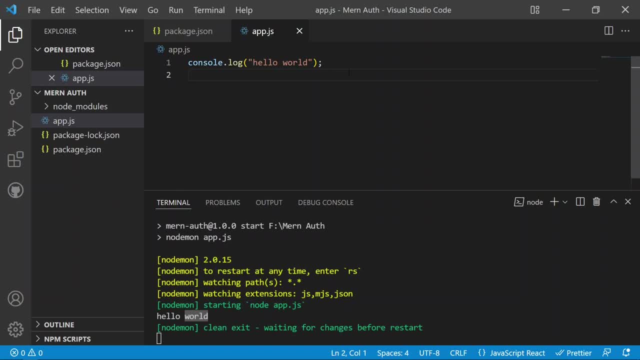 the file changes. so whenever any file changes will happen again, like like we have the hello world and then if i will add the exclamation mark after that, so then you will see the node. one will automatically detect the file changes again and the hello world is being printed with the. 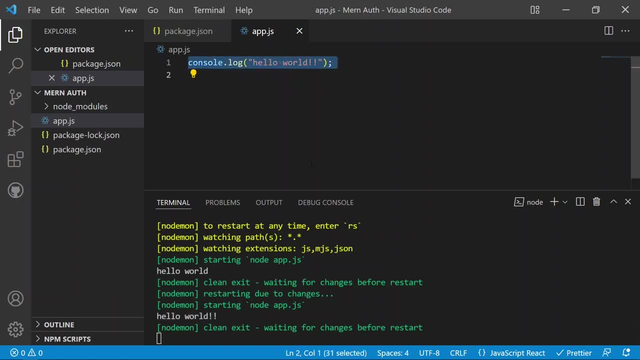 exclamation marks. so now we have completed the installation of the node one. so now the initial application is working fine and now we can just go and we can just install the expressjs in our application. so we can just stop this terminal by pressing the ctrl and the c and then the terminal. 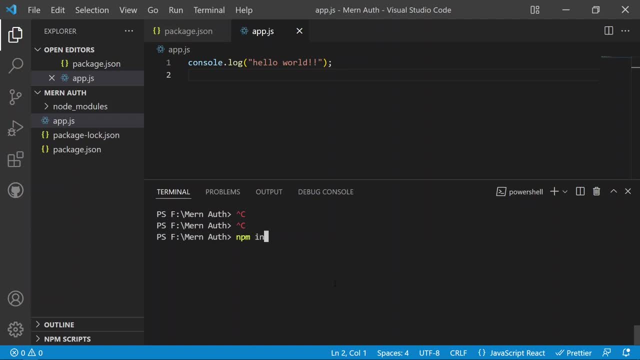 will be stopped, and then we can just install the express, so it will be npm install as the express, so the express will be installed. and we have seen about the express there. what is express? why do we need it in the introduction video as well? so we have to install the express now. you can. 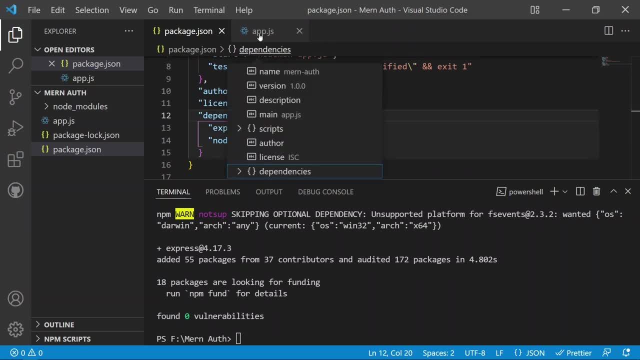 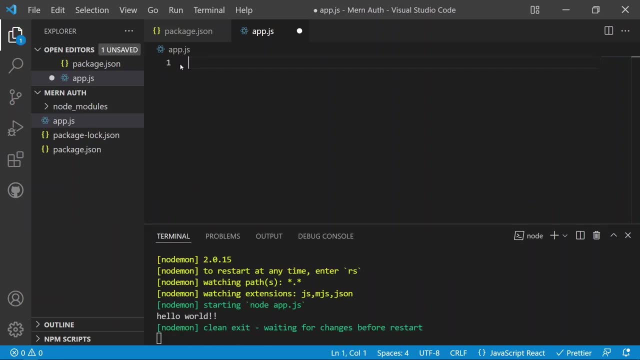 see that the express will also be installed in the dependencies, and now we can just create a basic application with the express as well. so it will be so now to create a new expressjs application. i will now remove this and i will first import the expressjs. so this will be the. 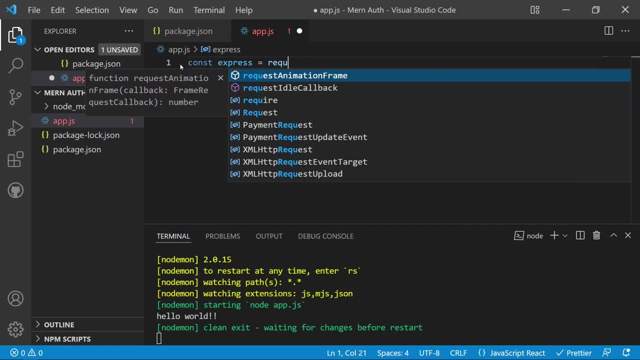 const as the express, it will be equals to require and the require is used to import some files in the nodejs. like we have installed the expressjs, so we have to get the express file also from the node modules. and now we have the express and now we have to add here the variable as the app. 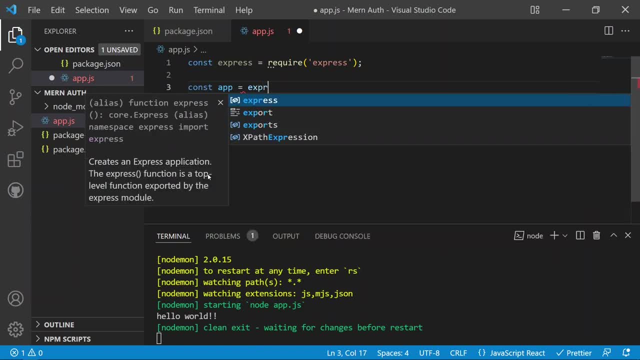 will be having the whole app functionality inside it. so app will be equals to the express and the express will give its reference to the appjs now and the and the app variable now holds all of the functionalities within the application. so now we can just write here: the app dot use. 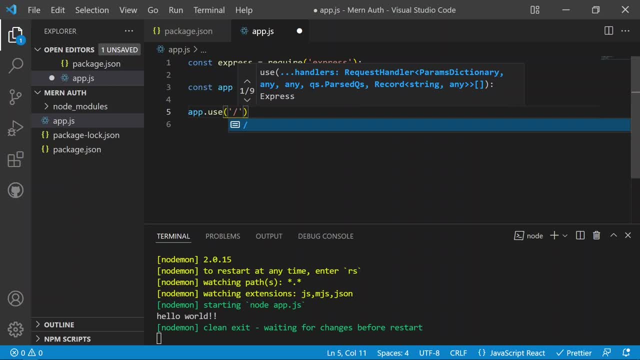 and the use is used to add a middleware for that, like middlewares for the routes, middlewares for the connections, middleware for everything. so we have here the appuse and then we have a default url, like whenever we will opening a port on the localhost or anything. 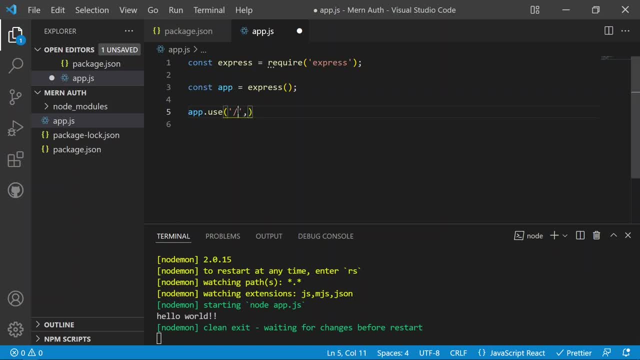 so it will be the default route, like we don't have anything after that slash. so it will be the default route and then we can add here the request response and the next as the parameters. so it will be the request response and the next, and then we can use here the response dot send. so we have to. 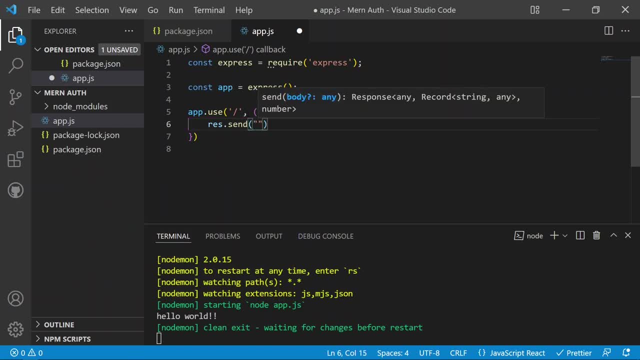 send here something on the server, so responsesend it will be equals to like we can send the hello there. so now we are sending, but now where is this server? so we have to create the server as well. so listen. so this server will be then listened to the localhost port 5000. so we have to specify: 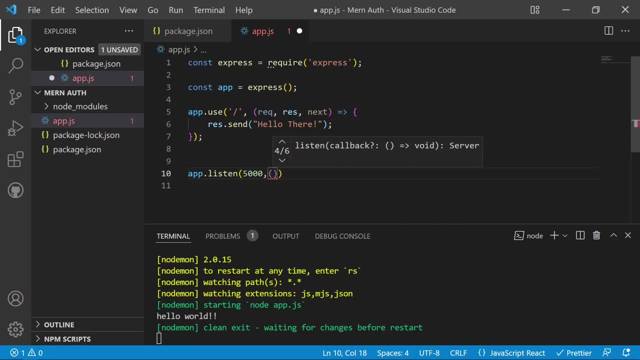 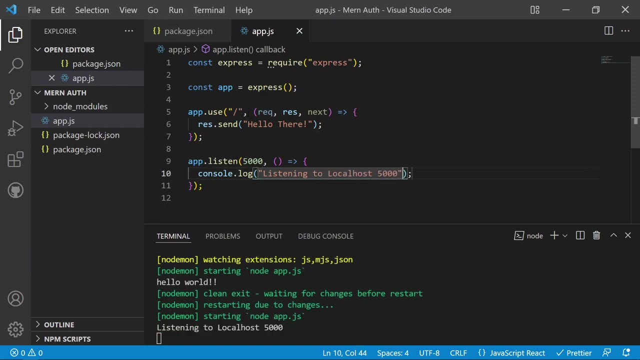 the port here, so we have the 5000 port and then we can also add a callback function here, so it will be the an arrow function inside that and then we can just add here the consolelog that listening to localhost 5000. so if i will now save, now we can see in the application if 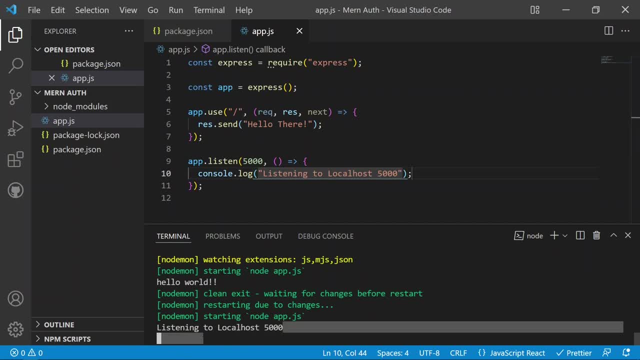 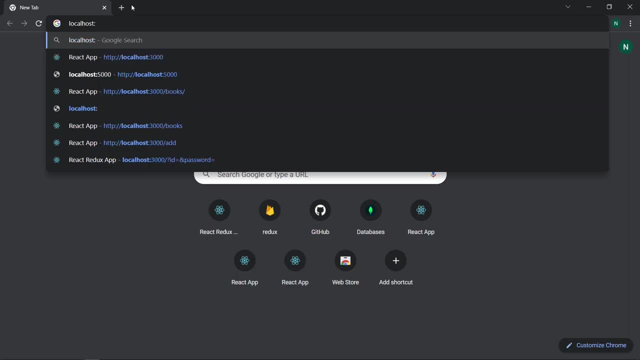 it is listening to localhost 5000. now it says it is listening. so we can just go to the chrome to see if it is sending the hello there as well. so we can just go to localhost at the port of the 5000 and to check. now you can see it is sending us the hello there on the localhost 5000. 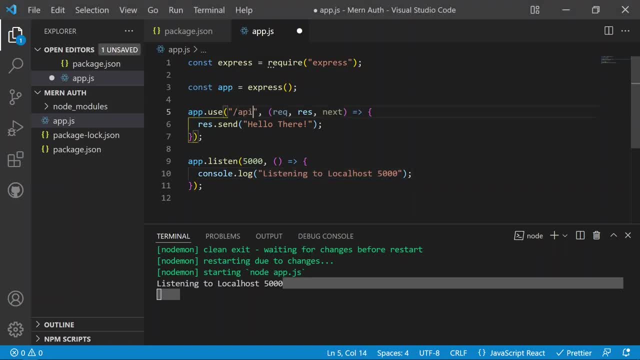 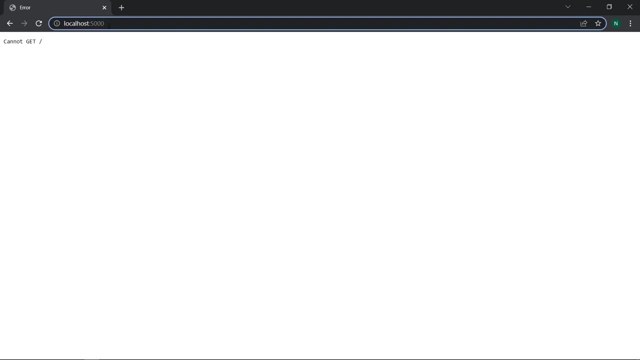 and if you will change the router as the anything like it will be the api. so we have to go to the api. so if you will just refresh it again now, you will see. it will show the cannot get. but when you will go to the slash api as we have defined, then you will see. so it will show us the hello there. 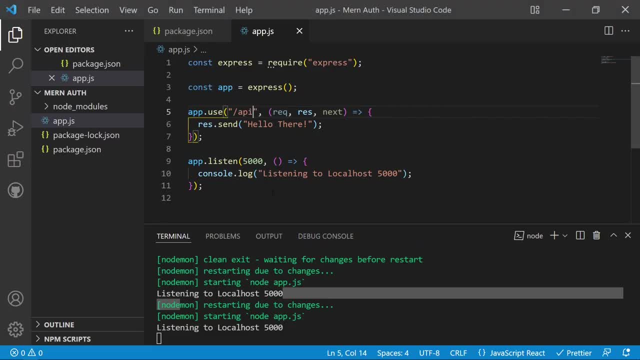 in the expressjs application. so now we have created a basic server with the expressjs as well, and now the next step is now we have to remove all of this, because it is just a basic application and we don't need to use it in our main application. so we can just remove everything. 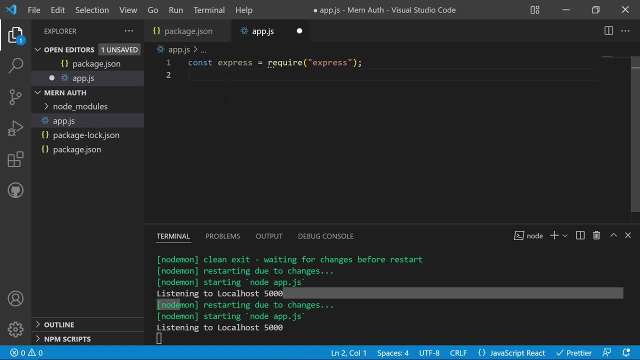 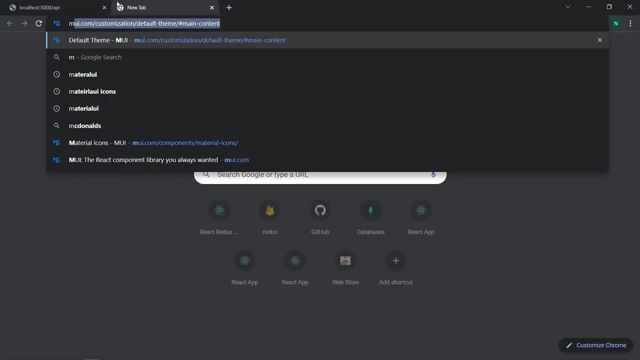 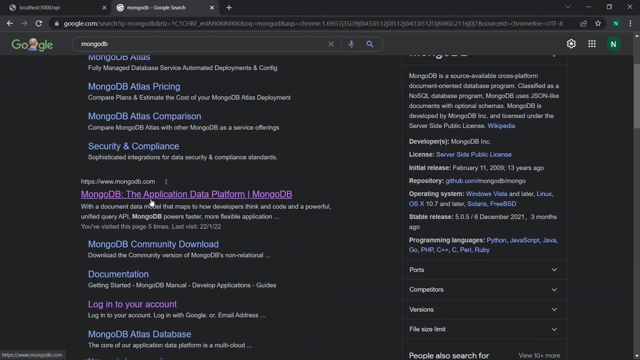 from there. so the expressjs will be there only for the import statement and now we can just go to the mongodb to install the mongodb packages. so first we need to go to the mongodb to create the database so we can go, and then you can see there will be the link of the mongodb the. 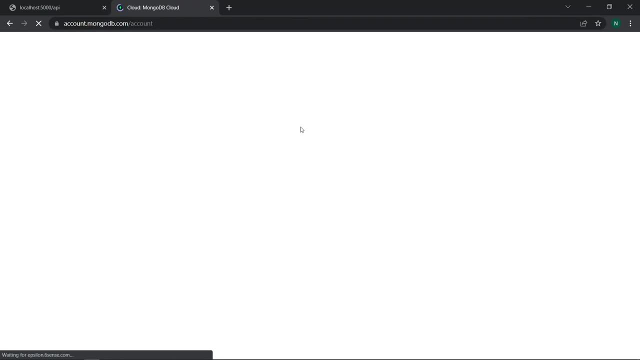 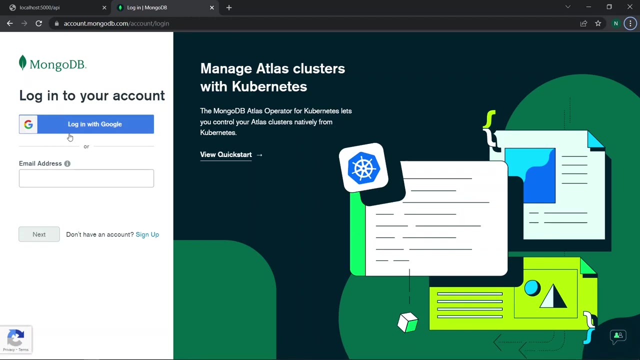 mongodb so we can just click on the sign in to sign in for the mongodb. so we have to wait. so then you will see there will be an option of the login with google. so we have to try this. or if you have the email or the password associated with the mongodb, so you can. 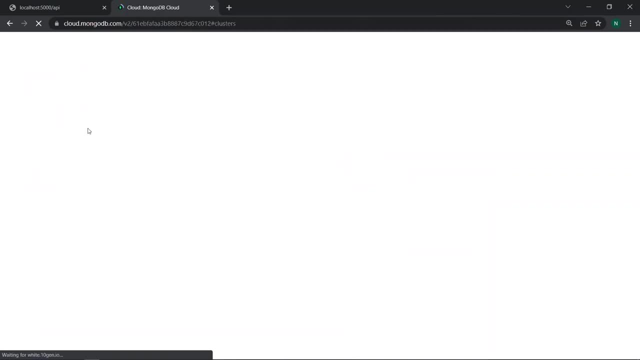 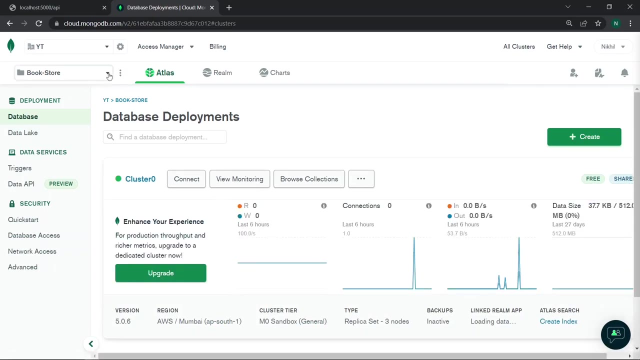 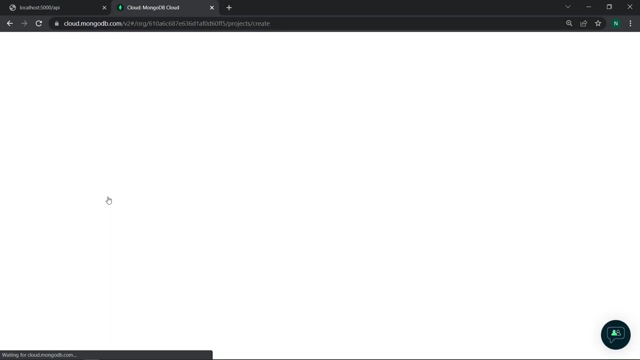 just try with the email and the password. but i will now go ahead with the google. so now you will see i have the previous databases here. but now i will start from the new project. so we have to go to the new project, so we have the new project here and then we can just create a. 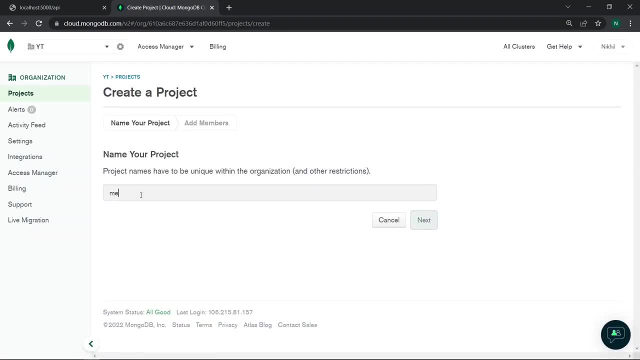 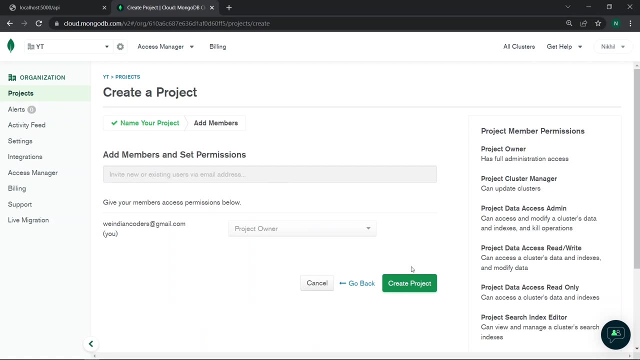 brand new project for our application. so the name of the project will be like the month auth, and then we can just create here the next, and then you will see, now we have the set permissions, but now we can just skip that and we can just click on the create project button. 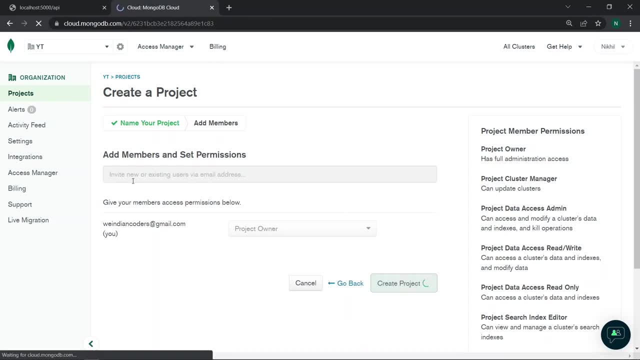 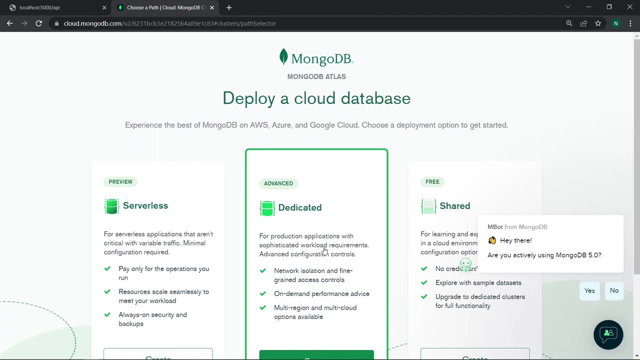 so it will create a new project for us in the mongodb. so then we can just set up our cloud database as well. so now you will see there is an option to build a database. so we have to click on that option and then you will see. now we have three options, like, if you will opt for the 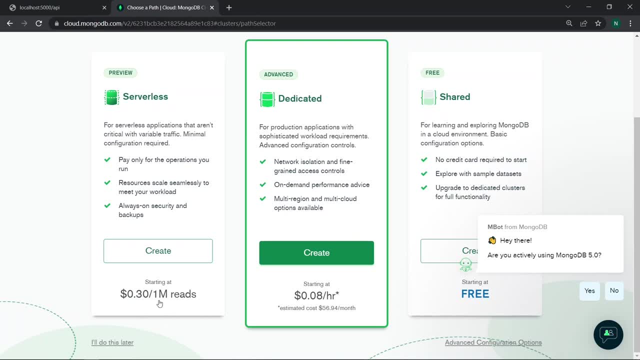 serverless, then it will cost you around 0.30 dollars per 1 million reads, and then you will see there is a dedicated as well, and then you will see there's a shared as well. but if you want to try with the free- and you can try with the free by clicking on the shared cluster so you can just 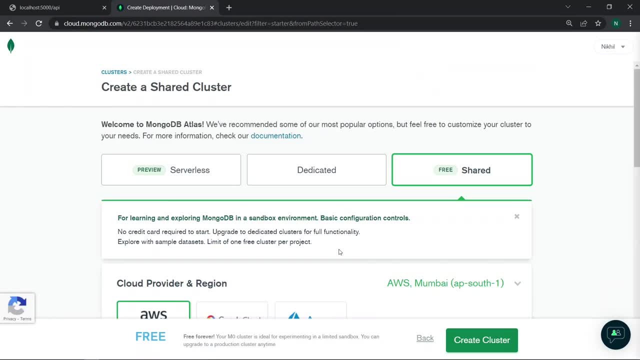 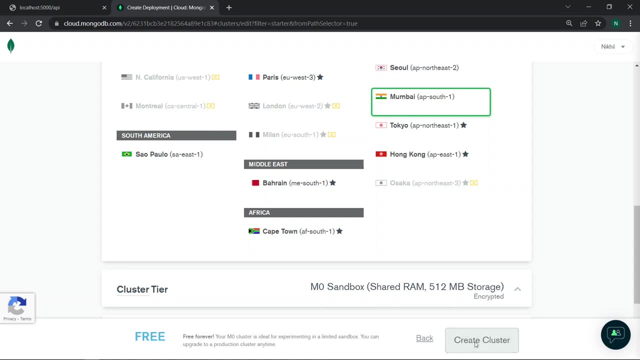 create here from the free as well. so now i will go ahead with the free as well. now you will see, now we have the default options. so i will now go with the default options again and click on the create cluster. so the new cluster is being created and then you can see. now we have some options like: 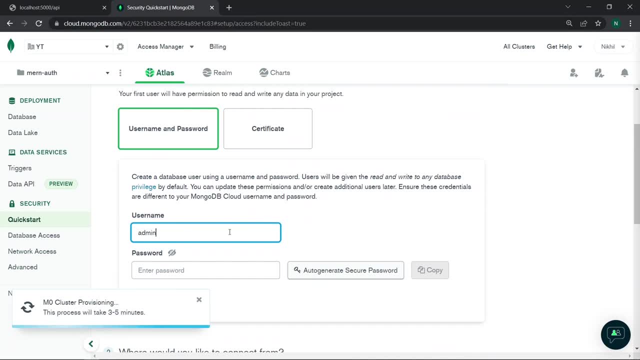 username and the password, so we can add a username as the admin and then we can just add any password here. so i will just generate the secure password from the auto generate option and i will just copy that password. so we have to save this password because there is no option, i think, to just reset. 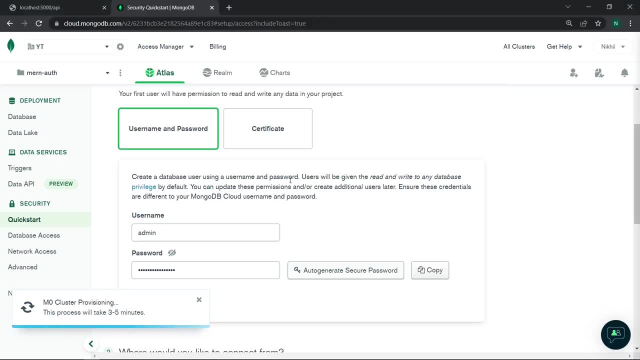 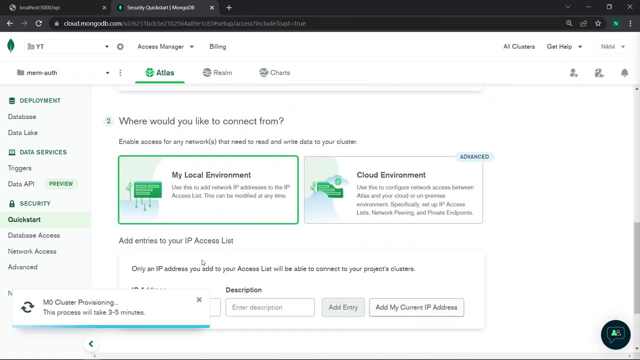 the password again. so i will now just save the password and then now we can just create a new user and then now you will see if the password is now working and that should be the password now. now we have some environments like where we want to connect, so i will add here the ip addresses. 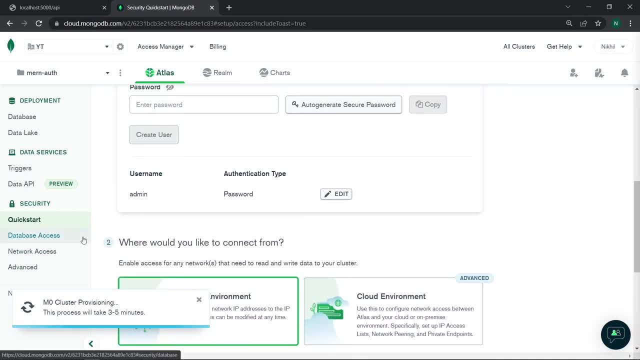 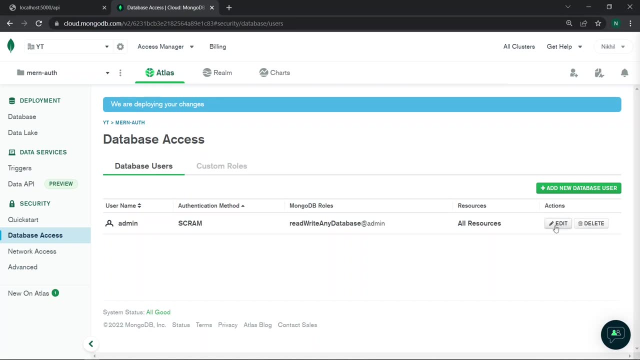 but now we can just skip that, because we need to access from everywhere. so we can just go to the database access. now we now, you can see, now we have the admin user and then you can just edit the options as well, and then we have the network access and you can just add here the ip address. 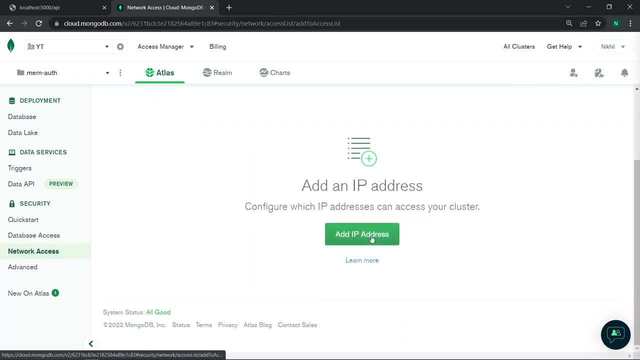 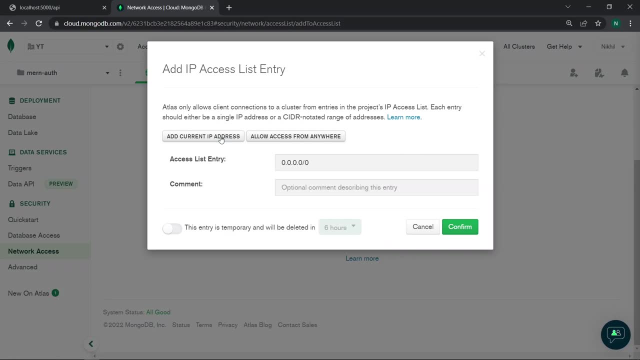 from below option so you can just click on the add ip address and you can just add as the allow access from anywhere. and if you want from only the specific ip address, so you can just add your current ip address as well. so if you will add from the current ip address, so it will be only. 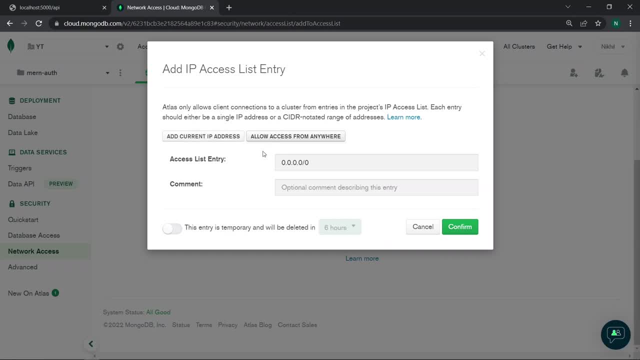 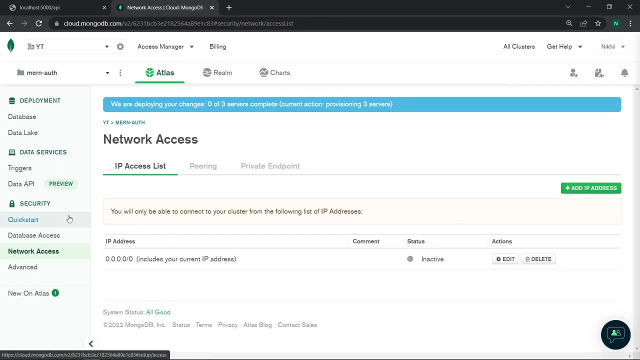 accessible from your current ip address only. but now for now, i will now click on the allow access from anywhere and i will now confirm so. then you will see now the changes will be reflected within few moments and then, once you will go to the database. now you can see, we have the database. 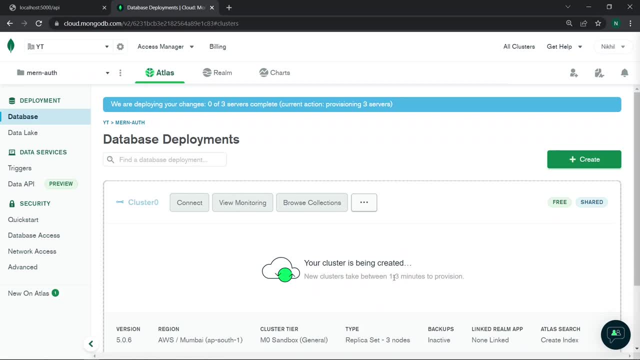 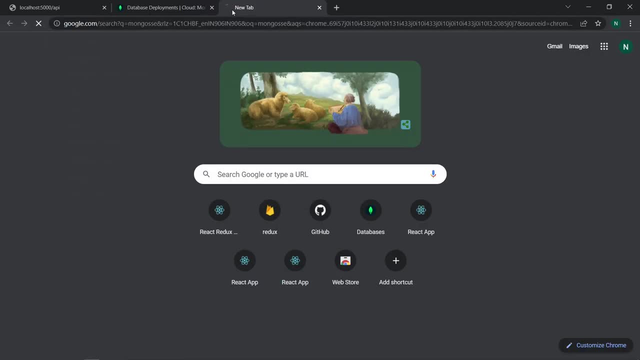 deployments. and now it will be deployed within zero to three minutes. now you can see one to three minutes it will be installed. until then we can just go and we can just install the mongoose. so we have seen about the mongoose in the introduction video, that what is the mongoose? 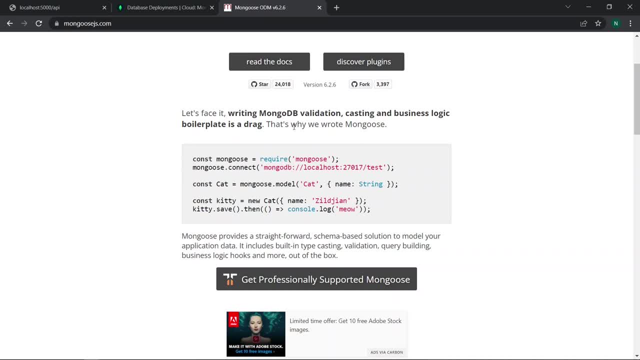 and why do we need it? because it provides us as access to just interact with the mongo db. so it is very simple and it is very easy to use to interact with the mongo db database. so we have to just install the mongoose, so we have to go to the terminal again and then we have to run the command. 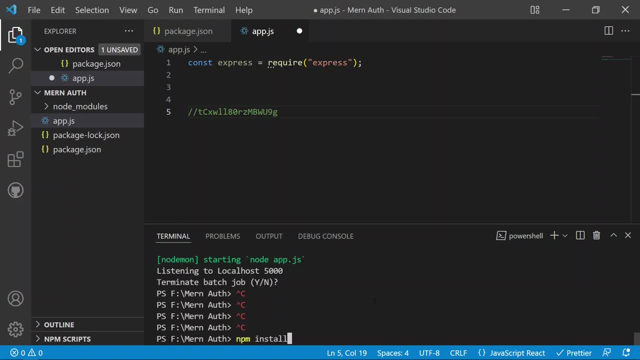 as the npm install as the mongoose. so the mongoose will be then installed in our application and then we can just connect our application with the mongoose and the mongo db. so they all will be connected. so the mongoose package is now installed and we can see the mongoose in the dependency section. 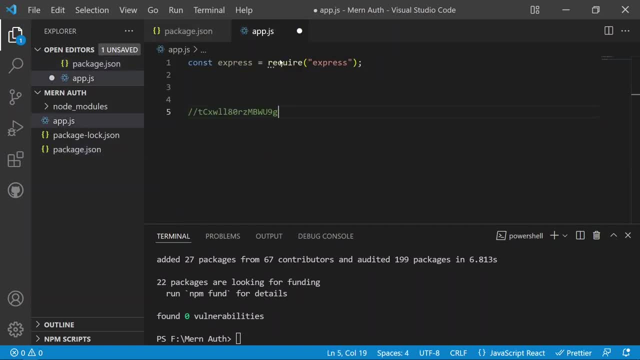 as well. now you can see, now we have the express mongoose and the nodemon, and then you will see now if now the database is also deployed on the cloud. so now the first step would be connecting our application to the mongoose, and then we can just connect the mongoose and the mongo db. 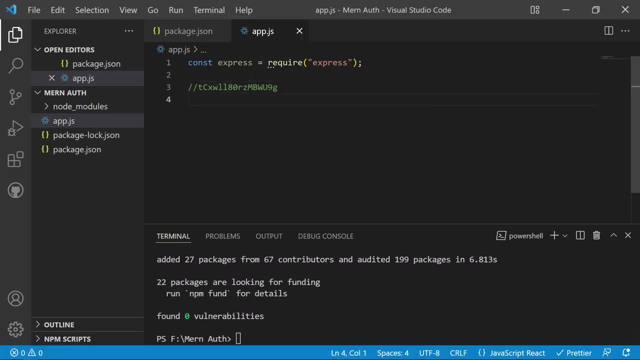 to the database. so now we can just connect our application with the mongo db database and for that we need to import the mongoose here. so const as the mongoose will be equals to the require again as the mongoose. and then we need to provide the app as well, so const app will be equals to the. 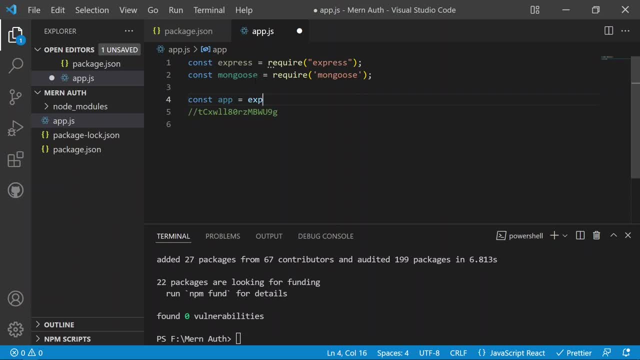 express again and we have to give all of the express functionality to the app. so it will be the const app equals to the express. and then we can just use the mongoose so to connect to the database. so it will be the mongoose dot connect. so the connect function is used to connect to the database. so first it needs a uri. 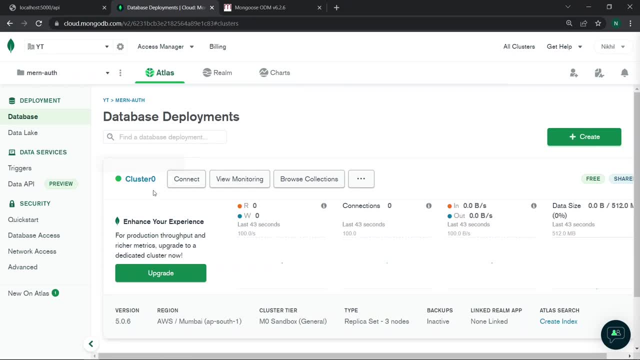 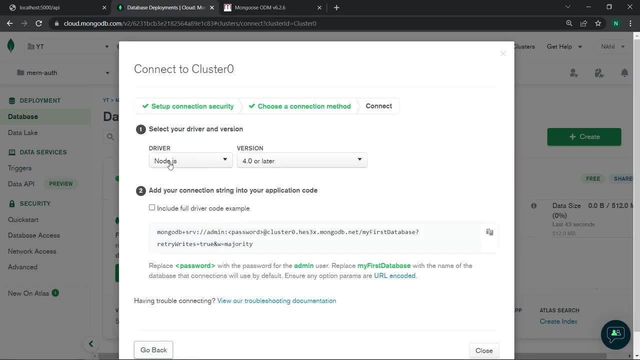 which is the string, so we can just go to the database cloud as well, and then we can just click on the connect. and then we have to click on the connect, your application, and then you will see, now we have the node js selected from there and then we can just copy here this uri, so this: 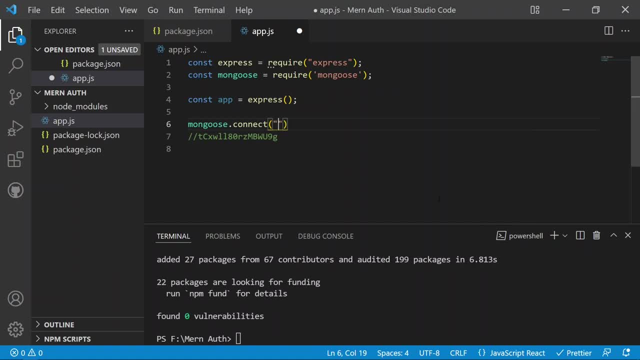 is a uri which we need to pass there, so it will be in the quotes. so now you will see it is now passed and then we can use here the then statement after this, because it is a promise. if you will hover over it, now you can see this type of a promise, so we can just add: 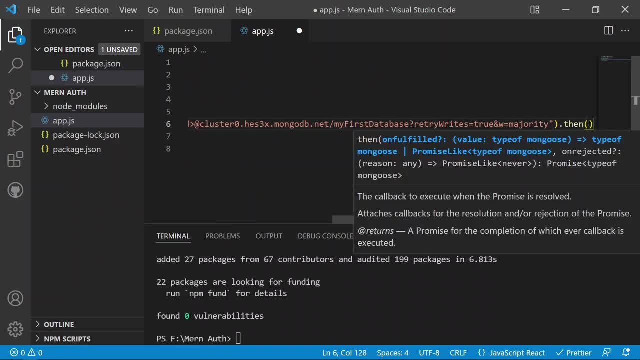 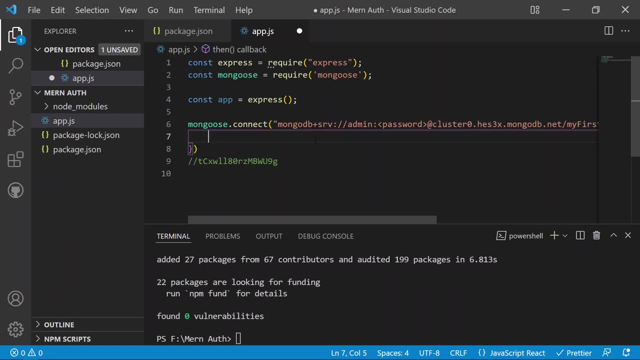 here the then statement as well. so whenever the connection will be succeeded, so we can just create here the then and then we can just add some functionality here, like then. so once the application will be connected to a database, then we have to open the server like app dot listen. 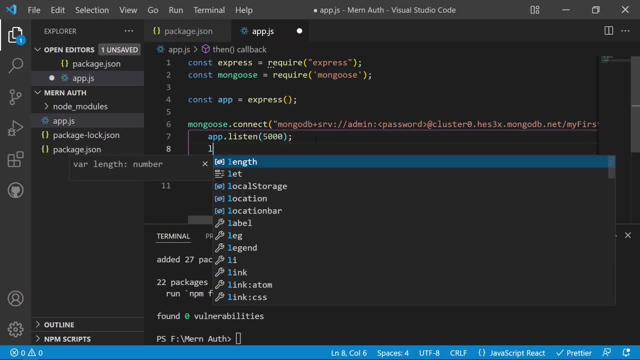 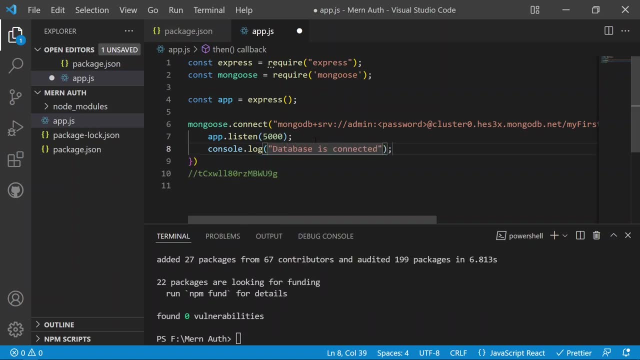 on the port of the 5000, and then we can just add here the console log statement as well. like, the database is connected and i am listening to localhost port 5000. so this is the console log which i need to enter here, and then you will see. 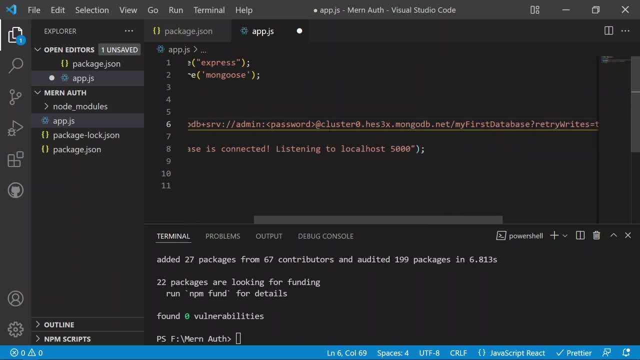 now in the connect function. now we have the mongodb and then we have the password. so this is not the password which we need to use. so we have to replace this password from here and then we need to write the password which we have copied from there. we have to write this password after the admin slash colon, and then there is a new thing. 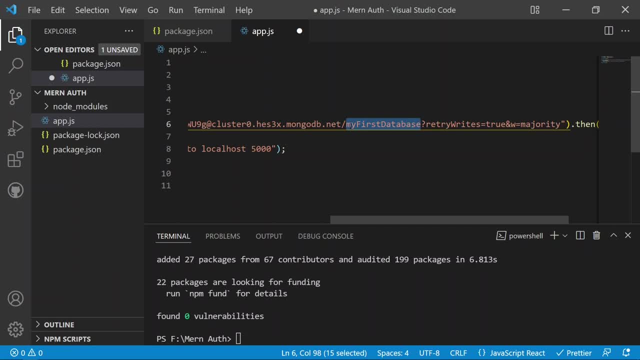 here, which is the my first database. so this is the default database which will be created by the mongodb. so we can just change this if we want to change our database name, like i will add as the murn dash auth. so this will be my database name, or i will now add this: 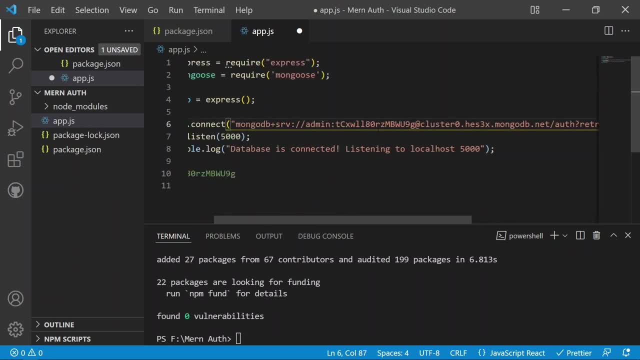 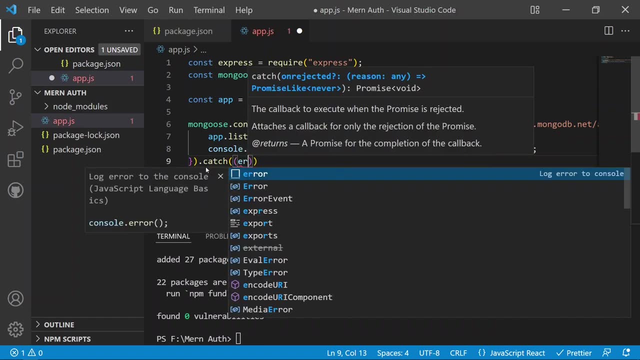 to the auth. so this will be my database name as the auth and then you will see we have the connection and then we can also provide the catch statement. so if there would be any error, so we can just console dot log the error which we will receive from the parameter and 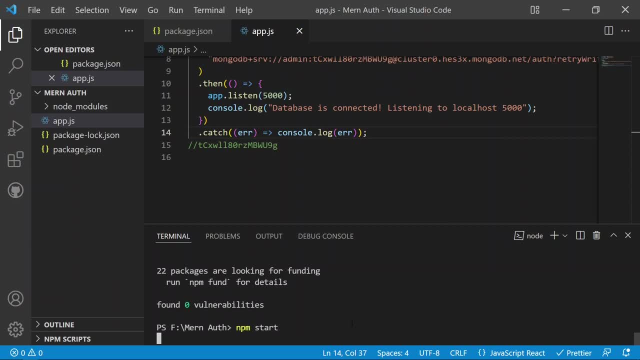 if i will now save and if i will now just start the server again from the npm start. so then now you will see the database is connected and the connection is successfully created and it is listening to the localhost 5000. so now everything is working fine. and now 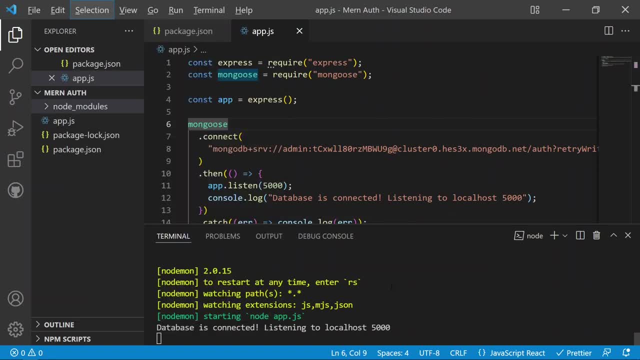 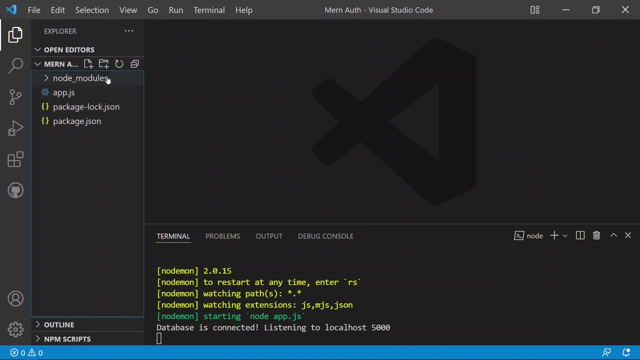 we need to build the functionality of our application. so now the application is connected to the database and now we can build the full functionality of our application. so first we need to build the folder structure. so first i will create a folder here and it will be the model, and the model will contain a user model inside that. so we can just create a. 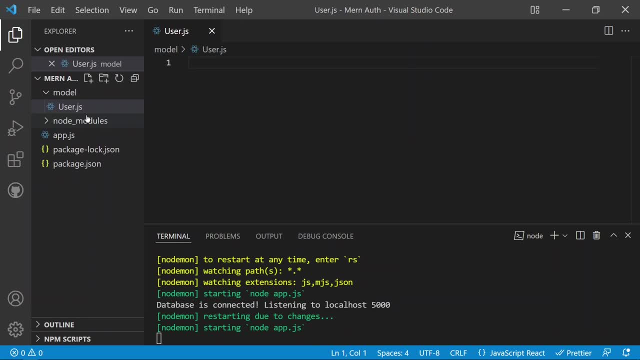 file as a user- dot js, so it will be the user model. and then we can just create another folder, so it will be the routes, which will contain all of the routes of the user. so we can just create a new file as a user, dash routes, dot js, so this file will contain all. 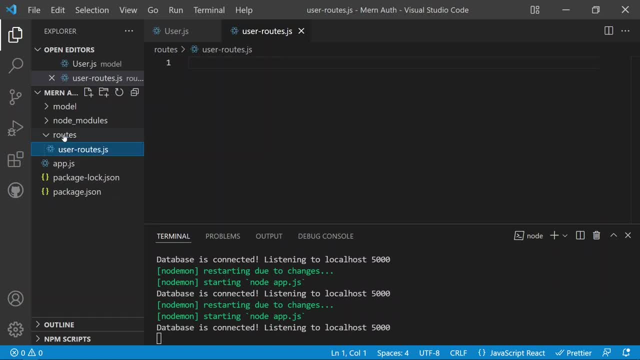 of the routes from the express js, and then we can build and then we can create another folder here as the controllers. so it will the controllers, so the controller folders now we have created, and this folder will handle a new file inside there, so it will be the. 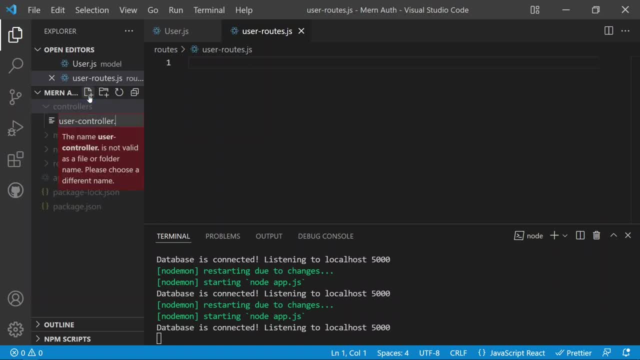 user dash controller dot js. so this file will handle all of the controlling operations of the routes. so once the user will go to the route and then we need to write the controller functions here. so these are the functions which will control the routing operations. so now we have created the folder structure, so now we can just go to the user and then. 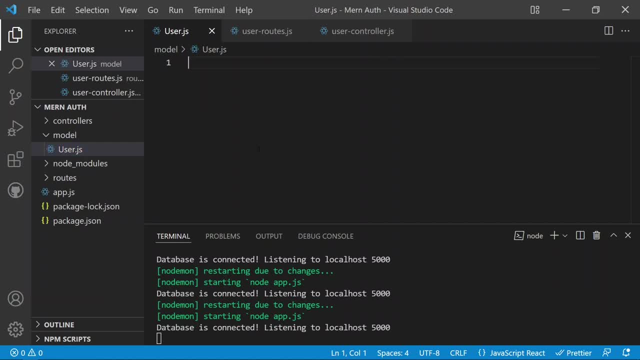 can just create here the model for the user. so the model of the user will contain some things like: it will be: the first we need to import the mongoose to create the model. it will be: the mongoose will be equals to the require and it will be the like the mongoose, and then we can just use the schema. 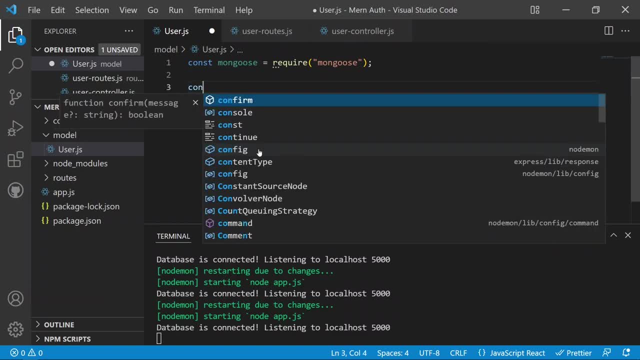 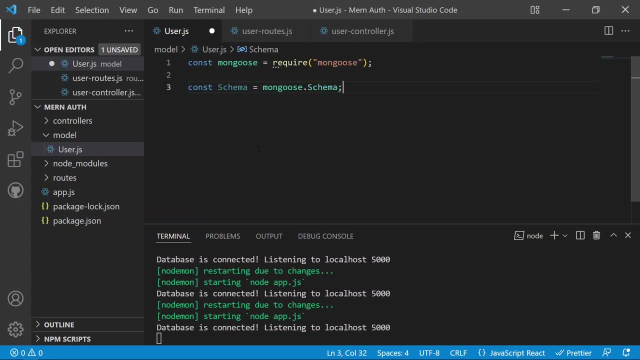 so we need to build the schema of the user first. so it will be the cons and the schema equals to the mongoose dot schema. so we are now referring the schema to the mongoose dot schema and then we can just create here the new schema by having the new instance of the schema class. so we can 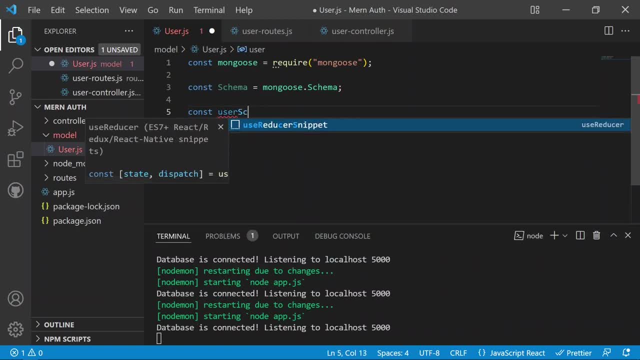 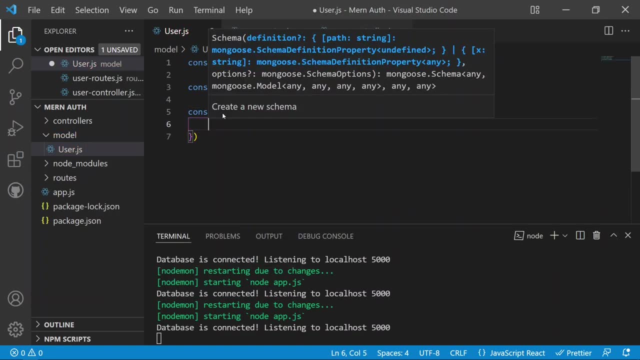 just create the schema as the cons user schema and it will be equals to the new schema of the mongodb database. now we have the new schema and then we can write here the objects inside that the first property of this schema will contain the name and it will be of the type of the string. 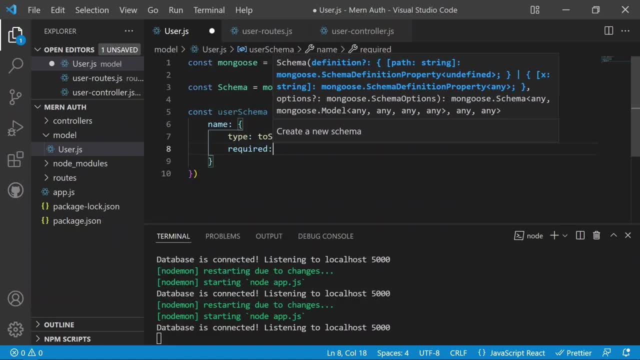 and then it will be the required field in our object, so the required it will be the true. so now we have the name and the field name is equals to the string. so it is now showing you the true string, but it is not the true string. so the name is the string and then the required field. 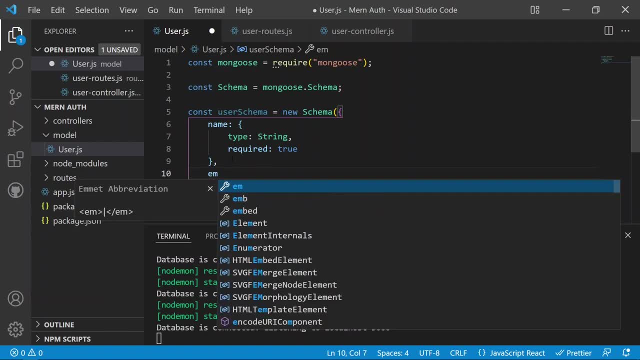 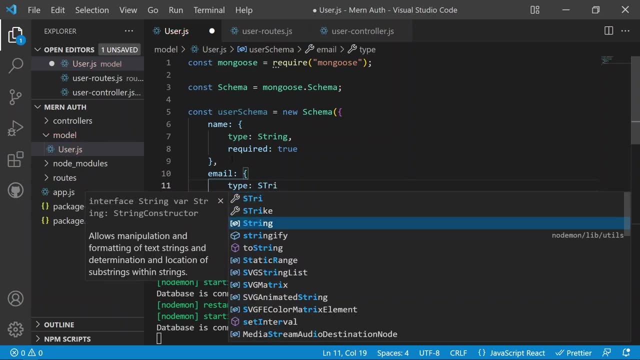 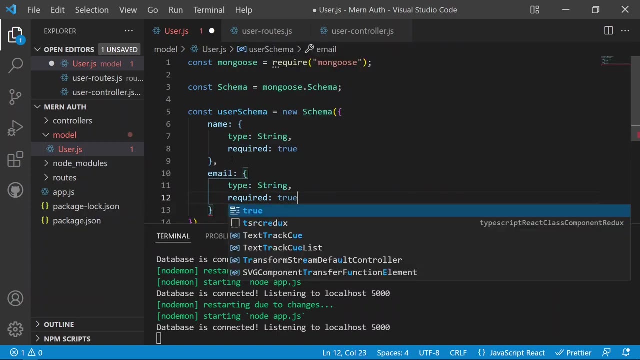 is the true, and then we need to write here the email of the user, through the email, and it will be of the type of the string again and it will also be the required. so the required prop will also be the true here. and then we need to write another property as the unique, because every user will have a unique email id. 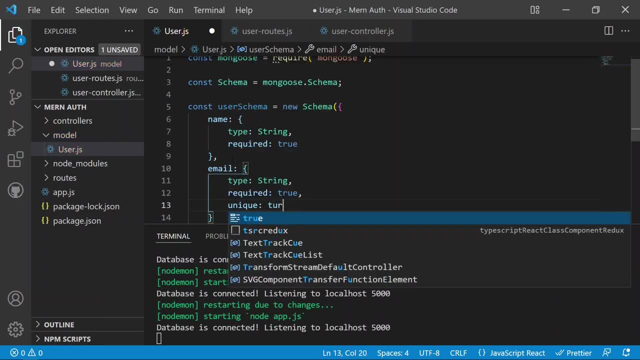 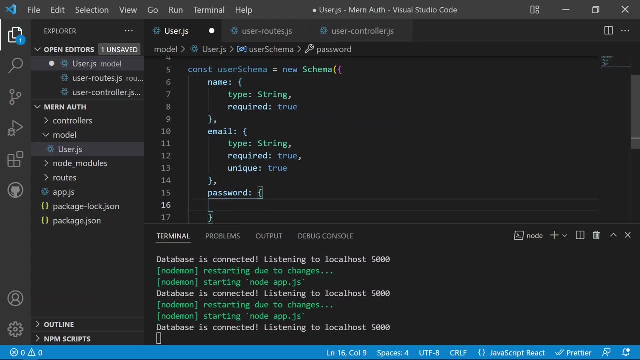 so we will add the unique prop as a true and then we need to add the password field. so the password field will contain the type again as the password, so to the type as the string, and then we can just add the required prop again. so the password is the required field and it is. 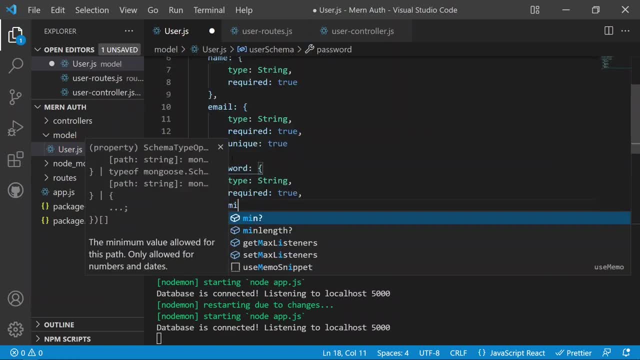 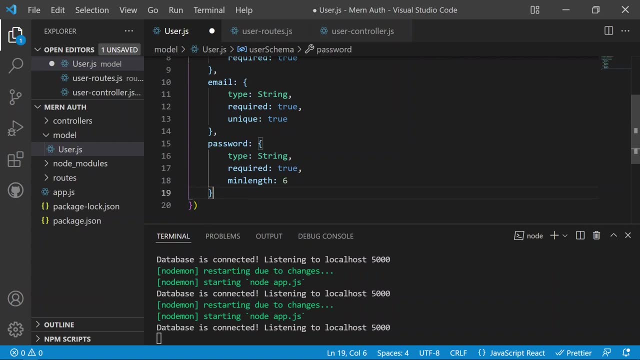 equals to the true. and then we can also add a one more field as the min length, so the password. so the minimum length of the password will be close to the like. we can add here the six for the minimum length of the password. so this is our schema of the user, which we have created now. so it will 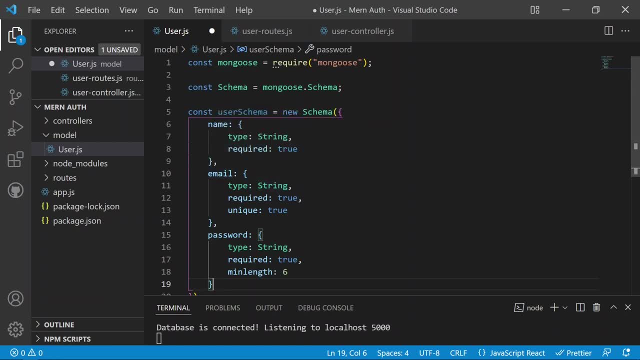 have a name, it will have an email which is of the type string and it is also the unique email. so if the email would be repeated again, so the mongoose will throw us an error and then you will see we have a password end also. so now we can just export the schema as the module. 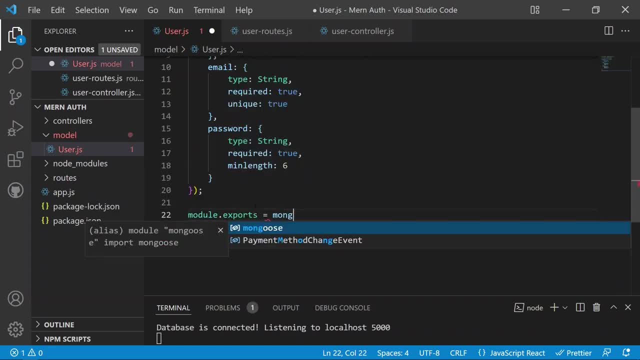 dot exports and it will be equals to the mongoose which we have imported dot model. so the model creates a schema and then it will export the schema. so we need to provide a name as the string. so it will the user and the you will be the capital and then the schema. so schema we have. 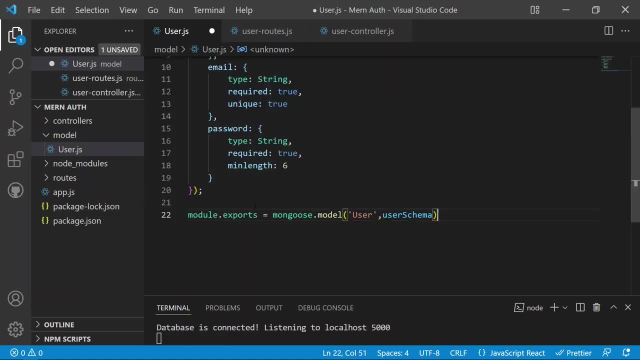 already created as a user schema. so the variable, the user schema, will be there. so now this will export the mongoosemodel as the user and in the mongoose it will be stored as the users, because there is a default naming convention in the mongoosemodel db database, like if you will add here the user, so it will be stored as users, because the first 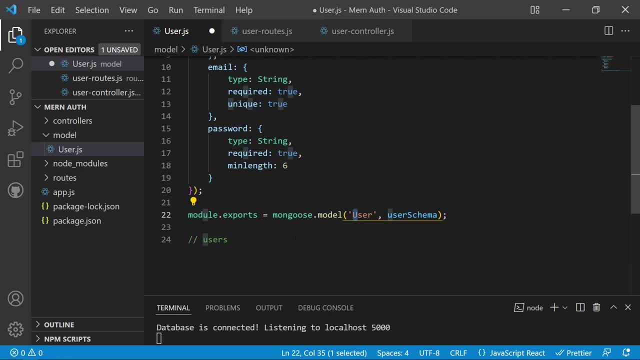 letter will also be the small case letter and then it will add here the plural form inside the mongo db. so all of the models name will be on the plural form in the mongo db collections. and now the schema is created and now we can just go to the user routes to create some routes. so to create some. 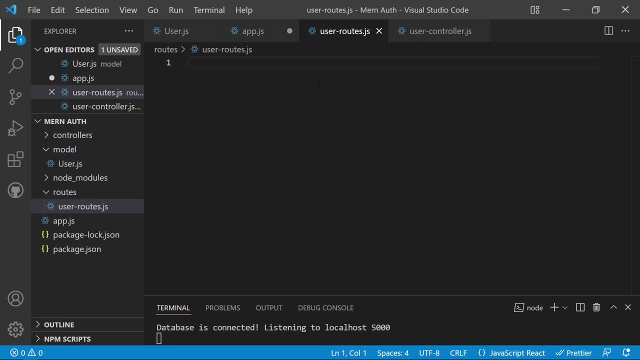 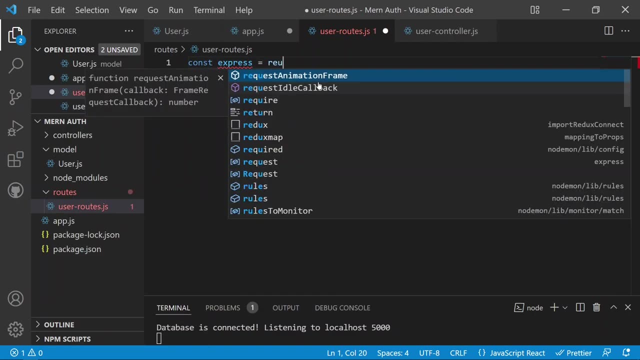 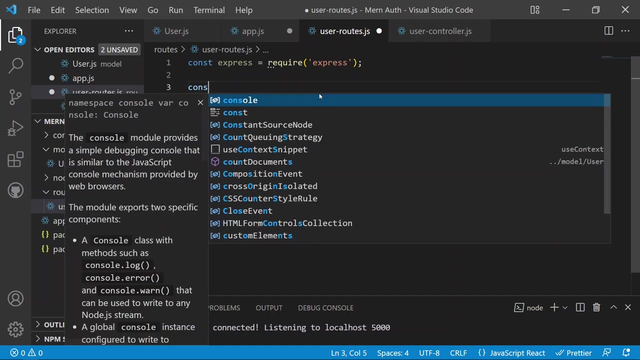 routes for the user schema to interact with the database. so we can just create the routes. so first we need to do as we need to import the express from the require as the express. again, after importing the express now we can use the router. so we have to declare a variable as the. 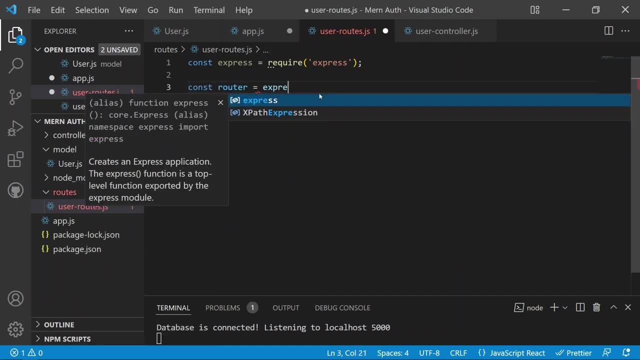 router and it will be equals to the express. we have imported the express, so the express has a function of the router. so now we can use the router and now this variable holds its reference inside that. so now we can just create some requests like: first, it will the router dot get. 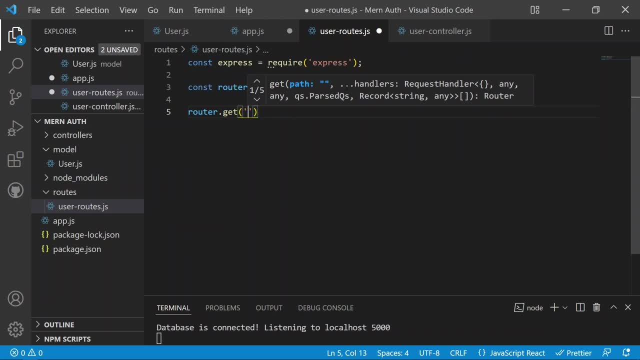 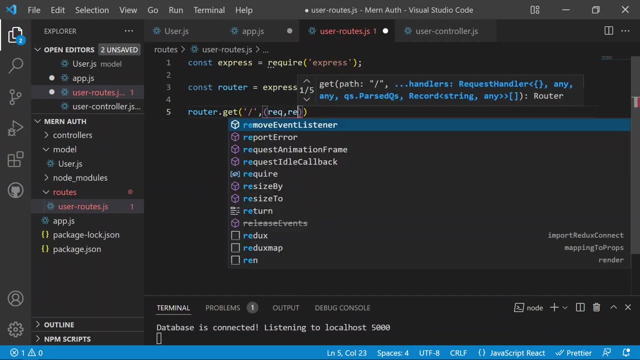 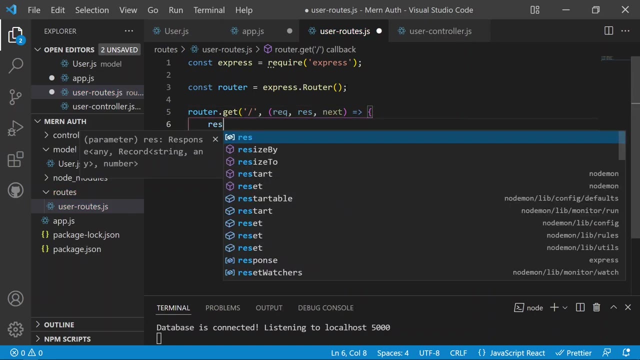 so we can just create a get request for the http and then the path will be like the. there will be only the default path which we have, and then we can just add a function like the request response and the next, as we did in the basic application from the express, and then we can just like just send something like response dot. 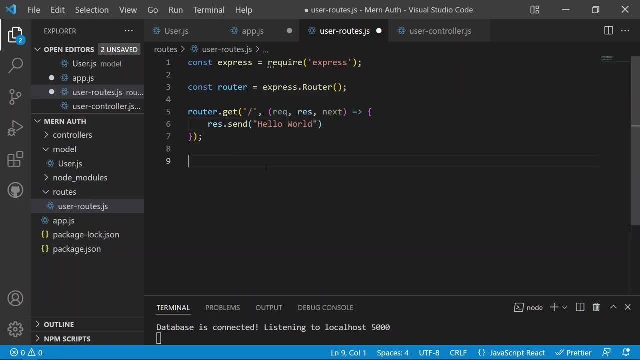 send, and it will be equals to like the hello world. now we need to export the router as well, so it will. the module dot exports will be equals to the router. so right now we only have the one route, but later we will have more routes there and then 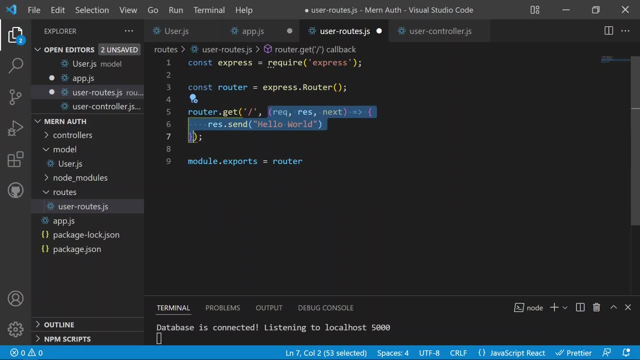 the all of the functions like this, like we have defined the callback function, so all of this function will be then in the controller's file. but now to just test the application if it is running or not. so we can just define here the router dot get and it is just a simple hello world. 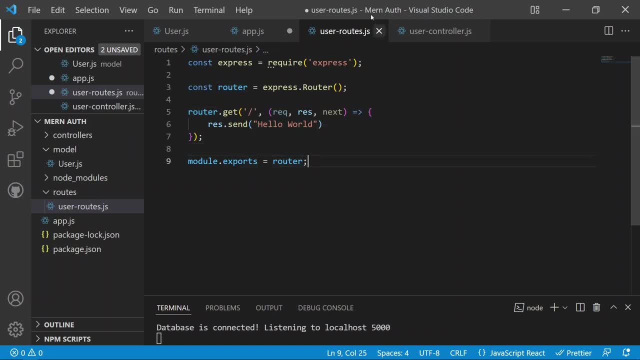 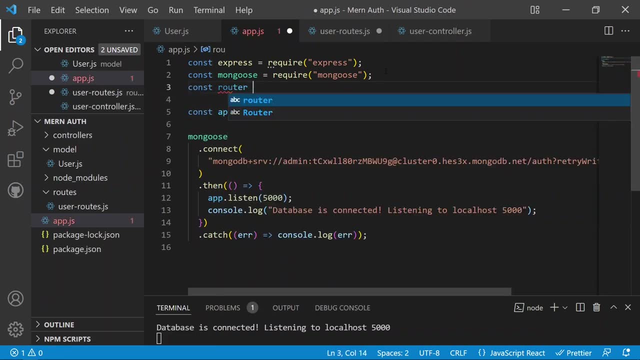 and then we are now exporting the router as a standalone module and then we can just go to the appjs to import the router. but with the const router will be equals to the. we can import the router here from the require again. so the require and it will be in the, i think will be in the. 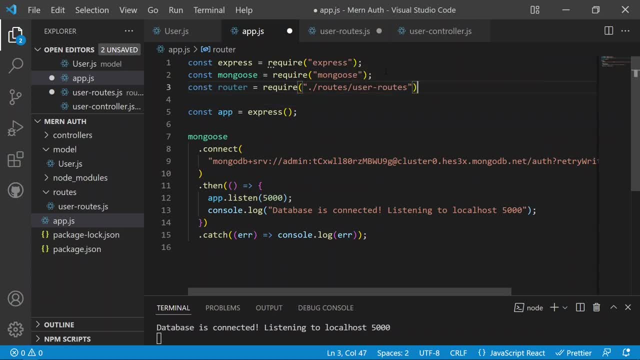 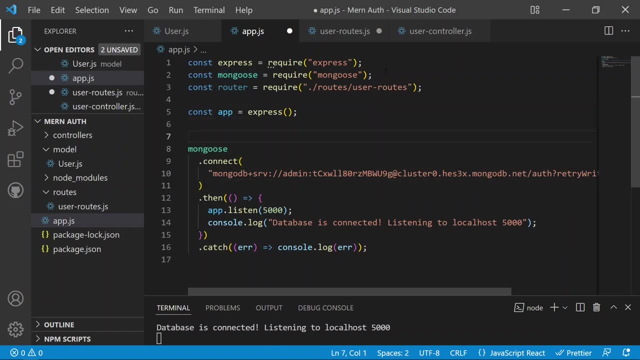 routes dash. we have the user routes file. so now user routes file is being imported and now we can just create here the middleware for us. so we need to create the middleware as the app dot use. so by default url will be like the backend or like the api, so we can add here the api and then we can. 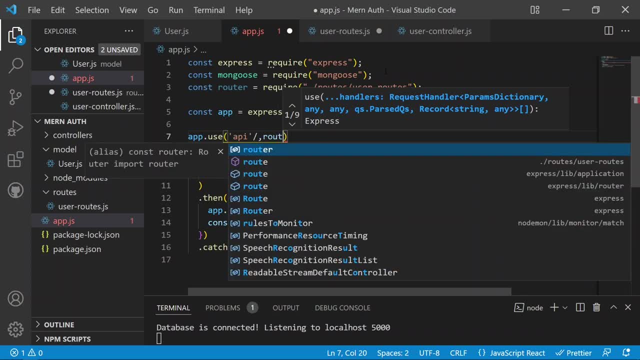 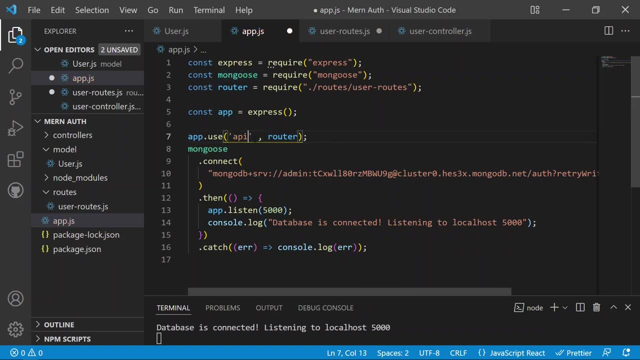 just add here the router, so it will the router. so now the router will handle all of the operations after the api there. so it will be there as the. so we have to add here the api as the slash api and then this will handle all of the. 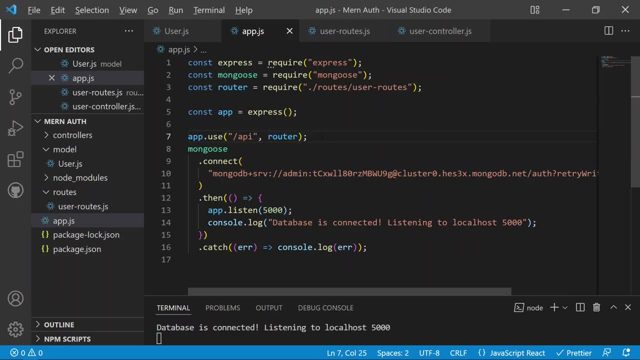 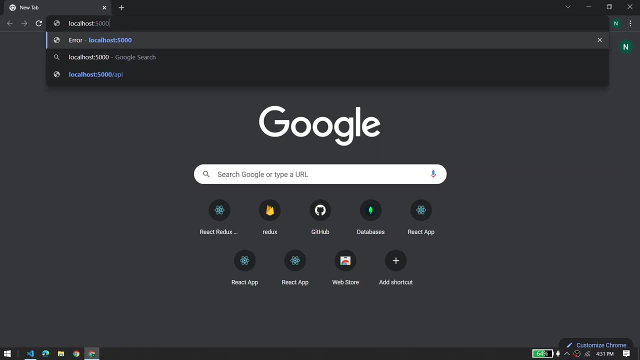 routing operations after the api. if i will now save, so now, if i will now just go to the chrome to test again, so now we can test the application by going to the local host, set the rate 5000, so then you will see. now it is showing us it cannot get, but once we will go to the api again. 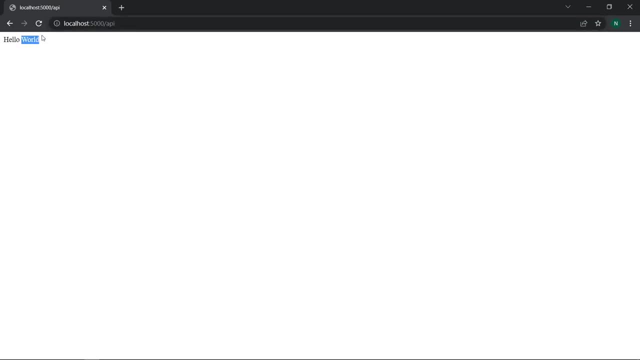 so it will show us the hello world there. so now is sending us the hello world. but now for all of the operations like this: like we cannot go to the chrome again and again, so we need to install something, like we need to install the postman, which is like a api testing tool so we can just install the postman from there. so now you will. 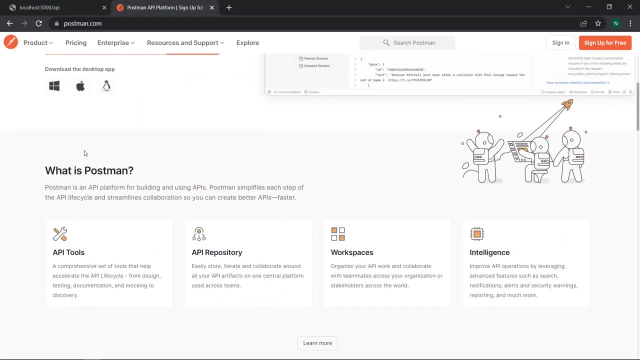 see, now we have the postman and then we can just download there the postman from this link. so you, so i am using the windows operating system to use the and to create the rest api. so if you are in the linux or in the macbook, so you can just try out with their, with your supported operating. 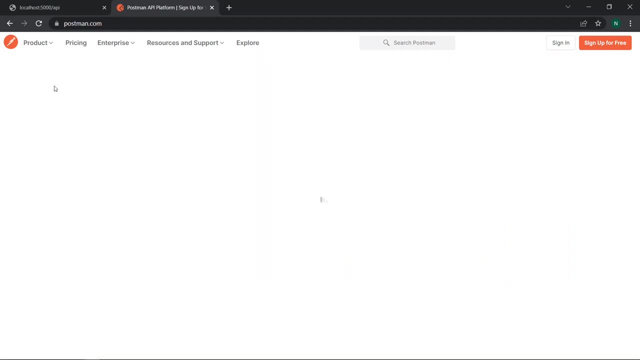 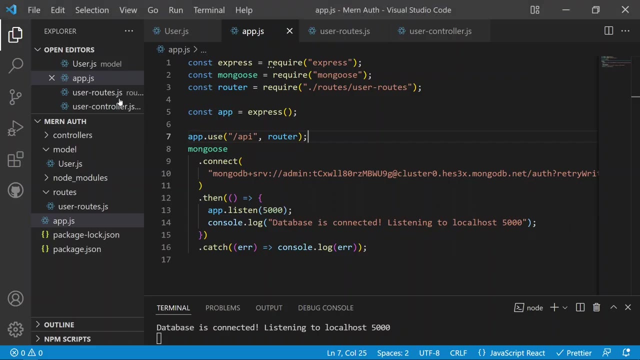 system. but i am on the windows, so i will try out with the windows. so i've already installed it in my machine so i don't need to install it again. so you can just install and you can just open the postman for the routes. so i will now go to the windows, select the postman to test. 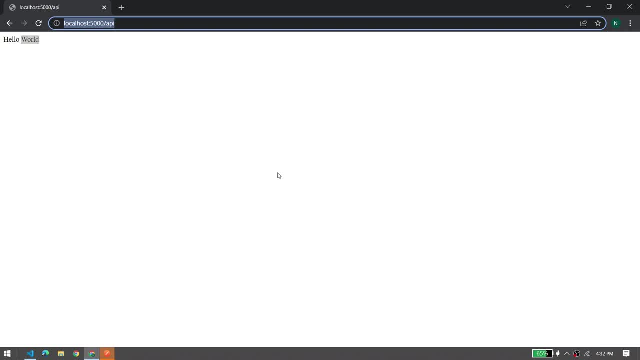 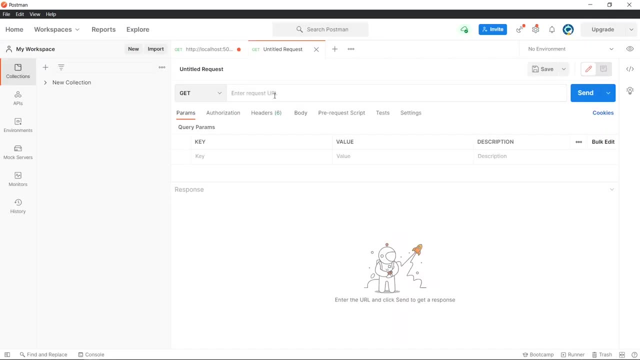 the route. so now you will see this is the screen of the postman, and then we can just enter here the url as well, like it will be the http slash localhost into the port of the 5000 and slash api. so once i will click on. 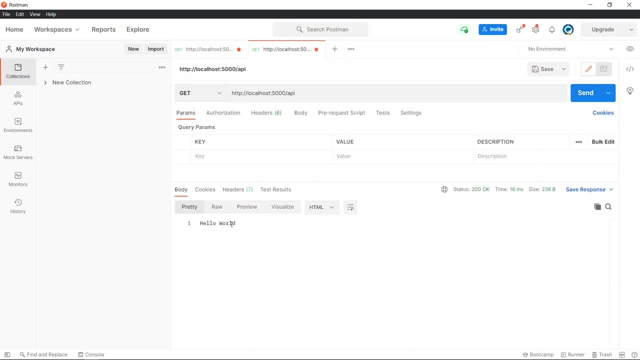 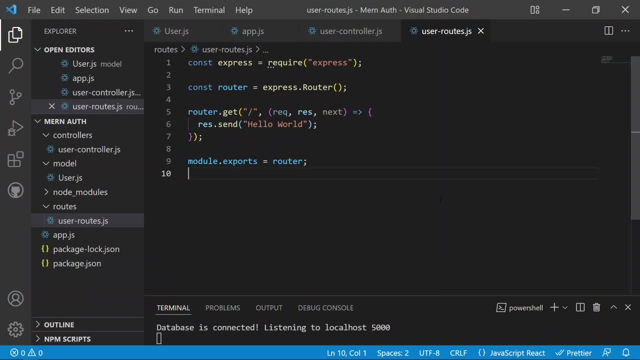 this send request and you can see this is the get message also. so then you will see it will show us the hello world. so now the basic application has been created and now we can start building the real routes for the http request. so i will now delete this route from here. so we have to create. 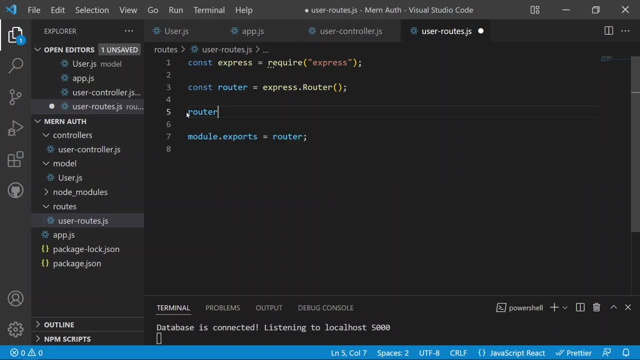 the new route for the signup functionality. so first there will be the signup functionality, so it will be the router dot post, so it will be the post request, and then we can just add here the slash and it will the signup, so it will the signup and we can add a controller function after. 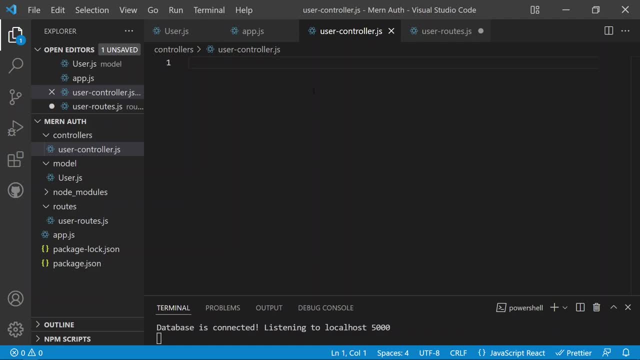 that. so we can just go to the controller and then we can just define here the controller for the signup function. so first it will be const as the user and it will be cost to the require. so first we need to require the user model which we have created, so it is in the model, and then it 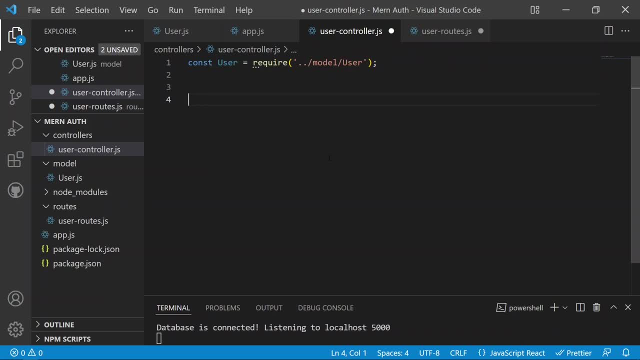 will in the user, so we need to import this user. now the user is imported and now we can just create a first function which is a signup. so it will the cons signup and it will be equals to a async function and it is a asynchronous task. so we have to define. 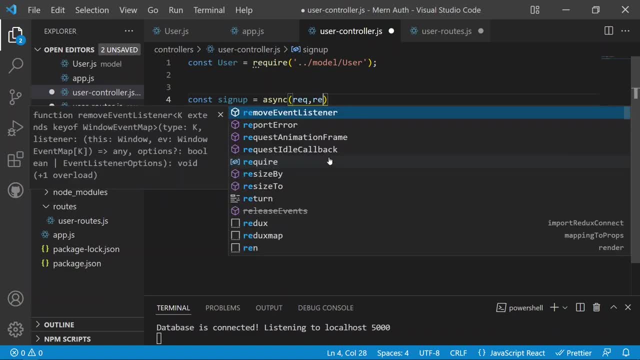 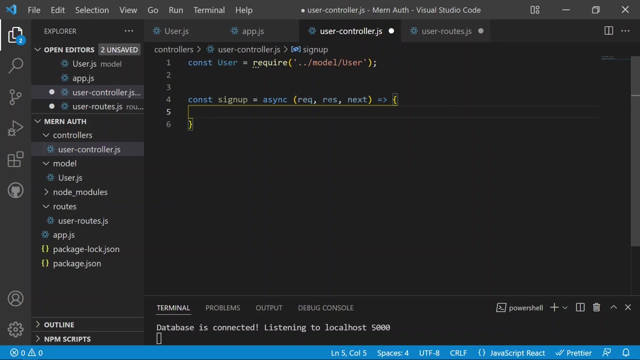 it as a async function, so first it will contain the request, then it will contain a response and then the next. the request is like, which we will get from the client and the response which we will send from our server, and the next is used to just move on to the next middleware after the. 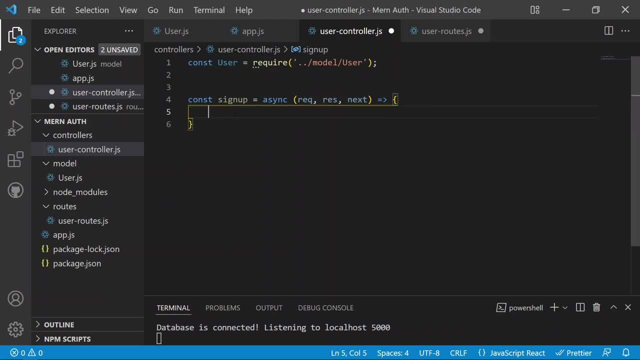 certain task. so now we have created the signup function and now we need to create the user. so to create a new user, now we need to create here some fields like: first it will contain the cons as the user, so it will be the new instance of this user, and then we can just add here the object. so first, now you can see, now we 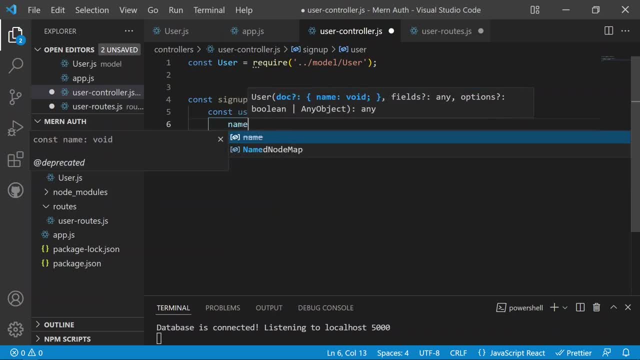 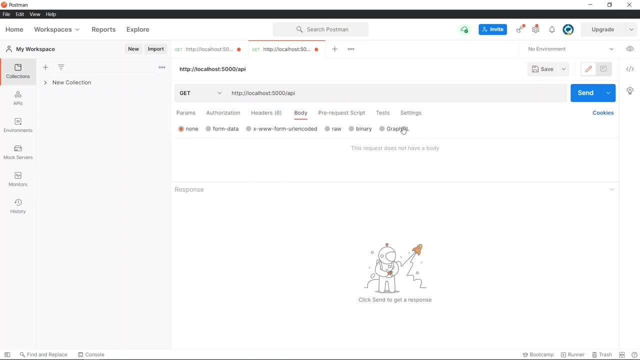 need to provide the document and for the document first we need to provide as the name which is provided there. so so the name will come from the requestbody. so the requestbody, just like, contains a key value pairs of the data, which is: we will submit it in the request body, like we will submit the request body from the postman and then in. 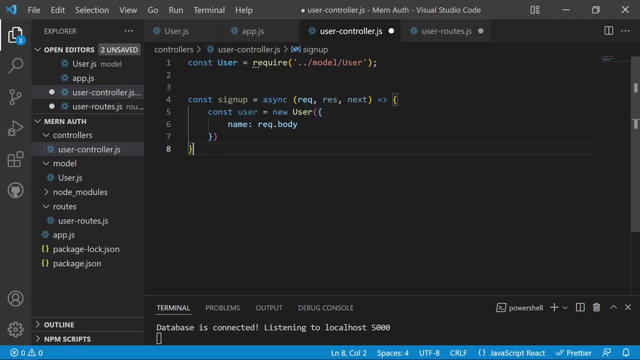 the json format. so it will contain a key value, pairs of the data. like we are now giving the name as a requested body, so it will contain a key as the name. so we need to provide the name as the key and then we can also provide here some. so if we can see about the email and the password, so 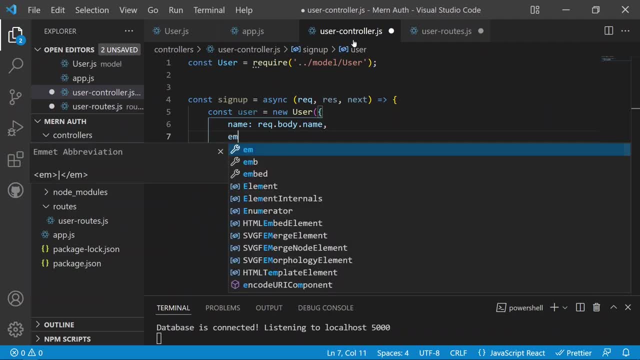 we need to provide the email and the password as well, so we can just go here. so after the name we have a email having an email field and the request dot body dot email. so now we have the email and now we can also define the password. so it will the password as the request dot body. 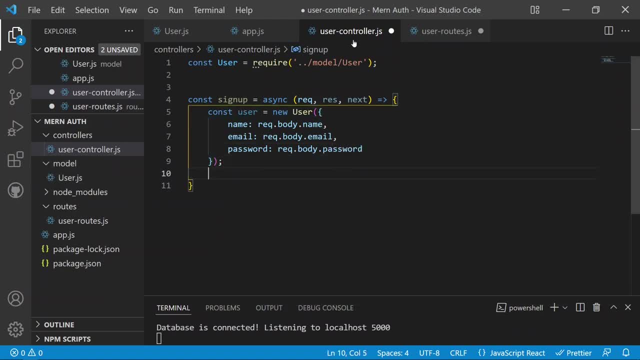 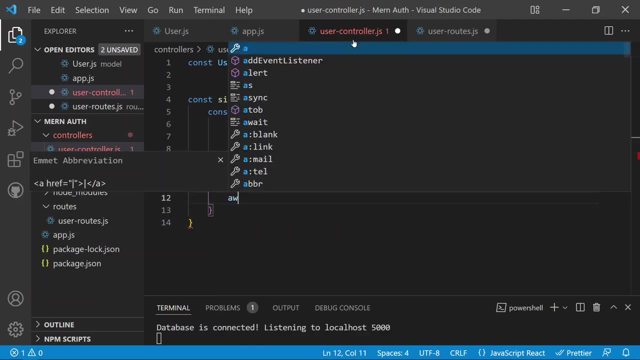 dot password and then it will create a new user for us and then we can just, and then we can just use the try catch block to save our users, like it will be the try, and then we can just create the await and then the new user which we have created as a user dot. 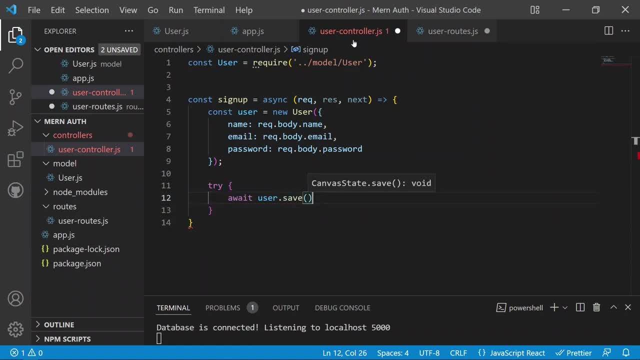 it will be the save. so save is a function which is available in the mongoose to save a document in the database and then we can also write here the catch statement as well, to catch if there is any errors. so we can just catch the error and then we can just. 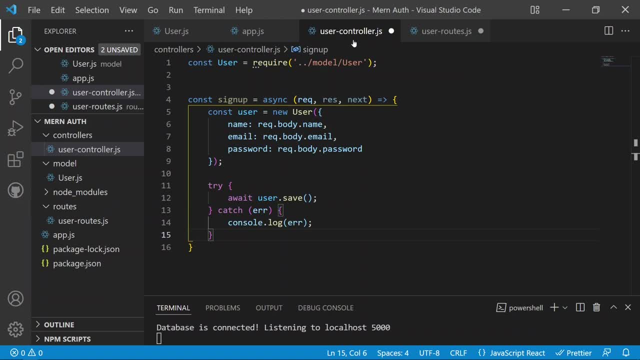 log it in the console, so it will the error. so now we are saving the user into the database and then we can just return something like return at the response dot status as the 201 which is created, and then we can just create here the json like a json and then we can. 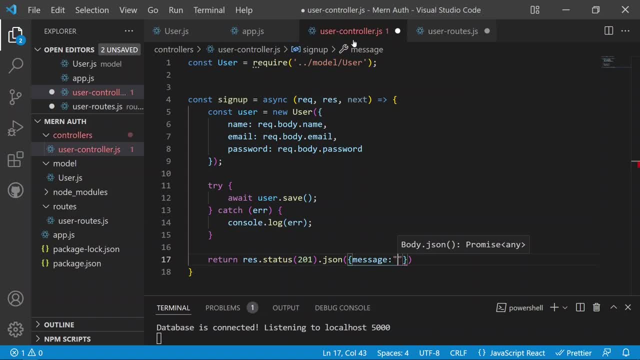 just add here the new user which we have created, like we can also send the user which we have created there, so it will be the user. so now we are now sending the http request for the signup and this is like a user and it contains a request, dot, body, dot name and. 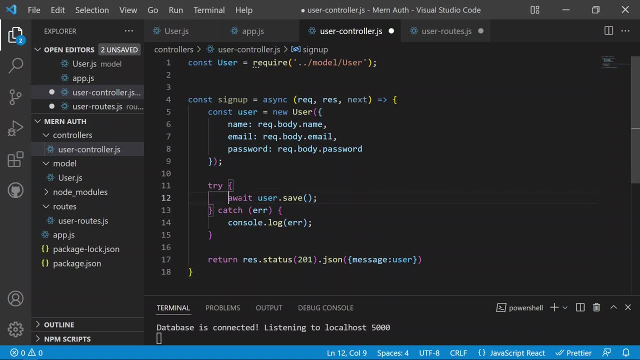 the email and the password as well. and then now we are now saving the document into the database with the user dot save function, which is used to save the document, and then we are now returning the status of the 201 as the json, which is the json. and then we are now. 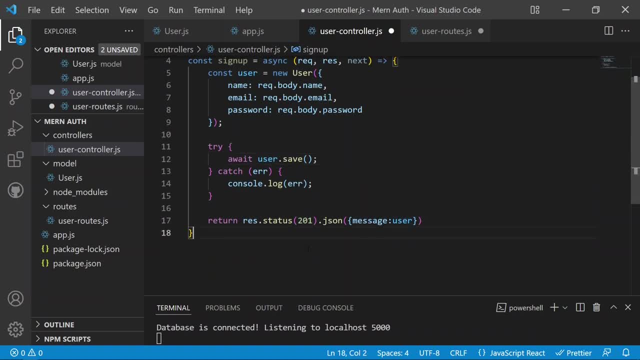 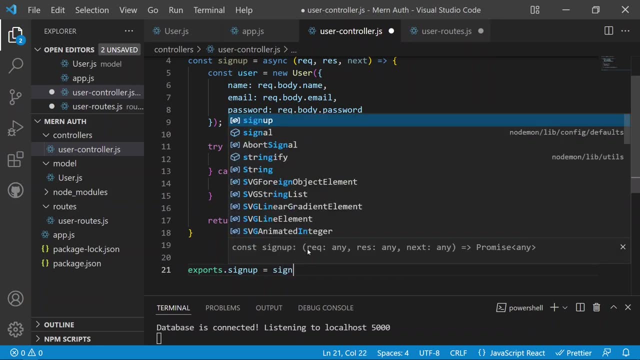 sending the json, which is equals to the message and the user, and then we can just export this function as well. like exports, it will be the exports dot the function name. like the signup, will be equals to this signup. so now we are exporting the signup function from there and 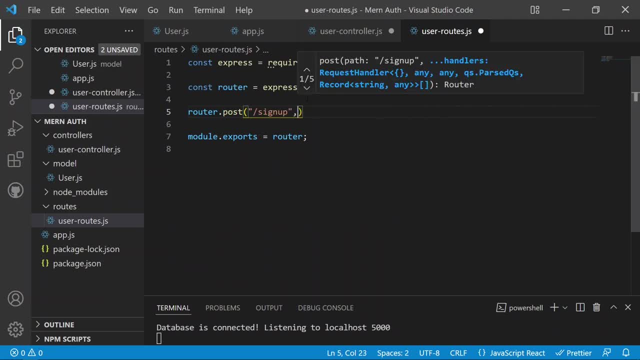 then we can now just go to the user routes and then we can now import the signup function from here but will do the signup. so now you will see the signup is imported from the user controller so we can use this signup here. so if i would now save in the end, if i would 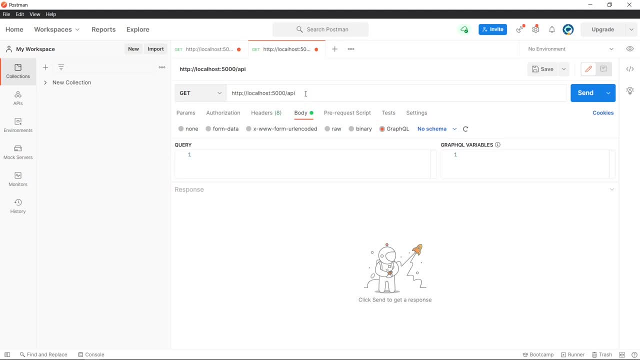 now go to the postmanual once again, slash api and slash it will be the sign up. so now we need- so now this is a post request, so we need to select the post from this drop down and then you will see there is a route as the sign up and then we can just add here the json body, here, like it will be the raw, and then 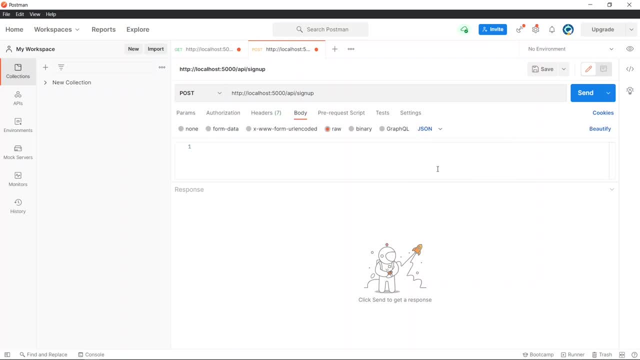 it will be the json from this drop down and then you will see now we have some fields like we have the name, so we can have a name like: i will provide my name here as the nickel and then it will the email, the email we can provide as a nickel at the rate- gmailcom, and then we can also provide a. 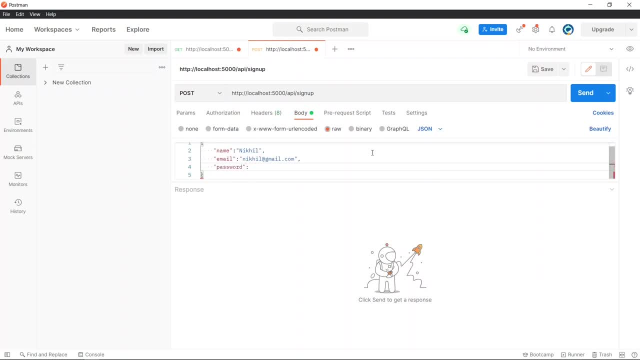 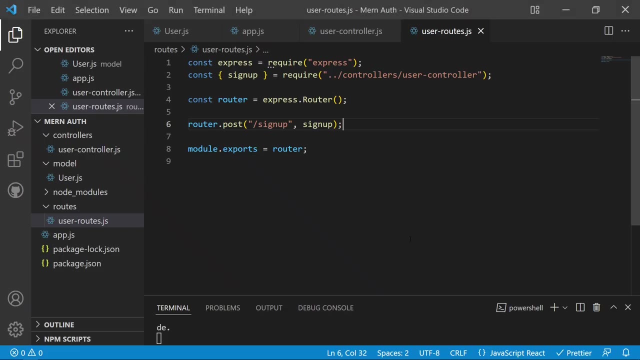 password. so the password will contain any password, like i would give a one, two, three, five, six, because the minimum length is the six. so now, if i would now send the request to the database, now we should see the success message. so sending the request to the database. so now there is an error. but what is? 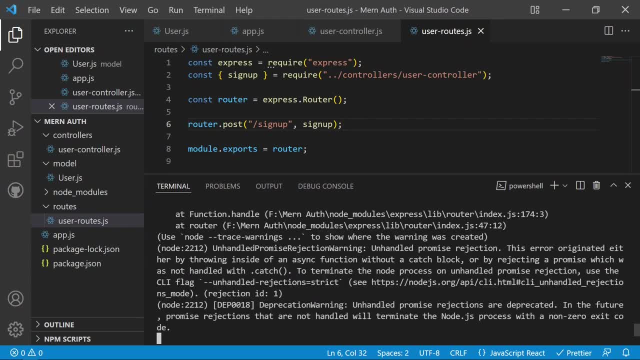 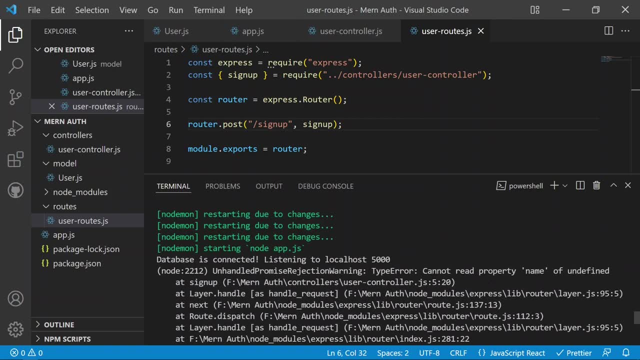 an error so we can see in the console and now we have the unhandled promise rejection warning, like there is an error. so this error, because now it is showing us that the cannot read property the name of the undefined, because now the server doesn't know that which type of 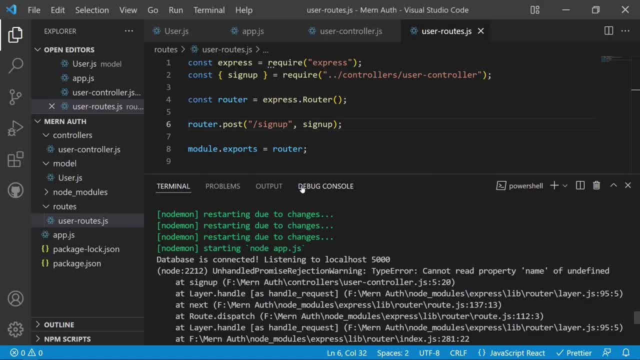 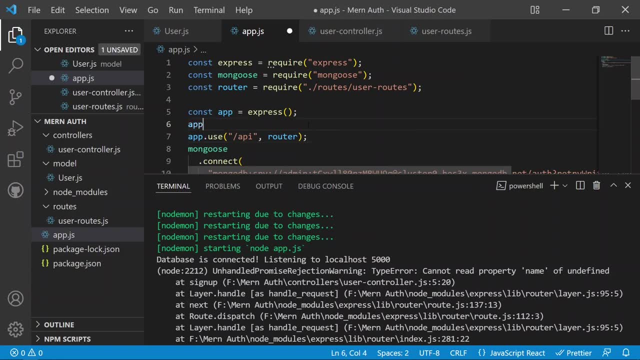 data it is expecting from the client. so we need to add here something to the server. like it will know that only the json data will be expected to the server. so we can use here the labuse, add a middleware, so this will be a middleware and then we can use the expressjson. so we are 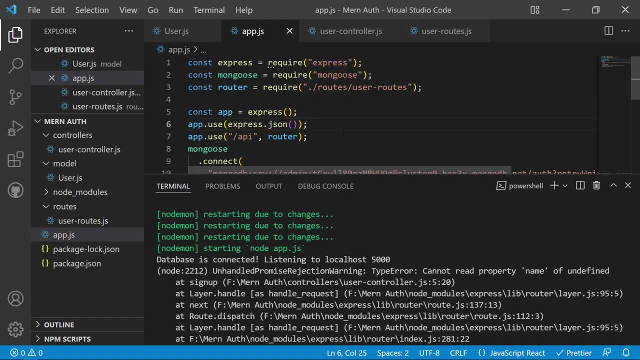 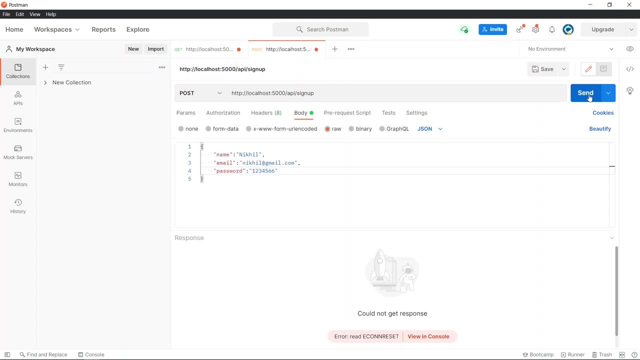 sending the json data from the client. so the server then will know that the type of the data is the json data. so we can just accept that. if i will now send the request again, now you will see the request has been sent to the database and then you will see. now we have all of the fields of the user, but we have two new fields. 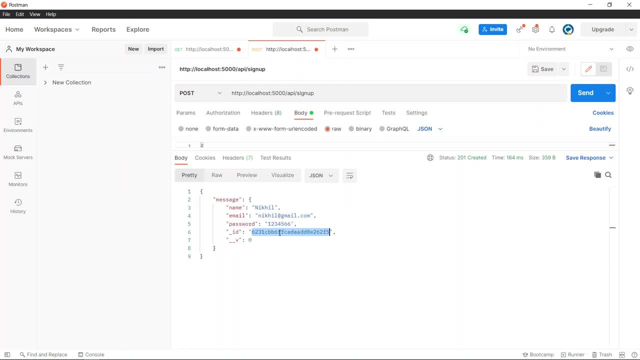 like id and the v the id. it is like the id which the mongodb gives us. so now this means that our product is now successfully sent to the mongodb and it is giving us the id in return, and then you will see the status is also the 201, which is the mongodb, and then you will see the status is also. 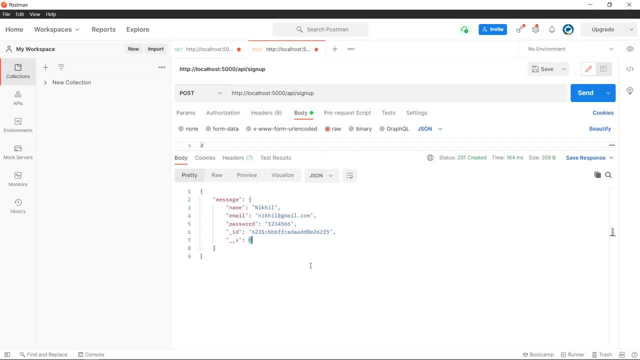 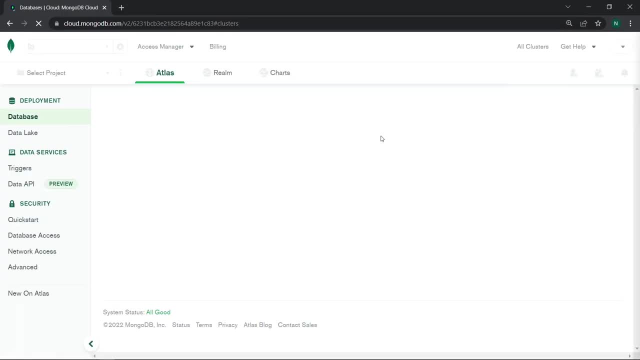 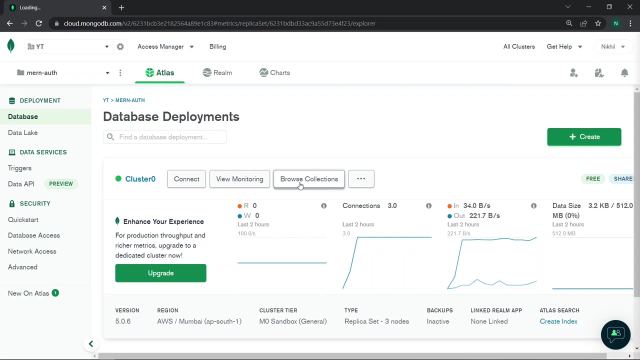 the 201 which is created. so if you are not sure that the user is now in the mongodb, so you can go to the mongodb and then you can just search for the user there. now you can just click on the browse collections, the collection which we have- and then we can just go to the- i think- the users collection. 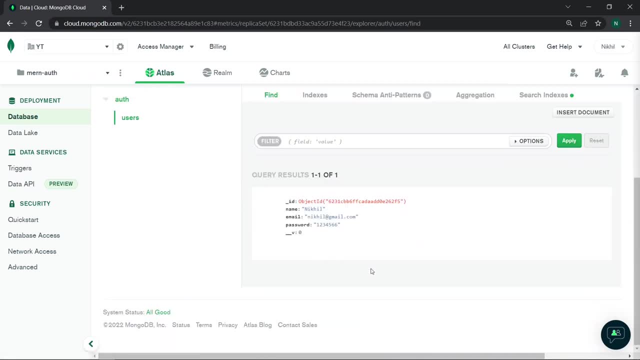 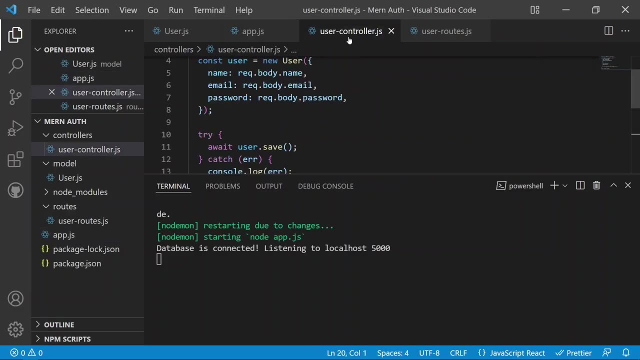 we have. now you can see, the auth is a database and the user is a collection. now you will see, now we have the database user inside our collection, now we have the user. so now the signup functionality is completed. but there is one thing which you need to add: their validations. 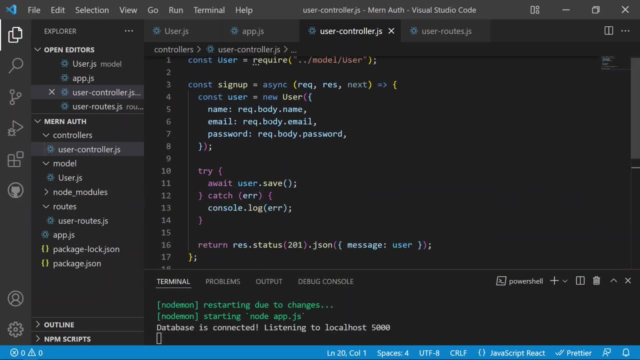 after that, like you are just declaring a user as the new user and you are now providing all of the details there, and if you will provide the user as the same email, so it will throw us an error because we have not defined the user there, but it will still send the request to the database. 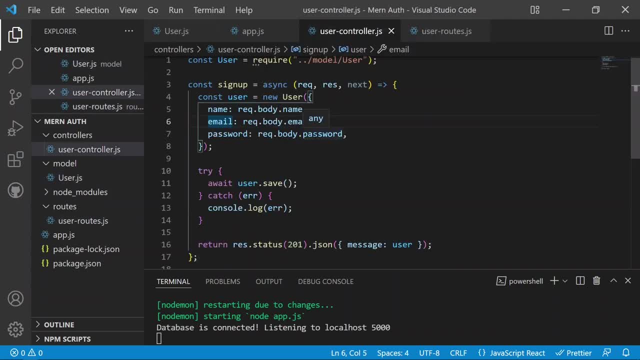 so we can just stop that and we can just validate before it send the request to the database and then we can just return something like: this email is already there, so we can just add here some let's. so we can just create a variable as the let as existing user. 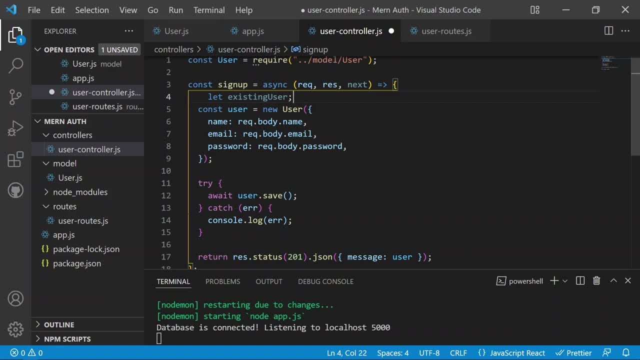 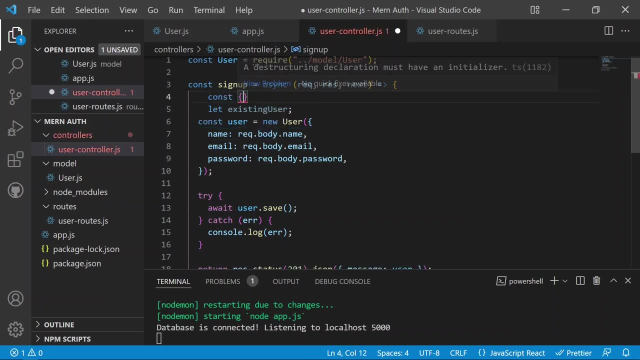 the existing user will be by default an empty value and then we can also destructure the requestbody from there, because we don't need to write always the requestbody, requestbody. so we can just create an object and we can just destructure all of these fields from the request. 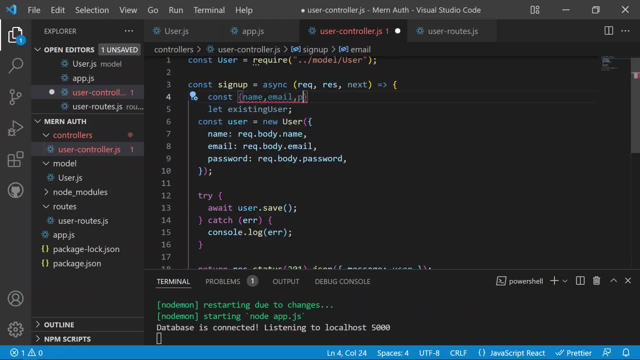 body, like the name, like the email, like the password, and it will all be coming from the request body. so we are now destructuring everything from the requestbody and instead of this name and the requestbodyname, so we can just remove the, the name and the email and the password as well. 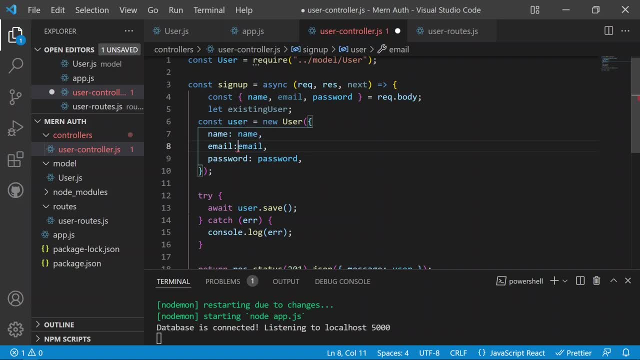 so now we are sending the name as the name and the email and the email and the password and the password, and then we can also remove this name and the name here. also because- and the es6 provides us a new way- that if your name, if your key and value pairs are of the same variable name, so you can just 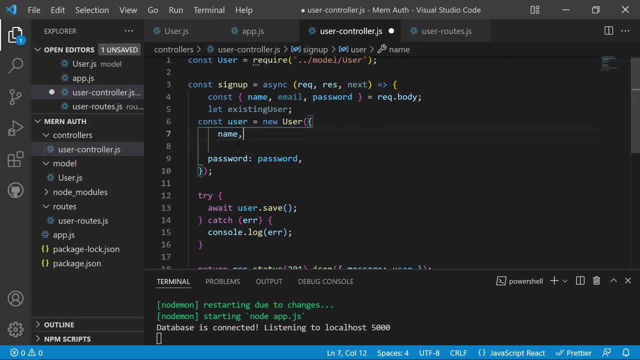 define as the same thing, like the name, which i will provide as this. so it will be acted like the name colon, the name, the key value pair. so we can just provide here the name and the email and the password here and we can just remove the password from here. so now you will see, so we have. 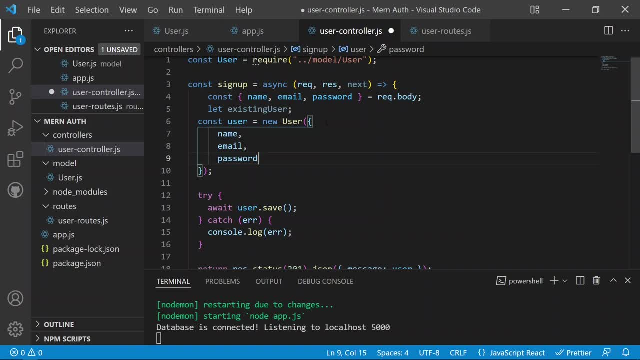 destructured successfully all of the details. so now we can just create a validation, like we are now defining the existing user, so we can just write here the try catch block again with that try and then we can just check the existing user, like if the existing user, so we can just check in the user model which we have. so 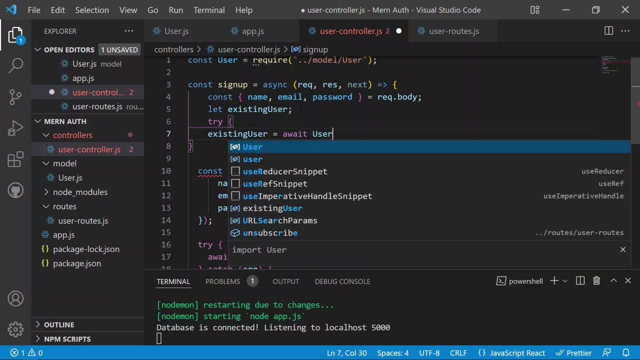 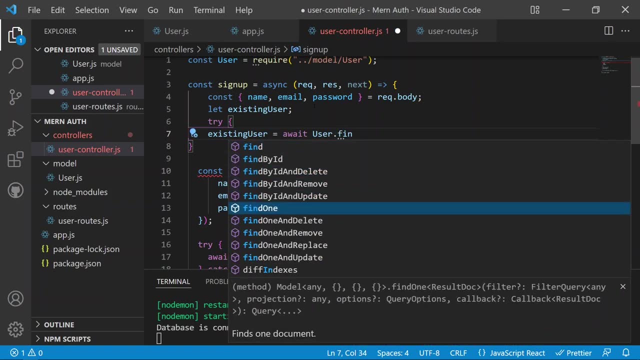 it will be await function because it will await for the task and it is an asynchronous task. so to the user model which we have imported, and then we can just call here the function as the find one which will find a record in the user, and then we can just add an object, and then you will. 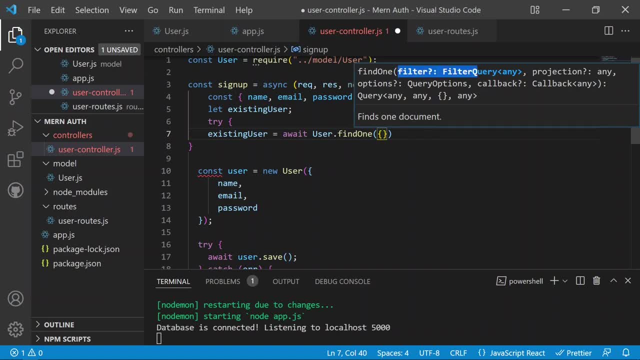 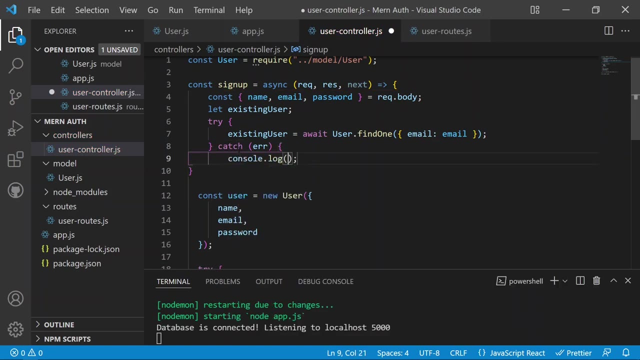 see it will be having a filter query so we can just add a requiry, like if the email is already there in the mongo db, so we can just check that field, like even if we provided the catch as well, like it with the error. so now we are now checking if the existing user is already there in the mongoose. 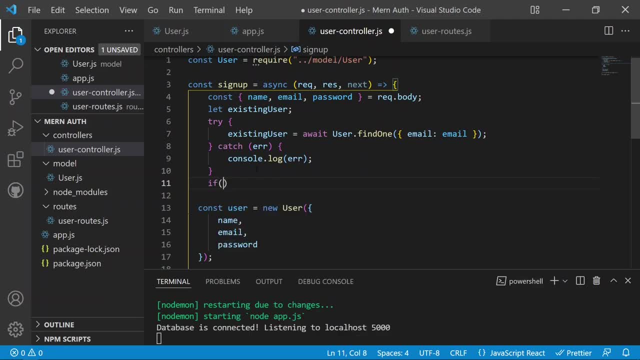 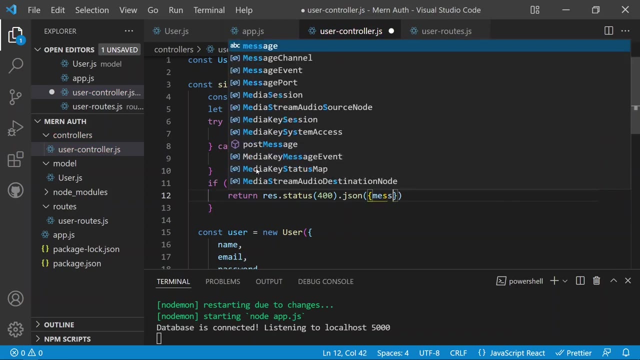 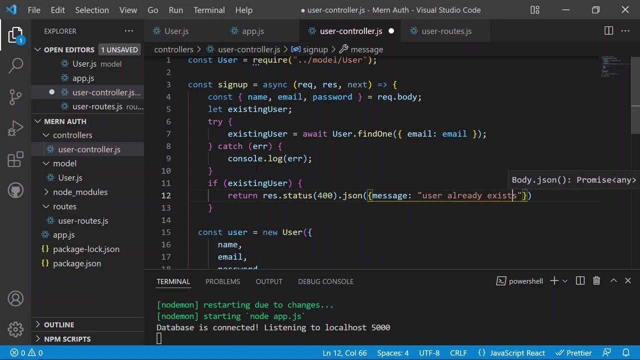 database in the mongo db database. so we can just check, like if the existing user is there, so then we need to just return, as the response dot status will be equals to like the 400, and then we can just add a json message also, like the message will be there as the user already exist, so it will. 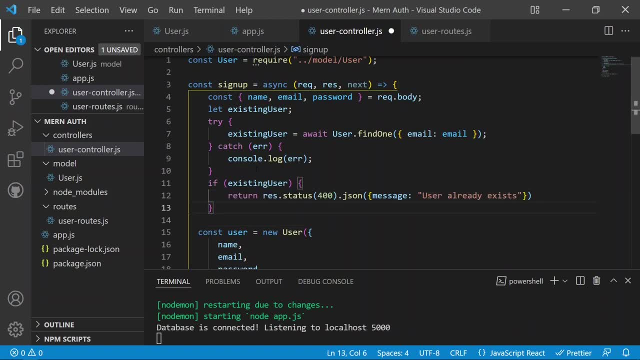 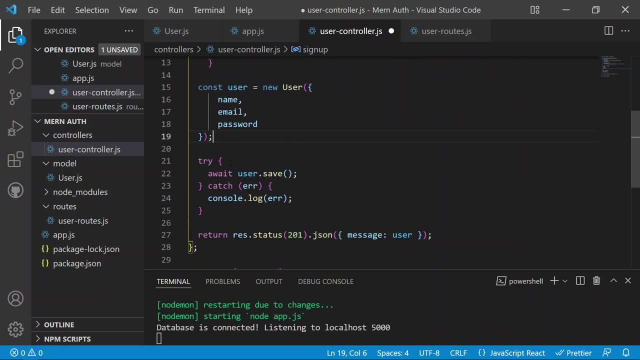 be a message which will be throw with for the validation purpose and else after this, after checking this, now we can just add here the user which is equal to the new user, and then we can just try and catch with the statements, and then we can just add here the return statement like the: 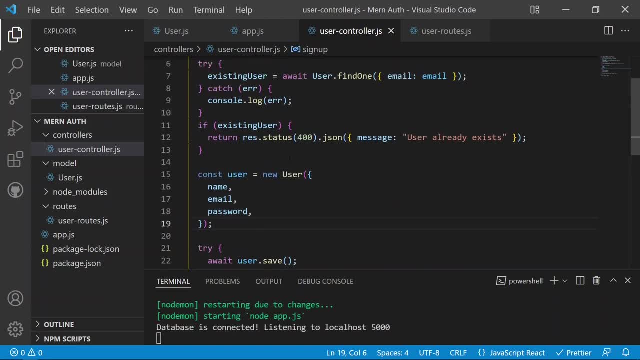 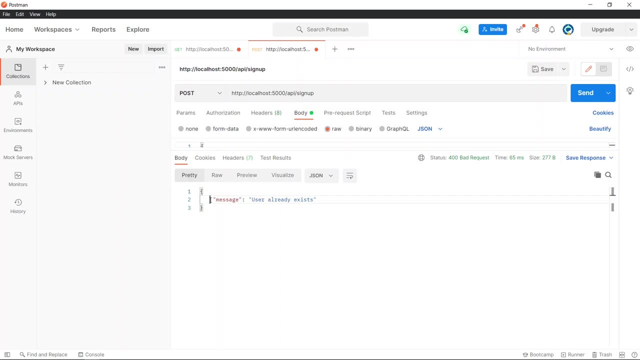 return status equals to 201. so if i will now save, now we have added some validations here, so now if i will now send this record again to the database, now you will see it will throw us a message that the user already exists. so now we can see we have. 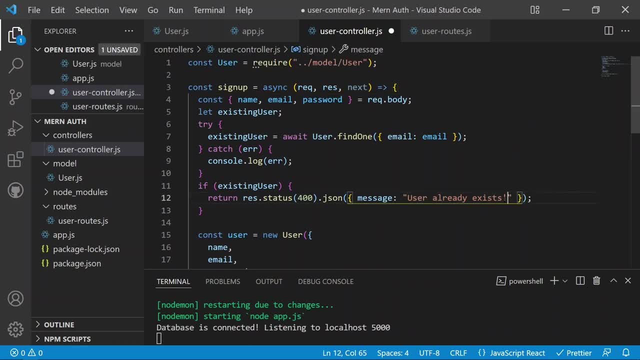 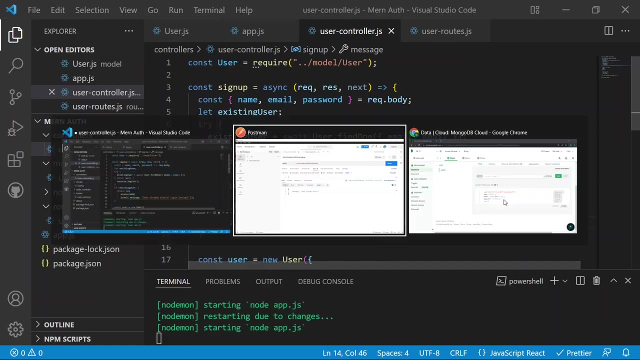 the validation of the user. if the user is already exist, so we can just now register the user again. so we can just add a functionality like the login instead. so we can just build here the login functionality after the user has been created. so after that, if i will now just send, 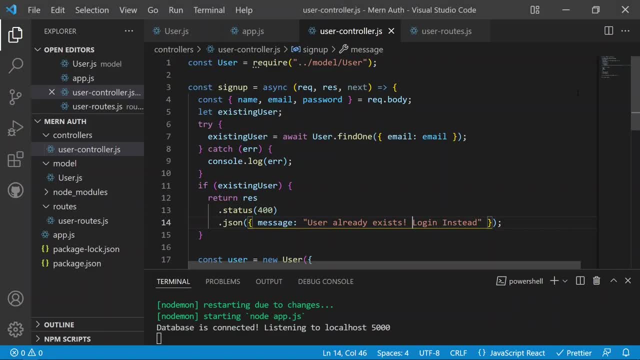 again. now you will see the user already exists and the login instead. so now the user is there. now we need to build the login functionality. like the user will be logged in now, so we can just create the user functionality as the login. so now, before moving ahead to the login route, 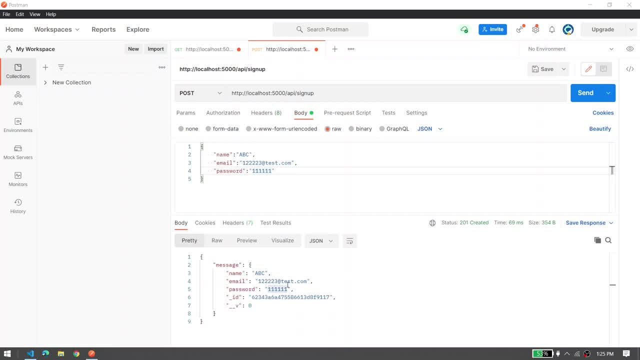 we can see that we are storing the same password in the database which we are receiving from the requestbody. so if i now send a new request to the database, a new sign up request, and if i now click on the send now, you can see. now we are getting the same password. 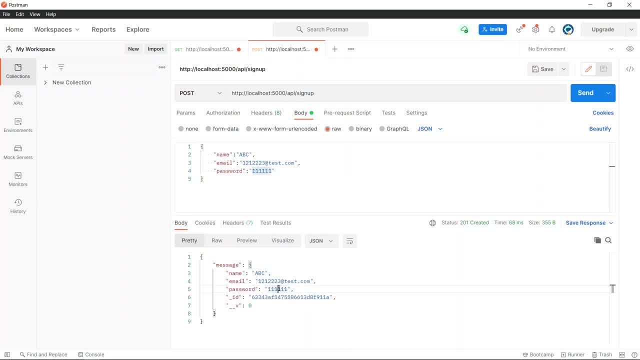 which we are now receiving from the user. but it's not a good option, like if, by chance, our database is hacked, so we will be exposing every details of the user, including the password, to the hacker and now hacker can do anything with that. and we have another use case that if we are building a backend server and suppose we have a team which is working, 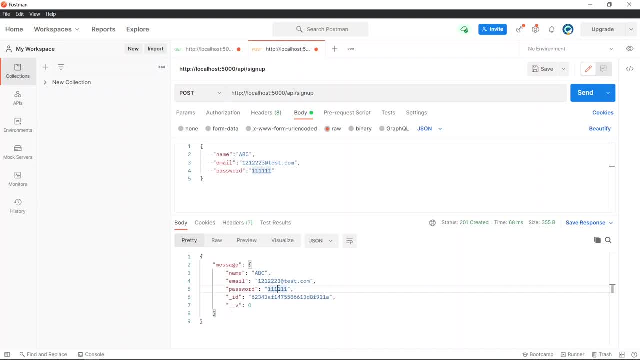 on. so we can't share the password of the users with our team and it is confidential information about the user. so what we would do in both the scenarios, so it's not the right way of storing it in a database. we have to see the solution that how can we store the passwords. so the solution can be we can just: 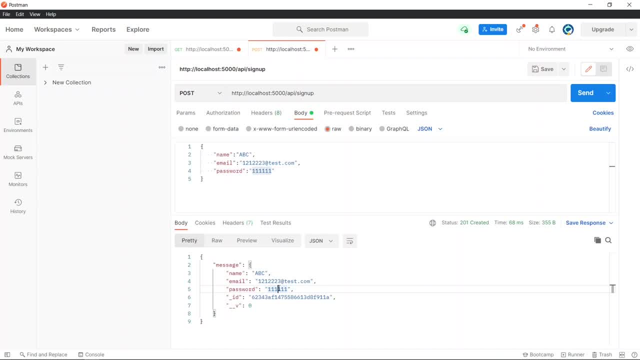 encrypt the password of the user and then we can store it in the database so that it can't be directly exposed in the database and it will be a hashed string and it will not be easy for the hacker to decode it. so we will encode the password and the hacker needs to decode it to get the user's. 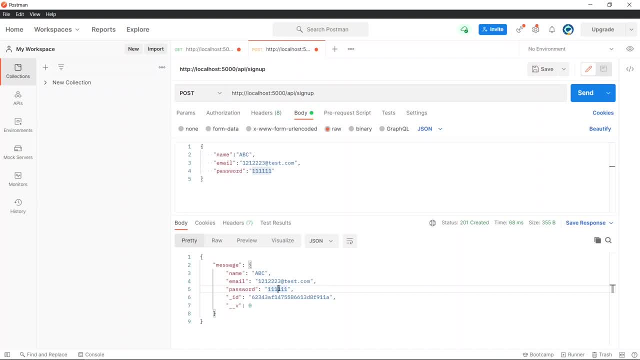 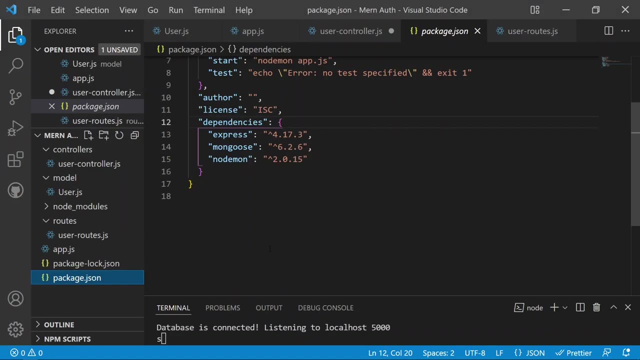 details. so that's the right way of storing in the database. but now how do we encrypt that? so for that we can use a package name, which is the bcryptjs, to just encrypt and then the decrypt, the password for checking the user information. so i will now go and if i will now install the bcryptjs from there, so i will. 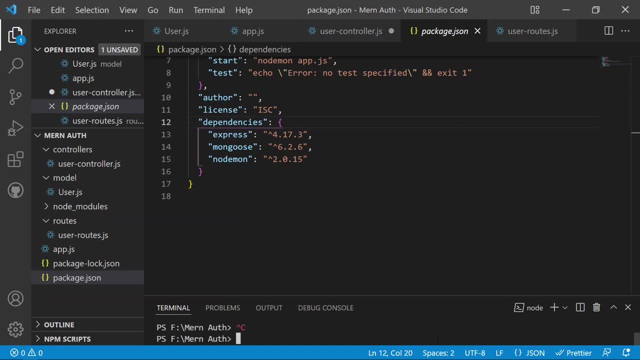 now stop this terminal. and now we have to install the bcryptjs, npm install as the bcryptjs, and now the bcryptjs is now installed, and then we can go to the user's database, and then we can go to the user controllers, and then we can see that whenever we are sending a new sign up request. 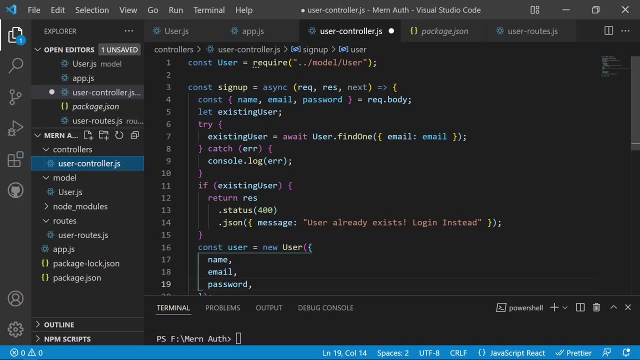 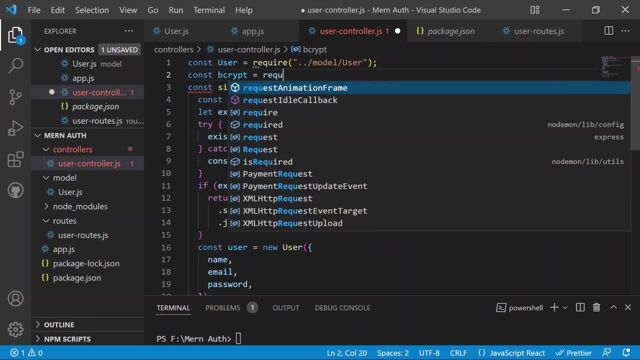 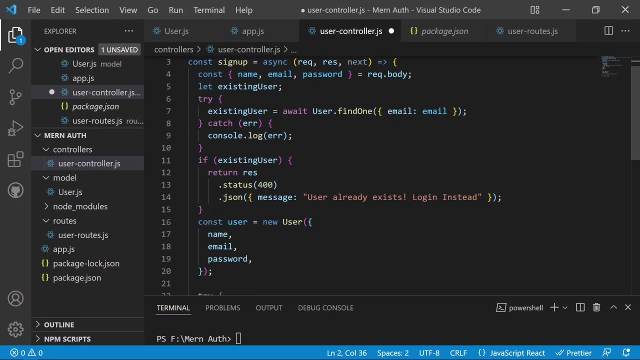 then we should now encrypt the password using the bcrypt. so first we need to import the bcrypt, so it will the const, as the bcrypt will be equal to require, and then we will be requiring the bcryptjs from there- bcryptjs. so now we have imported the bcrypt whenever we are storing a new password. so 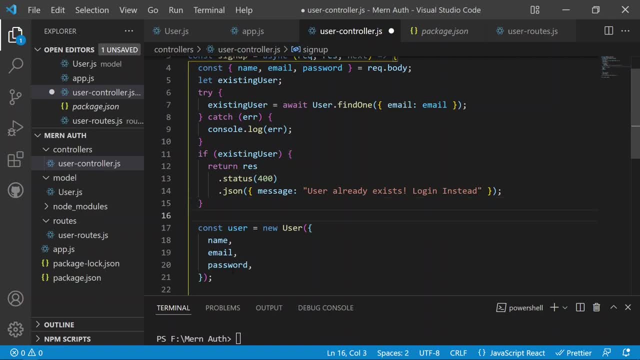 then we can just create a hashed password before that. so if the existing user is there, and then as the 400 and we are sending a message as the user already exists and the login instead. so here after that we can just store a password as the hashed password, so it will the const as the hashed. 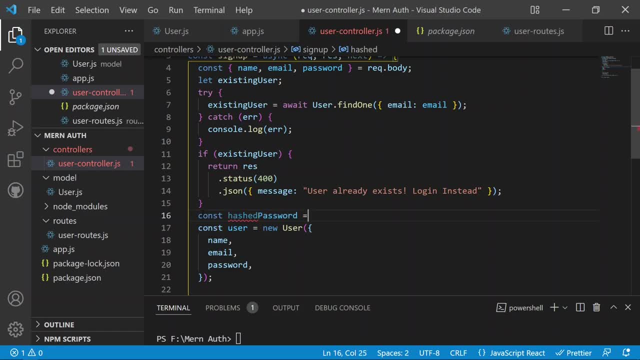 password and it will be equals to the bcrypt which we have now imported: bcrypt dot- hash sync. so we have a function which is the hash sync, which is a synchronous way of hashing the password, so we can just hash here the password and then we can just store the password as the hashed password instead. 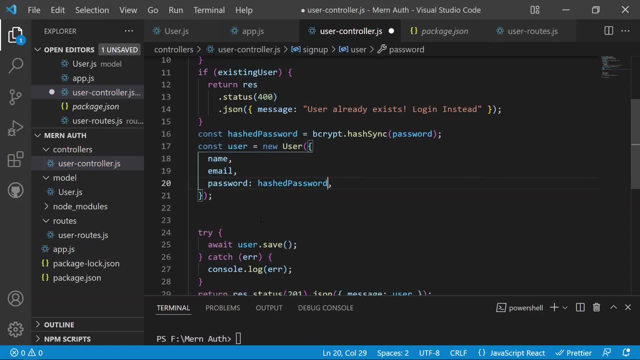 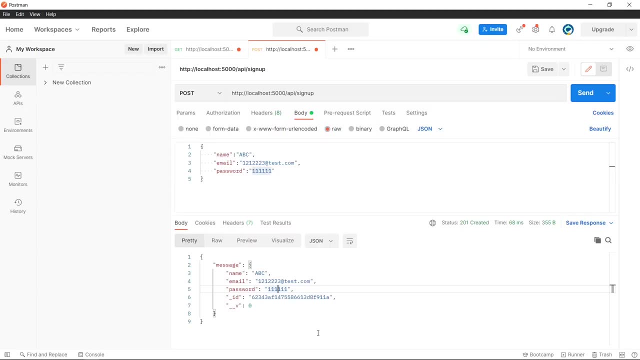 of the direct password which we are now getting from the user. so if i will now save and if i will now just restart the application by writing the npm start and then we can just check again in the postman, so if i write a new email like this, like nt at the rate test dot com, and i am sending the 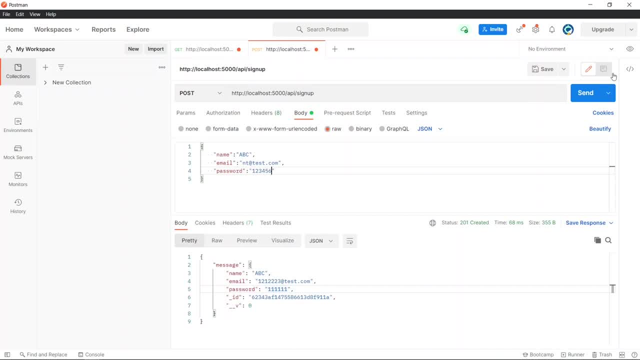 password as the one, two, three, four, five, six, and if i am just sending a new post request, now you can see the password is the password, and if i am just sending a new post request, now you can see the password is different. now you can see, now we have a hashed password in the database. so this is what. 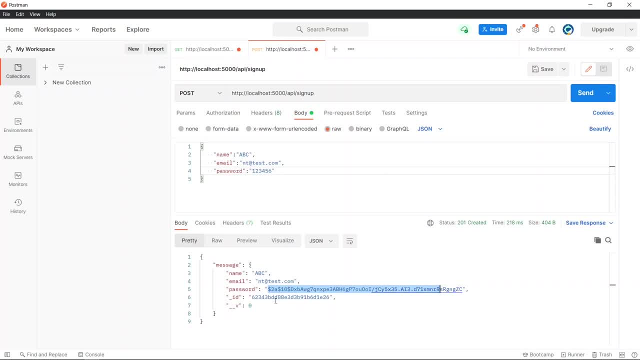 we wanted like. we don't want to expose the password to the hackers, even to our team as well, so we want to store it as a hashed password, so that it would be very difficult to encode this password. so it's the right approach. now the signup functionality is completed, and now we want to log in the user. 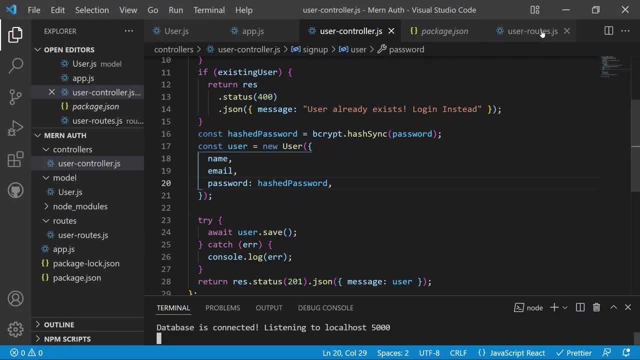 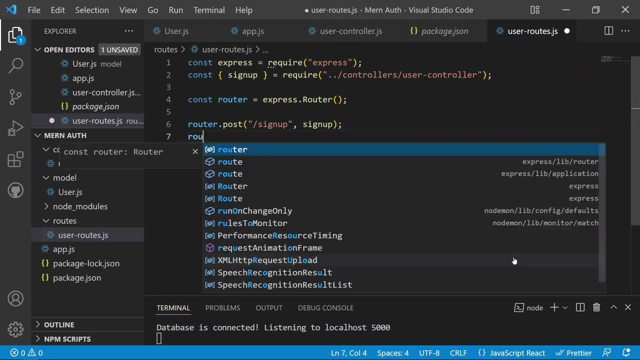 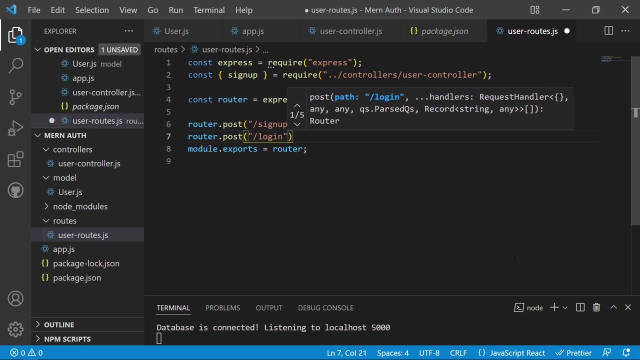 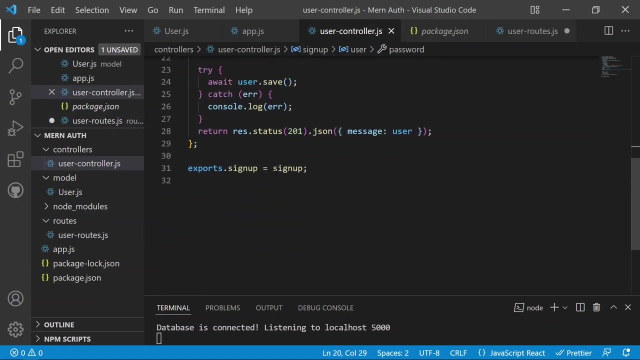 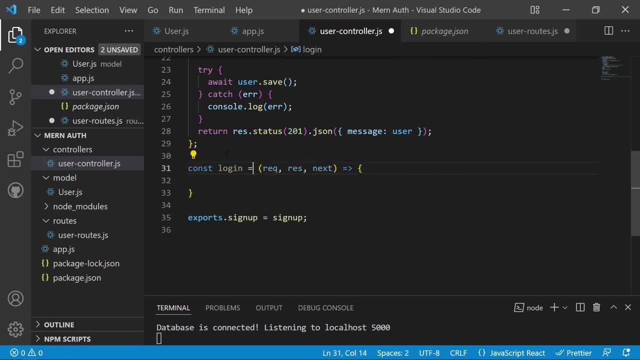 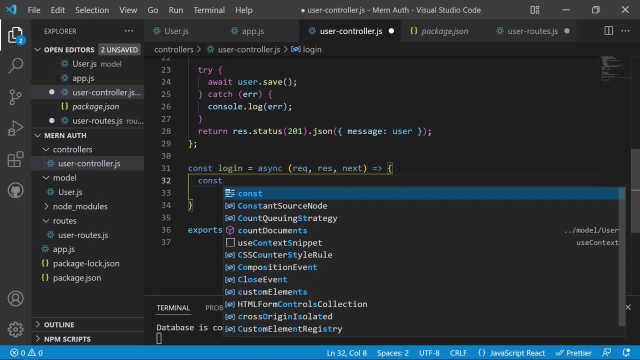 will be an arrow function once again and this will also be the asynchronous function, because these all are the asynchronous tasks and then same. we can get the details of the user via the request body. so do the email and the password. so we need the email and the password for the login. 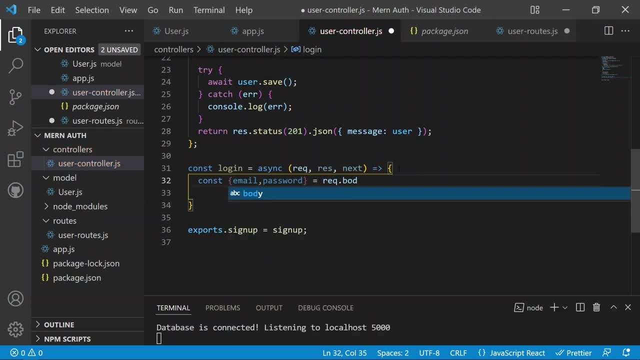 functionality. so we will be getting it from the requestbody again and then we can just check like we can just now declare a existing user again like let existing user, which will be equals to like by default it will be undefined. and then we can just use here the try catch block and then we 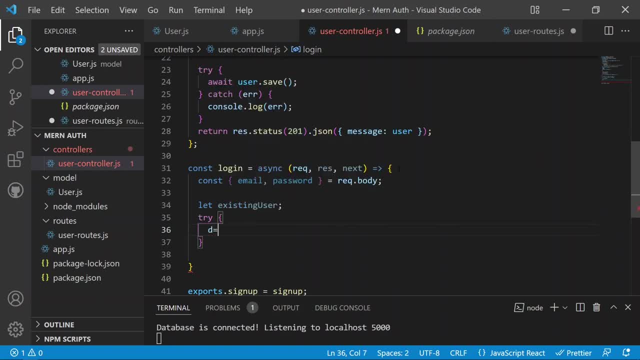 can just check if the user exists or not, so it will be existing user once again. existing user will be equals to the await and then we can just find one record again, like it. will the user model dot find one and we need to pass a query here in the object, like the email. 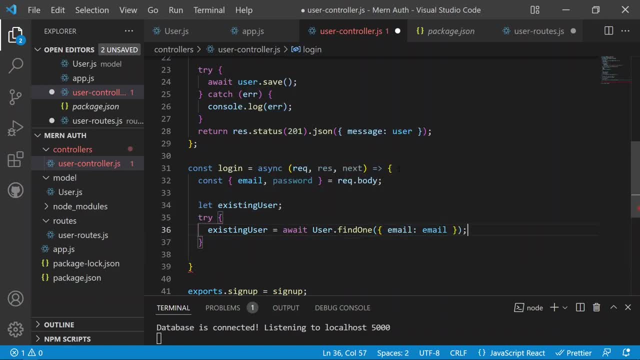 would be the email which we will be using, like email will be equals to the email and then if the user will, then the find the request and then we can just log in the user. so now here in the catch blocks, so we can just return the error like return new error, and the new error would be the new error. 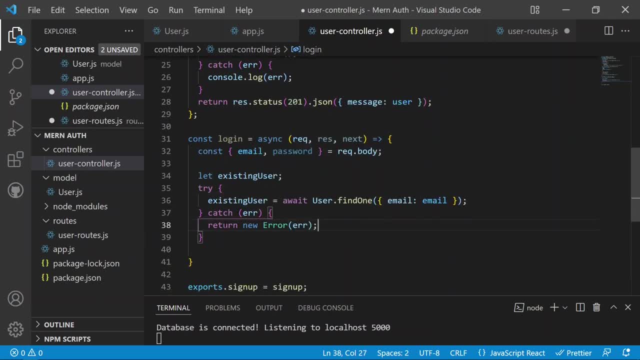 which we are now receiving from the track as block and now when we have the existing user, so we can see if we don't have the existing user and we can just return the server with the response dot status and the status would now would be 400 dot json. we need to send the json again and it will be like: 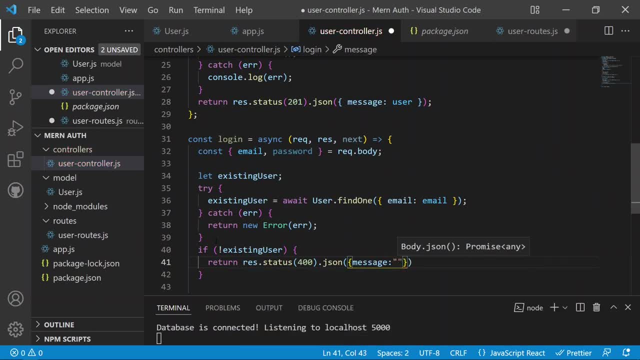 the message, and the message can be anything like the user not found, dot. and it will sign up. so we are sending a message as the user not found and the sign up, please. and now we can see. and now we have hashed the password of the user. but now how can we check? 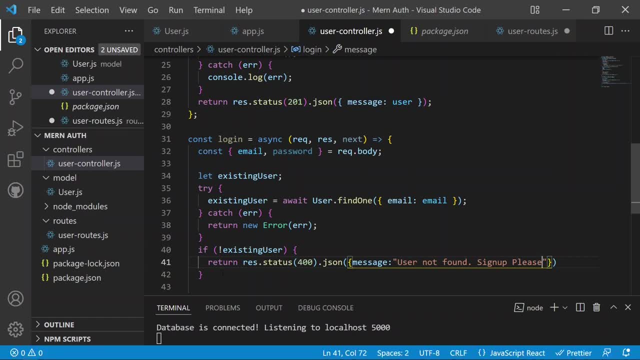 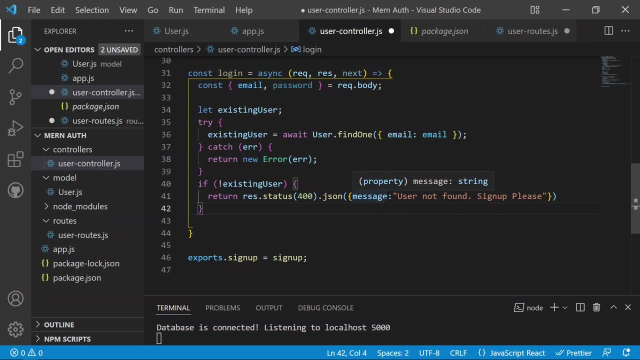 the password. so now we can see if the existing user is not available, then we are returning the response dot status as the 400 and we are sending the message as the user not found and please sign up. but now how do we check the hashed password with the actual password of the user and the? 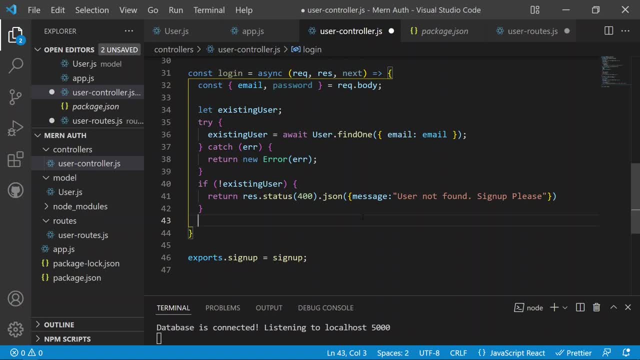 solution is very simple again. so we can compare the password with the bcrypt again. so the bcrypt provide us a way to just hash a password, so it will be the const as the is password correct. so we can just declare a variable as the is password correct. and we have a function in the bcrypt js like 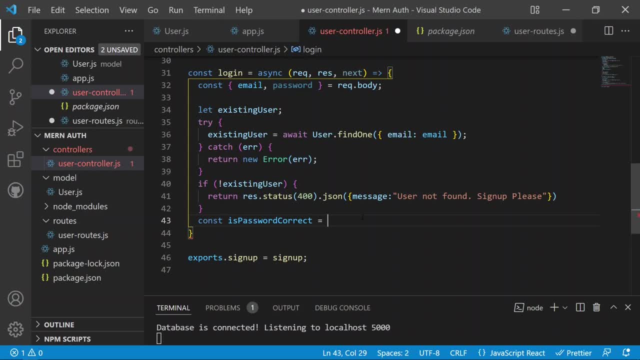 sync, which just synchronously compare the password and then returns a boolean, so we can just use that. it will the bcrypt dot compare sync and then we can just use that and then we need to pass here the password of the actual password, like there. we are now sending the password which we are receiving. 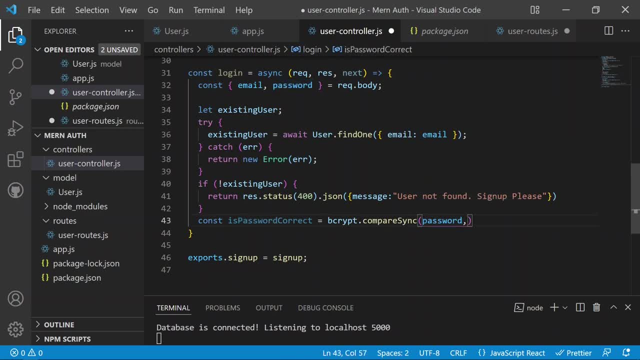 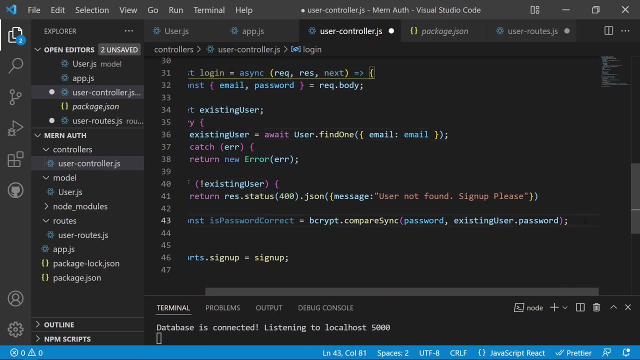 from the requestbody. and then the second parameter is from which password we need to compare. so we need to compare it with the existing user dot password, so the existing user. if we have the existing user, then have the password as well, and then we will compare the existing user with password. so then we can see. 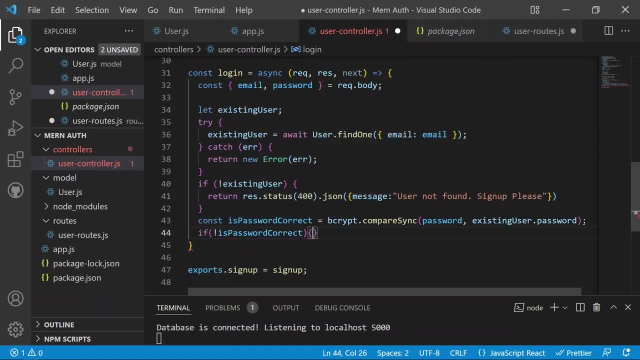 if not, so that if the password is incorrect, then we can just return again like the return response dot status and it will be equal to the 400 once again as the unauthorized, and then we can just send again the json again with the message and the message can be again like the invalid, invalid. 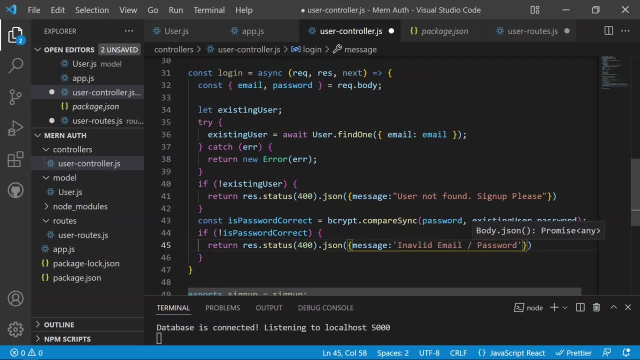 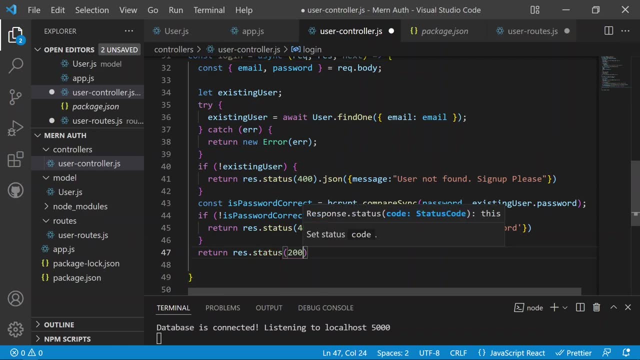 email or the password. so then we will send this request, but no, so if the password is now correct, then we can just return the response dot status as the 200, which is the success, and then we can just send a json message once again as the message and the message would be like: successfully. 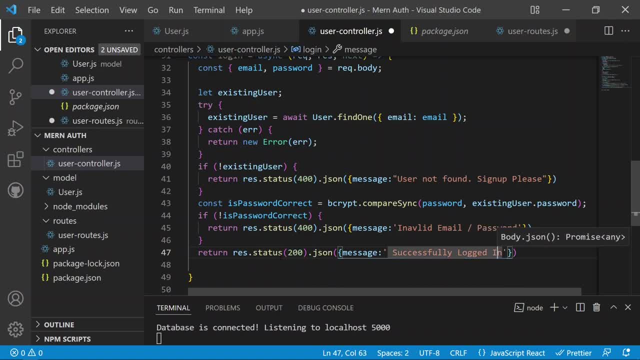 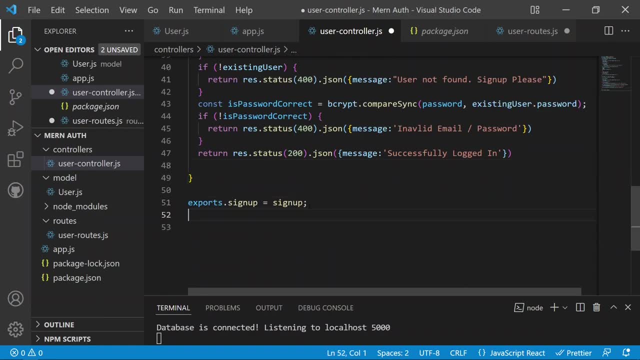 logged in, so we will send this message to the user, if everything is okay. so if i will now save and if i will now just try out sending the request, and before that we need to just export this as well, like it will be the exports dotted with a login and it will be the login function which we have. 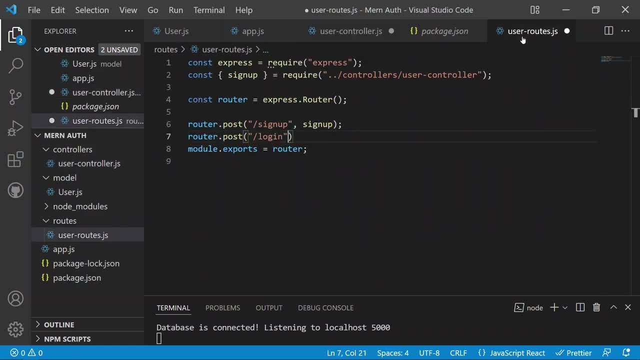 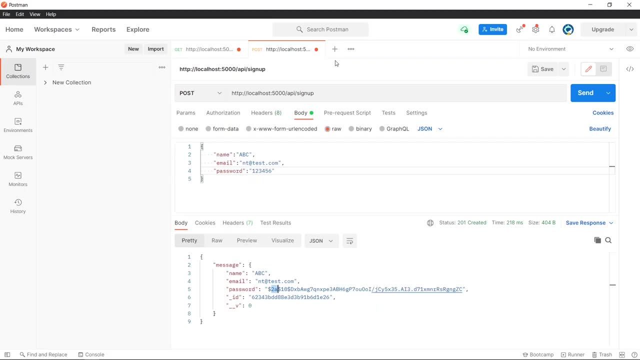 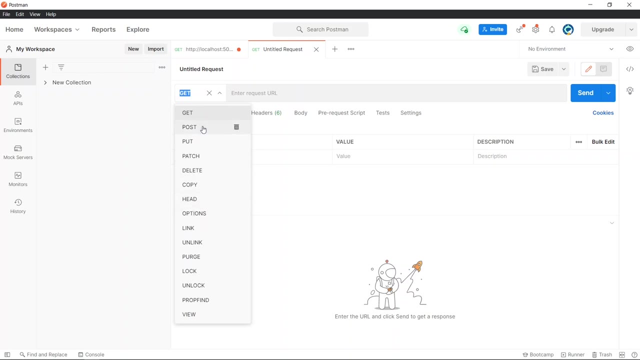 now created, so it will be the login, and then we need to use the login in the user routes as well, so it will the login. so if i would now save and if i would now check the request again now i will now test with the sign up. so first i will now sign up the user like it will the sign up, so it will. 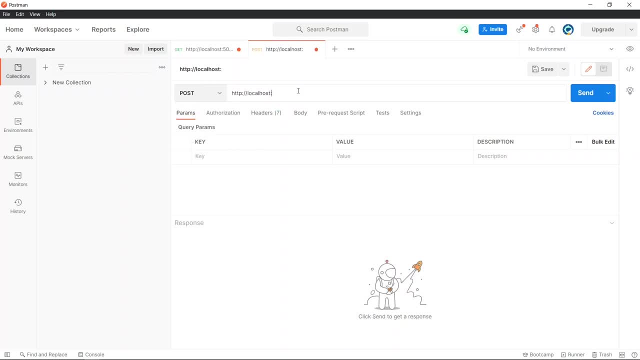 be the post request and the url will be the local host at the rate 5000 port and then we'll sign up and then the requestbody would be. we need to send the raw, once again the text, we need to send the json, and the json data will contain a name of the user, so we need to send here the name, the name. 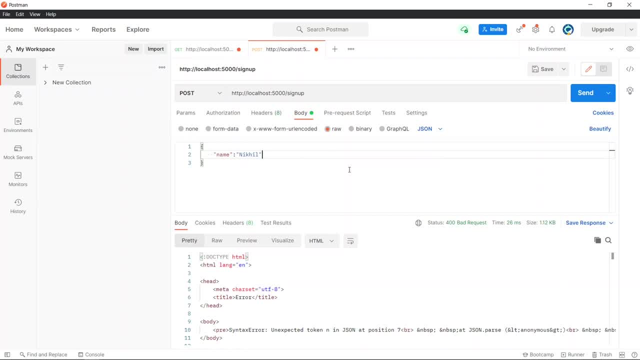 will be like nickel. i am sending my name once again and i am sending email, as the email and the email would be like nikh at the rate testcom, and we are sending the password as well, like password and the password would be. i am sending the one, two, three, four, five. 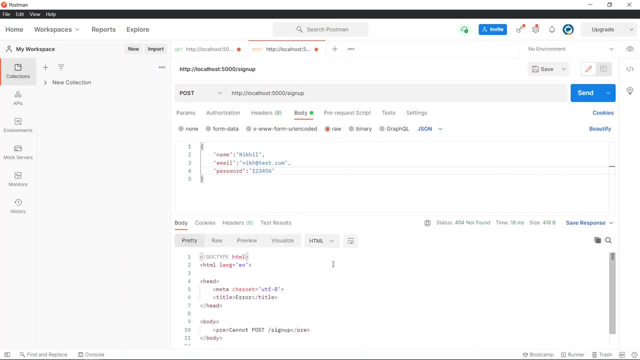 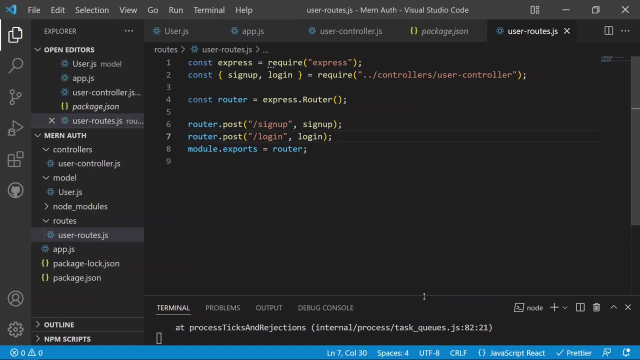 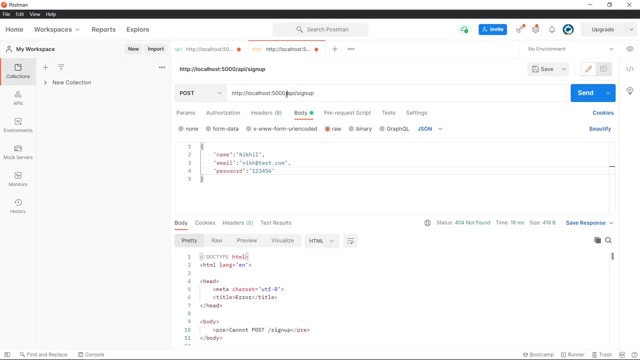 six and if i now send the new user to the sign up request. now you can see. now i think there is an error like four or four not found, so we have to see what is there with the request. so unexpected json token at the position seven. so it will be the api and then we need to send the request now. 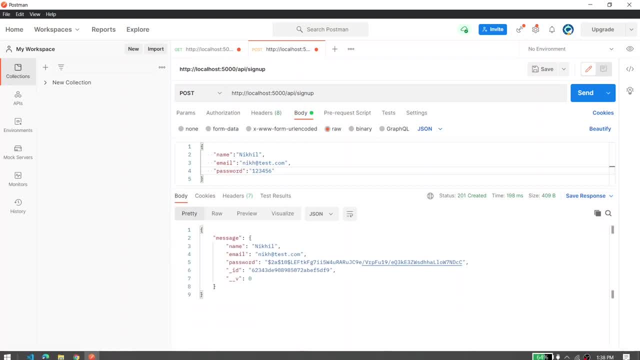 you can see, now the response is successful. now the response is the 201 which is created, and then we are sending a nickel and the nickel at the rate testcom and we are storing the hash. so we can just check the same details with the login now. so we can just now create a login request. 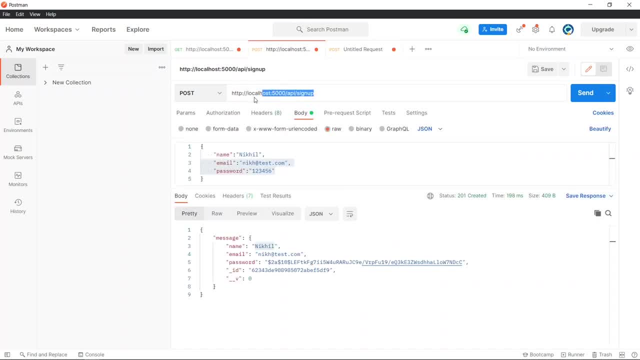 it will the login http request, the url will be the same and then we need to just remove the sign up from there and then we need to enter the login there, a login, and then the body will contain again the raw and it will contain the json format once again. and if i will now just add here the json, 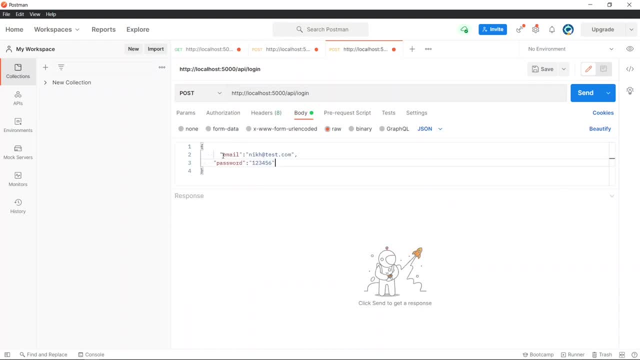 so i will copy this and i will paste this here, and if i will now just send the request of the post and this match is now. you can see, now we are successfully logged in to the database and now the status is also 200, which is okay. so now we have completed the login and the sign up and now we have successfully. 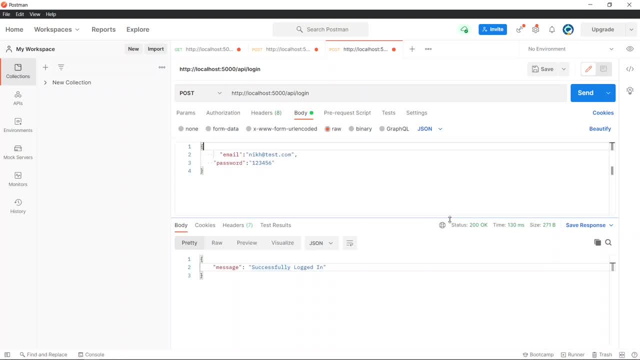 created a login and the sign up functionality in our application and it is good to see, as we have stored the hashed password and now the password is fully secure and we can also log in. but now what do we need to do after the login? so we need to authorize the user. now the authentication is done. 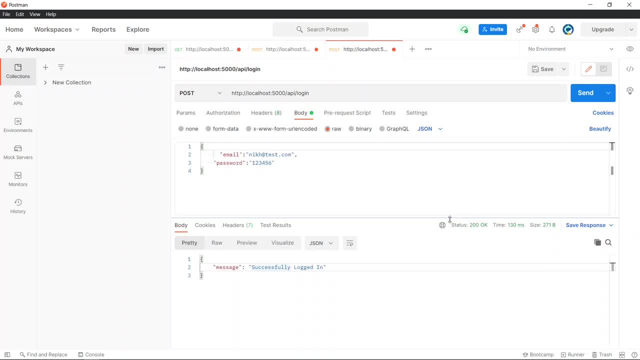 authorize the user. so after the login, we need to provide user the access to use our services, of our application services. but how do we provide the access? so we can provide a token to the user to provide access, and that token will be very confidential and it will contain the details of 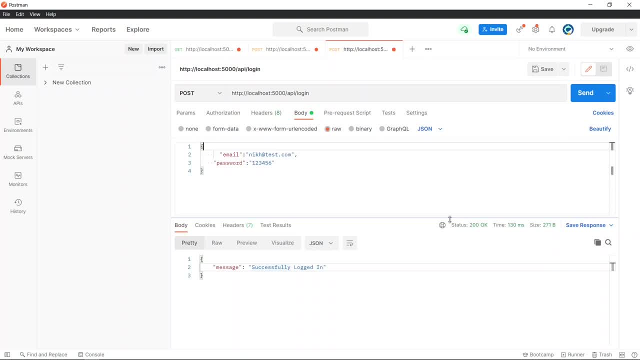 the user, like id or the email, and after a specific time the token will be expired, like after an hour. the token will then expire and then keep the user logged in into the application. so we can just regenerate the token and keep the user logged in and we can also destroy the access of the user as 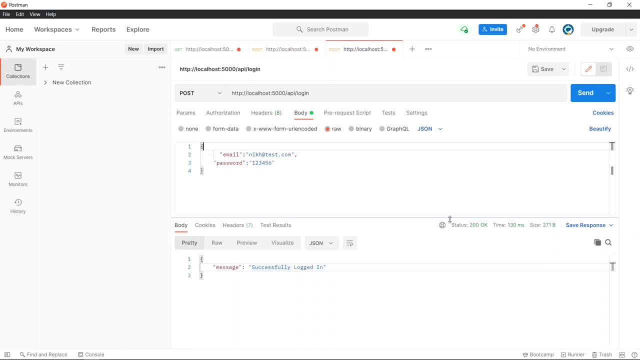 well, but we can generate a jwt token, which is a json web token- and i'm sure you have heard before- which will help user provide some access to use our application. so, for example, like we can generate the token now, user have to provide us the token to get the details. 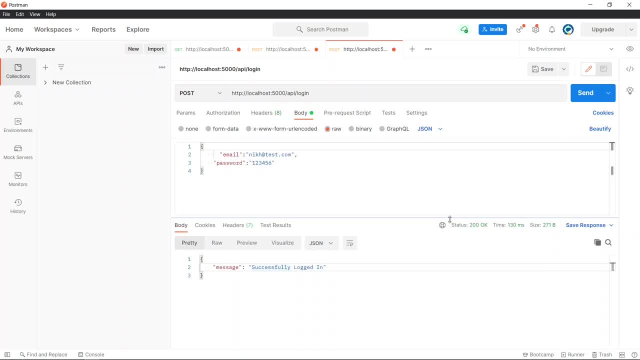 like for this application, we will just show user the details of the user, like its email and the password. but if you are working with the big application, then you can offer services after the login and the authorization, only when the user will then provide you the token. so the user 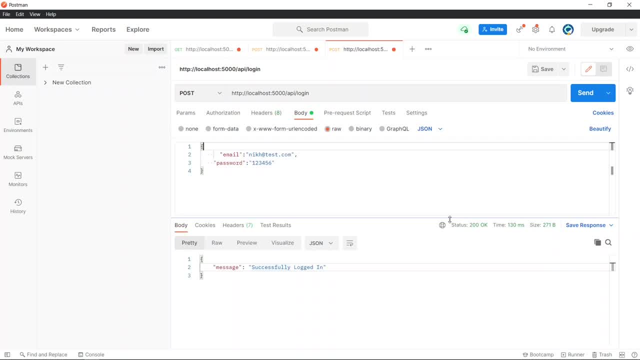 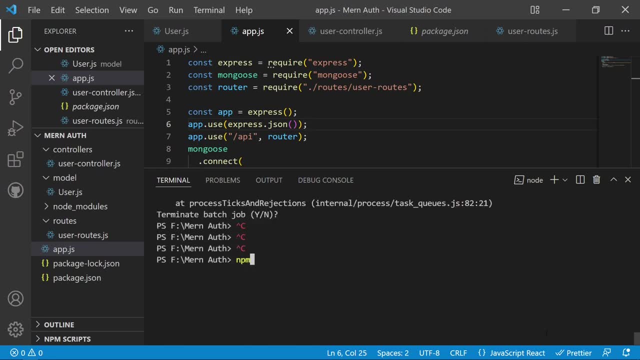 will provide your token and then you need to offer the services to this. so now we can generate the token. so for generating the token we need to go to the application once again and then we need to install a new package. it will be the json web token. so this package will help us to generate a jwt token to provide the access to the user and 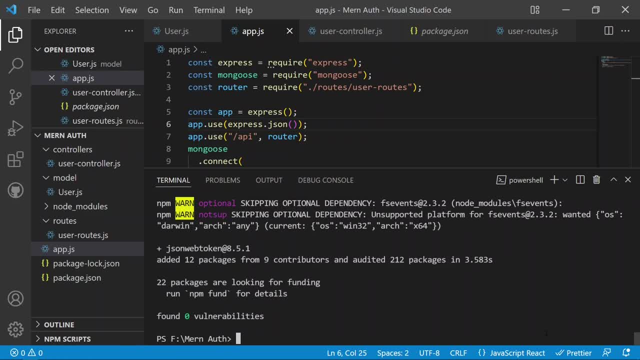 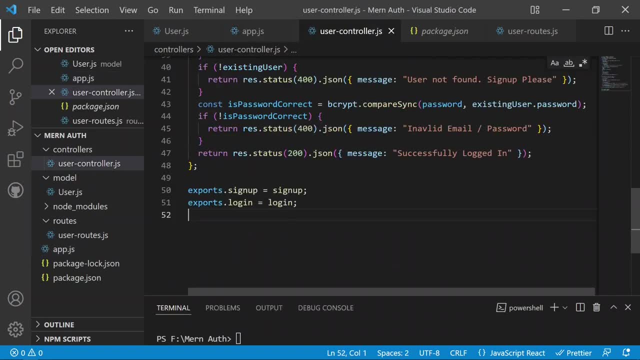 this token will provide access by encrypting the details like the id of the user. so now let's start generating the token for the user to provide the access. so now in the users controller, when we are declaring the login and when we are using the login. so after the password is correct, then we 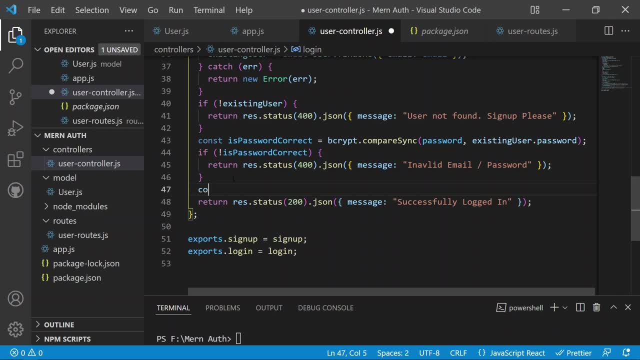 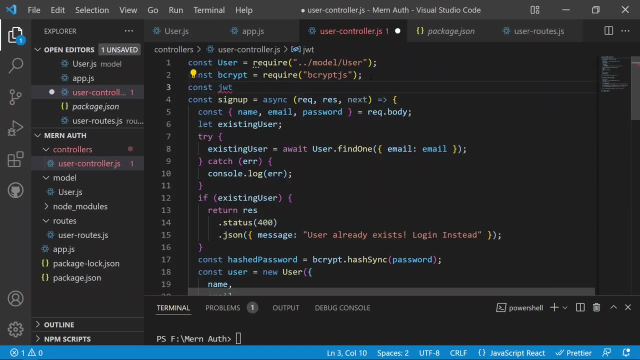 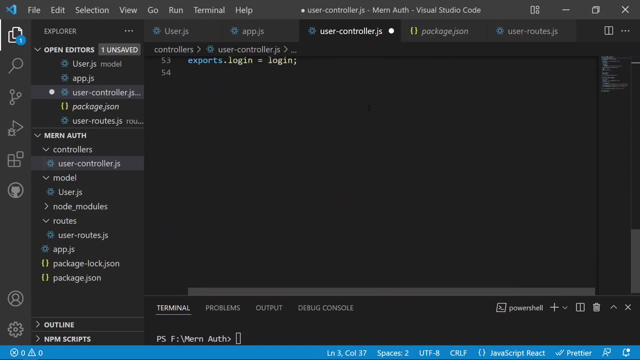 can generate the token to the user. so we can generate the token by just importing the json web token first. so it will be the const as the jwt and it will be close to the require, and the require will then contain a json web token. so now we have imported the json web. 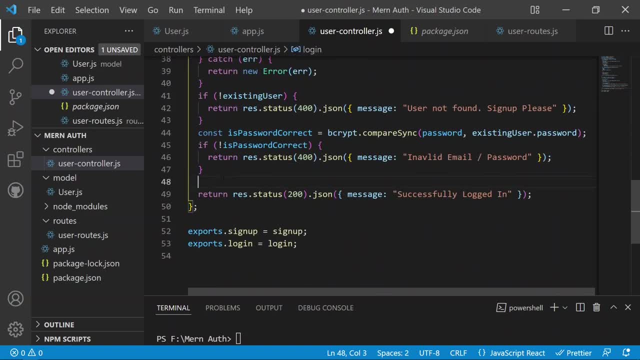 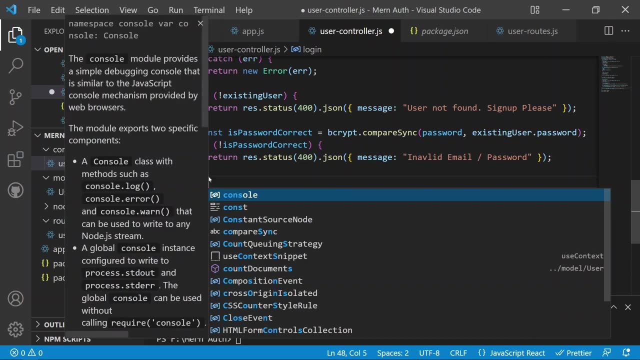 token. so now, after the user details are correct, so after everything is correct, so we can just generate the token. so now we can generate the token after the password is correct, so it will be the const as the token. so this is a token variable which we will generate, and then we have 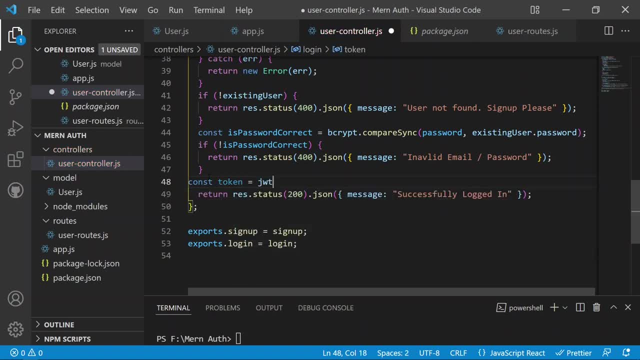 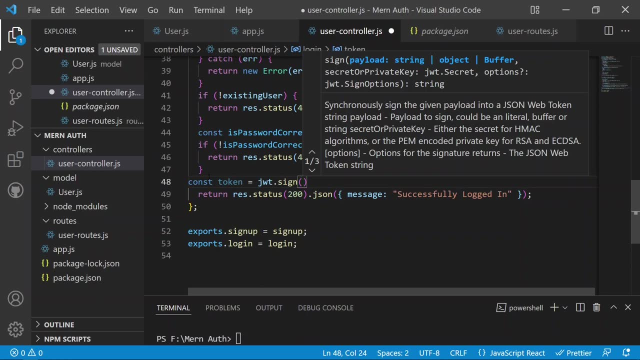 to generate the token and it is the sign. so it will be the jwt which we have imported, dot sign. so we have the sign function which signs the token to the user. so first, the first parameter contains a payload, which can be a string, an object, or it can be a buffer as well, so the payload. 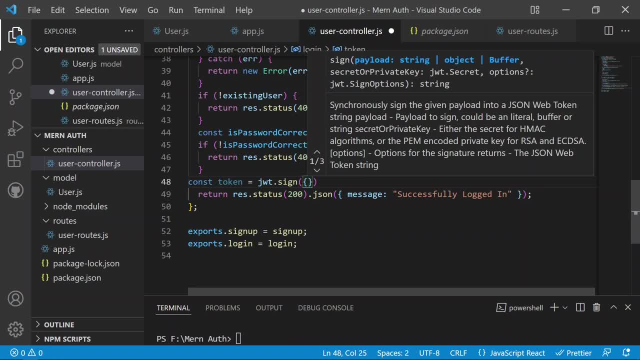 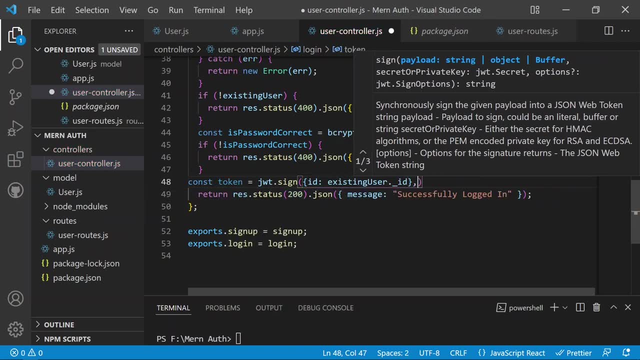 contains a data which we need to encode, so it can be an object in this case, like we can just encode the id of the user by providing the existing user dot id and the second parameter, zar vullássart called secret key. so this is very important, so we should have a secret key and 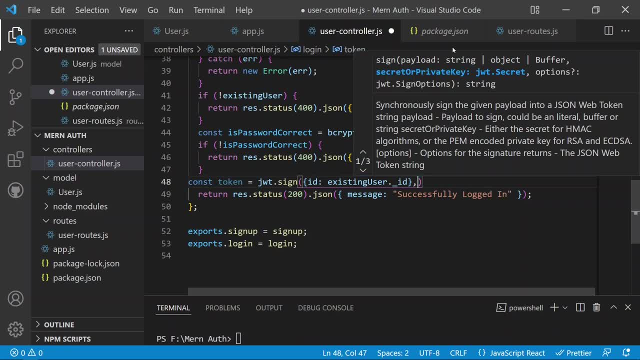 you need to make sure that this key is not shared with anyone. so this is a fully secret key which is used to encode this token and with this secret key, only then, we can decode the information as well. so you need to make sure that it is not accessible by anyone except you or the team. 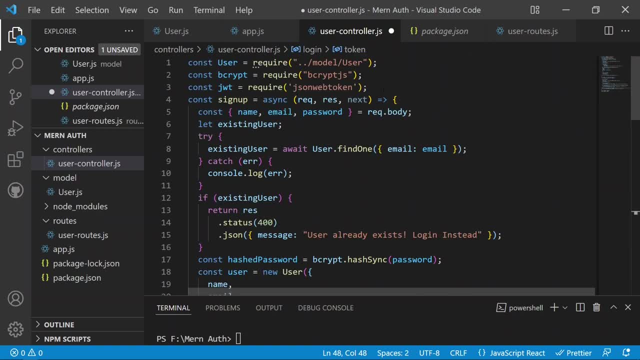 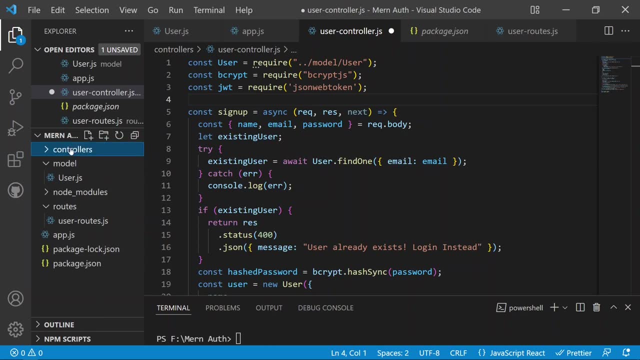 so it will be a secret key. so by default now we can generate a secret key at the constant here. but i prefer you and in the end we key in the environment variables by creating a dot env file. so we will store the secret key there. but for now, only now, we can generate a constant as secret key, like it will be the jwt secret. 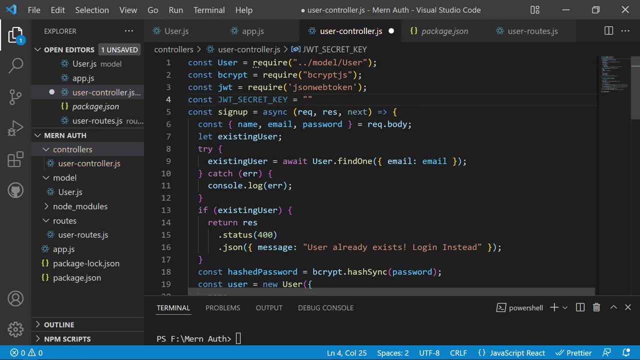 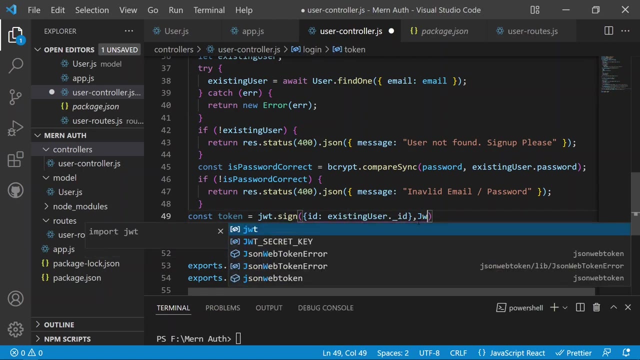 as the key and it will be equals to like secret key can be anything like it with the my key or anything. so in this case we can now declare the secret key as the my key. so there, after we are signing the user, then we can add the secret key as it will be the jwt secret key, and then we need. 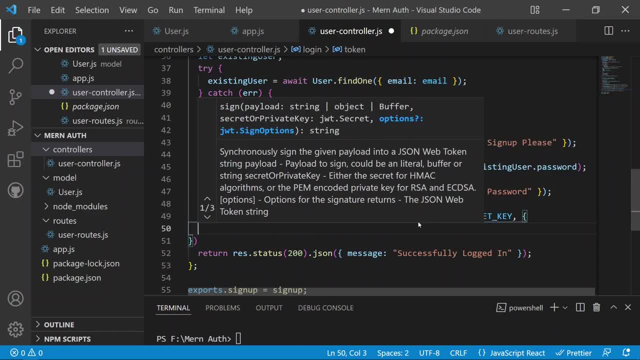 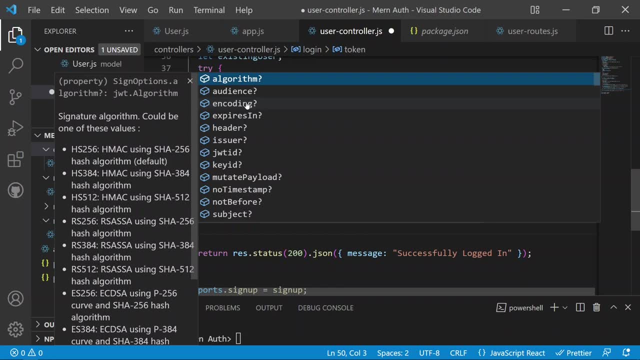 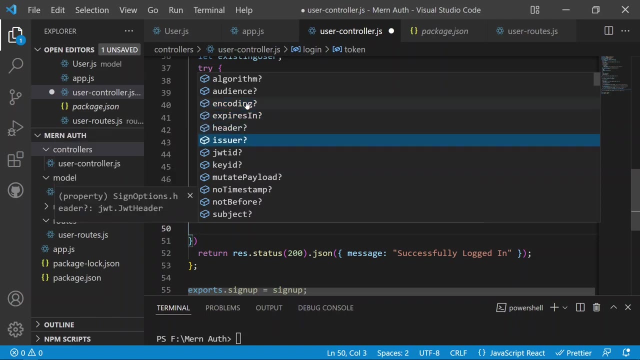 to add another parameter and it will be a object. and now we have some options like we can define the algorithms like hs-256, hs-384 and any algorithm. so by default it is the hs-256, so we can use that. and then we have audience, we have the encoding, we have the encoding properties like jwt. 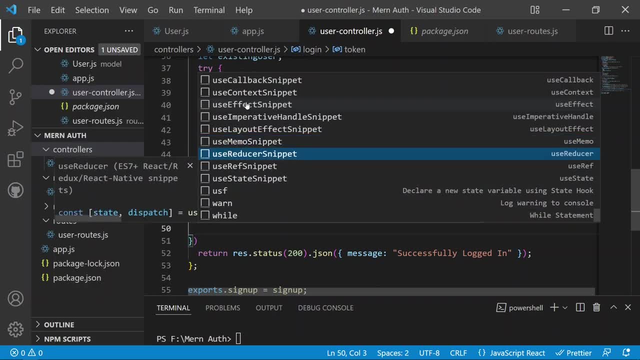 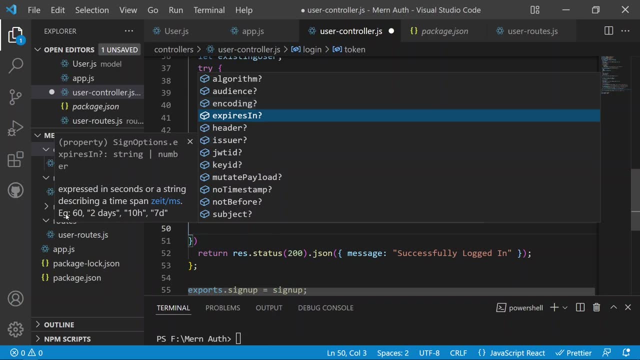 id, key id, and we have a lot of properties to use, but here in this case we will just use only one property which is expires in, and the expires in property you can see here like example equals to six t. like it will be a time span, it can be a two days, a 10 hours or the seven days as well. 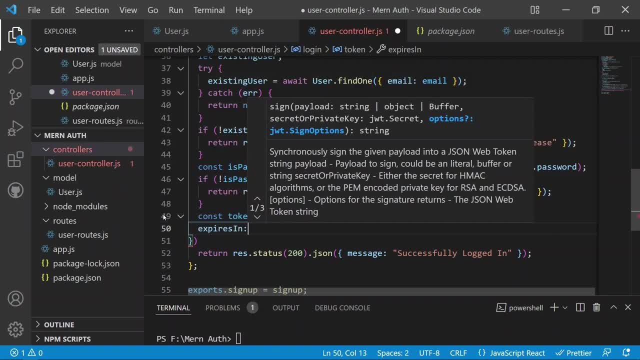 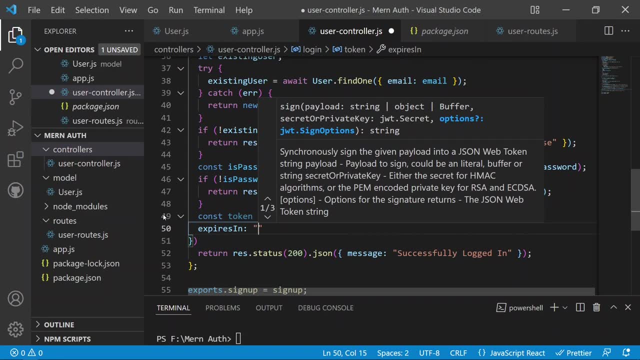 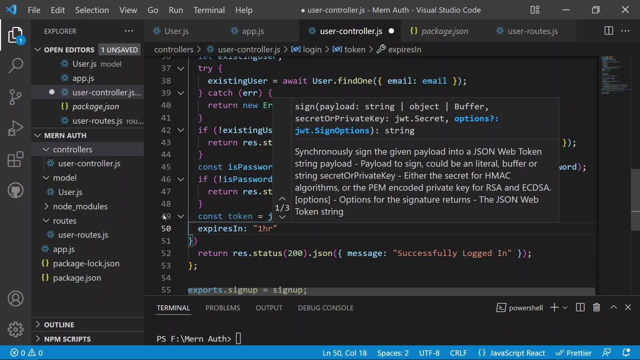 so this is the property expiring which we need to use, and the expires in property will define that after how many time span, after how much time the token will expire. so in this case we can just use as the one hour or the two hours or the three hours as well. so after that the token will expire. 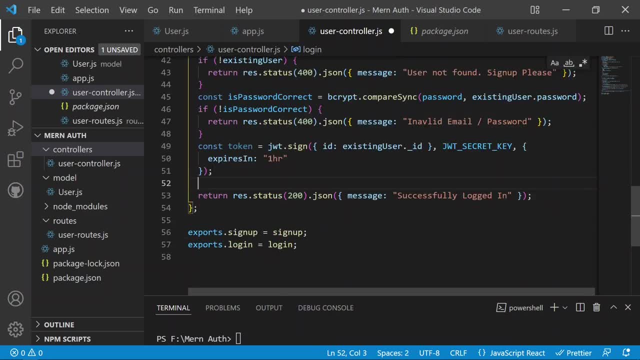 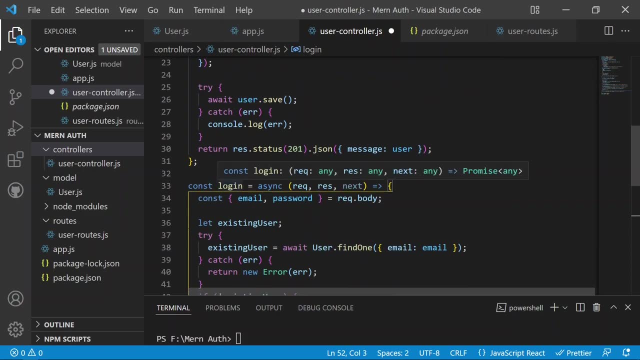 so then we can use this. expires in there. so now we have generated the token after the login, and then once we will get the information of the user- like we are now only defining the login route, but whenever we want to verify the token, then we can use another route here by defining here the user. 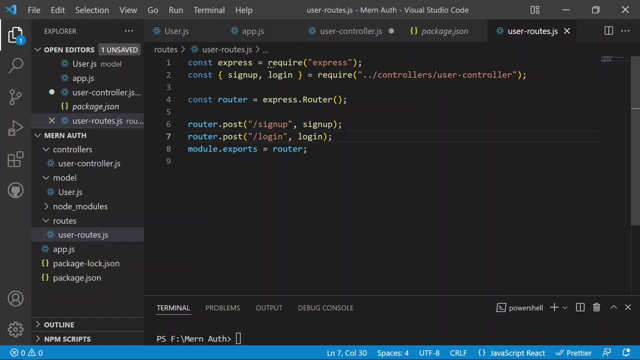 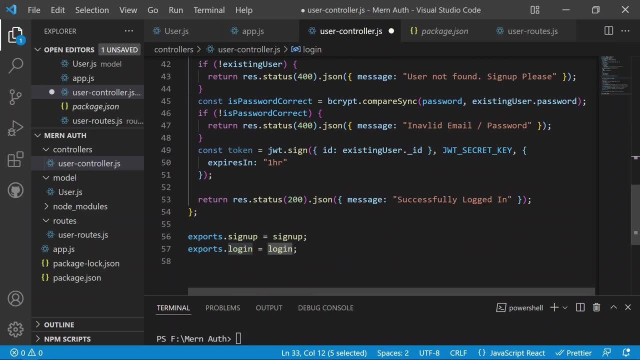 route in which we will send user their information and for that first we will verify the token which we are now sending here. so now we are sending the token and now we can just send the token. whenever the user will be logged in, we can send a message and then we can send the user as well. 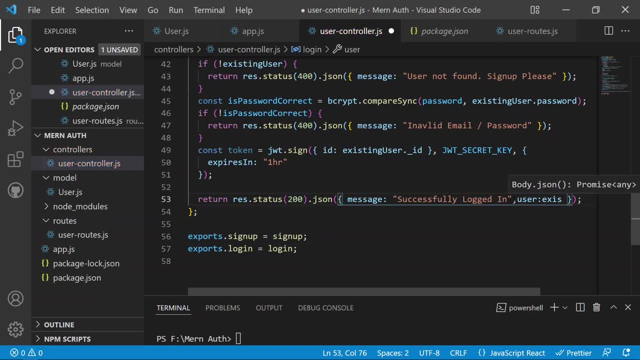 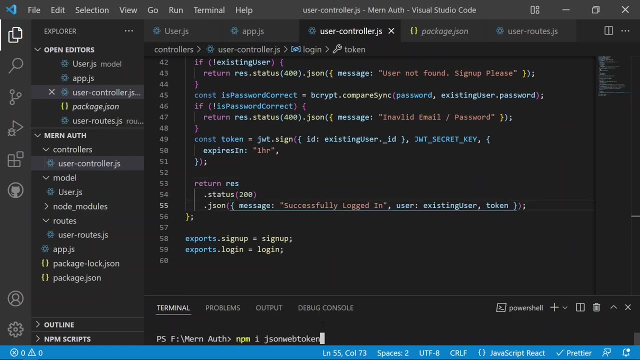 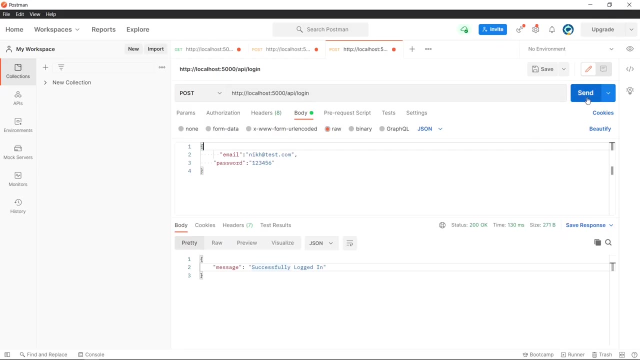 like the existing user. existing user is there and then we can also send the token as well. so if i will now log in again, so if i will now see if the token is sending or not, so we can start this server. like a database is connected and now, if i will now just send again the login request, 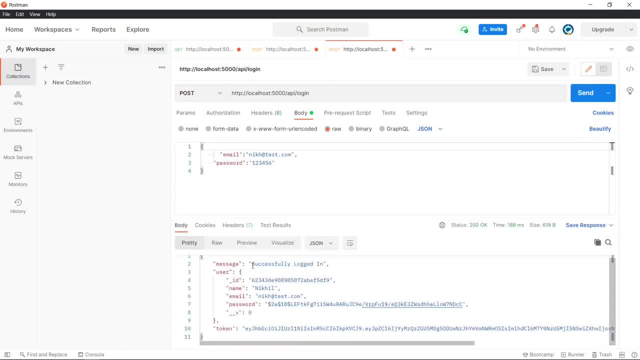 so now, you can see, now we have some information. now we have the message, which is called a successfully logged in, and then we have the user, and then we have the every details of the user, including the password, and then we have the token as well. so now this is the token, and it is very 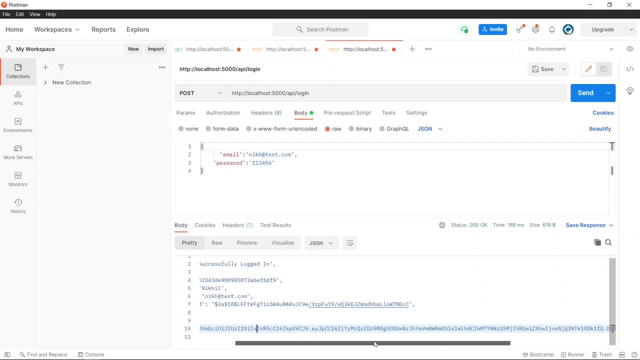 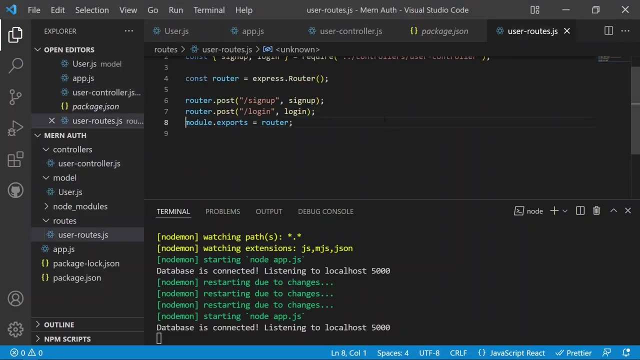 big token to just decode, then you will see this is the algorithm used as the hsa256 to just encode this token. and this token contains the id of the user, so it is encrypted id. so now we have the token after the login. and now where do we use the token to authorize the user? so we can just go to. 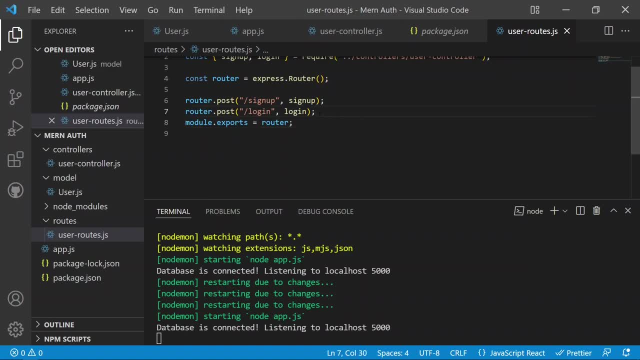 the user routes and then we can just declare another route where the user will ask for their information, like for example, the email or the password or for the name. so we can just declare a new route for the router at the routerget and in this get request user will ask for the information like slash, it will. 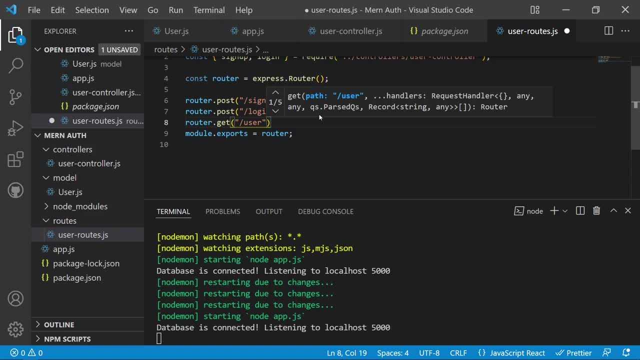 be the user. and then here there is a tricky part, like here: we need to first verify the token which we have sent through the login, so to authorize the user now we have to just access the token of the user which we have now sent. so we need to provide the access token to every request after. 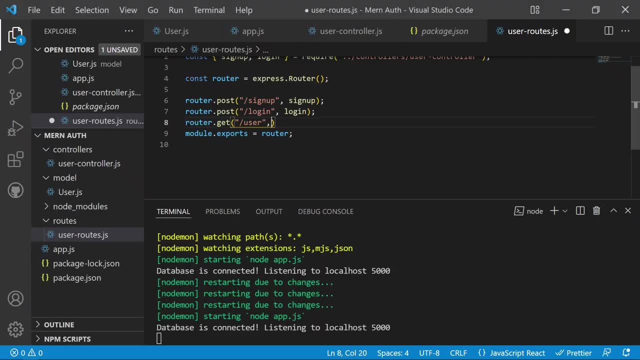 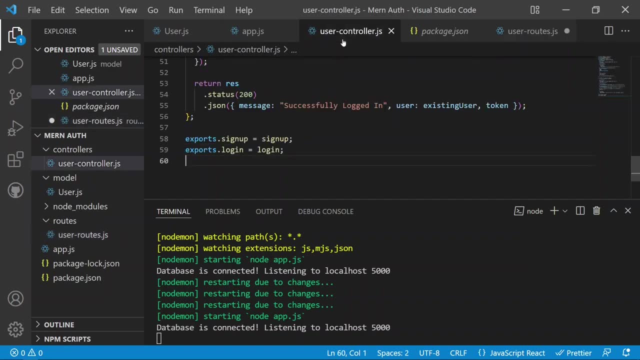 that. so we need to then verify the token, and then we need to verify the token and then we need to just share the information to the user. so first there will be a new middleware as the verification of the token, so we can just create a new function after that. so it will be as a cons as the verify. 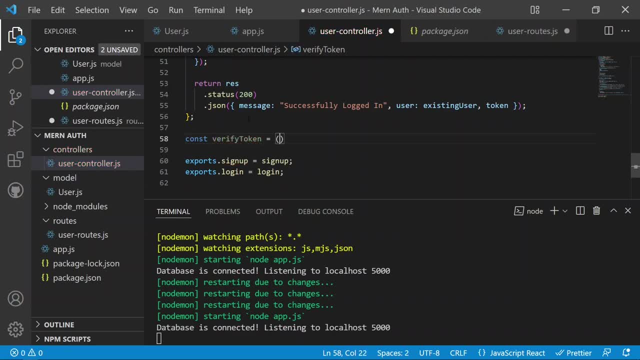 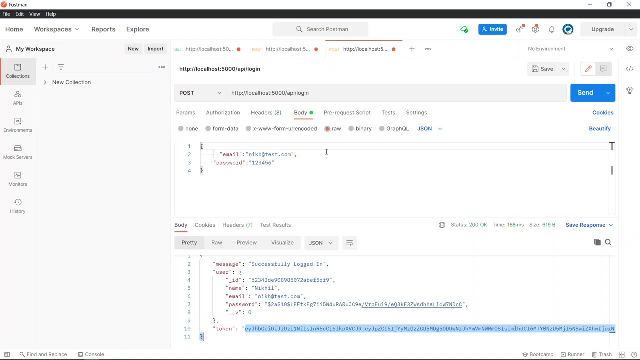 token and it will be construct the request and the response and the next, and then this will be an arrow function once again and this will act as a middleware again, and then we need to send the token. but now how we can send the token and how can we just get the token so we can send the? 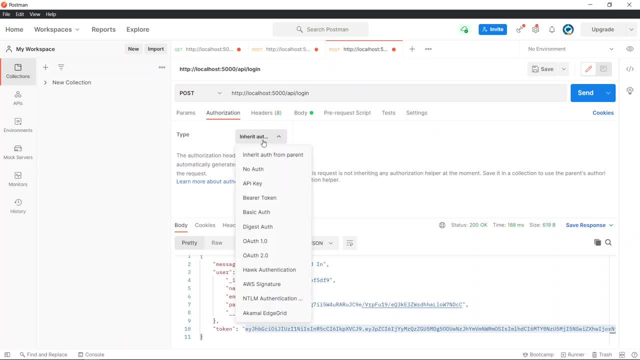 token. and now in the authorization tab here now we have some types so we can just select the types and then we can just select any of the type. but in this video we will go with the beer token, so we will send a beer token with that. like we have the token same. it will be copied there, so we need to. 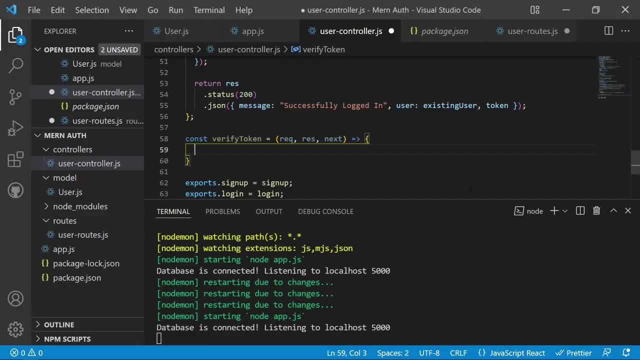 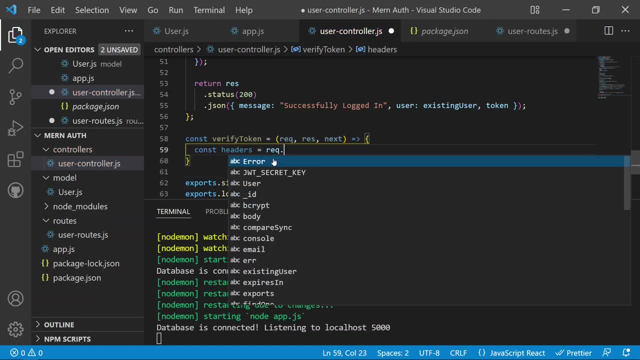 remove that. so we will use the beer token with that and now to access that we need to get the token. so it will be like the const as the headers and it will be equals to the request dot headers we have. so it will be the authorization. so the spelling should be same as the authorization. so 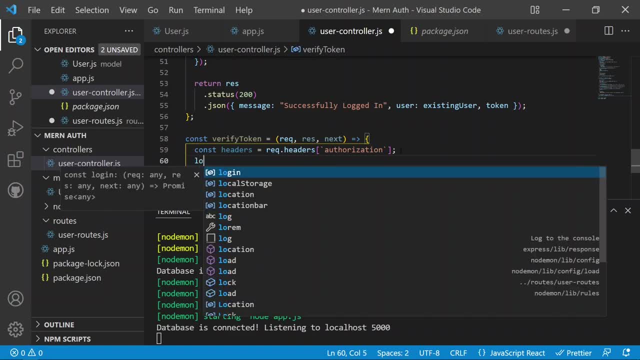 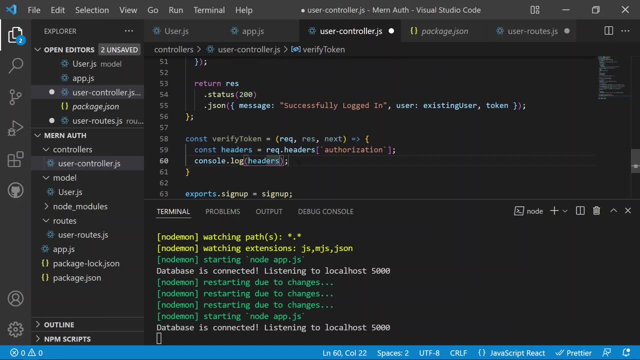 now you can see. now we have the request: dot headers authorization. so if you will just consolelog the information of the headers, so then now you will see. so i am now just consolelogging the information and then we will now just exports dot as the verified token and it will be equals to the 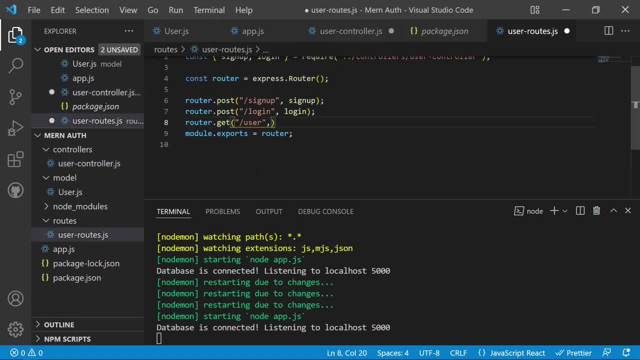 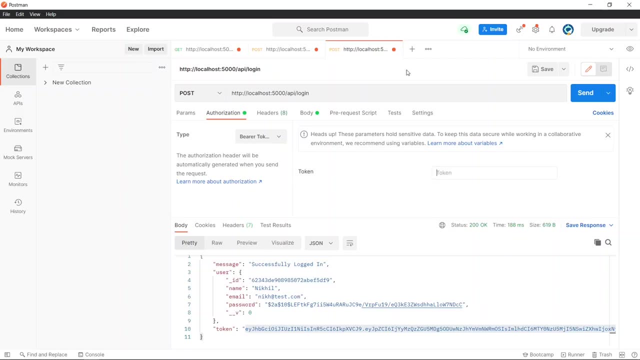 verified token once again, and then we will use that same into the user routes as the verified token. first for now we are using only the verified token. so now i am sending a get request from there. so the url should be the same. so after the login it should be the user. 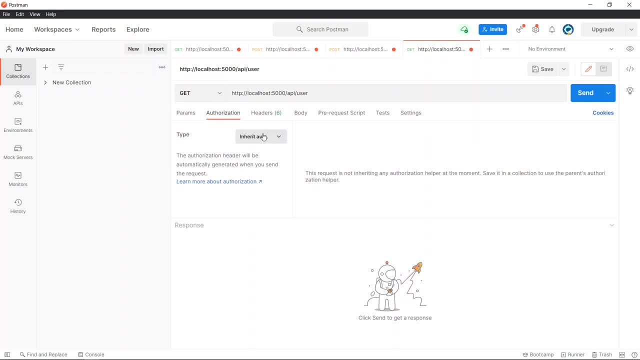 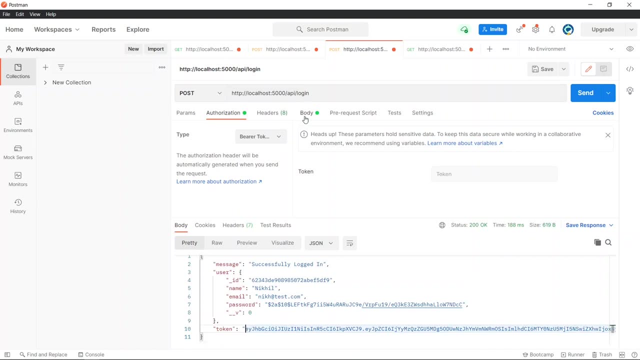 and then it will be a get request and then we need to select the authorization and then we need to send the bearer token and for the bearer token which we have received the token from after the login, for only this user, for only nickel at the rate testcom. so so this token is only valid for 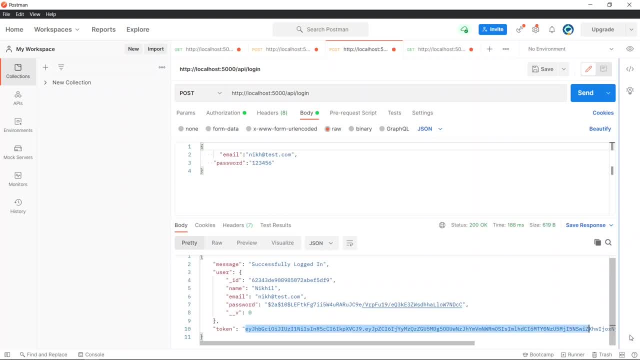 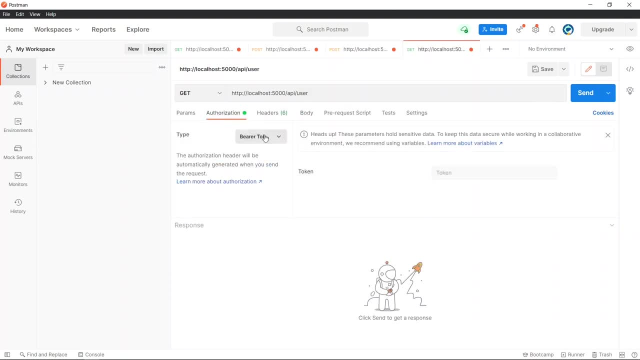 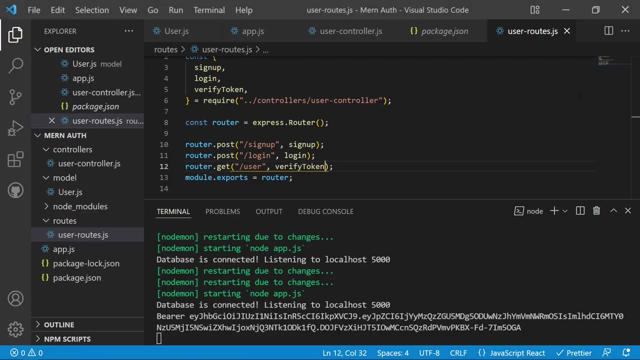 email id. so then we can just use this token- so i have now copied- and then we need to go to the get request and then we need to select the authorization, select the bearer token, and then we need to paste the token here and if i will not just send the request there now, you will see. now we have the token, which we have now. 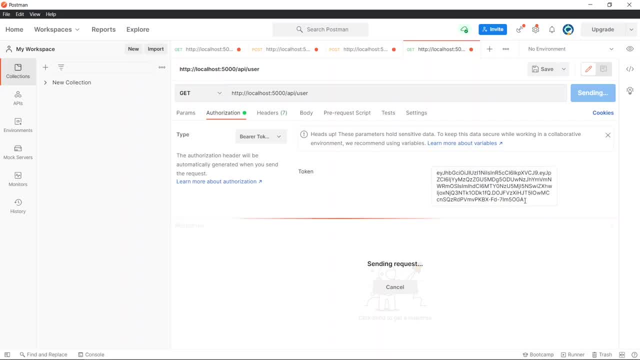 sent and it is the same token. now you will expand, you will see, in the end there is a 5 o, g, a and we have the same token here. and then we have a bearer in the front as well, because we have a bearer in the front as well, because it's a bearer token. so now we have the access to the. 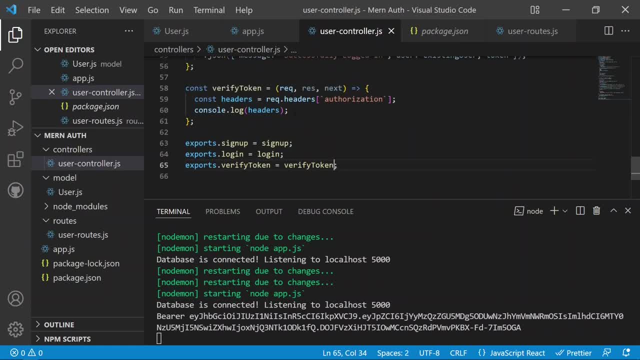 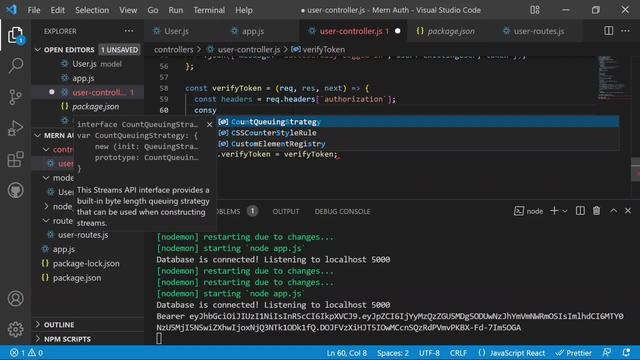 token and now we need to verify the token. so after that we can just verify the token. so we can just retrieve the token from this bearer token by just splitting the token. so it will be the cons token and it will be equals to the headers and it will be dot split. so we will just split. 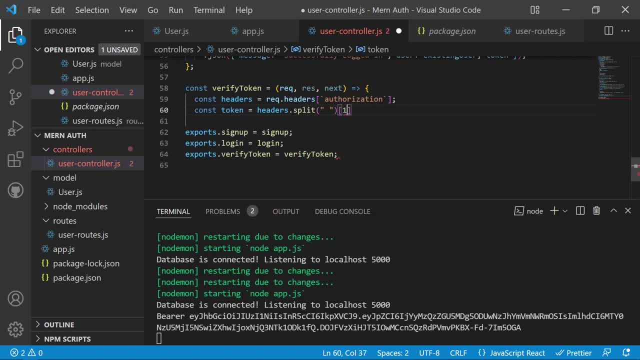 the headers into the space and then we will access the first number index from there. so we need to access the token. so it is a zero index, it's a first. so this splits just splits the string into the arrays, and then we are now sending the arrays at between the spaces. so it will be acted. 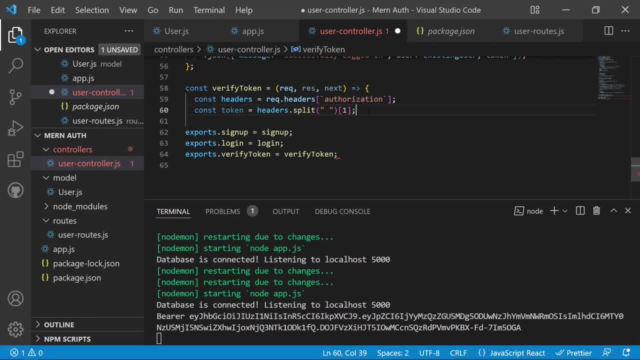 as a two arrays bearer and this token, and then we are extracting the first index element and then now we have the token and now we need to verify the token. so it will be so we can check, like, if we don't have the token, so then we can just send a request as the response. dot status as like the. 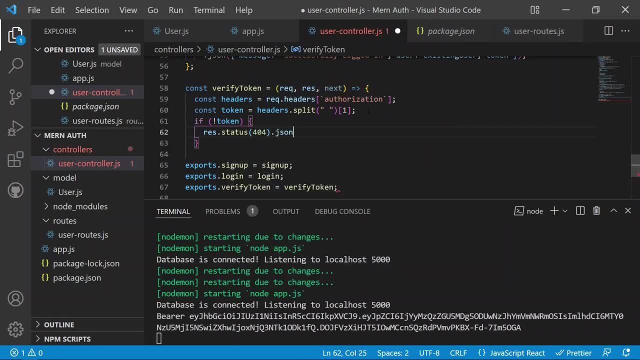 and it will be dot uh, json. it will be like the message, like the string: it will not token found and then after we have the token, and then only we can just access the user. so to verify the token, we have a function again in the jwt to verify the token. 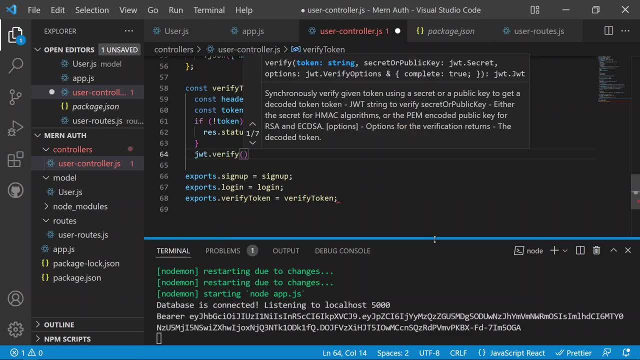 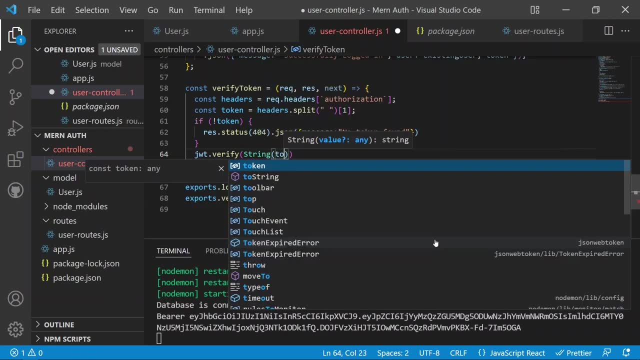 and it is a jwt dot- verify- and then it is a verify method. so we need to add the token, so we can just convert the token into the string, so it will be the token and then we can just use the token there. so after that we need to provide the secret key. 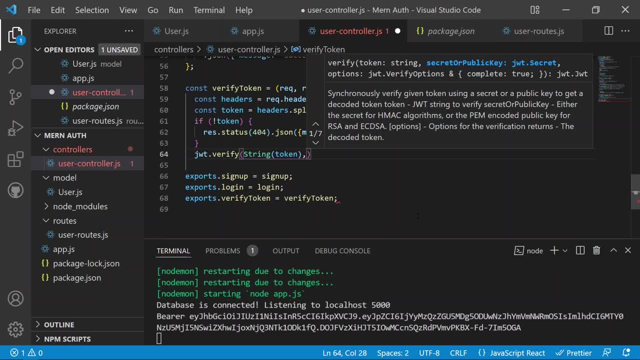 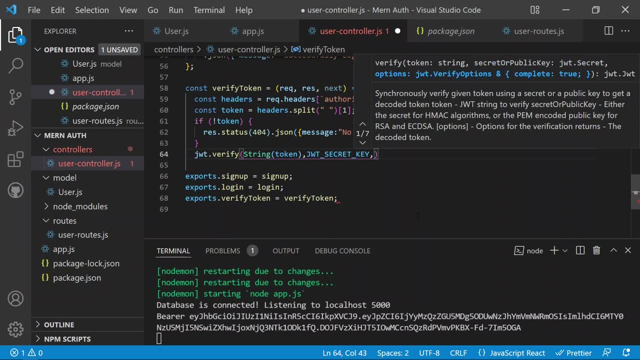 again, which we have generated there. so we have generated the constant as the jwt secret key. so then now you will see, now we have the token, and then there can be a callback function after that, like completed or not. so we can just generate a callback function. so the first parameter is the 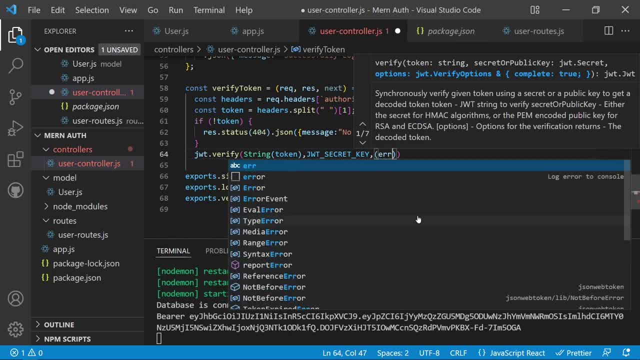 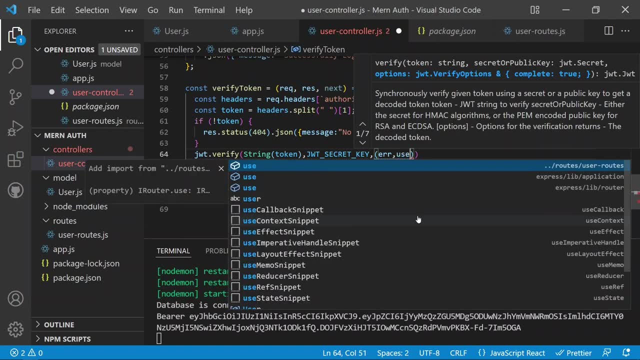 error. so if there is error in validation of the token, if, like, the token is wrong, and then we have the error, and then we have the information like decoded information, so we can use the decoded information as the user, because we have uh generated the user id with that so we can just 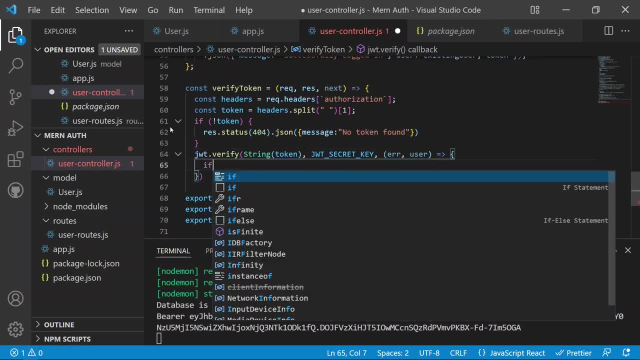 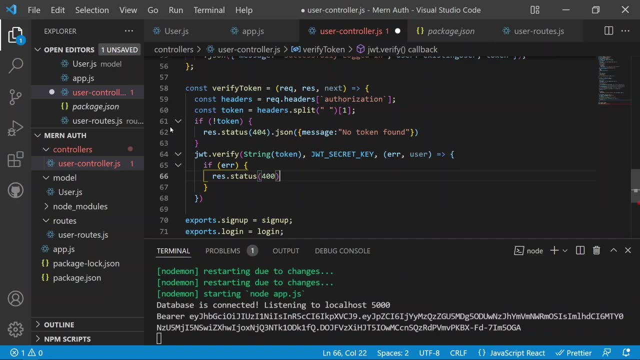 give you the arrow function after that and then if there is an error and then we can send the message at the response dot status, it will be caused to the 400 at the unauthorized and the json which contain a message inside. that message can be like invalid token. 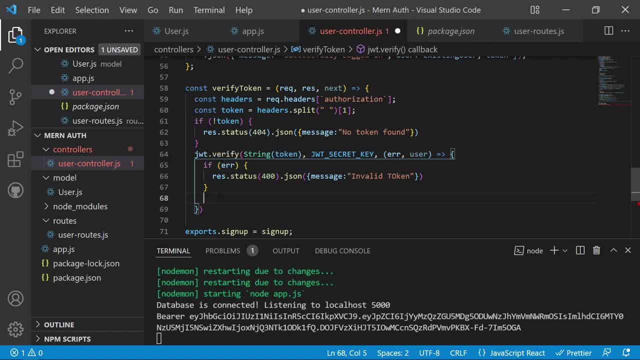 or after that, after we have sent the request there, and then we have the user. if it is not there, so we can just return here as well. so if it is not there, so then we can use the user. so now we have the user which have the decoded information. so if you will just consolelog the 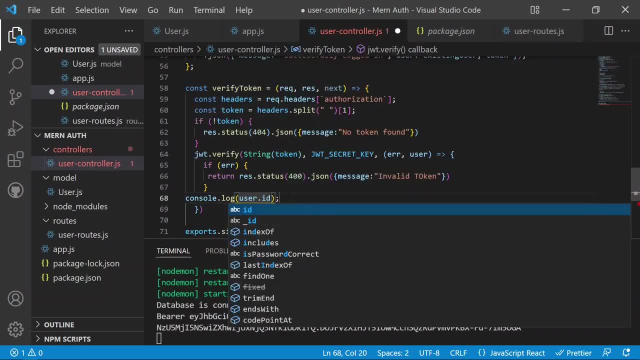 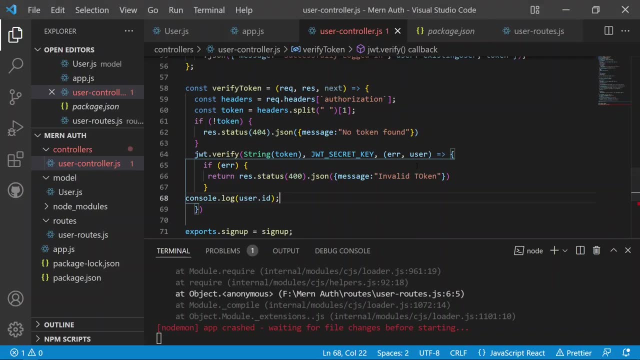 user there, userid which we have then, uh, encoded into that. so if you will just consolelog and then you can try again with that, so if i will now send the request again, so i think there is an error. so now you will see, now we have the unexpected end of inputs, so i think there is an. 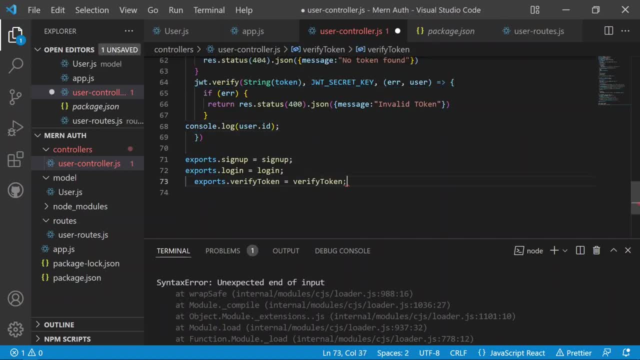 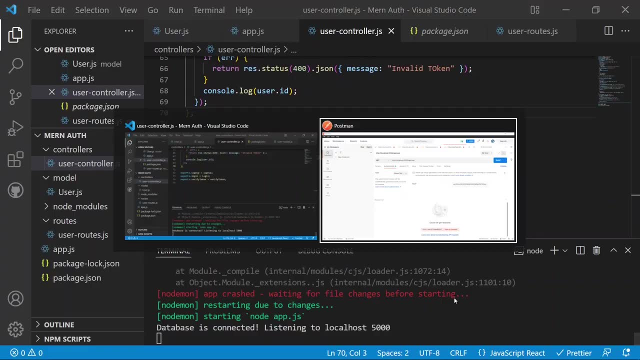 error, because now we have now generated exports or verified token there, so after that we need to just add a release there. now you can see, now the application is started and then we can just generate a new get request. so click on send request now you can see, now we have the database. 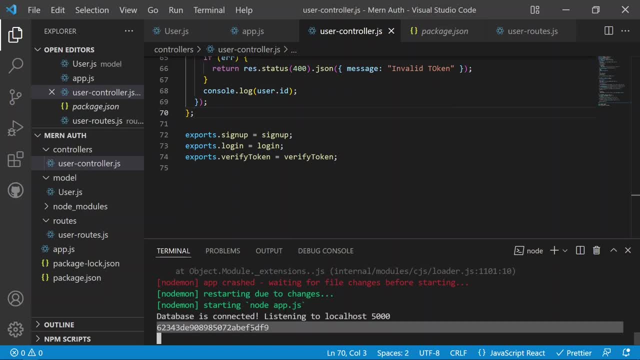 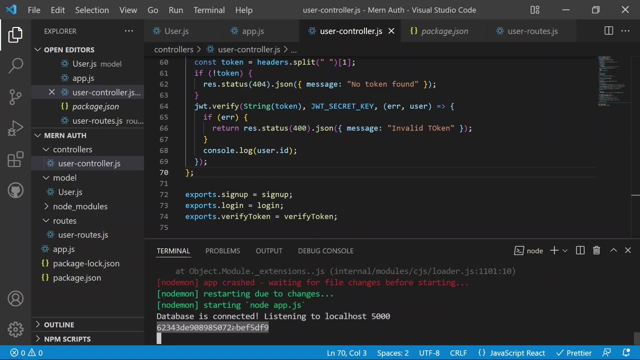 is connected and now we have the id of the user. so now we have now verified the token, and now the token is correct, and now we have the id of the user and then we can just move on to the get user and then we can generate another. 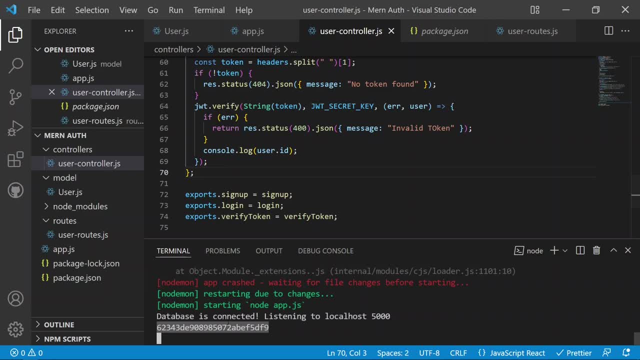 middle function to get the details of the user from this id. so now we have successfully decoded the token from there and then we can just get the id of the user by going to the user routes so we can generate the new route after that. so it will be the cons at the get user and it will be equals to. 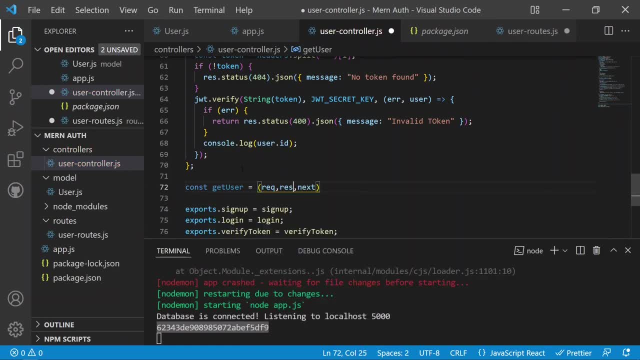 the request response and the next, and it will be a asynchronous task and then it will be a arrow function. so before that we need to send the id of the user to this middleware. so for that we need to just send here the request dot id so we can generate any of the parameter, any. 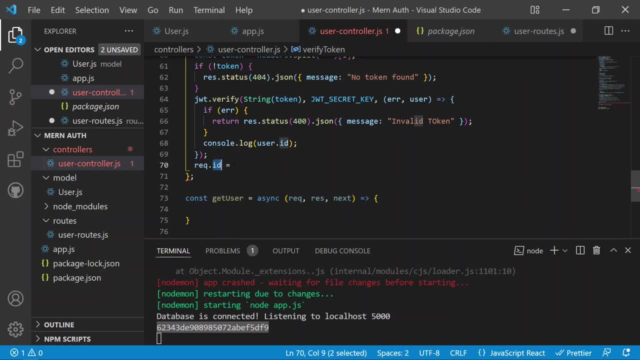 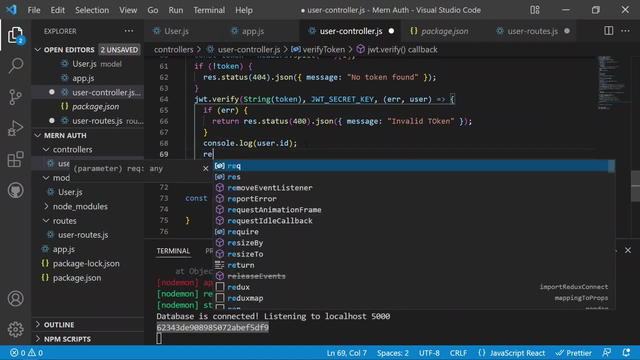 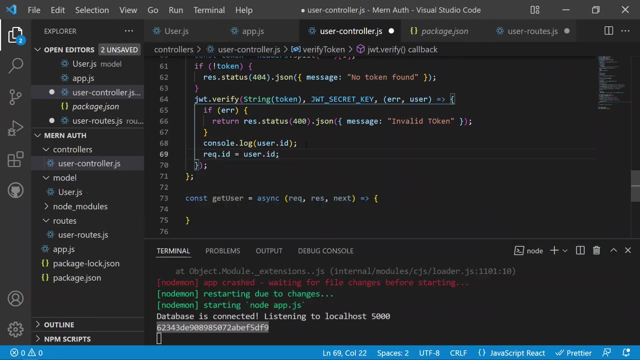 of the name or variable with that, with the request object. so request dot id. i will provide here the user. user will be there, i think. so it will be the user request dot id. it will be the user which we have now decoded dot id. so we have now sent the request dot id as the user dot id and then we can. 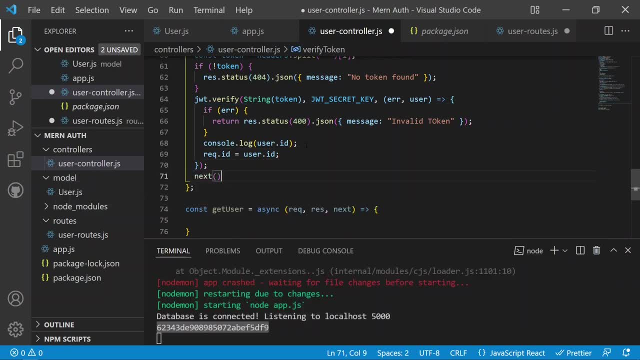 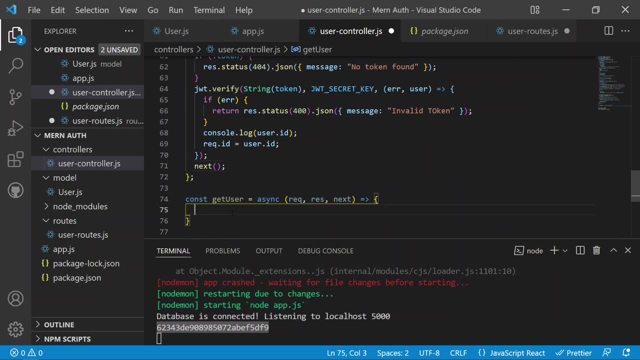 just move on to the next middleware after that. so we have now sent the request dot id as the user, so we can just use the next middleware and next, after the authorization, after the verification is completed, and then we will move on to the get user function so we can just get the id of the 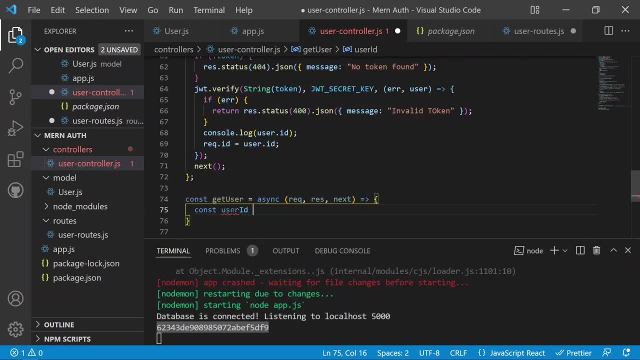 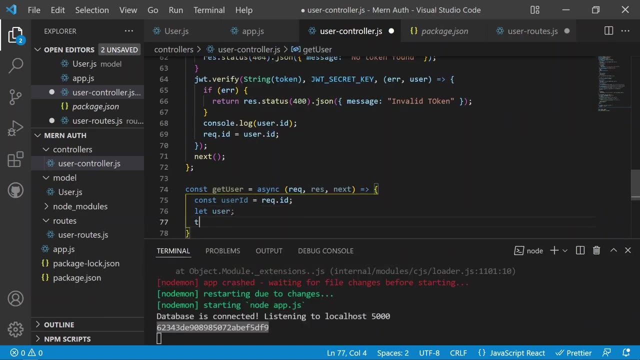 user from the const as the user id and it will be also requestid, which we will receive from the parameters from there, and then we can complete this by generating a let as the user and it will be like the undefined by default, so then we can just use the try catch block once again. 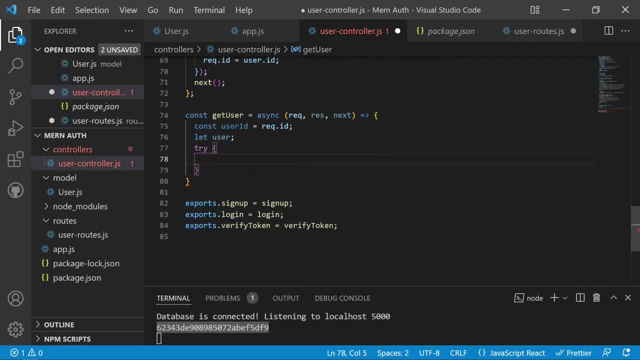 so i will now expand this. so now we have the try catch block and then we can generate, as the user will be equals to await, and then the user. we have the model of the user dot find method, so we will find the user by its id from the find by id method and then we can generate the id and then we can. 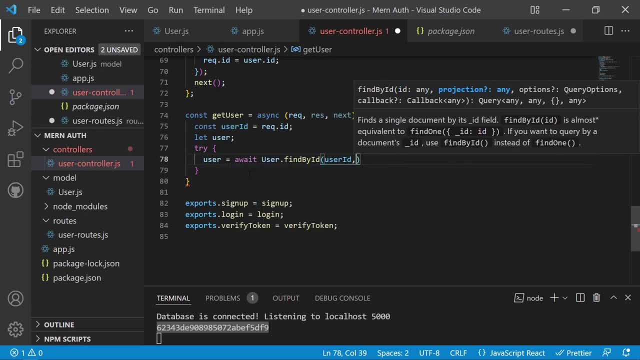 just send the id which we have got from the requestid, and then we need to get all of the details instead of the password. so we can use here the minus sign and then the password. so it will be like the undefined by default. so we can just send the id which we have got from the requestid. 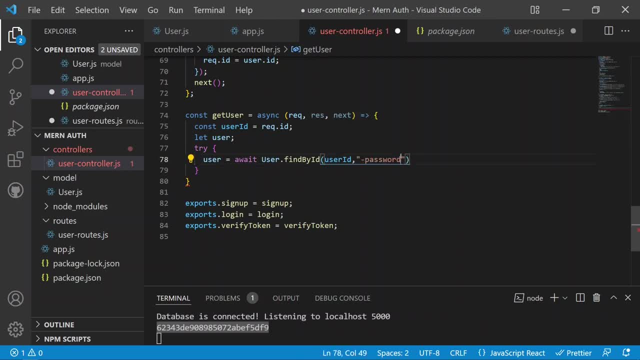 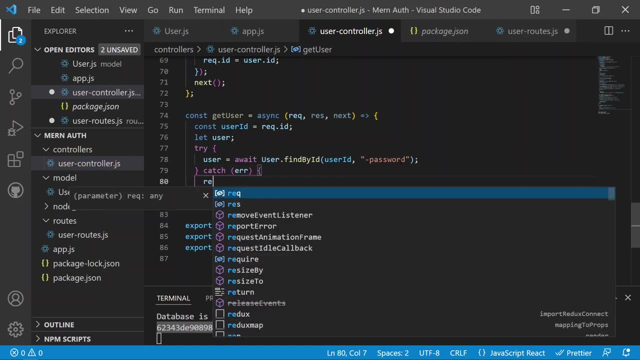 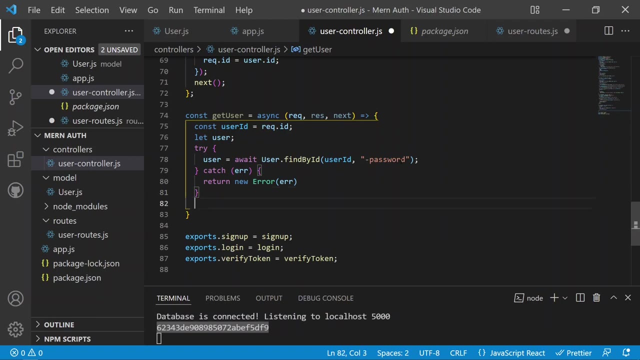 will just remove the password field and it will send all of the data of the user from that. so now we can just get the user and then we can use the catch block also if there is an error. so we can just return new error as the error in that. and now we are using try catch block and then we can. 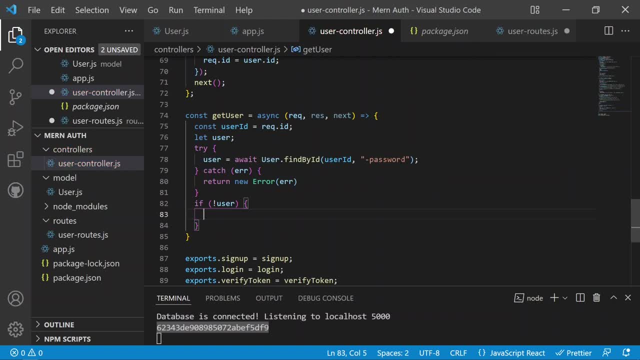 just validate again, like if we don't have the user, and then we can just send here as the response, as the return at the response- dot status again- and it will be like the 404 because we don't find the user, and then we can just send. 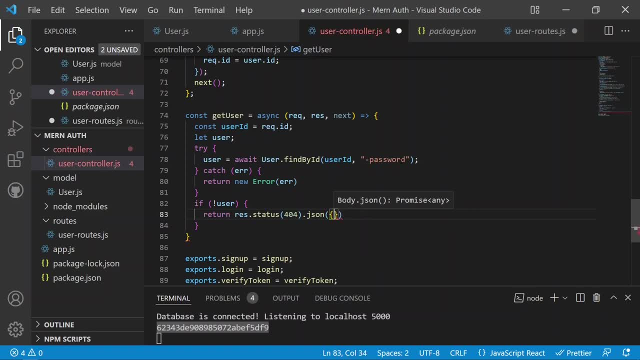 the json once again like: uh, it will be the message as the user not found. so now we are sending the message after the validation and then after everything is fine, so we can just return as this response: dot status and it will be the 200 and then dot json. 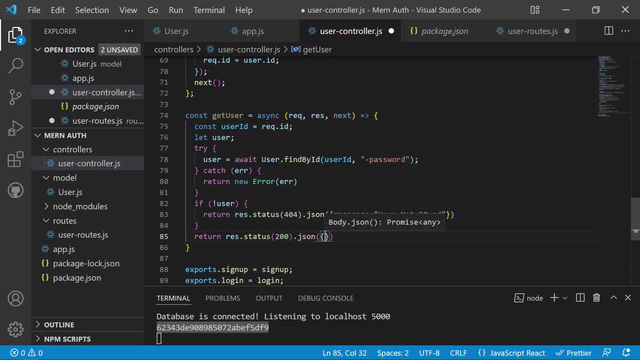 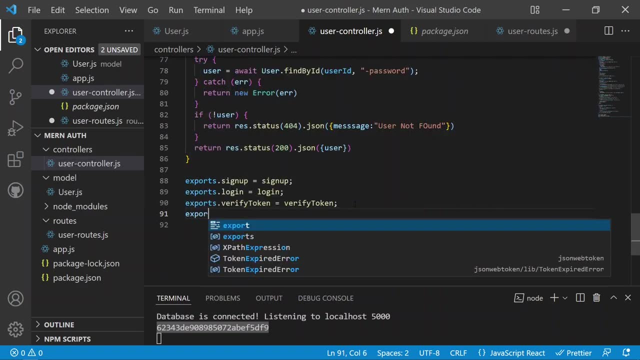 we can send the user, so it will be dot json and then we can send the message as the user only. so now we are sending the user. so if i will now just export this as well, exports dot we have now get user will be close to the get user function once again. 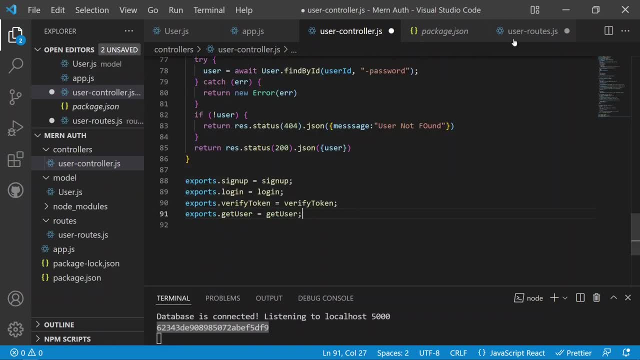 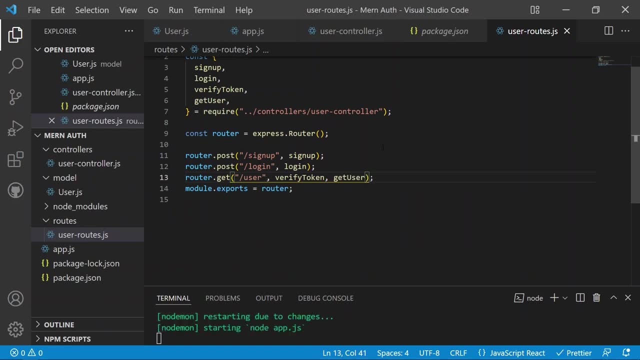 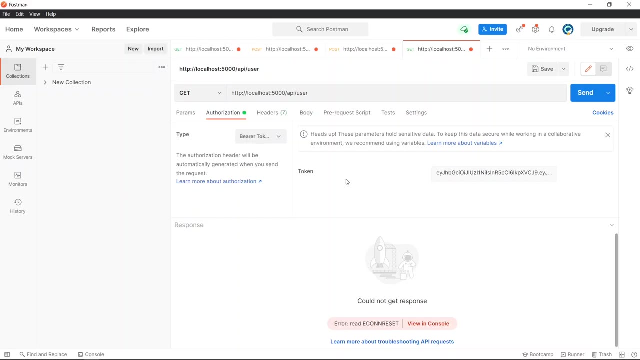 so then after that we can now use this in the user routes and then we can generate the, so we can just get the user route by the get user. so now we have exported that and then we have imported there. so after the verification of the token, and then we will move ahead to the get user with 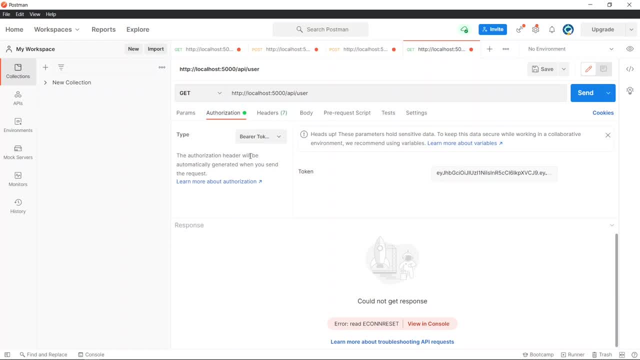 the next function and then we will get the details of the user. so now we have provided the authorization again, because the validity is one hour. so if I will now just click on this end, now you can see, now we have the information of the user. so now, because we have decoded the token, we have now got everything and now 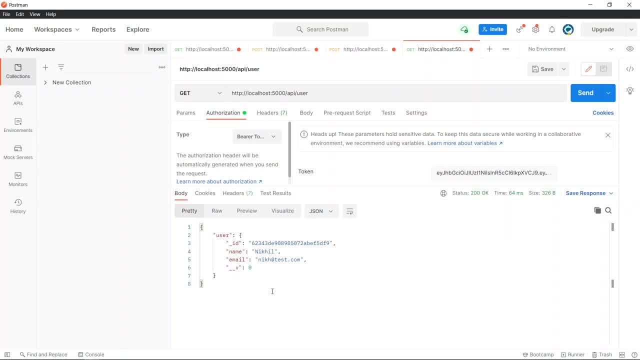 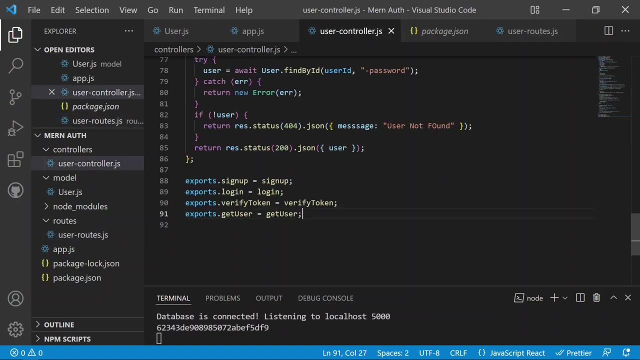 we have completed all of these steps in the JWT and now we have our fully secure application. but one thing missing, which you will see later. and then now we are getting the user object with its ID, with its name, with its email and everything instead of the password, because now we have now excluded the password from the 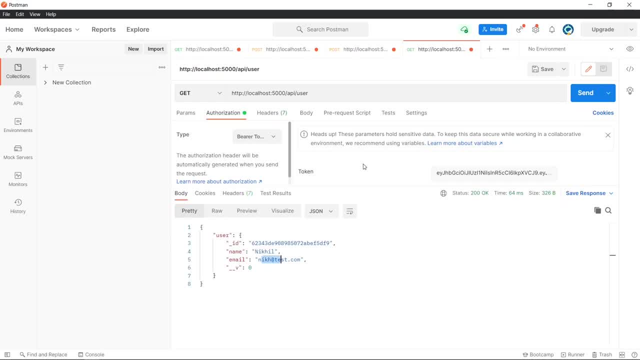 user controller. so now we have provided everything, and now everything is working perfectly fine, and there is something which you need to know. so now we have completed the JWT part, and this is the way in which modern applications are created, so they just encode the information of the user. 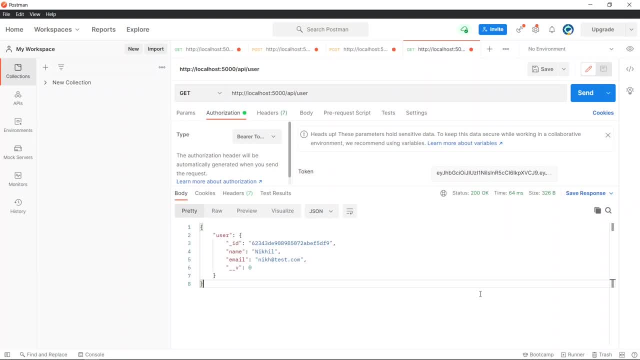 like that. so they just encode the information of the user like that, the id or anything like the user id, the user's id, user's email or anything with the jwt token, and then they decode it and then they try to get their information from it and then they will get. 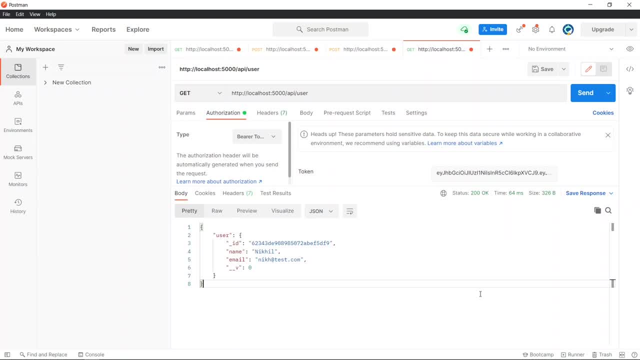 the information and then they will retrieve the information to the user. so this is how the modern web works. so now we are providing the token for every request, and it is a very good approach, and it is a modern approach as well. so we can store the tokens into the local storage of the browser. 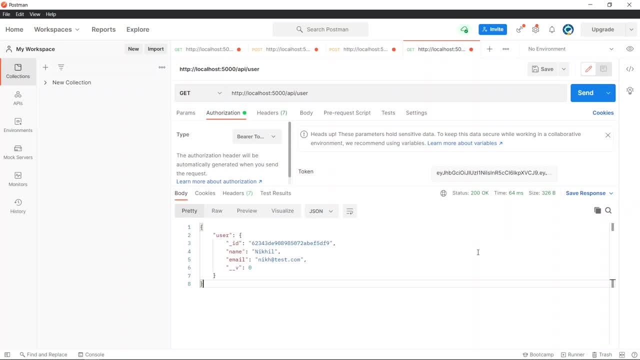 or into the sessions, or into the cookies, or into the memories as well. but is this a good solution to store the token in the memories in the browsers where all of the javascript code can be accessible to you via the developer tools? so is this a good approach? but then where can we? 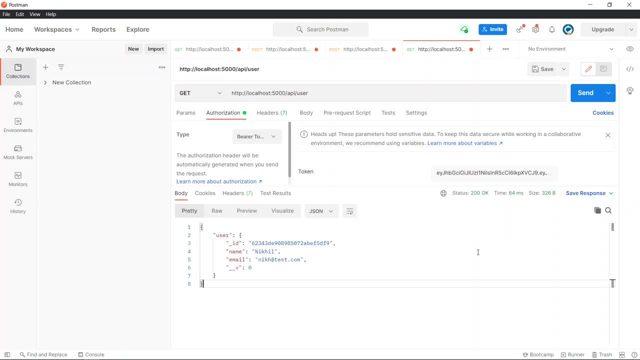 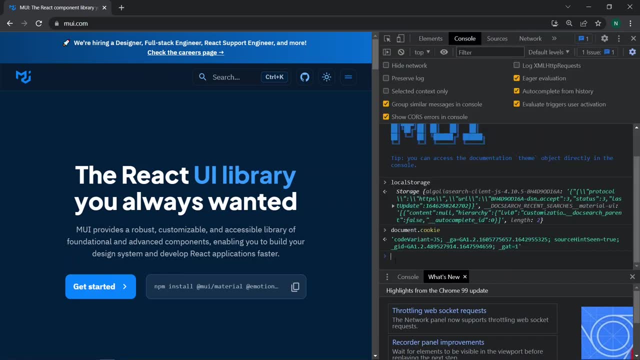 store the token in the front end. so if you will store the token into the local storage- so i am now currently into the material ui website- so if you will check the console now, you can see. if you will just click on the local storage now, you will see. now you. 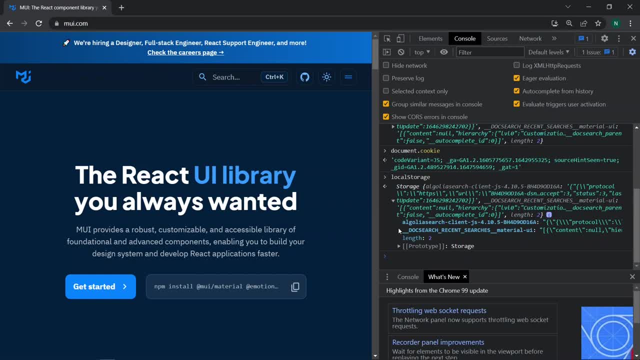 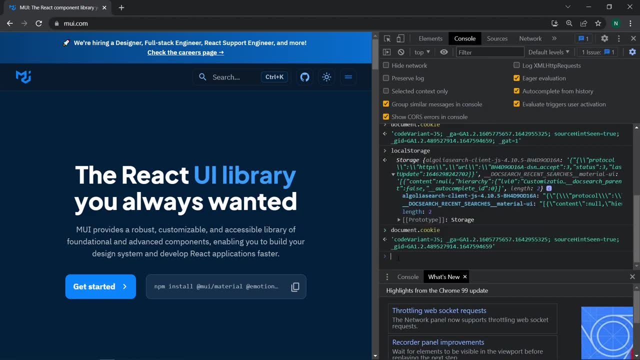 have accessed the local storage of the browser and then if you will store the token into the cookies, like it will be document dot cookie, so the cookies will also be accessible to you, and if it is accessible to you, then it can be accessible to any hacker as well, so you can go. 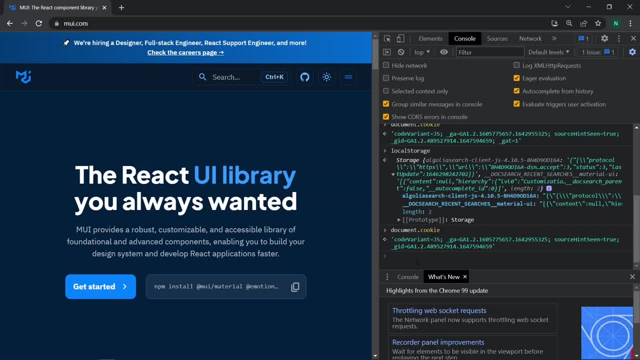 to developer tools and do certain things with your application, and it can break your application as well if any hacker will steal your token. so here comes a new topic. so are you getting my point? so where can we store the token? so in the modern web applications we also have a new threat called the. 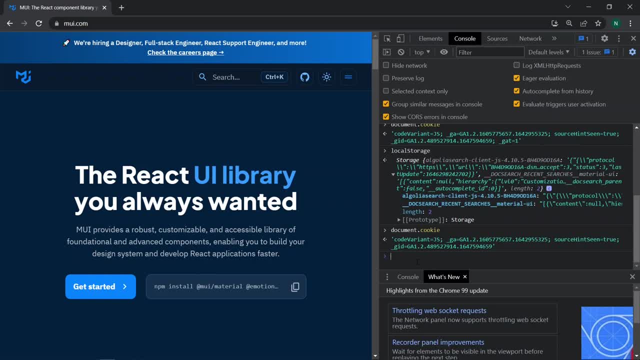 xss attacks, which are the cross-site scripting attacks, where the attacker or the hacker adds a script to your application and pretend to be you and it can steal your access token and then can do plenty of the things which are not good to your application and then the application can be. 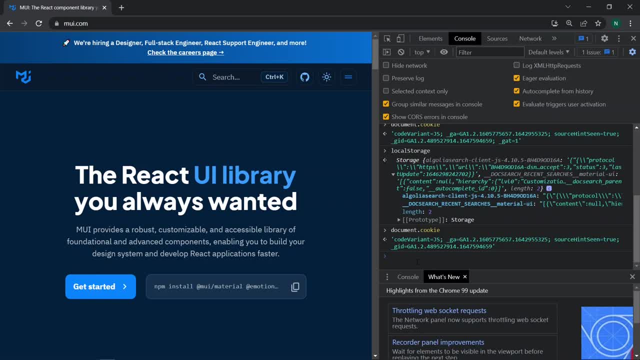 hacked and then it will be bricked. so this is a big problem. so where can we store the access token if we have the hackers onto there? so the solution is we have- we still have- a solution- is we can store it in a cookie. but wait, the cookies are accessible to the browsers, but this cookie will be made from the. 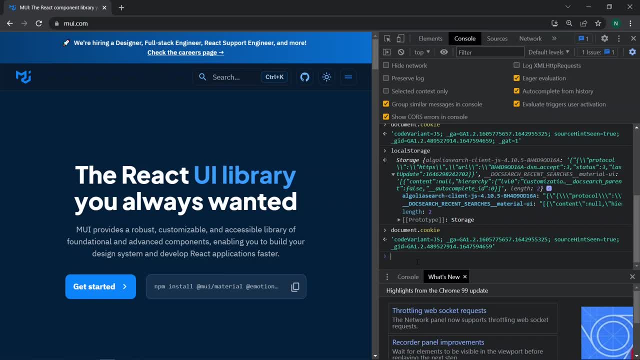 backend and it will be an http only cookie, and i have done a lot of research on this before creating this project and i came to note that storing the access tokens in the http only cookies is the most secure option to secure the web applications. but how does all this work? so we have a solution which is: we have a solution which is: we have a. 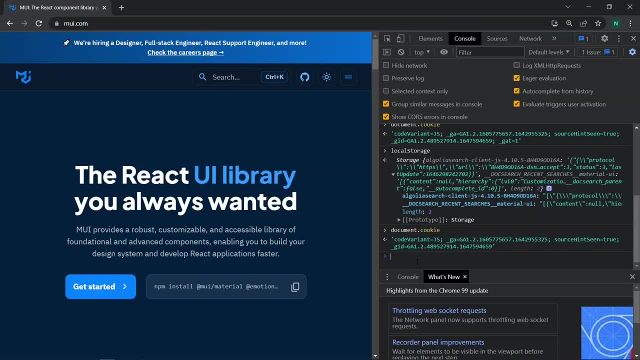 cookie that works. so we store a cookie from the back end, not from the front end, and we store a cookie from the back end and then we will send it to the front end and then the cookie will not be accessible to you. but still a problem that if it is not accessible to you, then where do we send the? 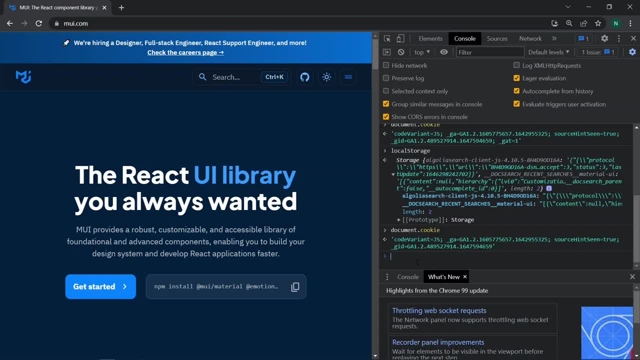 access token. so in the front end, whenever we are sending the request, we will send the request from the xeos. so the xeos provides us a way where we can send back the http only cookie which we will receive from the back end, to the back end again. so we will receive a http only cookie from the. 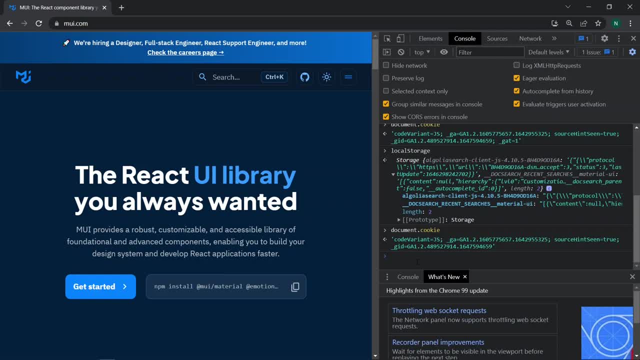 back end to front end and then after every request after that. so there is an option in the xeos so we can just send back the same cookie again, but it is still not accessible to you. so it can be a very good solution: storing the http only cookie and getting the key back from the client and then 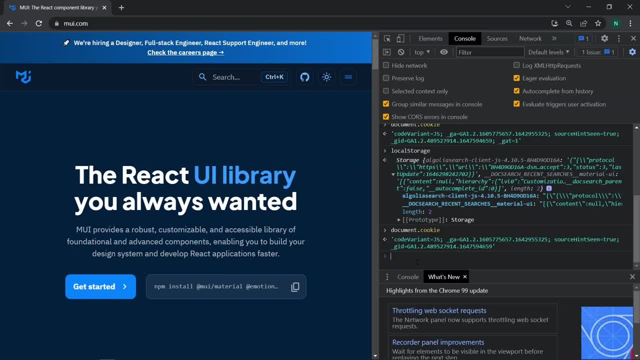 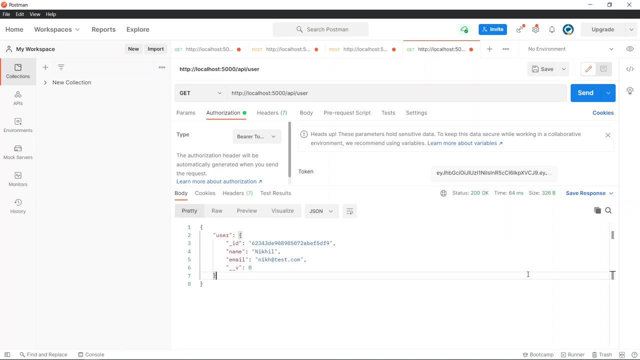 verifying and then providing the access to the user. so that's a lot of discussion about that, so let's go ahead. so postman have a default settings to send back the http, only cookies. so we will test it on the postman first and then, if everything will work fine, and then we will get into the 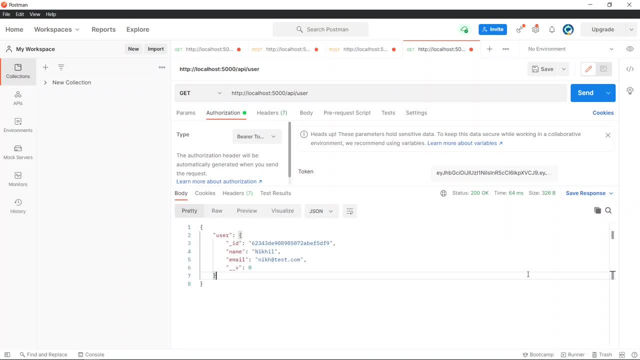 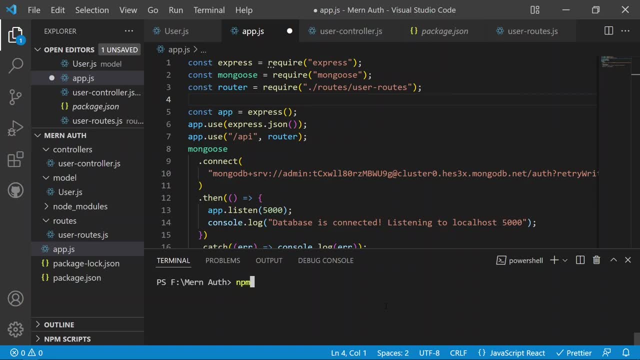 front end building the front end application, and then we will use that with the react and the xeos. so now to use and send the cookies, we need to install a package named cookie parser, so it will the npm install as a cookie dash parser. so after this package we need to use the cookies and then 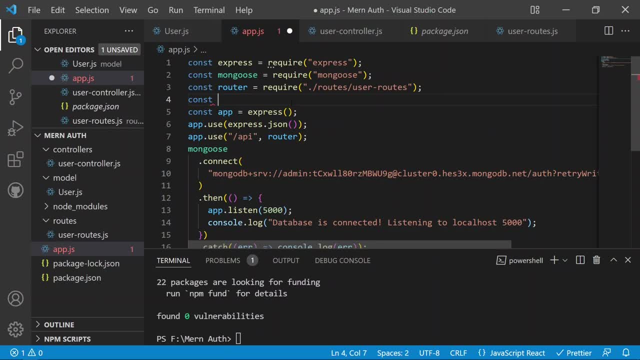 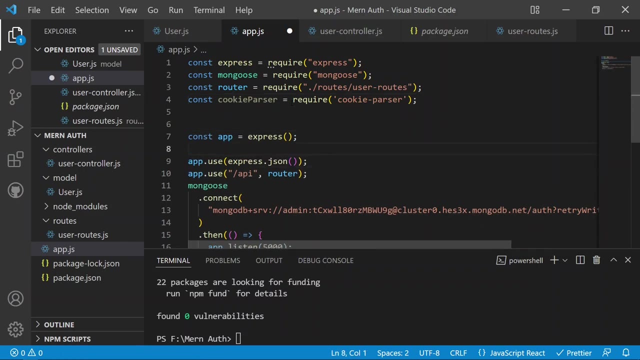 we can just import the array as icons, as the uh key parser, and it will be equals to the require. and then we need to add here the cookie parser after the require. so now we have imported the cookie parser and now we need to add it into the middle ways as well. so before any middleware, so we can use here the app dot use and 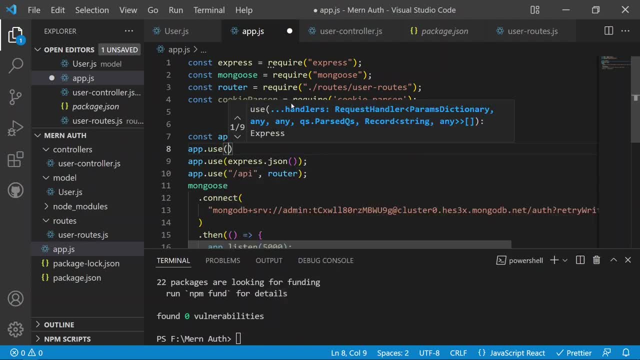 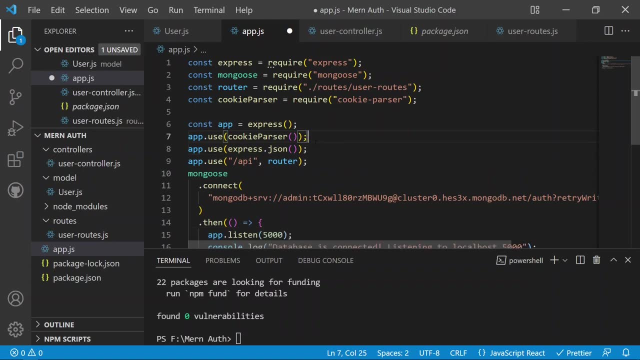 it will be the, so it will the app dot use and it will be the cookie parser. so we need to add here the cookie parser and then we need to call this function. so now we have now imported the cookie parser and then we can use the cookie parser in our application. so now i am restarting the. 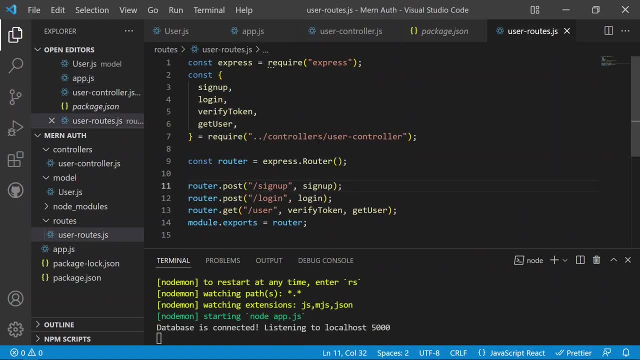 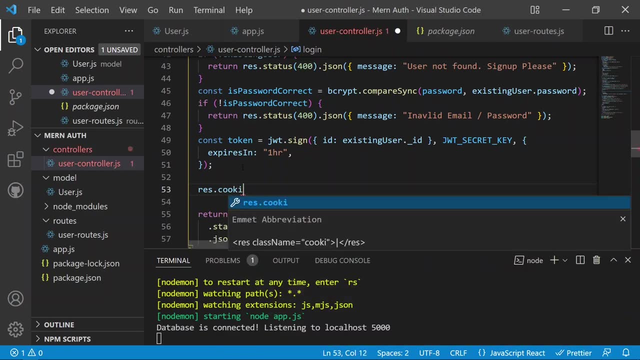 application again, and then we need to go to the user routes after the user is logged in, so after the token is created, and then we can just say that the response dot cookie and it will be the function to add the cookie. now you can see responsecookie. we can provide a name. 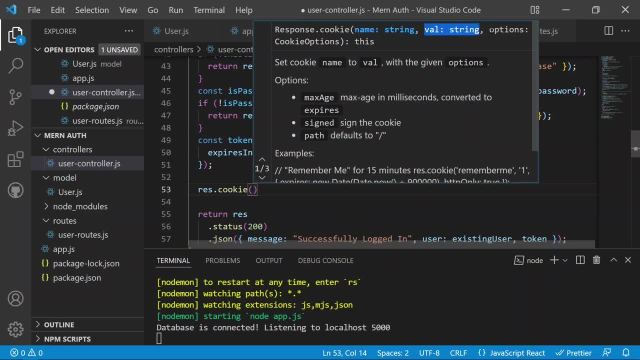 of the cookie, then we can provide a value and then we can provide some options in the third parameter and the options can be like maximum age, the expires, like when the cookie will be added up. so here i will provide some options in the third parameter and the options can be like maximum age, the expires, like when the cookie will be SEALED, like when the cookie will be AM FROM TV WHEN THE COOKIE WILL BE ADDED. hochl. 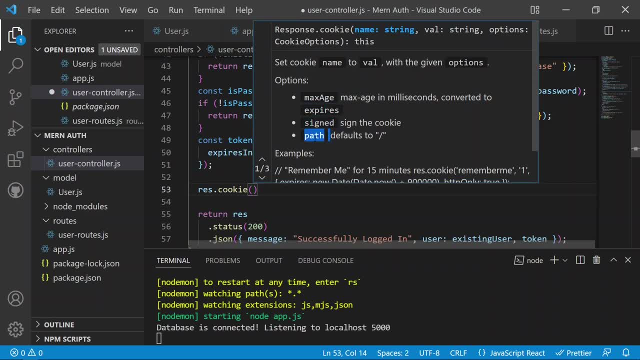 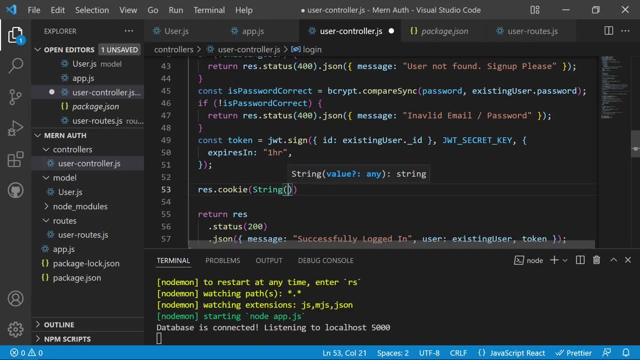 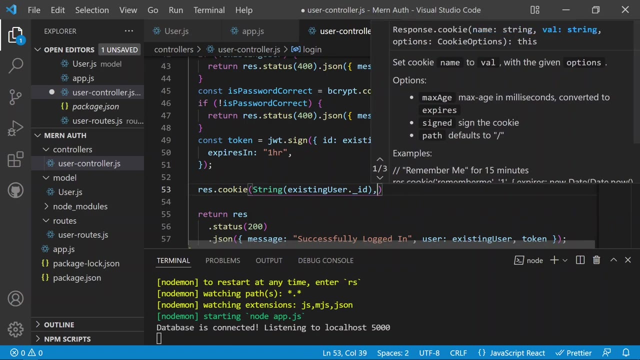 expired and then the sign is true or not and the path. so we can just add these things. so first it will provide a name, so we can just add a name as the id of the user. so we can just add the id, like we have the existing user dot underscore id. so this is the id, so this is the name of the cookie. 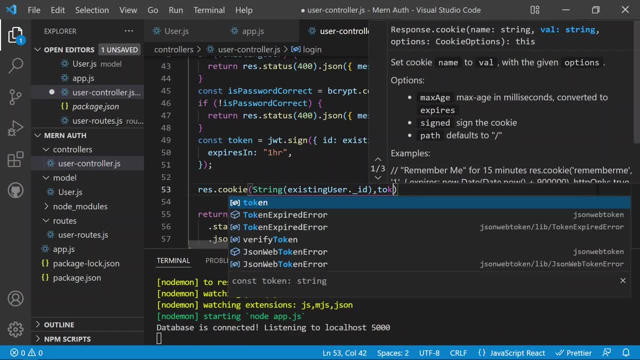 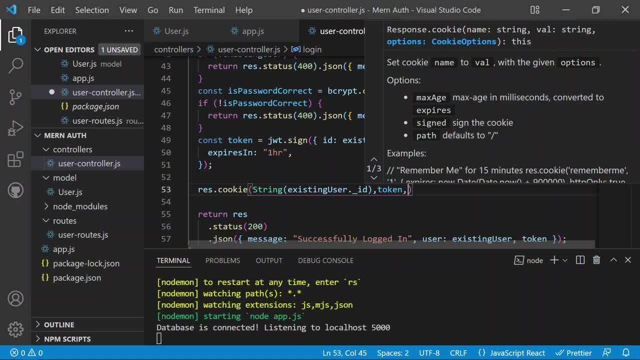 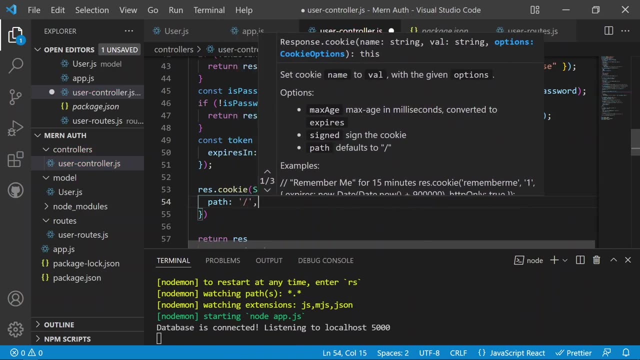 and then the value of the cookie would be the token. so we will send the token and then we will check the token of the user after the cookies and then we can just add here some options in our object. so at first it will be the path and the path will be can be just, it will be the by default. 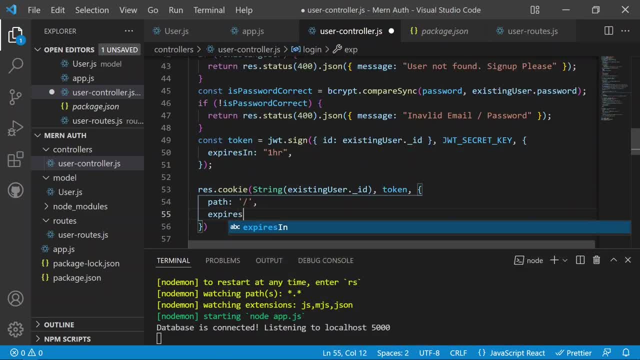 blank path and then we can just add here the expires, and the expires will be there, and then we can just add a new date here. that's the new date because it need the date in the expire, so when the expired will be there. so we can add a date dot now in the new date, so it will provide. 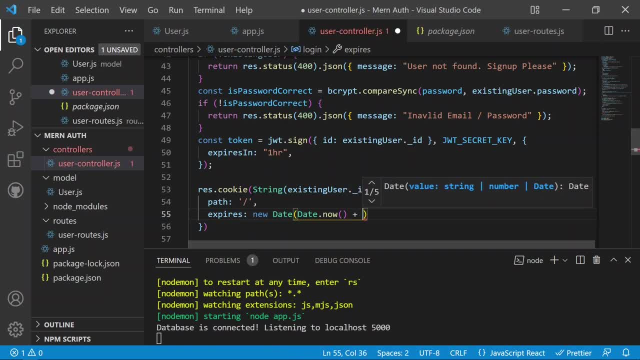 a number and then we can just add, like, if we want to cookie for just seconds, so we can add the thousand, because a thousand milliseconds is just one second. so we can just add the cookie for 30 seconds for now, and then after that we need to add the http only. so if i do not provide the http only in that 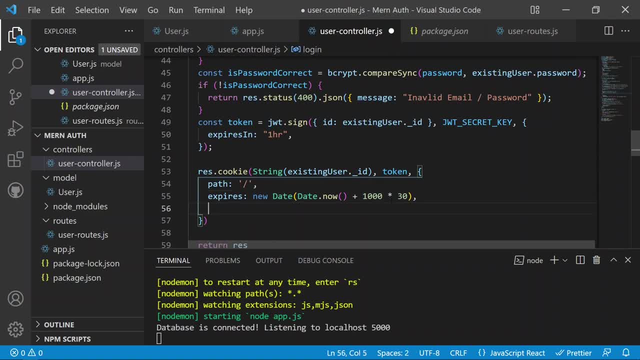 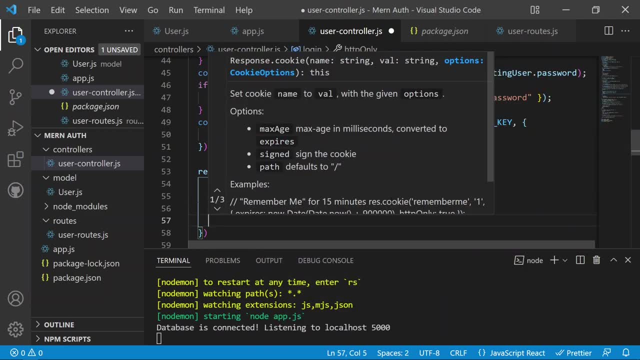 so then it will be accessible to the front end. but we need to provide the http only also, so it will be the http only. so we need to provide it to the true, and then we need to provide a one more property as the same site. so for the security reasons we can provide the same site and give. 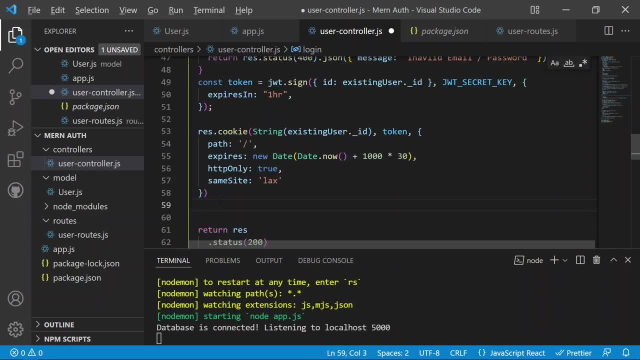 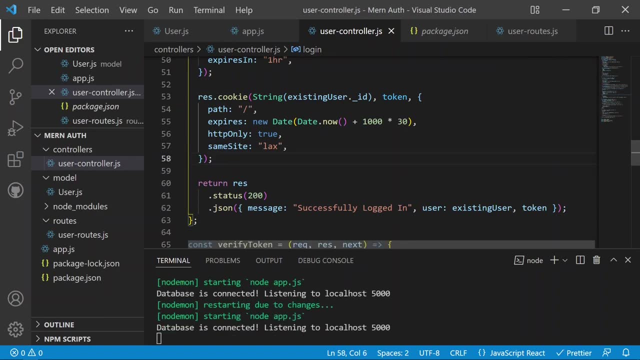 a value as the lax. so now we are sending the cookie. so now we are sending the cookie with the response dot cookie after the token is created. so if i will now save and if i will now just go to postman to send the request again, now i'm in the postman and now we need to go to the login route and then we have. 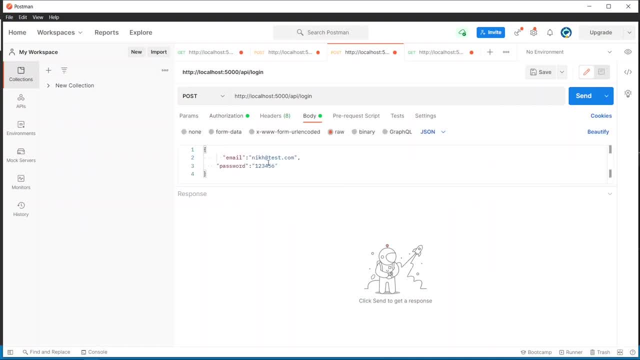 the authorization and my token is now expired, which i sent for this. so if i will now send this again, now we should see the cookie there now. you will see. now we have some data that the user is successfully logged in and then we have token and then if we want to send the token to the postman, 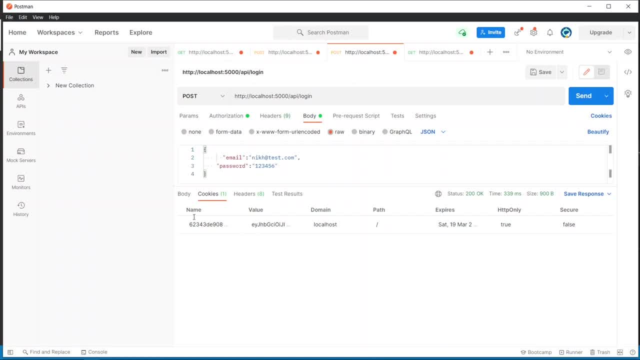 if you will go to the cookies tab now, you will see we have a cookie like: the name of the cookie is the id of the user, and then the value has the token, and then we have the domain of the localhost and then we have the path and we have the expires in property, also like the, it will expire after 19. 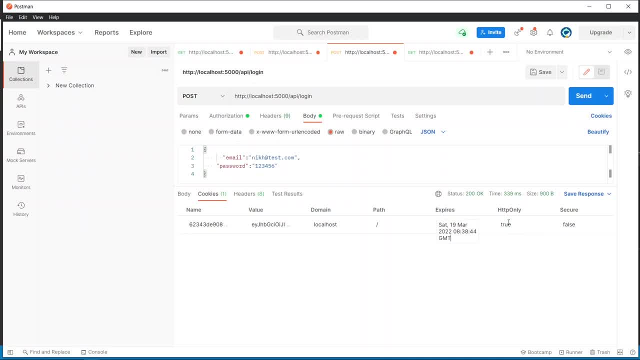 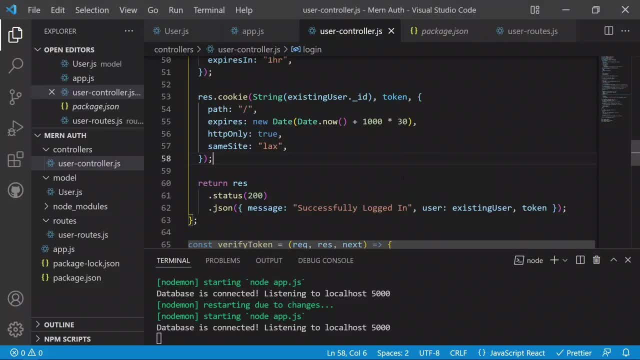 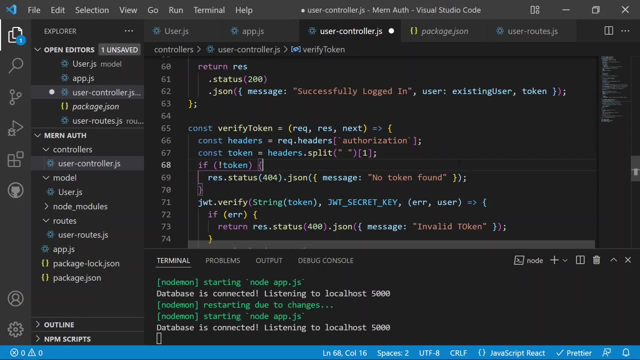 march after just 30 seconds. and then it is the http only cookie, because we have not provided the http only and it will not be overall accessible to the front end. so now we have provided the cookie and now we need to get the toki in the verify token, because then we need to verify the token. 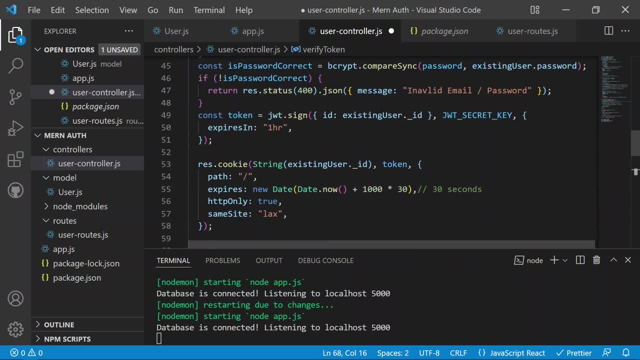 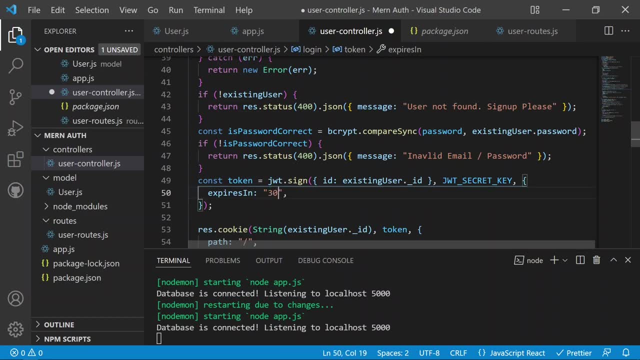 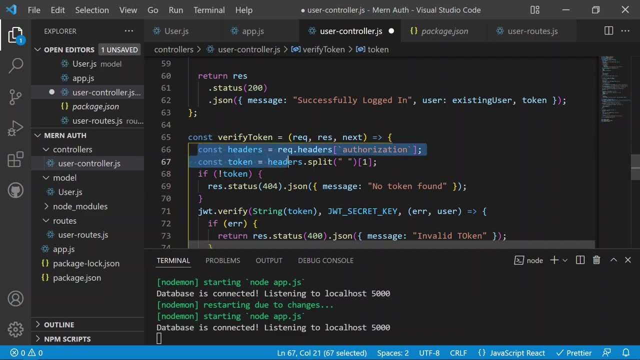 as well. so we have specified the cookie for just 30 seconds and then we have specified the JW token for one hour, so we can just increase or decrease that to the 30 seconds as well- 30s so it will be added to the 30 seconds, and then we need to go to the verified token now and then, instead of this. 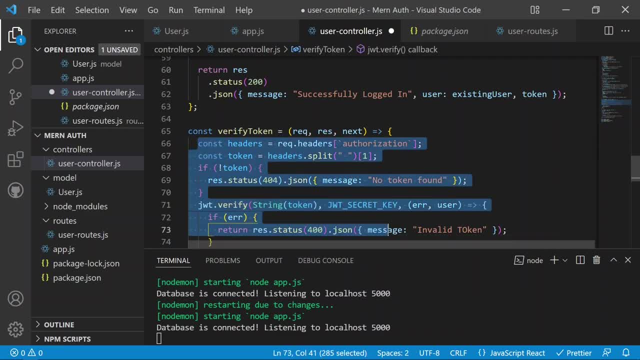 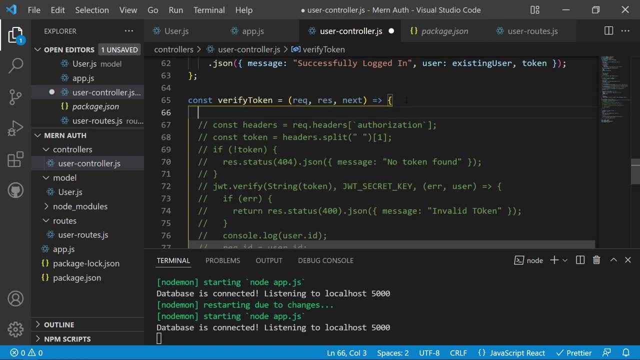 headers. we can now just remove these headers and then we can just comment all of the functionality for now in the verified token, so we can just comment it out and then in the verified token. now we have the cookie in the request dot headers, so we can just get the cookie like cookies and it will be equals to the request dot headers. now we 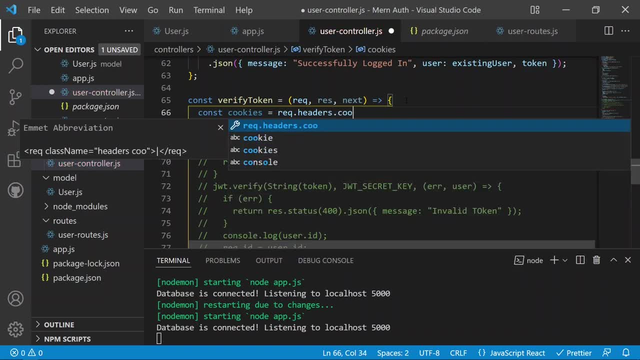 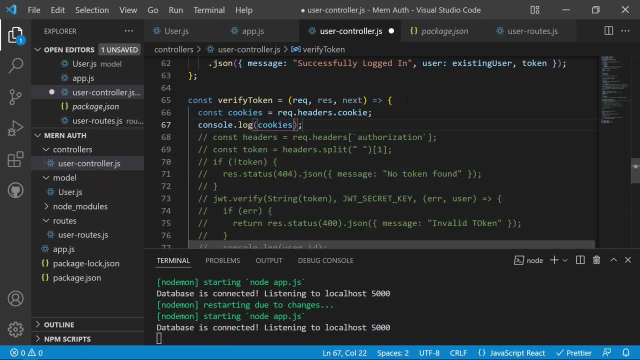 have the cookie in the request dot headers and it will be the cookie. so we can just use that cookie and then we can just console dot log that variable as the cookies. so now let's see if we are getting the cookie back in the request or not and then first we need to just log in the user again for 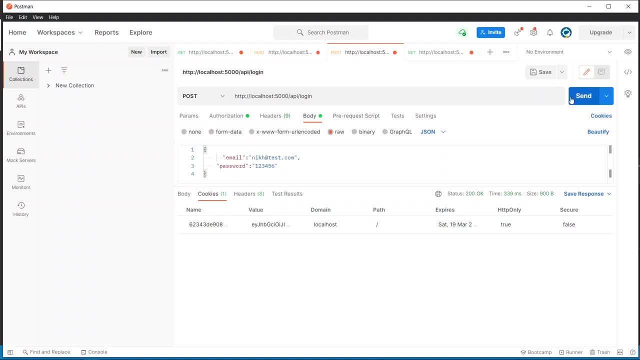 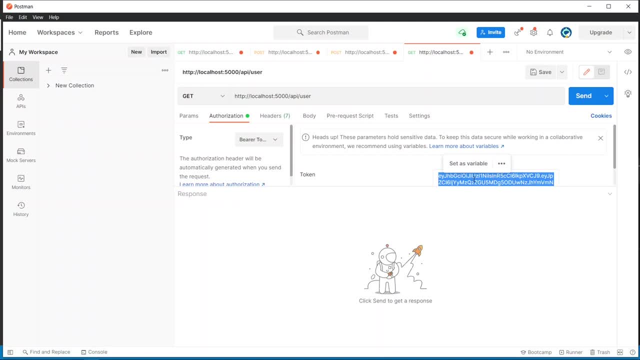 the 30 seconds, because the user will be expired in 30 seconds. so we can just send the request again. now the request is being sent and then we can just use that, get request again for the user, and then we need to remove this bearer token as well. click on the send. so now you can see, now we are getting back. 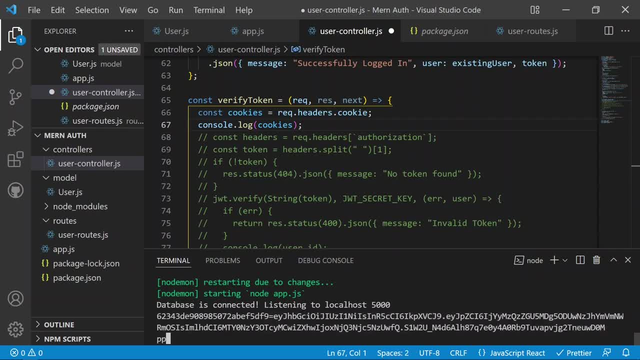 the cookie after the request and the cookie will be equals to. like you can see, it is the ID equals to the token. so now everything is working fine and we are getting back the cookie in the request dot headers. so now we have the cookie and now we can just split the cookie with the equals to. 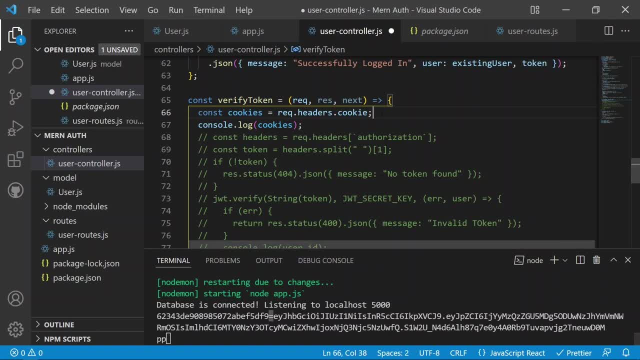 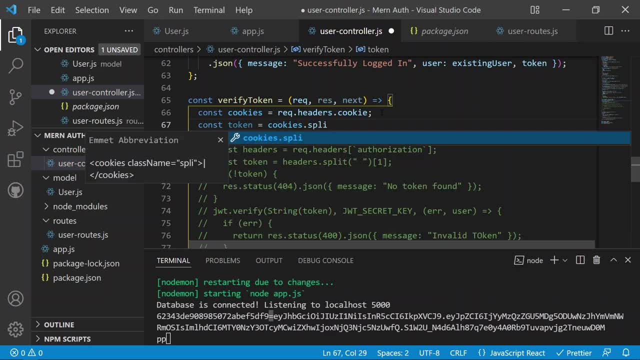 sign and then it will be divided into two parts. so we can just get that. so it will be the const. as the token. again, it will be equal to the cookies. we have dot split. so now we are splitting the cookies and we need to split it with the equals to sign. so it will be the equals to sign and then we need 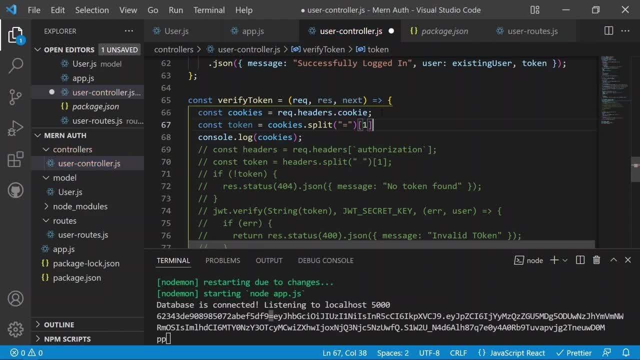 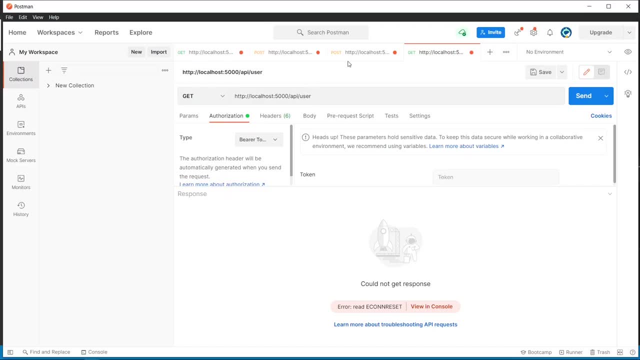 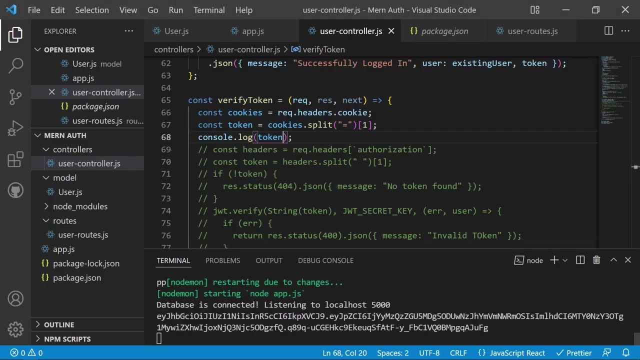 to get the first index. so it will be the like the: we need to get the first index after that and then we will get the token. so if I will now just console dot, log the token again and if I will now just send for the login again as the post again, get the token, send now. you can see, now we have the token. 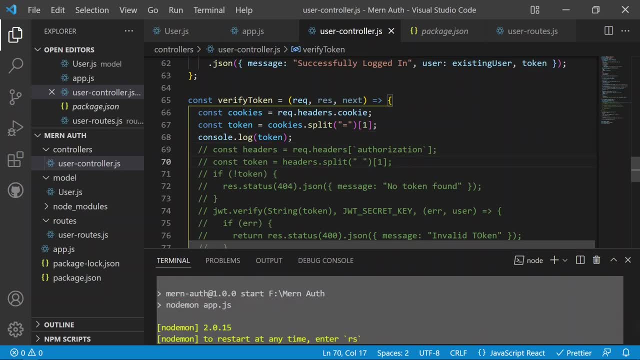 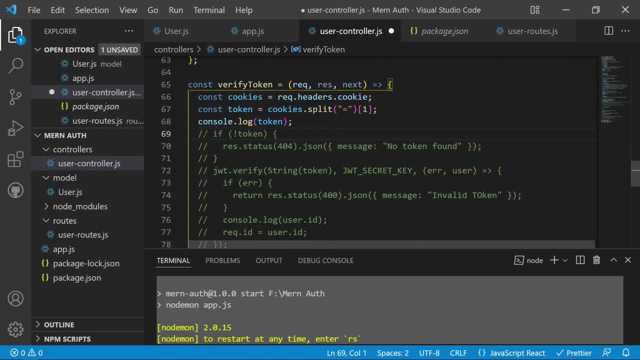 which we have received from that postman. so now we can just stack all of the things again from the headers, so we can just remove from the headers there and this const token again, and then you can see, now we have everything working fine, and then we need to just uncomment everything, and now you 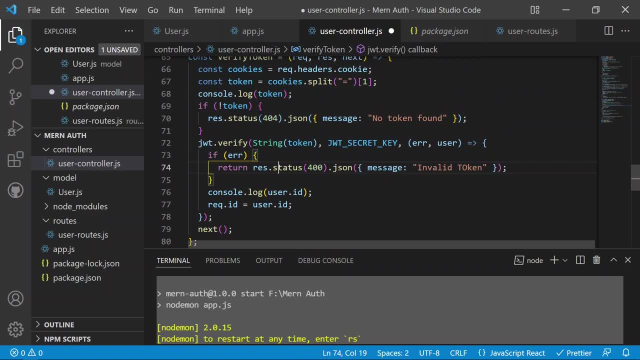 can see. now we have the token and now we are now splitting the token with the equals to sign. then we have the token and then we are already verifying. if we don't have the token, then we have to send the responsestatus as the 404 and in the message we have to send that no token found. and then we 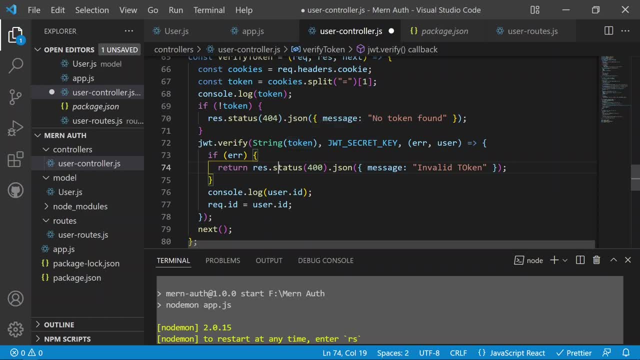 can just check in the jwtverify that if we have the token, if it is equals to the token and if the verification is successful, then we can just return the. we can just check the userid which we have decoded from there and then we can just attach the id to the request and then it will be equals to. 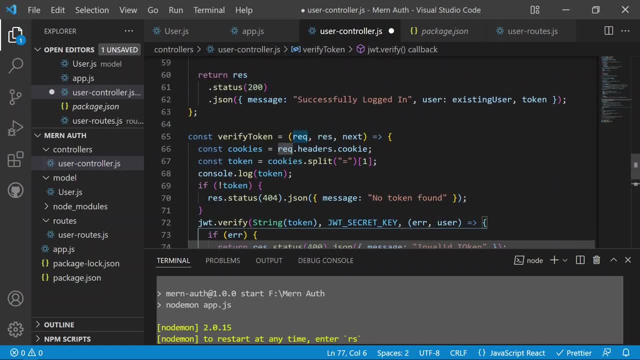 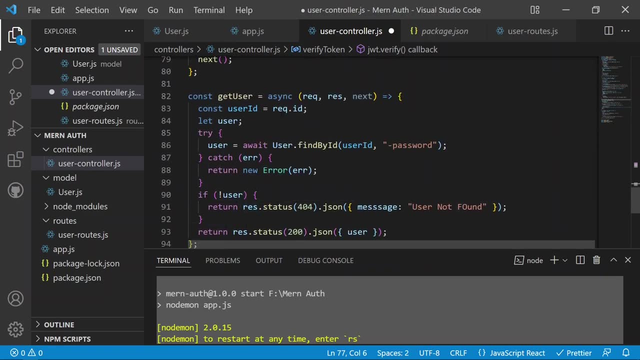 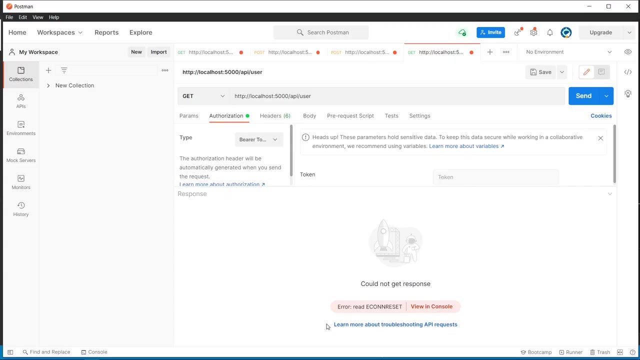 the userid which we have decoded, and then we are moving on to the next middleware, and the next middleware we have the get user, because now we are already getting the user id from the requestid, so we don't need to change this at all. so if i will now save all of the things and if i will now just go, 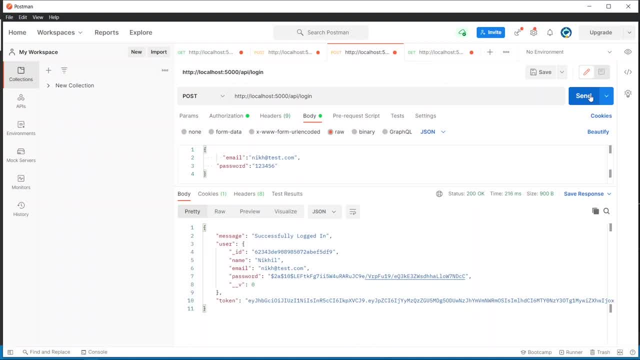 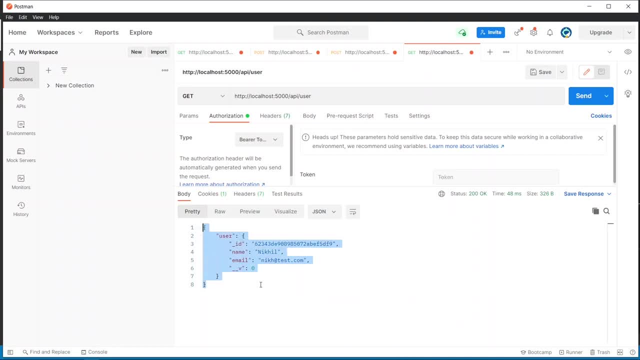 to the postman once again. set the request after the login, send the user. we have the token. send the get request again and then we should see the user. now you can see, now we have the user and now everything is working fine. and now if you will wait for 30 seconds to see if the token is expired or not, so we have to wait for. 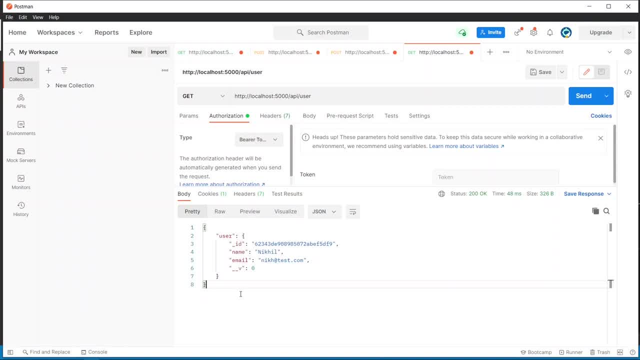 30 seconds. so we can just wait. i will stop the video and i will just continue the video after 30 seconds. so now, after 30 seconds, now we can check again. so if i will now click on this and request, now you can see: cannot read properties of undefined. and now you can see the token is being. 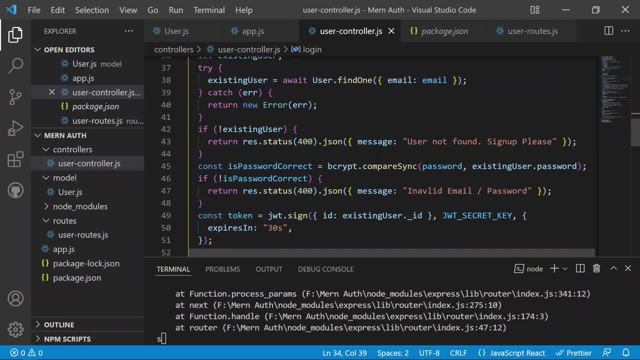 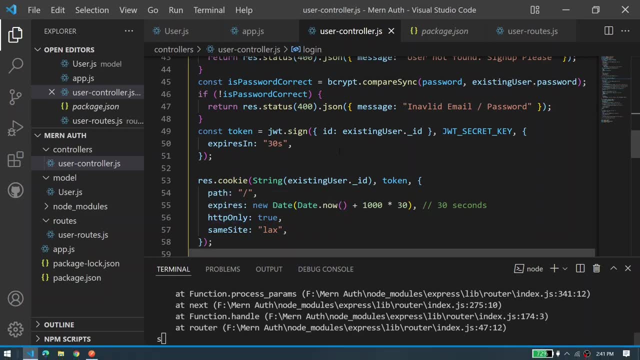 expired and now everything is working fine. and now we are setting up the cookies after the user is logged in and the expiration time is just 30 seconds and the cookie will also be logged in, and then we are just verifying the token to get the user and then we are attaching the requestid to. 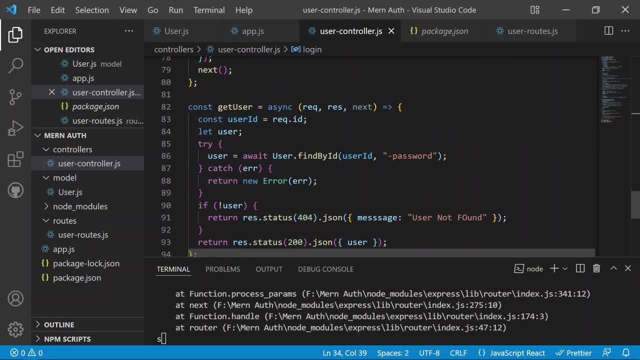 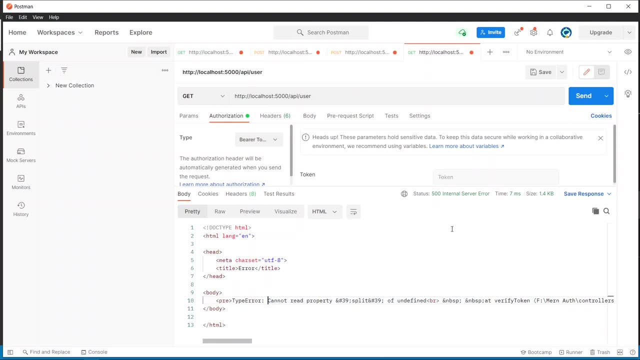 the userid and then we are fetching the user. so now everything is working fine. and if i will now just click on the get user again and then you will see the cannot read properties of undefined, because now the token is expired, but if i will now still log in again, if i will now get the user, 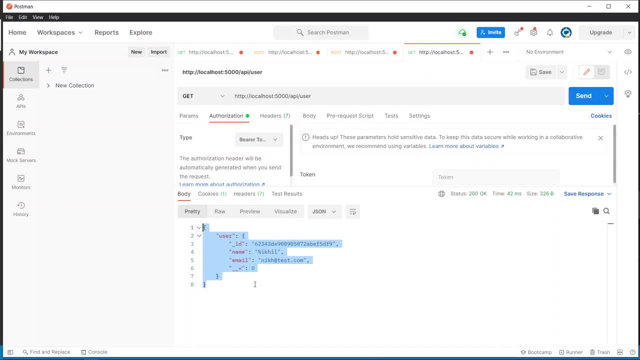 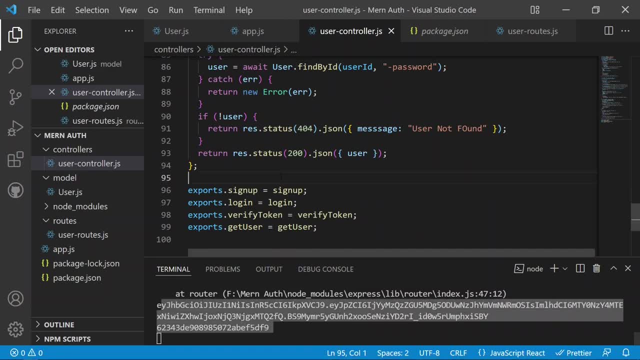 again, and the user will be there, because now the user is currently logged in and now it will be expired in 30 seconds. so everything is working fine and now you will see we are getting the token and the id as well. so now everything is up and running and now we need to build the front end to test it. 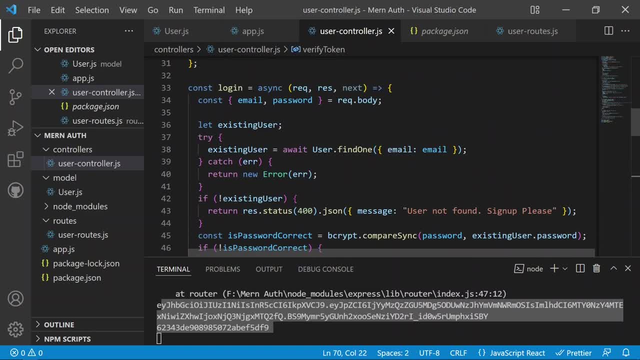 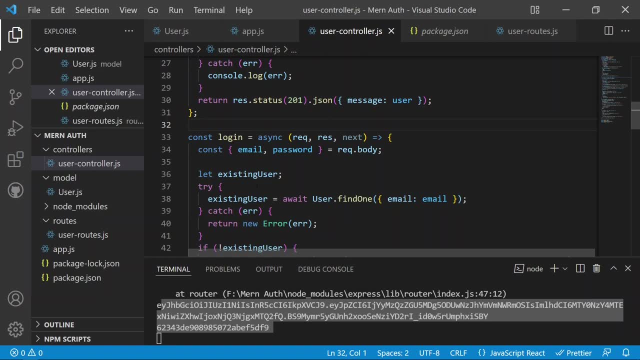 on the front end if it is working on the front end as well, and after the front end will be created. so we need to keep the user logged in again, because we can't keep the user logged in for just 30 seconds, so we will create a refresh token after the routes. so here we have, some routes like first: 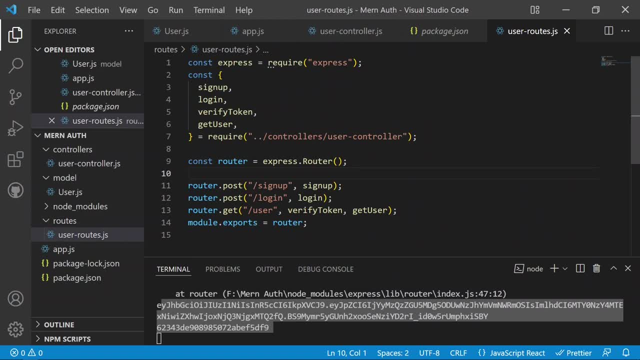 we have the post route for the sign up, then we have the login, then we have to get the user, where we are first verifying the token and then we are getting the user and then, after this, we will create a new route for the verify token after the front end application. 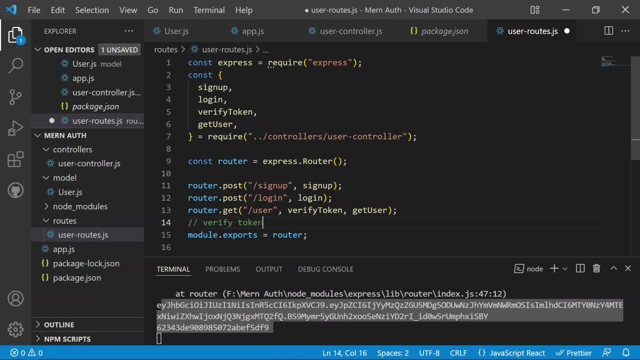 because when the user will be logged in, then we need to keep the user login after the 30 seconds as well, so we need to create a verify token if the user is still there on the website. so now let's start building the front end application, because now the back end is now over and the only thing 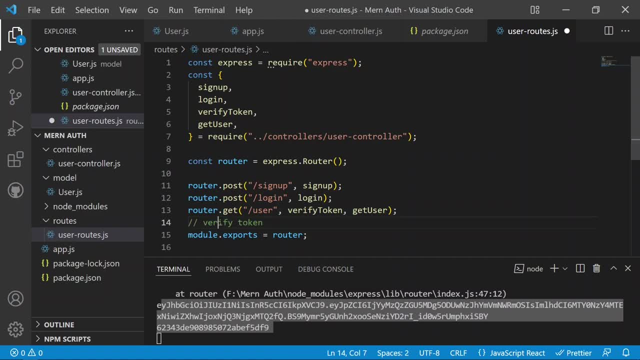 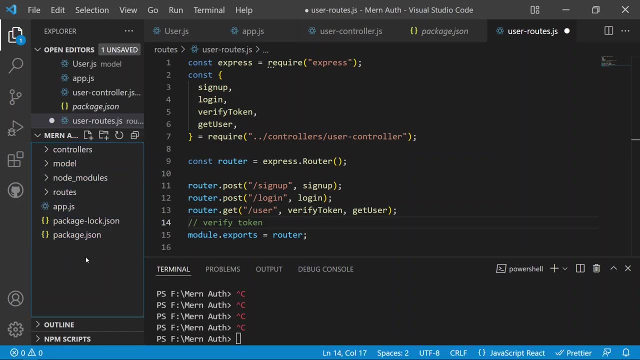 which is remaining is the verify token, and this part will be built up after the front end. so now let's start building the front end with the react. so now we can build the front end. so now we can just build this application from the front end, and i will now create a new folder as the back end. 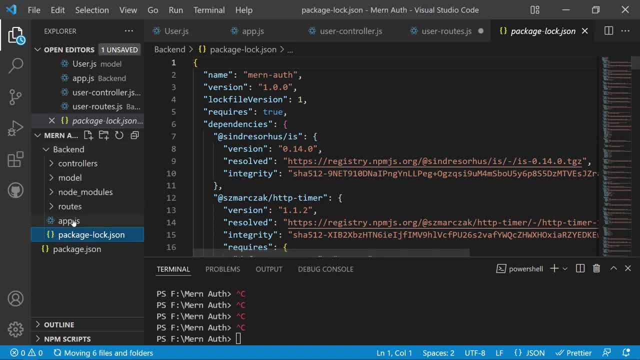 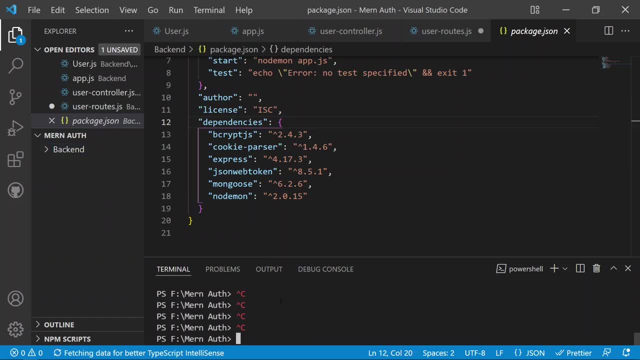 and i will now move every folder and every file there to the back end. so it will be going to the back end then, and then we will just fetch everything from the back end after that, so the packagejson will also be from the back end. so now we can just create a new react application there. 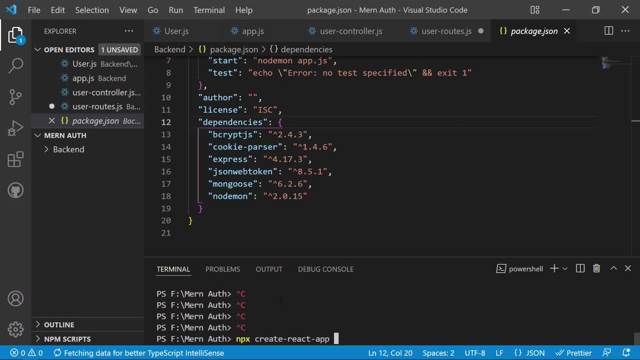 with the npx create dash, react dash app. so the name will be like the front end. so we need to build this application. so now we have created the command to install the react application and now we need to wait till the react app is installed. and now the react app is now installed. 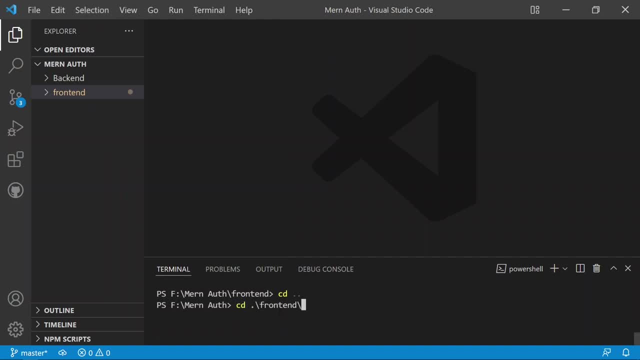 and now we can move on to the front-end folder, so to the CD, to the front-end, and now we can just start the application from the NPM start, and then the application will be up and running with this command. So we have to wait till it compiles and till it loads the react app for us. and now the 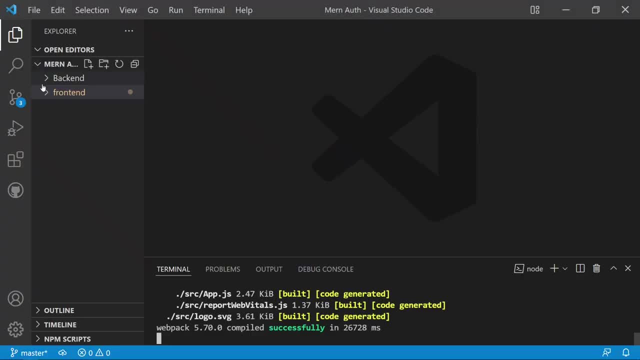 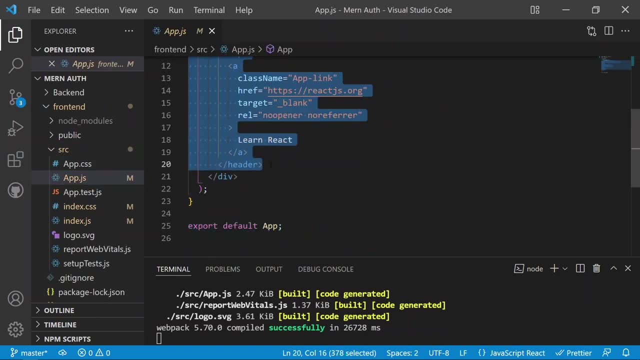 react tab is now compiled and it is up and running and now we can just go to the front-end, we can just go to the source and then in the appjs, then we can remove some unnecessary code from there. so we need to remove from the header till the header and i will also remove the class name. 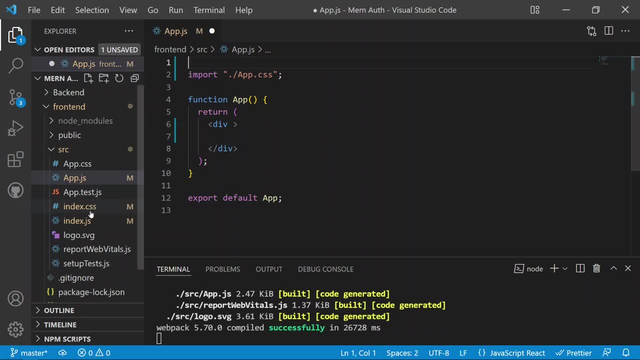 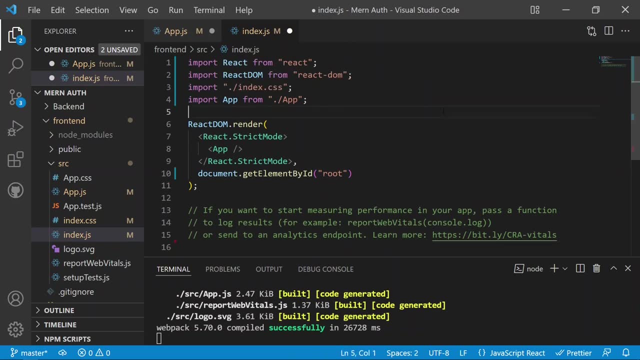 equals to the app, and then we can also remove the logo as well, and then we can just go to the indexjs. also, we can just remove the report web vitals, and then we can also remove the import as well, and then we can just go to the appcss to remove the basic styling, and then we can just 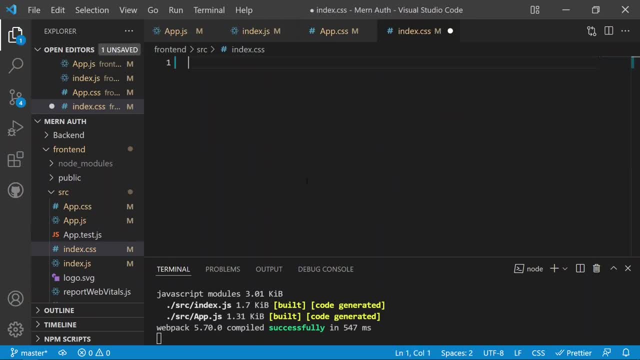 also go to the indexcss also and then we can just remove everything and then we can just add the star with the margin and the margin will be zero because by default the margin is the 12px on the browsers. so we can just remove that. and now we should see there should be nothing on the. 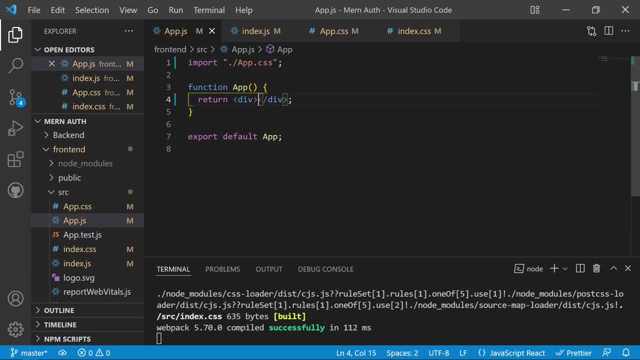 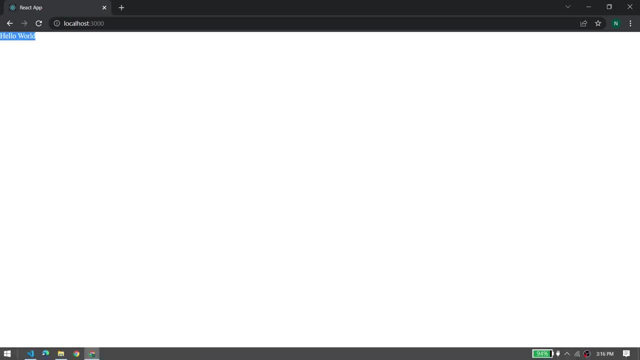 screen and now in the appjs we can just add here the hello world, so the hello world, and now we can save. now we should see the change onto the screen. now you can see hello world without any margin or without any padding from there, and now we can install some packages. 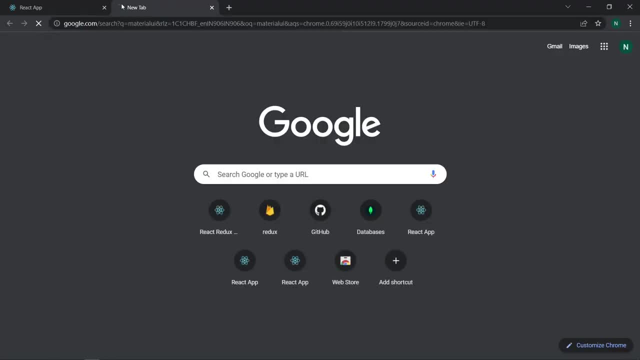 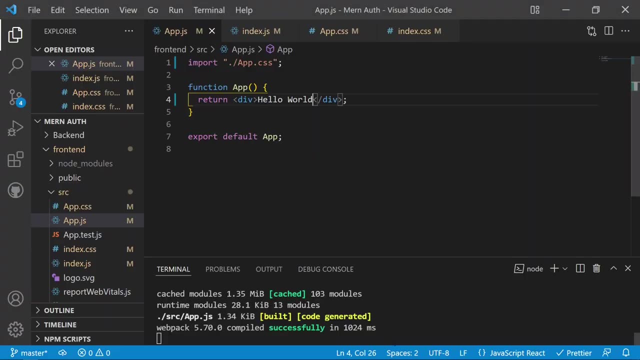 like we can install the material ui. so we need to go to the material ui to install that. so we can just go to the very first link of the material ui and we need to get this command to install that we can just stop the server again and then we can just add the command as the npm install material. 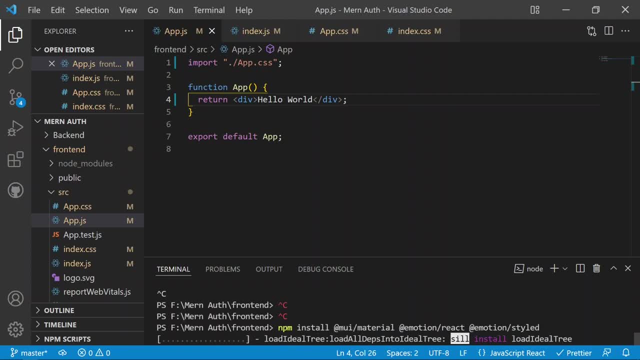 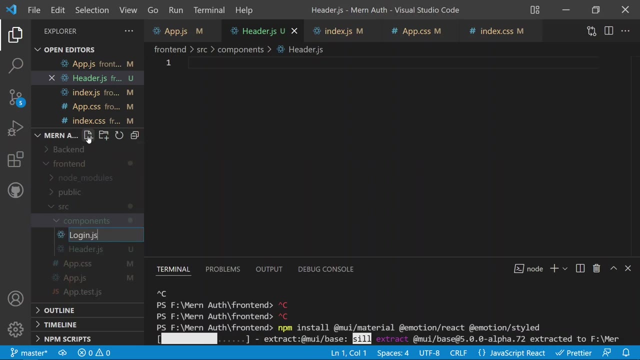 ui, so it will be installed. until then we can just create the folder structure like in the source. we can create a components folder and then we can build the components first, as it will be the header dot js, and then there will be the login dot js, and then there will be the signupjs as well. 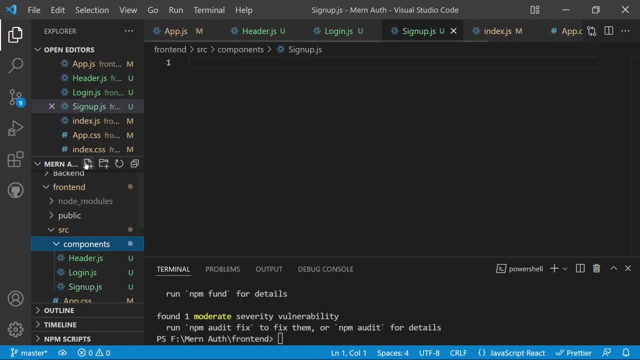 and then there will be the welcome page as well, so with the welcome dot js. so in the header we will just click on the buttons like the login and the sign up, and then the login in the signup components will appear, and then we will just, and then after 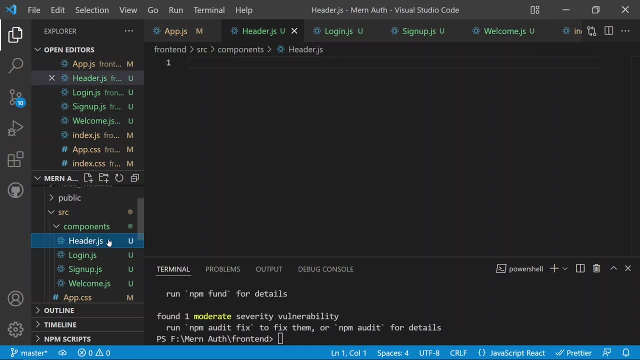 the successful login. we can just go to the welcome page. first we will build the header, so i will add the basic setup of the react application by the rafce command. so then now we have the header, and now we can just use the header into the appjs. so 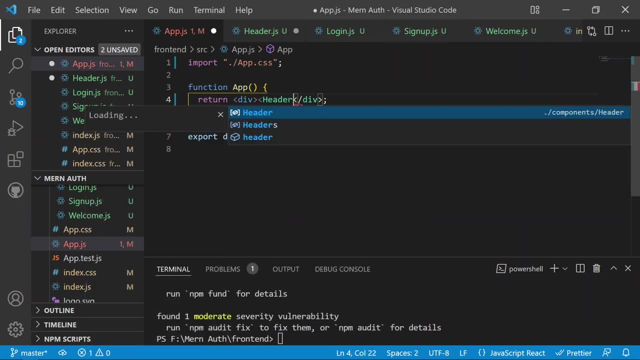 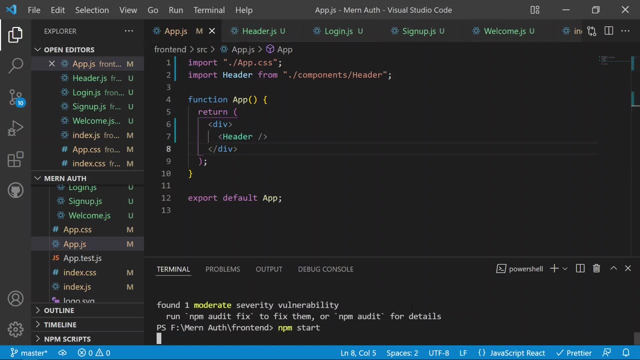 we can just import that, so it will be the header. so the header is now imported and then we can just save the application to see the changes. we can just start the application again as the npm start to see the changes and then the header will be there onto the screen. and now we have 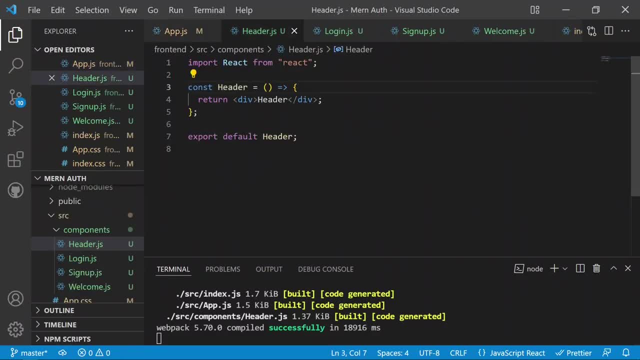 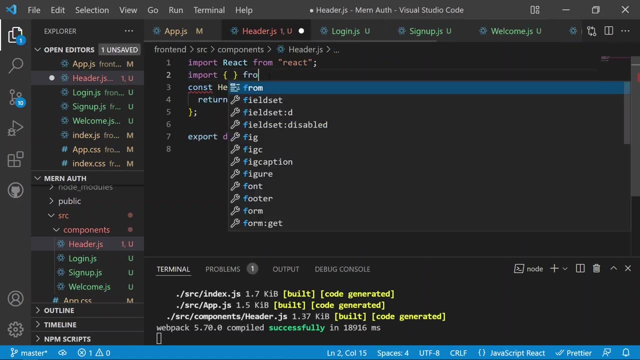 have the header onto the application. so first we need to go to the header and then we can just remove the header from there, and then we need to import something from the material UI. so we need to import something from the material UI, so it will be the UI material and then the something. 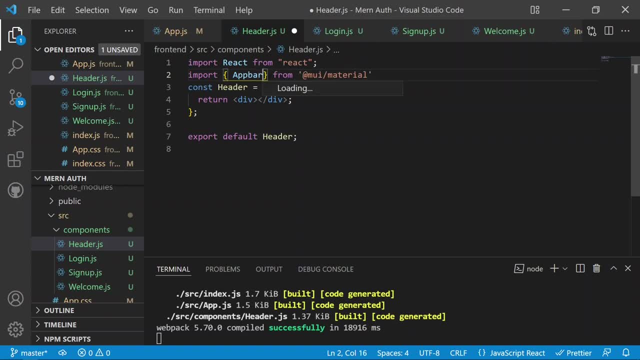 will be the app bar. so it provides a basic structure of the navigation bar and it provides a blue background color onto that. so we need to just import the app bar from there so we can use the app bar here as well. so it will just app bar and then you will see inside of this if I will now. 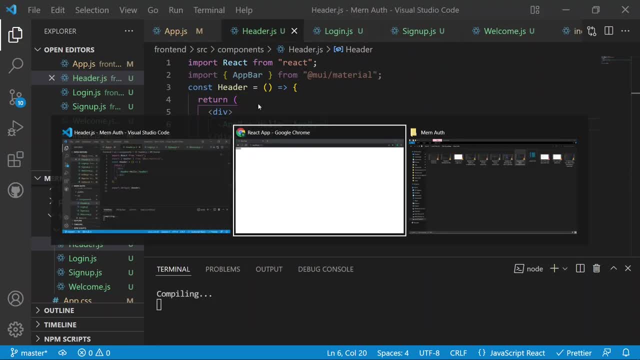 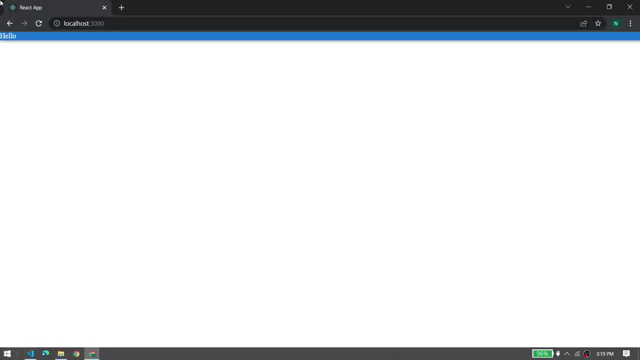 add the hello world. so there will be the hello world inside the app bar. so now, if I will now save, now we should see the changes onto the screen and now you can see it is compiled and now we can just go to the header. now you can see, now we have the hello there and then we can just add the. 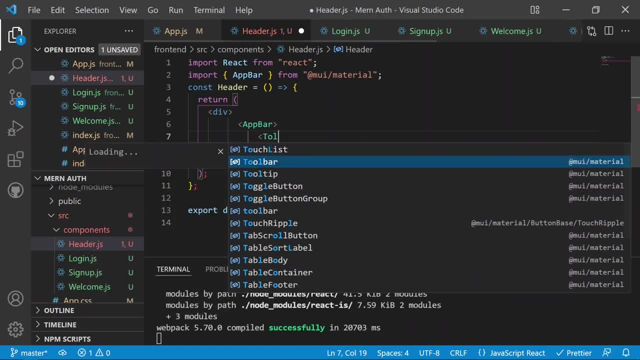 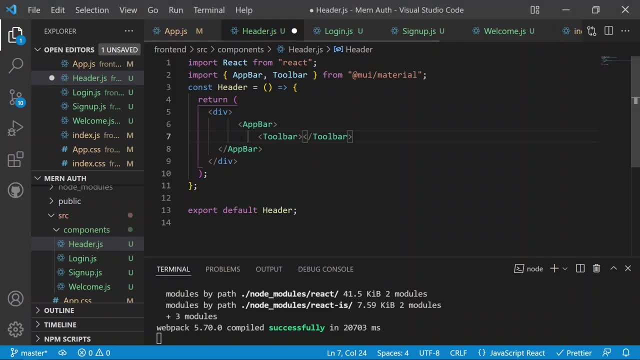 toolbar inside that and the toolbar provides us a styling inside the navbar. so by having the toolbar it will just increase the size of the main header with the header length looks in the real world applications and then we can just use the toolbar and then we can just add. 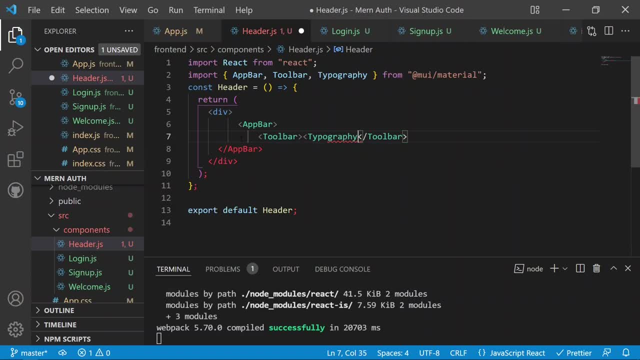 something like that: the typography inside that. so the typography allows us to add some text inside the material ui, so it will allow us to add some text. and then we can just provide the variant as well, and the variant defines as the which type of tag do we use. so we can just provide as the h3, as 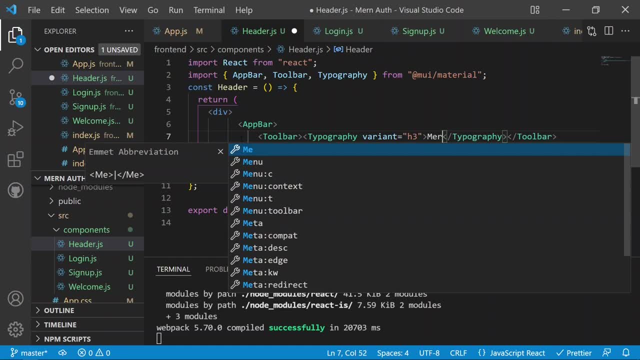 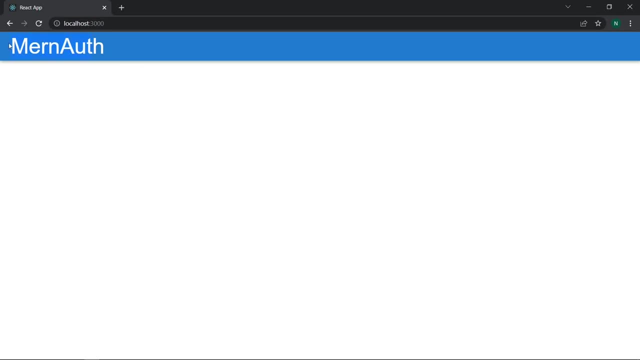 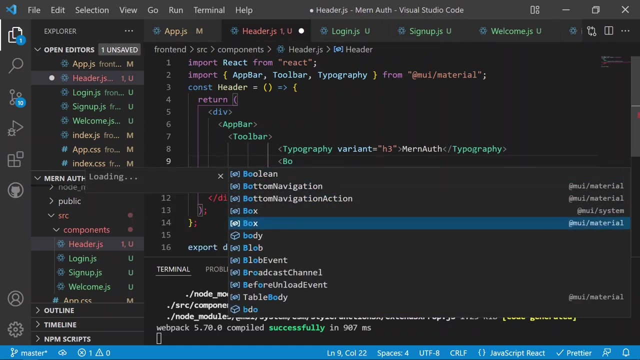 the heading and then we can just add the heading as the mern auth. so we can just save that. and if i will now save, now you can see we have the mern auth and now we have created the header with the material ui and then after that we can create a box like a div, so the box in the material ui just 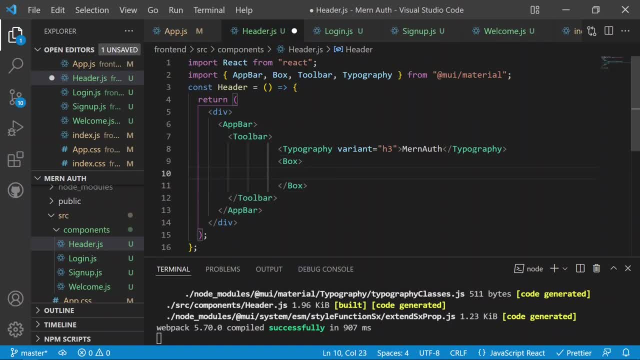 act like a div. so we can just add a div inside that and then inside this div we can add some tabs, like we can have a tabs, so the tabs is used to provide some tabs in the material ui, and then we can just have the children tab inside that. so this tab is the parent tab and this tab is a child. 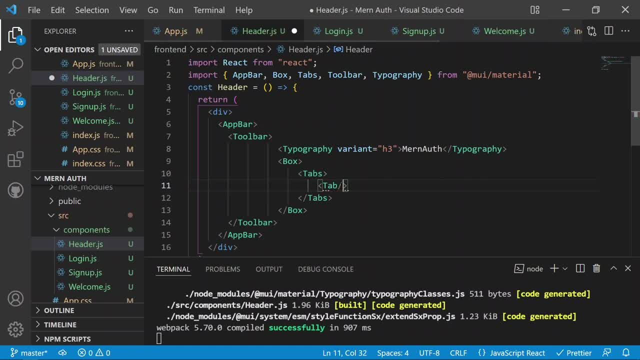 inside that we can just remove that you. then we can just add here the symbol tab i set and we can just import that also, and then now we have them tab and now we can provide the label as well of the tab and the label can be equals to: 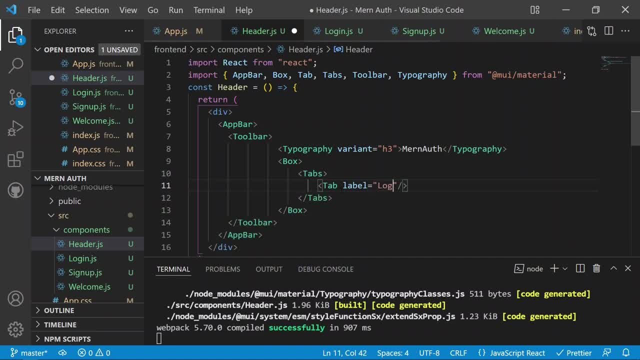 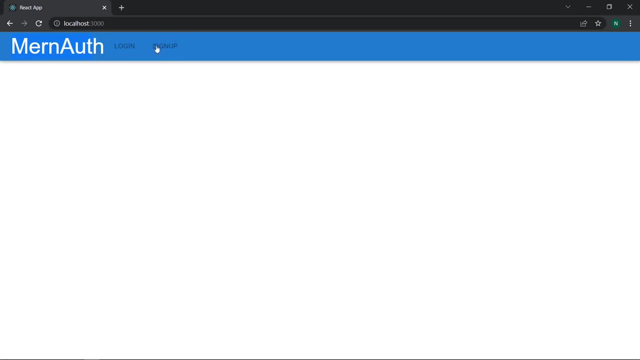 like we can just provide the label as the login and then we can provide a one more tab here as the and it can be a sign up, so it will sign up, and then we can just save. now we can see, now we should have the tabs as the login and the sign up there and once we can click on the login, now the login. 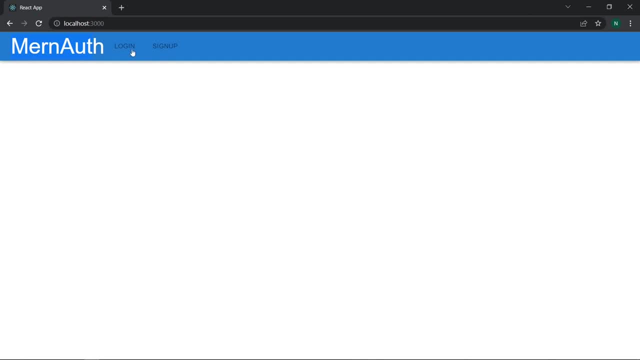 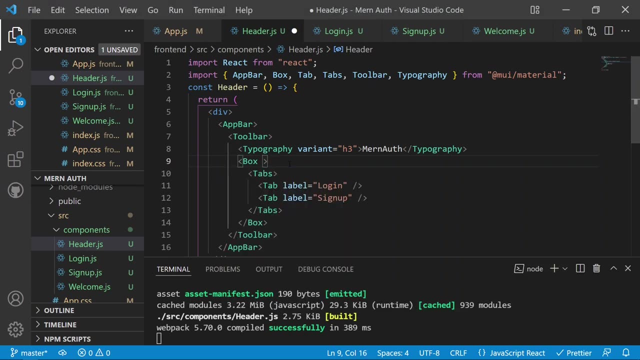 screen should appear and then, once we will click on the sign up, then the sign up screen should appear and then we can just move that box on to the right. so we can just move that. so it will be the. so it will be having the sx prop to add some styling into that and the styling can be the margin. 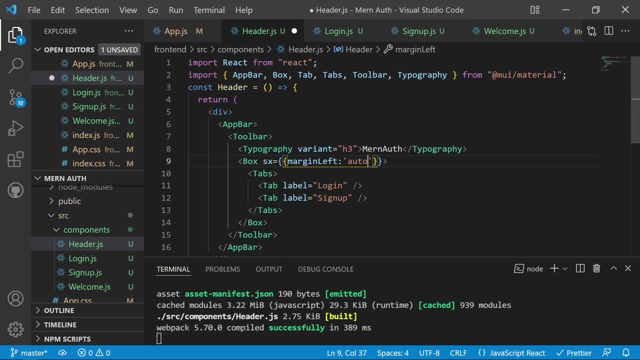 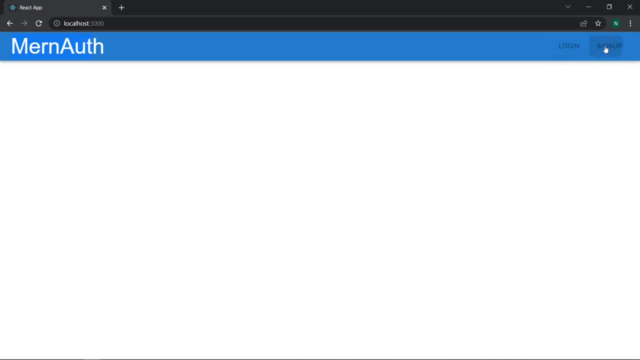 left, so it will be the auto, so it should move to the right. i think so now. you can see, now we have the login and the sign up and now it is moving to the right. so these are as the links and we can just provide some colors into that, like it will be the. 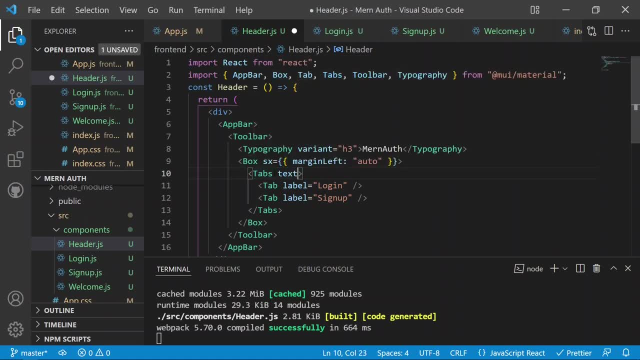 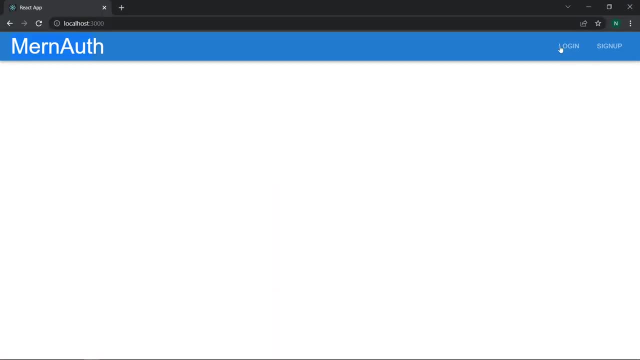 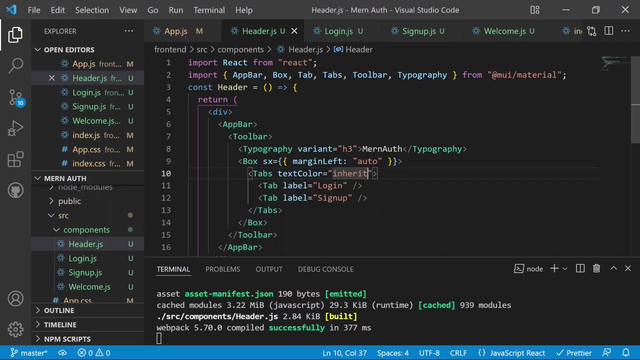 text color into the tabs. so with the text color and we can provide as inherit, so it will be inherited from the background. now you can see, now we have the login and the sign up buttons inside that and now the tabs are working and now we can see the tabs with the colors and now we can just add a. 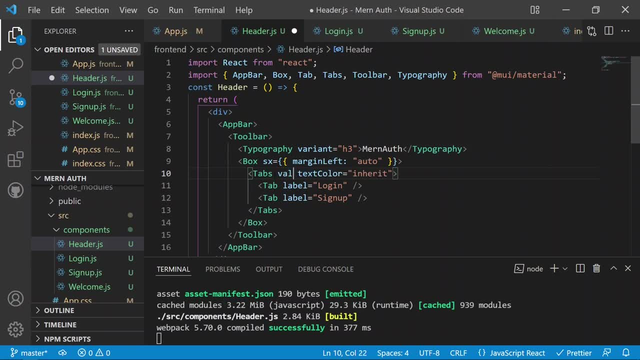 indicator color to the tabs. so we can just add a value to the tabs, like we can define a value of the tab. so if we will define a value of the zero, so it will start from the children, like this tab has the two children, so it will start from zero. 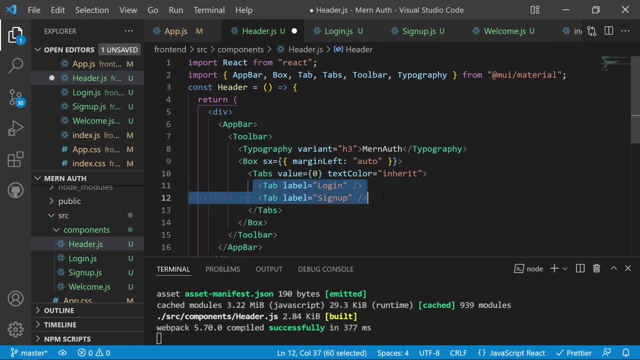 index and it will act like an array because the tabs are now children of this tab. so it will start from the zero children, from the zero index, from the children's. so if you will just add the value as the zero, so this tab would be highlighted because it acts like an array. so now you can see the login. 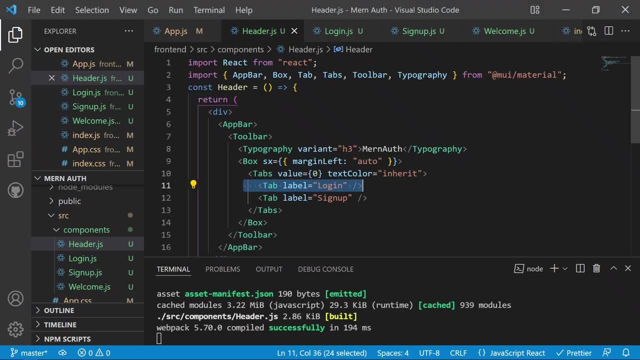 is now highlighted and the sign up is not highlighted. but if you will provide the value as the one now, you can see the sign up will be highlighted, so we can just change that. so after the tabs, we can provide an on change function also. i get the on change and the on change can be a. 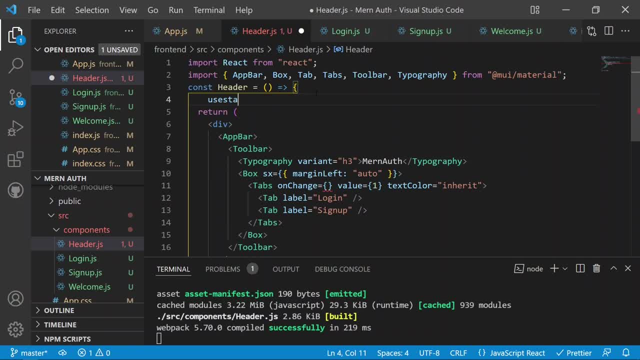 function and then we can just use the state here to change the state of the login and the sign up there. so we can use the use state snippet and then the first. it will the value and then it will the set value and by default it will be undefined. and then we can just use here the on change and it. 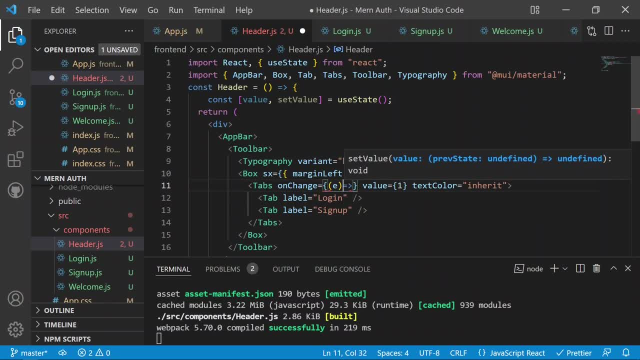 will contain an event. so it will be an event and after the event it will contain a value as well from the material ui. so we can just set the value of the tab as the material ui value. so if i would like the value can be like, we can just have the value of the value which we have defined in the 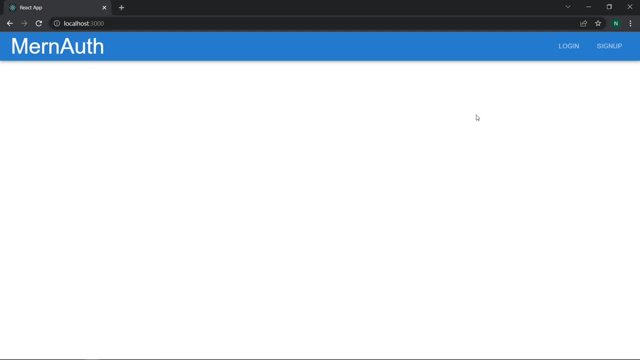 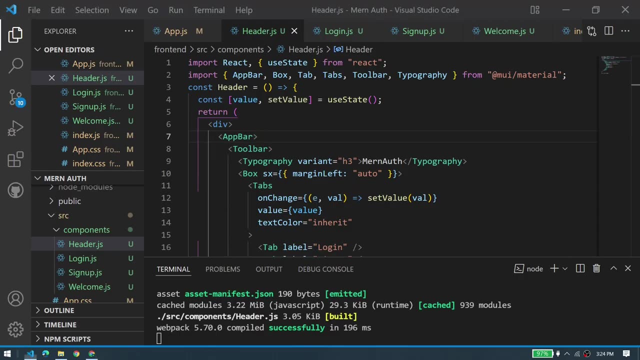 state. so if i will now save now, we should see the change onto the screen. so now, once i will click on the login- now you can see- the login will be highlighted, and once i will click on the sign up, the sign up will be highlighted, and then we can just add some colors as well, so we can provide. 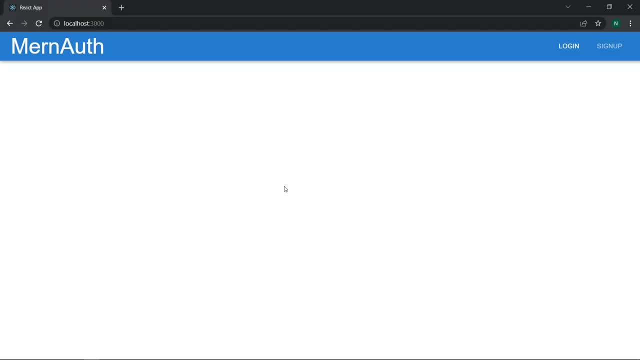 the indicator color. so if the login is highlighted, so we can just add the underline after the login. so indicator color would be secondary from the material device. so it will be like of a pink color again is highlighted with that and the sign up is also highlighted with that. so now everything is. 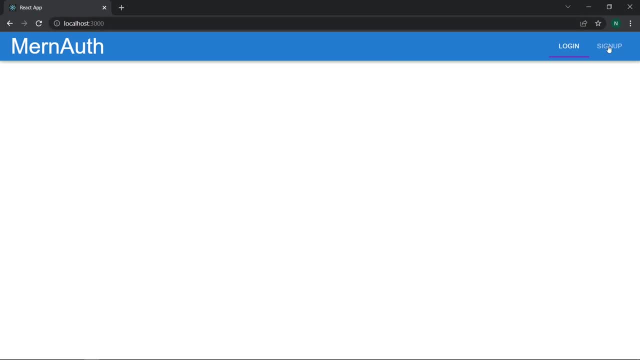 working fine till now. so now everything is working fine and all of the things are now highlighted. so now we have built the header and now we can build one more functionality. so once we click on the login, so we need to go to the login route and for the routing functionality in the react application. 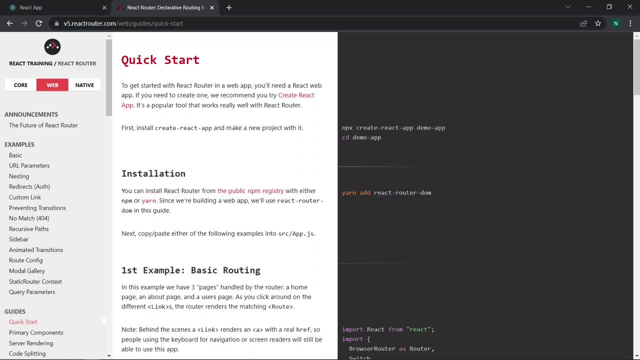 we know that we need to install some package and so we need to install the react router Dom so we can use that and if you are using the yarn, so then you can use with the yarn, with the yarn ad. but I'm using the npm, so I will now copy the package name from there and I will now add the package there. 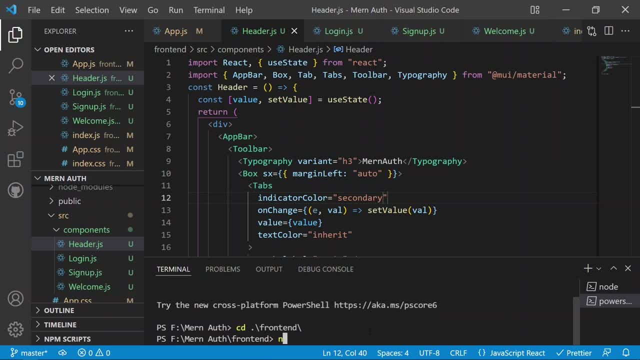 so after selecting the new terminal going to the front end, we can install the npm install react router Dom. so now the react writer Dom will be then installed, so we need to wait till it complete the installation. so now the react router is now installed and now we can use the. 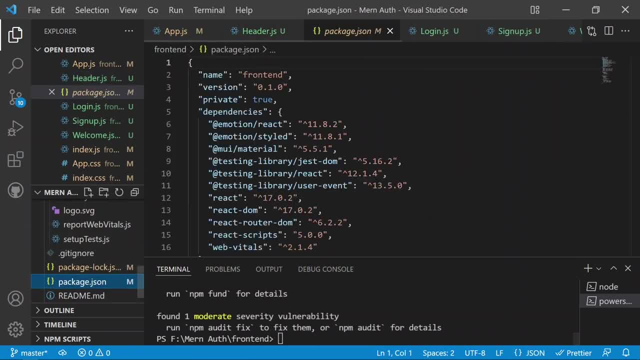 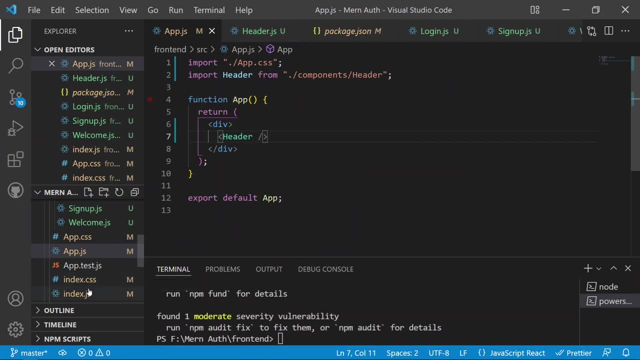 router and then we can see in the packagejson also if it is installed or not, and we can see the version as well of the react router Dom. so it is now installed and now we can just go to indexjs to use the routing and we need to wrap the app component with the browser router, which 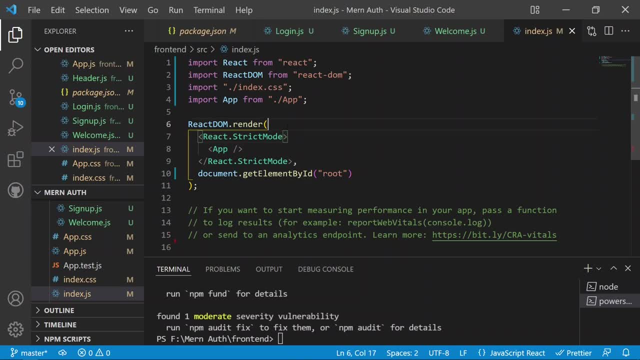 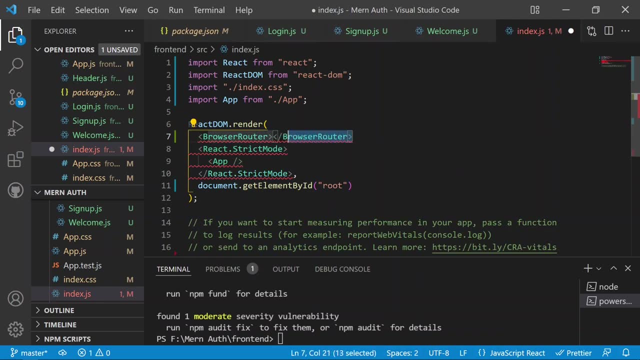 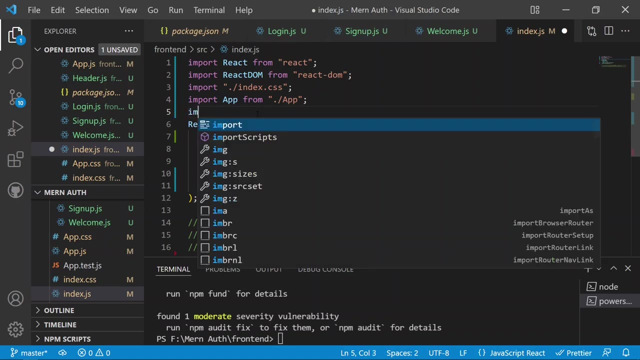 allows us to that, the routing functionality over the app functionality. we need to get the browser router and it will be imported from the react router, Dom. so we need to wrap everything from there to the here inside the react application so that the routing functionality should be there inside that and then we can just import the browser router. 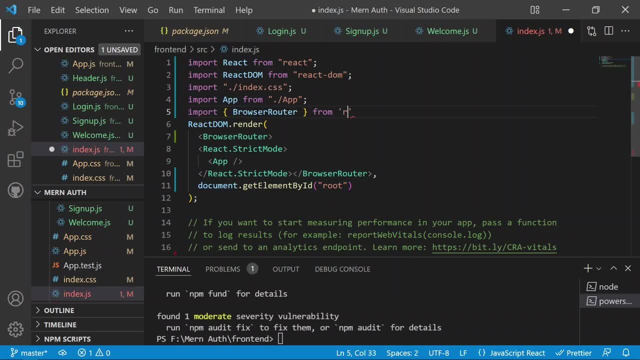 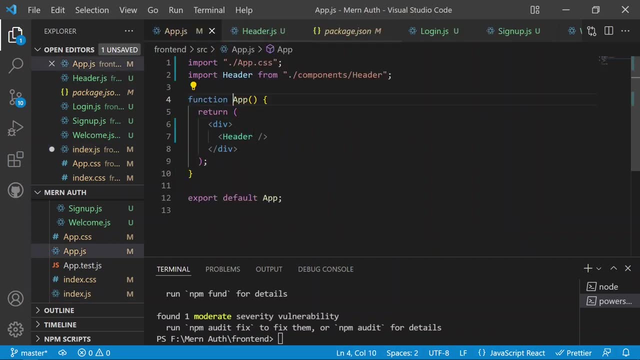 and it will be imported from the react router Dom. so now you will see it is now imported and now we can use the routes inside the appjs now and then we can just go to the appjs and inside this div. I will now remove this div with the header, so it will be the header tag and then we can use the header. 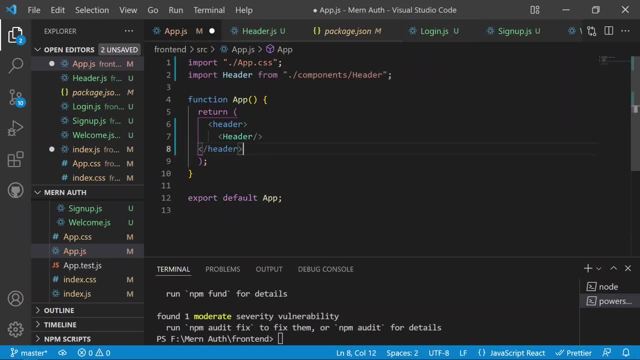 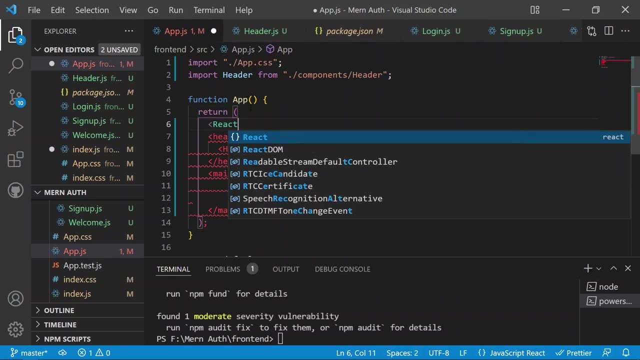 inside that and the header will be available in every route. so after that we can just define a main tag in the html and then we can just define a parent tag also, so it will be the react dot fragment and the tag dot fragment is like a wrapper which will wrap all of the components inside that, because 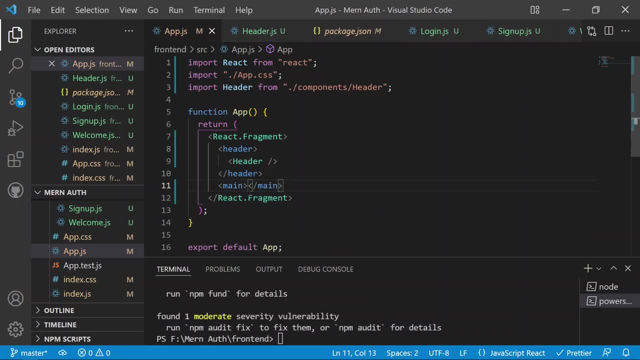 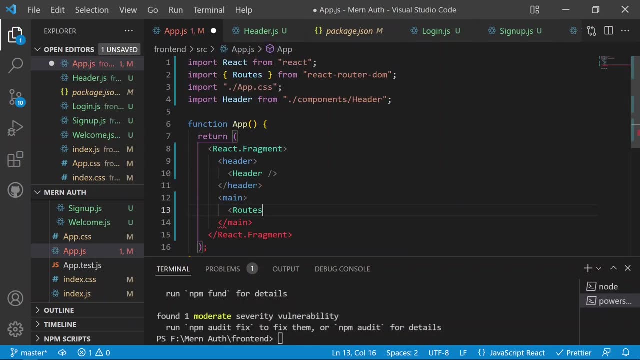 the rules of the jsx, so it should be having only a single parent. so now we are using the main and then we can import the routes. we can import the routes from the react router Dom, and then after that routes we can use the routes. we can just add here the single, single route which is the child. 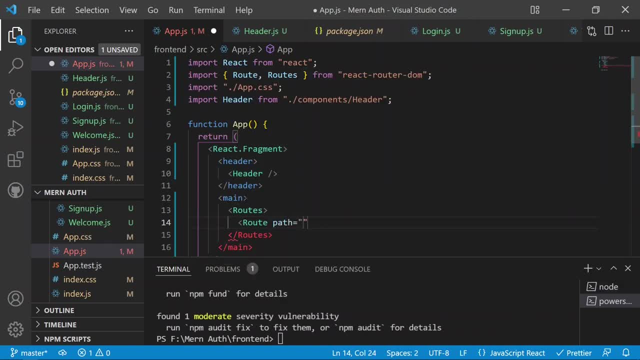 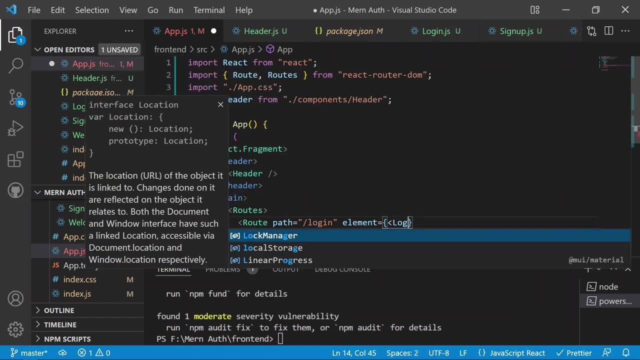 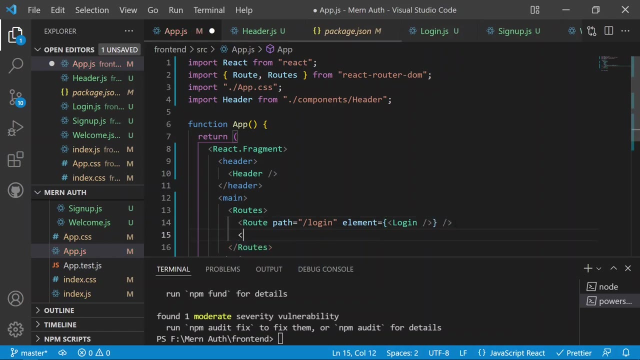 route inside that and then we can just provide the path of the route, like slash, as the login. so in this login we can just use the element, so the element would be the login component after that. so it will the login and then after that we can create another route and then it will the route again and then the path. 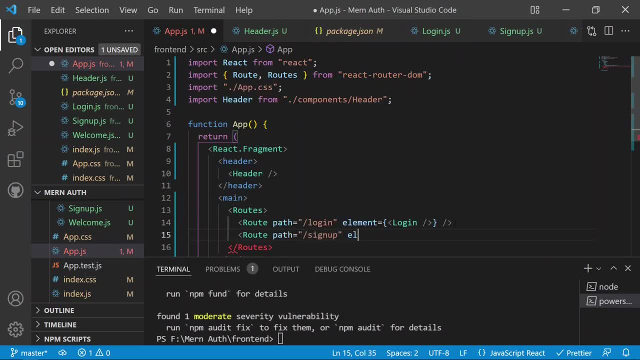 will be equals to the slash sign up with the react application and then we can provide the element. as the element would be like the, we can add a sign up element and then after that we can provide another tab like it will be. the route and Path will be equals. 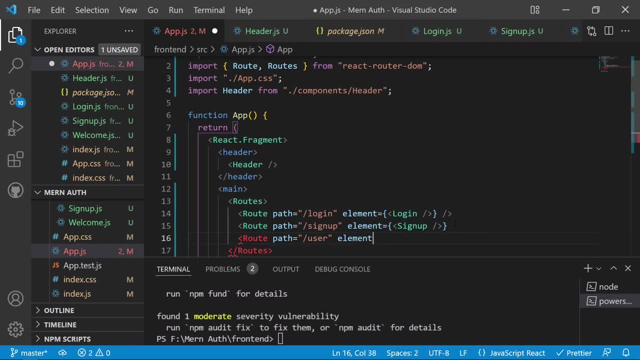 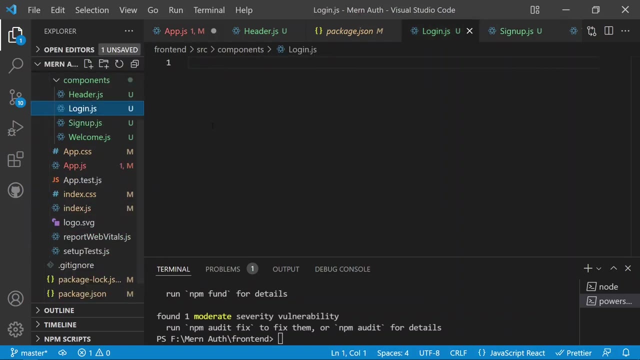 so the user will be having an element will be equals to the welcome. so in the welcome page we will show the user. so then we can define these components as well after that. so we need to go to the loginjs file which we have, and then we can just set a basic setup. after that, rafce and 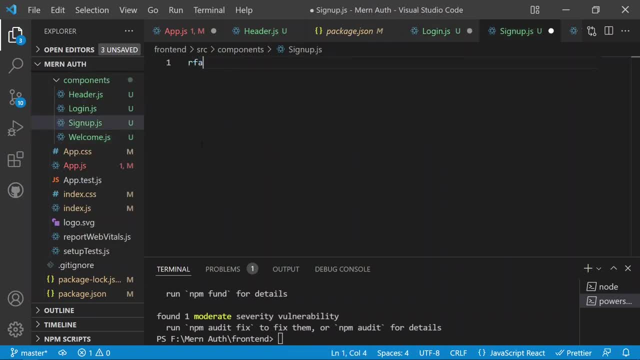 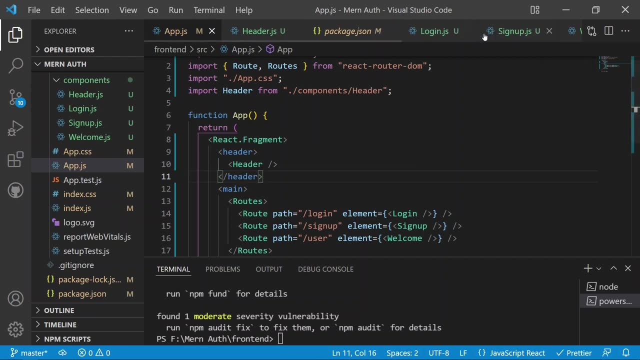 then we have a login and then we can have a sign up. so rafce, with the sign up as well, with the welcome as well, we need to add the rafce. so now we have defined the welcome page also, the sign up and the login page also, and then we can just import that also from the login. we can import the login. 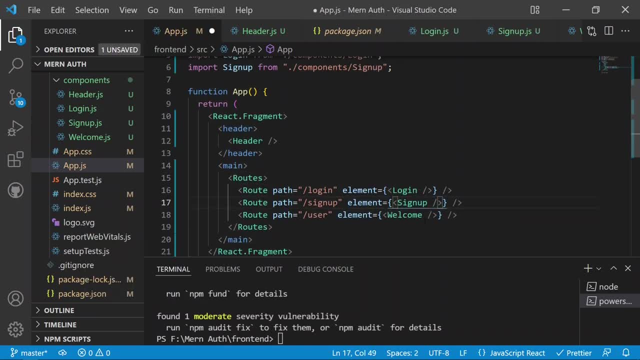 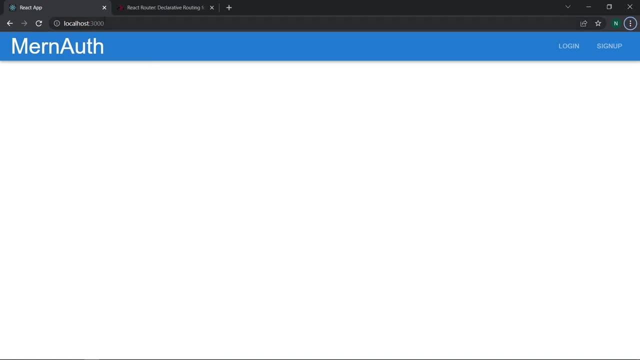 from the sign up, we can import the sign up and from the- i think- the welcome, we can import the welcome as well. so if i will now save, now we should see the changes onto the screen. so now you can see once i will move on to the login- slash login. so there should be the login page. 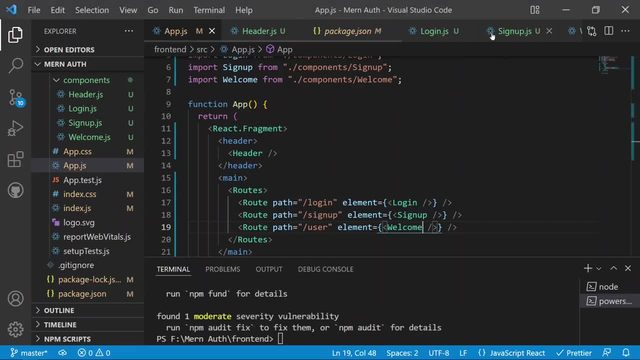 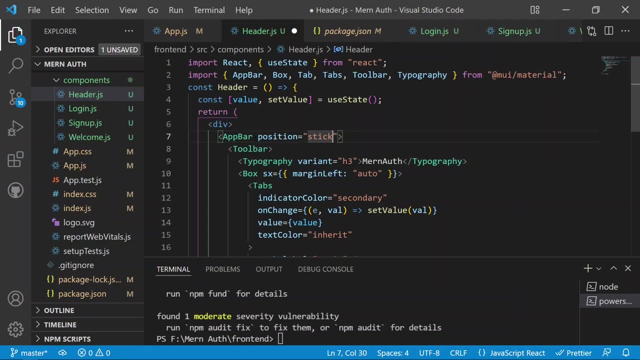 i think the content is hidden because of the bars. so we can just go to the header and then we can just go to the login page and then we can just go to the login page and we can just remove the position of it. so the position would be equal to the sticky, so that it. 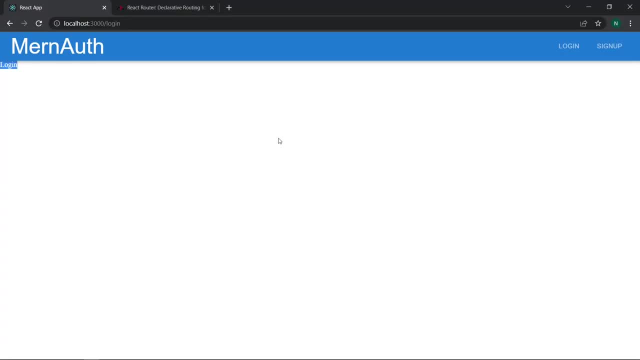 should be sticky to the top only. so now you can see we have the login. because the position was fixed, so the login was behind the app bar. and then now we can see if we can go to the sign up. so we should see the sign up page. now you can say we are into the sign up. 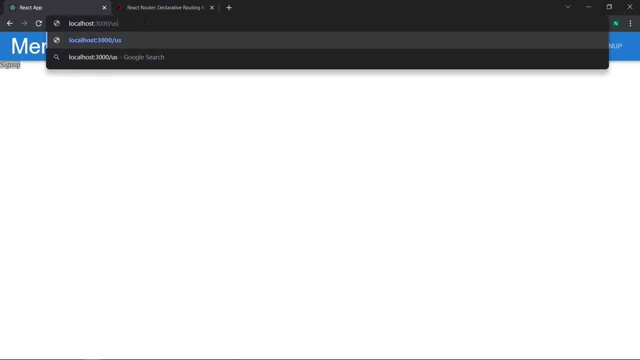 and if we are going to the user, so we should see the user details over there. now, you can see, now we have the welcome page onto the user, so now everything is working fine, so we can just fix that header. like: once we click on the login, we should reach the. 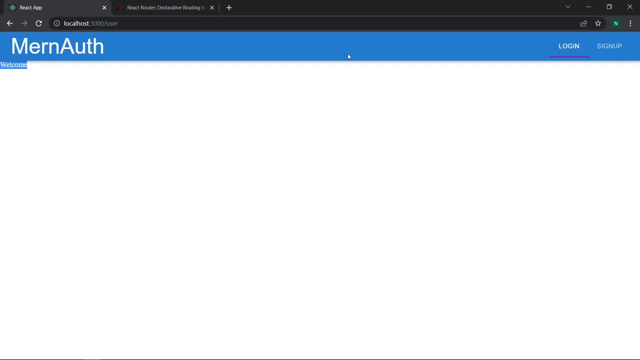 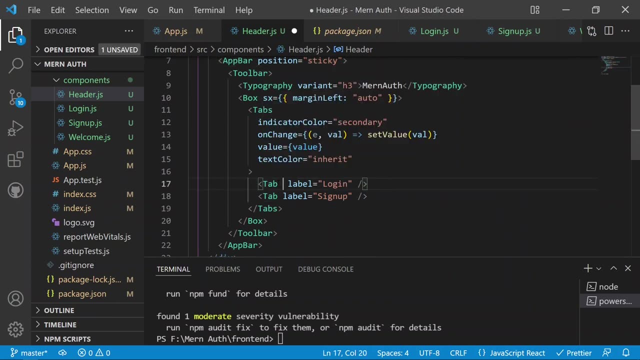 login route and once we will click on the sign up then we should reach the sign up. so we can just fix that functionality. so here in the tab so we can just add a component as the link component prop. so it will be having a link component and then we can just add a link component as the link. 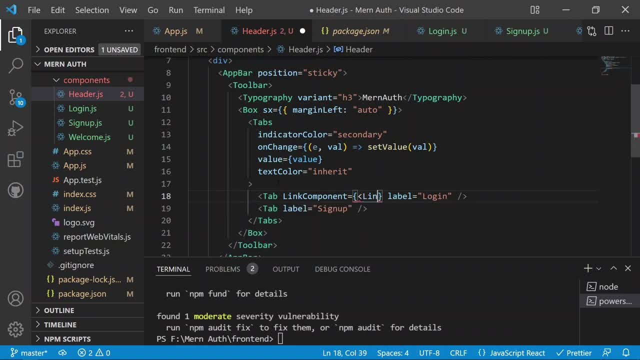 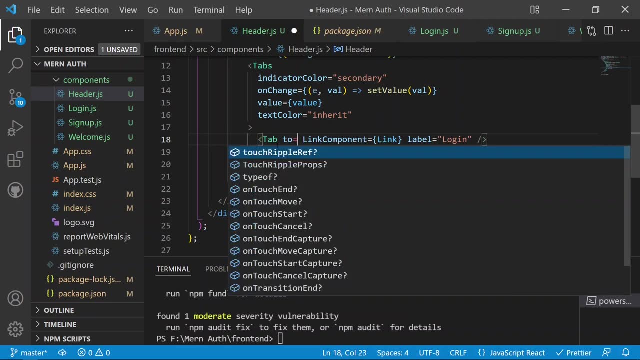 and it will be imported from the react router dom so we can just add here as the link component, so we can provide the two, because the links in the react router dom receives a two prop and then we can just use the two prop here in the tab now and then it will be the login. so it will 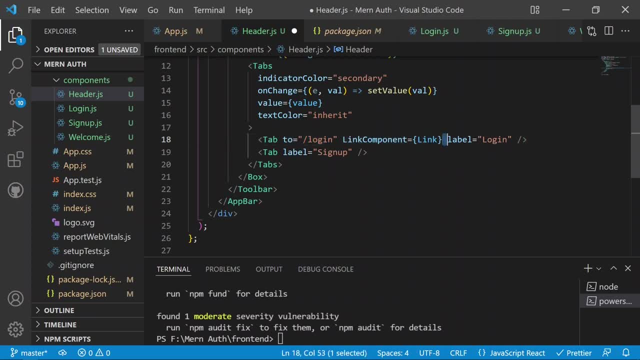 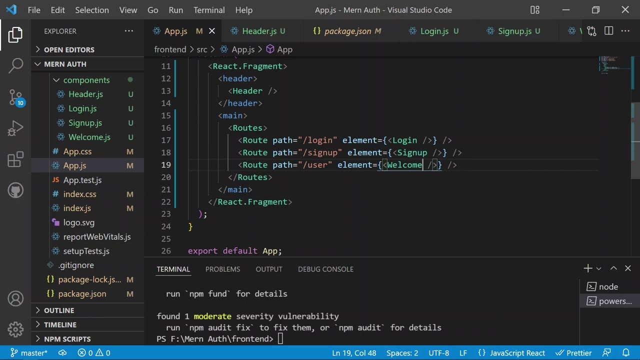 be acted like a link component now and the same. we can just use that component into the sign up as well, so it will be the two and the sign up, so it will be then moved on to the sign up. so once the tab will be clicking on the login, so it will reach the app component once again, and if the path is 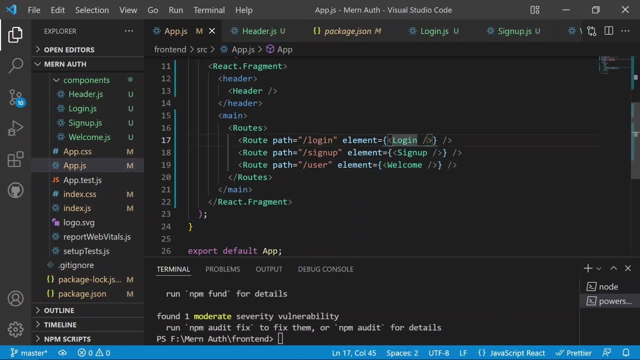 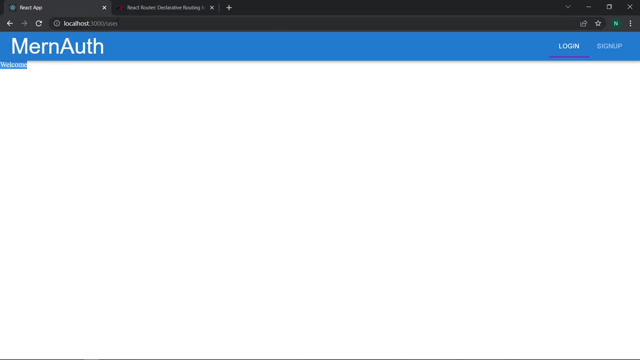 the login. it will then render the login component and the path. if the path will be close to the sign up, then it will render the sign up, and if we have the user path, then it will show us the user welcome. so now we can just remove that also. and now you can see, now we are in the default application and 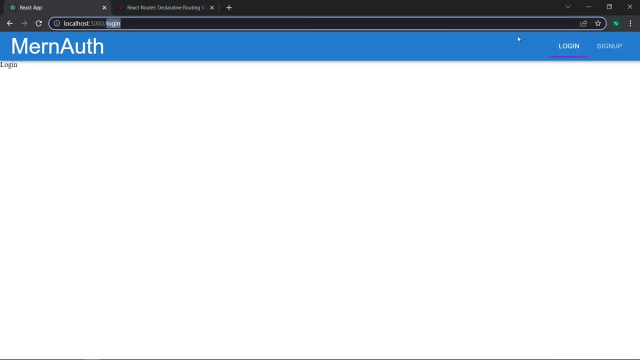 once I click on the login, so now you can see we are reaching the login route, and once we will clicking on this sign up. so now we are on the sign up path and without refreshing the page, and this is the big advantage of the react router dom- that we can now use the routing without refreshing. 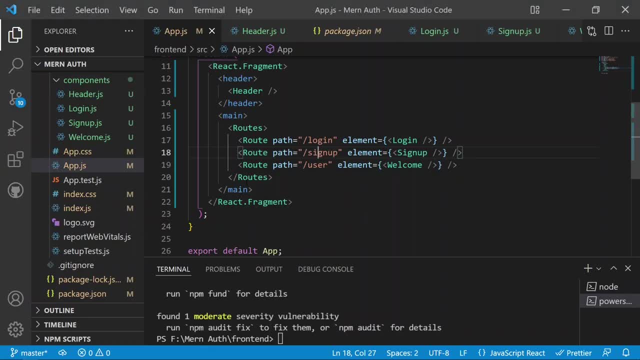 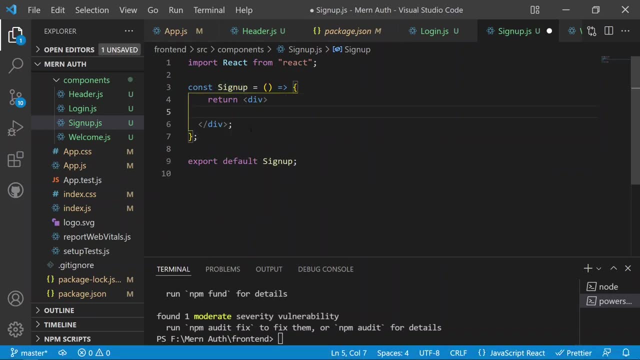 the page, because it's a single page application, and now we can build on the sign up functionality first, so we can just build that, so we can build the sign up forms here, so then we can just use the form tag here as the form, and then we can remove the action also and then in the form we 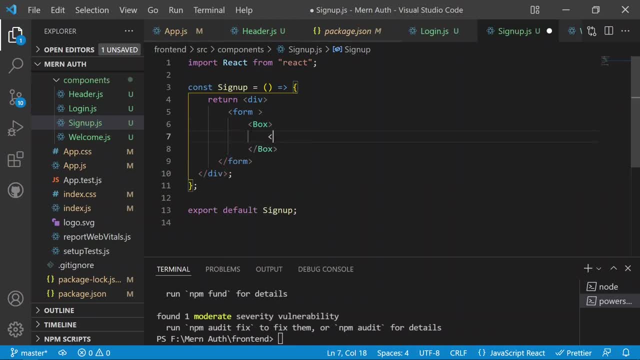 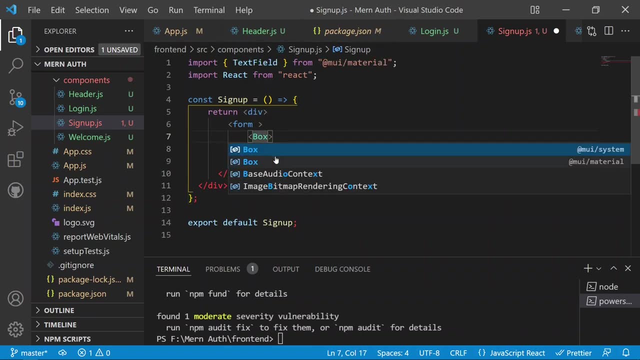 can use the box to provide some styling and then it will contain the text field from the material UI. then import it from the material UI, and we need to import the box as well from the material UI, so the text field. and then you can see: now the text field is there and then we can just provide another. 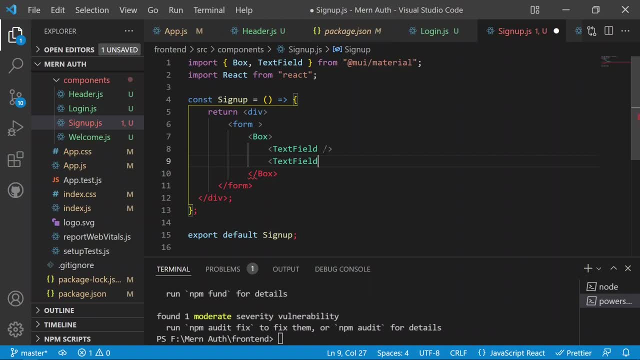 text field there, because we have the three text fields over there, so the text field two and then the text field three. so now we have the three text fields and then we will having the button over there. so it will the button. and the button will also be imported from the material UI and it will. 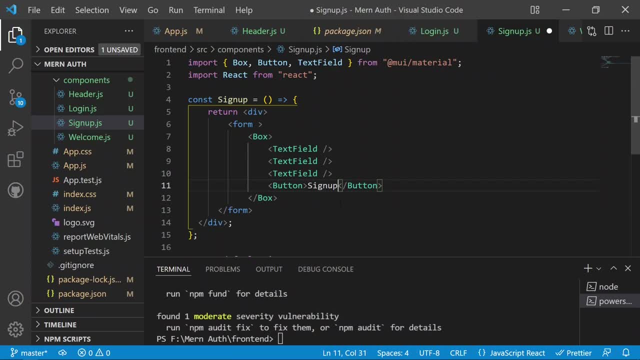 contain the sign up there. so now we are in the sign up and now you can see, now we are in the box and then we have the three text fields and then we have the sign up and then the type of it will be equals to the like submit, because we are in the form and then we can just add the on submit. 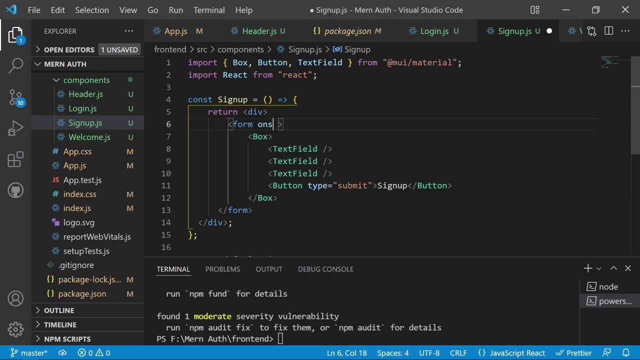 to the form also. so when the form will be submitted, so we will be having a function to control the submit, so we can just add a handle at the submit, so we can have this function as well. before that, so we can have a const as the handle submit will be equals to the function. 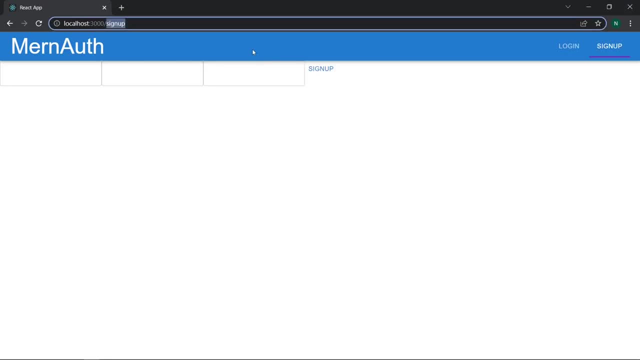 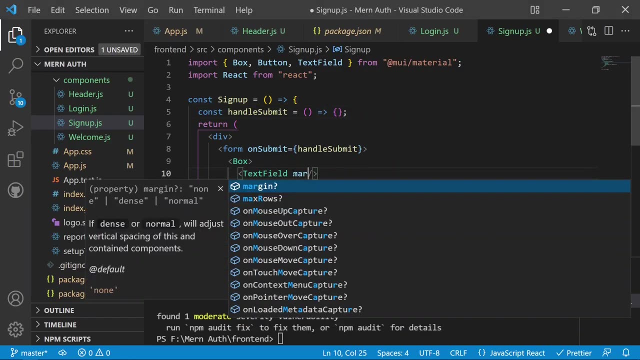 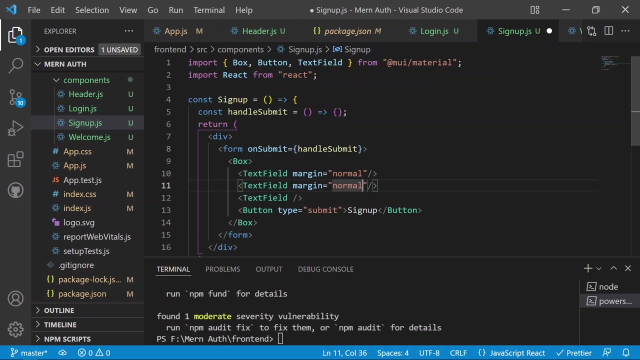 now you can see, everything will work fine. so if I will now save, so now we should see the form over there. now you can see, now we have the form and now we will have some styling over the form. like the stack field will contain the margin as the normal, and this will also contain a margin as the normal, and 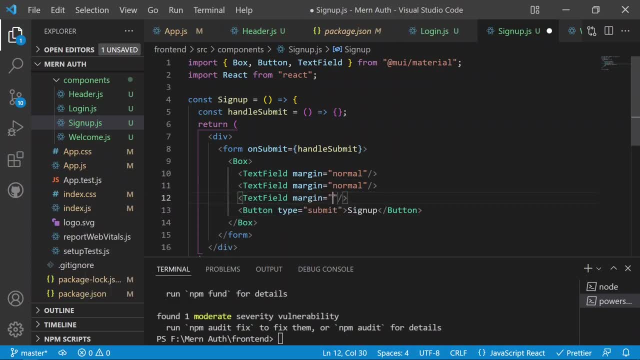 this will also contain the same as the margin, as the normal. so now we have the margin and then in the box we can just provide the display as the flex and then we can just add a flex direction to the column. so if I will now save, now we should see the change onto the screen. so now, if I will, 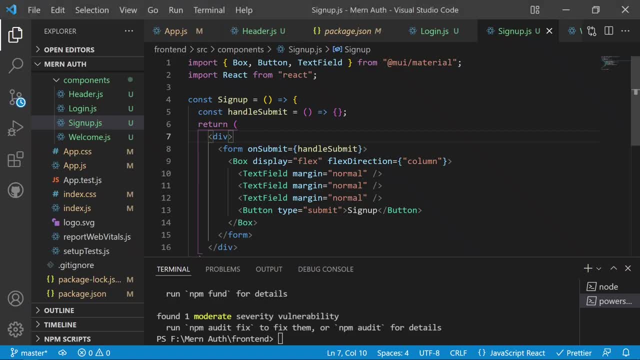 now save. now you can see, now we have the text fields and now we can just define the size of the box also, so the width drop into the box, so the width can be caused to like 300. so if I will now save, now, we should see the form as the 300 pixels and then we can just add a margin left. 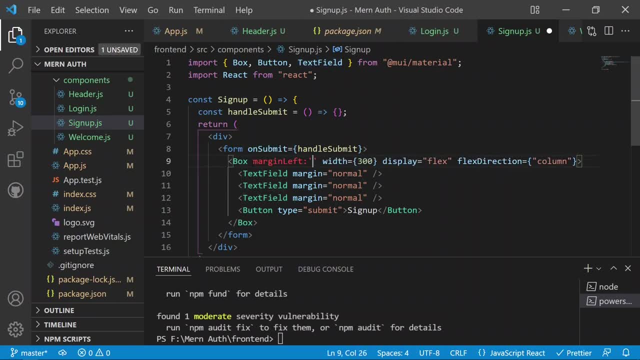 so it will contain the margin left, so it will contain the auto. we can also provide the margin as the right and it will also be the auto. so it will be in the center onto the screen. now you can see, now the form is in the center and 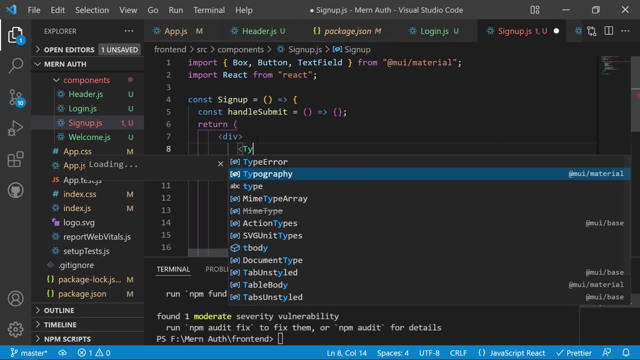 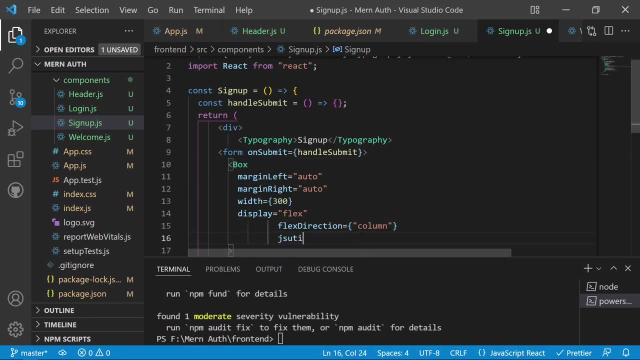 then before the form we can just add the typography as well, to add there like typography, like it is a sign up, and then in the box we can just add the justify content also, like justify as the center. so the form will be aligned into the center and the align items. 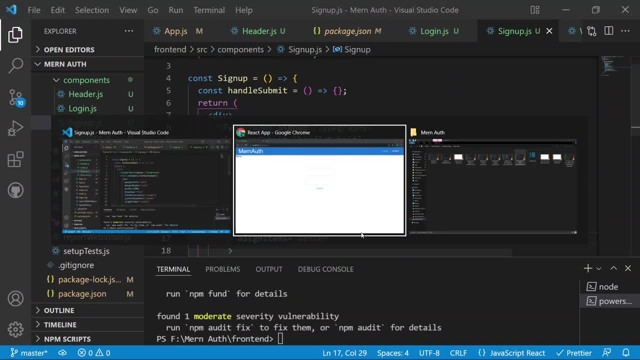 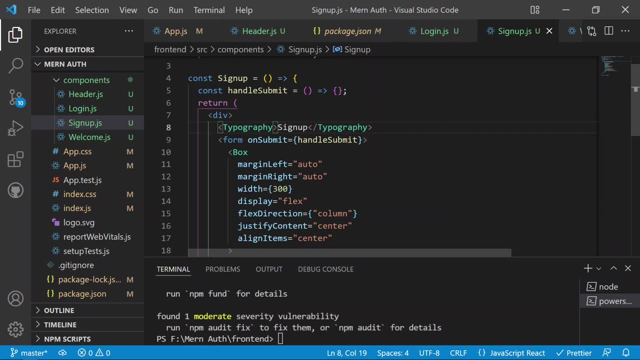 will also be equal to the center. so now we should see the changes onto the screen now. so now you can see, now we are in the sign up and now we can just add the typography with the variant will be equals to the h2 and then the variant will be added inside the box. oh, so, after the box we 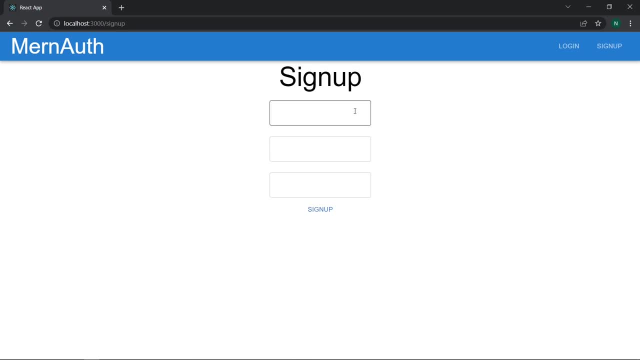 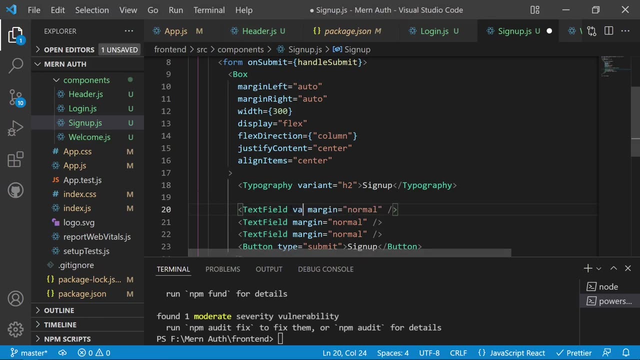 will having the variant. so now we should see the changes onto the screen. now you can see, now we have created the sign up form and now we need to design the text fields of the form. so we can just define that. so the variant will contain as the outline and then we can just add their- uh, placeholder. placeholder would be like: 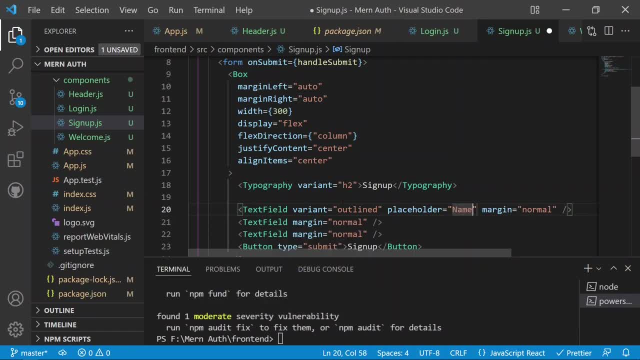 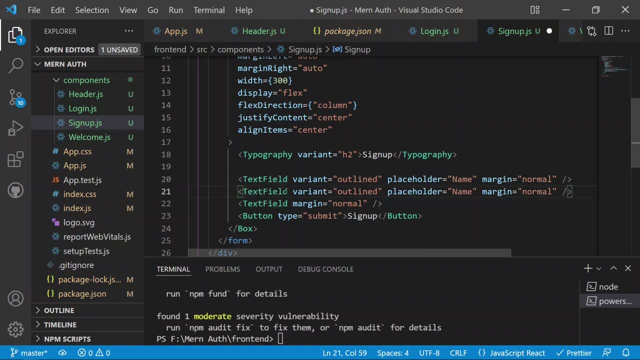 we can define here the name and then we can define it the values as well. so but we can define the variant and the placeholders to there as well in the text fields there. it will be having a variant outline and the variant outline there also and the name. it should contain the email and it should 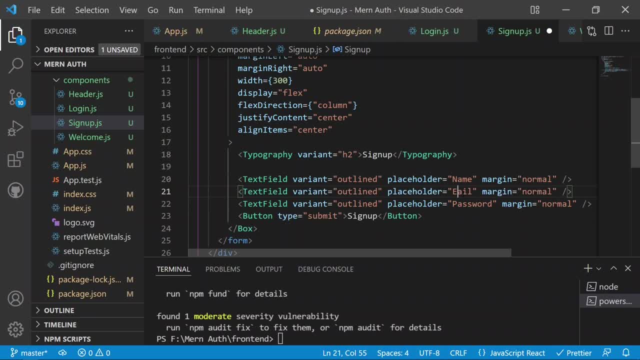 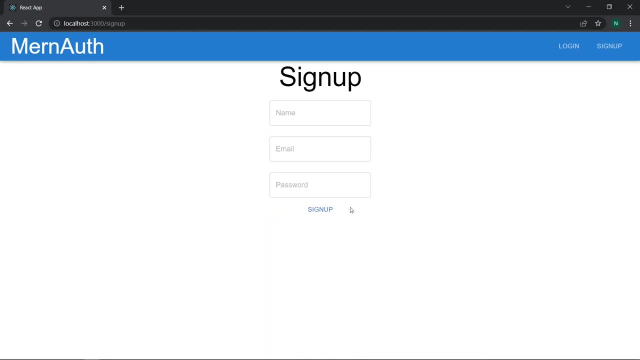 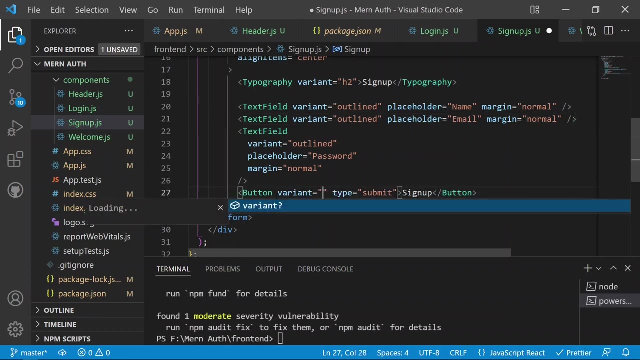 contain the password. so see the changes onto the screen now. you can see. now we have the name, we have the email and we have the password into the forms and we have the button as well, of the sign up, and then the button can contain a variant. again will be equals to like the content. so the button will be filled up with the. 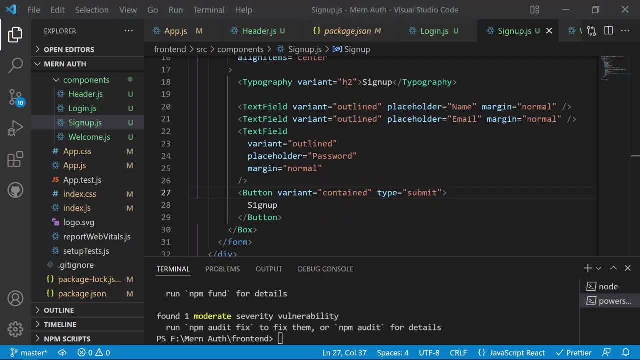 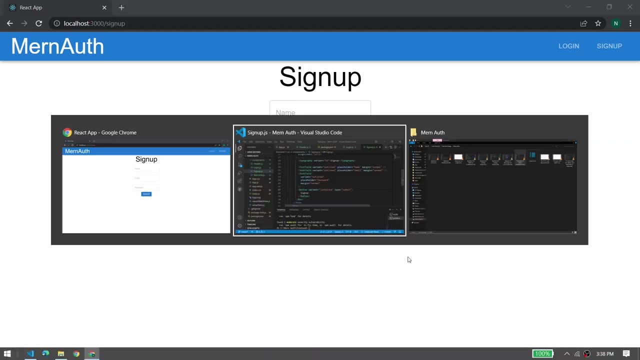 color. now you can see, now we have the sign up functionality over there. now the sign up functionality is completed. now the form is now designed and now we can just use some state to control the form and to use the state we can just move on to the uh react application. 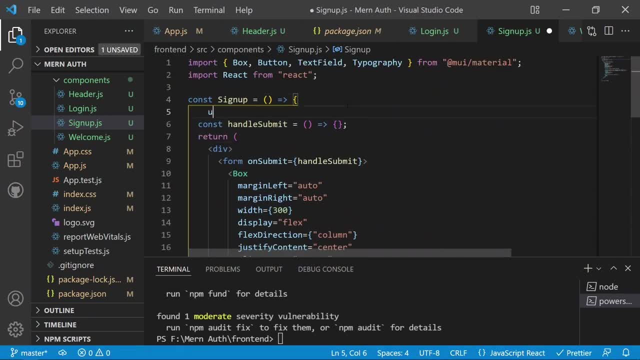 once again, and we can define here this state, so we need to define here the U state to handle the form, for the U state would be there and we can define some inputs to the form. like now: it will be having the inputs and then there will be the set inputs and then we will be having an object. 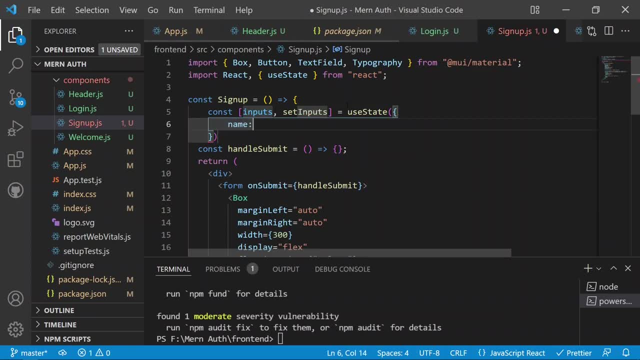 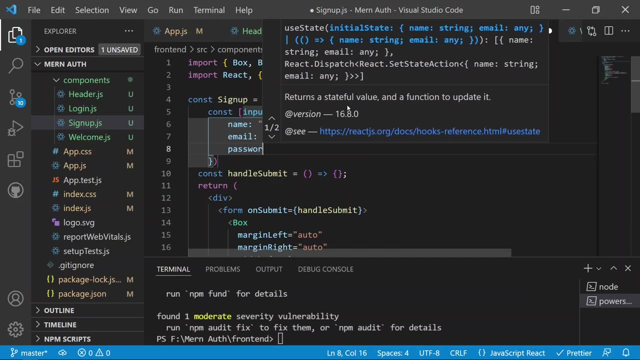 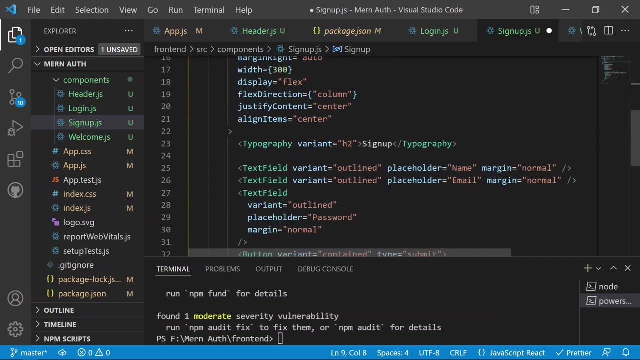 so the initial value of the state will contain a name, and the name property will be caused to the empty string and the email as well. it will contain the empty string and the password as well. it will contain the empty String as of now. we are now defining the state with the empty string, and then we can define a values to. 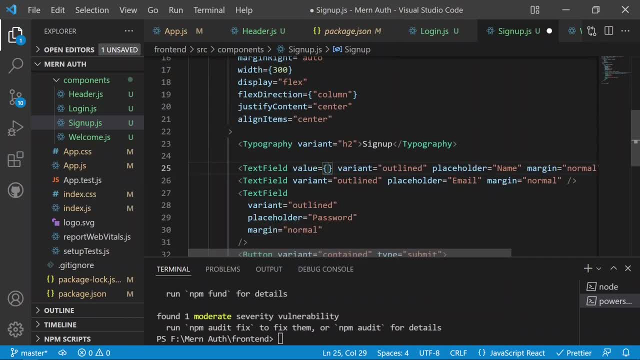 the text field also, like it will be having a value of the inputs that we have: input, subject, state, dot name and then inside the value here, so it will be equals to the inputs and it will having inputs- dot email and then we will be having a value again to the password. 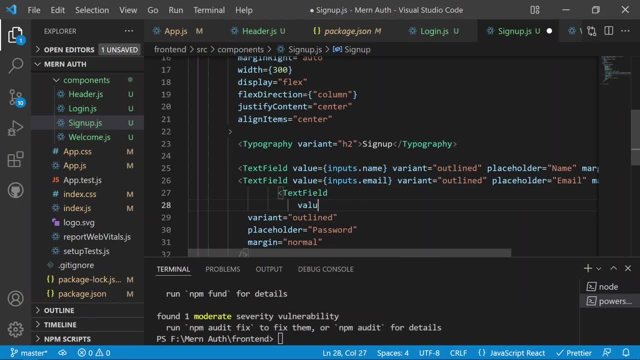 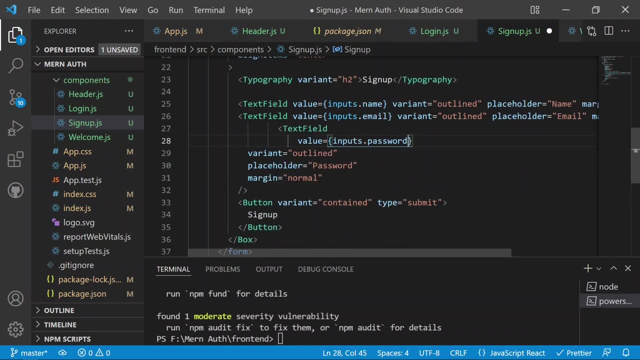 as well. inputs will be equals to the inputs dot password. so now we have seen everything and now we can define a onchange functionality also for that and for the email we can provide the type also, like it will be after type of the email and for the password the type will: 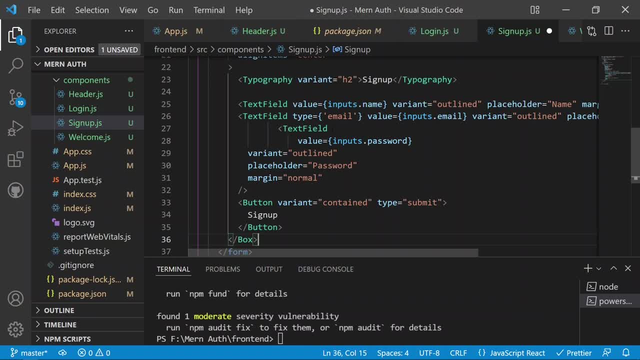 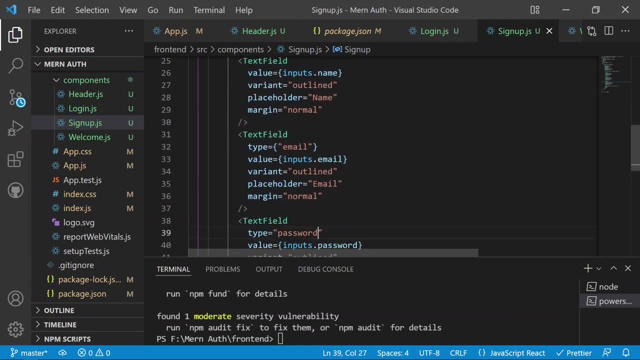 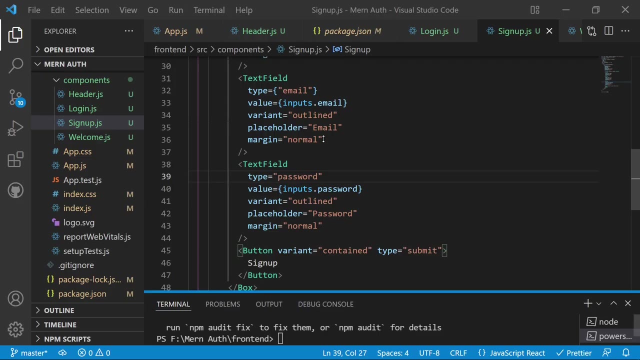 be the password of that. so i think the password field is there so we can define a type as the password. so now we have defined everything. so now we have define three textfields and then we have defined a button to sign up and now everything is working fine. now you can see, now we have the name, email and the password. 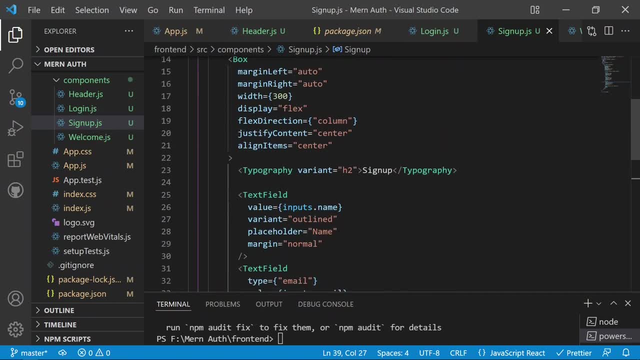 field, and now we can define a function to change the values of the text field, so we can define a onchange. so whenever the change will occur, so it will be having a onchange function, so it will handle change, so it will change the values of the inputs, so we can 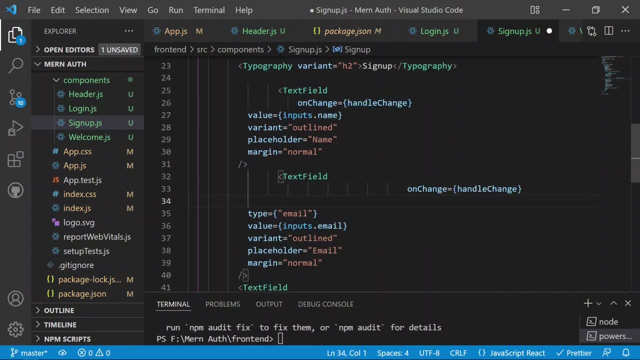 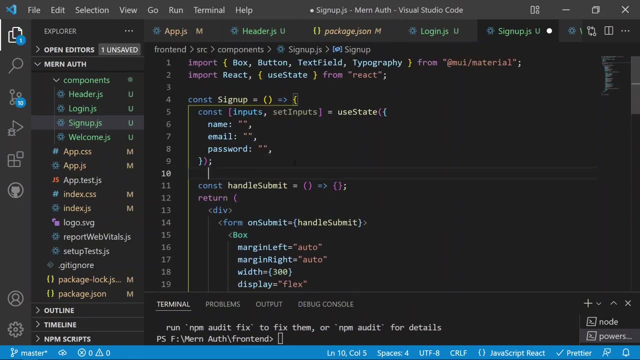 define a onchange after their text field as well, after this text field as well, and we after this text field as well. so now we can define a handle change function. so it will be the const, as the handle change will be equals to the function and it will be having a e as the parameter. 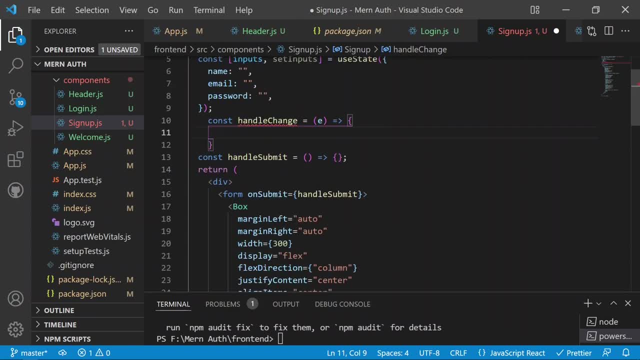 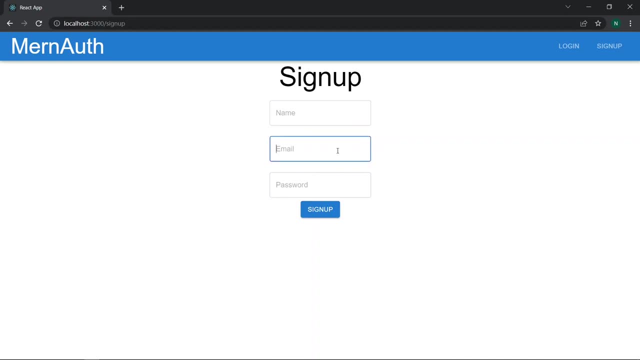 and then we will be having all of the things there and now we should see the changes onto the screen, because we have defined some function and now everything should work fine, and now we need to handle the state into the handle change function. so for handling the state we can define, 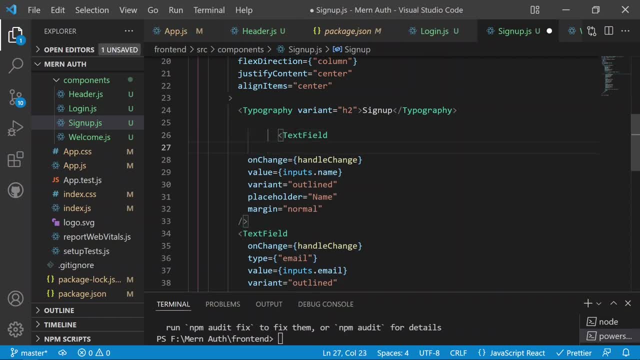 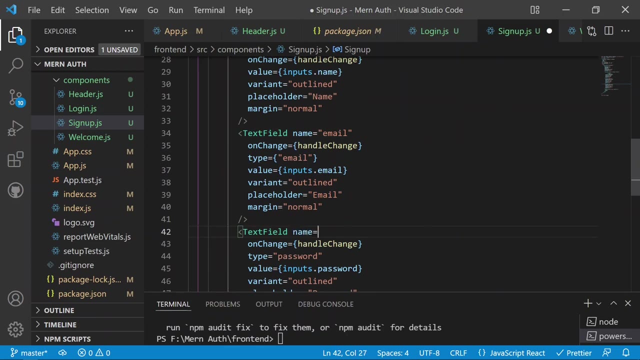 an identifier to the text field, like we can just identify the text field with their name or with the id. so we can define a name as this and we expect it will be the name, and then we can define here the name as the email and it will be having the password, so it will be the name equals to the. 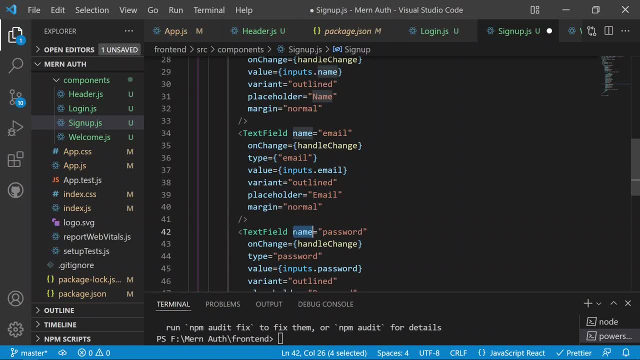 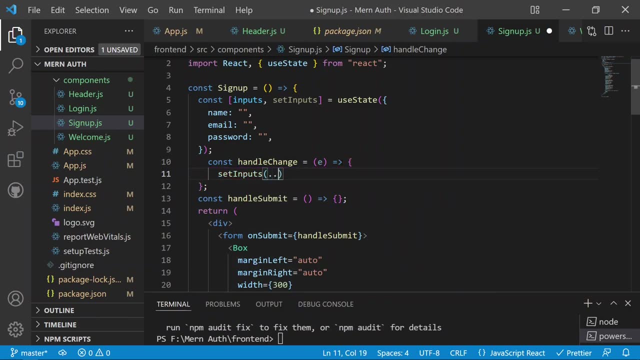 password. so now we have defined the identifier of the text field with the name and then we can just check and we can just set the state from there, like the set inputs, so it will contain the previous state you, so we need to just render the previous state first for it. 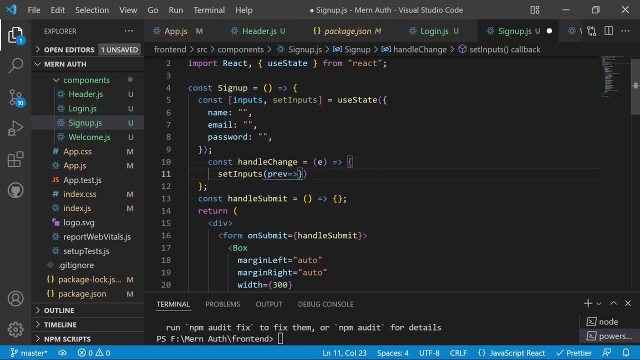 and then it will be having the previous state first, so it will be having an object with the previous state, and then we will be having the state here with the actual state. so here we will target the property names like e, dot, target, dot name, so the name of the text, field name. 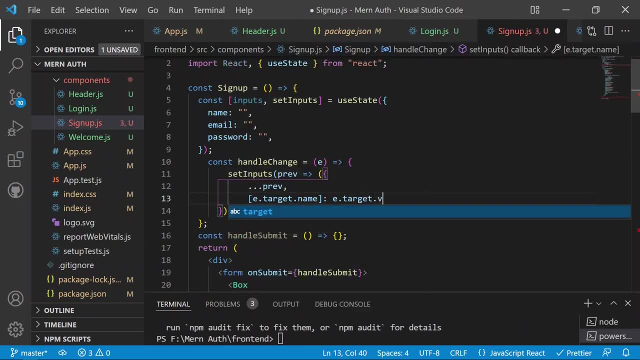 of the input and then the e dot target dot value. so if you don't know about this technique, so you can just console dot log it. so if you will just console dot log the e dot target dot name and then the value, so it will be the e dot target dot value. so whenever the field will be changed, so it will. 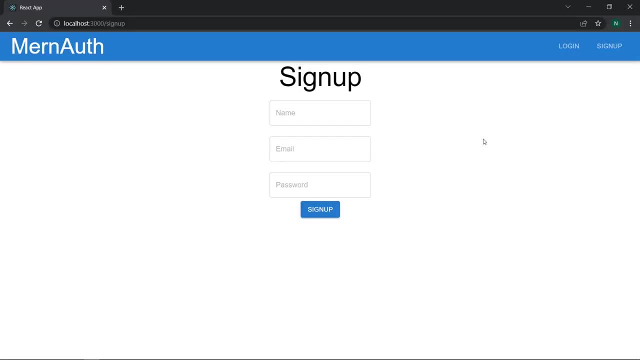 just target all of the things and now we can just go to the screen and we can just go to the inspect to check if everything is working fine. you can just go to the console now you can see, once you will provide the name like aabc. you can just go to the console now you can see, once you will provide. 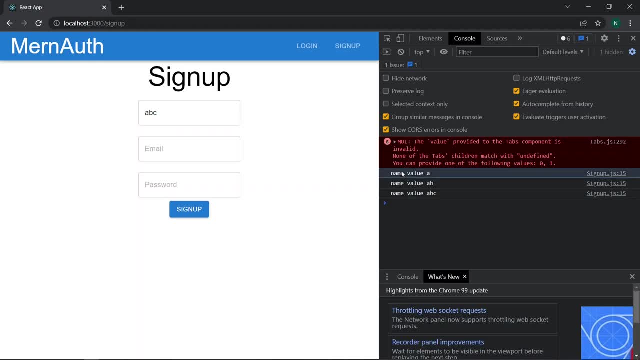 the name like aabc. you can just go to the console now you can see. once you will provide the name like aabc. now you can see the name. have we have the name of the name and then in the email once you will get anything, so you will get the identifier of the email, as the name and the value is equals. 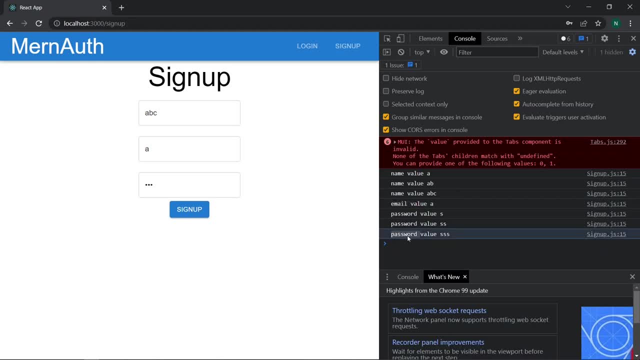 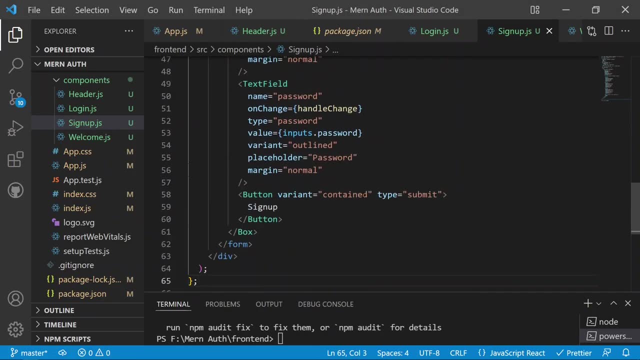 to the a and you can just check the identifier of the password and the value equals to the sss. so now we can just see everything is working fine here and then we can just handle the states here. so now you can see we have defined here some states and we can just remove that console log here. 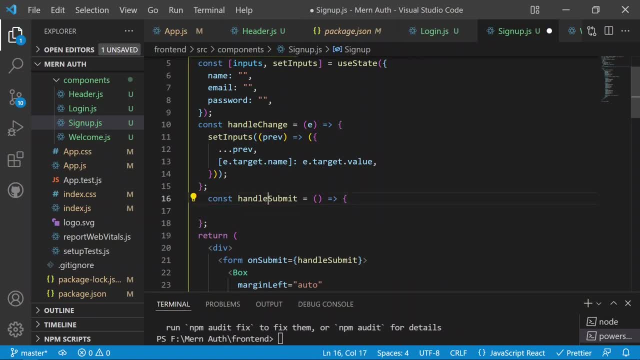 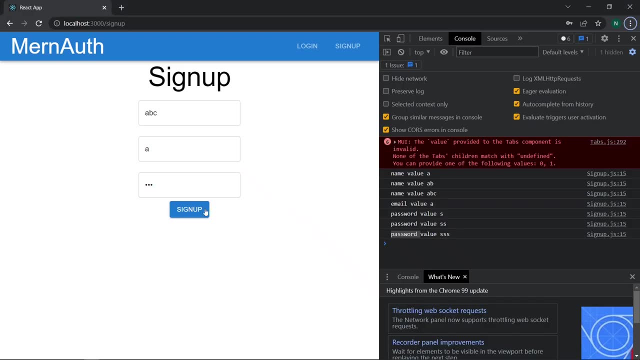 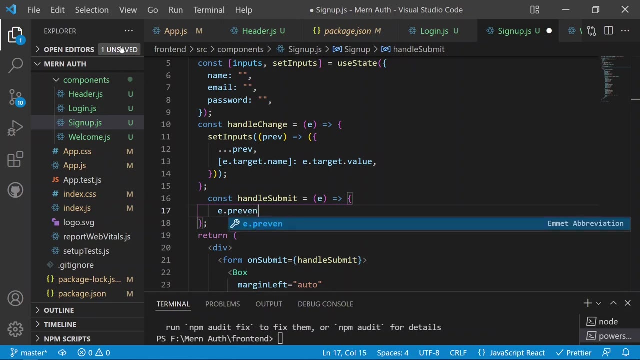 and now you can see once the handle submit would be there, so it will contain an event inside that. and then we can just prevent the default behavior of the forms in the html that once we will click on the sign up or any submit button, so it will send the form data and it will just refresh the page. so we can just prevent the. 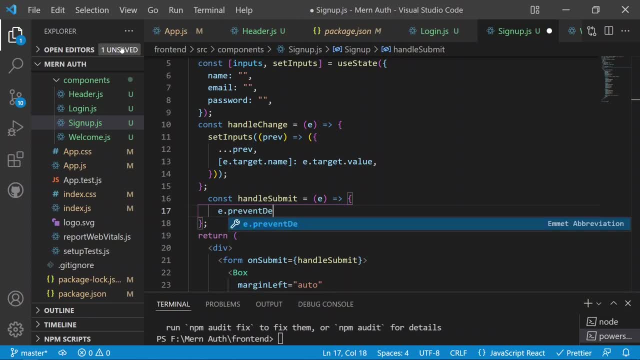 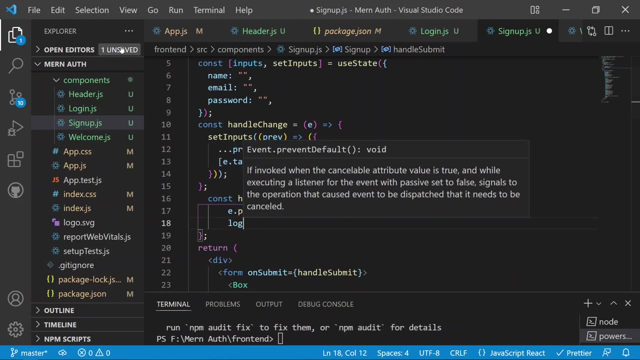 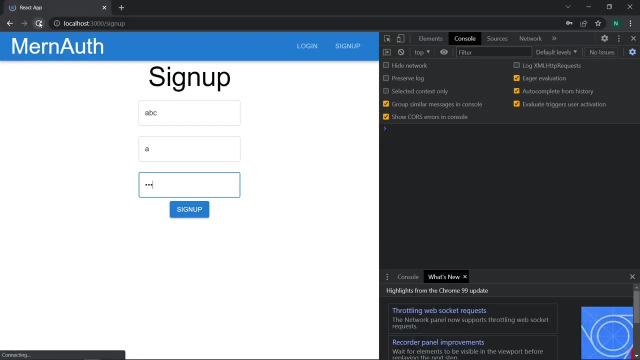 default functionality from the prevent default function. so we have a prevent default function, so it will just prevent the default functionality of that and we will just consolelog the inputs that we have. so we will just refresh the page and then we can just check again. like the name, i will add my name, nikhil. 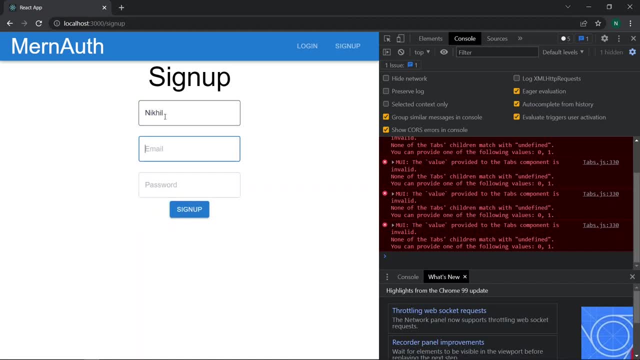 email as the abc at the rate test dot com and then we will have a password like one, two, three, four, five, six. so if i will click on the submit now, you should see the changes now. you can see. now we have the name object with the name as the nickel, the email as the abc at the rate testcom, the. 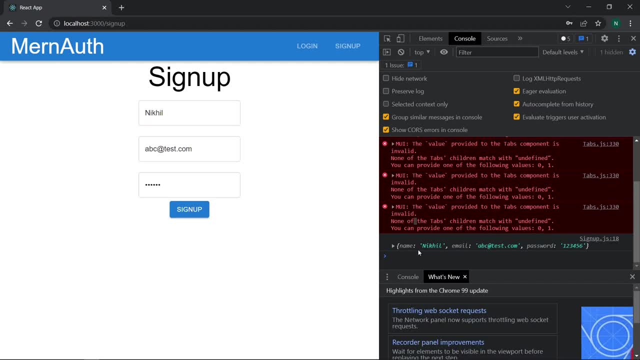 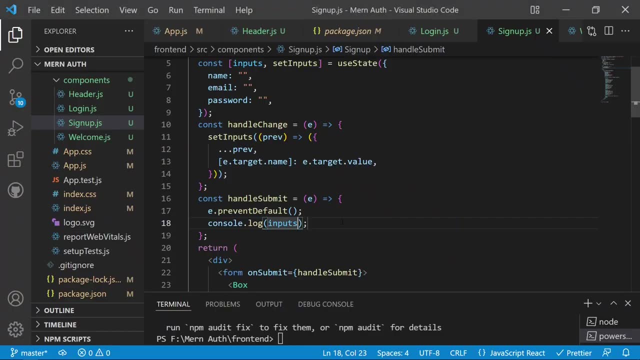 password equals to the 123456. so now everything is working fine, and after that you have the default style of the object, which is called the name of the object. when you click on that object we can just send the HTTP request. so now we can send the HTTP request there, and for that we can just install. 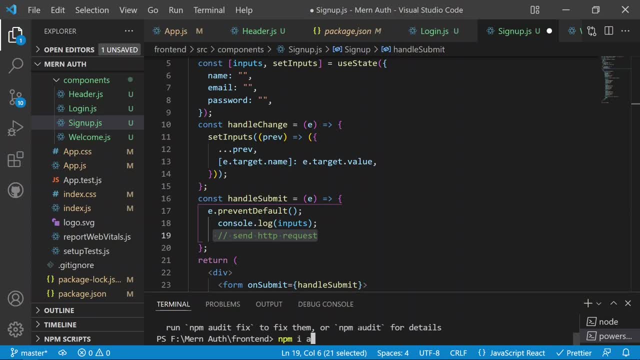 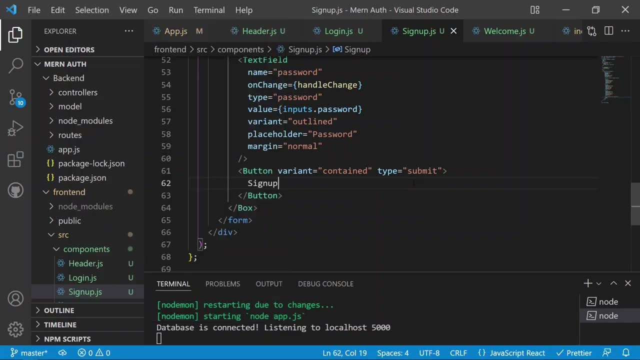 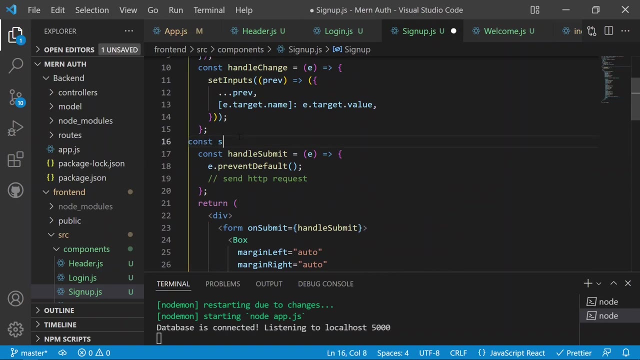 the XCOs from there so we can install the NPM, install XCOs to send the HTTP request. so the XCOs is now installed and now we can send the requests. so we need to go to the handle submit function and then we can just send a request here. so we can just create a function to send the. 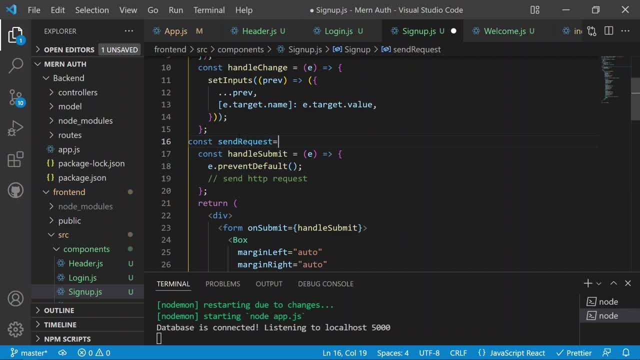 request at this send request and it will be equals to an async function. so it will be an async function and then we can just send the request from this function. now and now we can just declare a variable as the cons, as the response, and it will be the response which will send the request to the server. so it 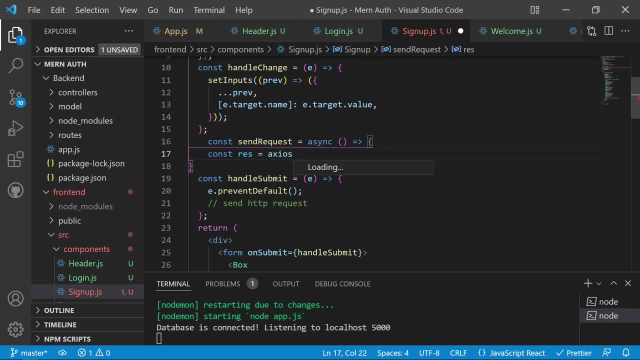 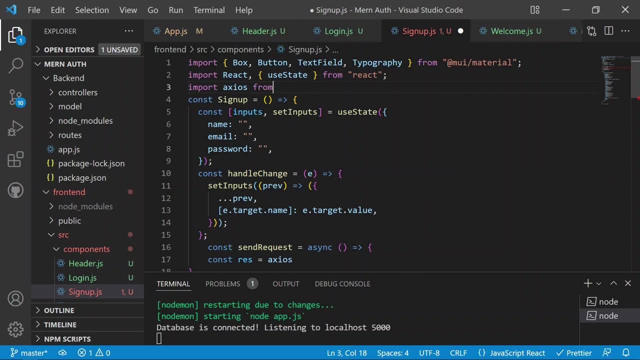 will be equals to the XCOs which we need to import. so the XCOs will be then imported. so we need to import the XCOs from the XCOs, so we can import the XCOs from XCOs, and then we can. 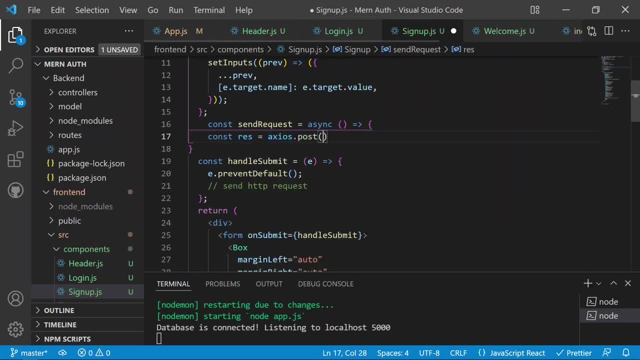 use the XCOs to send the request. like XCOs have a post function, so we can send a post HTTP request. so the URL will be HTTP slash, localhost and at the rate of the port of the 5000 slash, we have the API slash in the signup. 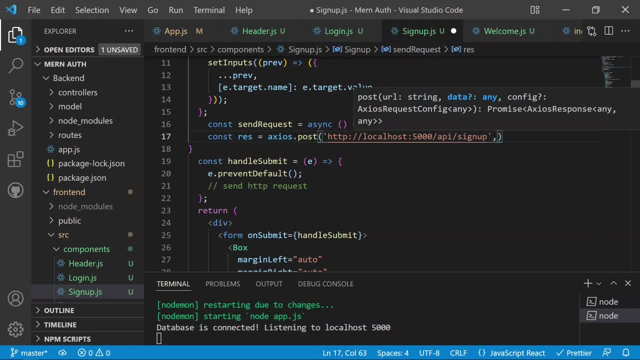 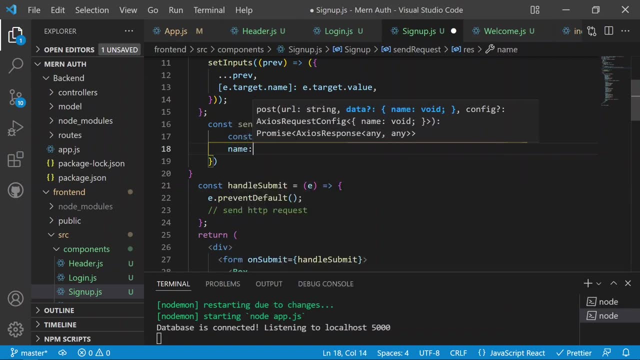 so now we are sending the signup request and in the second argument, then we need to send the data, and the data will be equals to which we need to send the data as the requestbody, so it will be the name. we need to send the name as the. 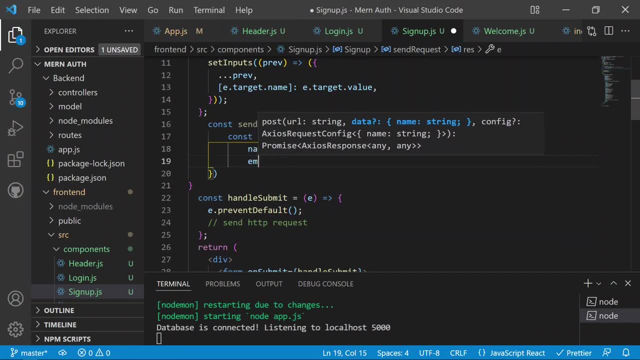 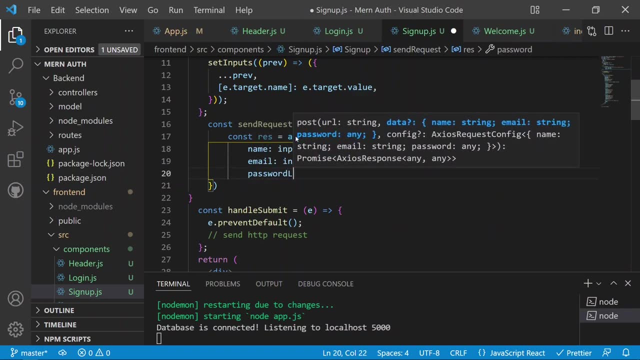 inputsname, and then we can send the email as well. email equals to the inputs Dot email- and then we can send a password, a password as inputs dot password. so we will send the data now in the request and then after the response. then we can add a clause statement of it also, because it is a promise, so we can. 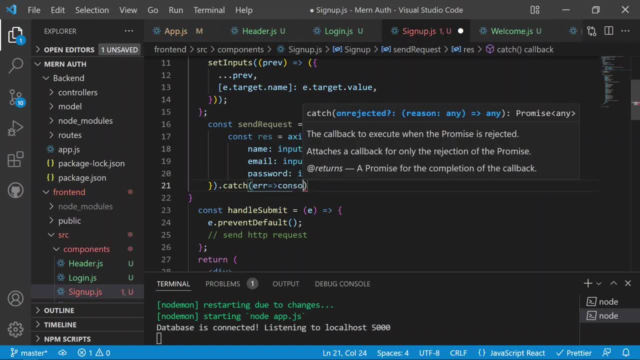 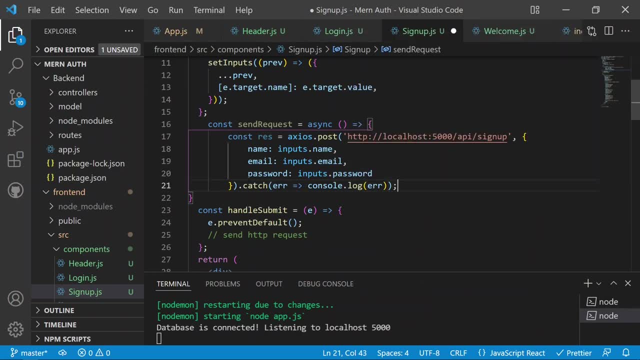 have a clause statement and we will have an error in the parameters and we will just console dot lock the error which we have. so we are now sending the error and then we are now solver logging the error and then it will be an asynchronous task. so we need to add the await as 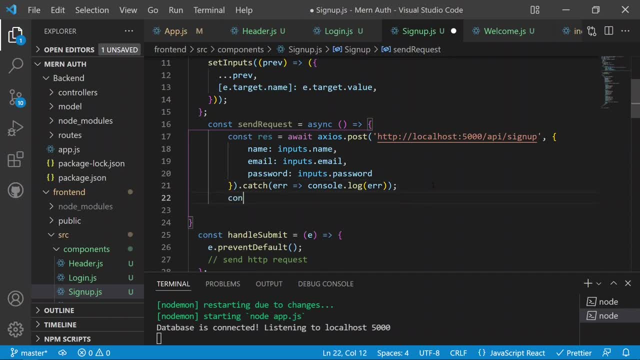 well, so it will be the await and then after the request, then we can get the data from the request. so the request. so to get the data from the request, we can declare a data variable and we can just get the await as the response which we are sending dot data. so the response. 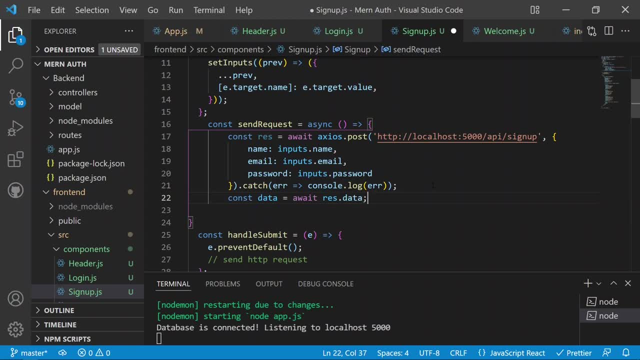 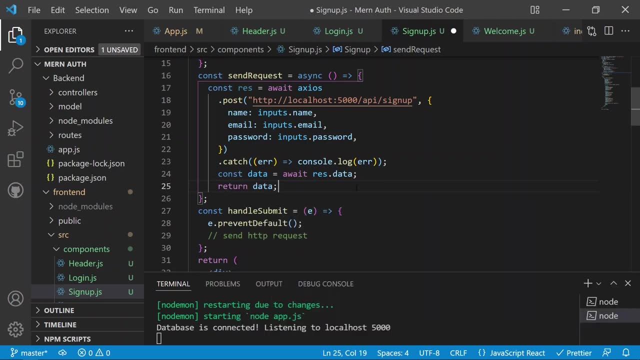 dot data is the property in the xos which gives us the data in the response which we will receive from the backend. and now after this, then we can just return the data over there- return data- and then after that in the handle submit function, now we can send the request. so it will just send. 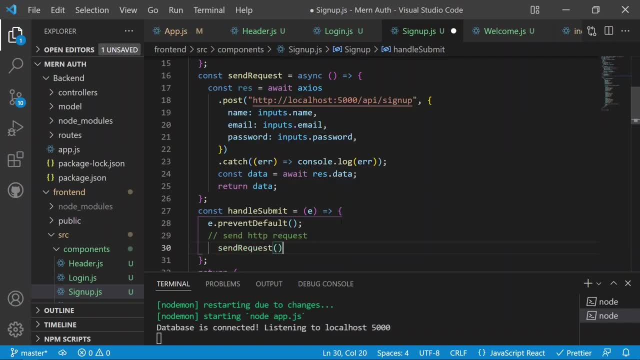 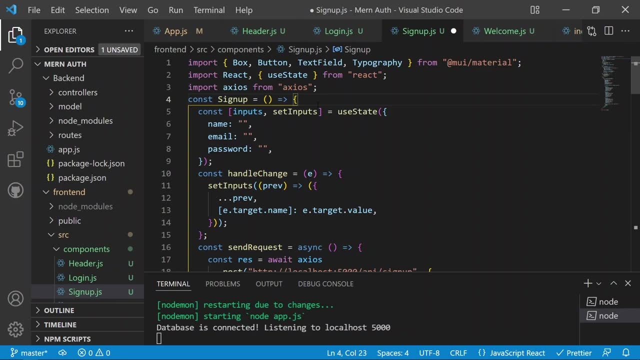 request. so we need to call the send request function and then after that we can just redirect the user to the login. so after this sign up is completed, then we need to redirect the user to the login so we can use the history to use to redirect the user. so we can just declare history. 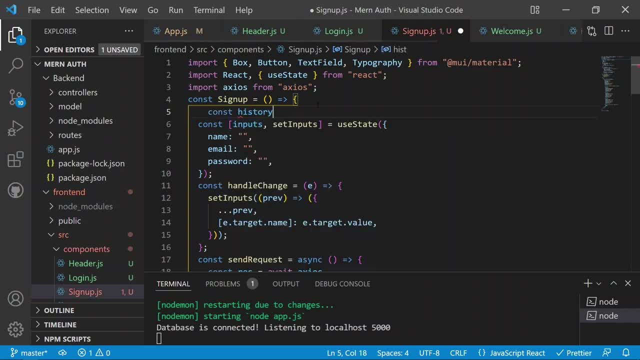 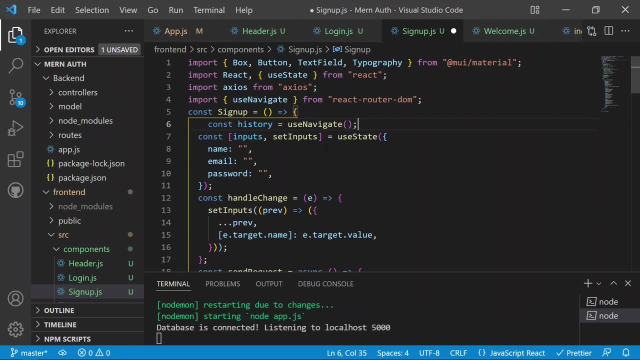 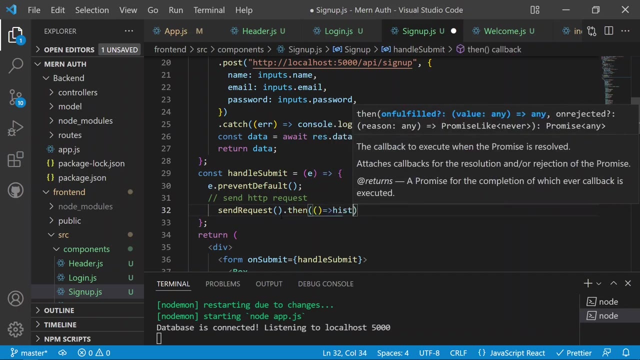 variable and the history will be equals to will be goes to the use navigator. so we have a use navigator from the react router, dom, so we can use that to declare the history and after the then statement we can use a history as well after the then inside that and there will be a callback function and we need to call the history. so 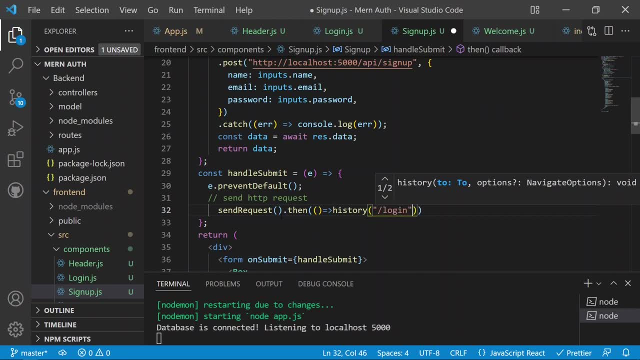 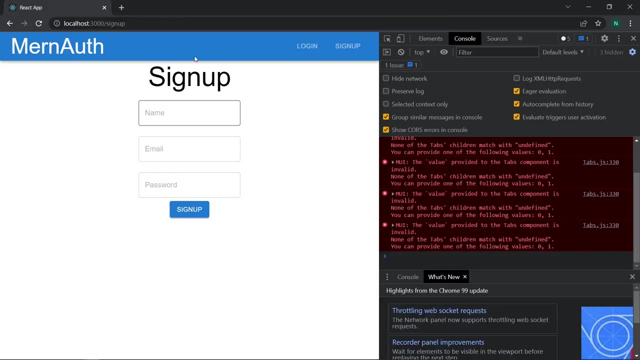 history will be there and after the history we need to redirect user to the login. so now, if everything would work fine, then we will be redirected to the login. so if i will now save and if i will now just go to the react application once again- now you can see, i will now refresh the. 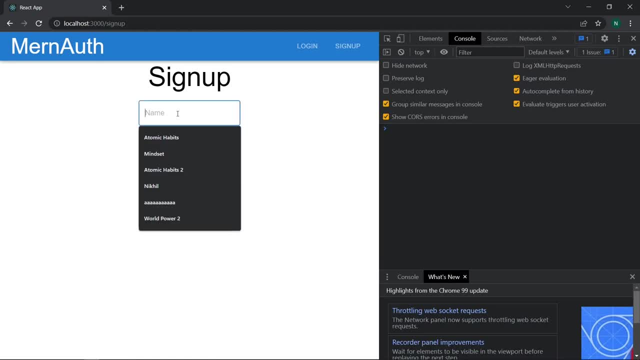 page and i will now just clean everything from the console. i will add the name as the nickel once again, the email as the nickel at that- test1.com, and the password will be 103456 if i will now click on this sign up. so now we should see all of the details, but i think there. 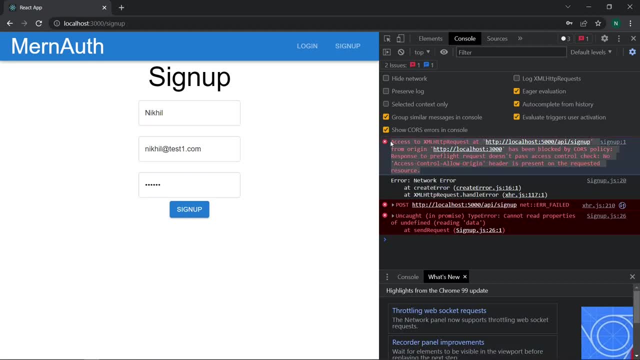 is an error, and this error is because, because we are now accessing, we are now sending the data from one server to another server, and the another server don't allow us to accept the data from the different server. so we need to allow that access, because it is a. 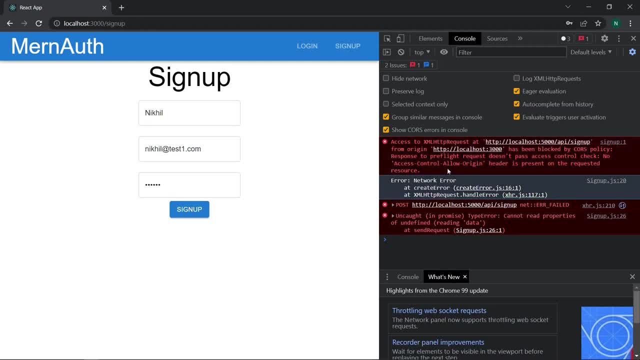 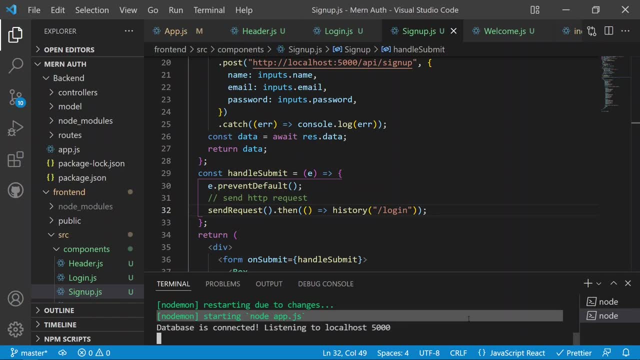 access controller origin and we need to add it to the allow only to from anywhere, so we can just access the allow from anywhere. we can just use the forced from the backend, so we need to stop the backend server from there and then we can just go to the backend application in the appjs. 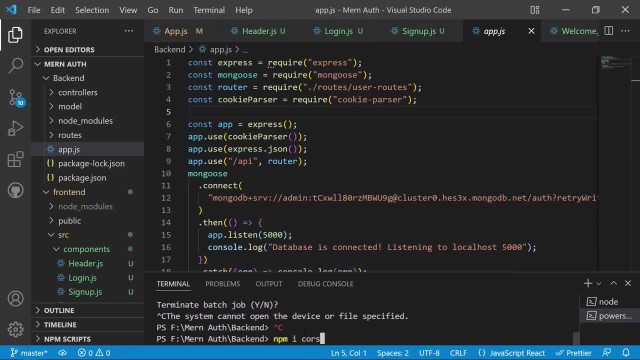 and then we can just install the course. so we need to install the course package to just remove this error and the course package will allow us to just allow access from anywhere to the origin. we can use the cort as well. so const will be cost. we require and the require will be having the course. so now, the course is now. 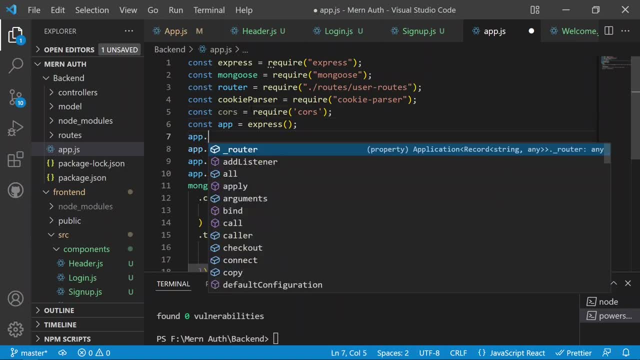 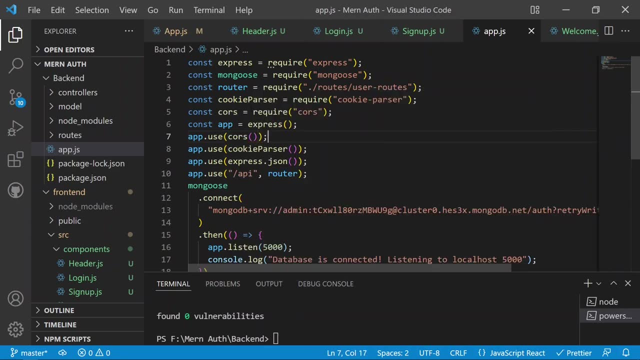 required. and now, after the apt-ret use, so before every middleware, so we can use the course, that will be the course. so we need to run the course function which we have imported. so now, after all of this, if i will now just save and if i will not just start the server of the backend again, 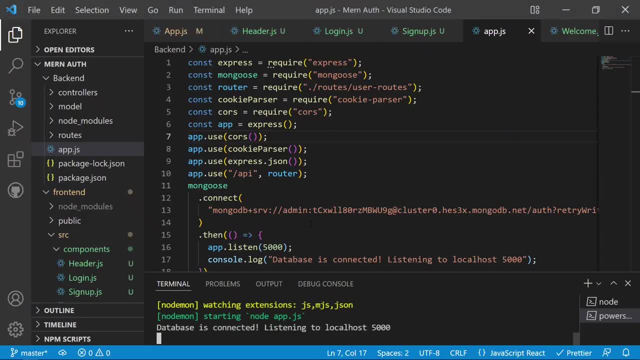 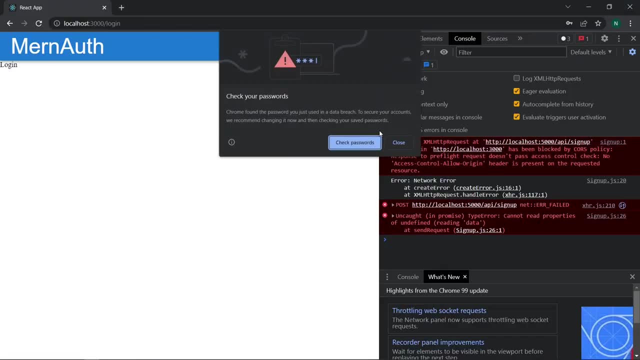 and now we should see. everything should work fine now. so now the database is connected, listening to localhost 5000 once i have a click on the sign up. so now you will see everything is completed and now we are redirected to the login, and now the user is already created there and now we need to. 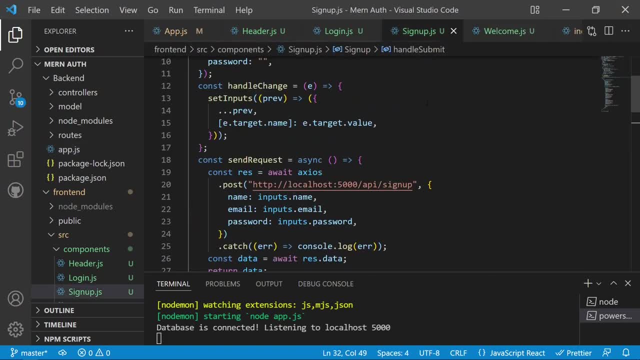 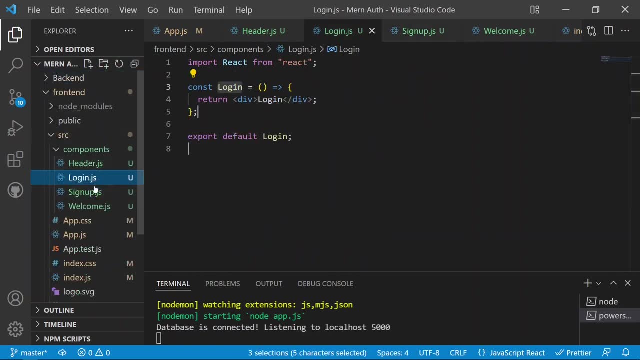 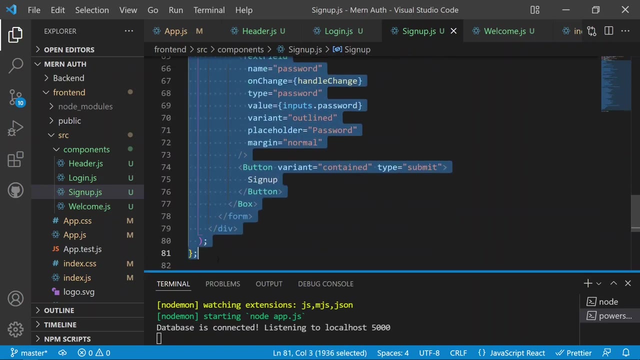 build the login. so now the signup is also done and now we need to build the login page. so we need to go to the- i think, the loginjs to build the page. so we can just get the layout from this sign up as well, so we can get the sign up layout from the inputs to handle change and then all of the data. 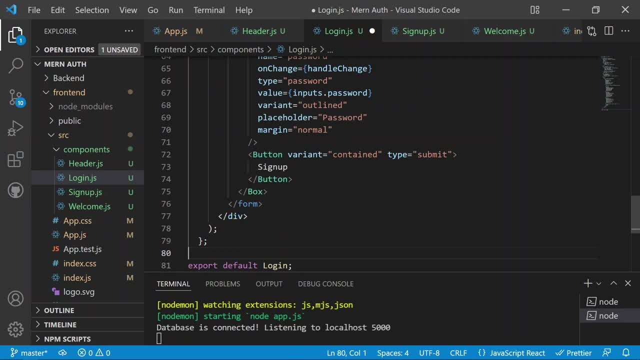 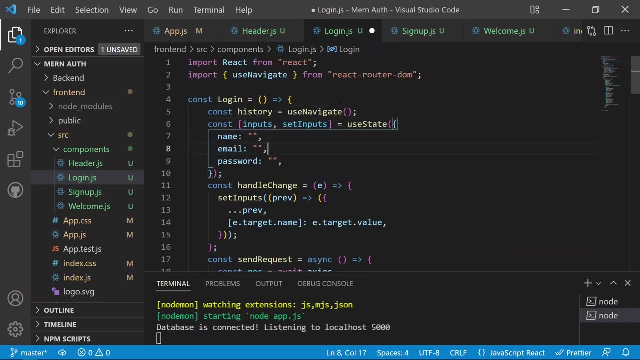 from the sign up so we can just paste that to the login. so now I have not paste it to the login. so we have the history, so we can use a new use- navigate- again, and then we have the use navigate and then we can have the handle change. also we have already declared. we have already declared: 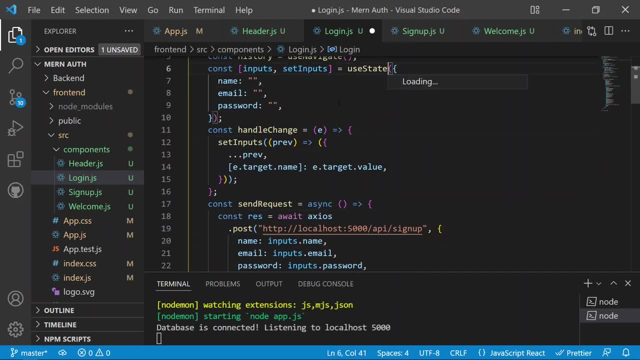 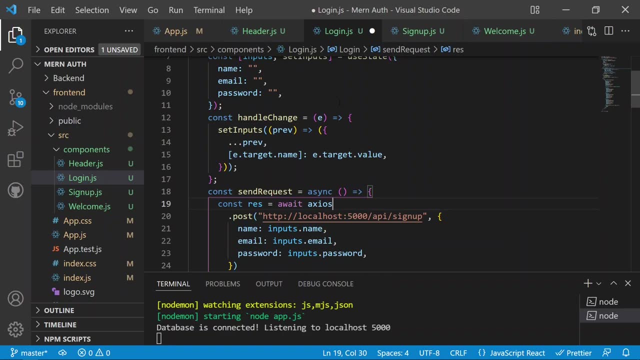 the state. so we have to declare the use state as well. so I will now import the use state from the react and I have now send requests function. so we need to import the axis as well. so Axios is now imported and then we can just import the. I think. I think we need. 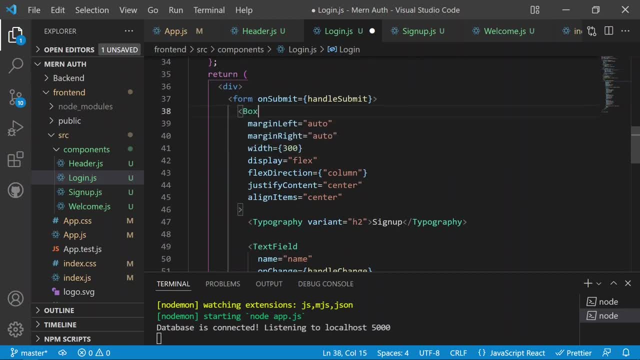 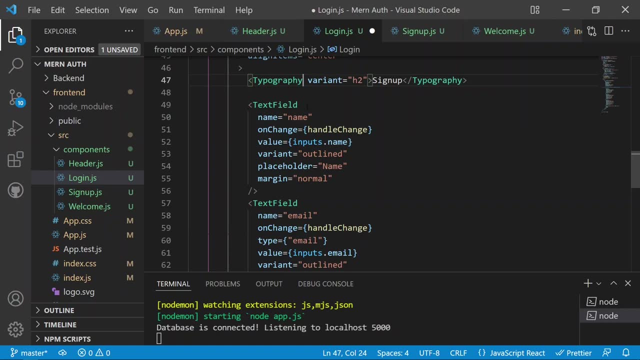 to import the box also from the materials ui- that will be mbm ui material. we need to import the typography as well, so we can import the typography. and then we can import the text field as well, so the text field will also be imported and we can import the button as well. 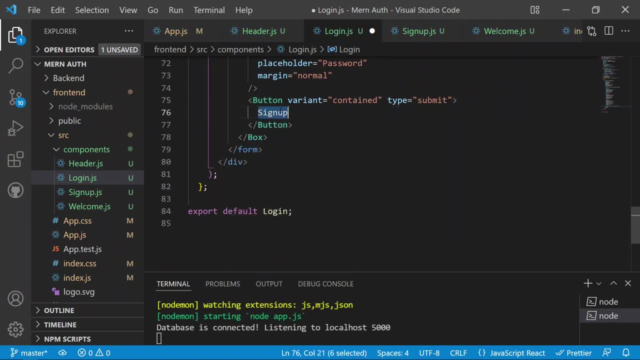 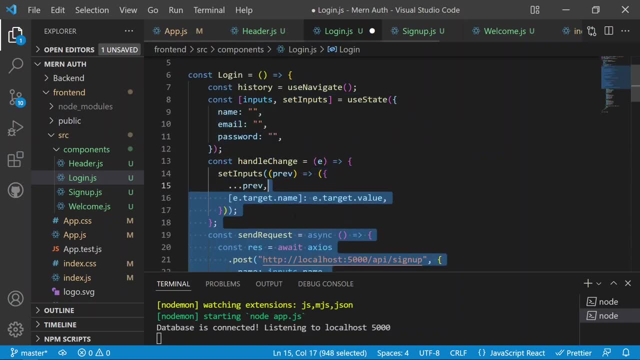 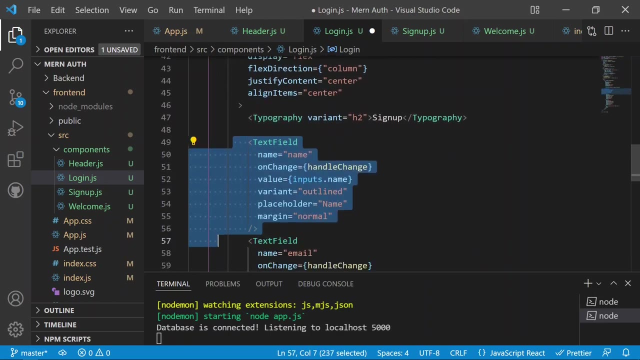 so the button is also imported and now, instead of this login, instead of the signup, we can add the login, and then we don't need the name field now because we are in the login now we only need the email and the password. so i will now remove the name from there and in the inputs also i will 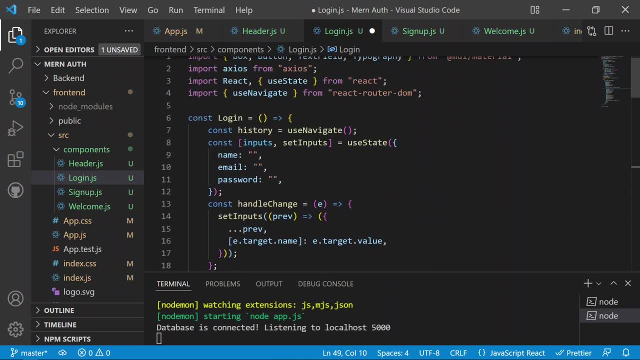 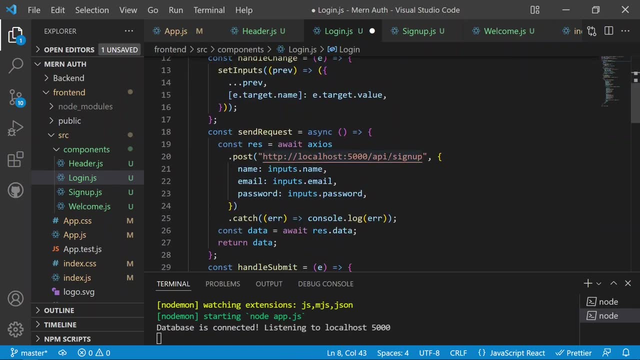 now add here all of these things, like now the name would not be required here and now, everything would work fine. and now you will see. now we have the send request function, but this time the url will be not the signup, the url will be the login. and now the url is login and now we need to add. 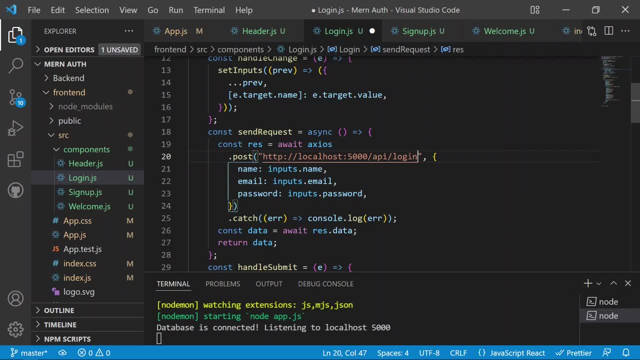 the login request there and then we need to send the data. so then we can send the data here. so login, and then we need to add the login request there and then we need to send the data. so then login, we have, we have. we need to send the email and the password after the login and now in the 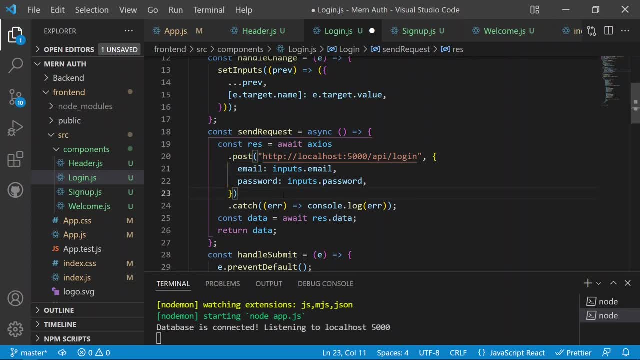 login request. the login request will provide us a token as we have built the functionality in the backend. so after the login will be completed, we will receive a token from the backend and it will be attached to the cookie. so if i will now save and if i will now just move on to the login page, 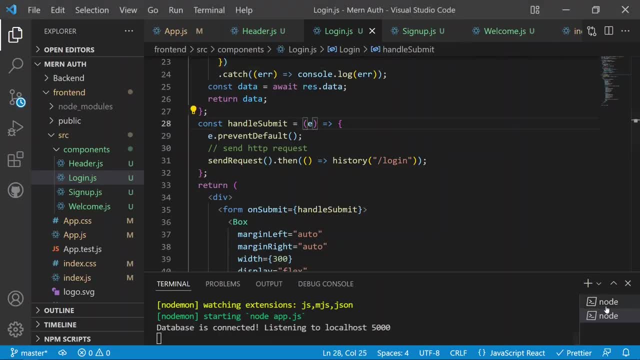 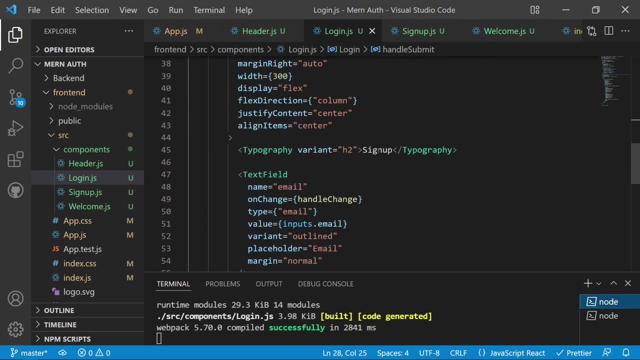 if i will now just refresh and if i will now just save there everything. now we should see, there should not be any errors. now everything is working fine and now, instead of this sign up, it will be the login. now the login is completed and now we need to send here the request. 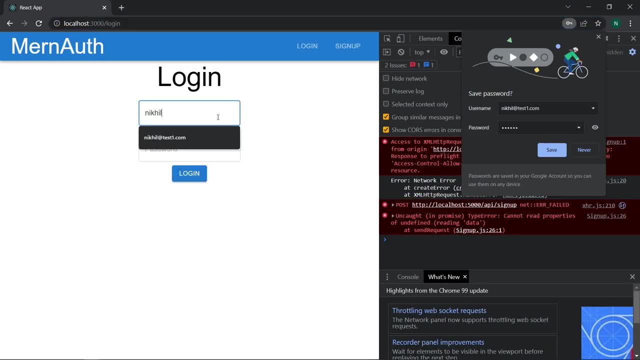 like. we can now send the request at the nickel, at the rate testcom, and then we can add a password as the 111111, as we have declared. so i will now remove everything from this console now. i will now click on the login and now we should see if everything is. 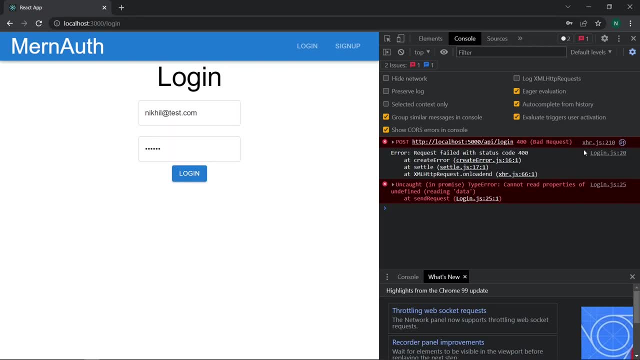 working fine or not. i think there is an error, like the http request is not working fine, so i will now add it to the login, the login request. so we will now add it to the login request. so we will now add it to the login request. so it is a bad request. cannot read properties. open defined data. i think. 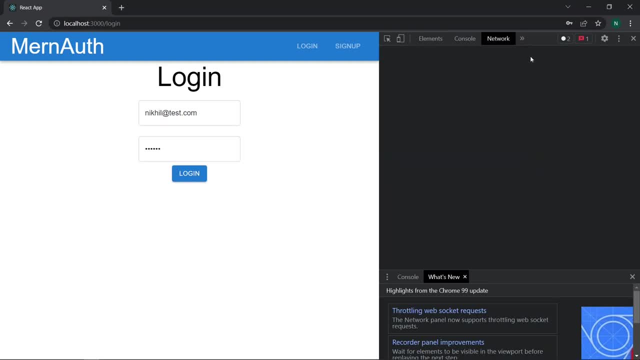 there is an error, so we can just check that error in the network and we can just check the error in the login. here is a login request. like the user not found, i think the credentials are wrong. so i now click on the sign up again so we can just add a new user in the sign up. so it will be the nickel. 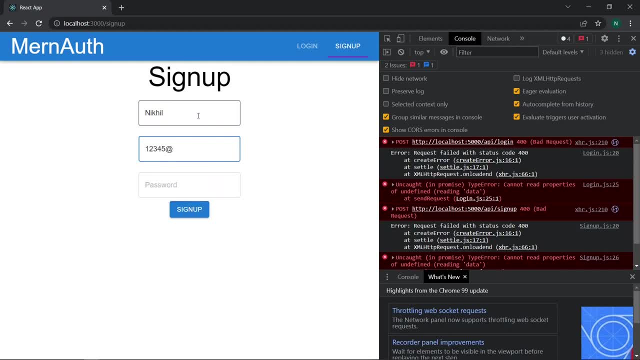 and it will be. the email will be like one, two, three, four, five at the testcom and then we can add a password as the 111111. i will now copy the cmail and then we'll log in to our laptop and we'll be able to see all the features that we have already been inside the laptop. i think we will be able to. 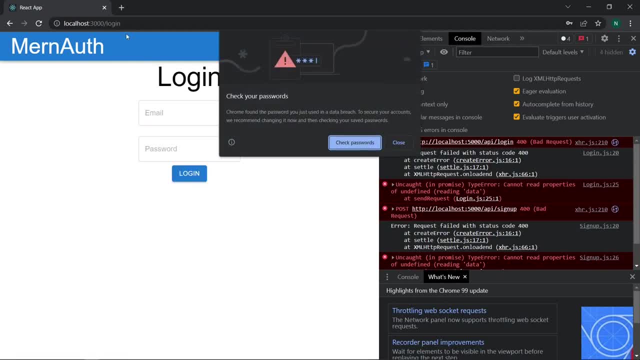 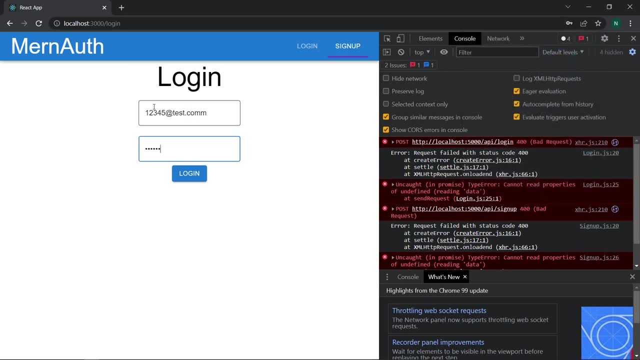 email and i will now just click on the sign up. so now we are signed up successfully and now we are into the login and then we can add the same email and i will add the same password: 111111. so now we should be redirected to the user space, i think. so we can just add here the functionality again that. 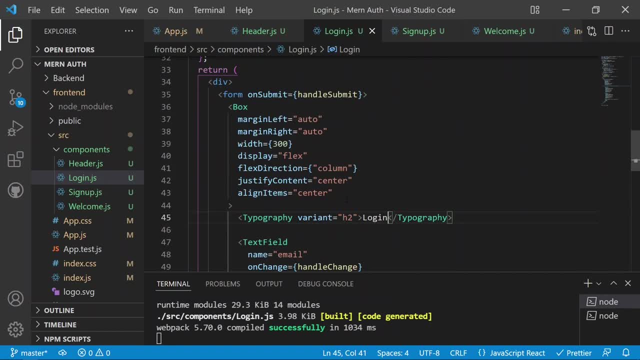 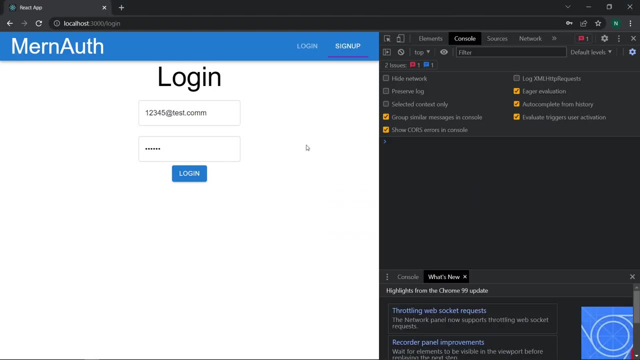 after the request is completed, then we need to redirect to the user space, so we need to go to send request, so it will be the users. so now, if i will now save, so now we should see the screen. so now, if i, if everything would work fine, then we would be redirected to the user. if i will now 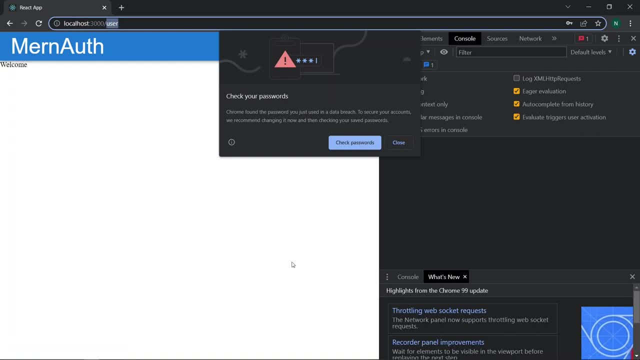 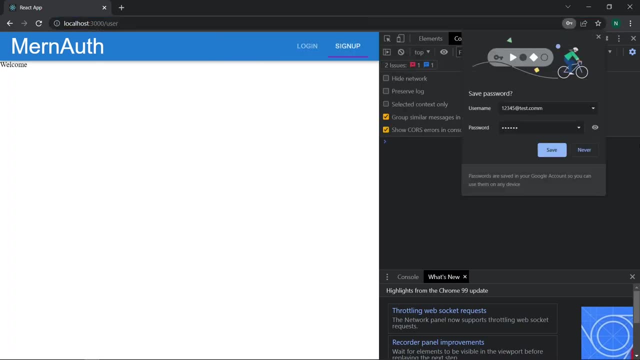 click on the login, so now you will see: now the login is successfully done and now we are redirected. so now you can see: the login is successfully done and now we are redirected to the user. and then we can now just save this. and if i will now just check the network tab, if i will now click on the 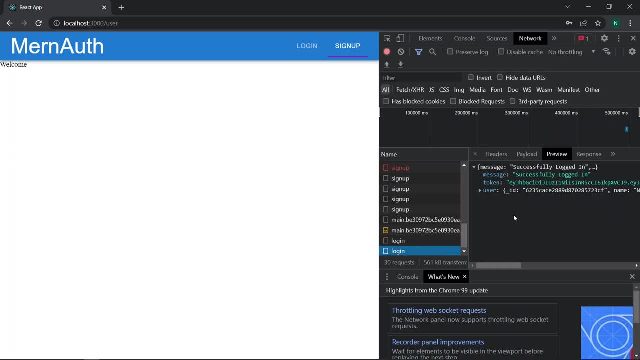 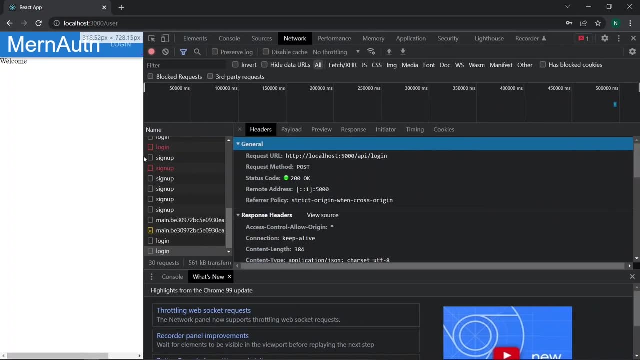 login again. i think if i will now click on the login this now you can see now we are successfully logged in. but if you will check the headers over there, i will now just expand it. so now, if i will now just check the headers here now you can see the status code is 200. okay, and 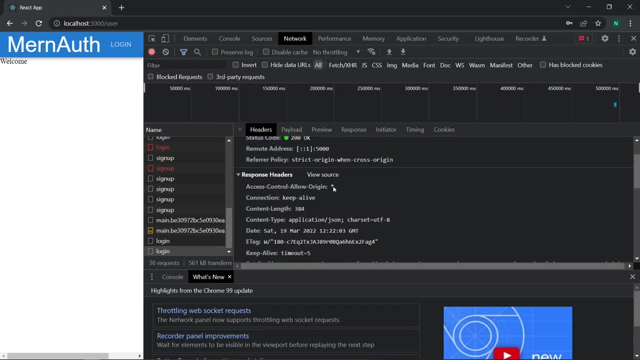 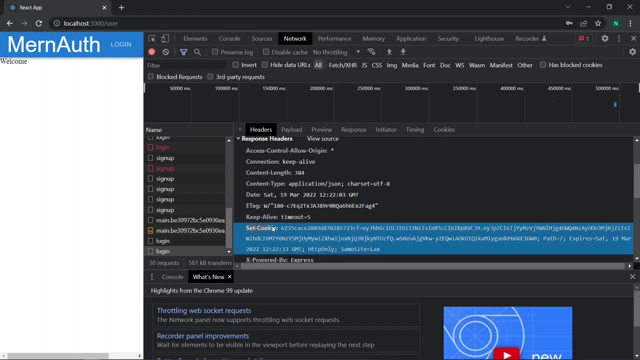 then you will see access control, allow origin. now it is having the star which will allow from everywhere, and it is giving you this star. but if you will just check below now, you will see there is a set cookie which we are receiving. so this is a cookie which we are now receiving there into the 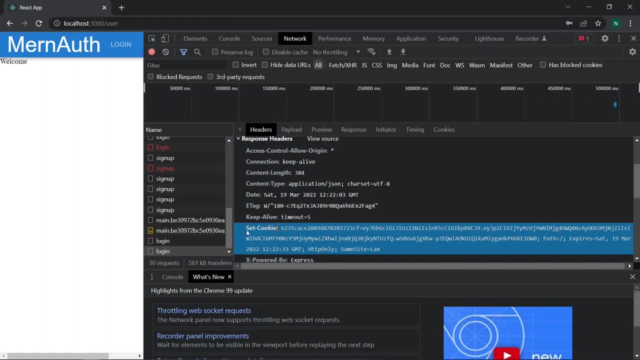 front end and this cookie is being set from the back end. so we are getting this cookie in the front end also, but, as i discussed before, so if you will add this cookie to the front end, you will see that the cookie is being set from the back end. 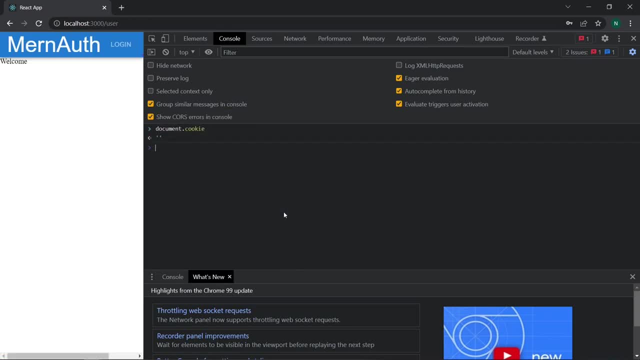 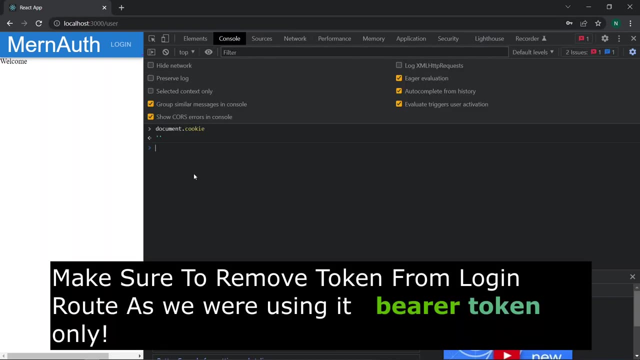 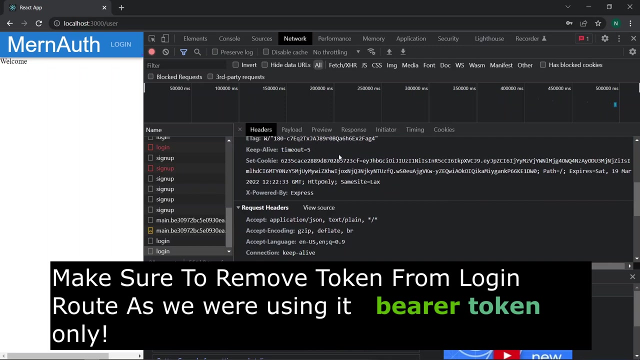 access that cookie in the documentcookie, then it will be empty string because it is not accessible to you in the front end. so we are already secure in that and i think no any hacker can get or steal our token from there and we are getting the token only in the http only cookie. so here is our token. 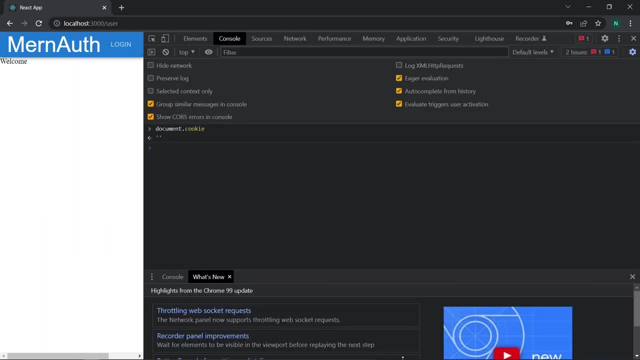 ey and then the token. so here is our token and we are not storing our token even in the local storage, even in the memory or in the cookie or in the session storage, but it is completely secure and it is not accessible to you, even you as well, because we are there on the front end and it is not accessible to the front end. 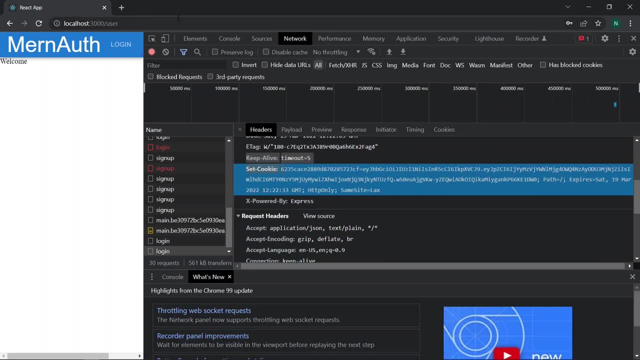 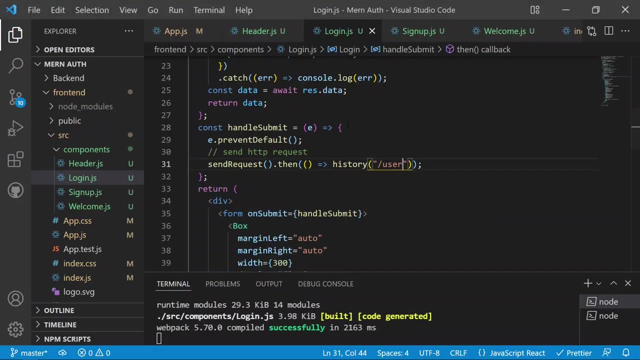 and it is completely secure. and then we can just go to the user space to get the user from this token, and then we can just go to the user's page now in the welcome page. so now we can just go to the welcome and then we can just send the request in the welcome. so now we will go to the welcome. 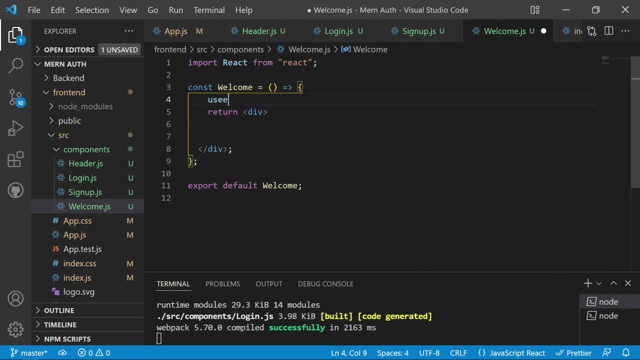 there we can just use the function as the use effect, so it will be the use effect. so we need to add the use effect here inside that so we can just send the request from the use effect. i will add a function there to send the request after that and the use effect is used to. 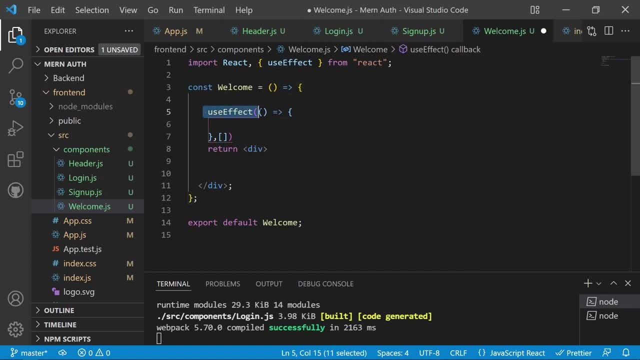 so once the component is being rendered, so the use effect then will run. so we can use here the. i think the we can use the function at the send request again and it will be caused to the function again and then we can use here like the we can just send the request. 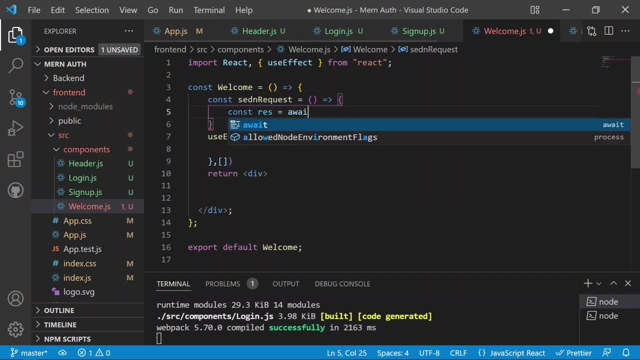 as the const response will be because, to the await, we need to send the request to the xeos xeos. we need to import the xeos so we can import the xeos from there, import xeos from the xeos, and now the xeos is more imported and now we can use the xeos dot get. so this will be a get. 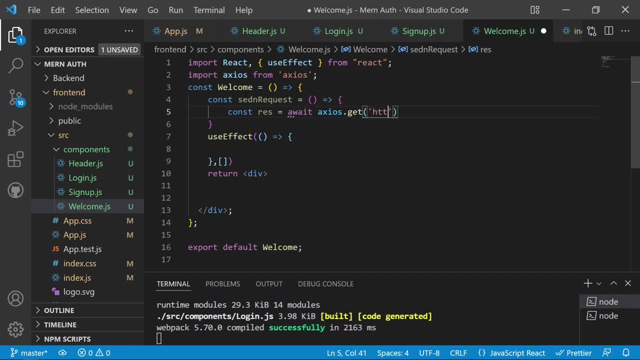 function and now we need to add here the url, so to http. there's localhost url will be 5000, slash, api, slash user, so we can import the xeos from there. and now we can import the xeos from there. so after that, once we will send back the response, once we will send back the cookie to the back. 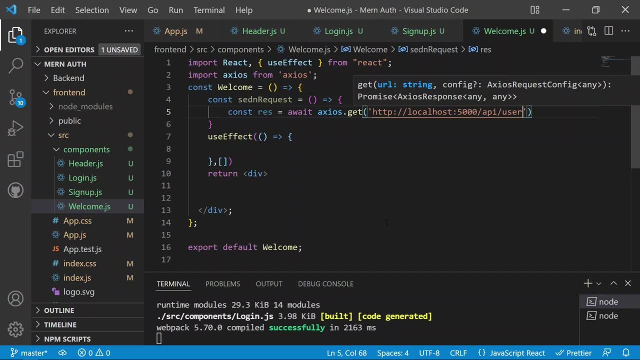 end. so it will check the token and it will decode the token and it will get the id and it will send us the user. so this is very long process but it is a very secure process. and after the user, to send back the data which we receive in the cookie we need to use here an object and the object we 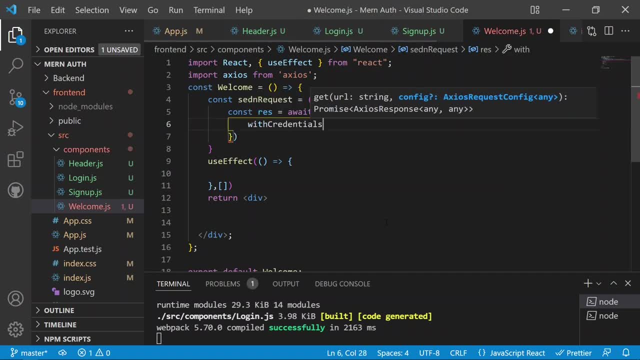 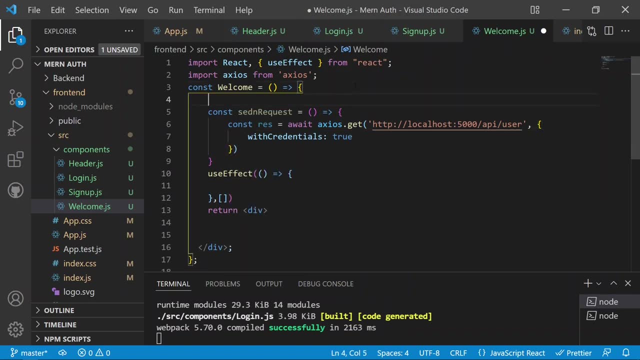 have a property of the with credentials. so we need to use a with credentials property to the true and then we need to send the with credential request after every request. so we can just add here the defaults in the xios. so we can just add a by default at the xios dot defaults. so by default. 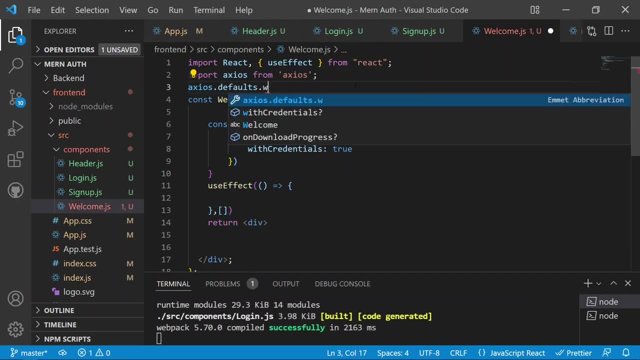 the xios will send the request with the with credentials also always so it will be. the with credentials will be equals to the true. so now we are sending that request and now we can now just add a catch statement after that. to do the catch we need to get the error. we can just console. 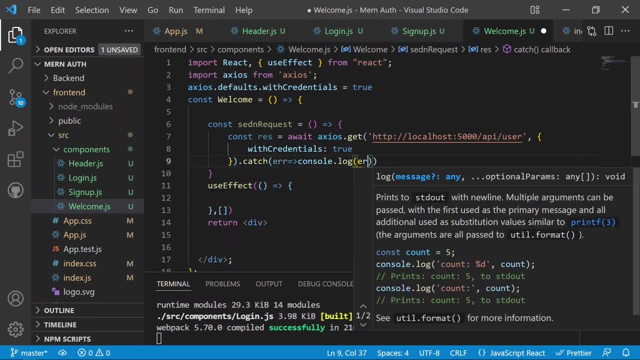 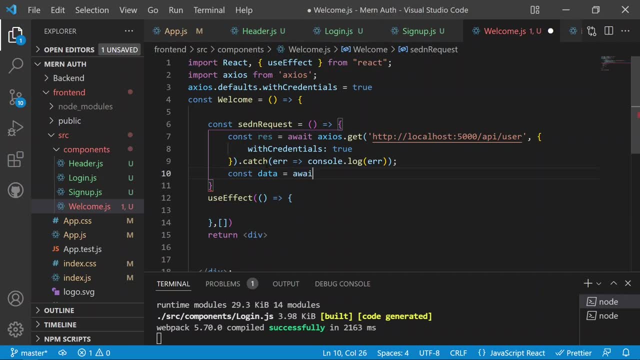 dot lock the error that we have. so now we are having the error and then we can just add a data variable, also data, and it will be equals to the await again the response dot data. so we will get the data from there and then we can just return the data and the send request is. 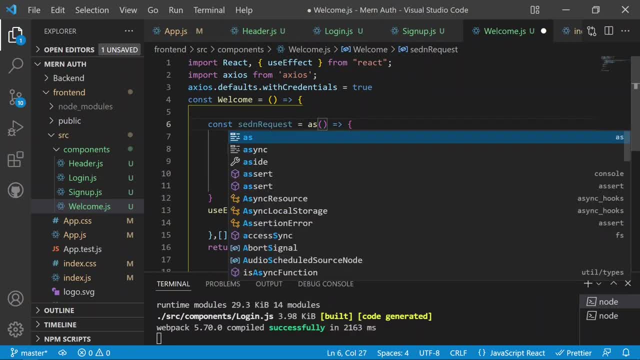 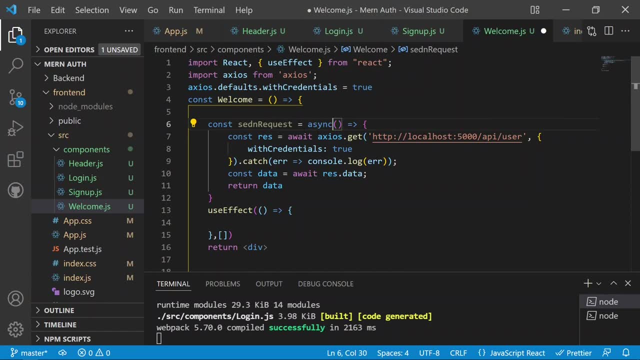 the async function, always because we are using the await. so now everything should work fine. and we have already declared the send request, and now we are going to send the request, and now i think everything should work fine, and now in the use effect. i will now run this. 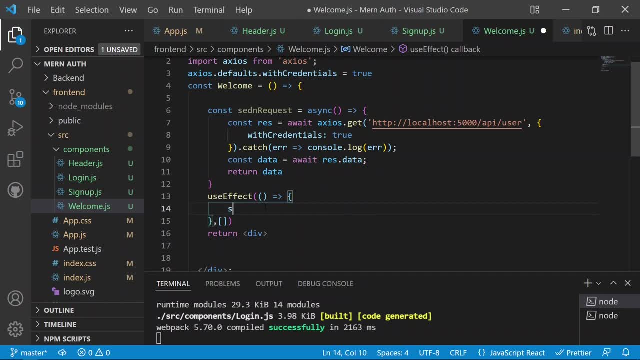 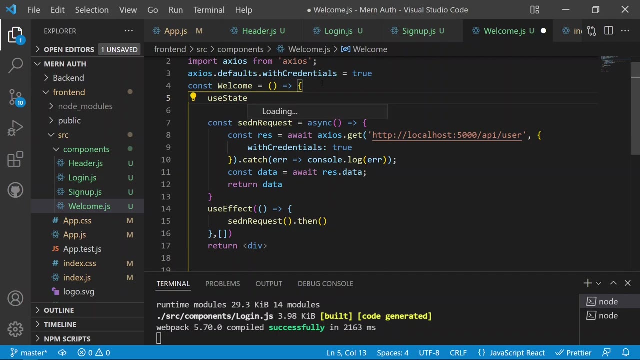 uh, get user function like the send request, so the send request would be there and we can use a then and we can use a state variable also to add the user. so it will. the use state as the use state will be there, so we can add a use state as the user. 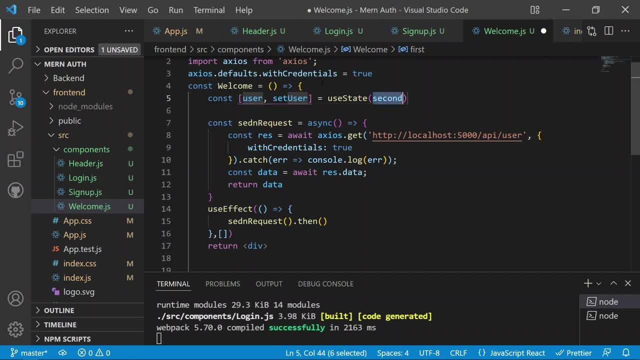 and the set user function with that. so the user and the set user and by default it will be the undefined. and then then when we will get the data from that, and then we will use the set user and it will be the data dot user which we will receive, or we are receiving, i think, the message from there, so we can. 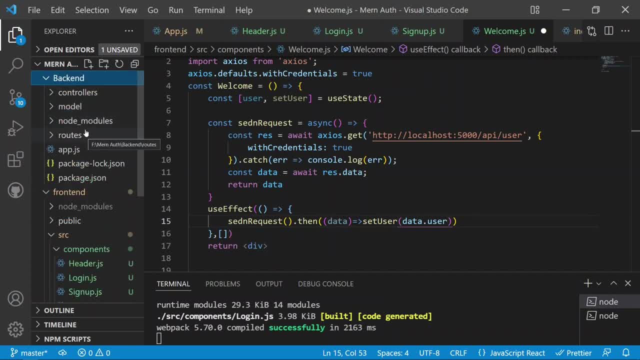 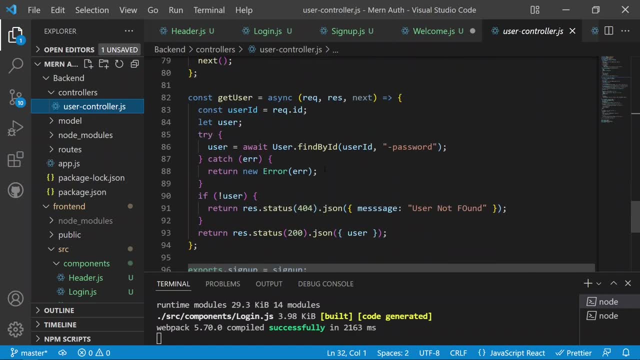 just go to the back end to check what we are getting. so we need to go to the controllers. we need to go to the user controller to see what we are sending after the user is successfully logged in. so we are now sending the user there. so we need to get the user. so we can just get by entering. 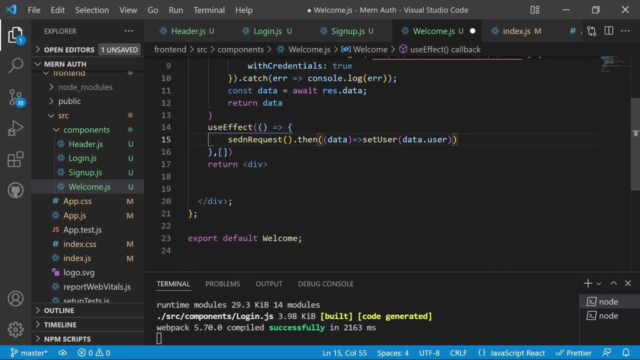 the data dot user. so now, after the: so then we can add a conditional statement here. so when we will have the user and then we will just create h1 tag and in the h1 tag we will just add the user, so it will be the user dot name. so when we will add the user, so we will just show the user dot name there. 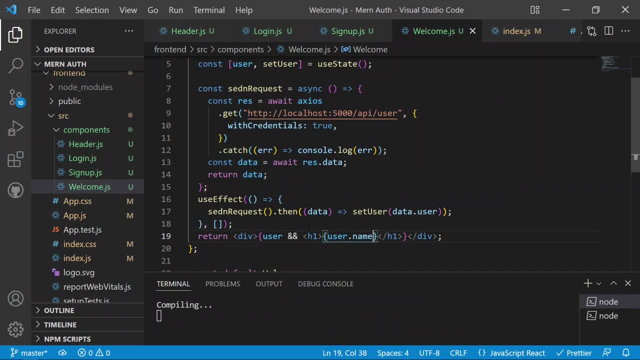 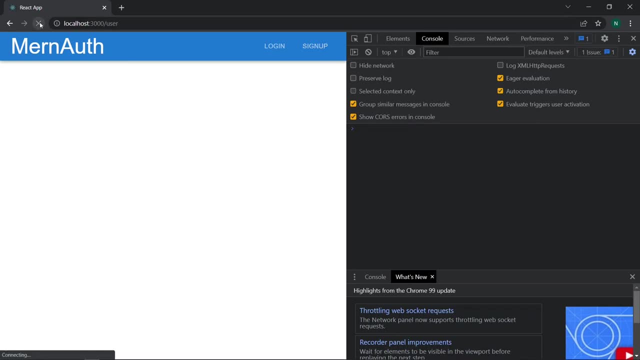 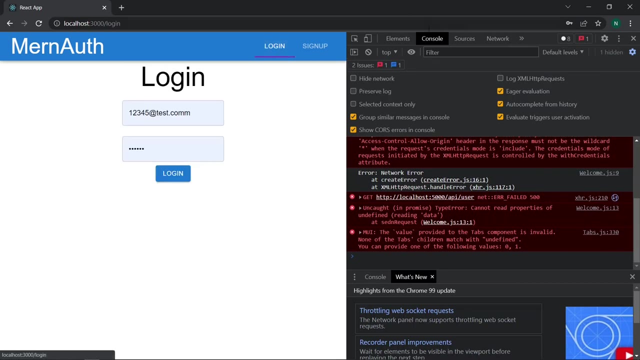 so if i will now save, so now we should see the changes onto the screen. so now we are in the chrome once again. now you can see there is an error again. so now we need to refresh the page again there. so now we can just click on the login and now we can just log in again, the user which we have. 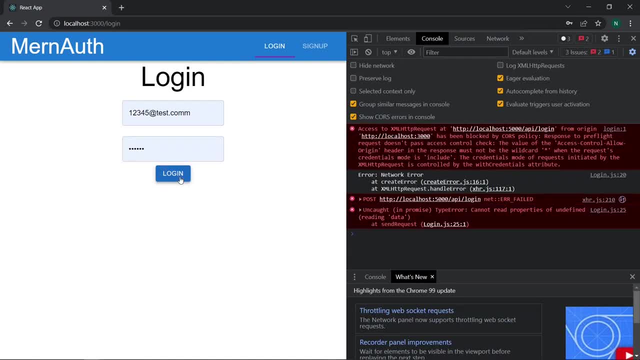 i will now click on the login, so now we are not redirected to the user's page. i think there is some error and this error is because we are now sending the request from a different url server, but we are having the access to giving the data and to get the data, but we don't have access to. 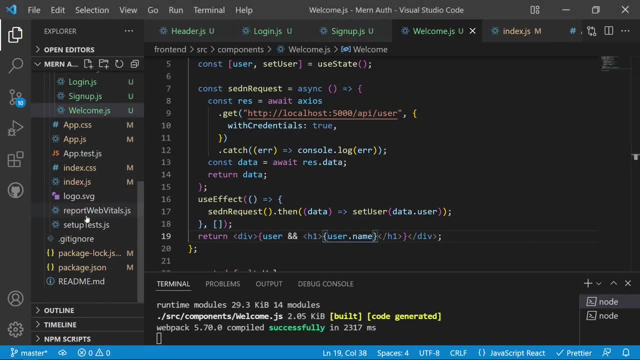 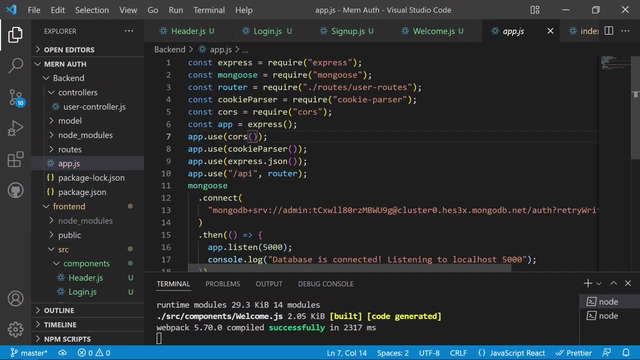 send the cookie to the back end. so we are not sending the cookie to the back end, so we are just sending the data and to get the access for that cookie we can go to the appjs once again of the backend and then, after we are requiring the course, then we need to add some origins also. 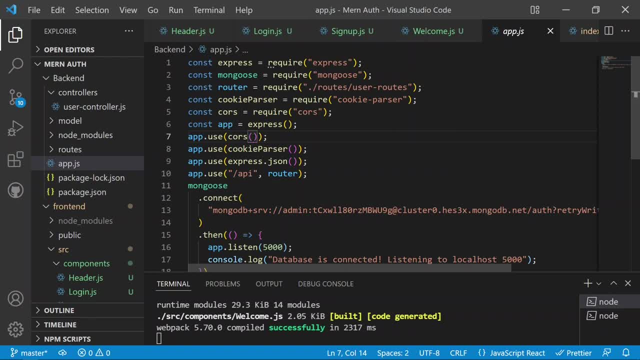 because now we are sending some credentials from the xeos and for that we need to add some properties like credentials, because now we are sending the credentials from the xeo, so credentials will be equals to the true to get the credentials and we need to specify the origin as well. so in 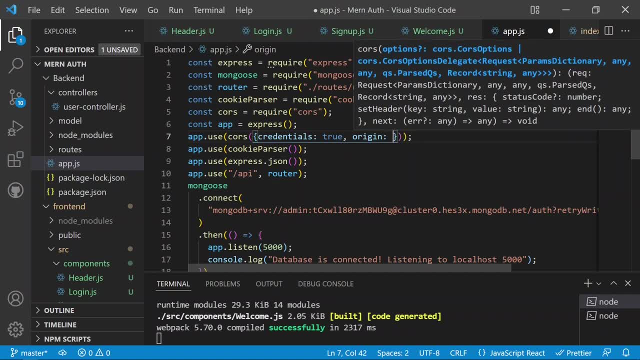 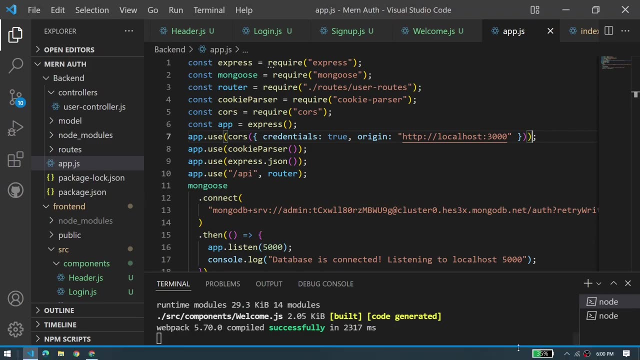 which origin we need to send the data or to receive the data. so we can just add the origin as the http slash localhost at the rate of the port of the 3000 and we are now sending the data from there. so if i will now save and if i will now just go to these login screen once again to see if 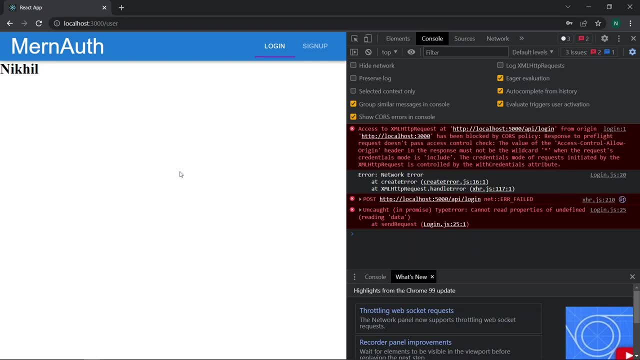 everything is working fine or not. i will now click on the login once again. now we are redirected to the user and now, you will see, now we have the username there. so now we are getting the name of the user, nickel, and now it means that everything is working totally fine. so we have now successfully- 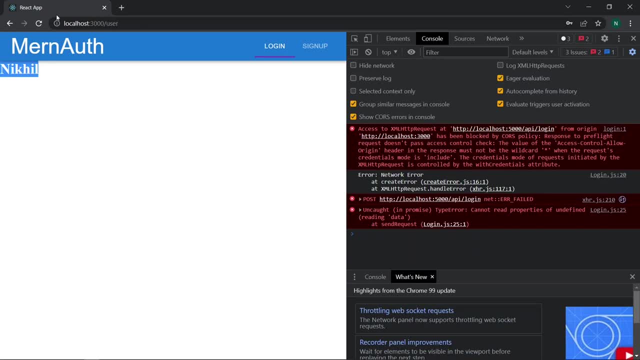 built the most secure backend that we have and we have already declared everything there and once, if you will refresh the page after the 30 seconds, so it will be gone. so once you will refresh the page, so now you will see there will be an error, i think. so now you will see there is an error that 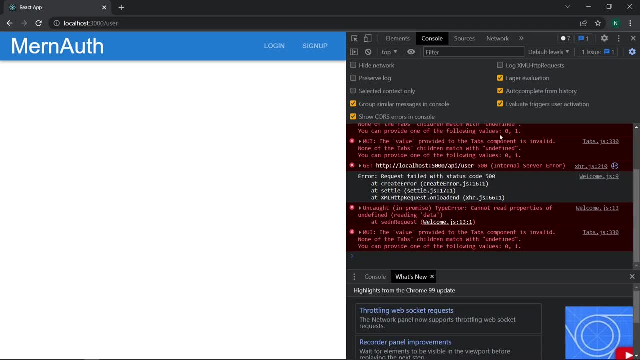 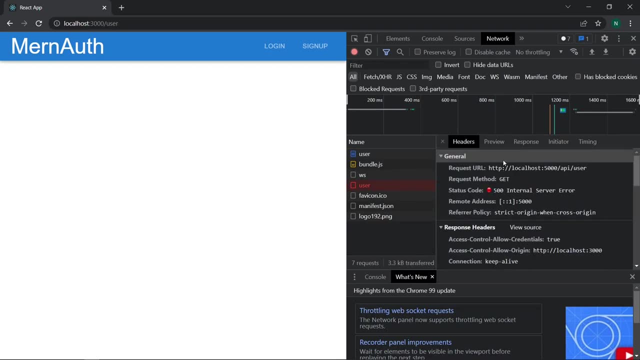 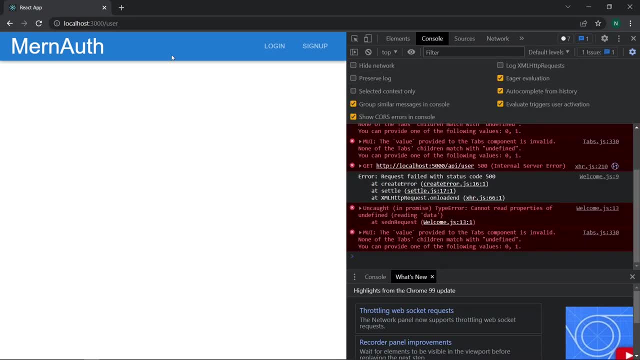 undefined. so now it means that everything is working totally fine and we are getting the working totally fine and we are getting the user in the front end without having their id in the url, user in the front end without having their id in the url and with pure credentials, which we are now. 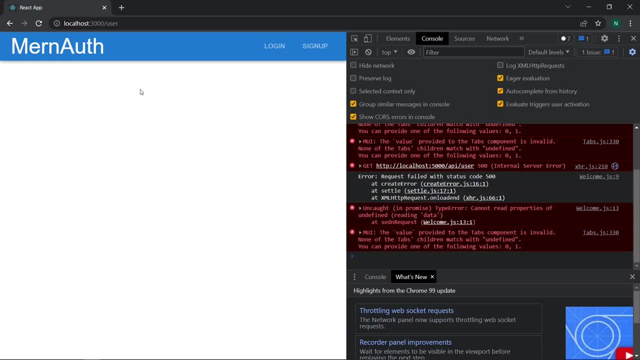 and with pure credentials, which we are now. sending the cookie to the front end and getting the cookie, sending the cookie to the front end and getting the cookie to the back end again. so everything is to the back end again. so everything is totally working fine. so this error is coming because the token is getting expired and we are not able to generate. so this error is coming because the token is getting expired and we are not able to generate. so this error is coming because the token is getting expired and we are not able to generate. the new tokens so to fix this problem. the new tokens so to fix this problem. 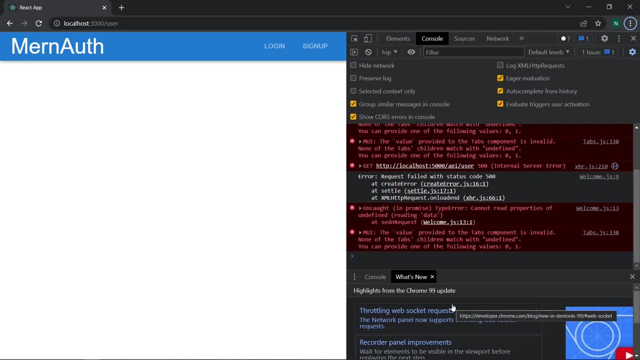 the new tokens. so to fix this problem, there are two solutions. the first one is there are two solutions. the first one is there are two solutions. the first one is: either we can increase the time limit of, either we can increase the time limit of, either we can increase the time limit of the token, like an hour or day or any. 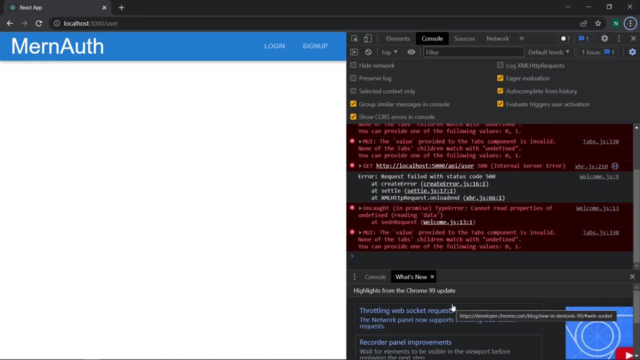 the token like an hour or day or any. the token like an hour or day or any number of days. and second, we can just number of days. and second, we can just number of days. and second, we can just refresh the token again and again after. refresh the token again and again after. 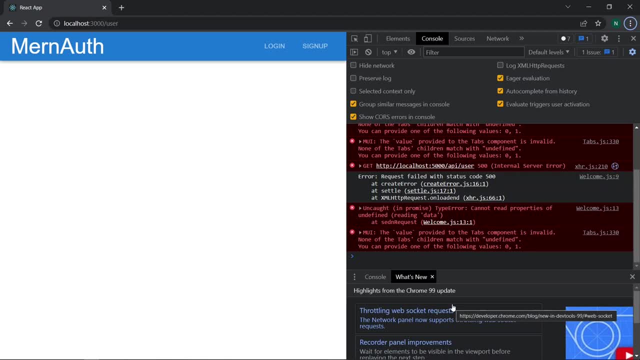 refresh the token again and again after every request, and it will be a pure every request. and it will be a pure every request and it will be a pure authenticated version because the excess authenticated version, because the excess authenticated version, because the excess token will be then expired and we will 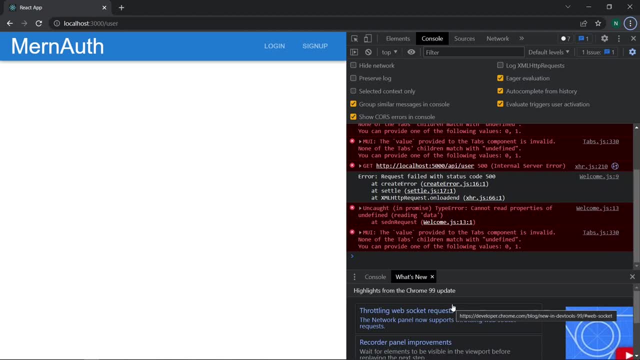 token will be then expired and we will token will be then expired and we will be generating the new access token after be generating the new access token. after be generating the new access token after a time span of every 15 to 30 seconds. a time span of every 15 to 30 seconds. 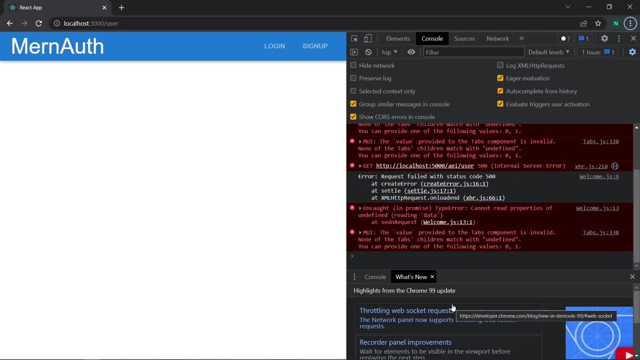 a time span of every 15 to 30 seconds. and with this approach, the application, and with this approach, the application and with this approach, the application can be complex, but for the security can be complex, but for the security can be complex, but for the security reasons, we should always have a complete. 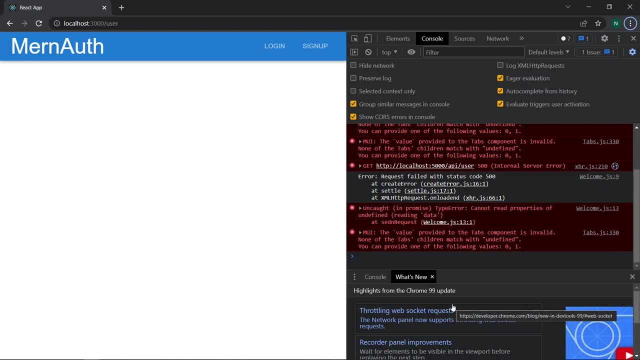 reasons. we should always have a complete reasons. we should always have a complete and a secure backend to run the and a secure backend to run the and a secure backend to run the application. we can move ahead with the application. we can move ahead with the application. we can move ahead with the second approach so we can generate a. 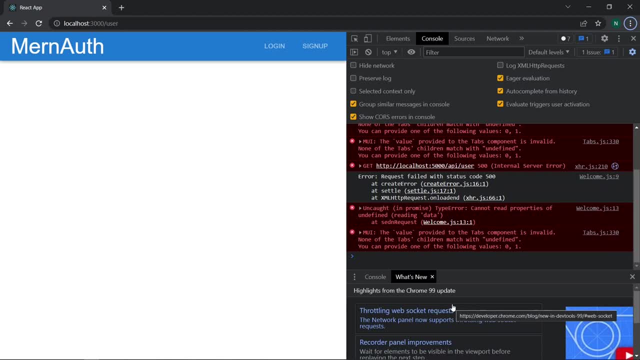 second approach so we can generate a second approach. so we can generate a refresh token route in the backend after refresh token route in the backend after refresh token route in the backend after every 30 seconds, so the token will be every 30 seconds, so the token will be. 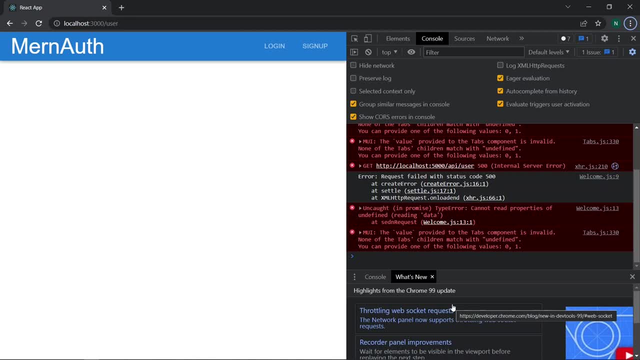 every 30 seconds. so the token will be then refreshed, and then we will reset, then refreshed, and then we will reset, then refreshed, and then we will reset the cookie as well. so let's start with the cookie as well. so let's start with the cookie as well. so let's start with this approach, and then we need to go to. 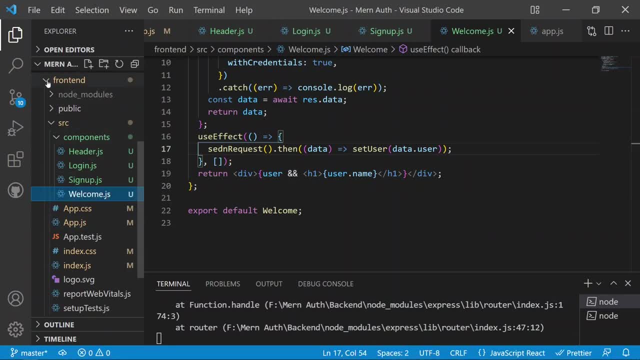 this approach and then we need to go to this approach and then we need to go to the backend to complete this approach. so the backend to complete this approach, so the backend to complete this approach. so we need to go to the backend folder and we need to go to the backend folder and 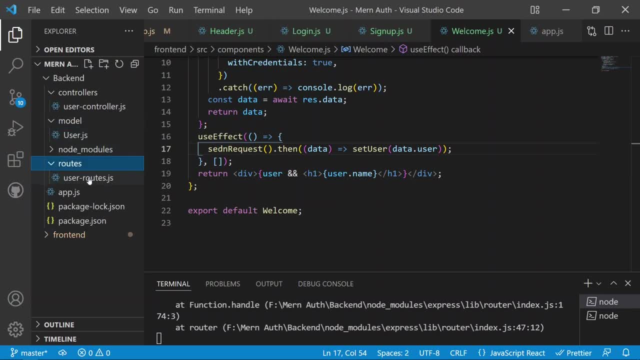 we need to go to the backend folder and then we need to create a new route. after then we need to create a new route. after then we need to create a new route after the routes, so we can just create a new: the routes, so we can just create a new. 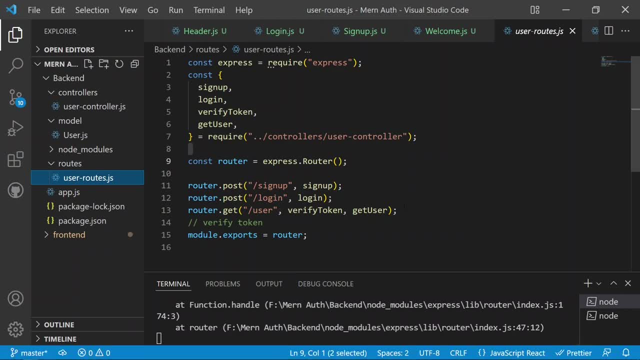 the routes, so we can just create a new route, route, route, and after all of the routes, now we can. and after all of the routes, now we can. and after all of the routes, now we can declare a new route with the router, declare a new route with the router. 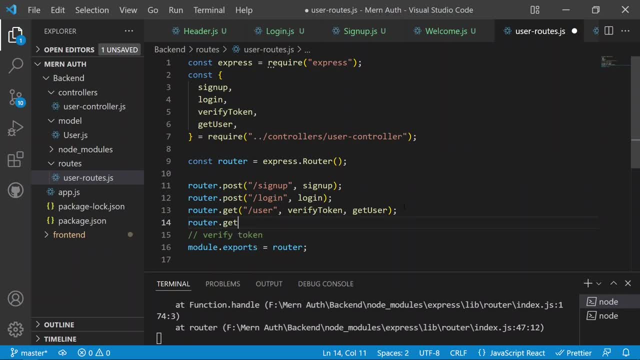 declare a new route with the router, and it will be: dot get request and it and it will be: dot get request and it and it will be dot get request and it will be, will be, will be of the slash at the refresh, of the slash at the refresh. 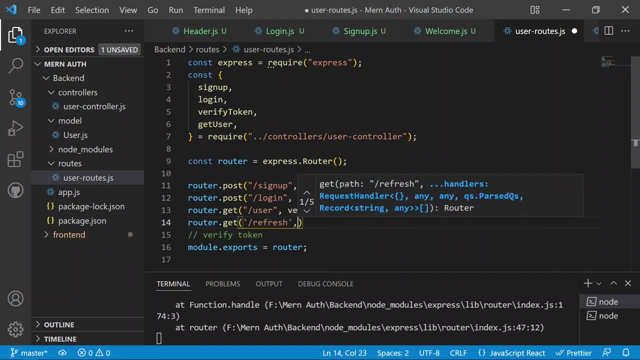 of the slash at the refresh, so it will be the refresh and then we, so it will be the refresh and then we, so it will be the refresh, and then we can just have some functions after there, can just have some functions after there, can just have some functions after there, so we can have the functions in the. 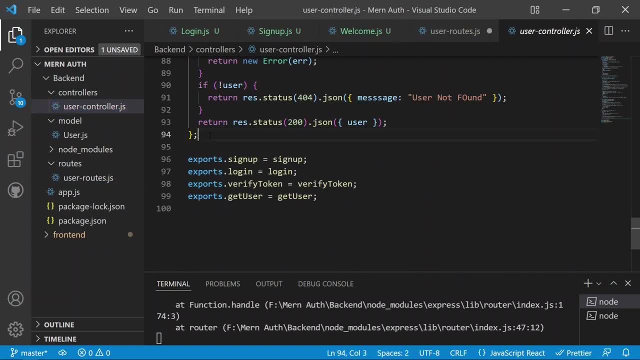 so we can have the functions in the, so we can have the functions in the user's controller. so we can just go and user's controller. so we can just go and user's controller. so we can just go and we can just create a refresh token here. 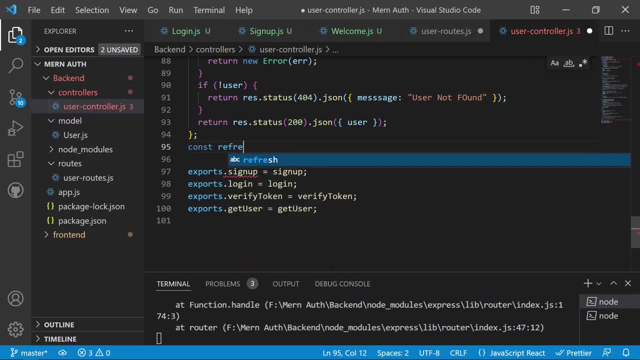 we can just create a refresh token here. we can just create a refresh token here, so it will be like the const, so it will be like the const. so it will be like the const, const, refresh token, const, refresh token, const, refresh token. and it will be because of the function. 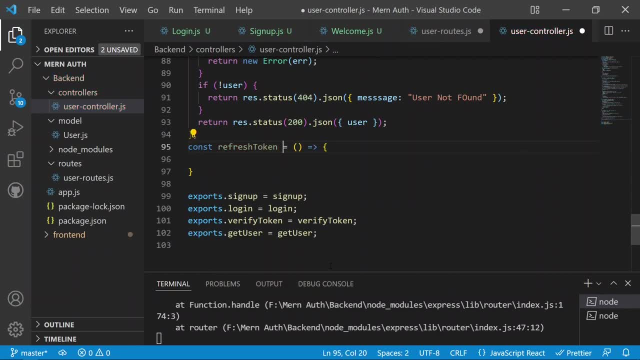 and it will be because of the function, and it will be because of the function and then we can just have the request, and then we can just have the request, and then we can just have the request response and the next there as the response and the next there as the. 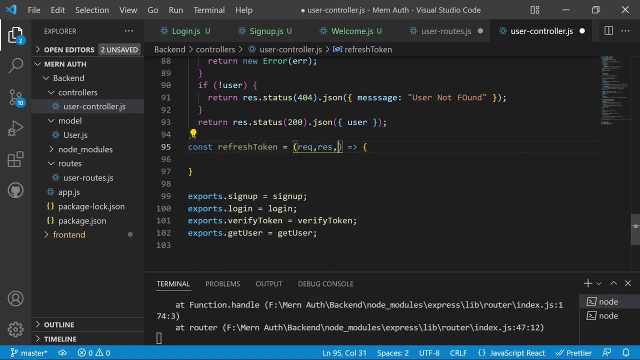 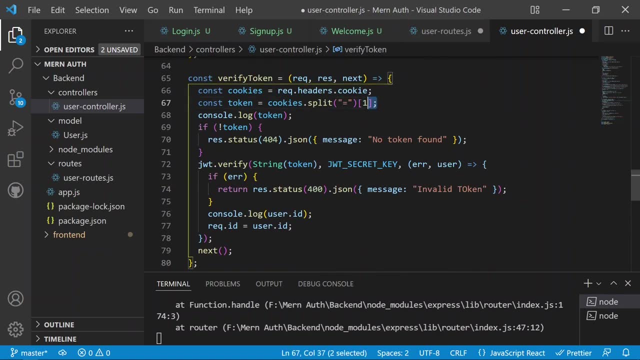 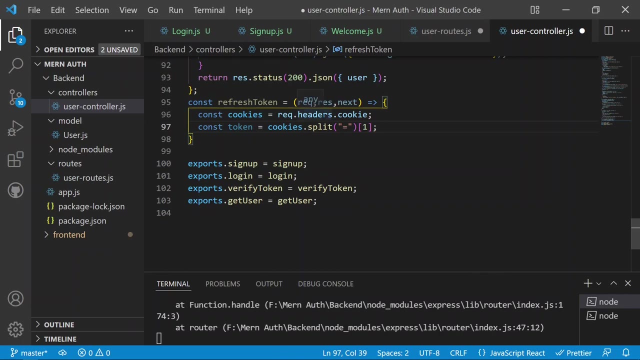 response and the next there as the variable. so it will the request response variable, so it will the request response variable, so it will the request response and set and set, and set, and then we can get these cookies from and then we can get these cookies from, and then we can get these cookies from the cookies request dot header. so once, 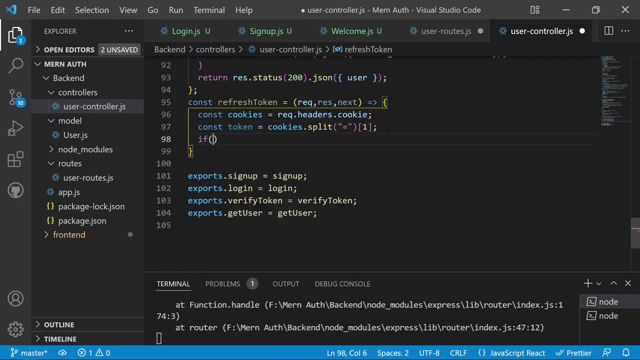 the cookies request dot header. so once the cookies request dot header, so once we will get the cookie from the request, we will get the cookie from the request, we will get the cookie from the request dot header and then we can check if we dot header and then we can check if we. 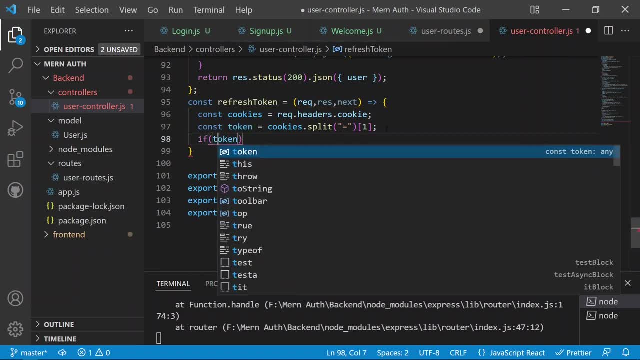 dot header, and then we can check, if we don't have the token, don't have the token, don't have the token, and then we can just check like so we. and then we can just check like so we. and then we can just check like so we can declare here the previous token there. 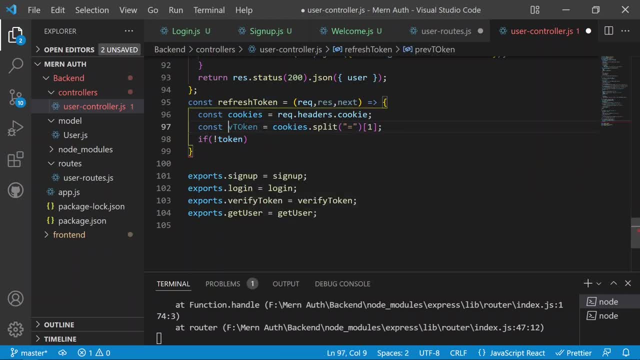 can declare here the previous token there, can declare here the previous token there. so it will the previous token, so it will the previous token there. so if we don't have the previous token, so if we don't have the previous token, so if we don't have the previous token, and then we can just return as the 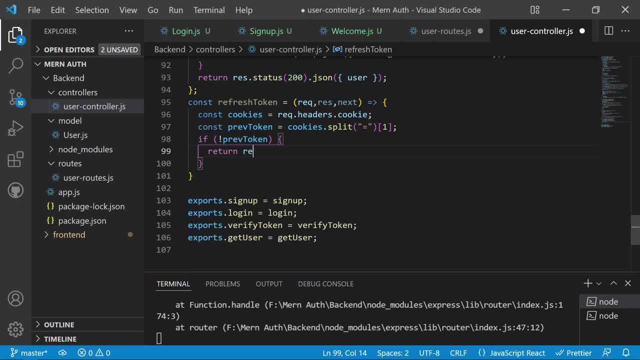 and then we can just return as the and then we can just return as the restore as the response dot status and the status will be the 400 as the and the status will be the 400 as the and the status will be the 400 as the unauthorized, and then we can just send. 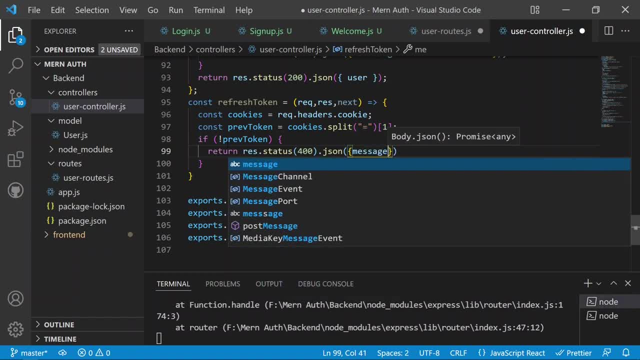 unauthorized, and then we can just send unauthorized, and then we can just send the message at the json and the json. the message at the json and the json, the message at the json and the json, will contain a message, will contain a message, will contain a message, and the message will be: then the couldn't. 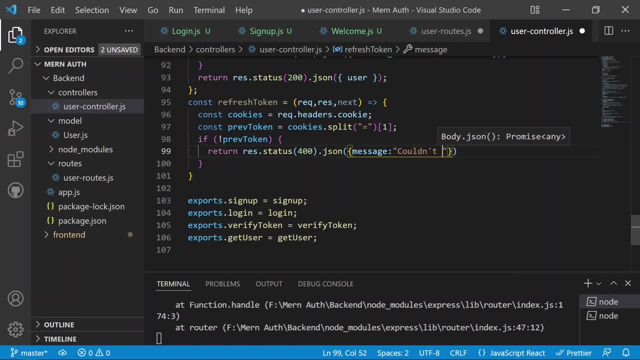 and the message will be then the couldn't. and the message will be then the couldn't find token. so we can have this message, and then so we can have this message, and then so we can have this message, and then, after the token is there, and then in the 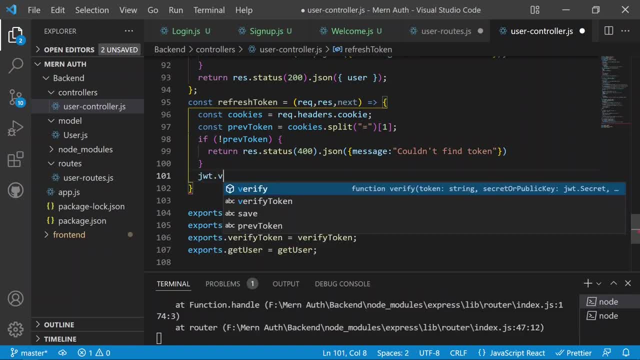 after the token is there and then in the after the token is there and then in the else case, then we can verify the token else case. then we can verify the token else case. then we can verify the token. like the jwt dot verify. like the jwt dot verify. 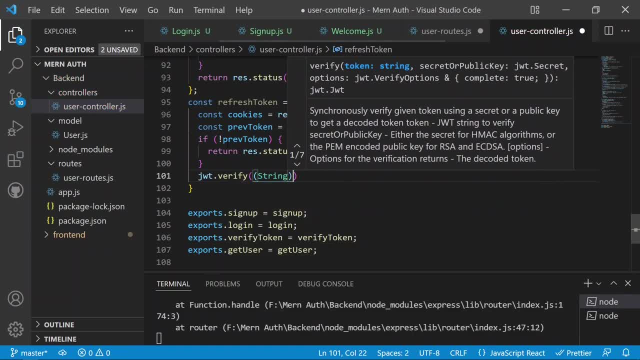 like the jwt dot verify. so we can just verify the token with. so we can just verify the token with. so we can just verify the token with the converting it to the string and it the converting it to the string and it the converting it to the string, and it will be like the string. 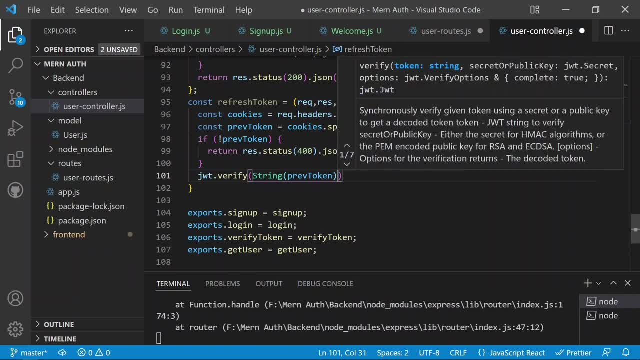 will be like the string will be like the string as the previous token that we have and as the previous token that we have and as the previous token that we have, and then we need to compare it with the, then we need to compare it with the, then we need to compare it with the security key by giving the security key. 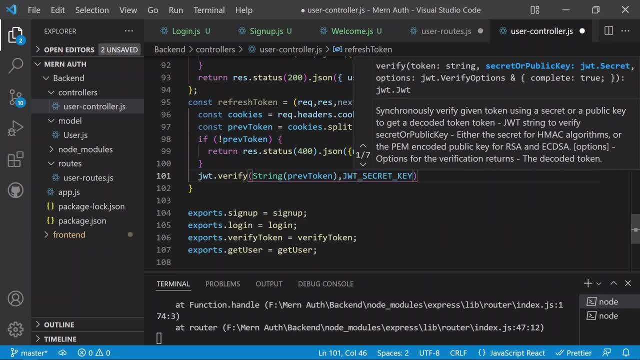 security key by giving the security key. security key by giving the security key. so it will be like the. so it will be like the. so it will be like the jwt secret key, and then we can just check jwt secret key and then we can just check jwt secret key and then we can just check the decoded parameters, also like the. 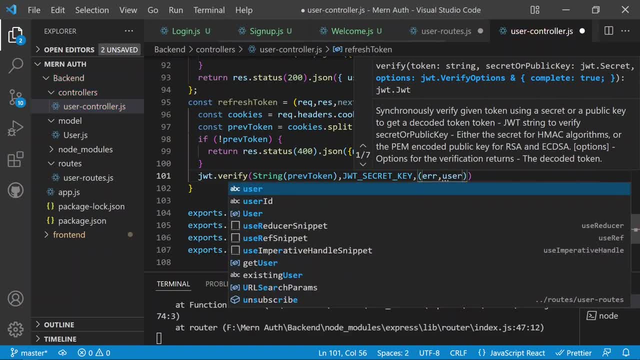 the decoded parameters also like the. the decoded parameters also like the error. first we do the error and then it error. first we do the error and then it error. first we do the error and then it will. the user which is decoded now will. the user which is decoded now. 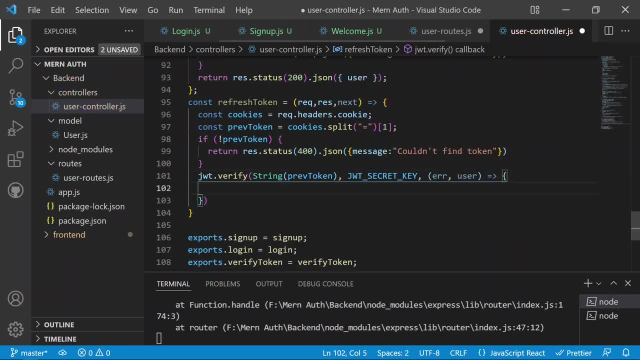 will the user which is decoded now, and then we can just generate the function, and then we can just generate the function, and then we can just generate the function with there, with there, with there as the callback, and then we can check if as the callback, and then we can check if. 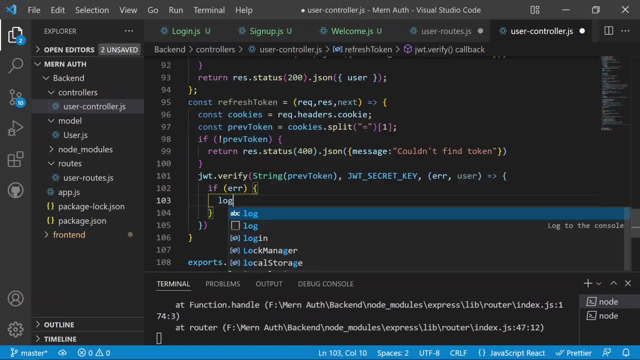 as the callback, and then we can check if there is any error, and then we can just: there is any error, and then we can just: there is any error, and then we can just consolelog the error, consolelog the error, consolelog the error, and then we can just also return at the. 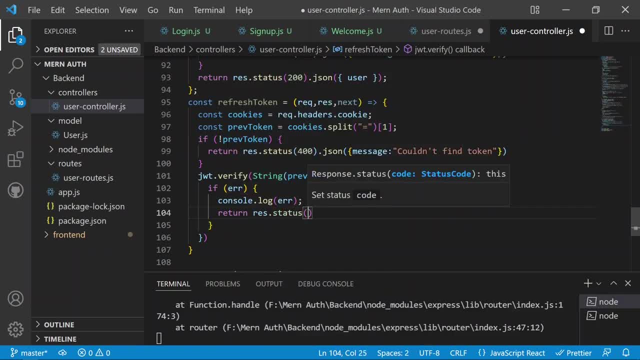 and then we can just also return at the, and then we can just also return at the responsestatus, responsestatus. responsestatus will be equals to like the 403, and then will be equals to like the 403, and then will be equals to like the 403, and then we can just 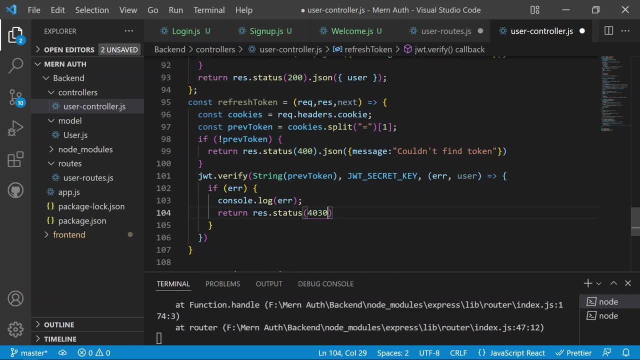 we can just. we can just send the error to the user as well. send the error to the user as well. send the error to the user as well as the 403, and then we can just add a as the 403, and then we can just add a. 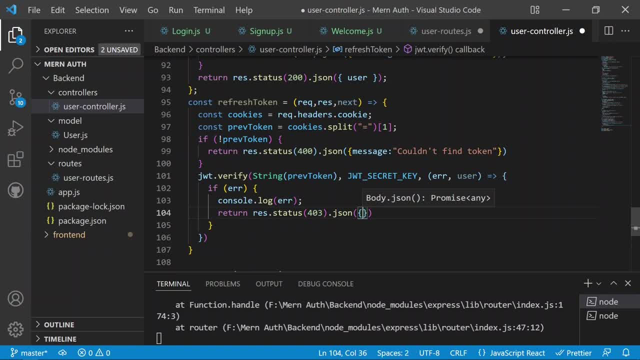 as the 403, and then we can just add a json, json, json, dot json, and then it will contain the dot json, and then it will contain the dot json, and then it will contain the parameters, parameters. parameters as the message, as the message, as the message and the message will be equals to like. 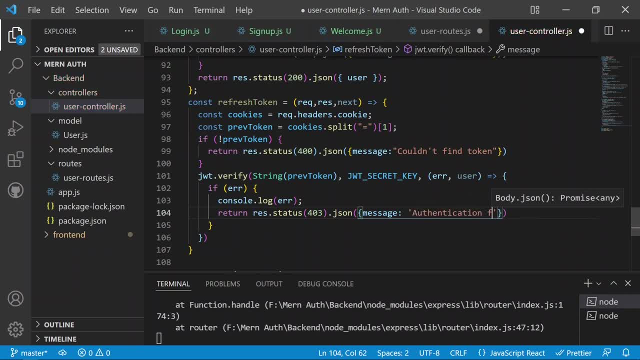 and the message will be equals to like and the message will be equals to like. we can just send as the authentication. we can just send as the authentication. we can just send as the authentication. failed because now we have the error. failed because now we have the error. 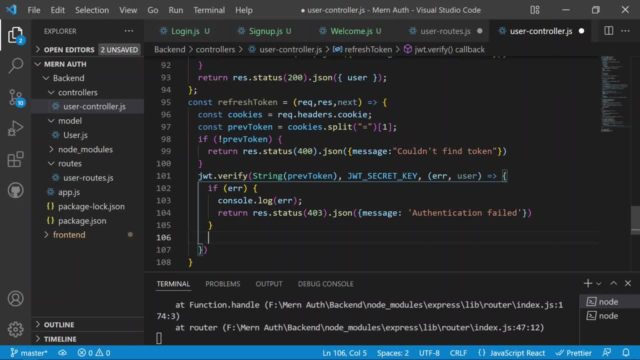 failed, because now we have the error and now the token is not verified, and now the token is not verified, and now the token is not verified. now we have the and now we are returning. now we have the and now we are returning. now we have the and now we are returning the token if we have any error. but 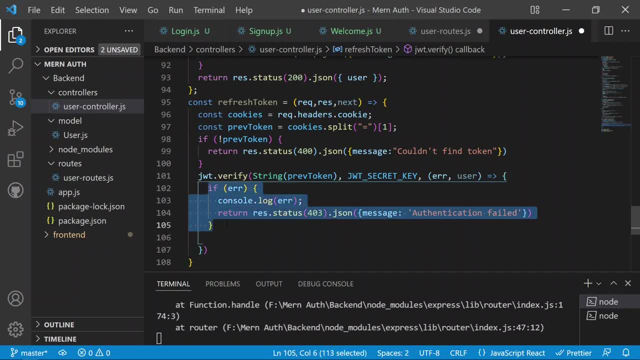 the token if we have any error, but the token if we have any error, but now if the token is successful, because now if the token is successful, because now if the token is successful, because now after the if case, so the if case will. now after the if case, so the if case will. 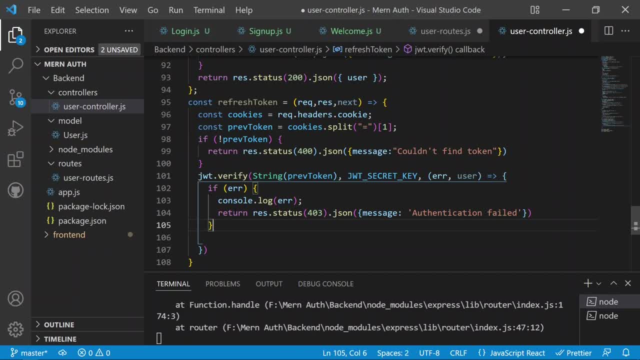 now, after the if case. so the if case will run, so the application will break, but run. so the application will break, but run, so the application will break. but now, if we don't have any error, and now. now, if we don't have any error, and now: 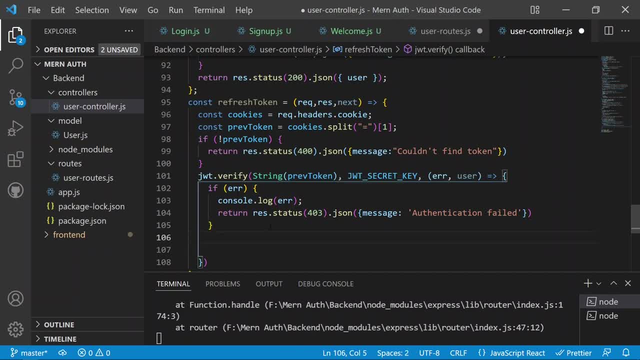 now, if we don't have any error, and now if we have the user and the token is, if we have the user and the token is. if we have the user and the token is successful and it is verified, so we can successful and it is verified, so we can. 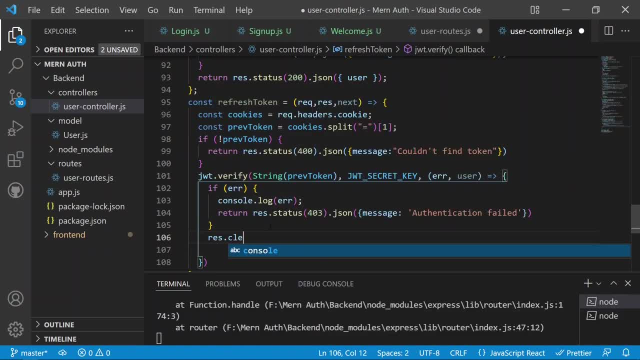 successful and it is verified. so we can just clear the cookie, just clear the cookie. just clear the cookie by having the response dot clear cookie, by having the response dot clear cookie, by having the response dot clear cookie function, and then it will be the userid which we 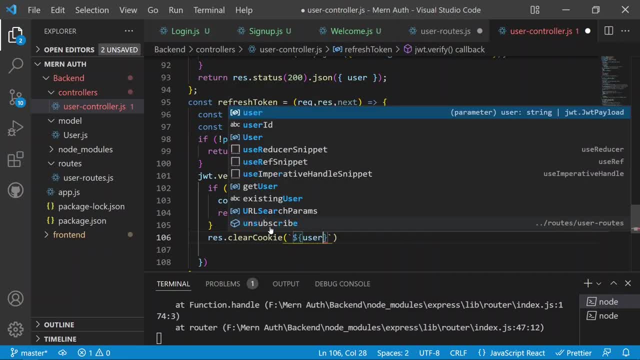 and then it will be the userid which we, and then it will be the userid which we will do, will do, will do uh decoding from the user, so it will be uh decoding from the user, so it will be uh decoding from the user, so it will be the user which we are decoding. 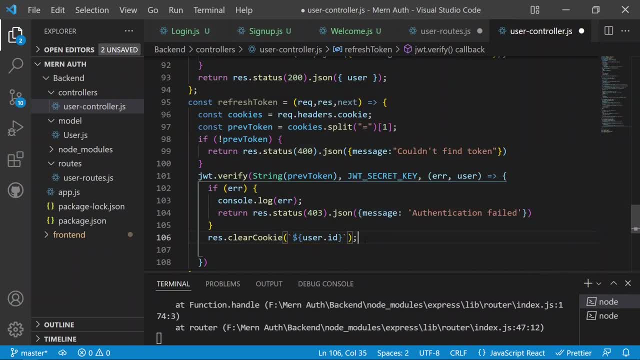 the user which we are decoding, the user which we are decoding, dot id. so we will just return the ids, dot id. so we will just return the ids, dot id. so we will just return the ids, and then we will return, and then we will, and then we will return, and then we will. 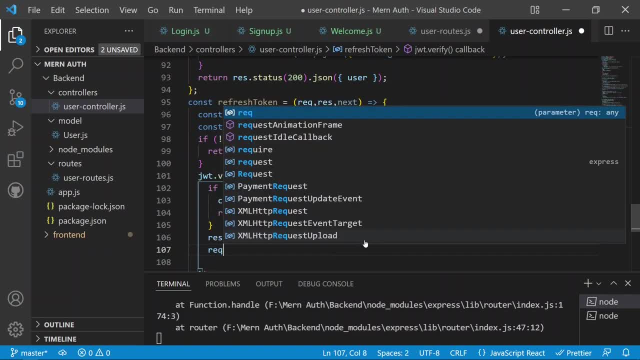 and then we will return, and then we will just clear the cookie from there, just clear the cookie from there. just clear the cookie from there. and for the headers also, then we can, and for the headers also, then we can, and for the headers also, then we can remove the cookie from the headers also. 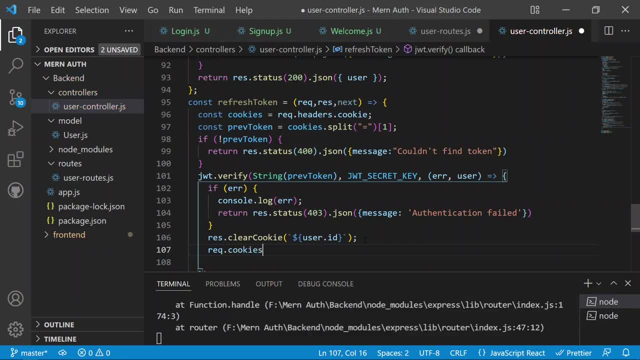 remove the cookie from the headers also. remove the cookie from the headers also. that will the request dot cookies, that will the request dot cookies, that will the request dot cookies and it will be like the cookies is and it will be like the cookies is and it will be like the cookies is objects. so we can just get the. 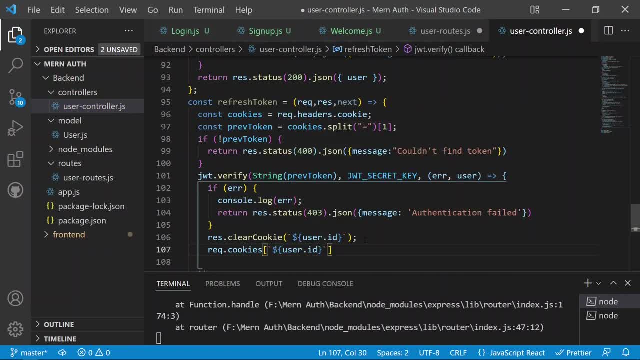 objects, so we can just get the objects. so we can just get the key of the user dot id. so we can just key of the user dot id. so we can just key of the user dot id. so we can just get, and it will, and we will just add it. 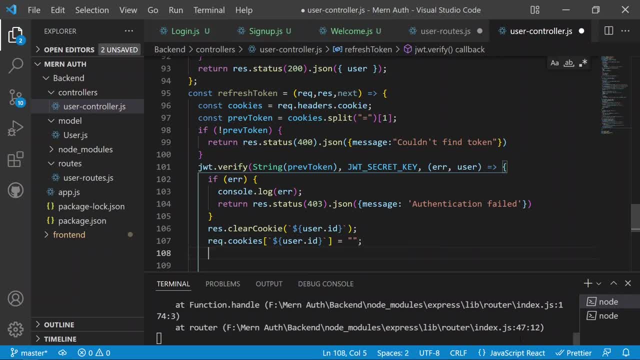 get and it will, and we will just add it get and it will, and we will just add it to the empty string, to the empty string, to the empty string. so it is the empty string now and then. so it is the empty string now and then. so it is the empty string now and then, after everything is done, then we can. 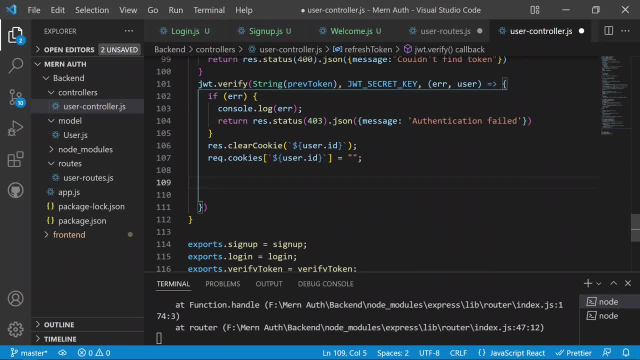 after everything is done, then we can. after everything is done, then we can generate a new token there. so now, what generate a new token there? so now, what generate a new token there? so now, what we are doing here? we are just verifying. we are doing here, we are just verifying. 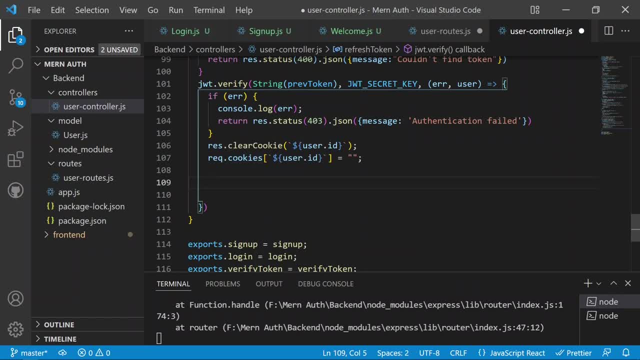 we are doing here? we are just verifying the token. if the token is successfully the token, if the token is successfully the token, if the token is successfully verified, then now we are removing the verified, then now we are removing the verified, then now we are removing the cookie, because the cookie contains a. 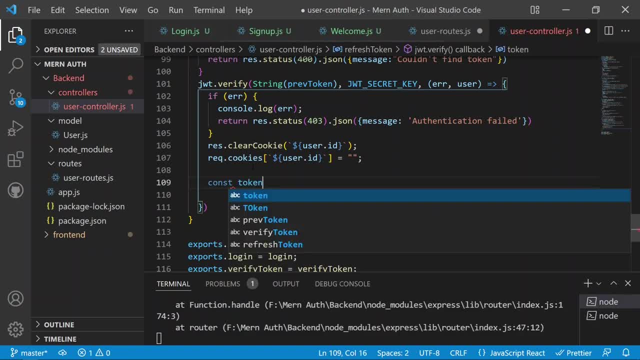 cookie, because the cookie contains a cookie, because the cookie contains a token, and then we will generate a new token, and then we will generate a new token, and then we will generate a new token, as it goes as the token will be. token as it goes, as the token will be. 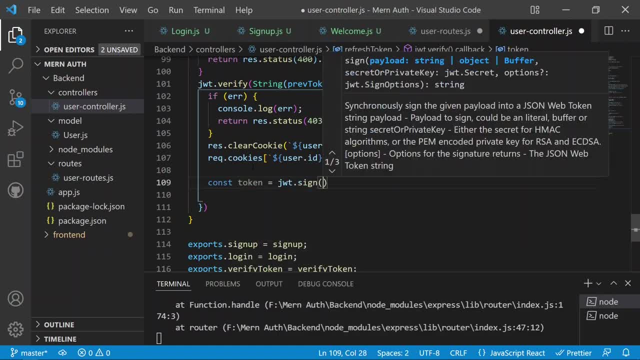 token as it goes, as the token will be: equals to jwt, again, equals to jwt, again, equals to jwt, again, dot sign and we will sign a new token. dot sign and we will sign a new token. dot sign and we will sign a new token with the parameter of the id as which we. 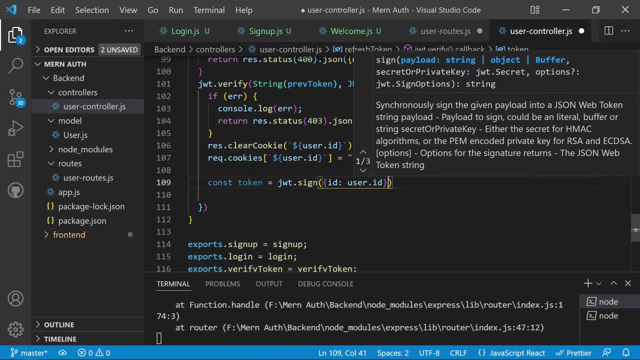 with the parameter of the id as which we, with the parameter of the id as which we will receive the userid which we have, will receive the userid which we have, will receive the userid which we have decoded, and then we can just add a decoded, and then we can just add a. 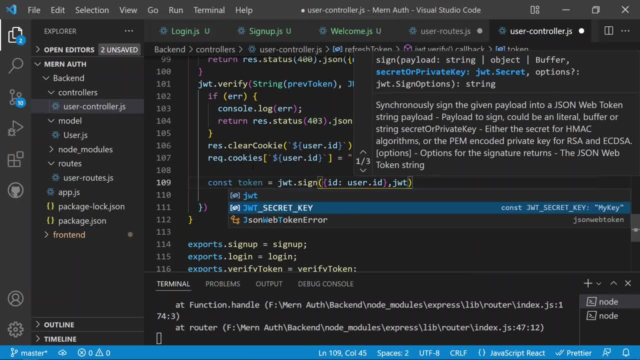 decoded, and then we can just add a parameter after that as a secret key, so parameter after that as a secret key, so parameter after that as a secret key. so we have already defined the secret key, we have already defined the secret key, we have already defined the secret key. and then we can just use an object and 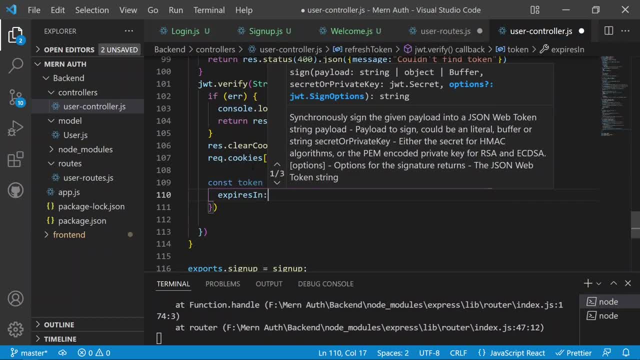 and then we can just use an object, and, and then we can just use an object and the object will contain an expires in the object, will contain an expires in the object, will contain an expires in property again, and we need to define the property again and we need to define the. 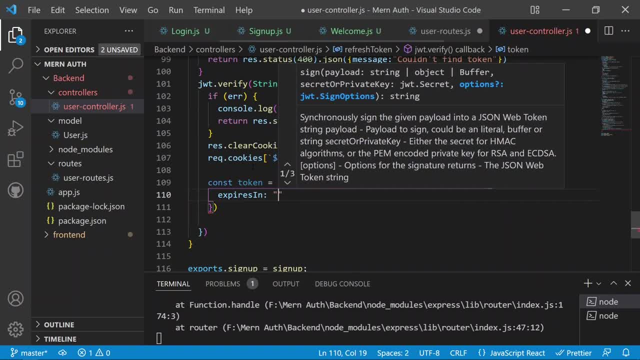 property again and we need to define the value, as again like the 30 seconds value, as again like the 30 seconds value, as again like the 30 seconds. so to the 30 seconds we are now defining, so to the 30 seconds we are now defining. 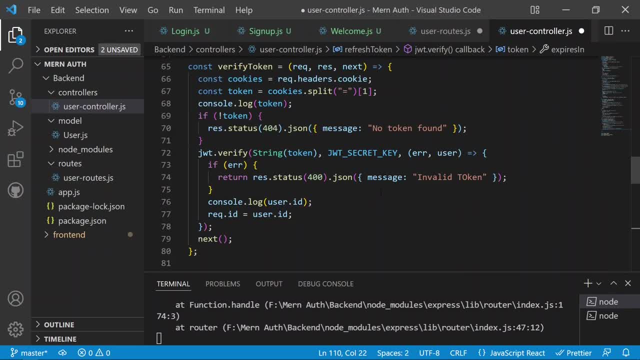 so to the 30 seconds. we are now defining the expires in property. so we are the expires in property. so we are the expires in property. so we are already defining 30 seconds in the. i already defining 30 seconds in the. i already defining 30 seconds in the. i think in the login as well, as we are. 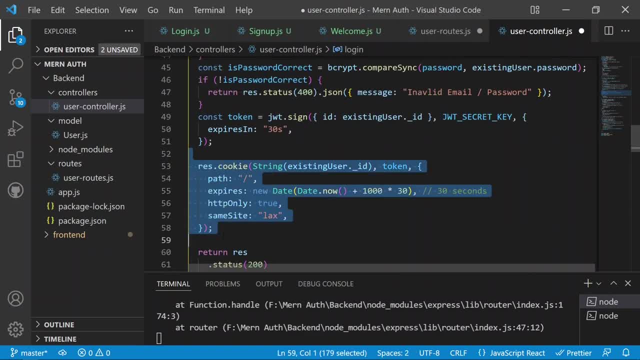 think in the login as well, as we are, think in the login as well, as we are defining in the 30 seconds. now you can defining in the 30 seconds, now you can defining in the 30 seconds. now you can see, and then we need to define the. 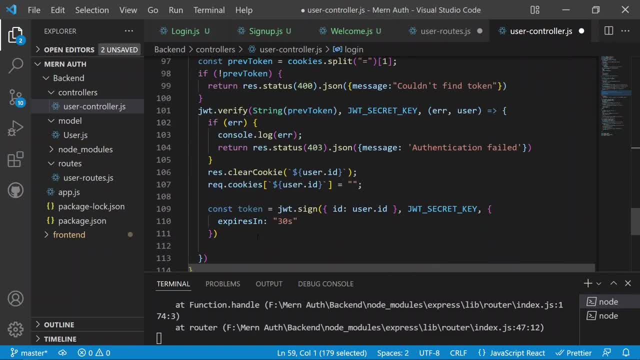 see, and then we need to define the see, and then we need to define the cookie as well again. cookie as well again. cookie as well again. so it will be the cookie after that, so after the expiration, so after the, so after the expiration, so after the, so after the expiration, so after the token will be created. then we can just 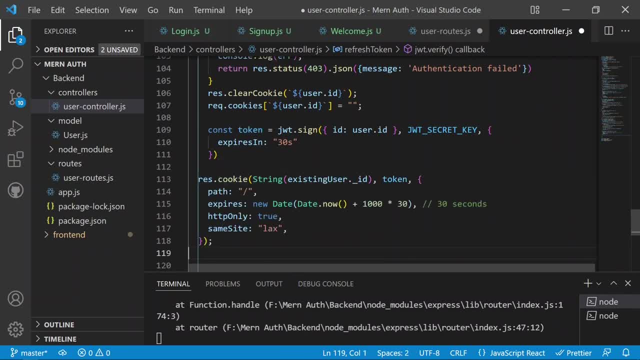 token will be created, then we can just token will be created, then we can just regenerate the cookie as well with the regenerate the cookie as well, with the regenerate the cookie as well, with the response dot cookie, and we are now response dot cookie, and we are now 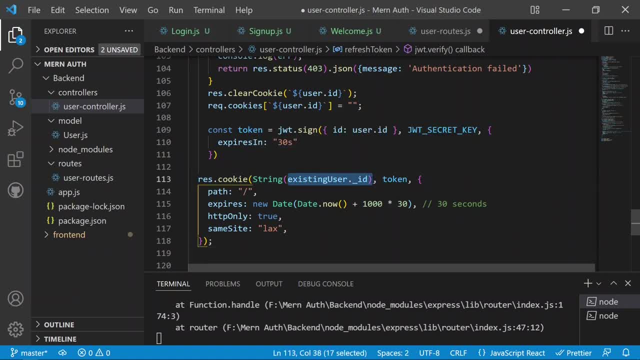 response: dot cookie and we are now sending the cookie. so now, this time, this sending the cookie. so now, this time, this sending the cookie. so now, this time, this will not be there, so it will be like the will not be there, so it will be like the. 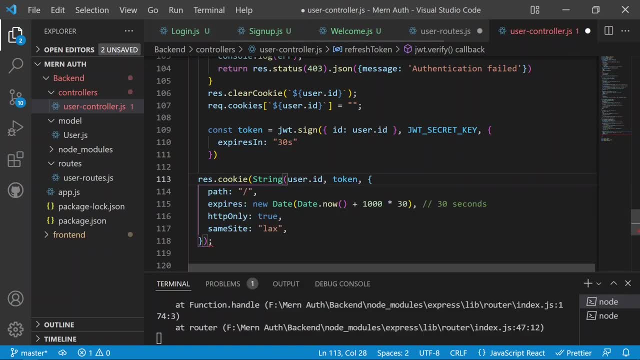 will not be there. so it will be like the id will be user dot id. so we are now id will be user dot id. so we are now id will be user dot id. so we are now getting the user dot id and then the. getting the user dot id and then the. 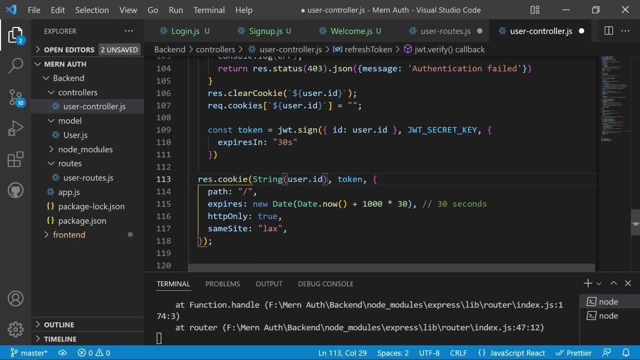 getting the user dot id and then the token, and then the path is equal to this token, and then the path is equal to this token, and then the path is equal to this and the expire is equal to 30 second is. and the expire is equal to 30 second is. 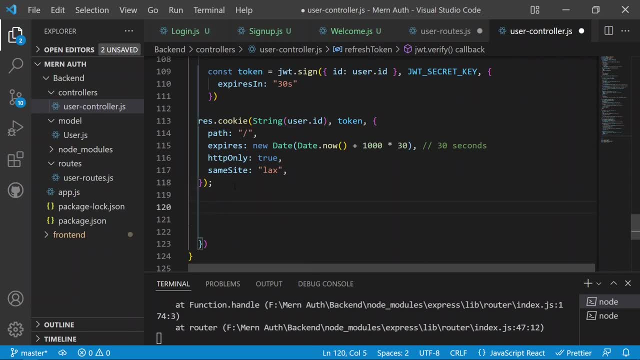 and the expire is equal to 30. second is again http only true, and everything is again http only true, and everything is again http only true, and everything is fine. and after the cookies generated: now fine. and after the cookies generated: now fine. and after the cookies generated, now the most important part now, the cookie. 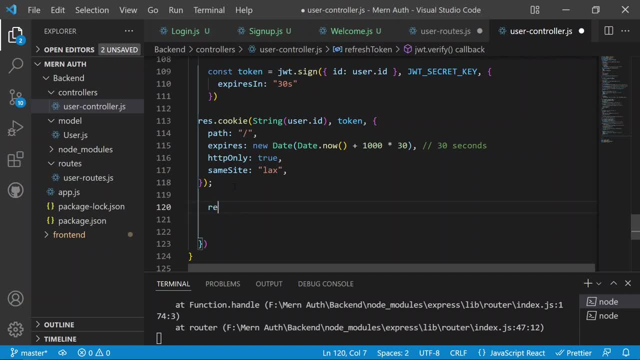 the most important part now: the cookie. the most important part: now the cookie is generated and the token is also is generated and the token is also is generated and the token is also regenerated. and now we need to again add regenerated. and now we need to again add: 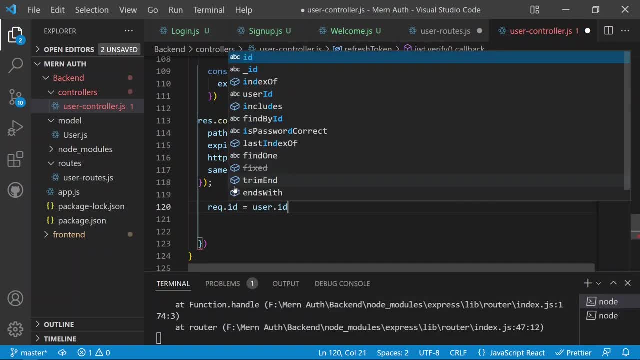 regenerated and now we need to again add the requestid, which will be equals to the requestid, which will be equals to the requestid, which will be equals to the userid which we have decoded, the userid which we have decoded, the userid which we have decoded. so now for this id. now we want to move. 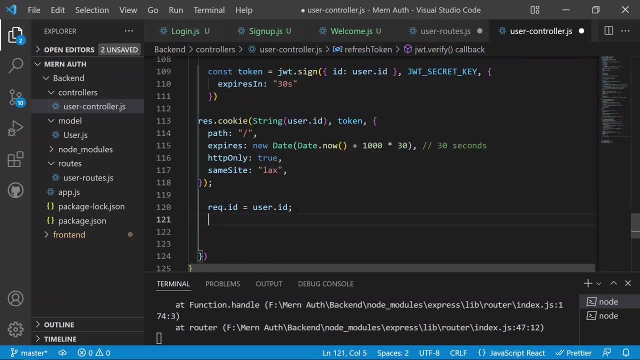 so now for this id. now we want to move. so now for this id. now we want to move on to the next middleware. after that, on to the next middleware, after that, on to the next middleware after that. so now we have the id and we are now. 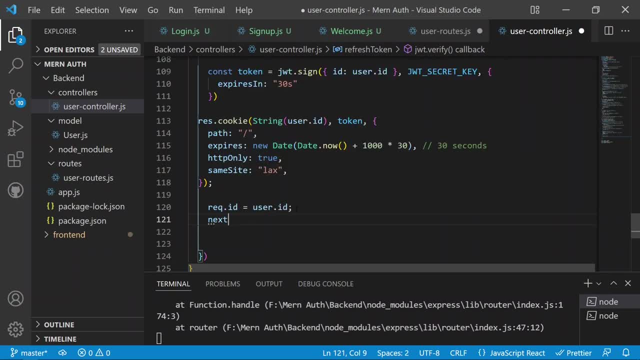 so now we have the id and we are now. so now we have the id and we are now attaching the requestid with the userid, attaching the requestid with the userid, attaching the requestid with the userid and now, after that, we can just move on. 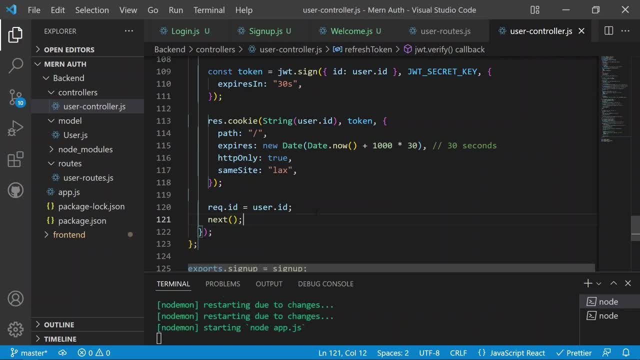 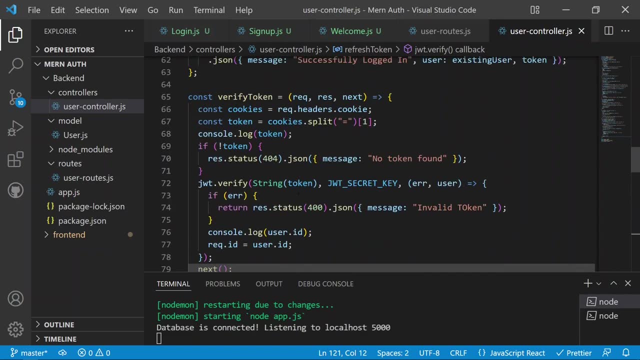 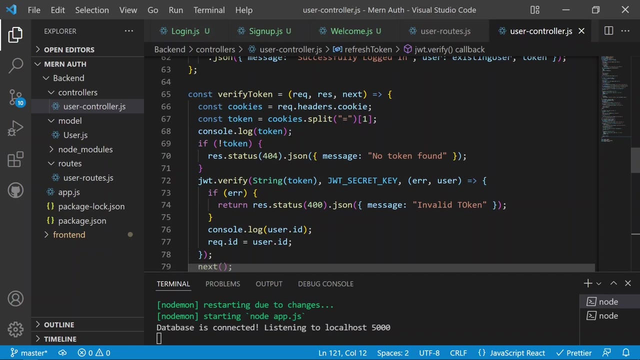 and now, after that, we can just move on, and now, after that, we can just move on to the next middleware and in the next, to the next middleware, and in the next to the next middleware and in the next middleware, the next middleware will be, and then, after the verification is: 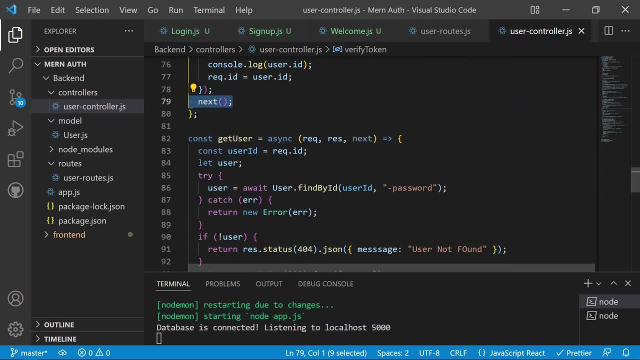 and then after the verification is, and then after the verification is successful, then we can just move on to successful, then we can just move on to successful, then we can just move on to the next, the next, the next, and then we can just show the user with: 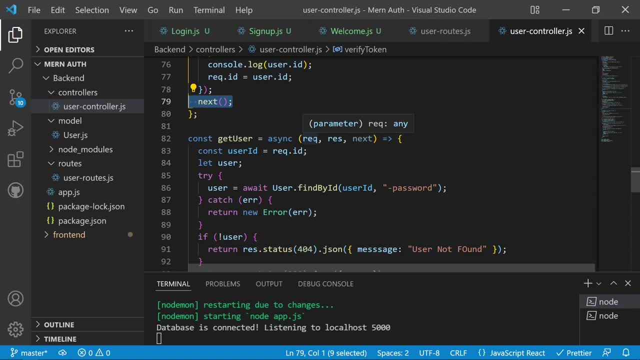 and then we can just show the user with, and then we can just show the user with the requestid, the requestid, the requestid. so this is very complex logic, but it is so. this is very complex logic, but it is so. this is very complex logic, but it is very good logic for the security reasons. very good logic for the security reasons. very good logic for the security reasons. so then we can move on to the route. so so then we can move on to the route. so so then we can move on to the route. so, after the token is going to the, 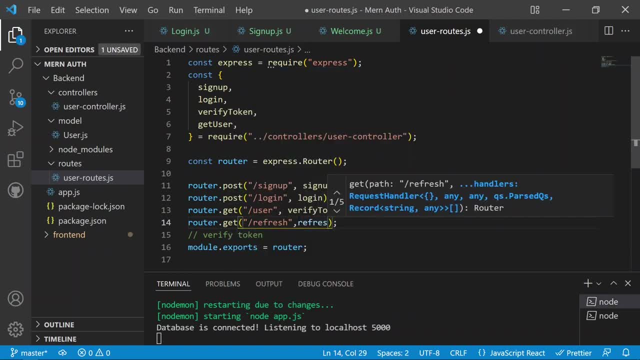 after the token is going to the: after the token is going to the refreshed, then we can run a refresh refreshed. then we can run a refresh refreshed. then we can run a refresh token, token token. so we need to export the refresh token. so we need to export the refresh token. 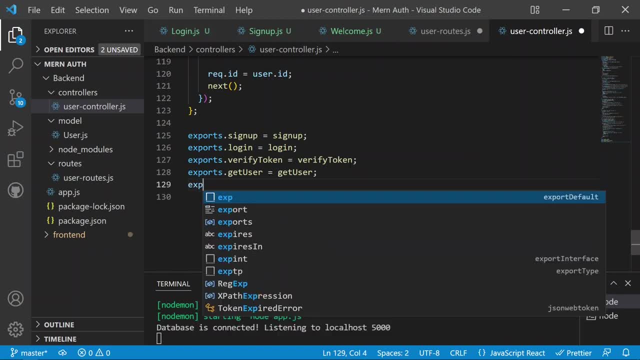 so we need to export the refresh token as well. so it will be as well. so it will be as well. so it will be: export dot refresh token will, because export dot refresh token will, because export dot refresh token will, because so refresh token. so now we're exporting. 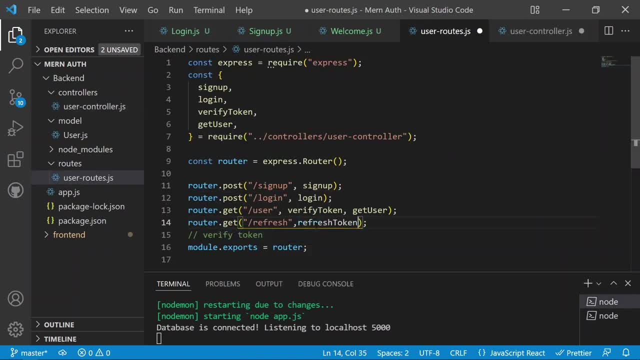 so refresh token. so now we're exporting so refresh token. so now we're exporting the refresh token as well, the refresh token as well, the refresh token as well, and then we are now just adding the, and then we are now just adding the, and then we are now just adding the refresh token. 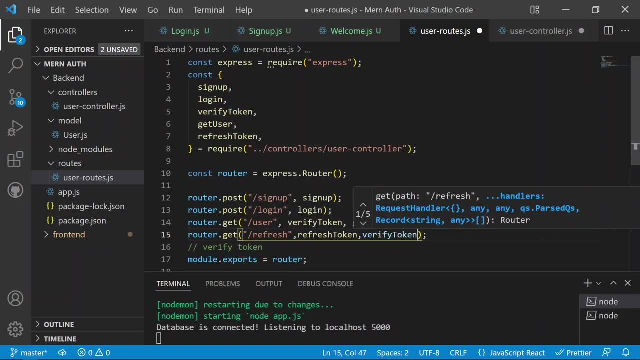 refresh token, refresh token. and after the refresh token, now we will. and after the refresh token, now we will. and after the refresh token, now we will. verify the token as well again. verify the token as well. again verify the token as well. again verified token. and then, after the 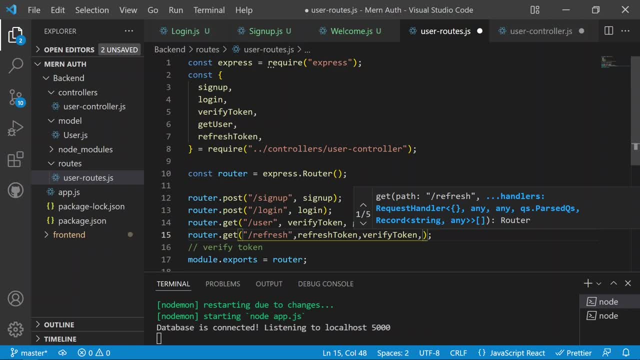 verified token, and then, after the verified token, and then after the refresh is completed, verify is completed. refresh is completed. verify is completed. refresh is completed. verify is completed, and then the final thing will be which, and then the final thing will be which, and then the final thing will be which will be the get user. so now we are. 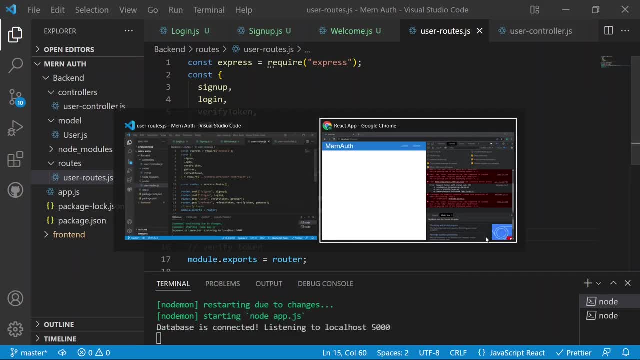 will be the get user. so now we are will be the get user. so now we are defining the get user. so if i will now defining the get user, so if i will now defining the get user, so if i will now save, and now in the front, and now we 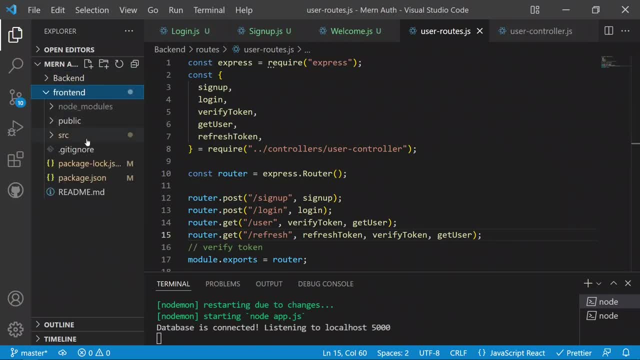 save, and now in the front, and now we save. and now in the front. and now we need to work in the front end. to just need to work in the front end, to just need to work in the front end to just send the request after every time span. 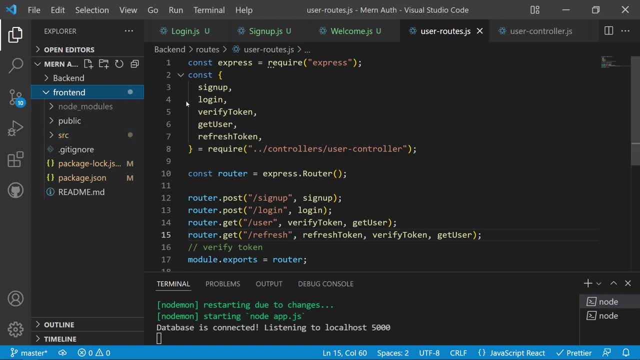 send the request after every time span. send the request after every time span of 30 seconds. so we can just do that of 30 seconds. so we can just do that of 30 seconds. so we can just do that. and for the request, so request can take. 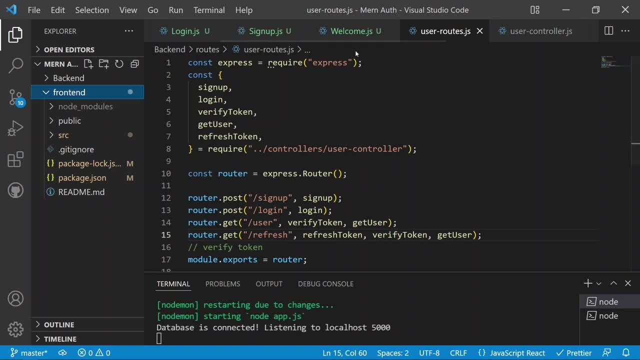 and for the request, so request can take. and for the request, so request can take time because it is an asynchronous task time. because it is an asynchronous task time, because it is an asynchronous task, so we can just go to the user controller. so we can just go to the user controller. 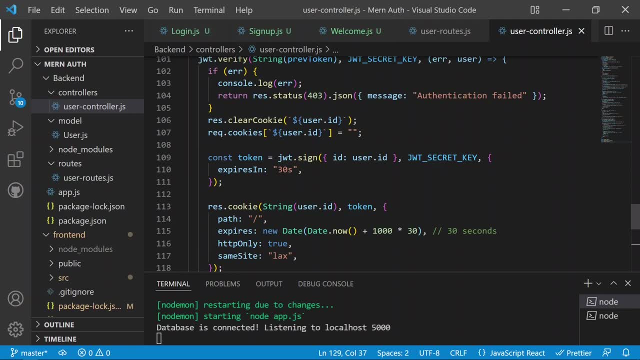 so we can just go to the user controller and then we can just increase the time, and then we can just increase the time, and then we can just increase the time limit of the 30 seconds to 35 seconds. limit of the 30 seconds to 35 seconds. 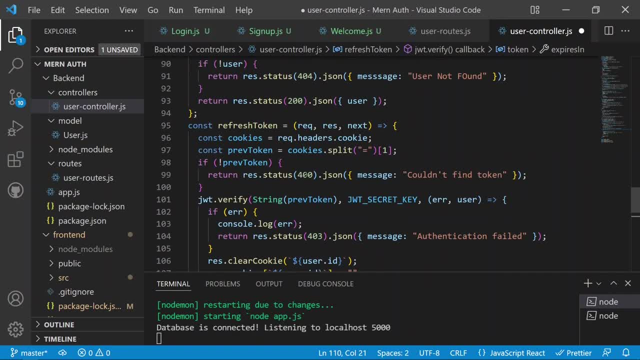 limit of the 30 seconds to 35 seconds. so it should be the. it should not be the. so it should be the. it should not be the, so it should be the. it should not be the exact time of that, so we can just remove. exact time of that, so we can just remove. 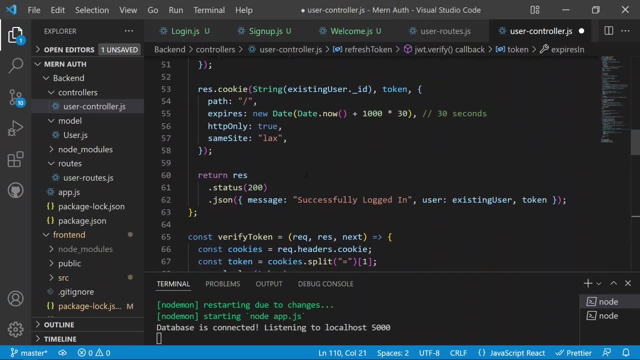 exact time of that. so we can just remove that, the time span of this, that the time span of this, that the time span of this, and then we can just remove that time, and then we can just remove that time, and then we can just remove that time span from the. 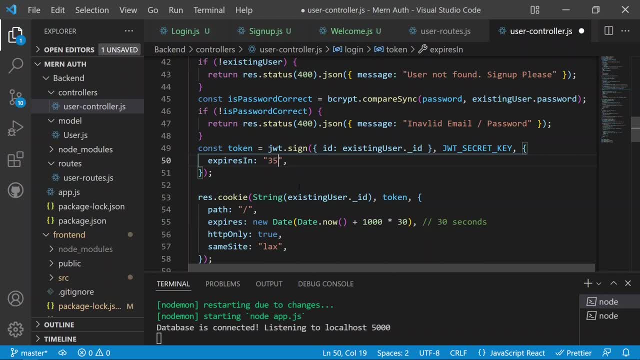 span from the span from the login as well, it will be 35 seconds. login as well, it will be 35 seconds. login as well, it will be 35 seconds. so after the 30 seconds, the cookie will. so after the 30 seconds, the cookie will. 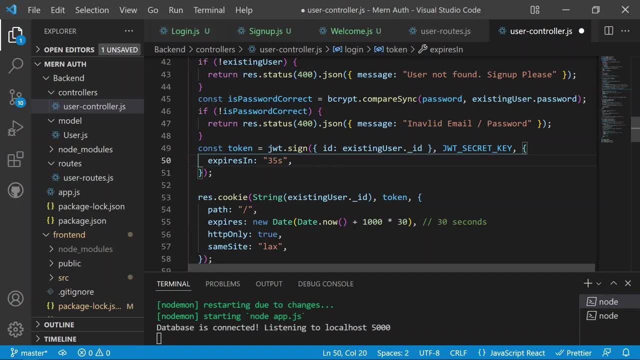 so after the 30 seconds, the cookie will so after that, so after that, so after that 30 seconds, the cookie will be then removed. 30 seconds: the cookie will be then removed. 30 seconds: the cookie will be then removed and it will remove the token as well. 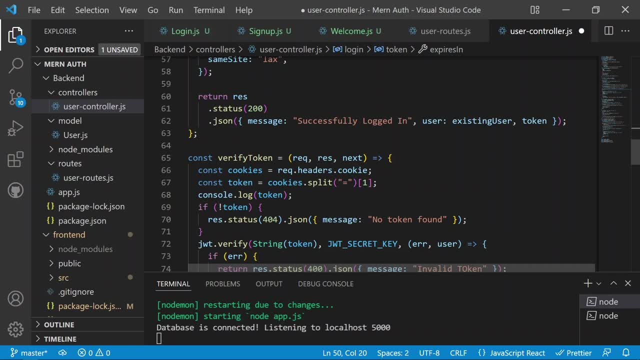 and it will remove the token as well. and it will remove the token as well. so the again the token will be generated. so the again the token will be generated, so the again the token will be generated. for the 35 seconds, but for the 35 seconds. but. 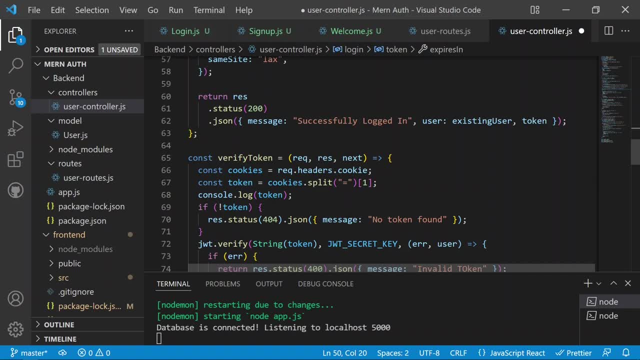 for the 35 seconds, but after the 30 seconds we will just destroy. after the 30 seconds, we will just destroy. after the 30 seconds, we will just destroy and we will just create a new token and we will just create a new token and we will just create a new token so we can just move on to the user. 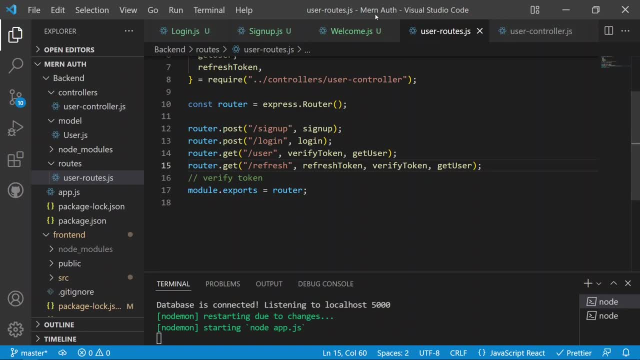 so we can just move on to the user. so we can just move on to the user routes again, and then everything is routes again, and then everything is routes again, and then everything is working fine, and then we need to go to working fine, and then we need to go to. 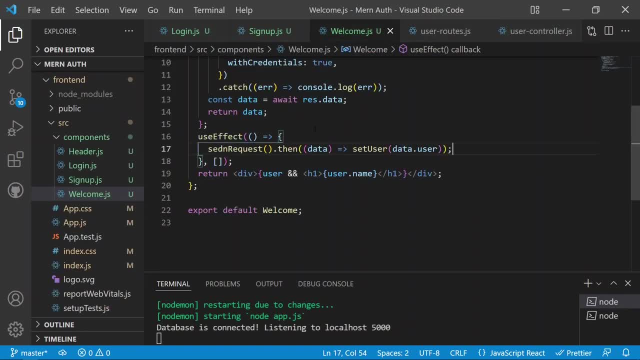 working fine. and then we need to go to the welcomejs in which we will send the, the welcomejs in which we will send the, the welcomejs in which we will send the request, request, request. so so here in the welcomejs, now we need. so so, here in the welcomejs, now we need. 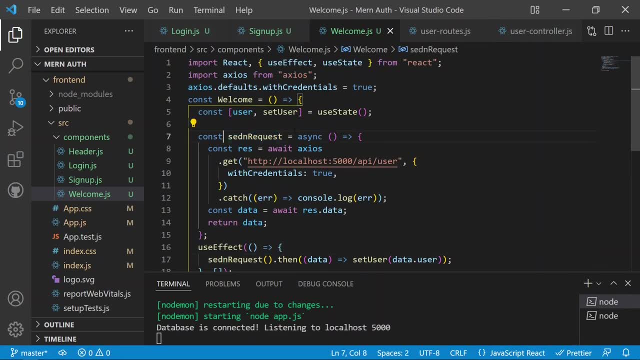 so so here in the welcomejs: now we need to generate a new function. now we need to generate a new function. now we need to generate a new function. now we need to create a new function, to create a new function, to create a new function as the refresh. so it so, before the send: 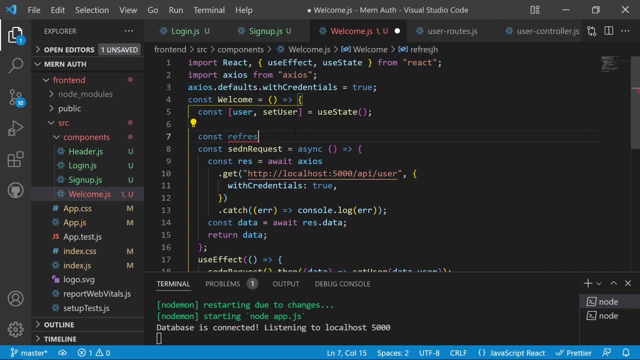 as the refresh. so it so before the send. as the refresh. so it so before the send request. i will generate a new function request. i will generate a new function request. i will generate a new function as the refresh token and it will be equals to a token. and it will be equals to a. 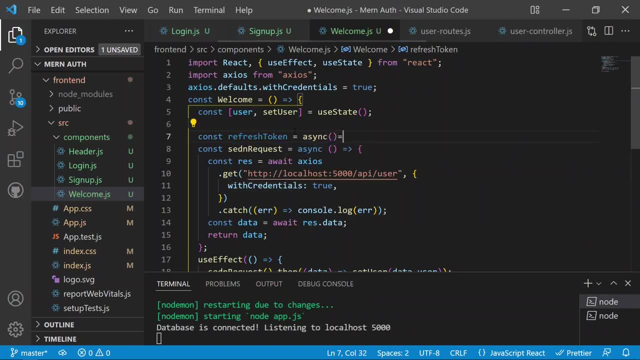 token, and it will be equals to a asynchronous function again as the async. asynchronous function, again as the async. asynchronous function, again as the async, and then we can just generate a new, and then we can just generate a new, and then we can just generate a new response variable, again as the response. 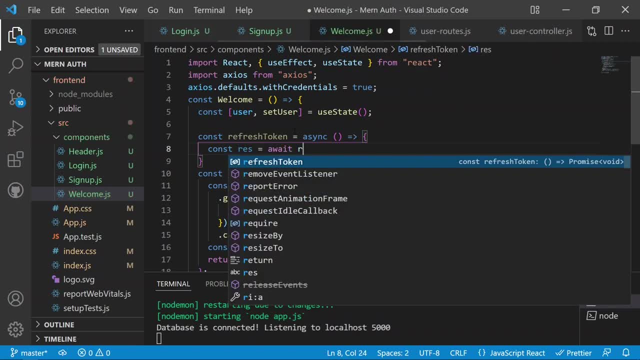 response variable again as the response, response variable again, as the response will be equals to the await and it will will be equals to the await and it will will be equals to the await and it will be like the be, like the be, like the. uh, i think the axios which we have, 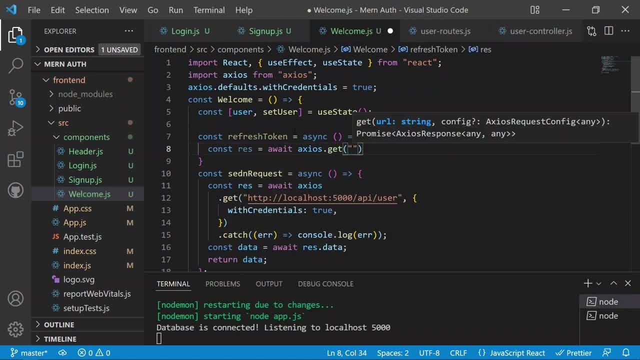 uh, i think the axios which we have, uh, i think the axios which we have, imported dot get, and this is a get http- imported dot get, and this is a get http- imported dot get, and this is a get http request, and then we can just add the. 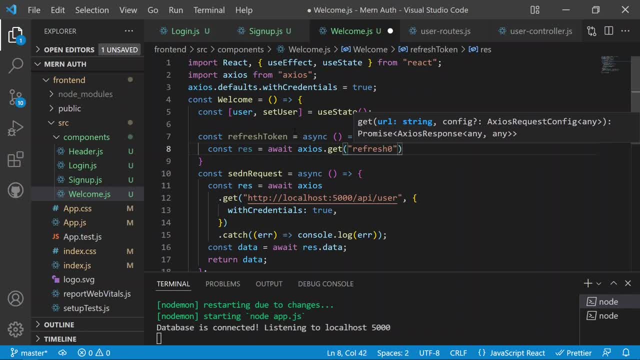 request, and then we can just add the request, and then we can just add the refresh, refresh, refresh, refresh is there, and then after the refresh is there, and then after the refresh is there, and then after the refresh. so i think the route will be refreshed, so. so i think the route will be refreshed. so 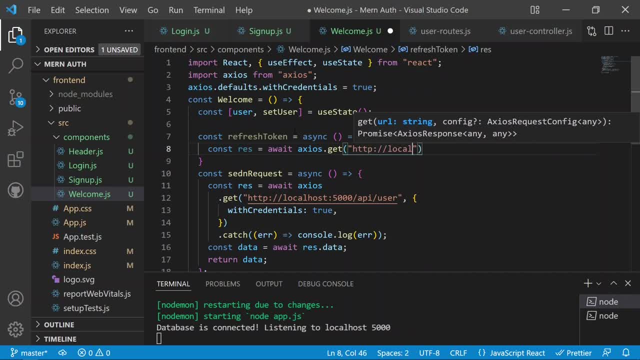 so i think the route will be refreshed. so the http, the http, the http, localhost, localhost, localhost. at the report of the 5000, then api, then at the report of the 5000, then api, then at the report of the 5000, then api, then refresh. 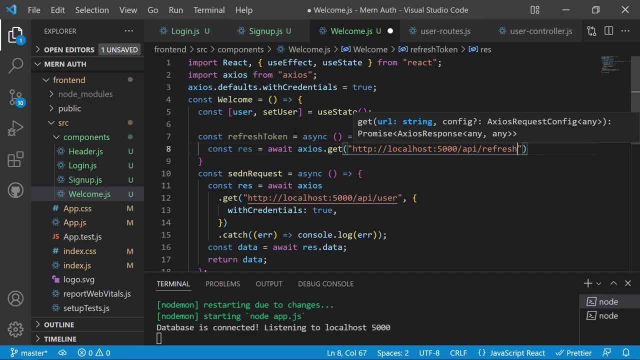 refresh, refresh, so we will send the refresh as well after. so we will send the refresh as well after. so we will send the refresh as well after that. that that. so if the route will match the refresh, so if the route will match the refresh, so if the route will match the refresh, so it will work. so now it is the refresh. 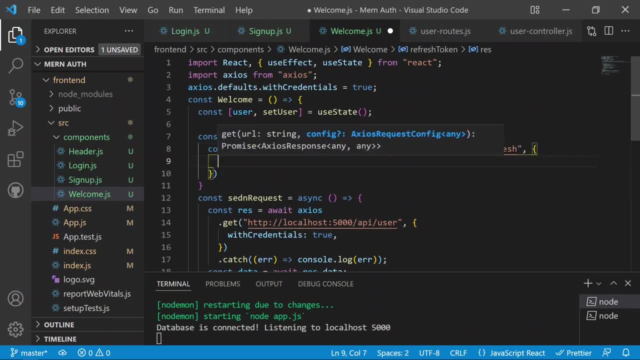 so it will work. so now it is the refresh. so if the route will match the refresh, again it will work fine. and in the, again it will work fine. and in the, again it will work fine. and in the second object: now we need to again send. second object: now we need to again send. 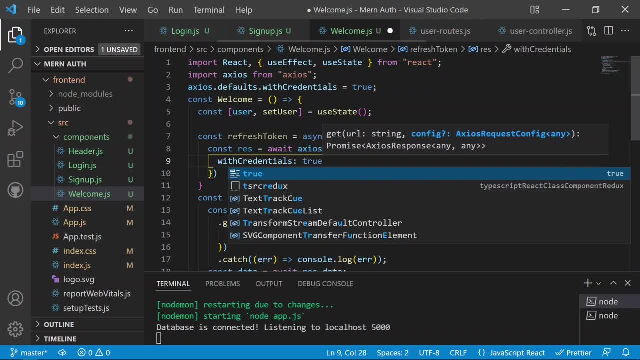 second object: now we need to again send the width credentials, the width credentials, the width credentials, and it will be equals to the true because, and it will be equals to the true because, and it will be equals to the true because we need to send the credentials also to 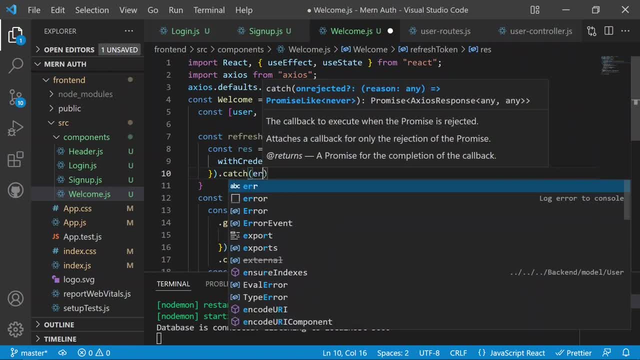 we need to send the credentials also to. we need to send the credentials also to verify the token. verify the token, verify the token, and then we can just catch the error. if, and then we can just catch the error if, and then we can just catch the error. if there is any error, then we can just. 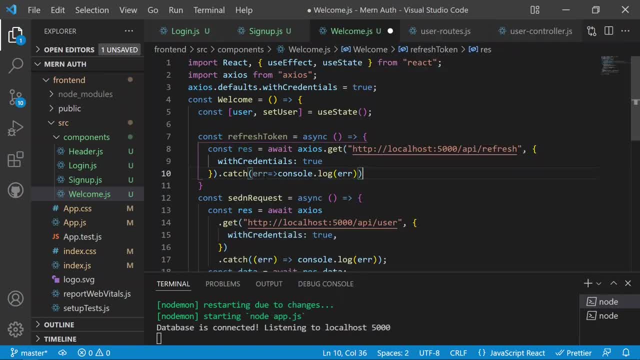 there is any error, then we can just: there is any error, then we can just consolelog, consolelog, consolelog, the error that we receive, the error that we receive, the error that we receive. so after the response, then we can just. so after the response, then we can just. 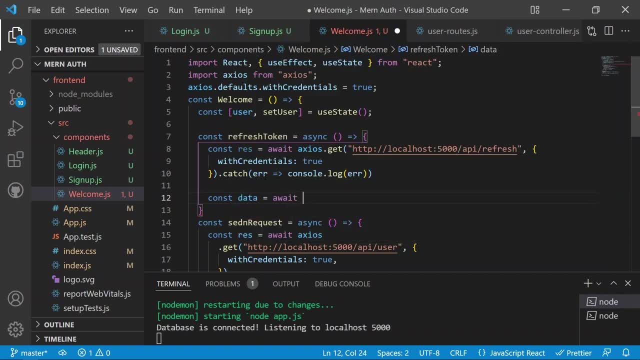 so after the response then we can just get the data again: cause data will get. get the data again: cause data will get. get the data again: cause data will get the await at the response- dot data. the await at the response- dot data. the await at the response- dot data. so if everything is successful, then we 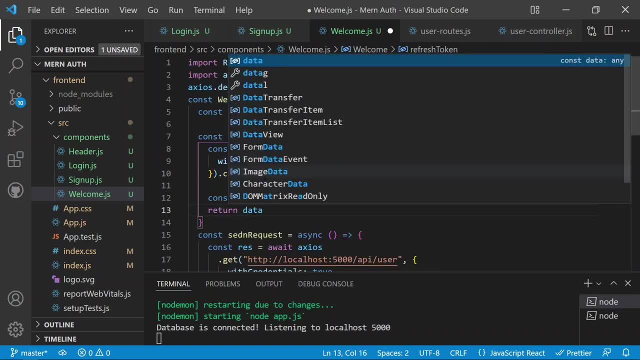 so if everything is successful, then we. so if everything is successful, then we can just get the data, and then we will can just get the data, and then we will can just get the data, and then we will just return the data, just return the data, just return the data and then after that, now we need to use. 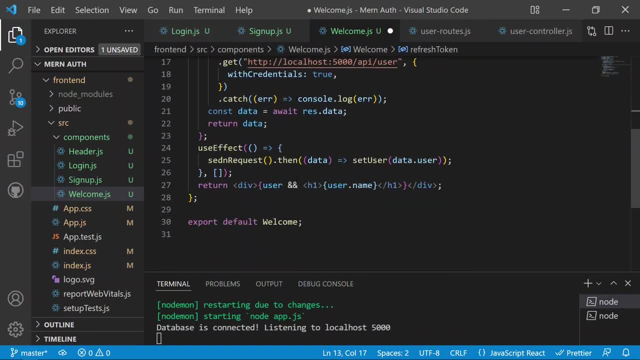 and then after that, now we need to use, and then after that, now we need to use the set interval method from the, the set interval method from the, the set interval method from the after every 15 seconds. so we need to do after every 15 seconds. so we need to do. 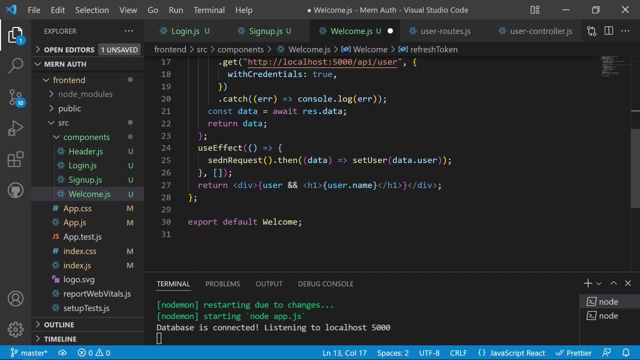 after every 15 seconds. so we need to do that. so we can just go to the use that, so we can just go to the use that, so we can just go to the use effects. so for the first render, so i effects. so for the first render, so i. 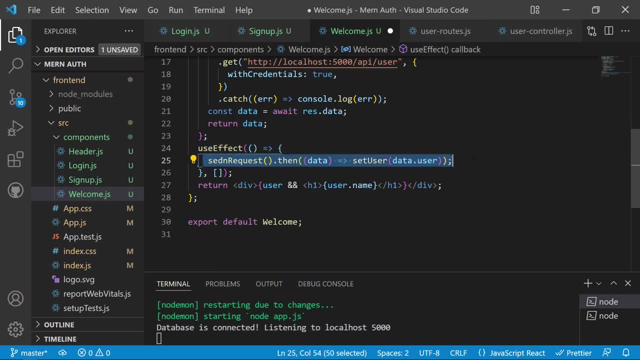 effects, so for the first render. so i think in the use effect we need to think in the use effect. we need to think in the use effect. we need to create a logic that on the first render create a logic, that on the first render create a logic that on the first render we need to render the send request. 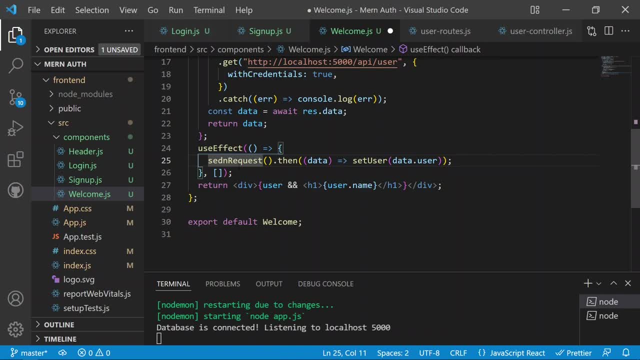 we need to render the send request, we need to render the send request, and after the first render then we need to. and after the first render, then we need to. and after the first render, then we need to render the refresh token. render the refresh token, render the refresh token. so for the logic, we can just generate a. 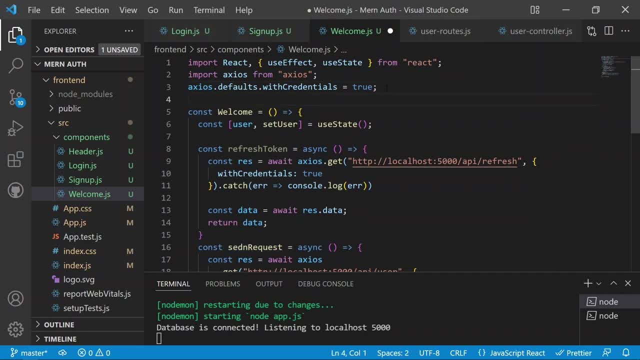 so for the logic, we can just generate a. so for the logic, we can just generate a new variable here, new variable here, new variable here. we can just create a new variable here. we can just create a new variable here. we can just create a new variable here, before the rendering, and it will be the. 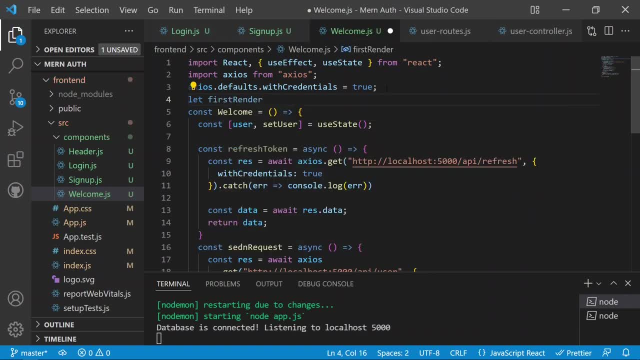 before the rendering, and it will be the before the rendering and it will be the let, let, let as the first render and it will be by as the first render and it will be by as the first render and it will be by default equals to the false. 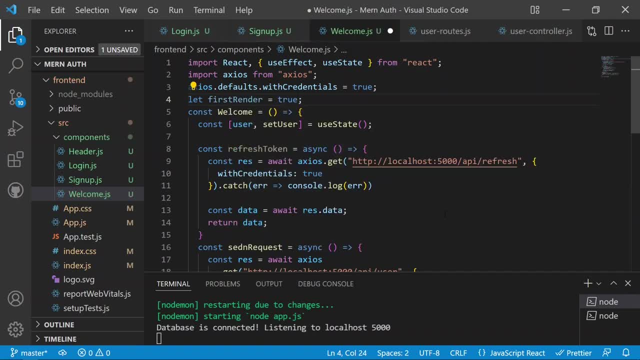 default equals to the false, default equals to the false, or like the first render will be equals, or like the first render will be equals, or like the first render will be equals to the true. i think to the true, i think to the true. i think so first render is true, and then we can. 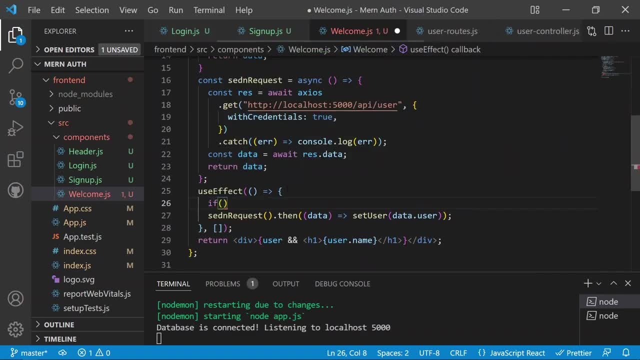 so first render is true and then we can. so first render is true and then we can just check in the use effect, like just check in the use effect, like just check in the use effect, like if we have the first render and then we need to just send the. 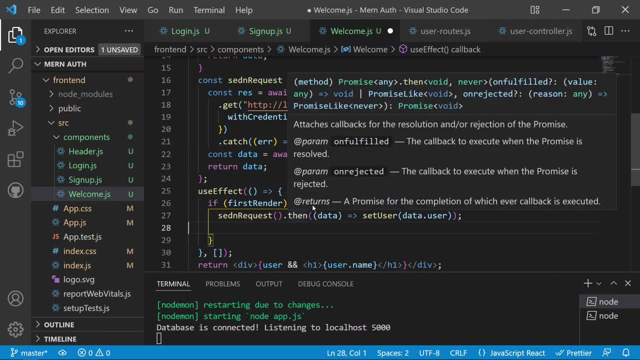 and then we need to just send the, and then we need to just send the request request, request to get the user, and after that so to get the user, and after that so to get the user, and after that so and after that. we can just use here like i. and after that we can just use here like i, and after that we can just use here, like i think we need to just update the first think. we need to just update the first think. we need to just update the first render as well. i like the first render. 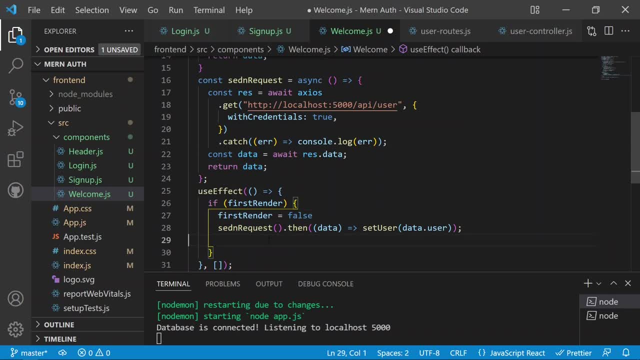 render as well. i like the first render render as well. i like the first render. equals to the false, equals to the false, equals to the false. so now for the first render, we are now. so now for the first render, we are now. so now for the first render. we are now sending the request to the user. 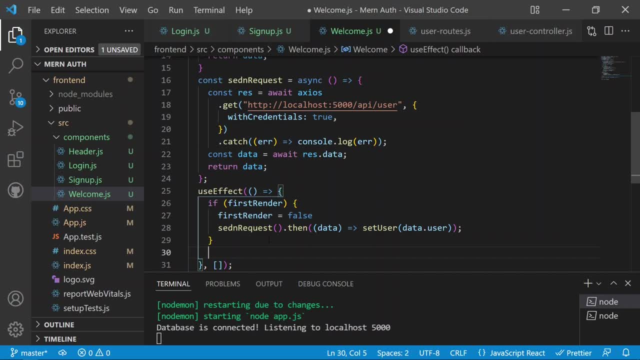 sending the request to the user. sending the request to the user. and if the first render is not there now, and if the first render is not there now, and if the first render is not there now, we can just use here the use effect. we can just use here the use effect. 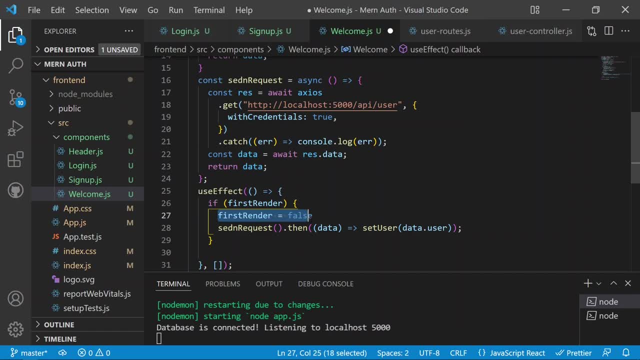 we can just use here the use effect: now if the first render is true, and now now, if the first render is true. and now now, if the first render is true, and now, we are now providing the first render, we are now providing the first render, we are now providing the first render equals to the false and we are sending. 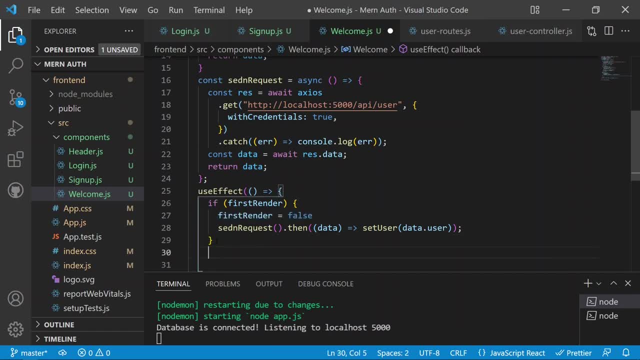 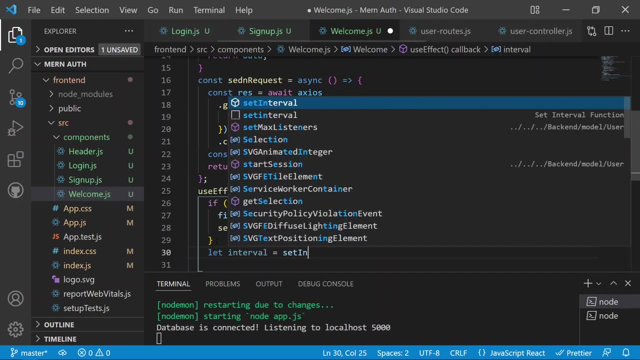 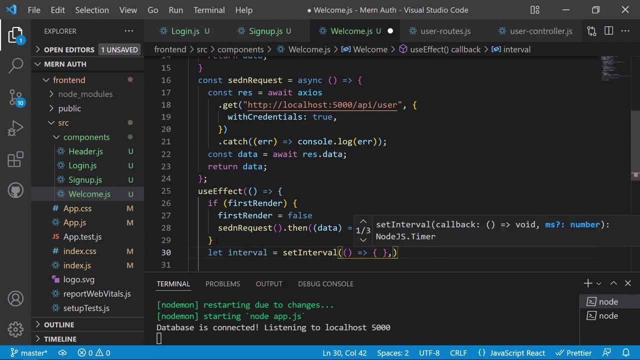 equals to the false and we are sending equals to the false and we are sending the request and in the else case we need the request and in the else case we need the request and in the else case, we need to provide here the milliseconds, to provide here the milliseconds. 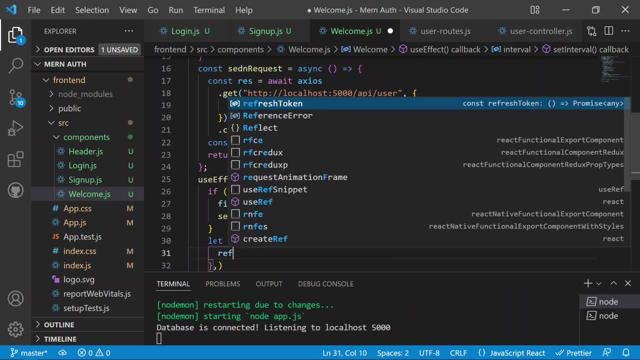 to provide here the milliseconds. so what we need to do in the set, so what we need to do in the set, so what we need to do in the set interval is we need to run the refresh interval. is we need to run the refresh interval, is we need to run the refresh token function. 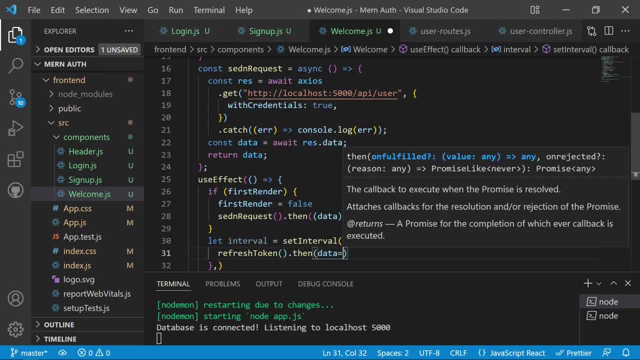 token function, token function. and then we need to send the data, and, and then we need to send the data, and and then we need to send the data, and then the data which we will receive. we then the data which we will receive, we then the data which we will receive. we will set user, again the data, so the set. 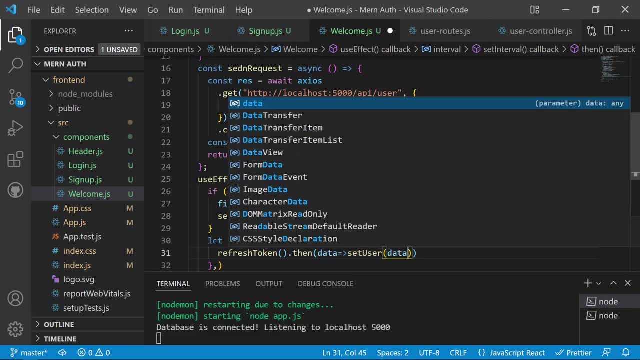 will set user again the data, so the set will set user again the data, so the set user will be equals to the data again. user will be equals to the data again. user will be equals to the data again. so this is the logic of it. and then now: 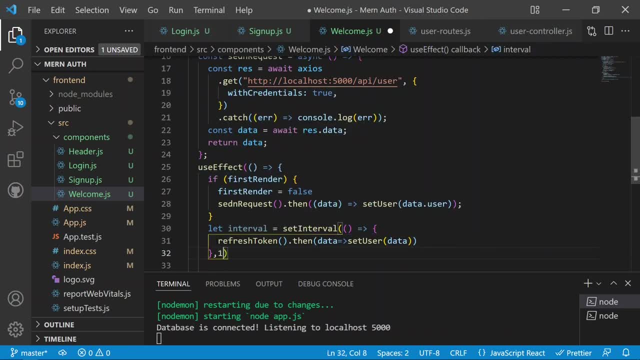 so this is the logic of it, and then now: so this is the logic of it, and then now we can see now if everything works fine. we can see now if everything works fine. we can see now if everything works fine, and now we can add a time span of around. 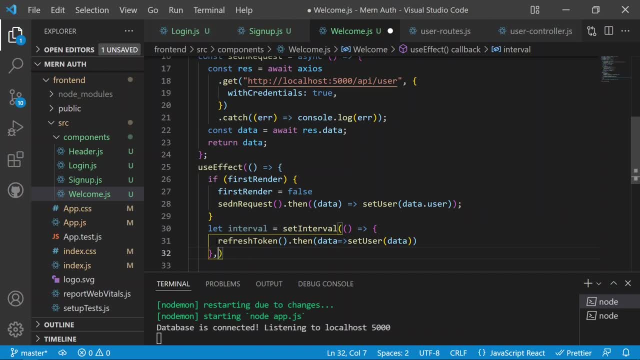 and now we can add a time span of around. and now we can add a time span of around, something like, something like, something like we are setting up the cookie, we are, we are setting up the cookie, we are, we are setting up the cookie, we are setting up the token for 35 seconds and. setting up the token for 35 seconds. and setting up the token for 35 seconds, and we are setting up the cookie for 30. we are setting up the cookie for 30. we are setting up the cookie for 30 seconds, so we can just run the refresh. 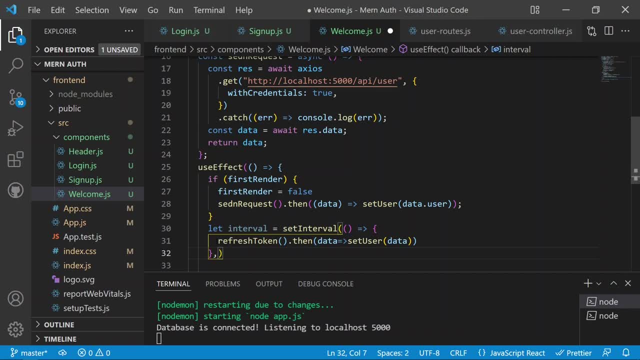 seconds, so we can just run the refresh seconds. so we can just run the refresh token after every. something like 28 token after every, something like 28 token after every something like 28 seconds or 29 seconds, so it will be seconds or 29 seconds, so it will be. 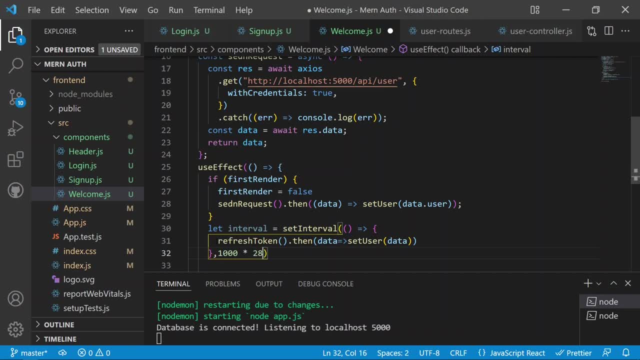 seconds or 29 seconds, so it will be thousand milliseconds, so it can be the thousand milliseconds, so it can be the thousand milliseconds, so it can be the 28. so after the 28 seconds, now we will 28. so after the 28 seconds, now we will. 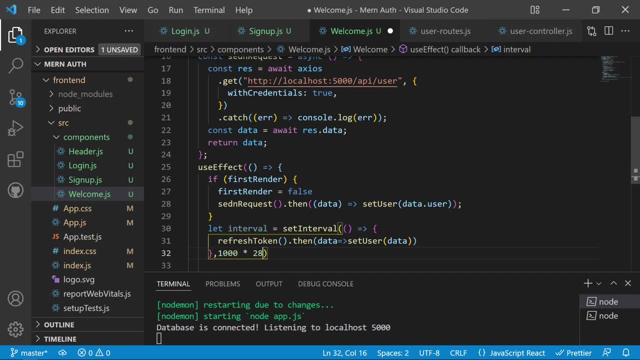 28, so after the 28 seconds now we will send the set interval function. so it send the set interval function. so it send the set interval function. so it will run after every 28 seconds and then will run after every 28 seconds and then will run after every 28 seconds and then it will run for the refresher out. so 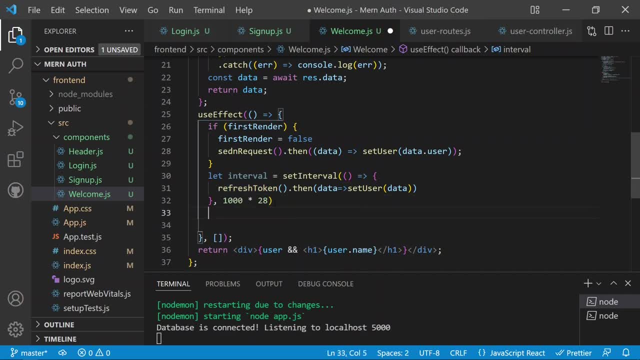 it will run for the refresher out, so it will run for the refresher out, so everything will work fine. and for that everything will work fine, and for that everything will work fine, and for that we need to also just return there. we need to also just return there. 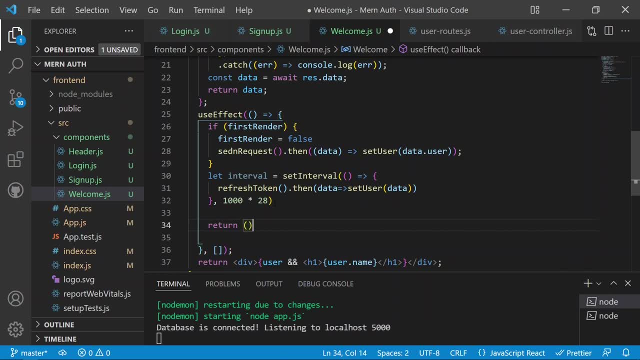 we need to also just return there something because we need to add a something, because we need to add a something, because we need to add a cleanup function also for the use effect. cleanup function also for the use effect. cleanup function also for the use effect to clean the interval after every. 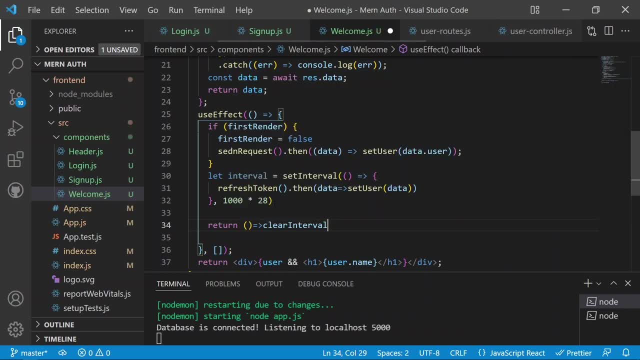 to clean the interval after every. to clean the interval after every 28 seconds, so it can be the clear 28 seconds, so it can be the clear 28 seconds, so it can be the clear interval interval interval, which is available already in the, which is available already in the. 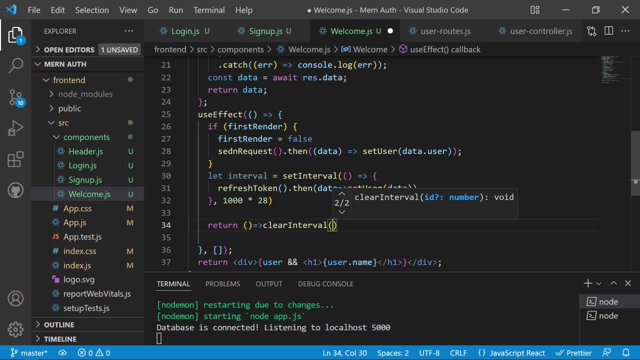 which is available already in the javascript vanilla javascript. so we can javascript vanilla javascript. so we can javascript vanilla javascript. so we can just clear the interval which we have just clear, the interval which we have just clear, the interval which we have defined, the interval, so this interval. 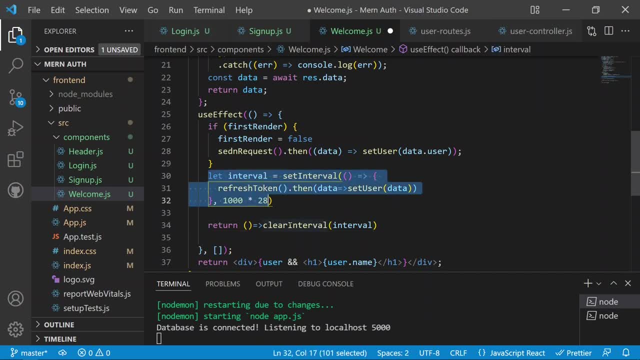 defined the interval. so this interval defined the interval. so this interval will always be expired after every 28, will always be expired after every 28, will always be expired after every 28 seconds once the cleanup is completed. seconds once the cleanup is completed, seconds once the cleanup is completed, and then we will generate a new interval. 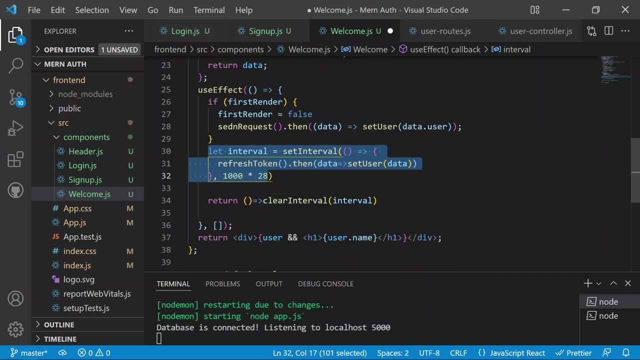 and then we will generate a new interval, and then we will generate a new interval, and then, if everything will work fine, and then, if everything will work fine, and then, if everything will work fine, then we can just then, we can just then, we can just have the username again and again. so now, 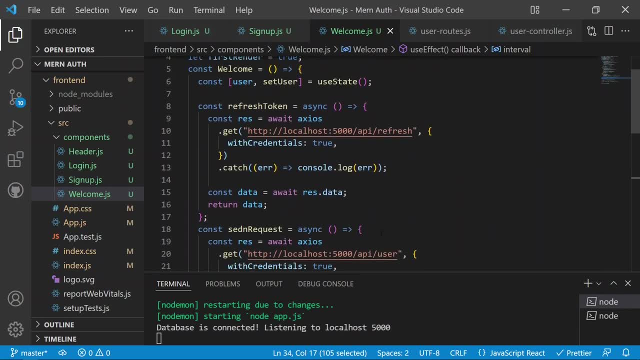 have the username again and again. so now have the username again and again. so now i think, if everything works fine, so we, i think, if everything works fine, so we. i think, if everything works fine, so we need to save, need to save, need to save, and then we can just go to the node. 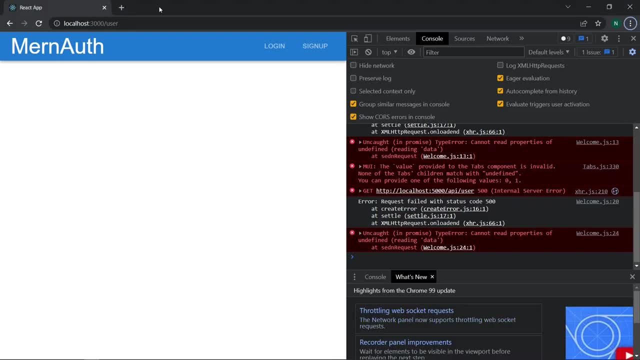 and then we can just go to the node, and then we can just go to the node again, again, again. so i think there is an error. so first we. so i think there is an error, so first we. so i think there is an error. so first we need to remove everything from there. we. 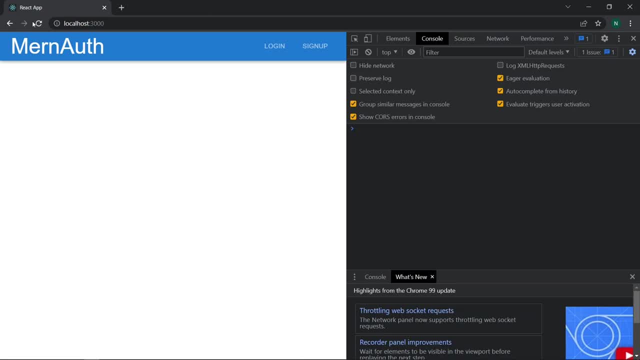 need to remove everything from there. we need to remove everything from there. we need to go to localhost thread 3000, need to go to localhost thread 3000, need to go to localhost thread 3000, and then we need to just remove the and then we need to just remove the. 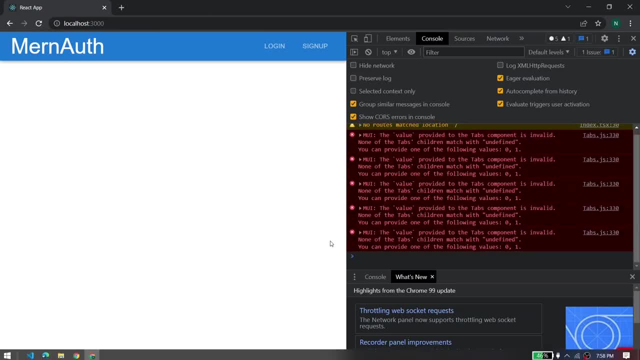 and then we need to just remove the cache as well. so i will remove the cache cache as well. so i will remove the cache cache as well. so i will remove the cache. and then now we need to run the request. and then now we need to run the request. 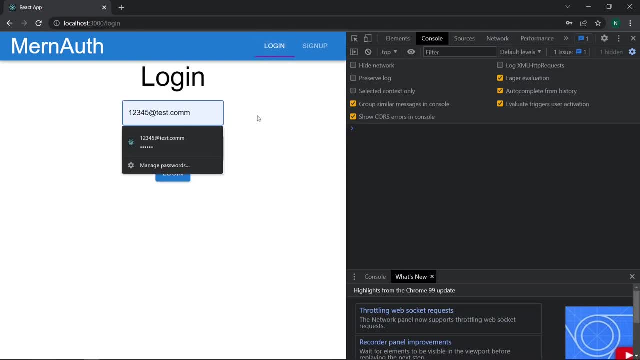 and then now we need to run the request. so first we need to go to the login. so first we need to go to the login. so first we need to go to the login, and i have already saved all of the. and i have already saved all of the. 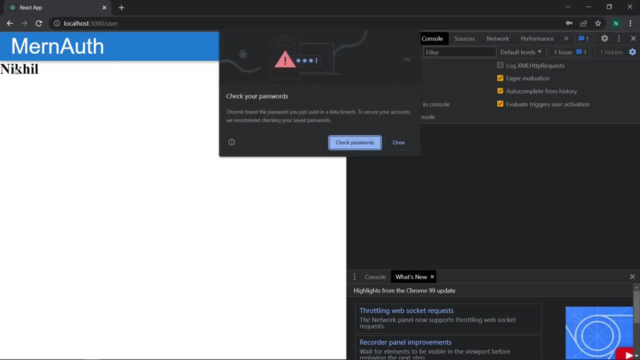 and i have already saved all of the things. once i will click on the login things, once i will click on the login things, once i will click on the login. so now you will see, now we have the name. so now you will see, now we have the name. 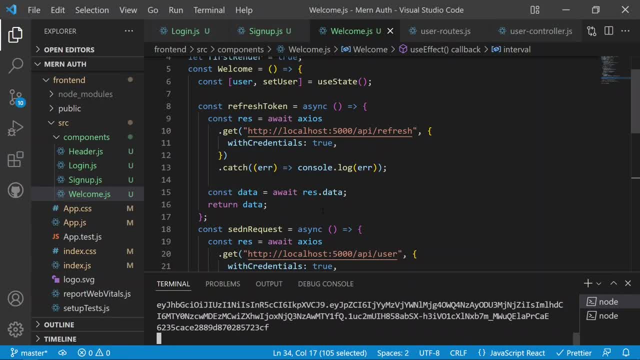 so now you will see, now we have the name nickel, so now we can just check after nickel. so now we can just check after nickel. so now we can just check after every. i think 28 seconds if everything is, every. i think 28 seconds if everything is. 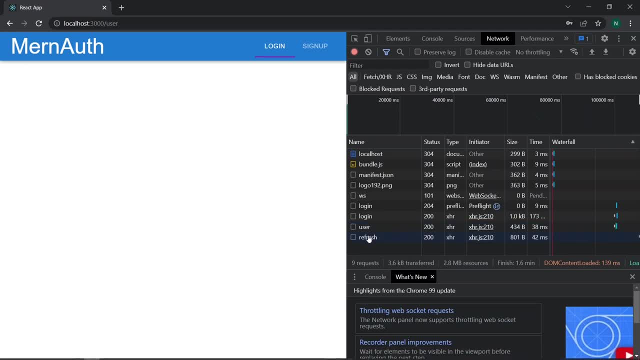 every, i think, 28 seconds, if everything is working fine, working fine, working fine. and now you will see the refresh is, and now you will see the refresh is. and now you will see the refresh is getting again, and now you will see the getting again, and now you will see the. 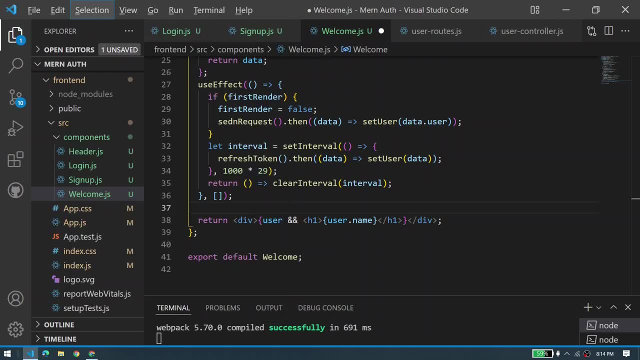 getting again. and now you will see, the refresh is working, refresh is working, refresh is working, and now we are getting the user, and now, and now we are getting the user, and now and now we are getting the user, and now the refresh is also working. fine, and now, the refresh is also working fine. and now the refresh is also working fine. and now we need to fix one thing. so now we need to fix one thing. so now we need to fix one thing. so now, when we are getting the user from the, when we are getting the user from the, 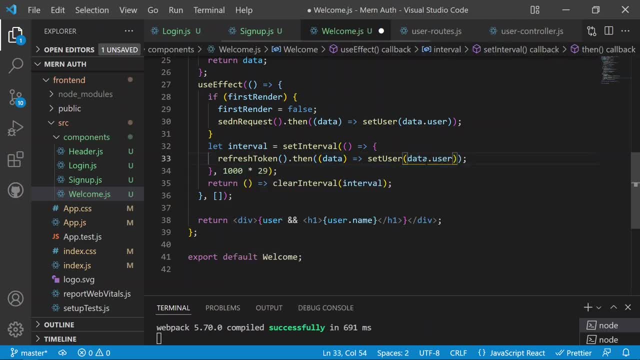 when we are getting the user from the set user. so we need to add the data dot set user. so we need to add the data dot set user. so we need to add the data dot user and not only the user, so it will be user and not only the user. so it will be. 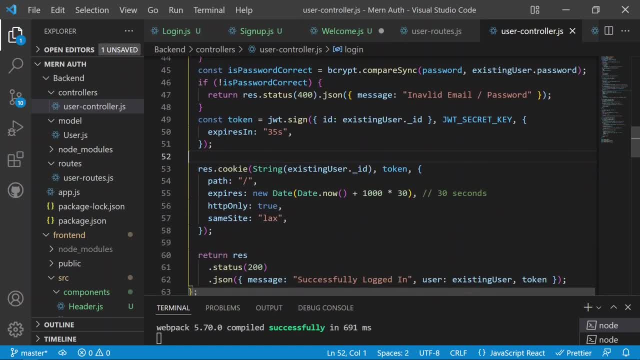 user and not only the user. so it will be here. so once the user will log in, then here. so once the user will log in, then here. so once the user will log in, then we need to add some conditions. so before we need to add some conditions, so before. 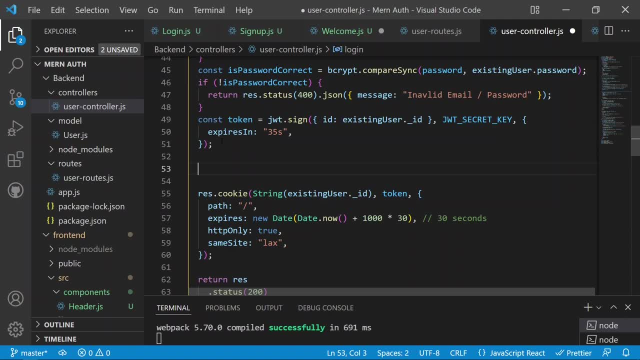 we need to add some conditions. so, before creating the cookie, we need to check. if creating the cookie, we need to check. if creating the cookie, we need to check if the cookie already exists, then we need the cookie already exists, then we need. the cookie already exists, then we need to remove that cookie and then we need to. 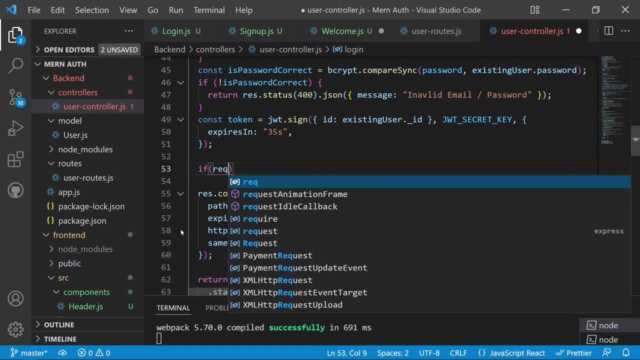 to remove that cookie, and then we need to to remove that cookie and then we need to generate the new cookie. so if we have generate the new cookie, so if we have generate the new cookie, so if we have the request, the request, the request dot cookies which we have the object, so 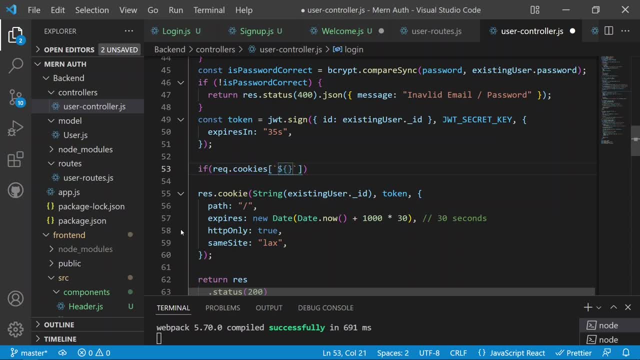 dot cookies, which we have the object. so dot cookies, which we have the object. so if the request dot cookies contains, if the request dot cookies contains, if the request dot cookies contains the cookie for the existing user dot id, the cookie for the existing user dot id, the cookie for the existing user dot id. dot id is there. underscore id is there. 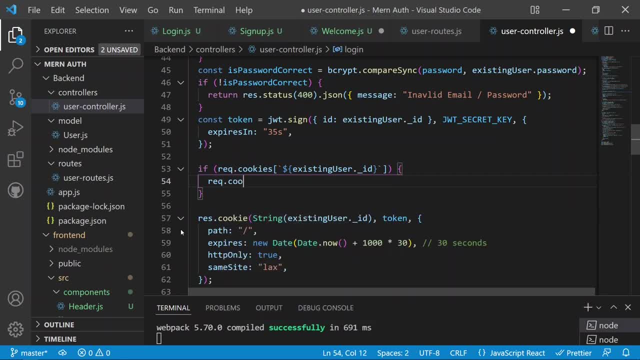 dot id is there? underscore id is there. dot id is there. underscore id is there, which is the mongodb, and then we need to which is the mongodb, and then we need to which is the mongodb, and then we need to add the request dot cookies. add the request dot cookies. 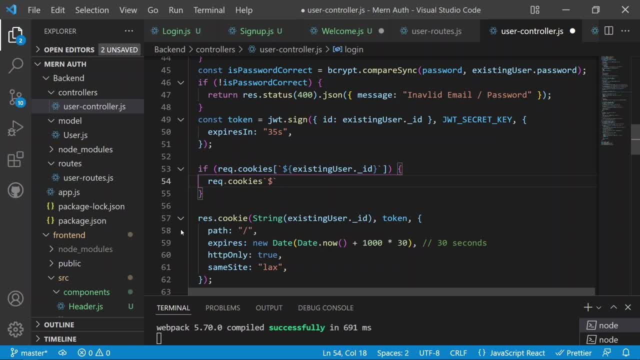 add the request dot cookies of that user, of that user, of that user again. we need to write this thing as this again. we need to write this thing as this again. we need to write this thing as this: i think we need to add here into the. i think we need to add here into the. 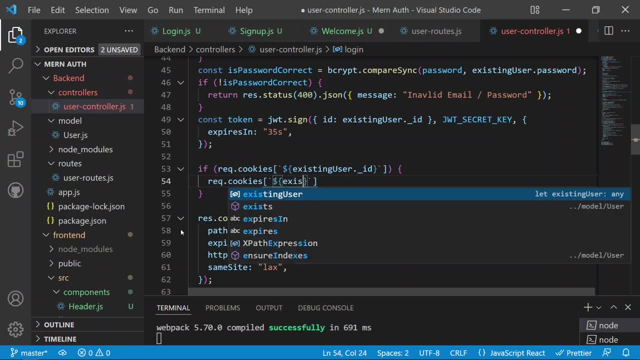 i think we need to add here into the brackets and then we need to add then brackets, and then we need to add then brackets and then we need to add then the existing user dot underscore id. will the existing user dot underscore id, will the existing user dot underscore id will be equals to the empty string. so we 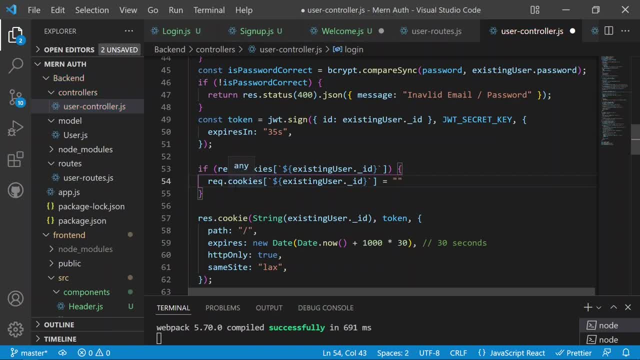 be equals to the empty string. so we be equals to the empty string. so we will just add the empty string after will just add the empty string after will just add the empty string after that cookie. so it means that if we will that cookie, so it means that if we will. 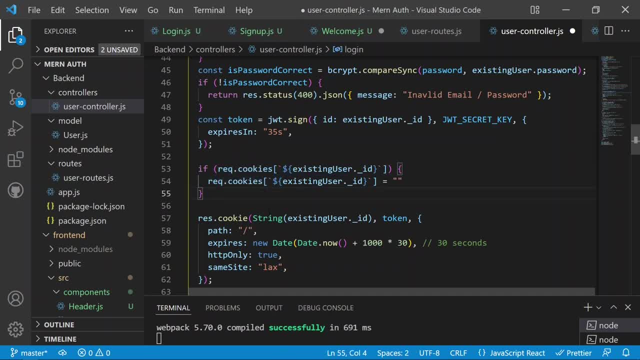 that cookie. so it means that if we will get the cookie from there, so it will be get the cookie from there, so it will be get the cookie from there, so it will be the empty string, and then we will just the empty string, and then we will just. 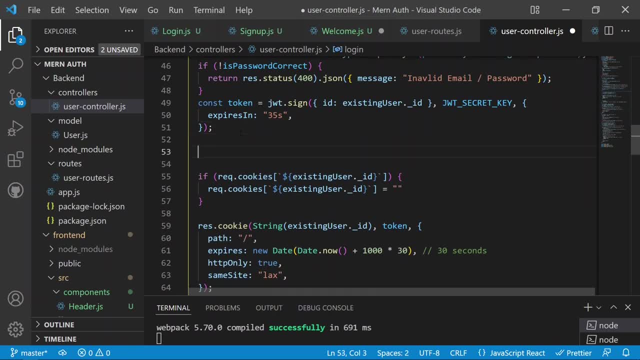 the empty string and then we will just regenerate the cookie. so after the token, regenerate the cookie. so after the token, regenerate the cookie. so after the token is regenerated, then we can add: one more is regenerated, then we can add: one more is regenerated, then we can add one more log here to check if everything is. 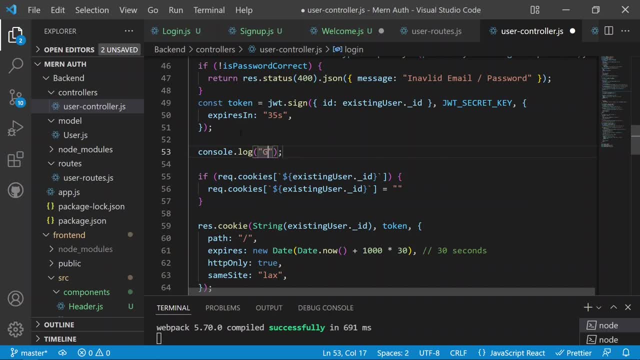 log here to check if everything is. log here to check if everything is working fine again. we will check again. working fine again, we will check again. working fine again, we will check again. so it is like the generated. so it is like the generated, so it is like the generated token. 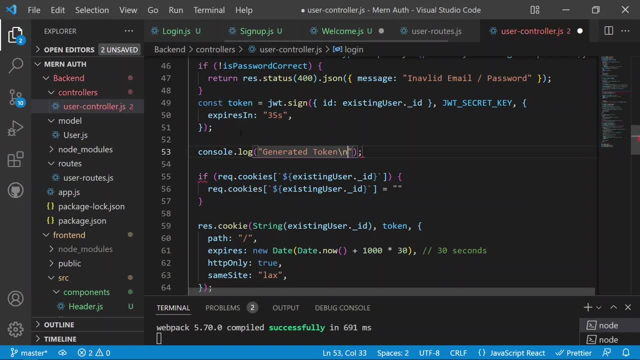 and it will enter a new line, and then we can add some token after, and then we can add some token after, and then we can add some token after there. so it will be the token which we there, so it will be the token which we there, so it will be the token which we have recently generated, and then in the 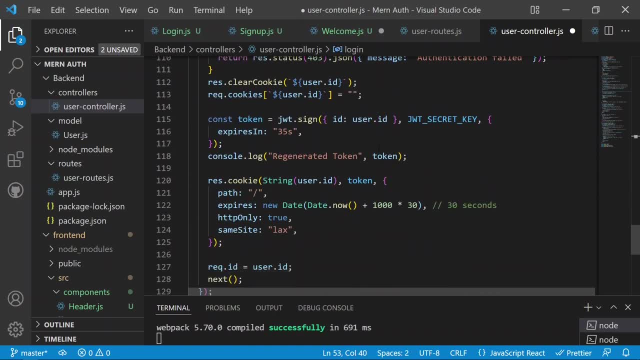 have recently generated and then in the have recently generated, and then in the refresh token. so we need to go to the refresh token, so we need to go to the refresh token, so we need to go to the refresh token again, and then after the refresh token again, and then after the. 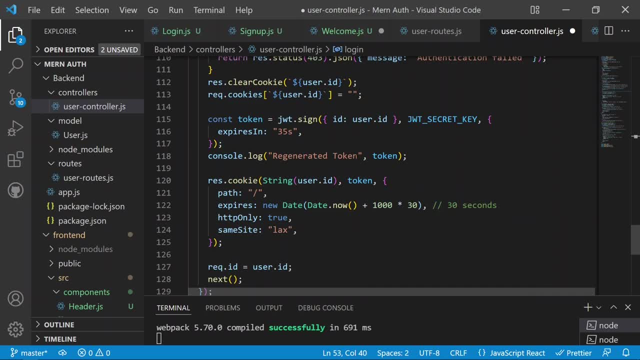 refresh token again and then after the token is generated, and then we will add: token is generated and then we will add: token is generated and then we will add a regenerated token here again, and then a regenerated token here again, and then a regenerated token here again, and then i will add a slash n over there to add: 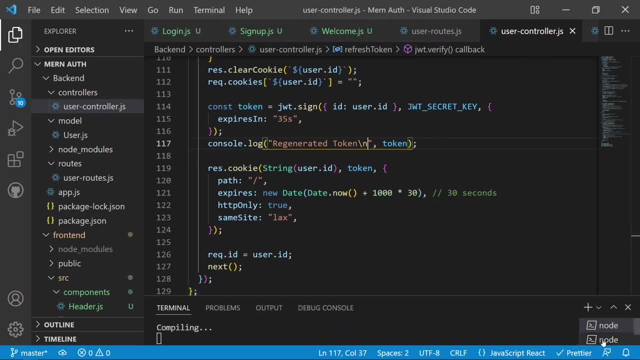 i will add a slash n over there to add. i will add a slash n over there to add it into the new line. so now, if i will it into the new line, so now, if i will it into the new line, so now, if i will now save and if i will now just go to 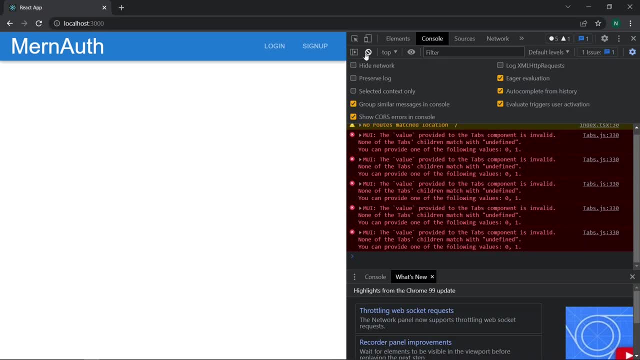 now save, and if i will now just go to now save and if i will now just go to the node and we need to just run the the node and we need to just run the the node and we need to just run the application again, i will now remove. 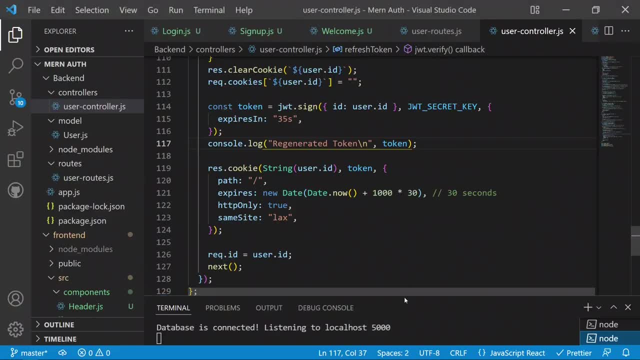 application again. i will now remove application again. i will now remove everything from there. everything from there, everything from there. and now we need to check the locks, so, and now we need to check the locks, so, and now we need to check the locks, so we need to just expand it. now we can. we need to just expand it now we can. we need to just expand it now. we can see now. once the user will log in like: see now. once the user will log in like: see now. once the user will log in like: one, two, three, four, five at the latest. 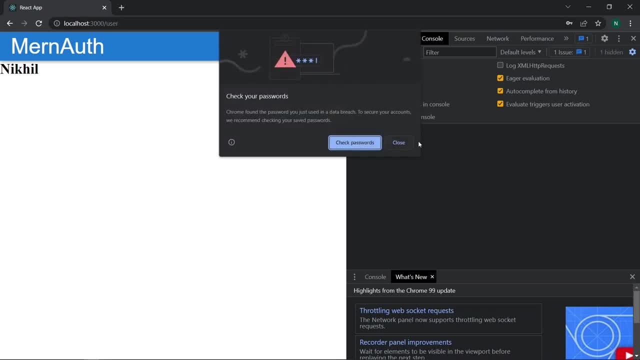 one, two, three, four, five at the latest. one, two, three, four, five at the latest dot com. once i will click on the login dot com, once i will click on the login dot com, once i will click on the login. now we can see. now we have the nickel. 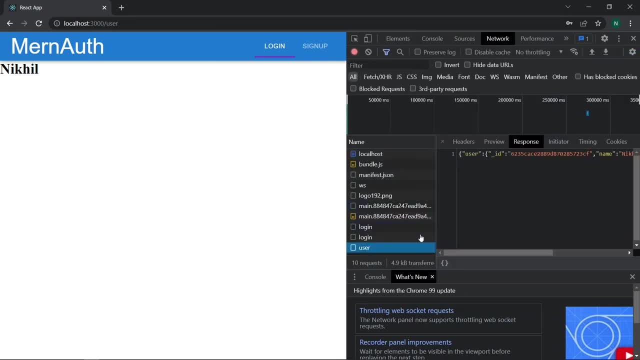 now we can see. now we have the nickel. now we can see. now we have the nickel onto the window and in the network, we onto the window and in the network, we onto the window and in the network. we can see everything is working fine for. can see everything is working fine for. 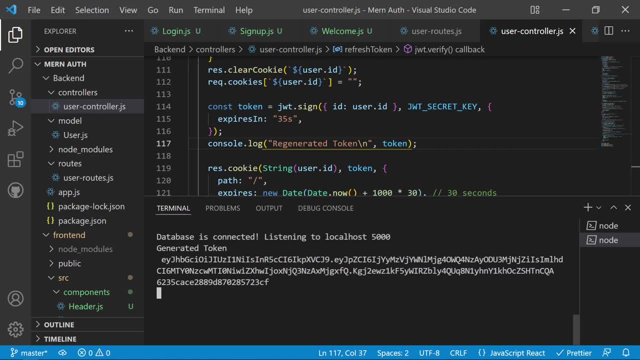 can see everything is working fine for the user, and now the response is okay, the user. and now the response is okay, the user. and now the response is okay. and then now we can see we have a. and then now we can see we have a. and then now we can see we have a generated token, and this is a token. 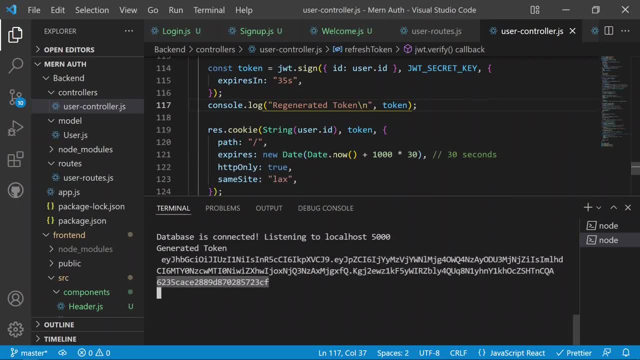 generated token and this is a token generated token and this is a token. it is highlighted and this is the id i. it is highlighted and this is the id i. it is highlighted and this is the id i think. we are also logging the id of the think. we are also logging the id of the. 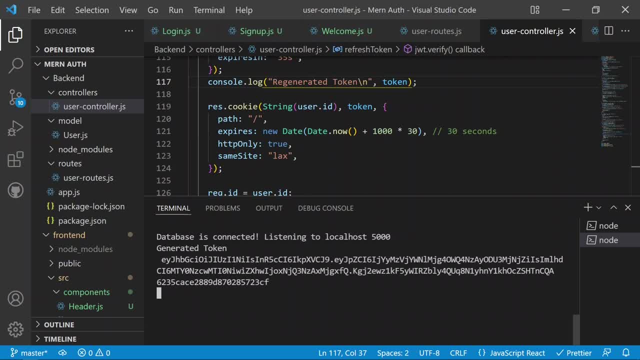 think we are also logging the id of the user. but now we have to check if user. but now we have to check if user. but now we have to check if everything is working fine and and if everything is working fine and and if everything is working fine and and if the regenerative token and the 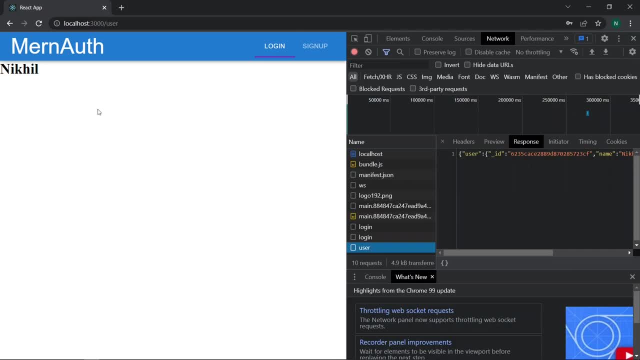 the regenerative token and the. the regenerative token and the generative token is different or not, generative token is different or not, generative token is different or not, and if the user is currently again. and if the user is currently again and if the user is currently again logged in or not. so we need to check. 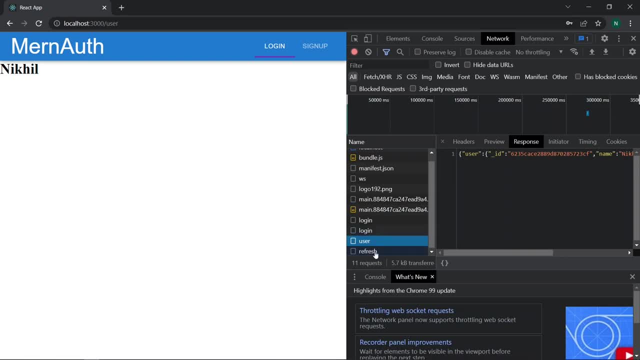 logged in or not. so we need to check logged in or not. so we need to check the refreshed out into there. so we so the refreshed out into there, so we so the refreshed out into there, so we. so now we can see we have a refresh out. 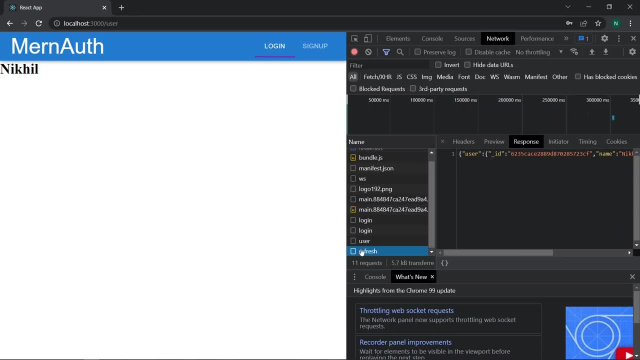 now we can see we have a refresh out. now we can see we have a refresh out over there and it contains a user which over there, and it contains a user which over there, and it contains a user which is the object of the id. so now the 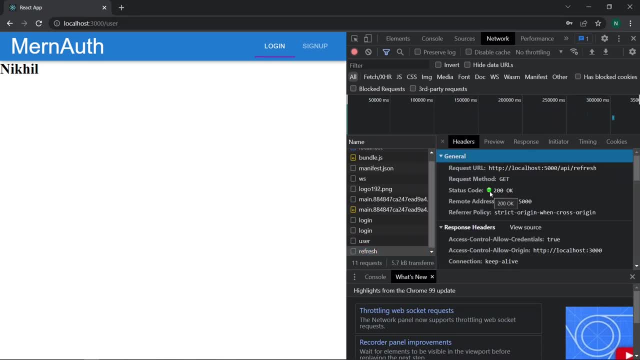 is the object of the id, so now the is the object of the id. so now the response is successful. we can see the response is successful. we can see the response is successful. we can see the header: the get equals to 200, okay, and it. header: the get equals to 200, okay, and it. 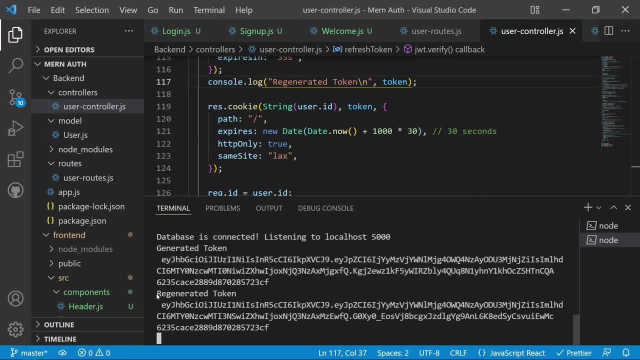 header the get equals to 200, okay, and it is a green light. and then now we can see is a green light. and then now we can see is a green light. and then now we can see in the logs also now the regenerative in the logs also now the regenerative. 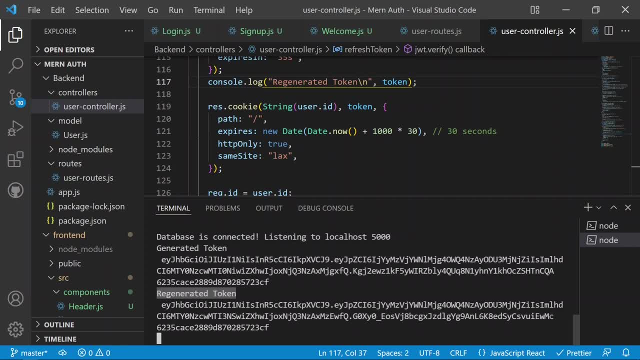 in the logs also. now the regenerative token is different from there and in the token is different from there and in the token is different from there and in the end it contains a cqa and it contains a end. it contains a cqa and it contains a. 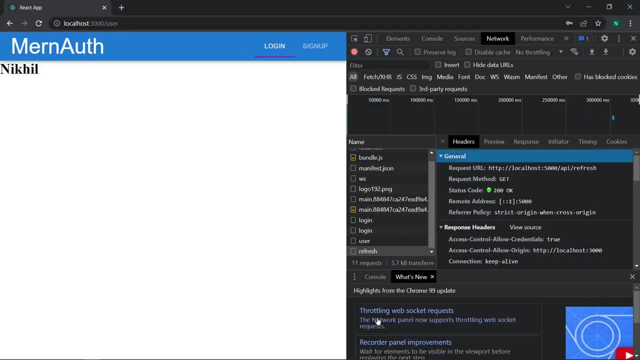 end. it contains a cqa and it contains a w and mc. so now everything is working w and mc. so now everything is working w and mc. so now everything is working perfectly fine. so now we can check in perfectly fine. so now we can check in perfectly fine. so now we can check in different browsers as well. so i will. 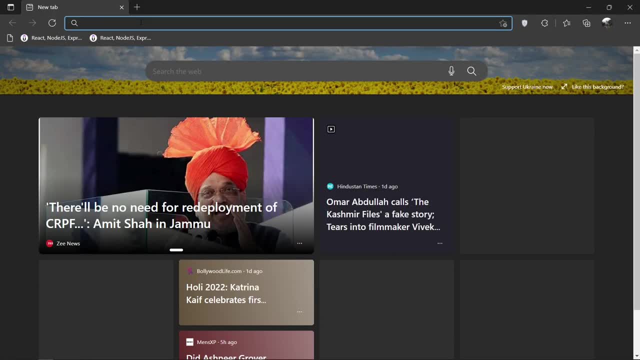 different browsers as well, so i will different browsers as well. so i will open a h browser here, so i will open. open a h browser here, so i will open. open a h browser here, so i will open that browser and i will now just send a that browser and i will now just send a. 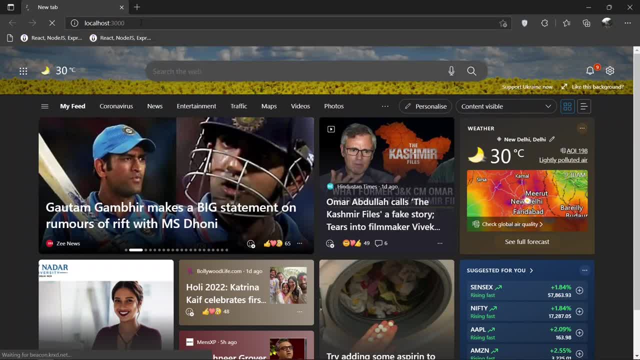 that browser and i will now just send a request from that browser. so it will. the request from that browser. so it will the request from that browser. so it will the localhost 3000. so i have now opened. localhost 3000. so i have now opened. 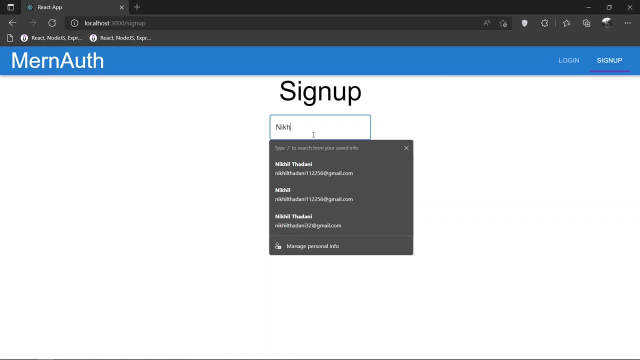 localhost 3000. so i have now opened that, and now i will click on the signup that, and now i will click on the signup that, and now i will click on the signup. select a new user as the nickel again. select a new user as the nickel again. 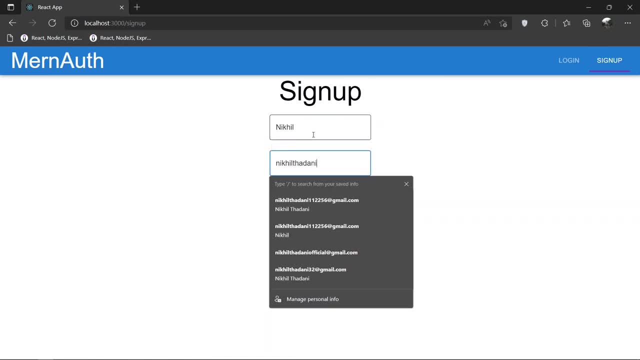 select a new user as the nickel again, the email will be nickel. the email will be nickel. the email will be nickel th a d a n i at the rate th a d a n i at the rate th a d a n i at the rate. gmailcom. 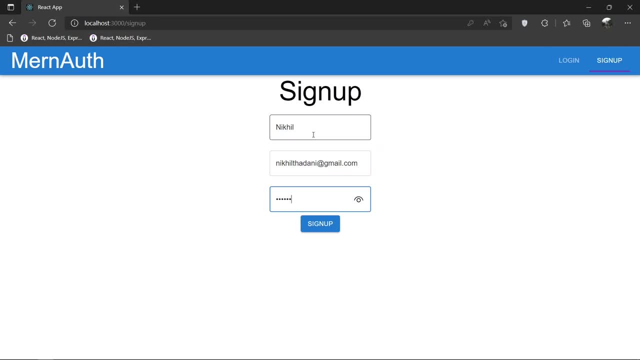 gmailcom- gmailcom. so i have at the email the password will. so i have at the email the password will. so i have at the email. the password will be same: one, one, one, one, one one. i will be same: one, one, one, one, one, one, i will. 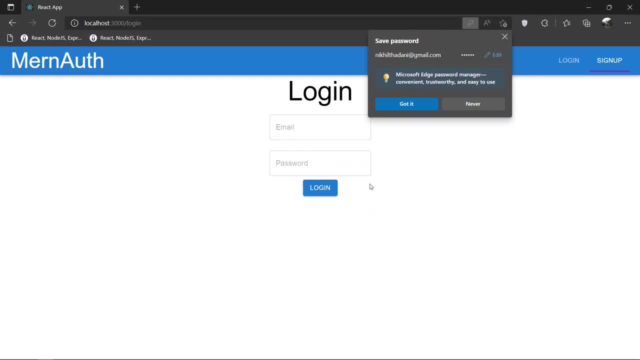 be same one, one, one, one, one one. i will click on the sign up. click on the sign up, click on the sign up. so now we can see everything is okay. and so now we can see everything is okay. and so now we can see everything is okay. and now we are redirected to login, so i will 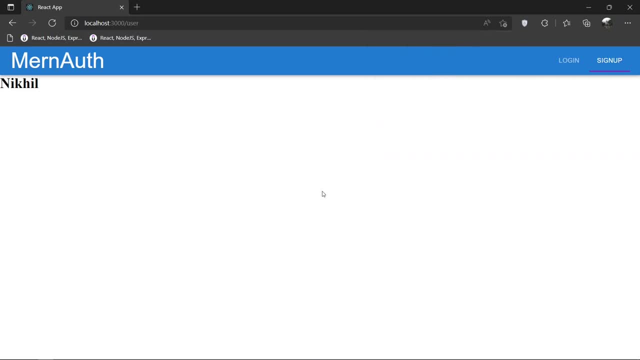 now we are redirected to login, so i will. now we are redirected to login, so i will now add the credentials here and i will now add the credentials here, and i will now add the credentials here and i will now click on the login again. now we can. 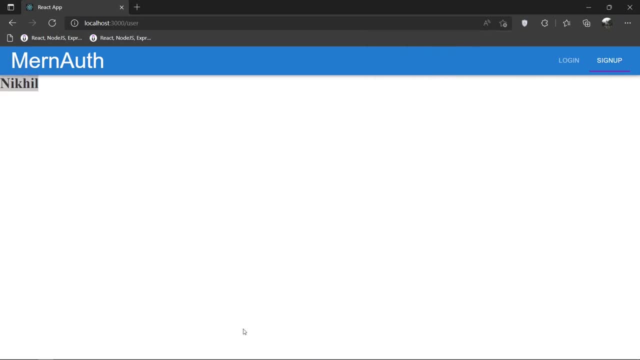 now click on the login again. now we can now click on the login again. now we can see: now we have the user and now if i see now we have the user and now if i see now we have the user and now if i will now just click on the inspect here. 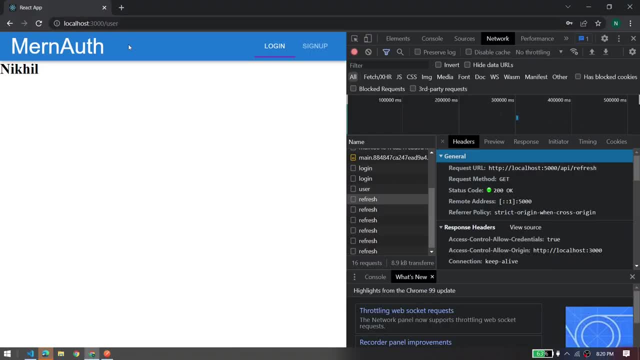 will now just click on the inspect here. will now just click on the inspect here again. so now everything is working fine again. so now everything is working fine again. so now everything is working fine, even in the chrome browser, even in the, even in the chrome browser, even in the. 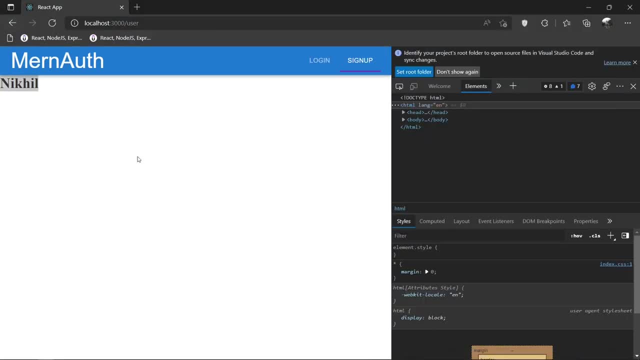 even in the chrome browser, even in the different user: it is working fine. and different user: it is working fine. and different user: it is working fine. and even in the edge browser it is working. even in the edge browser it is working. even in the edge browser it is working totally fine. so everything is working. 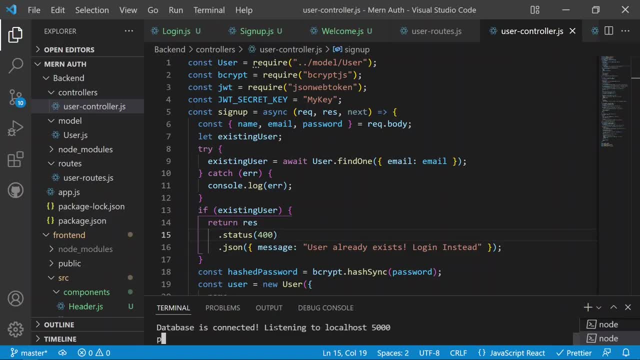 totally fine. so everything is working. totally fine, so everything is working fine. so now this is our application, fine. so now this is our application, fine. so now this is our application, which we have built, and now the which we have built, and now the which we have built, and now the application is fully complete, but one. 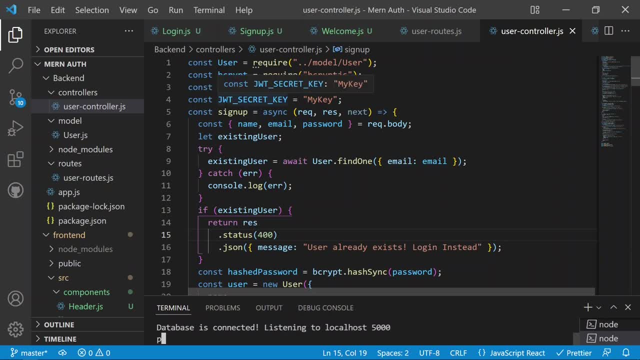 application is fully complete. but one application is fully complete, but one thing is remaining. so we are storing. thing is remaining, so we are storing. thing is remaining. so we are storing the jwt key as a constant, but it should. the jwt key as a constant, but it should. 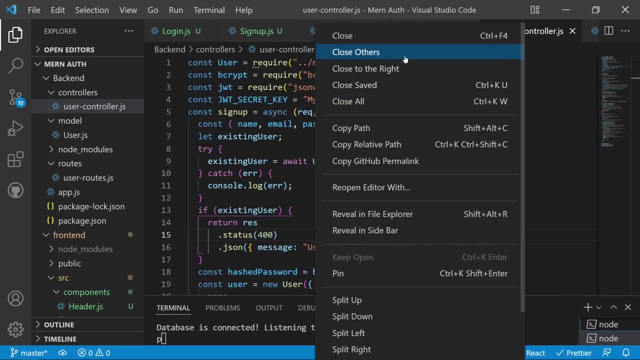 the jwt key as a constant, but it should not be stored as a constant in any ways, not be stored as a constant in any ways, not be stored as a constant in any ways. so we should now remove that and now for. so we should now remove that and now for. 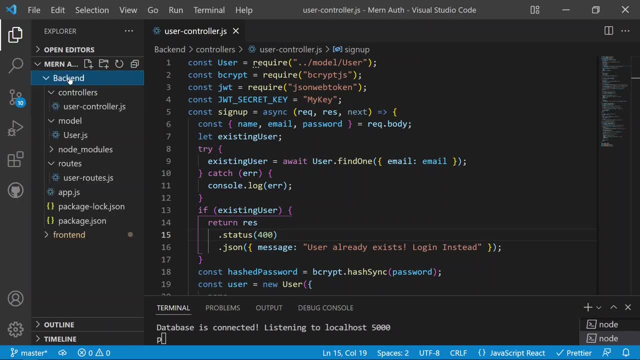 so we should now remove that and now for that we can install a new package as a that we can install a new package as a that we can install a new package as a dot env which will just store the dot env, which will just store the dot env, which will just store the jwt key in the env file and the mongodb. 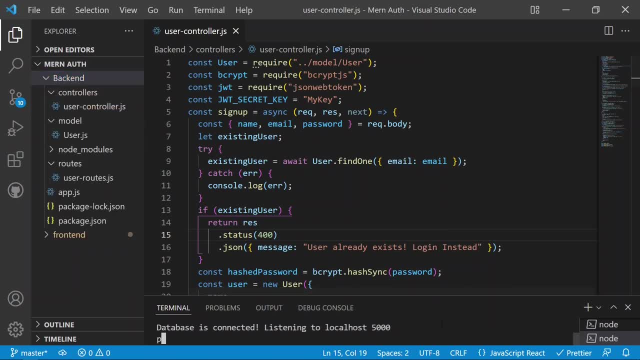 jwt key in the env file and the mongodb jwt key in the env file and the mongodb password also in the env file. so we can password also in the env file. so we can password also in the env file. so we can now just create and we can now just stop. 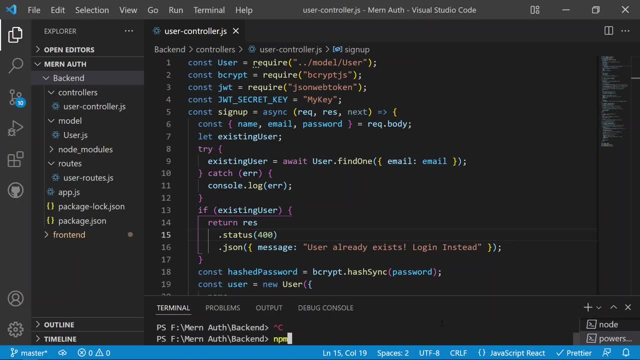 now just create and we can now just stop. now just create and we can now just stop the server. and we need to install the, the server. and we need to install the, the server. and we need to install the dot, env, dot, env, dot, env. go through the npm installed at the dot. 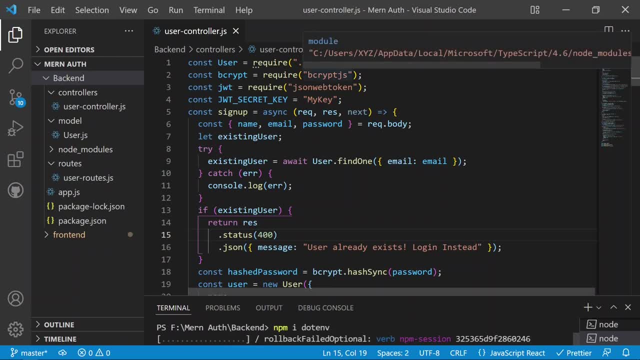 go through the npm installed at the dot. go through the npm installed at the dot env to add all of the things in the env env. to add all of the things in the env env. to add all of the things in the env. and then we need to configure that also. 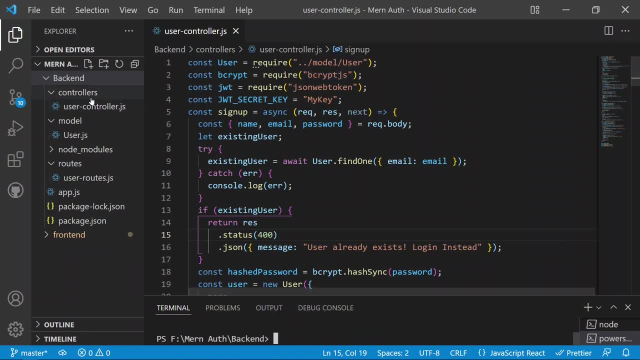 and then we need to configure that also, and then we need to configure that also. so after the env is installed, and now we so. after the env is installed, and now we so after the env is installed, and now we need to move on to the appjs from there. 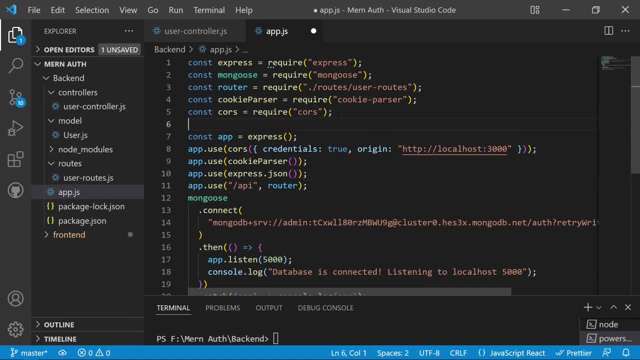 need to move on to the appjs from there, need to move on to the appjs from there, and then we need to just use that, so it, and then we need to just use that, so it, and then we need to just use that, so it will be the require. 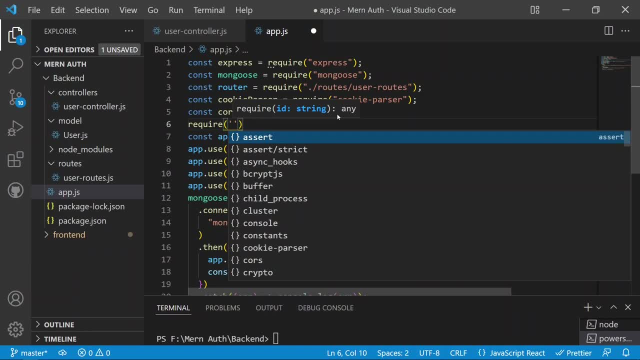 will be the require will be the require, so it will be directly. we are requiring, so it will be directly. we are requiring, so it will be directly. we are requiring. and now we are now configuring directly, and now we are now configuring directly, and now we are now configuring directly, so it will be the dot env which we have. 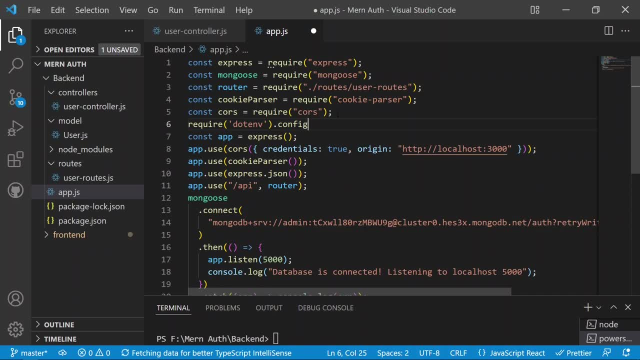 so it will be the dot env which we have. so it will be the dot env which we have currently installed. it has a method of currently installed. it has a method of currently installed. it has a method of the config, so the config will be there. the config, so the config will be there. 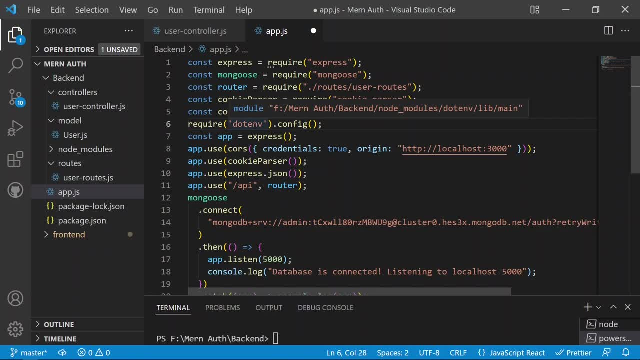 the config. so the config will be there and now we will call the config. so after: and now we will call the config. so after: and now we will call the config, so after that the env files will be working and that the env files will be working. and. 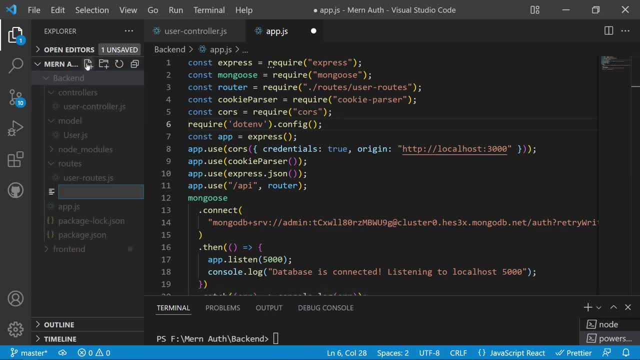 that the env files will be working and in the backend, in the main root file. so in the backend, in the main root file, so in the backend in the main root file, so we can generate a new file. we can generate a new file, we can generate a new file. i think we have to generate a new file. 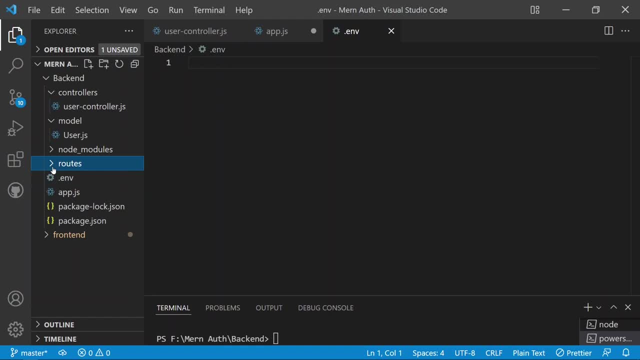 i think we have to generate a new file. i think we have to generate a new file as a dot env. so now we have generated a as a dot env. so now we have generated a as a dot env. so now we have generated a new file, new file. 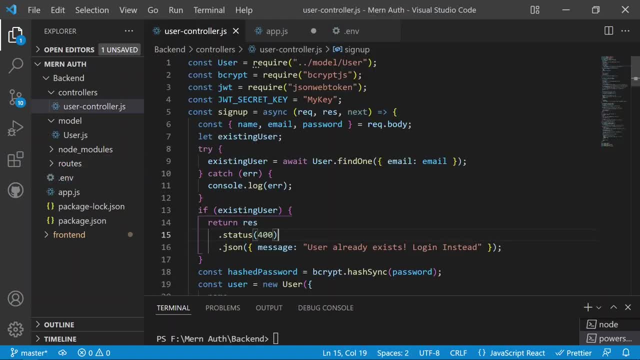 new file. so we can just go to the env and we can. so we can just go to the env and we can. so we can just go to the env and we can just set the token, just set the token, just set the token to there. so then i will now just copy the. 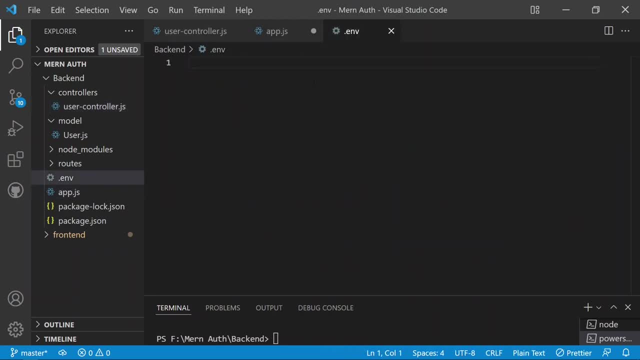 to there. so then i will now just copy the to there. so then i will now just copy the token from there and i will now just token from there, and i will now just token from there and i will now just paste the token to in the env file. 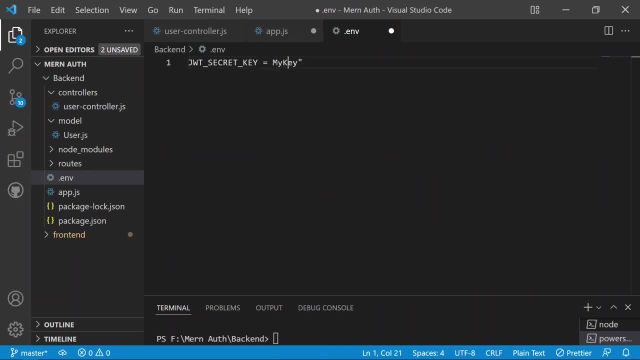 paste the token to in the env file. paste the token to in the env file, so it will be the jwt secret key. equals. so it will be the jwt secret key. equals. so it will be the jwt secret key. equals to the my key and you can define any. 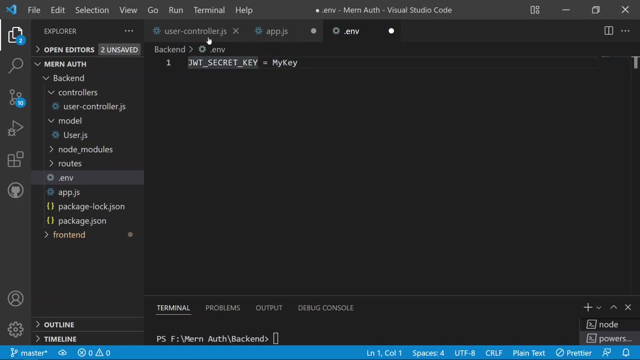 to the my key and you can define any to the my key, and you can define any other key as well. so now i have defined other key as well. so now i have defined other key as well. so now i have defined that, and now you can just go to the user. 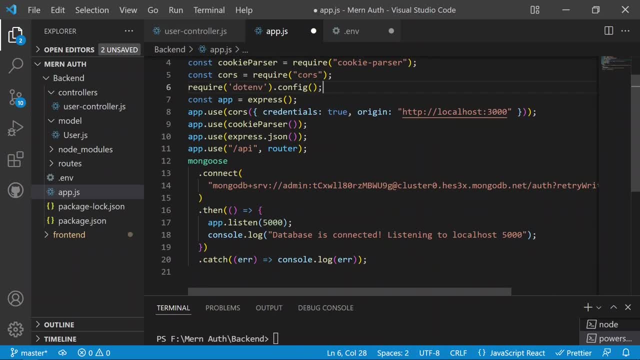 that, and now you can just go to the user that, and now you can just go to the user- i think appjs- and then you can also- i think appjs, and then you can also- i think appjs, and then you can also store the password of the mongodb there. 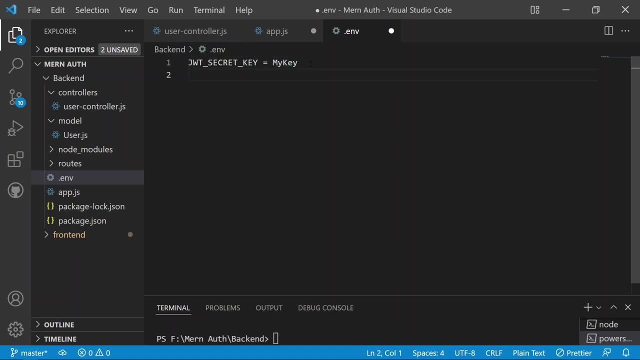 store the password of the mongodb there. store the password of the mongodb there as the password as it, and it will be as the password as it, and it will be as the password as it, and it will be equals to the password, like into the, equals to the password, like into the. 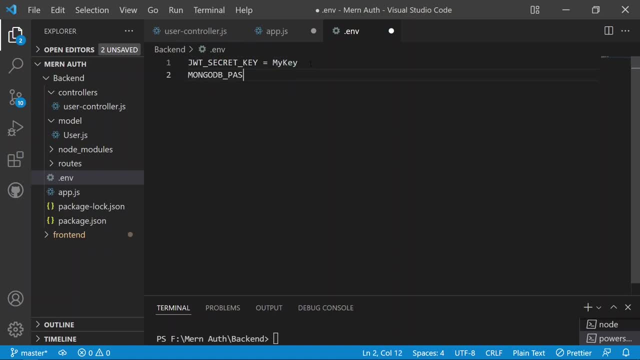 equals to the password, like into the password or mongodb password or mongodb password or mongodb password, will be equals to the password, will be equals to the password, will be equals to the equals to the password which you have just equals to the password which you have just equals to the password which you have just copied. so you can do that and then in. 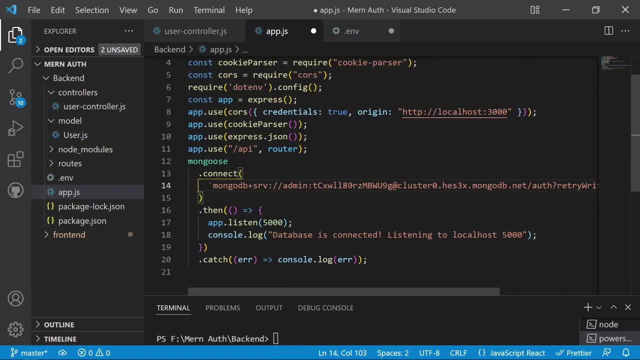 copied, so you can do that, and then in copied, so you can do that, and then in the appjs instead of this. so you can the appjs instead of this. so you can the appjs instead of this. so you can just use here the template details and. 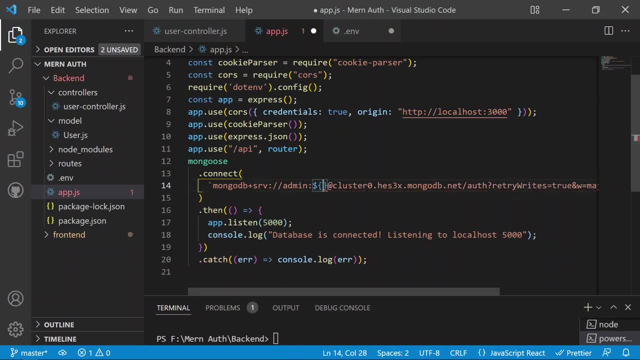 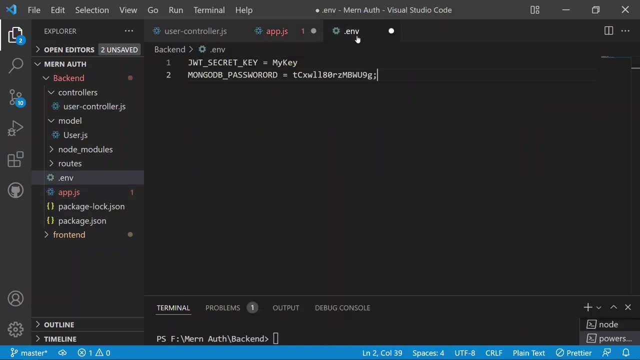 just use here the template details and just use here the template details and then you can just remove that add here. then you can just remove that add here. then you can just remove that add here. the like, the process, dot, env, dot, env, dot, env, dot. the name, like we have now defined, the. 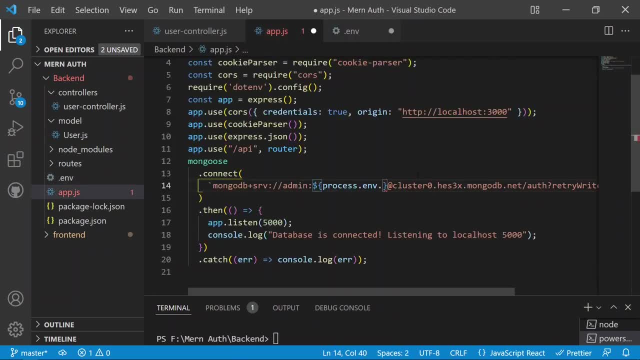 dot the name, like we have now defined the dot. env. dot the name, like we have now defined the env name as the mongodb password. so you env name as the mongodb password. so you env name as the mongodb password, so you can just use that. can just use that. 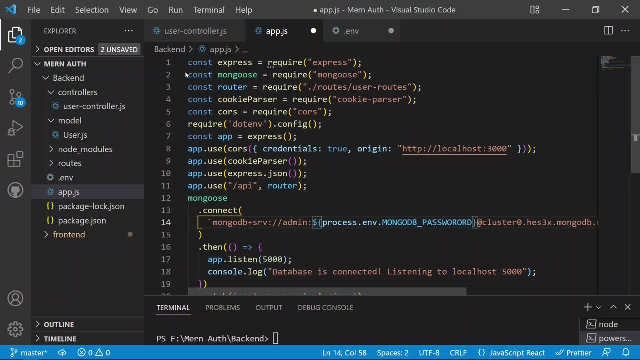 can just use that mongodb password and then after that you mongodb password, and then after that you mongodb password and then after that you can use here the dot env in the user's, can use here the dot env in the user's, can use here the dot env in the user's controller in the secret key as well. so 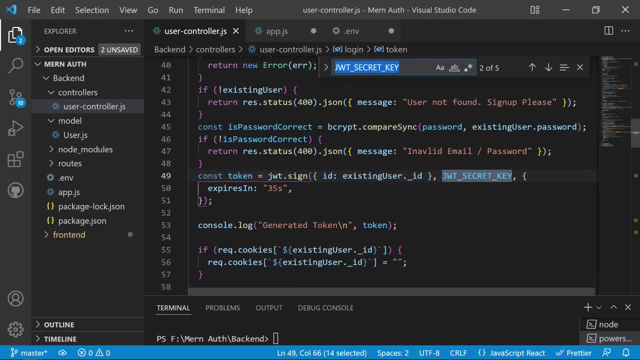 controller in the secret key as well, so controller in the secret key as well. so whenever we are using the secret key, so whenever we are using the secret key, so whenever we are using the secret key, so we can go to secret key here. so here we. we can go to secret key here, so here we. 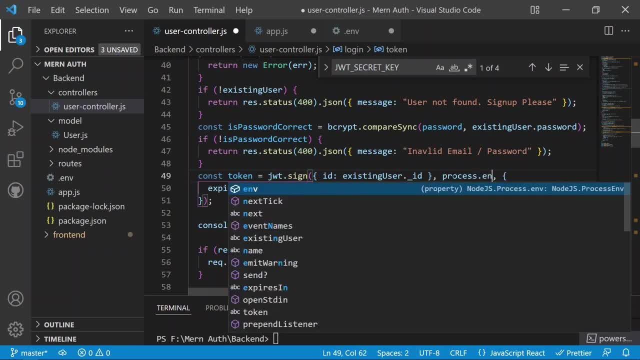 we can go to secret key here. so here we can use the process, can use the process, can use the process dot env dot. we have the variable dot env dot. we have the variable dot env dot. we have the variable as the. i think we have the jwt secret. 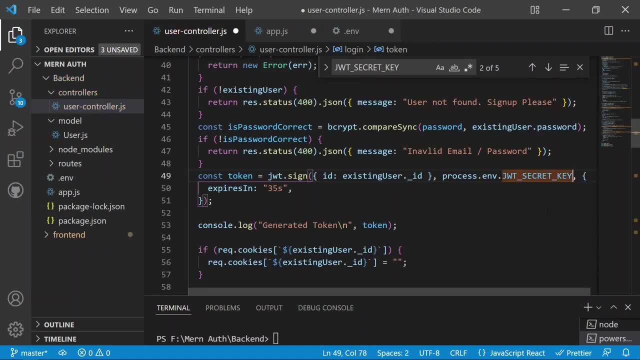 as the. i think we have the jwt secret as the. i think we have the jwt secret key, so we can just copy that we can just key. so we can just copy that we can just key. so we can just copy that we can just paste there at the secret key. so now we 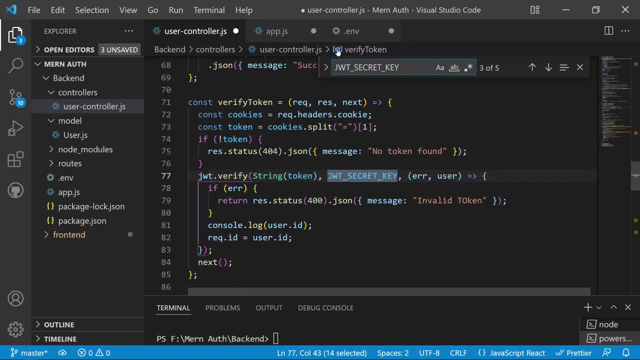 paste there at the secret key. so now we paste there at the secret key. so now we have used that and here also in the have used that, and here also in the have used that and here also in the verify token, so we can use that as the. 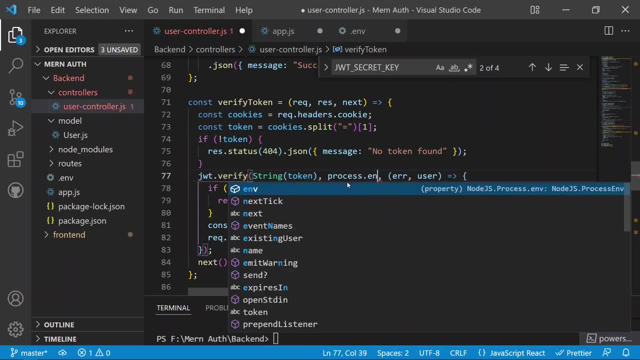 verify token. so we can use that as the verify token. so we can use that as the process process. process dot env dot the jwt secret key. so we dot env dot the jwt secret key. so we dot env dot the jwt secret key. so we can use that. 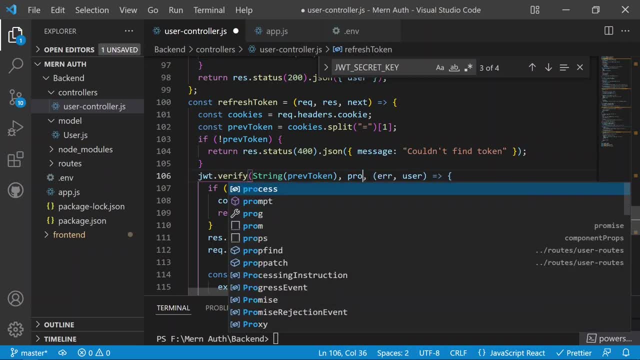 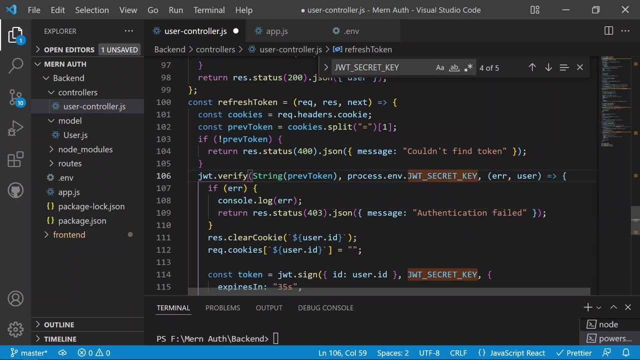 can use that, can use that, and here also we need to add that as the, and here also we need to add that as the, and here also we need to add that as the process, process, process, dot, env, dot, jwt, secret key, and here also we need to do that. 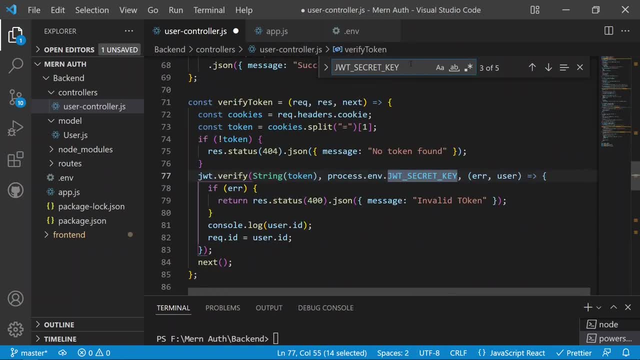 and here also we need to do that. and here also we need to do that. it will be the process: dot env, dot jwt. it will be the process: dot env, dot jwt. it will be the process: dot env, dot jwt. secret key, so now. secret key, so now. 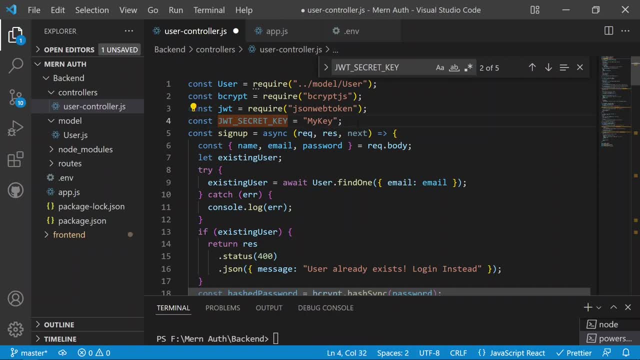 secret key. so now everything is working totally fine, and everything is working totally fine, and everything is working totally fine, and then we can remove that jwt secret key. then we can remove that jwt secret key from there also. so i will now remove from there also. so i will now remove. 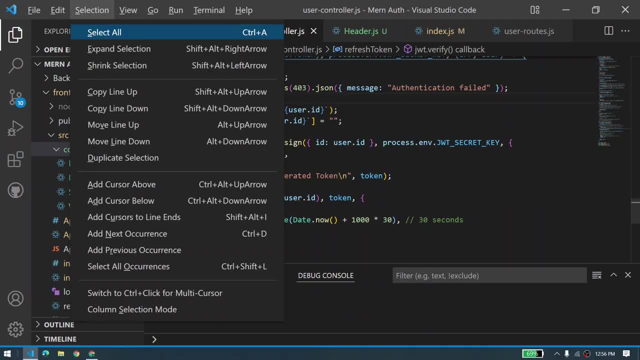 from there also. so i will now remove there and everything will work same as there, and everything will work same as there and everything will work same as before and now the application is almost before and now the application is almost before and now the application is almost complete, and the only thing which is 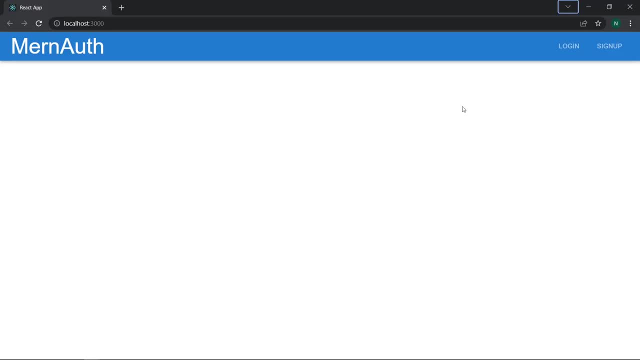 complete, and the only thing which is complete and the only thing which is remaining now is the logout. so we need remaining now is the logout. so we need remaining now is the logout. so we need to build the logout functionality as to build the logout functionality, as to build the logout functionality as well. so once the user will log in, then 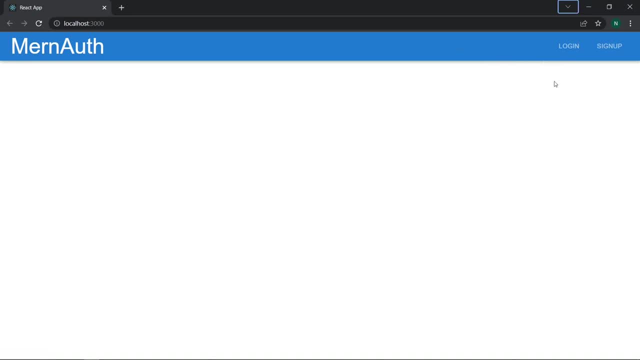 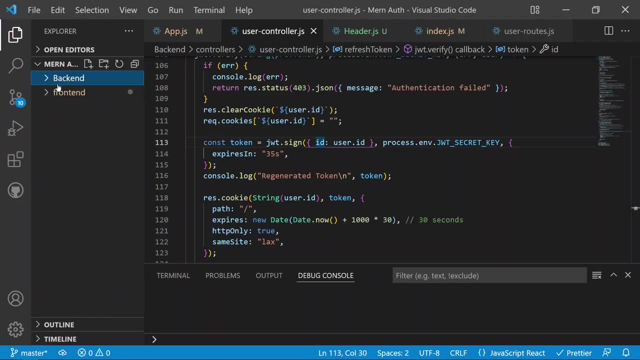 well, so once the user will log in, then. well, so once the user will log in, then we need to show logout, and once the we need to show logout, and once the we need to show logout, and once the cookies of the user and in the front end. 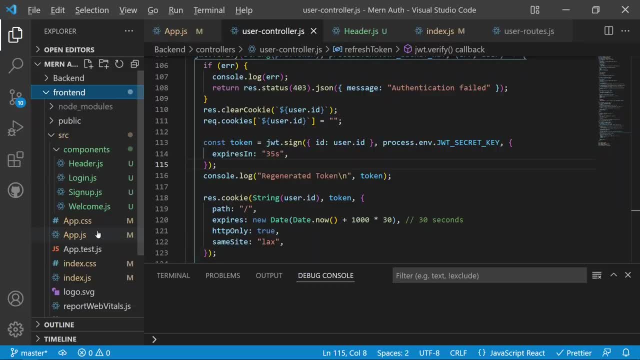 cookies of the user and in the front end, cookies of the user and in the front end, we can just create the functionality of. we can just create the functionality of. we can just create the functionality of the login, the login, the login. so when the state is the login, then we. 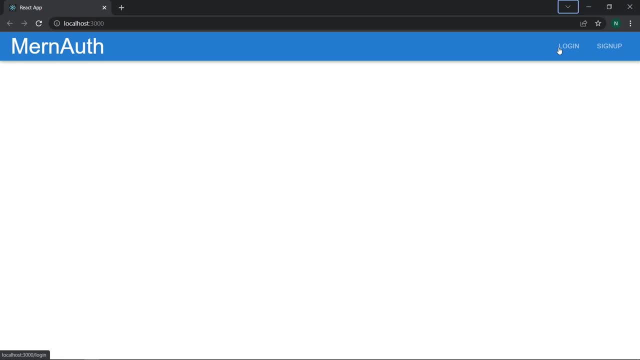 so when the state is the login, then we. so when the state is the login, then we need to show user the logout and when need to show user the logout and when need to show user the logout and when the state is the logout, then we need to. 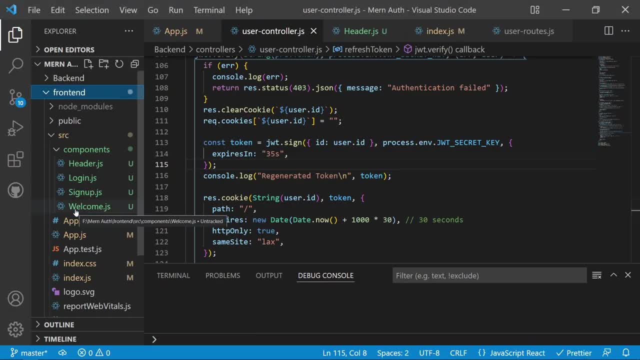 the state is the logout, then we need to. the state is the logout, then we need to log in and the sign up buttons log in and the sign up buttons log in and the sign up buttons. so for that in the front end we can use. so for that in the front end we can use. 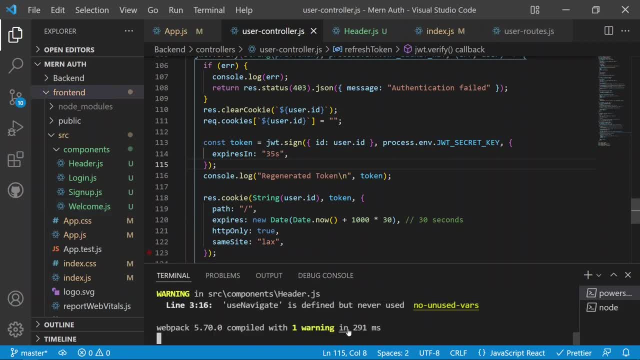 so for that, in the front end, we can use the redux which will help us to do that, the redux which will help us to do that, the redux which will help us to do that. so first we will move on to the front. so first we will move on to the front. 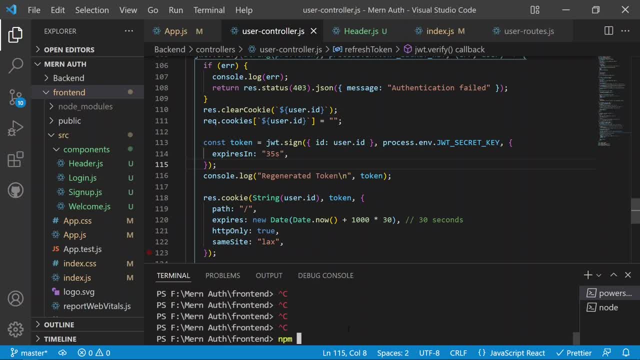 so first we will move on to the front end. first we will work on the front end end. first we will work on the front end end. first we will work on the front end. we will install the redux, so it will be. we will install the redux, so it will be. 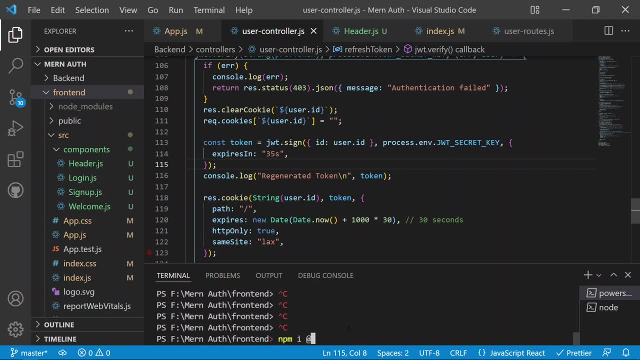 we will install the redux, so it will be the command of the npm install and we the command of the npm install and we the command of the npm install. and we need to install the redux js toolkit. need to install the redux js toolkit. need to install the redux js toolkit, which is a redux library to help us in. 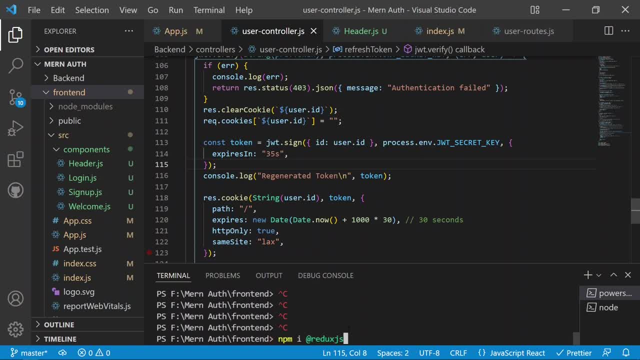 which is a redux library to help us in, which is a redux library to help us in the react applications. it will the redux the react applications. it will the redux the react applications. it will the redux js toolkit. and then after that we need to install, and then after that we need to install. 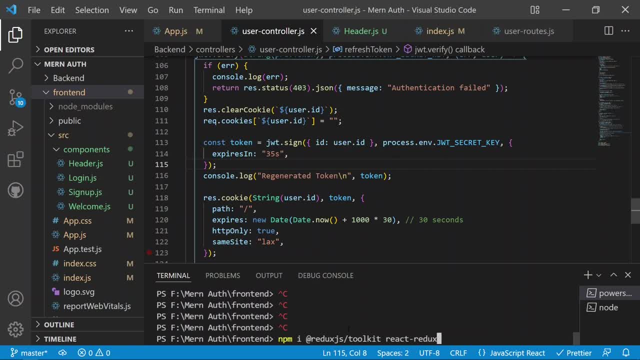 and then after that we need to install the react redux also, the react redux also, the react redux also. that will the react redux. so we need to, that will the react redux. so we need to. that will the react redux. so we need to install these two packages for the redux. 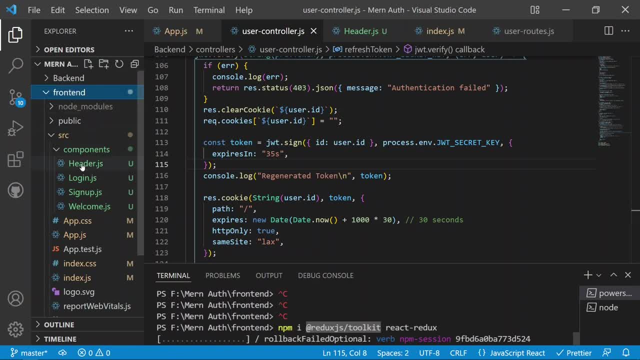 install these two packages for the redux, install these two packages for the redux, and then we need to work on the front, and then we need to work on the front and then we need to work on the front end first, so in the front end, in the end. first so in the front end, in the 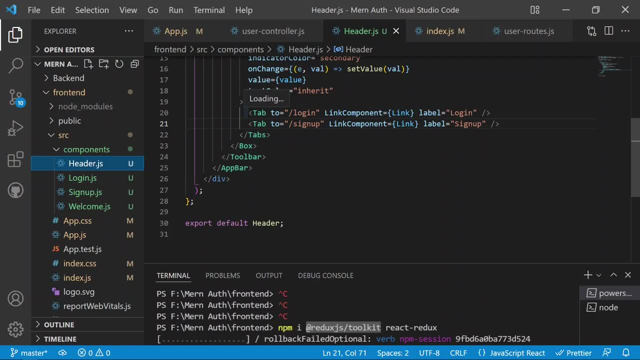 end first. so in the front end, in the header. now we have the two routes for header. now we have the two routes for header, now we have the two routes for the login and the sign up, and then we the login and the sign up, and then we 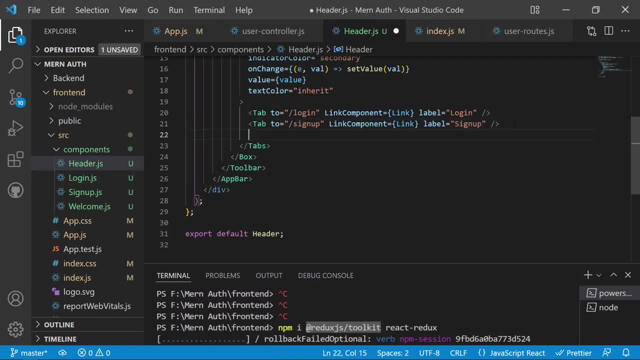 the login and the sign up, and then we can create one more tab for that, can create one more tab for that, can create one more tab for that for the logout, so we can just move on for the logout. so we can just move on for the logout, so we can just move on and we can just copy and paste a new. 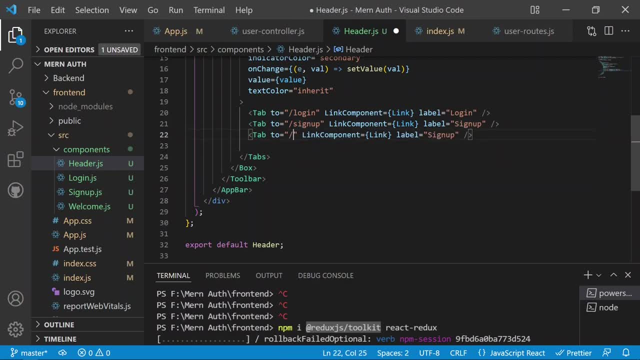 and we can just copy and paste a new. and we can just copy and paste a new tab, and the two will be considered tab and the two will be considered tab and the two will be considered default route and then the link. default route and then the link. 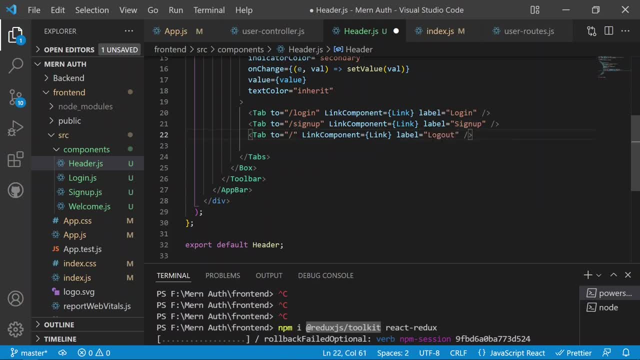 default route and then the link component would be same and the component would be same and the component would be same and the label will be the logout. now we have label will be the logout. now we have label will be the logout. now we have created the logout label also. so after: 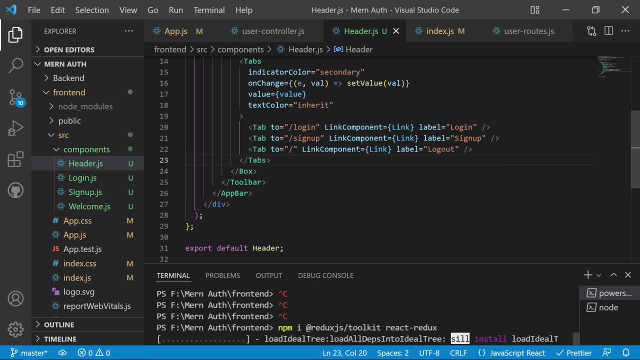 created the logout label also. so after created the logout label also. so after the logout route: now we need to wait the logout route now. we need to wait the logout route now. we need to wait till the redux installs and then we can. till the redux installs, and then we can. 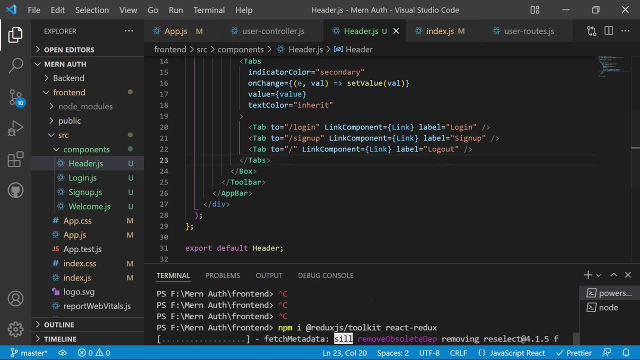 till the redux installs and then we can just create here the store functionality, just create here the store functionality, just create here the store functionality of the redux and the redux is used to of the redux and the redux is used to of the redux and the redux is used to create just a central data store which. 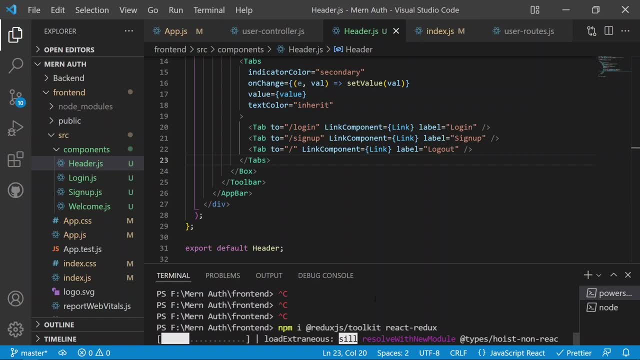 create just a central data store which create just a central data store which is only the one data store in the whole, is only the one data store in the whole, is only the one data store in the whole application. so it will handle the state application, so it will handle the state. 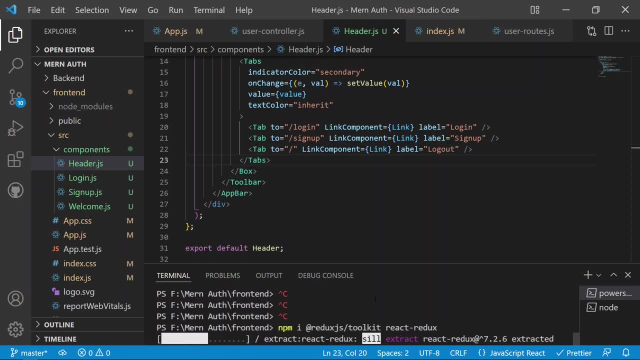 application so it will handle the state of the login and the logout and then we of the login and the logout, and then we of the login and the logout and then we show the user the changes according: to show the user the changes according: to show the user the changes according to the state: 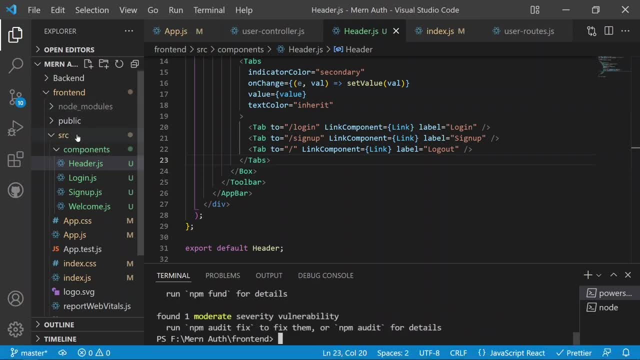 now, the redux is now installed. and now, now the redux is now installed. and now, now the redux is now installed, and now we can just move on to the source. we can just move on to the source. we can just move on to the source. we can just create a new folder as the. 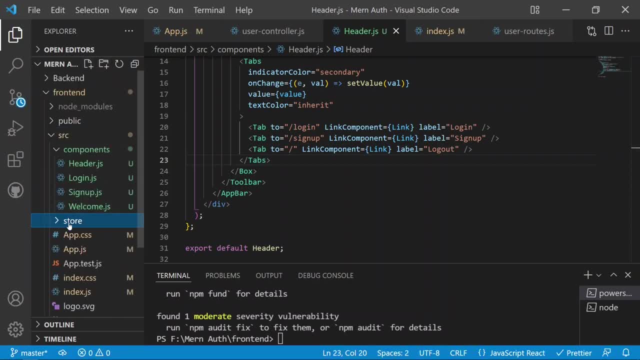 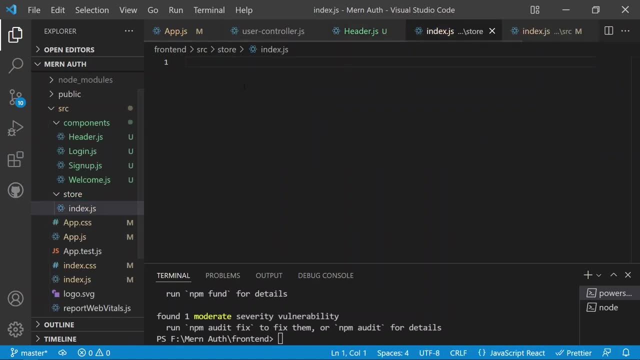 we can just create a new folder as the. we can just create a new folder as the store store. store the create slice and it will be imported from the redux and it will be imported from the redux. and it will be imported from the redux. gs toolkit- gs toolkit. 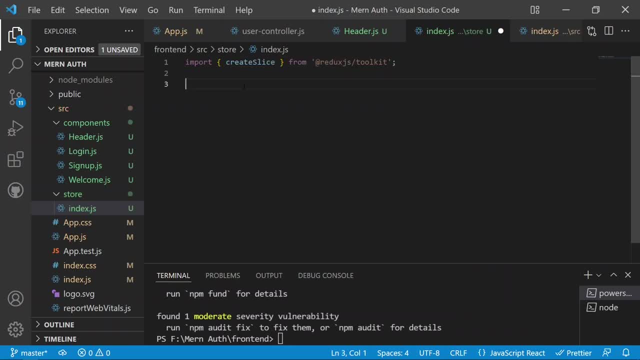 gs toolkit. so the slice will help us to create the. so the slice will help us to create the. so the slice will help us to create the slice. and the slice can contain the name slice. and the slice can contain the name slice. and the slice can contain the name: the reducer functions, the initial state. 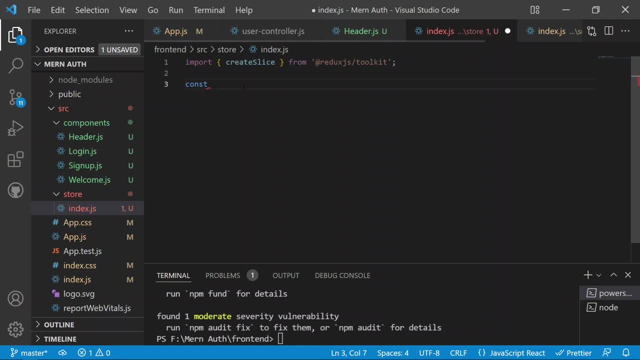 the reducer functions, the initial state, the reducer functions, the initial state, and everything which we need so we can, and everything which we need, so we can, and everything which we need so we can just create the slice for the, just create the slice for the, just create the slice for the authentication, so it can be the auth. 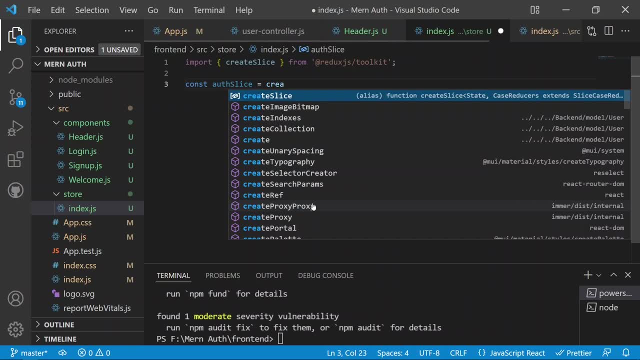 authentication, so it can be the auth authentication, so it can be the auth slice, slice, slice, and it will be equals to the create and it will be equals to the create and it will be equals to the create. slice that we have just imported, slice that we have just imported. 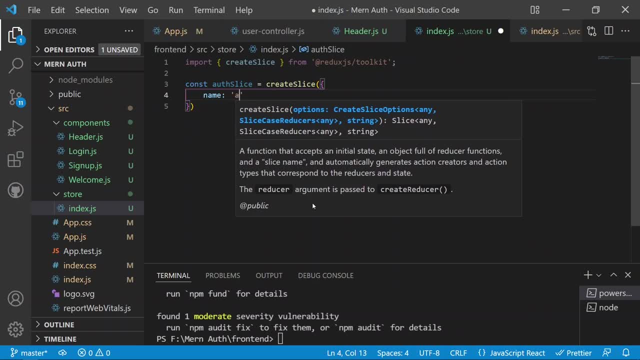 slice that we have just imported, and then we can just provide here the, and then we can just provide here the, and then we can just provide here the name and name can be the auth and name. name and name can be the auth and name. name and name can be the auth and name should be in the string, and then we can. 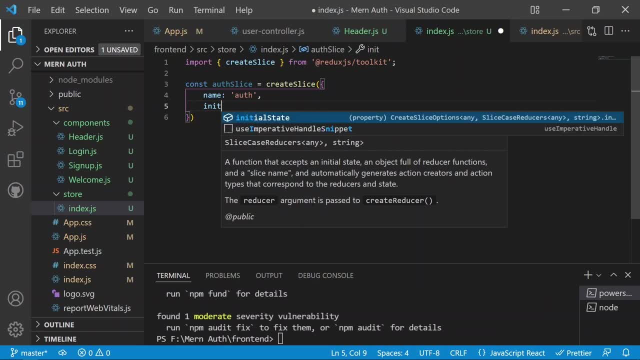 should be in the string, and then we can. should be in the string, and then we can just provide some initial state. just provide some initial state, just provide some initial state. so we need to provide the initial state. so we need to provide the initial state. so we need to provide the initial state of the application in an object. so it 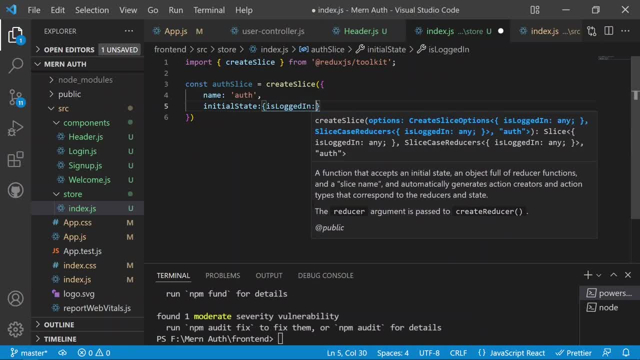 of the application in an object, so it of the application in an object, so it will contain the is logged in will contain the is logged in will contain the is logged in property and by default in the initial property. and by default in the initial property and by default in the initial state, it will be the false. 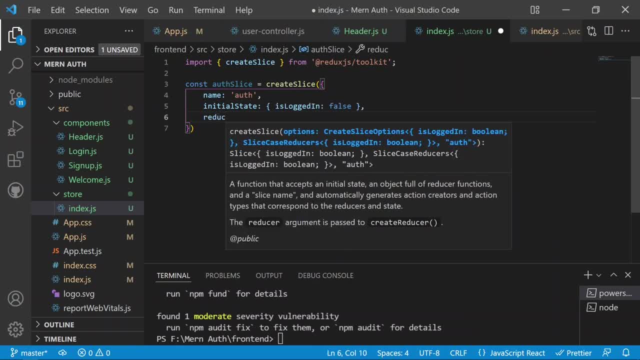 state, it will be the false state. it will be the false. and after the initial state, then we can. and after the initial state, then we can. and after the initial state, then we can define some reducers, define some reducers, define some reducers, so it will be the reducer functions now. 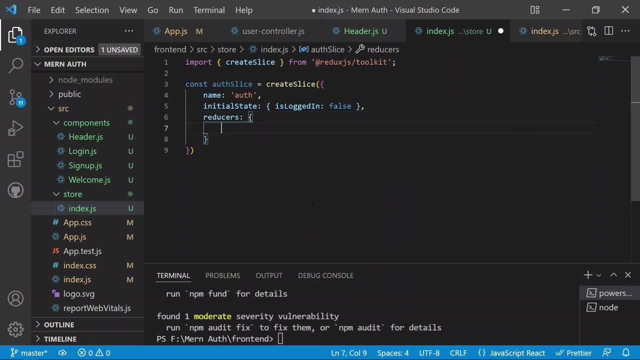 so it will be the reducer functions now. so it will be the reducer functions now and it will be an object and in this and it will be an object and in this and it will be an object and in this object. now we can generate the functions object, now we can generate the functions. 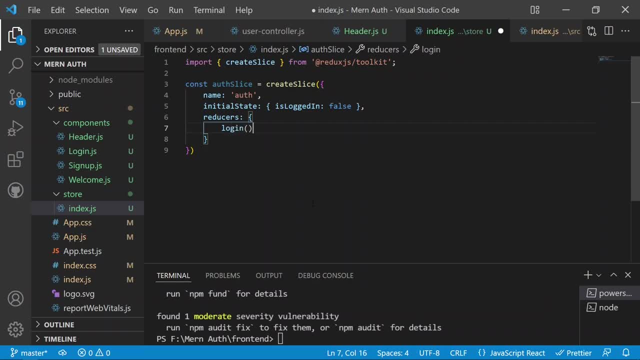 object. now we can generate the functions. so first it will be the login function, so first it will be the login function. so first it will be the login function and there is a login function, and then and there is a login function, and then and there is a login function, and then they have to do the logout function as 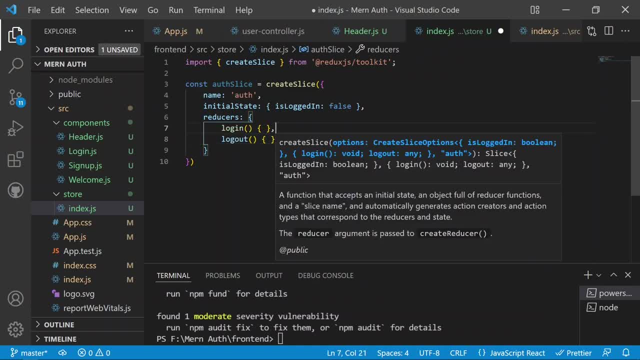 they have to do the logout function, as they have to do the logout function as well. and then in the login then we need to get, and then in the login then we need to get, and then in the login then we need to get the state as the parameter. 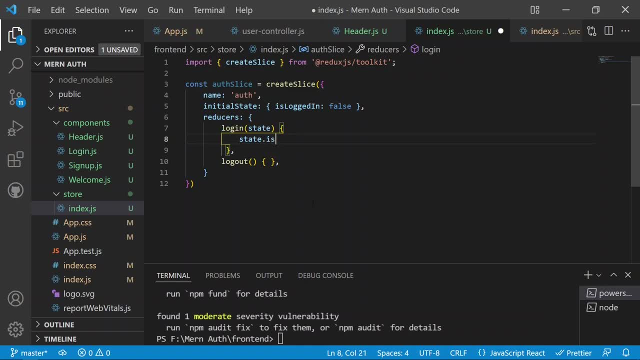 the state as the parameter, the state as the parameter, and then we can just change the state as: and then we can just change the state as: and then we can just change the state as. the state dot is logged in. the state dot is logged in. the state dot is logged in. property will be equals to the 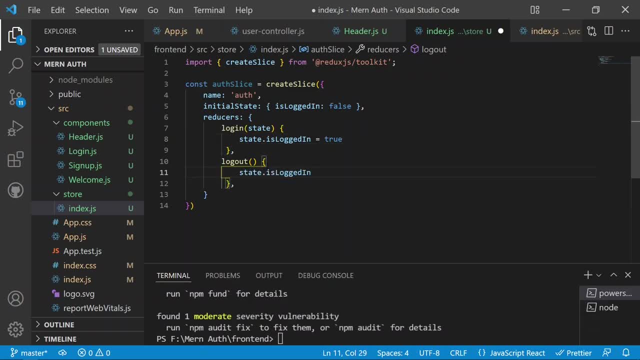 property will be equals to. the property will be equals to the. and then in the logout we can just. and then in the logout we can just. and then in the logout we can just: generate at the state the state dot is. generate at the state the state dot is. 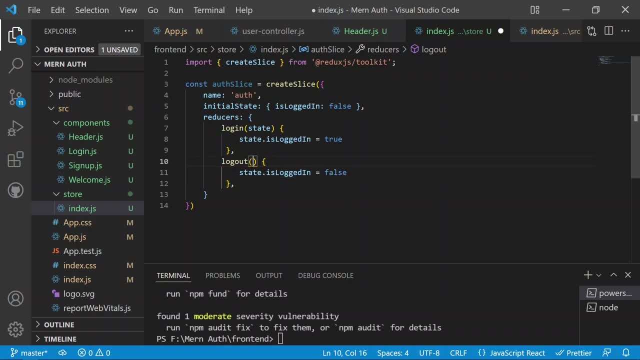 generate at the state. the state dot is logged in will be equals to the false. logged in will be equals to the false. logged in will be equals to the false. so we have now generated the state, and so we have now generated the state, and so we have now generated the state and the logout will also contain the state. 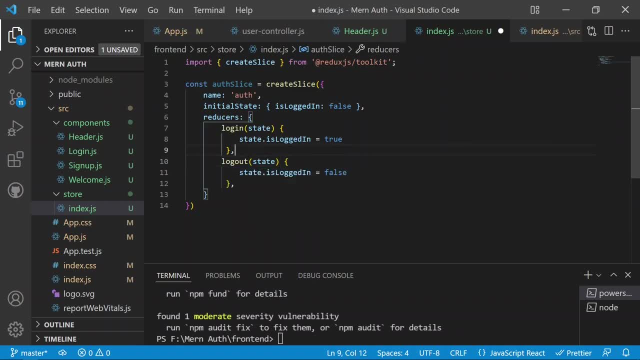 the logout will also contain the state. the logout will also contain the state inside that. so in the login we are now inside that. so in the login we are now inside that. so in the login we are now changing the state of the login to the. changing the state of the login to the. 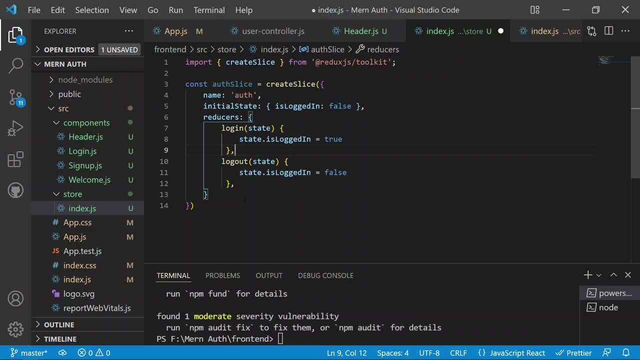 changing the state of the login to the true and in the logout we are now moving true and in the logout we are now moving true and in the logout we are now moving back the state to the false and after. back the state to the false and after. 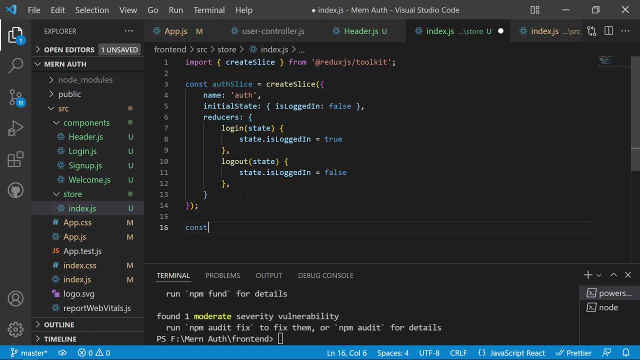 back the state to the false, and after that we need to export this slice also, that we need to export this slice also, that we need to export this slice also, so we can just export this store, so we can just export this store, so we can just export this store. functionality of the redux. so we are now. 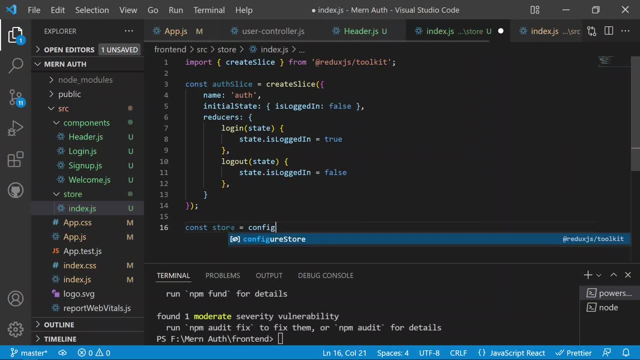 functionality of the redux. so we are now functionality of the redux, so we are now exporting the redux store from having exporting the redux store, from having exporting the redux store from having the configure store, so the configure the configure store, so the configure the configure store, so the configure store will be then imported again from. 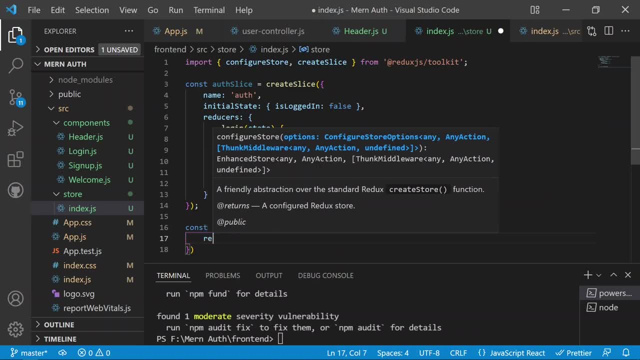 store will be then imported again from store, will be then imported again from the reduxious toolkit, and it will the reduxious toolkit and it will the reduxious toolkit and it will contain our object, so it will contain, contain our object, so it will contain, contain our object. so it will contain the reducers, so all of the reducer will. 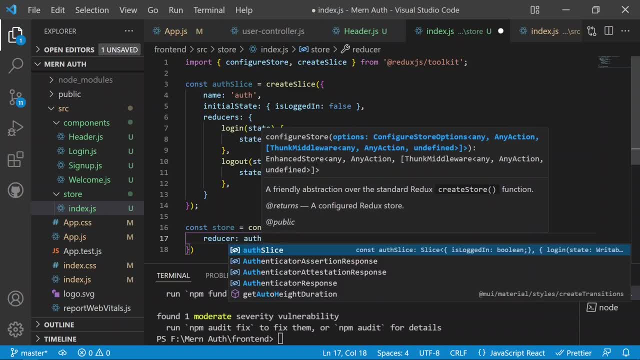 the reducers, so all of the reducer will the reducers, so all of the reducer will be then exported in there, so we can just be then exported in there. so we can just be then exported in there, so we can just export the reducer as the auth slice dot. 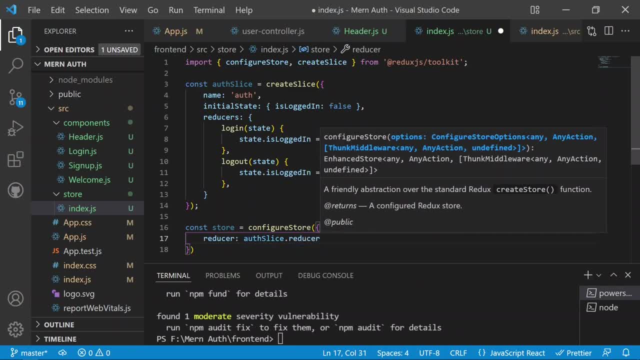 export the reducer as the auth slice dot, export the reducer as the auth slice dot. reducer that we have, reducer that we have, reducer that we have. so we are now exporting the reducer only. so we are now exporting the reducer only. so we are now exporting the reducer only for the auth slice now, because we only 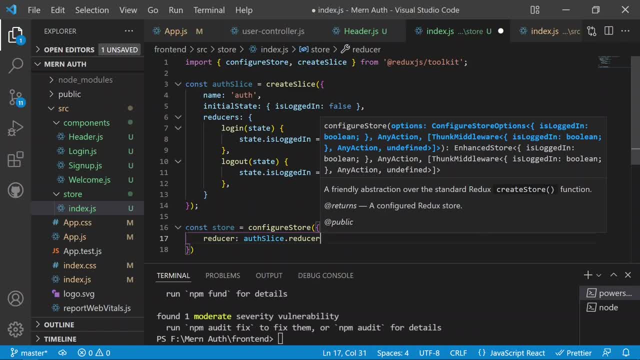 for the auth slice now, because we only for the auth slice now, because we only have the one slice in our application. have the one slice in our application, have the one slice in our application, and then we need to just export it, and then we need to just export it. 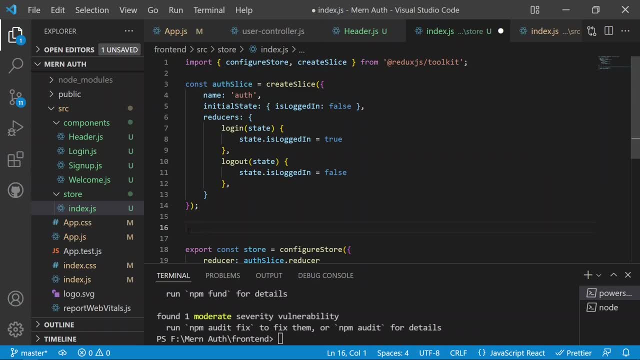 and then we need to just export it, and then for calling these functions then, and then for calling these functions then, and then for calling these functions, then we need to export the actions also. we need to export the actions also. we need to export the actions also. so we need to export the actions as the 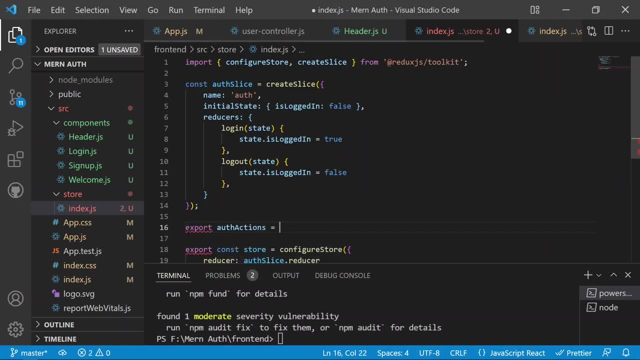 so we need to export the actions as the. so we need to export the actions as the auth actions, auth actions, auth actions, and it will be equals to the auth slice and it will be equals to the auth slice and it will be equals to the auth slice that we have. 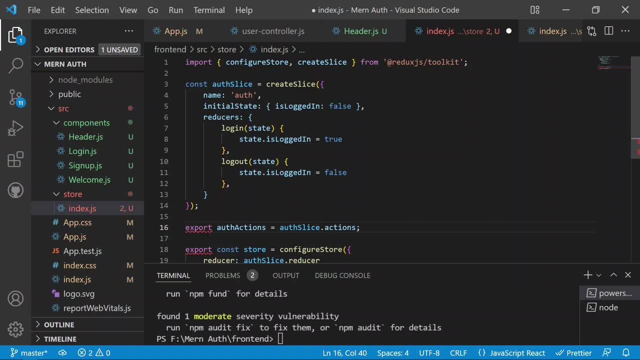 dot actions. so we need to export the auth dot actions. so we need to export the auth dot actions. so we need to export the auth slice dot actions. here also. slice dot actions here also. slice dot actions, here also. and now the redux store is completed. and now the redux store is completed. 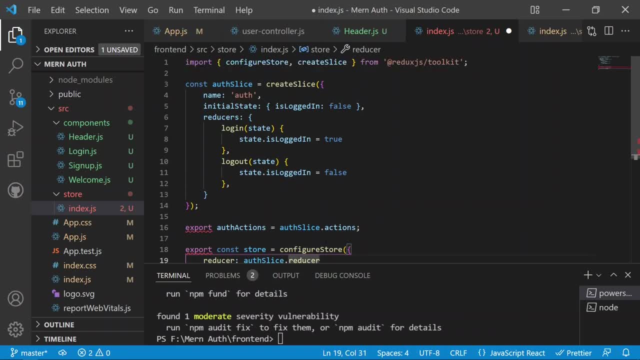 and now the redux store is completed, and now we need to import the redux store, and now we need to import the redux store, and now we need to import the redux store, and then we need to use the redux store, and then we need to use the redux store. 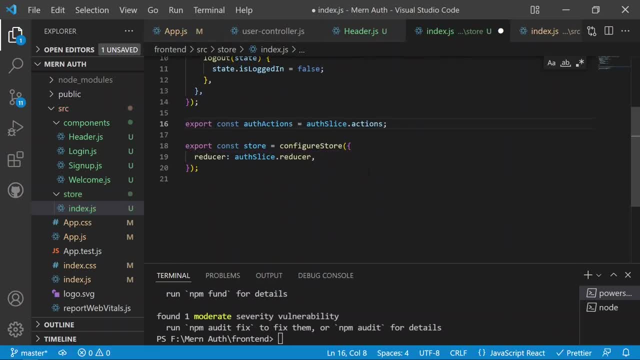 and then we need to use the redux store in the application, in the application, in the application. so then, after that, we can just move on. so then, after that, we can just move on. so then, after that, we can just move on to the indexjs, to the indexjs. 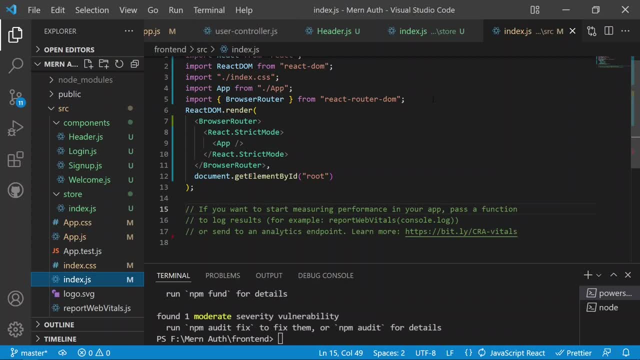 to the indexjs, which is the main file, which is a root, which is the main file, which is a root, which is the main file, which is a root file of our application, and then we can file of our application, and then we can file of our application, and then we can just import the provider. 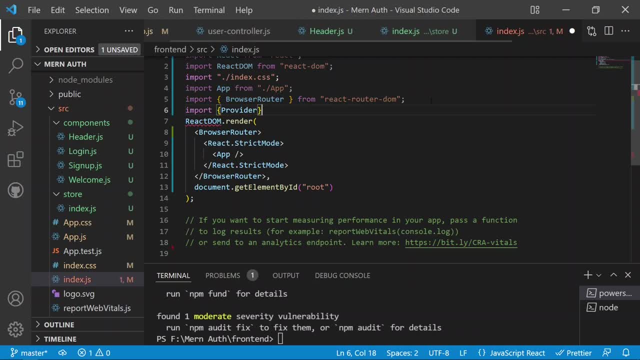 just import the provider. just import the provider from the react redux, so provider will from the react redux, so provider will from the react redux, so provider will help us to provide some redux store. help us to provide some redux store. help us to provide some redux store to the main application so we can just 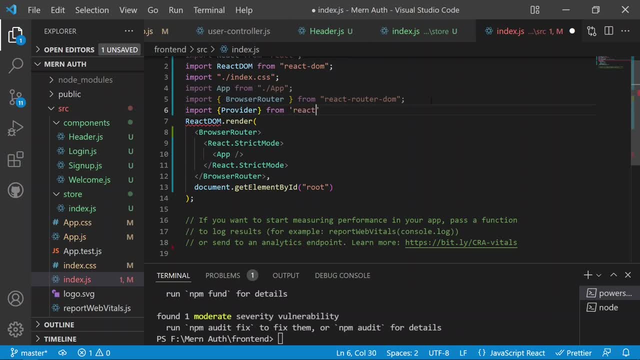 to the main application. so we can just to the main application. so we can just import the provider from the react redux, import the provider from the react redux, import the provider from the react redux that we have installed the package of, that we have installed the package of. 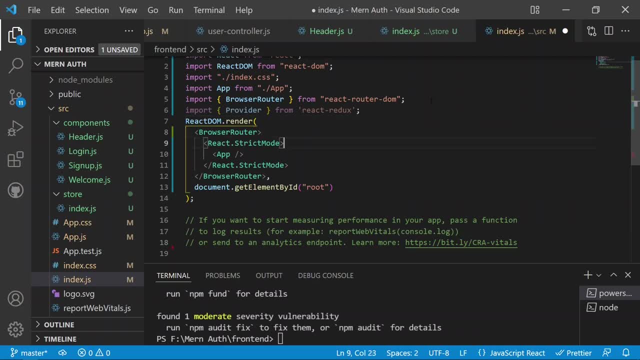 that we have installed the package of the react redux, the react redux, the react redux, and then we can just wrap the app. and then we can just wrap the app and then we can just wrap the app. component with the provider to provide. component with the provider to provide. 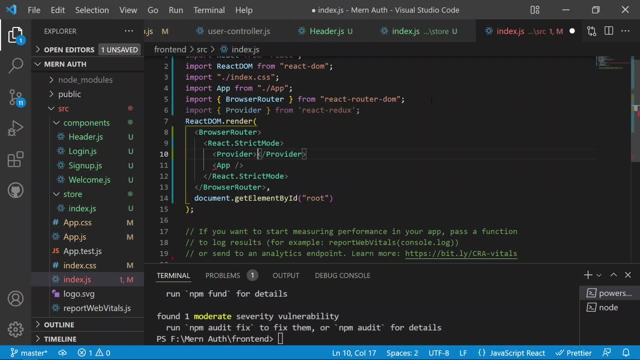 component with the provider to provide the redux functionality over the main app, the redux functionality over the main app, the redux functionality over the main app. component, component, component, and then we can just wrap the app and then we can just wrap the app and then we can just wrap the app component with the provider. 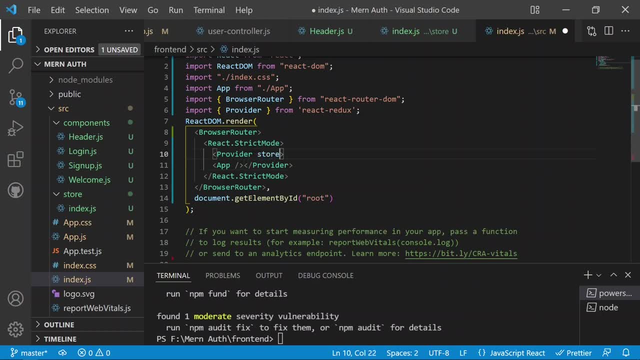 and then we can just provide here the, and then we can just provide here the, and then we can just provide here the store also in the provider, so it will store also in the provider, so it will store also in the provider, so it will contain the store. 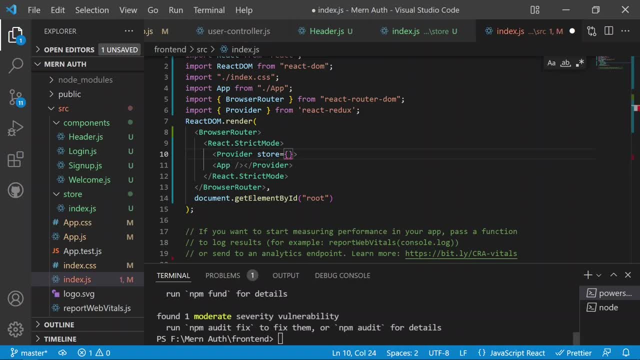 contain the store, contain the store, and the store will be equals to, and the store will be equals to the and the store will be equals to the store which we have just generated in store, which we have just generated in store, which we have just generated in which we have just exported from the 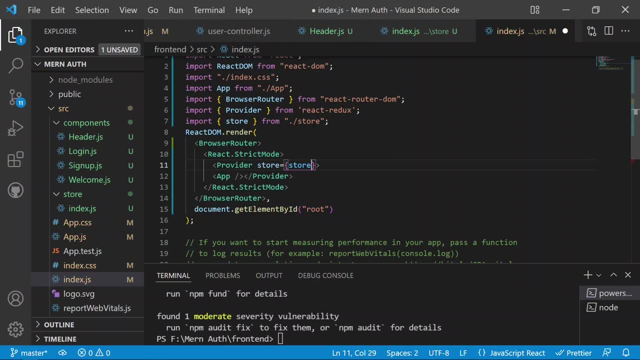 which we have just exported from the, which we have just exported from the indexjs store. so now we have now indexjs store. so now we have now indexjs store. so now we have now imported the store from the store index, imported the store from the store index. 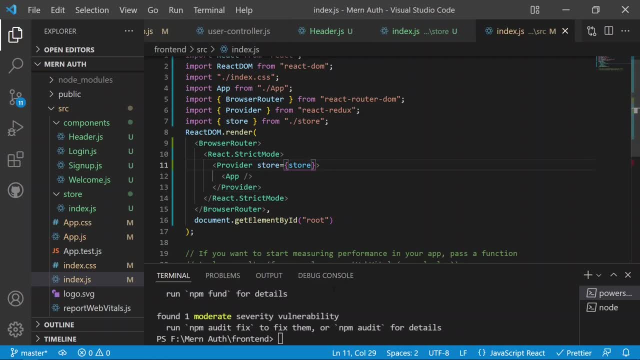 imported the store from the store indexjs, js, js. so now the app component has the full. so now the app component has the full, so now the app component has the full functionality of the redux functionality, of the redux functionality of the redux. so if i will now just save, if i will now 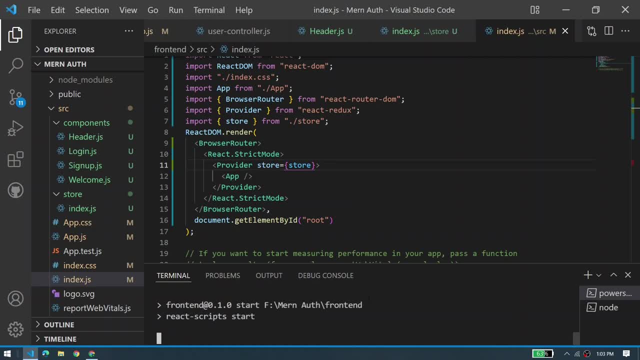 so if i will now just save, if i will now so, if i will now just save, if i will now just click on the npm start, if i will just click on the npm start, if i will just click on the npm start, if i will just start the server again, 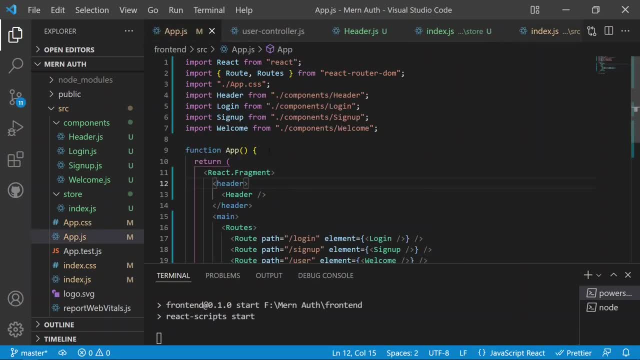 just start the server again. just start the server again, and then we need to move on to the app, and then we need to move on to the app, and then we need to move on to the appjs also- js also, js also- and then we can just get the store from. 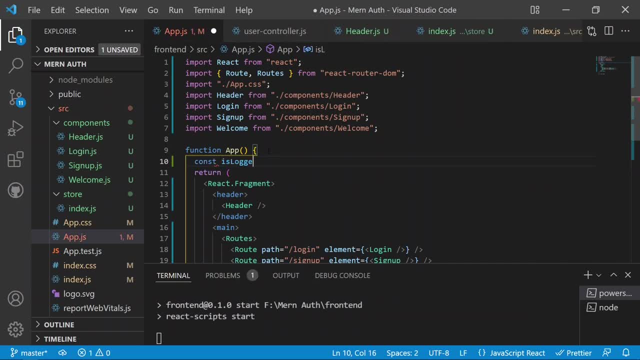 and then we can just get the store from, and then we can just get the store from the use selector hook. so we can just the use selector hook, so we can just the use selector hook, so we can just get the state of the is logged in. get the state of the is logged in. 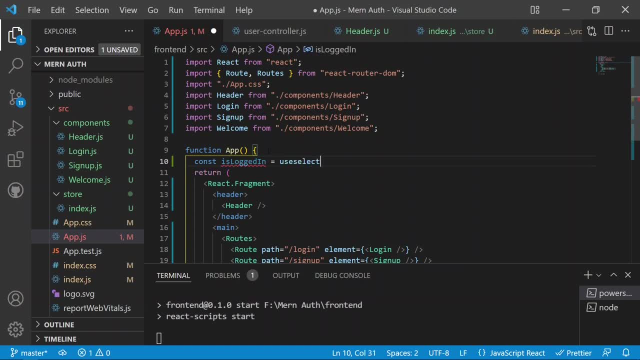 get the state of the is logged in in the redux from the use selector. will then allow us to grab the state. will then allow us to grab the state. will then allow us to grab the state so we can just use the use selector. and so we can just use the use selector. and. 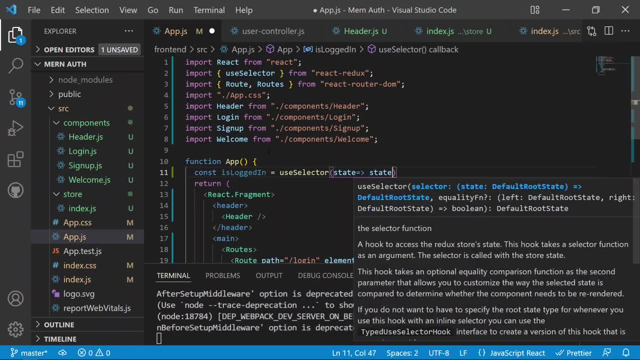 so we can just use the use selector, and it will contain the state as the. it will contain the state as the. it will contain the state as the parameter, parameter, parameter, and then we can just grab the state dot, and then we can just grab the state dot. 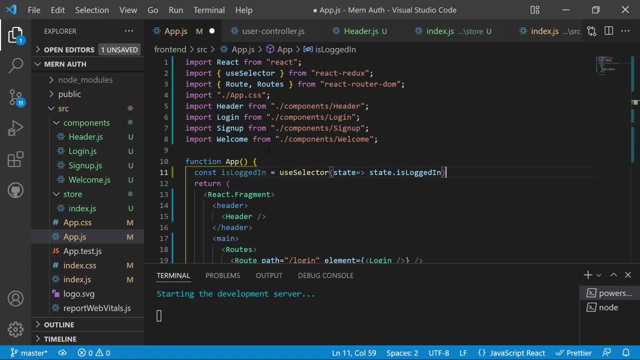 and then we can just grab the state dot: is logged in. property is logged in. property is logged in property. so we are now getting the access of the. so we are now getting the access of the. so we are now getting the access of the. is logged in property from there. 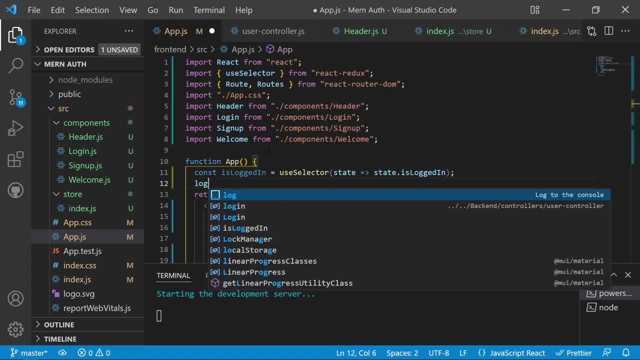 is logged in property from there. is logged in property from there. and if i will now just consolelog the and if i will now just consolelog the and if i will now just consolelog the. is logged in. is logged in. is logged in to check if the state is there or not. 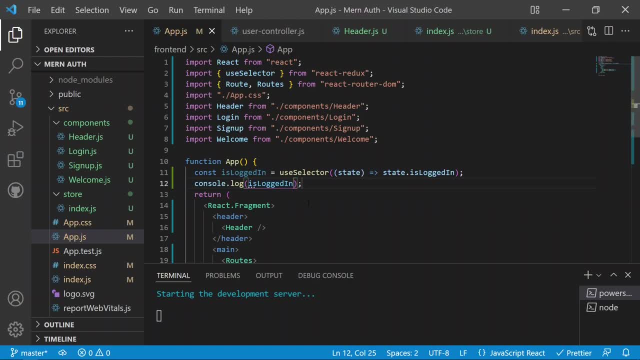 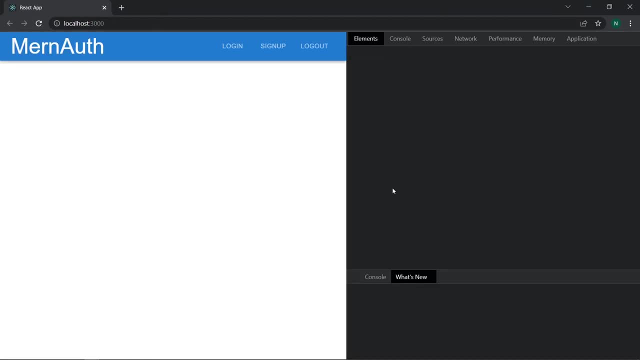 so now, if i will now save now, we should so now. if i will now save now, we should so now. if i will now save now, we should see the changes to the application. and now the application is compiled, and, and now the application is compiled, and, and now the application is compiled, and now, if i will now click on the inspect. now, if i will now click on the inspect now, if i will now click on the inspect now in the console. now we should see the now in the console. now we should see the now in the console. now we should see the state now. you will see, now we have the. 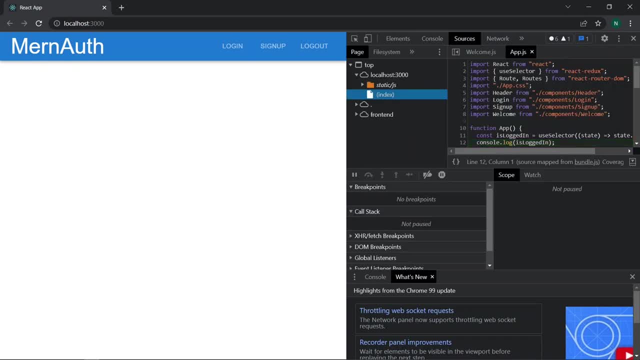 state. now you will see. now we have the state. now you will see. now we have the redux state, which is the false as of now. redux state, which is the false as of now. redux state, which is the false as of now because the is logged in, is now the false. 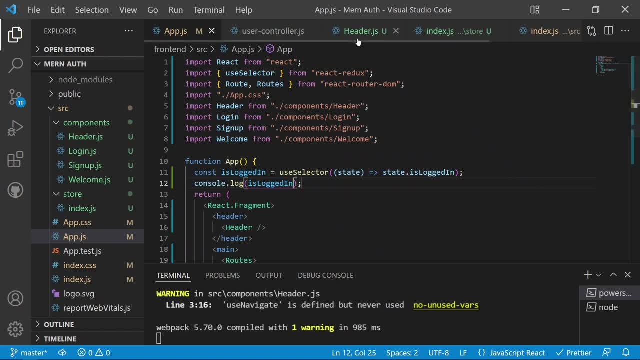 because the is logged in is now the false. because the is logged in is now the false, and now we can just use that is. and now we can just use that is. and now we can just use that is. logged in property in the header also. logged in property in the header also. 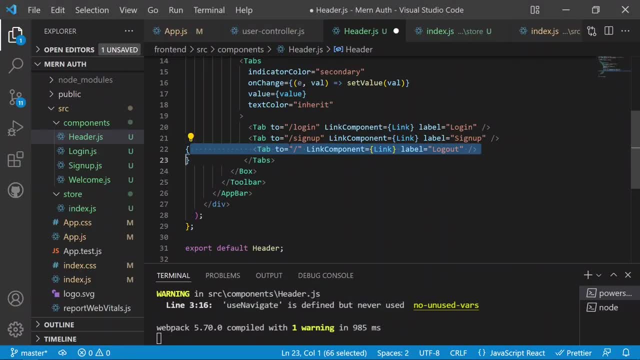 logged in property in the header also. so now we have the three routes in there. so now we have the three routes in there. so now we have the three routes in there. so we need to check if we have the is. so we need to check if we have the is. 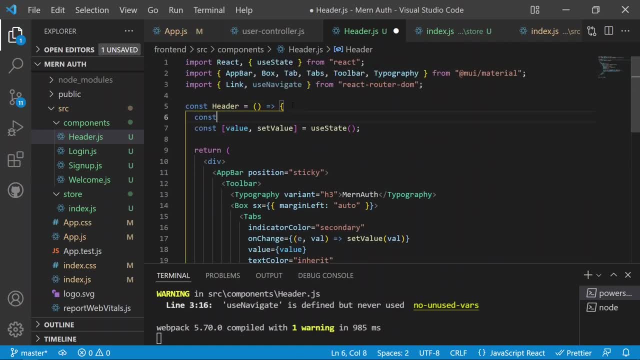 so we need to check. if we have the is logged in so we can just grab the is logged in, so we can just grab the is logged in, so we can just grab the is logged in here also. logged in here, also logged in here also. so const as the is logged in. 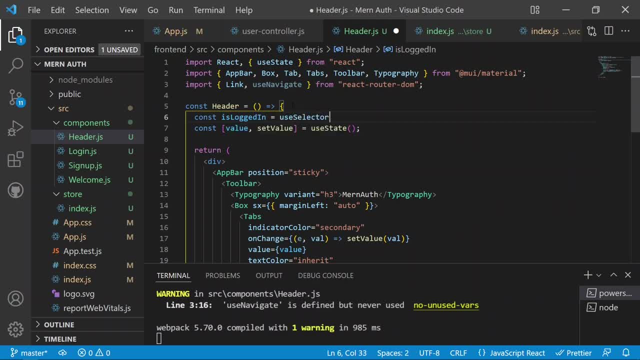 so const as the is logged in, so const as the is logged in and it will be equals to the use and it will be equals to the use and it will be equals to the use selector. so we can just grab the? u selector here. so we can just grab the? u selector here. 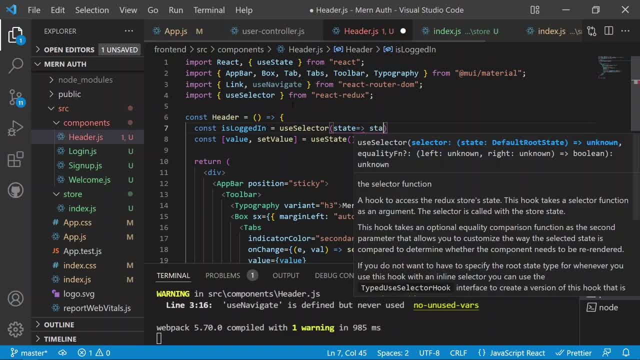 so we can just grab the u selector here. also it will contain the state as the. also it will contain the state as the. also it will contain the state as the parameter, and then we can just grab the parameter. and then we can just grab the parameter, and then we can just grab the state again from the state. dot is logged. 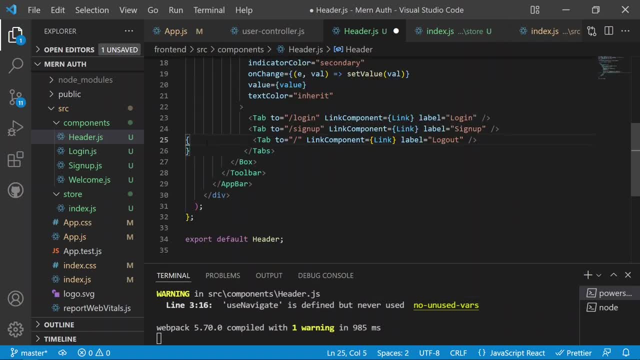 state again from the state dot is logged. state again from the state dot is logged in in in. so we can just add here the conditional. so we can just add here the conditional. so we can just add here the conditional rendering so when the is logged in, rendering so when the is logged in. 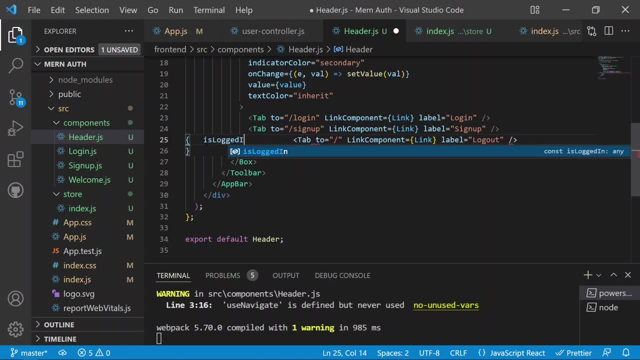 rendering. so when the is logged in property property, property will be the true, will be the true, and then only we need to render this tab, and then only we need to render this tab, and then only we need to render this tab. so if i will now save, so now we should. 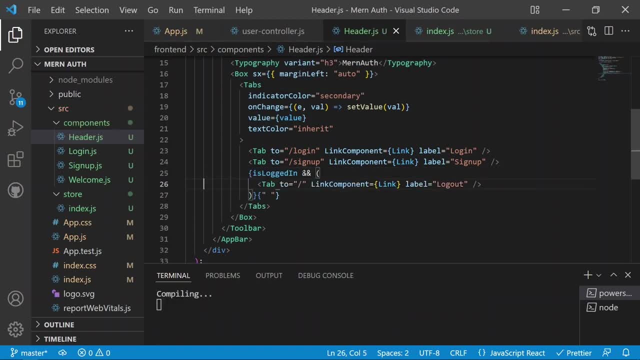 so if i will now save, so now we should. so if i will now save, so now we should see the changes onto the screen once. see the changes onto the screen once. see the changes onto the screen once again, again, again. so if i will now save, now we should see. 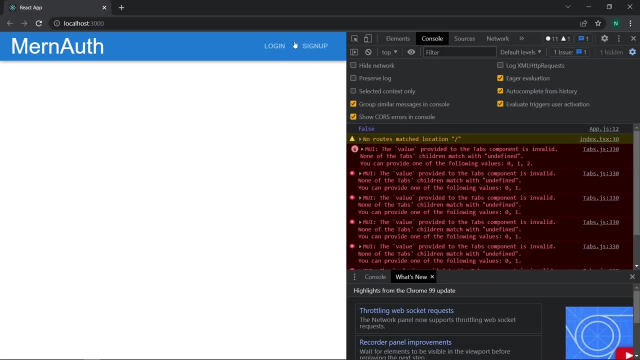 so if i will now save now we should see. so if i will now save now, we should see the changes like the logout should be, the changes like the logout should be, the changes like the logout should be removed. so now you will see the logout removed. so now you will see the logout. 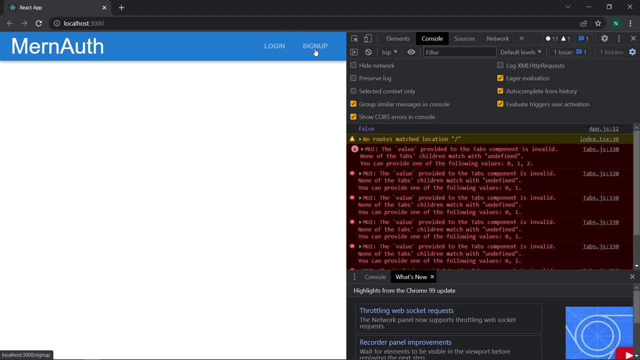 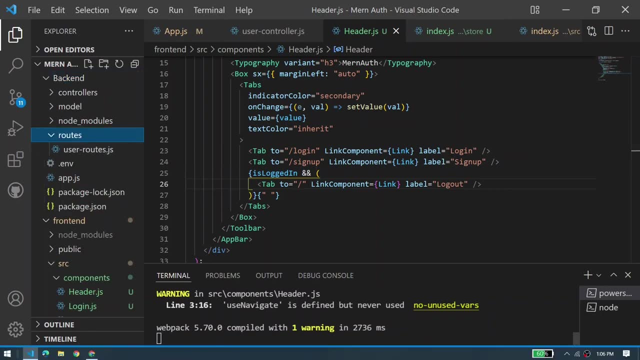 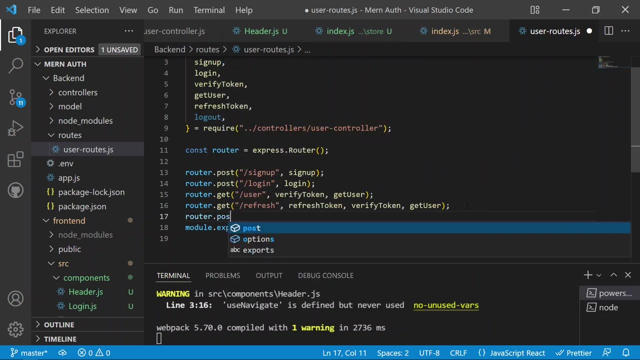 removed. so now you will see the logout is now not there. because now the is is now not there. because now the is is now not there because now the is logged in, logged in, logged in. so it will be the post request and the. so it will be the post request and the. 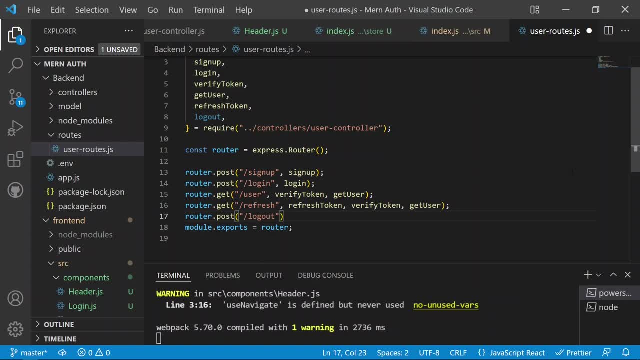 so it will be the post request and the route will be the logout route will be the logout route will be the logout and then after that we can just create, and then after that we can just create and then after that we can just create terms. here some controller functions: 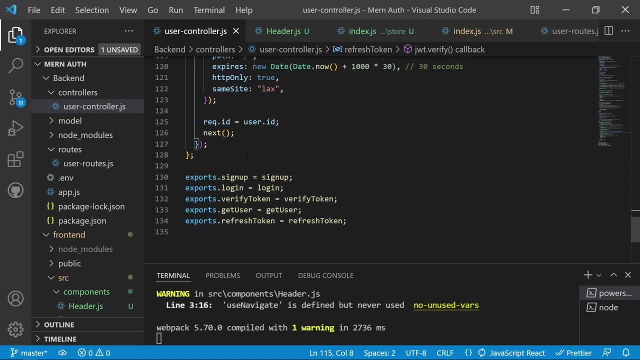 terms here some controller functions. terms here: some controller functions also. so we can move on to the user also. so we can move on to the user also. so we can move on to the user controller, controller, controller, and then we can just create a new, and then we can just create a new. 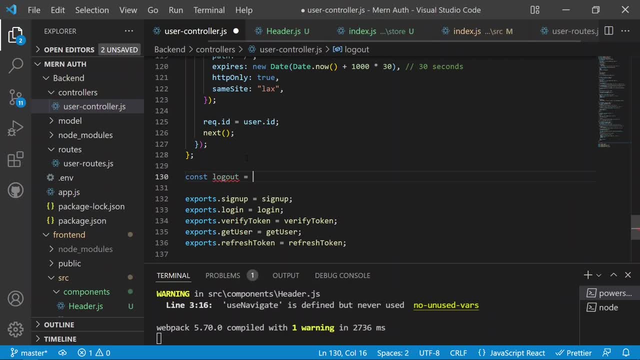 and then we can just create a new function here as the const logout function, here as the const logout function, here as the const logout, and it will be equals to the again the and it will be equals to the again the and it will be equals to the again the request response and the next. 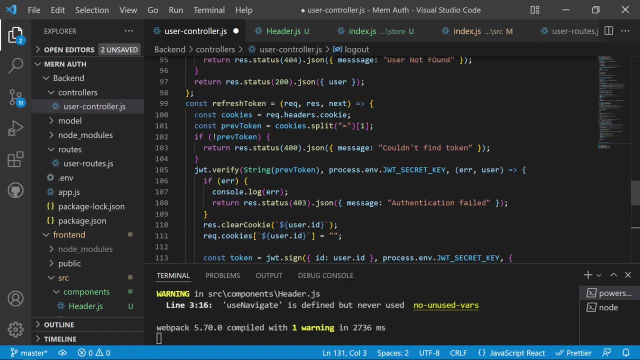 request response and the next request response and the next and for the logout. i think now we need. and for the logout. i think now we need. and for the logout. i think now we need to get some cookies again, so we can just to get some cookies again, so we can just. 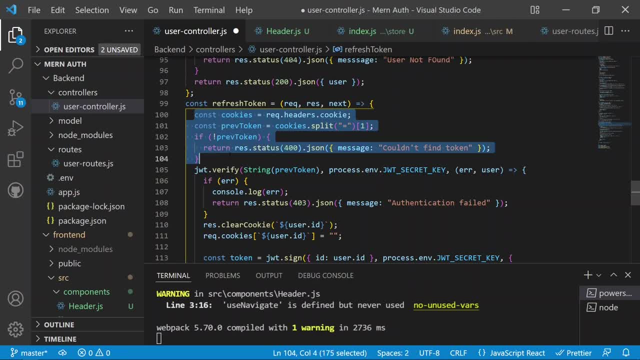 to get some cookies again, so we can just grab the cookies, grab the cookies, grab the cookies. and the previous token also, so we can, and the previous token also, so we can, and the previous token also, so we can just grab that, just grab that, just grab that. so i will now just copy from the 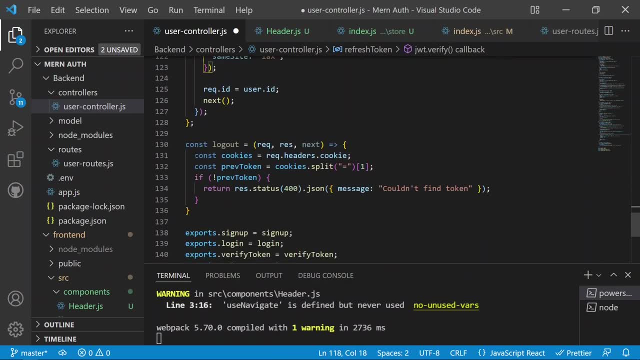 so i will now just copy from the. so i will now just copy from the verify token. verify token, verify token. and then now you will see: now we have, and then now you will see, now we have, and then now you will see: now we have the cookies and now we have the previous. 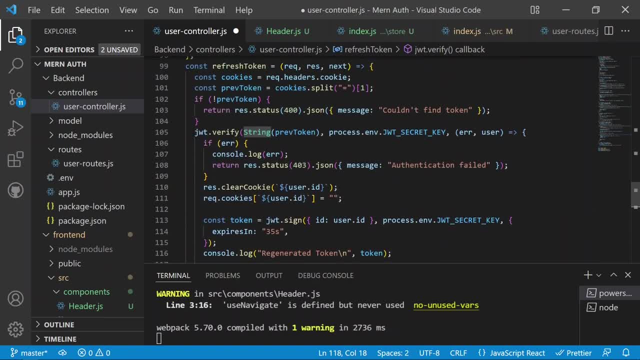 the cookies, and now we have the previous the cookies, and now we have the previous token, and then we can just check token, and then we can just check token, and then we can just check, and now we need to verify it again. so we, and now we need to verify it again, so we. 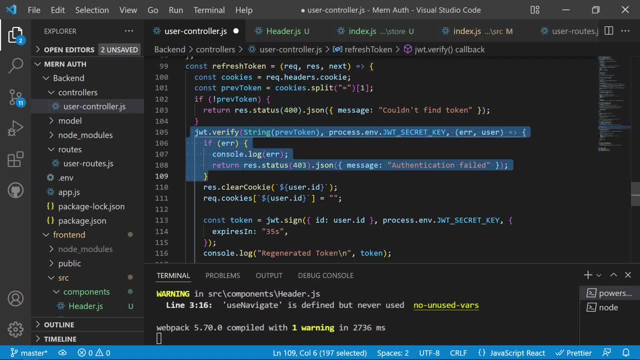 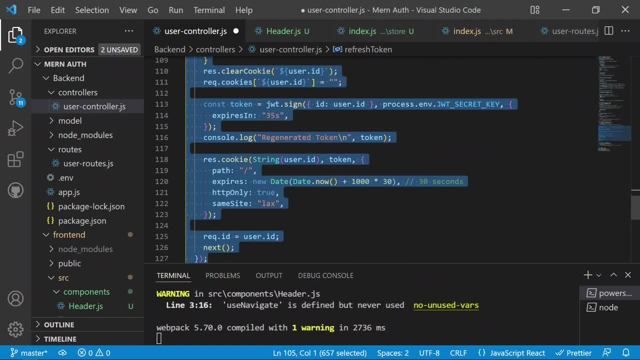 also for that, also for that. so i will now grab this, because now we. so i will now grab this, because now we, so i will now grab this, because now we need to verify the token as well. once we need to verify the token as well, once we. 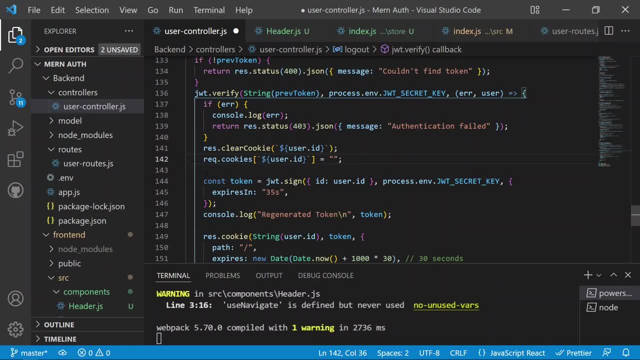 need to verify the token as well. once we then verified, then we are now clearing, then verified, then we are now clearing, then verified, then we are now clearing the cookie, and then we don't need to the cookie, and then we don't need to the cookie and then we don't need to create a new token again. so i will now. 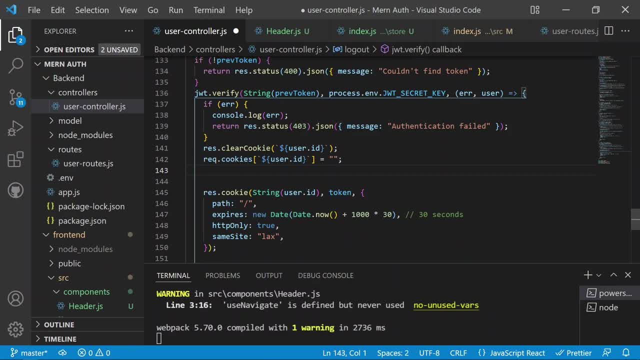 create a new token again. so i will now create a new token again. so i will now remove this from the consolelog. remove this from the consolelog. remove this from the consolelog. generated token as well, and then you generated token as well, and then you generated token as well, and then you will see, now we have the clear cookie. 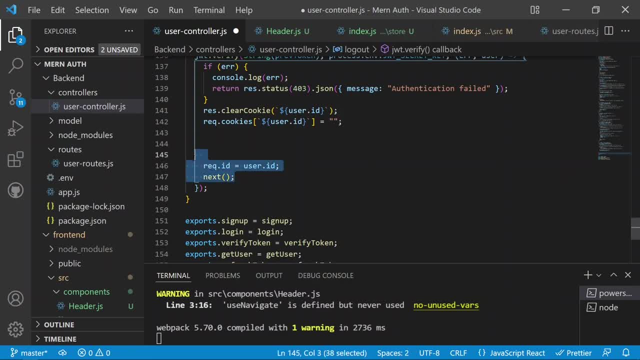 will see. now we have the clear cookie will see. now we have the clear cookie again. so i will now remove this as well again. so i will now remove this as well again. so i will now remove this as well and this as well. so now you will see now. 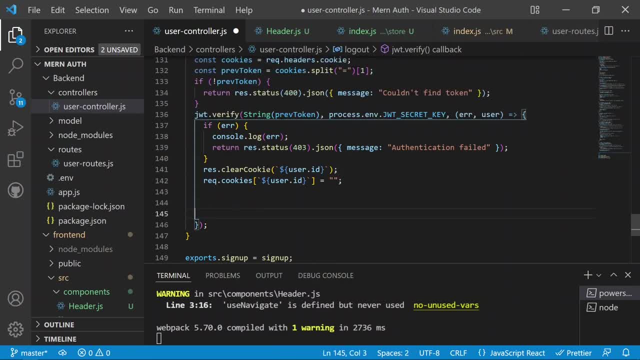 and this as well. so now you will see now and this as well. so now you will see: now we are in the, we are in the. we are in the jw2.verify so once the token will be: jw2.verify so once the token will be. 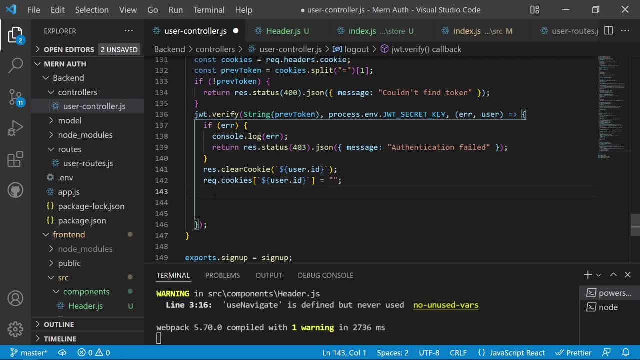 jw2.verify. so once the token will be successfully verified, then we need to successfully verified, then we need to successfully verified, then we need to clear the cookie. so now we are now clear the cookie. so now we are now clear the cookie. so now we are now clearing the cookie and then we need to. 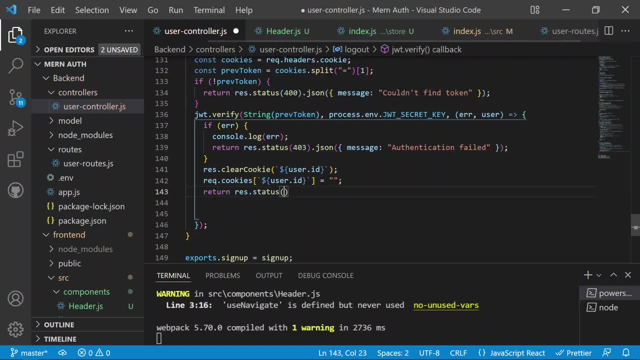 clearing the cookie, and then we need to clearing the cookie and then we need to just return as the response: dot status. just return as the response: dot status. just return as the response. dot status will be equals to the 200 and then dot will be equals to the 200 and then dot. 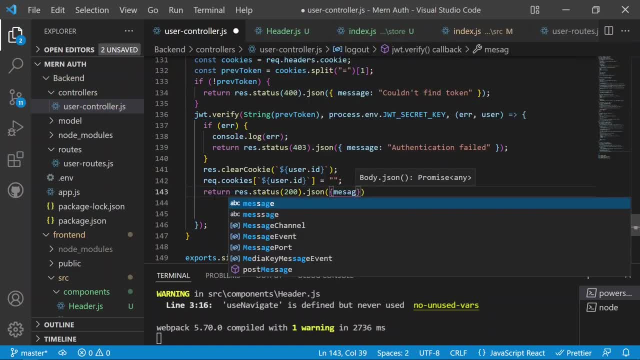 will be equals to the 200, and then dot json, json, json will be equals to it will contain the will be equals to. it will contain the will be equals to it will contain the message, message, message, and the message will contain that they and the message will contain that they. 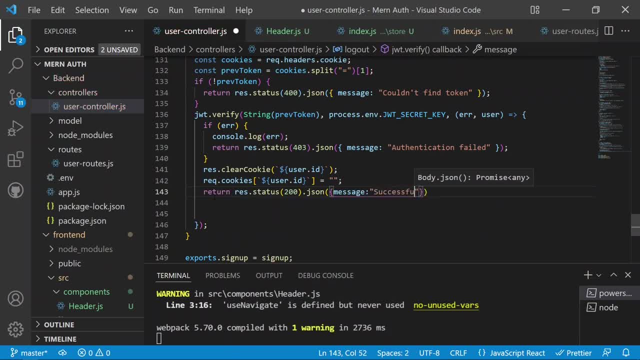 and the message will contain that they successfully logged out, logged out, logged out, so we can just grab that. so we can just. so we can just grab that, so we can just so we can just grab that. so we can just save now and now we can just. 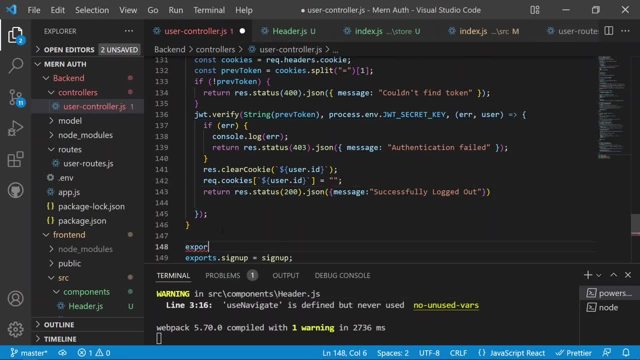 save now and now. we can just save now and now. we can just export the logout route as well. so it export the logout route as well. so it export the logout route as well. so it, with the exports, with the exports, with the exports, dot logout, dot logout. 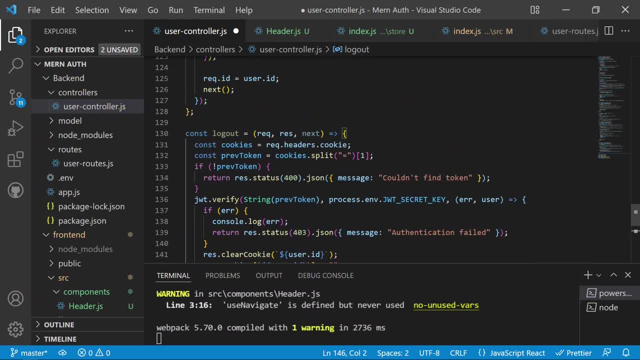 dot logout, and it will the logout, and it will the logout, and it will the logout. so now we are exporting the logout, as so now we are exporting the logout, as so now we are exporting the logout as well. and now we need to move on to the 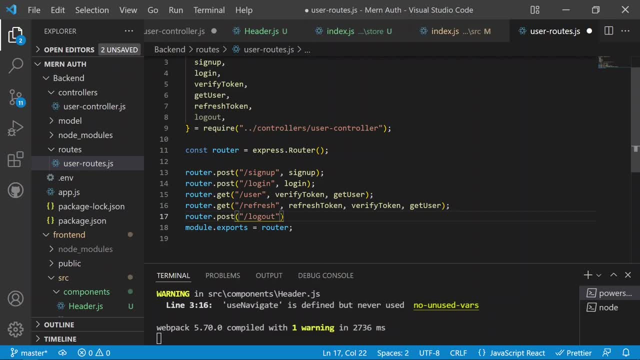 well, and now we need to move on to the well, and now we need to move on to the routes from the user routes, and then we routes from the user routes, and then we routes from the user routes, and then we need to grab here as a logout also. need to grab here as a logout also. need to grab here as a logout also. so for the logout first. we need to. so for the logout first, we need to. so for the logout first, we need to verify the token that we will receive. verify the token that we will receive. 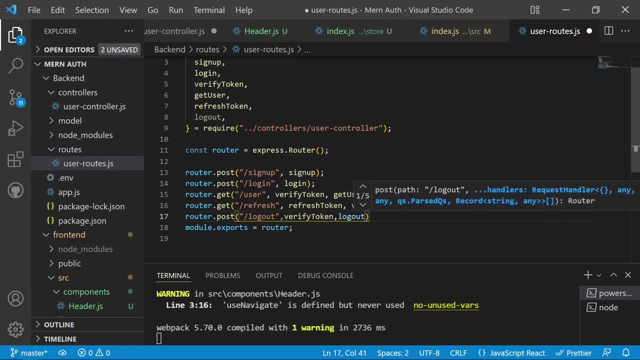 verify the token that we will receive from the front end. verify token from the front end. verify token from the front end. verify token. and then we will add the logout. so now, and then we will add the logout. so now, and then we will add the logout. so now everything should work fine. so now we. 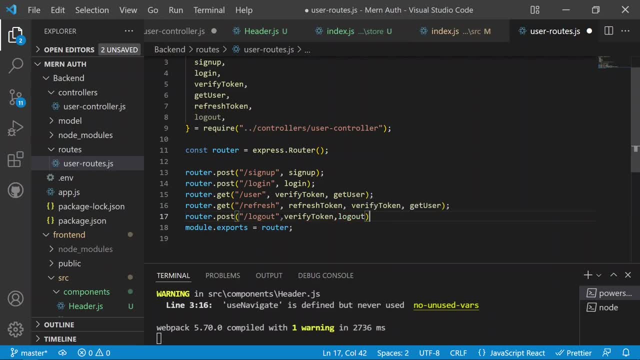 everything should work fine. so now we- everything should work fine. so now we are now importing the logout as well, are now importing the logout as well, are now importing the logout as well. so now we have imported the logout. so so now we have imported the logout. so 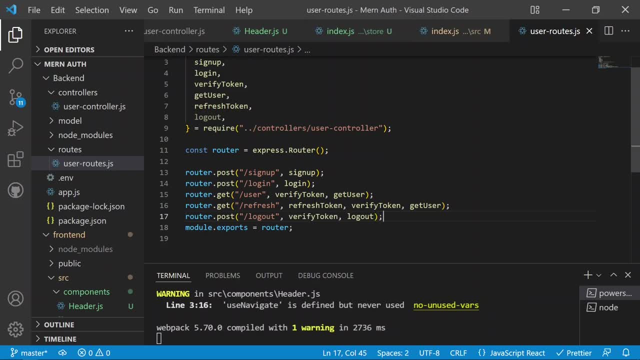 so now we have imported the logout, so everything now should work fine. everything now should work fine. everything now should work fine. and now we have created the logout also, and now we have created the logout also, and now we have created the logout also and it will be a post request. and it will be a post request, and it will be a post request. and now the backend work is complete, and and now the backend work is complete, and and now the backend work is complete, and now we need to move on to the front, and now we need to move on to the front. 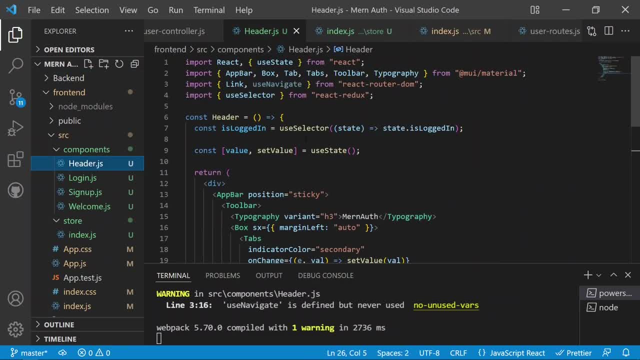 and now we need to move on to the front end again so we can just move on to the end again, so we can just move on to the end again, so we can just move on to the header, and then we can just header, and then we can just. 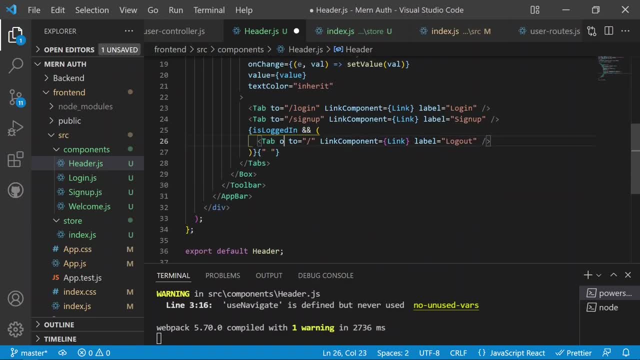 header, and then we can just call here some function on the on click. call here some function on the on click. call here some function on the on click of the logout tab of the logout tab. of the logout tab that will contain the on click that will contain the on click. 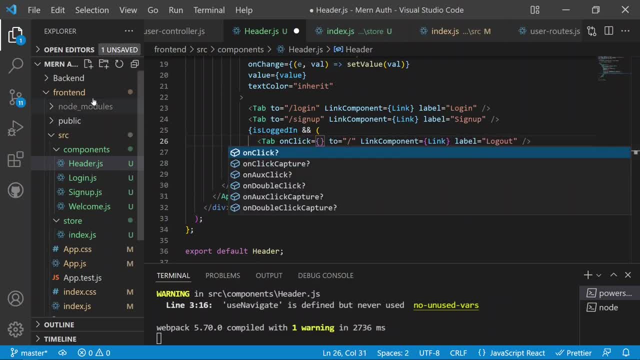 that will contain the on click, and in the on click we can now call and in the on click we can now call, and in the on click we can now call. here, the here, the here, the api for the logout. so we can just have api for the logout, so we can just have. 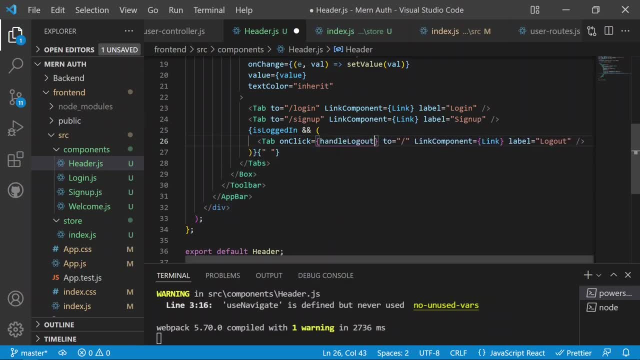 api for the logout. so we can just have a handle, a handle, a handle, logout function, logout function, logout function, and then we can just create the handle, and then we can just create the handle, and then we can just create the handle logout function in the header as well. so 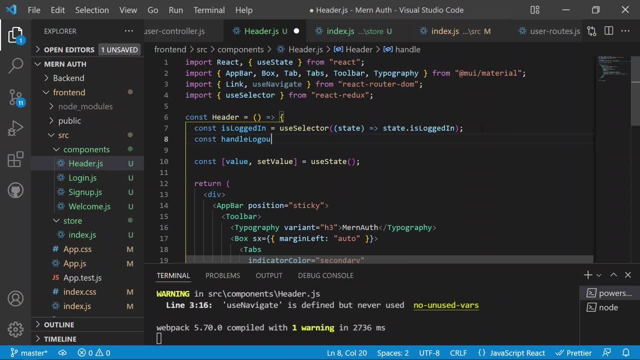 logout function in the header as well. so logout function in the header as well. so it will the const, it will the const, it will the const as the handle logout, as the handle logout, as the handle logout, and it will be equals to the function. and then for that i will now create a. 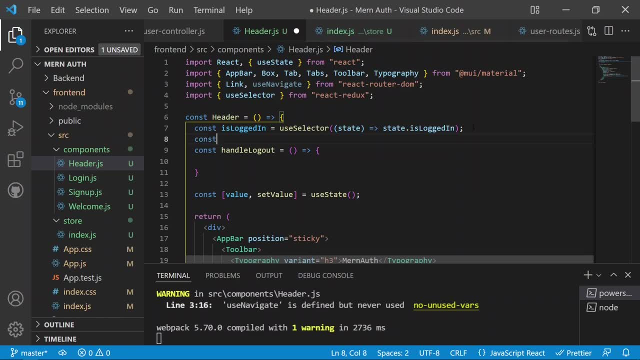 and then for that i will now create a, and then for that i will now create a new function for sending the request. new function for sending the request, new function for sending the request. so it will the const as the send logout. so it will the const as the send logout. 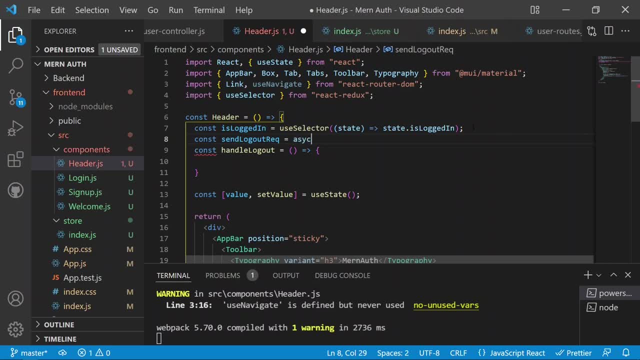 so it will. the const as the send logout request will be equals to a async request, will be equals to a async request, will be equals to a async function, and then we can just import the xios, and then we can just import the xios, and then we can just import the xios also at the xios. 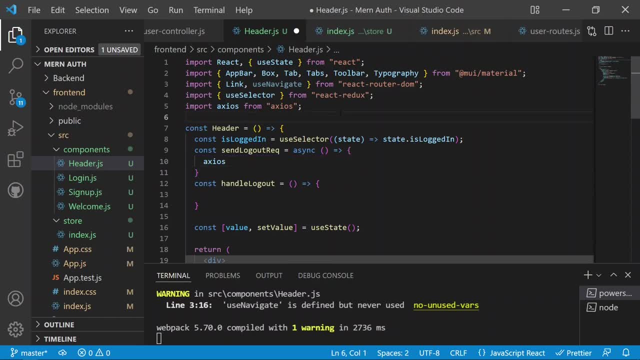 also at the xios, also at the xios. so now we have imported the xios, and so now we have imported the xios, and so now we have imported the xios, and now we need to create in some defaults. now we need to create in some defaults. 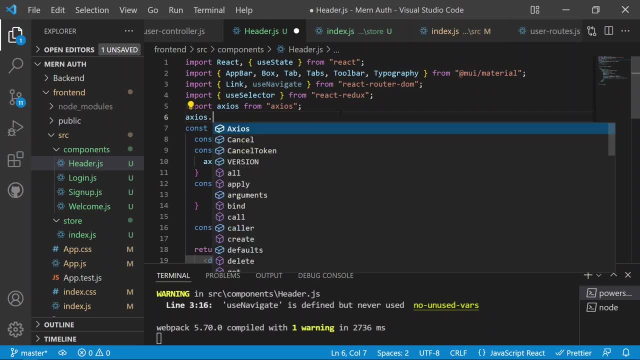 now we need to create in some defaults of the xios also. so the xios will of the xios also, so the xios will of the xios also. so the xios will contain the defaults as well. because we contain the defaults as well, because we 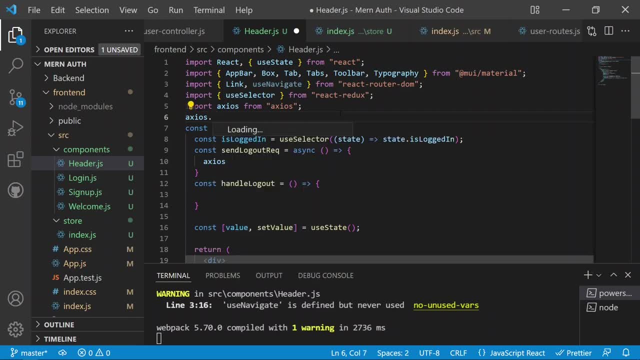 contain the defaults as well, because we need to send the credentials also. so the need to send the credentials also, so the need to send the credentials also, so the xios, it will be the xios, dot, xios, it will be the xios, dot, xios, it will be the xios, dot, defaults and dot. fifth credentials. 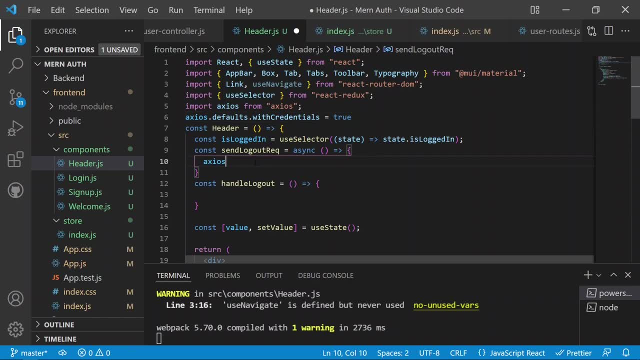 so the grid condition property will be so the grid condition property will be so the grid condition property will be: equals to the true, equals to the true, equals to the true, and then we can just send the request. so, and then we can just send the request so. 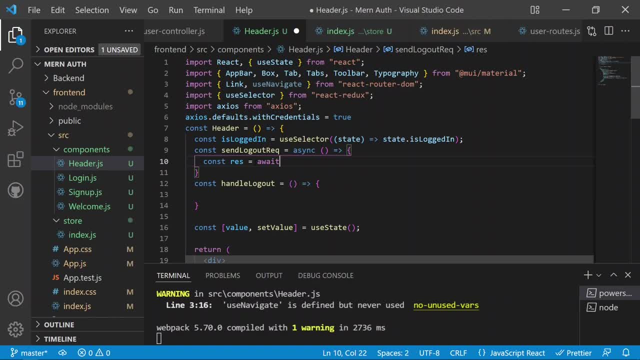 and then we can just send the request. so it will be the const as the response. it will be the const as the response. it will be the const as the response will be equals to the await. because it will be equals to the await, because it will be equals to the await, because it is an asynchronous task. 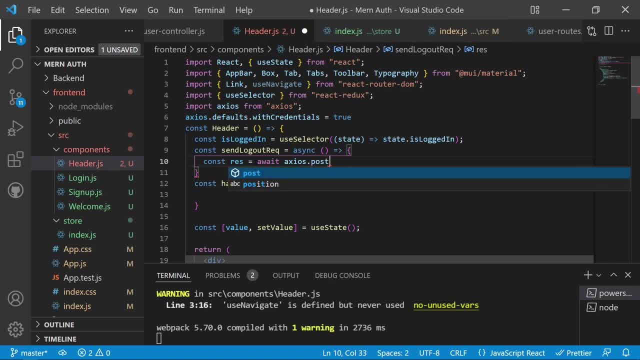 is an asynchronous task is an asynchronous task, so it will the await as the axios dot. so it will the await as the axios dot. so it will the await as the axios dot. post, post, post. so we are now sending the post http. so we are now sending the post http. 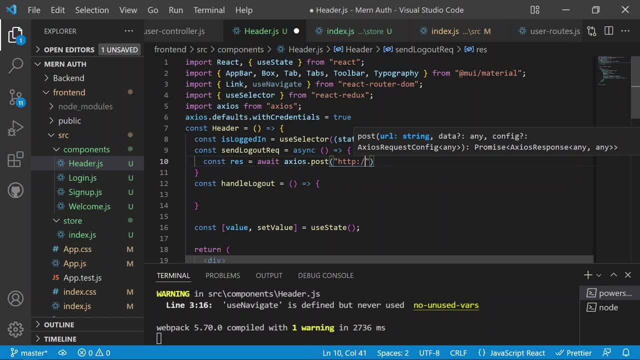 so we are now sending the post: http request request. request. so the url with the http, so the url with the http, so the url with the http: localhost, localhost, localhost. the port will be 5000 and it will be slash. the port will be 5000 and it will be slash. 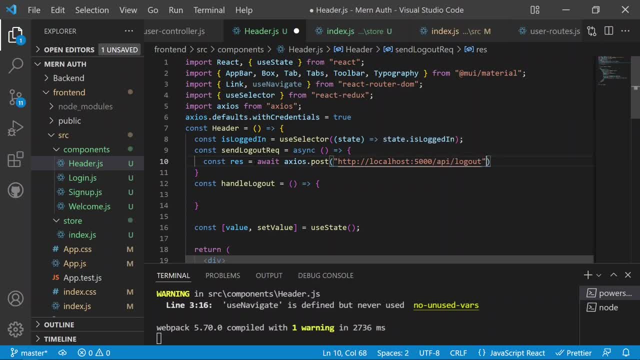 the port will be 5000 and it will be slash, api, api, api, slash logout. so this will be the route and slash logout, so this will be the route. and slash logout, so this will be the route, and then then then the second parameter is we need to send. 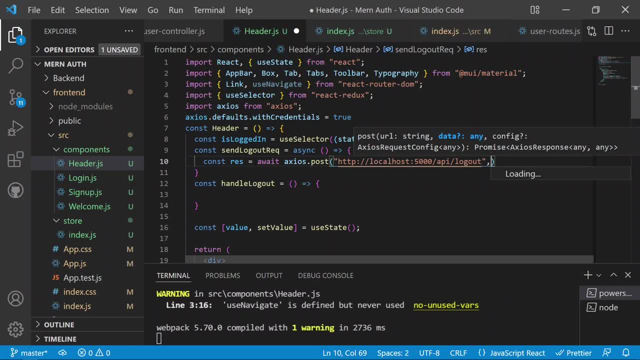 the second parameter is we need to send. the second parameter is we need to send here the data. so we don't have any data here the data. so we don't have any data here the data. so we don't have any data to send in the logout, so we can just. 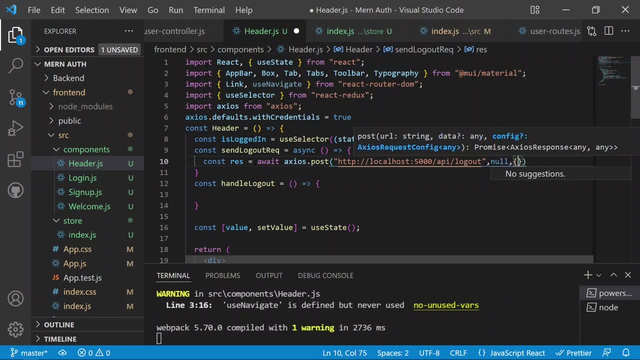 to send in the logout, so we can just to send in the logout, so we can just send here the null object. so now we are send here the null object, so now we are send here the null object, so now we are sending null. and then there in the 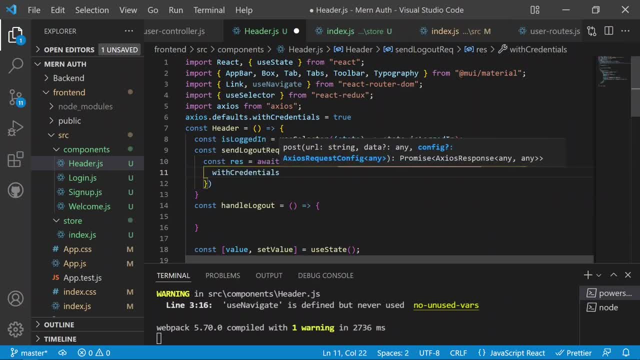 sending null and then there in the sending null, and then there in the config options, and then we can just send config options, and then we can just send config options and then we can just send the with credentials property to the true, the with credentials property to the true. 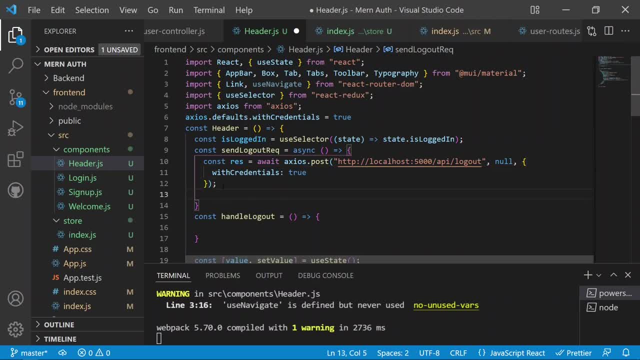 the with credentials, property to the true. so now everything should work fine. and so now everything should work fine. and so now everything should work fine. and now we can just have a condition like if now we can just have a condition like if now we can just have a condition like if the response 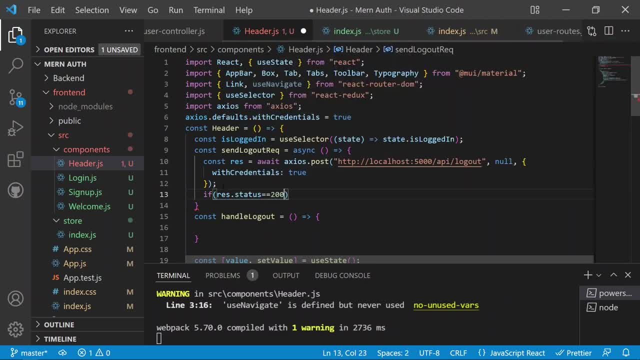 the response. the response: dot dot dot. i think the status equals to e200. i think the status equals to e200. i think the status equals to e200, and then we can just return response, and then we can just return response, and then we can just return response there. 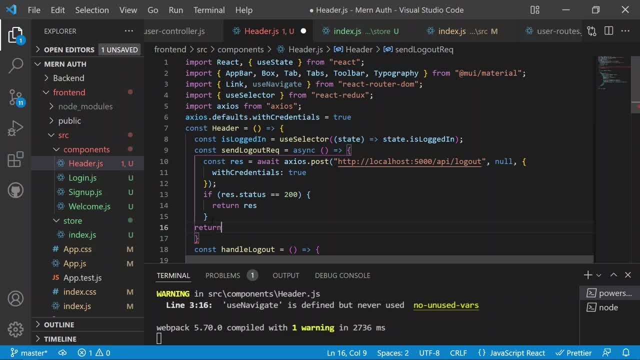 there, there, and then after the- if we can just check. and then after the- if we can just check, and then after the- if we can just check, we can just return the new error. we can just return the new error. we can just return the new error if there would be an error in the logout. 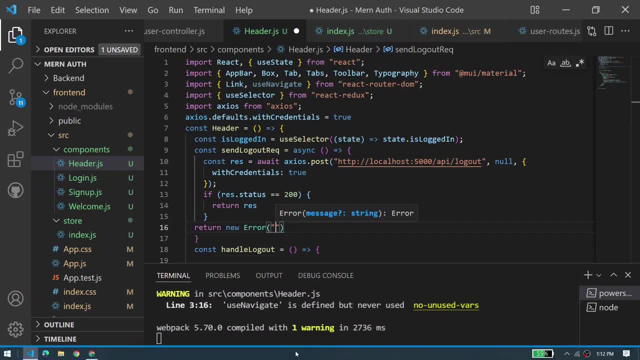 if there would be an error in the logout. if there would be an error in the logout, so we can just return the new error. so we can just return the new error. so we can just return the new error as the unable to log out log out. please try again. 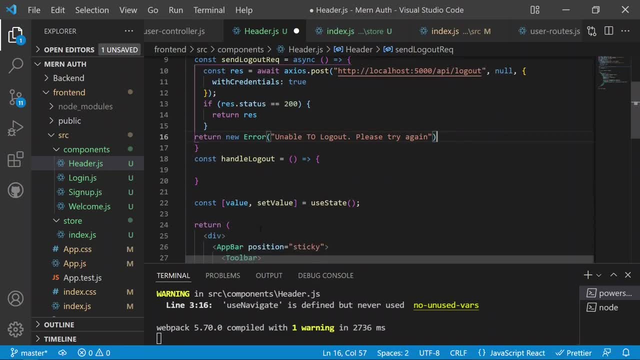 so now we are now sending the return. so now we are now sending the return, so now we are now sending the return statement if there is any error statement, if there is any error statement, if there is any error, and so we can just call this inside the 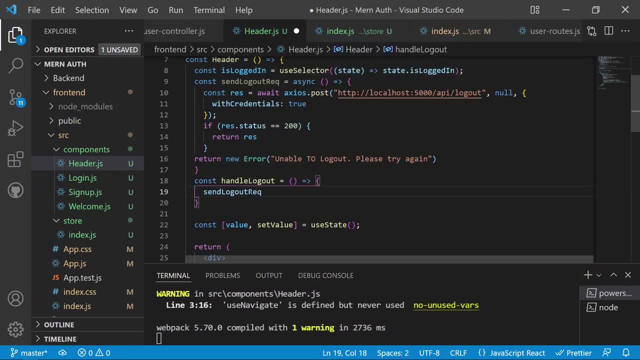 and so we can just call this inside the and so we can just call this inside the: handle logout. so it will send handle logout. so it will send handle logout. so it will send as the logout request and after calling as the logout request. and after calling as the logout request and after calling the send logout request. 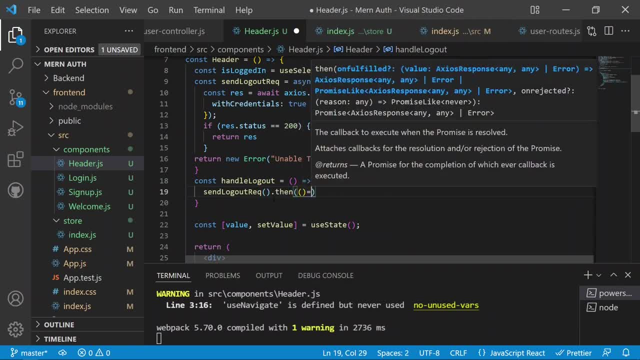 the send logout request, the send logout request, then we can use the then after that, then we can use the then after that, then we can use the then after that, because this is a promise, because this is a promise, because this is a promise, and then now we need to update this. 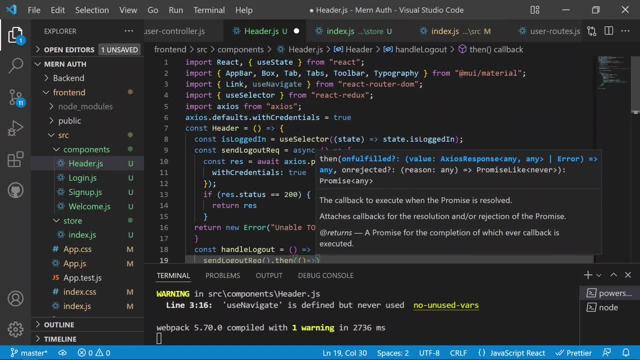 and then now we need to update this, and then now we need to update this state in the redux to the logout state in the redux to the logout state in the redux to the logout. so for that we need to use the use. so for that we need to use the use. 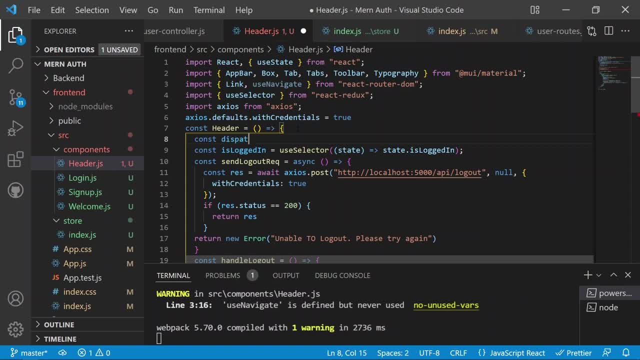 so for that we need to use the use dispatch to dispatch the action dispatch, to dispatch the action dispatch to dispatch the action total. the dispatch will be equals to total. the dispatch will be equals to total. the dispatch will be equals to the use dispatch. so the use dispatch will be then. 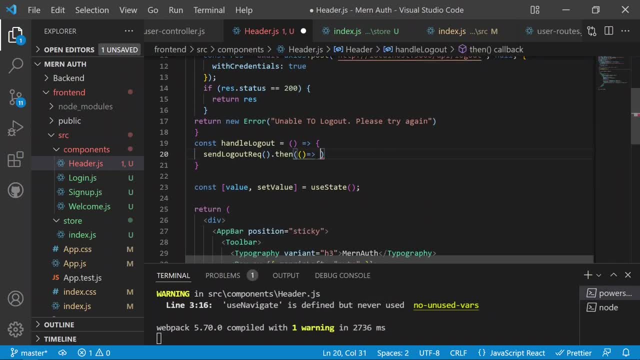 so the use dispatch will be then. so the use dispatch will be then imported from the react redux, imported from the react redux, imported from the react redux, and then we need to dispatch some action, and then we need to dispatch some action, and then we need to dispatch some action like the logout action. so it will the 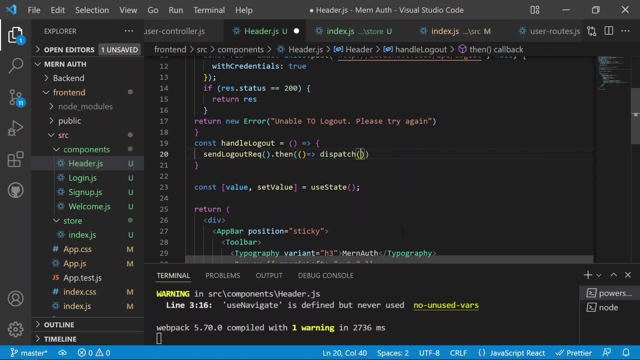 like the logout action, so it will the like the logout action, so it will the dispatch, dispatch, dispatch. and then in it, dispatch- now we need to. and then in it, dispatch, now we need to. and then in it, dispatch, now we need to just import the auth actions that we have. 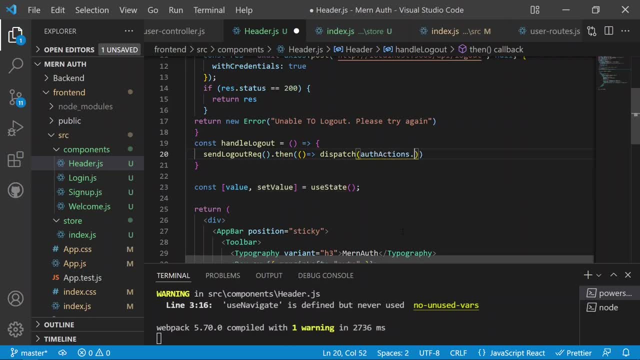 just import the auth actions that we have just import the auth actions that we have just exported, just exported, just exported from the redux. so it will the auth from the redux, so it will the auth from the redux, so it will the auth actions dot. then we have the logout. 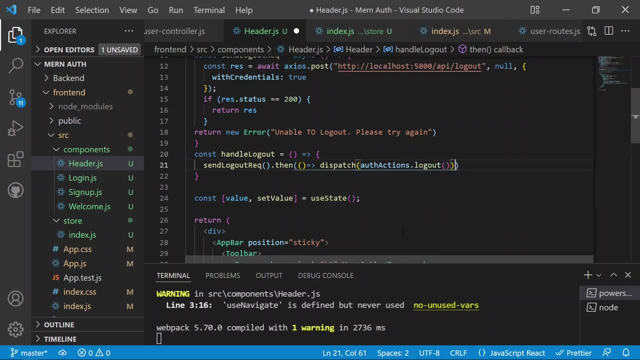 actions dot. then we have the logout actions dot, then we have the logout functionality over there, functionality over there, functionality over there. so we can just call the logout function. so we can just call the logout function. so we can just call the logout function from the auth actions. so after the login, 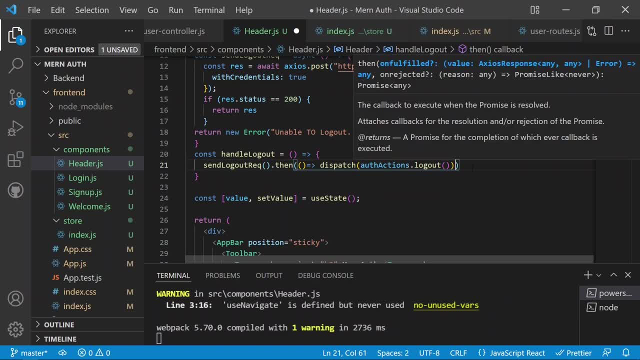 from the auth actions. so after the login, from the auth actions. so after the login request, then we are sending the logout request, then we are sending the logout request, then we are sending the logout request, and then we are moving ahead and request, and then we are moving ahead and. 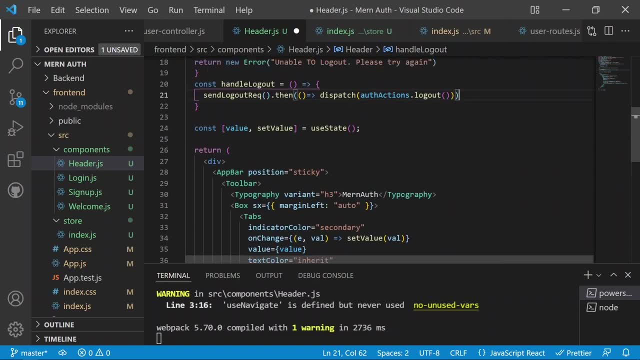 request, and then we are moving ahead, and then we are just going to the main route, then we are just going to the main route, then we are just going to the main route, which is the localhost 3000 only, which is the localhost 3000 only. 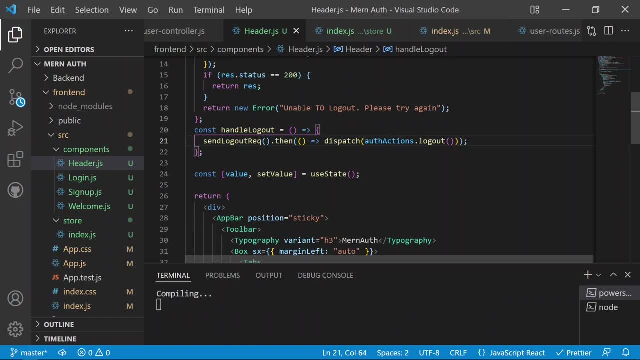 which is the localhost 3000 only. so if i will now save now we can check. so if i will now save now we can check. so if i will now save now we can check the application again, the application again, the application again. i think there is an error. 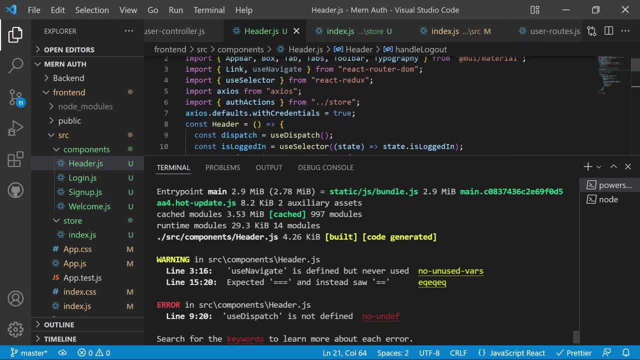 i think there is an error. i think there is an error. so use dispatch is not defined, so i so use dispatch is not defined, so i so use dispatch is not defined, so i think use dispatch is not imported. think use dispatch is not imported. think use dispatch is not imported, we can just import it again. 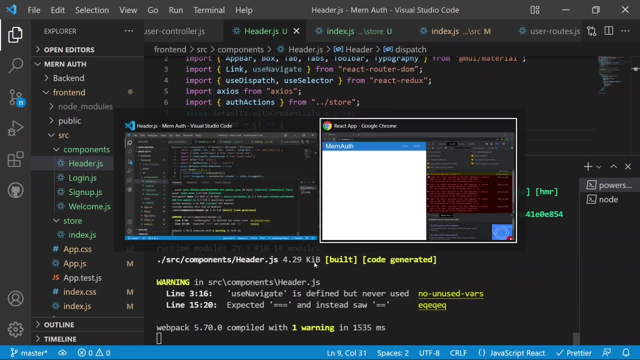 so now the use dispatch is also. so now the use dispatch is also. so now the use dispatch is also imported. now we can see there is no any imported. now we can see there is no any imported. now we can see there is no any error, error, error. and now we can move on to the 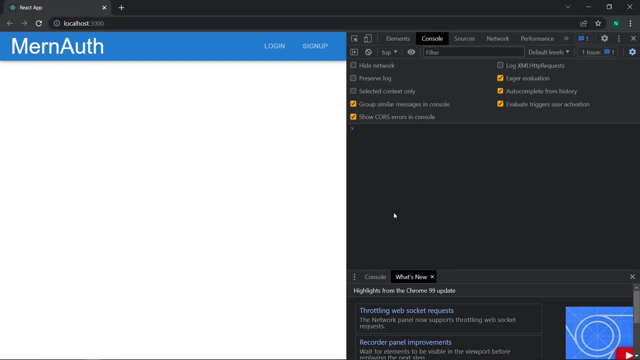 and now we can move on to the and now we can move on to the application again, and i will refresh application again, and i will refresh application again and i will refresh again, again, again. and now you can see: initially it is false. and now you can see, initially it is false. 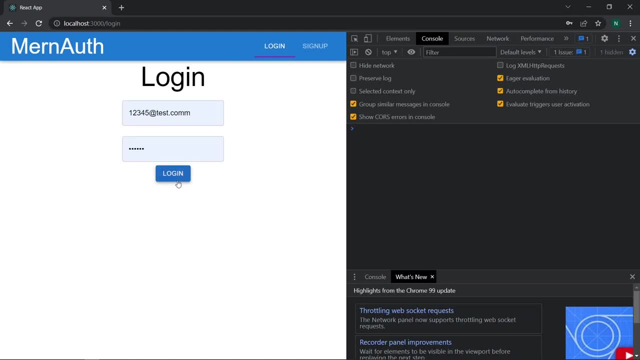 and now you can see. initially it is false. once i will click on the login, once i will click on the login, once i will click on the login, i will now log in. i will now log in. i will now log in. now you can see, now we have the user and. 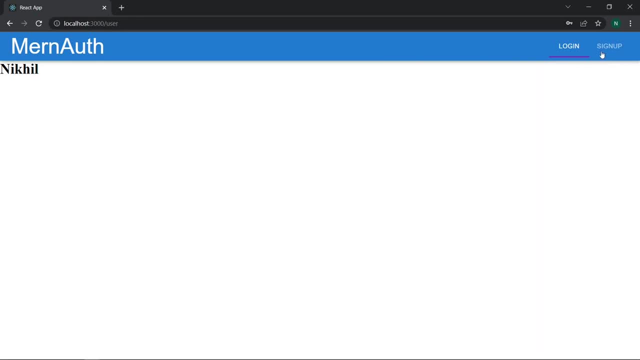 now you can see: now we have the user and now you can see: now we have the user and now the login is working fine. now the login is working fine, now the login is working fine and we don't see the logout route here. and we don't see the logout route here. 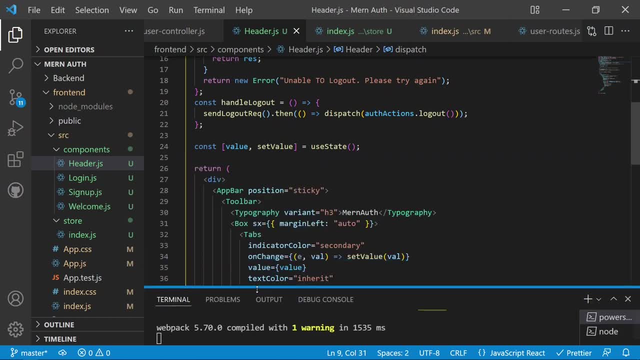 and we don't see the logout route here because i think we are not dispatching, because i think we are not dispatching, because i think we are not dispatching the action on the login, so we can just the action on the login, so we can just. 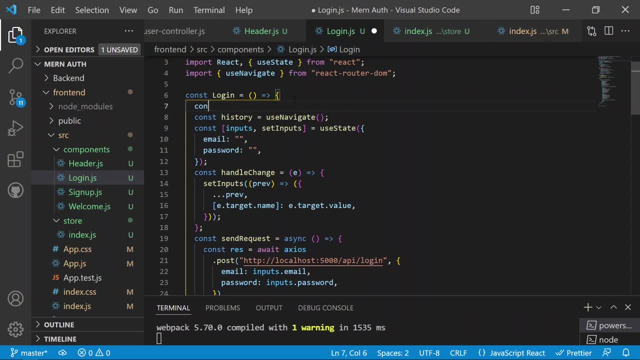 the action on the login, so we can just move on to the login again, move on to the login again, move on to the login again, and then we can just create the dispatch, and then we can just create the dispatch, and then we can just create the dispatch again like the cons dispatch. 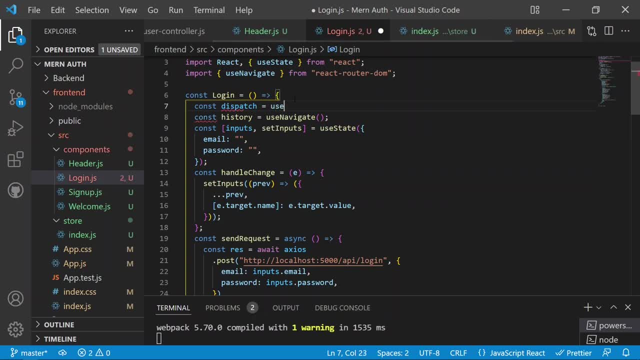 again like the cons dispatch, again like the cons dispatch. so we need to dispatch the login action. so we need to dispatch the login action. so we need to dispatch the login action here also. so it will use dispatch again. so use dispatch will be then imported and so use dispatch will be then imported and. 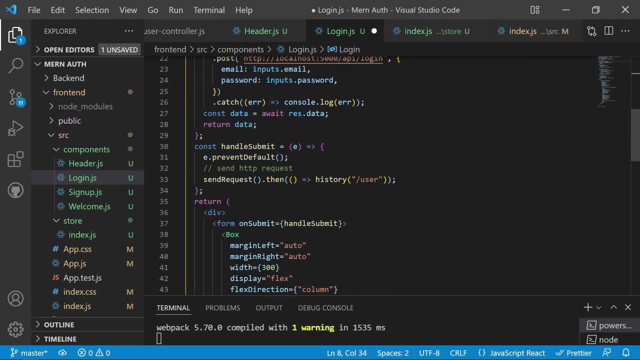 so use dispatch will be then imported, and then after the login is done, then after the login is done, then after the login is done, after the handle submitting done, and then after the handle submitting done, and then after the handle submitting done, and then we are now going to the history user. 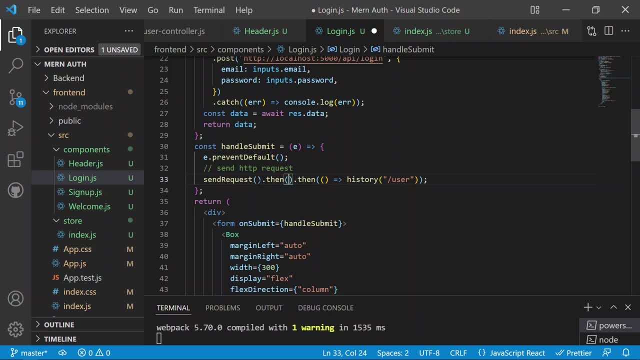 we are now going to the history user. we are now going to the history user, and before this, then we can just use on, and before this, then we can just use on, and before this, then we can just use on. the then again, the then again, the then again, and then this will be a callback again. 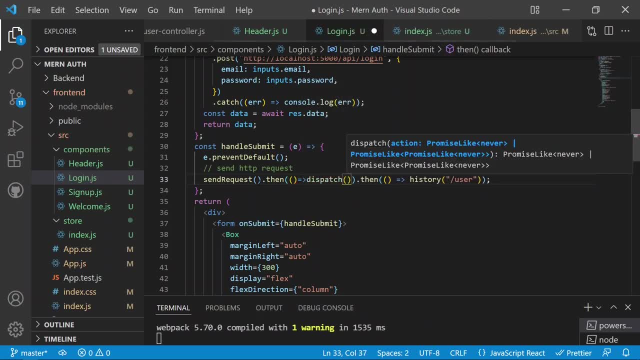 and then this will be a callback again, and then this will be a callback again. so we need to dispatch here, so we need to dispatch here, so we need to dispatch here. the action again, so it will be the auth. the action again, so it will be the auth. 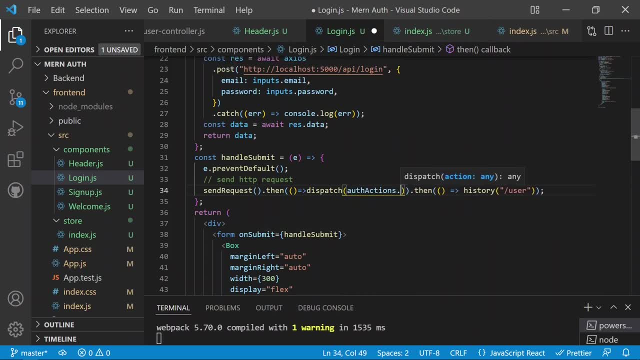 the action again. so it will be the auth action, action, action, auth actions. we will then import and it auth actions. we will then import and it auth actions. we will then import and it will dot login function. will dot login function, will dot login function. so we will call the login function there. 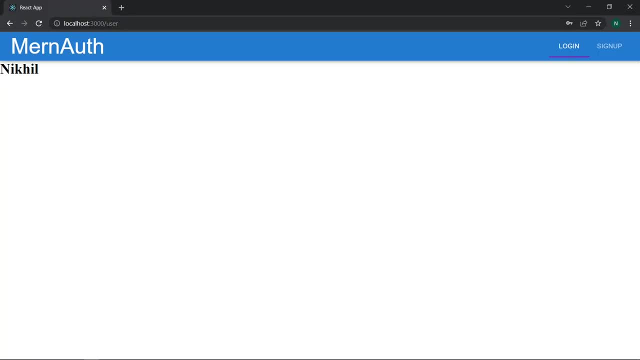 so we will call the login function there. so we will call the login function there after that, after that, after that, and then, if i will now just to remove, and then, if i will now just to remove, and then if i will now just to remove here the user again, 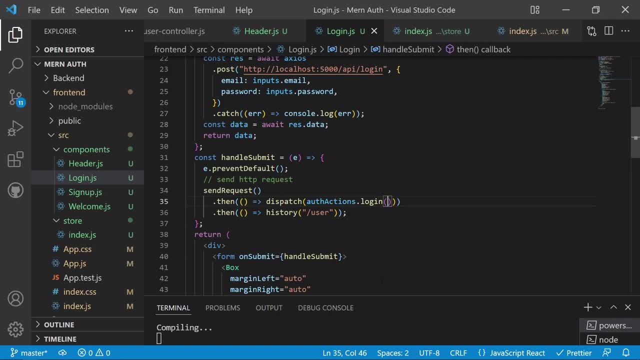 here the user again, here the user again, and then we can just restart the, and then we can just restart the, and then we can just restart the application. application application now. we should see. there should not be now. we should see there should not be now. we should see. there should not be any errors. so once i will click on the, 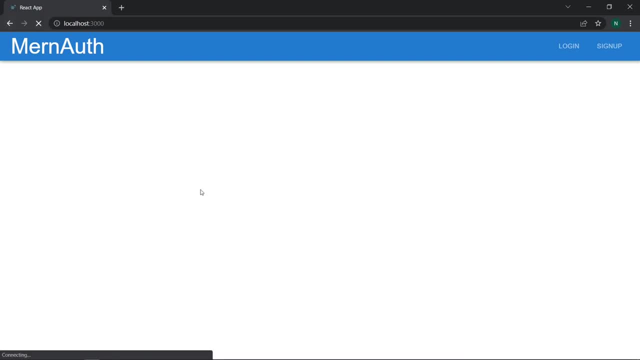 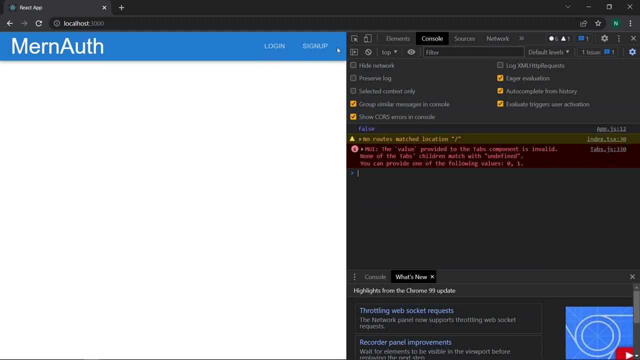 any errors. so once i will click on the: any errors. so once i will click on the login, login, login. i will now refresh again. open the. i will now refresh again. open the. i will now refresh again. open the developer tools now, once i will click on the login. 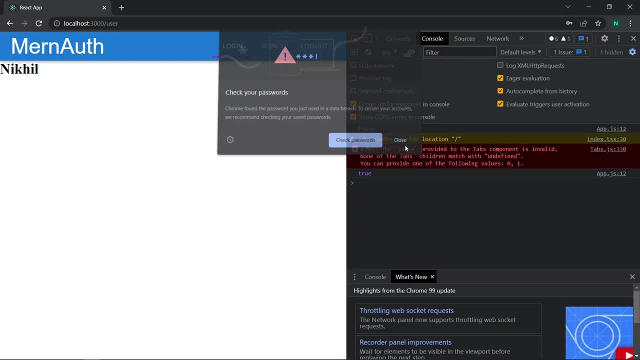 now, if i will now click on the login now, now, if i will now click on the login now, now, if i will now click on the login now we can see: now we have the login state. we can see: now we have the login state. we can see: now we have the login state of the true. now we have the redux rate. 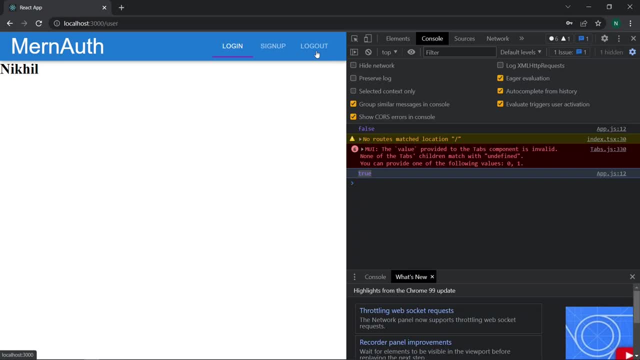 of the true. now we have the redux rate of the true, now we have the redux rate of two, and now you can see, now we have of two and now you can see, now we have of two and now you can see. now we have the logout route as well, and once i will 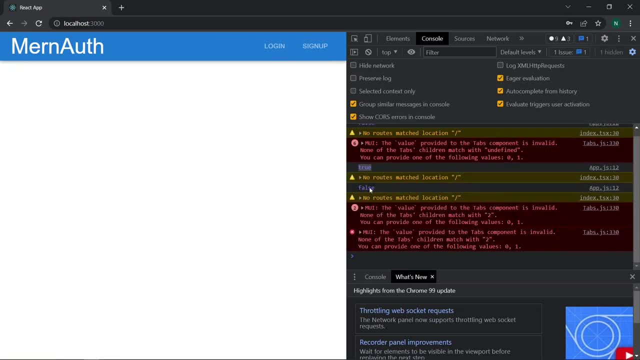 the logout route as well, and once i will the logout route as well, and once i will click on the logout. and now you can see click on the logout. and now you can see click on the logout. and now you can see. now the logout route is completed. 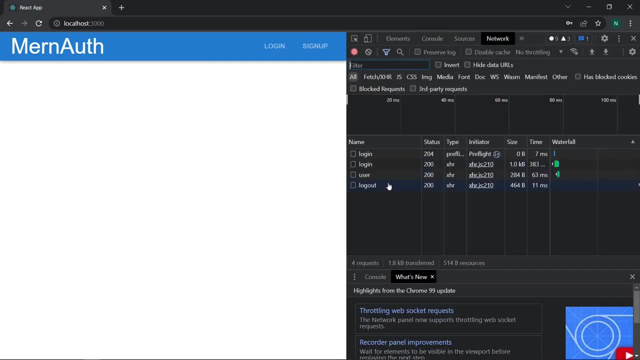 now the logout route is completed, now the logout route is completed successfully, and then, if i will now just successfully, and then if i will now just successfully, and then if i will now just check the network tag also, check the network tag also, check the network tag also. now you will see the logout tab is. 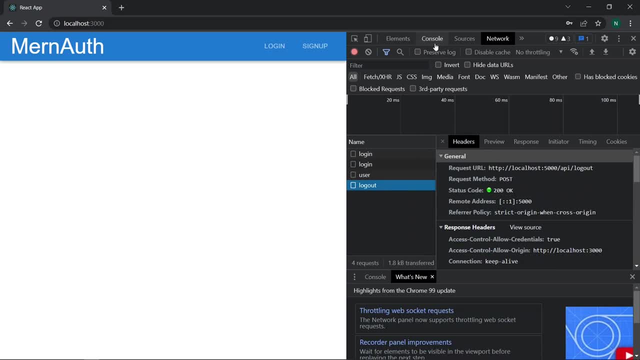 now you will see, the logout tab is- now you will see. the logout tab is successfully created, successfully created, successfully created. and now this status equals to 200, which. and now this status equals to 200, which. and now this status equals to 200, which is okay. and now everything is working. 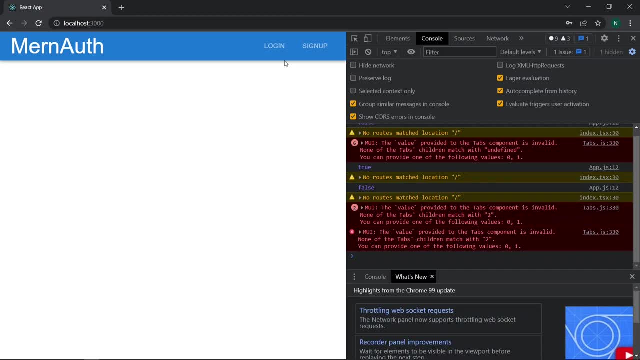 is okay, and now everything is working is okay. and now everything is working fine, and now we need to fix one more fine. and now we need to fix one more fine. and now we need to fix one more thing: when we are now logged in, and then thing: when we are now logged in, and then 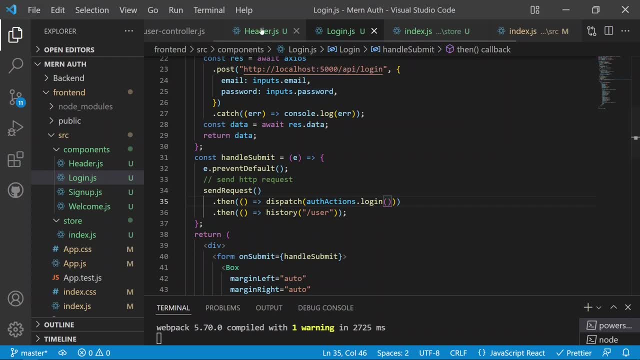 thing when we are now logged in, and then we can still see the login and the sign. we can still see the login and the sign. we can still see the login and the sign up. so we can just move on to the header up. so we can just move on to the header. 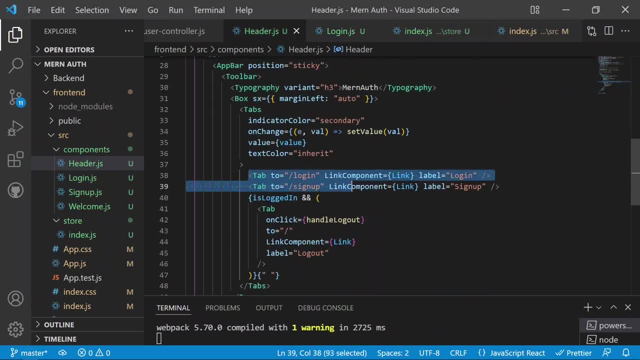 up, so we can just move on to the header again. we can just again, we can just again, we can just conditionally render these two tabs as conditionally render these two tabs, as conditionally render these two tabs as well. so we can just add here the: 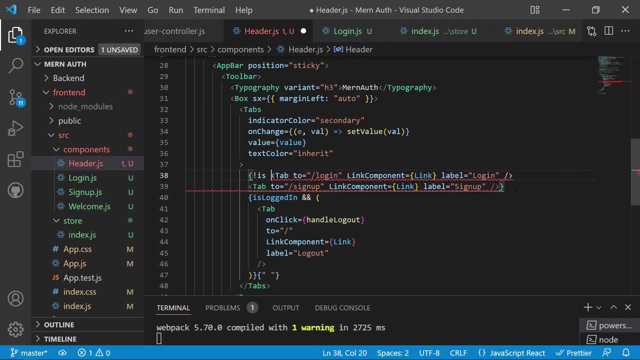 well, so we can just add here the well, so we can just add here the condition for the: if the logged in is condition for the, if the logged in is condition for the, if the logged in is false, if the is logged in is the false and if the is logged in is the false. and 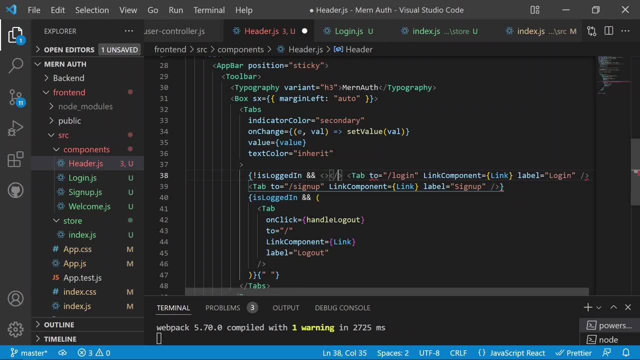 if the is logged in, is the false, and then only we need to render the tabs, then only we need to render the tabs, then only we need to render the tabs. so we can just wrap the tabs inside the. so we can just wrap the tabs inside the. 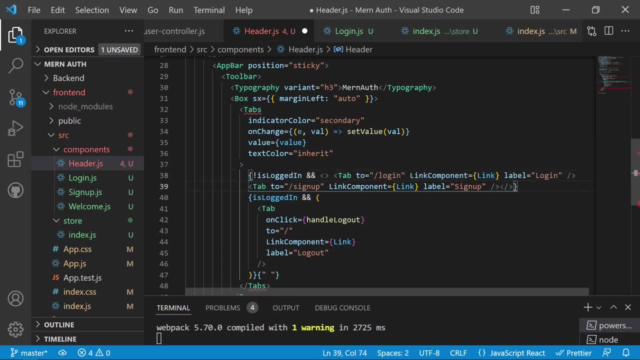 so we can just wrap the tabs inside the empty component as well. empty tags as empty component as well. empty tags as empty component as well, empty tags as well, well, well, so now we are checking the that if the. so now we are checking the that if the. 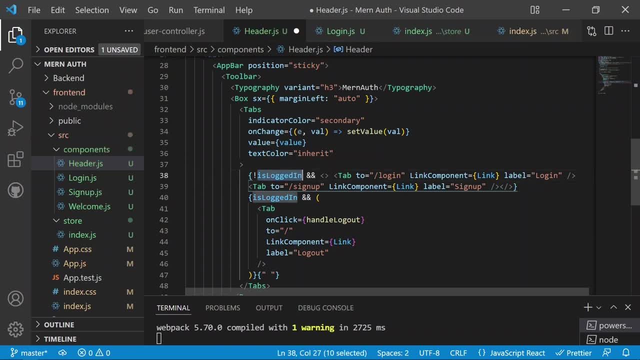 so now we are checking the, that if the is logged in property is false, and then is logged in property is false, and then is logged in property is false, and then only we need to render these two links, only we need to render these two links, only we need to render these two links. and now everything is working fine and 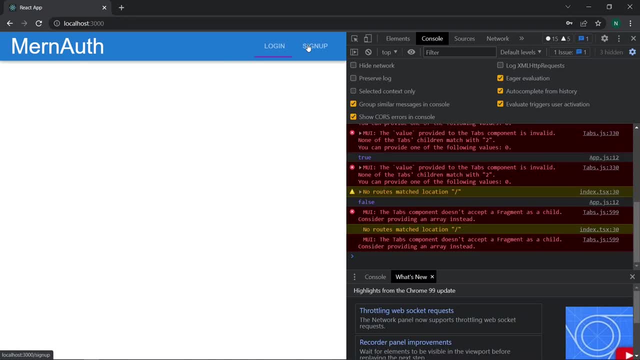 and now everything is working fine. and and now everything is working fine, and we have still only thing which is, we have still only thing which is, we have still only thing which is remaining, because, if i will click on the remaining, because if i will click on the, 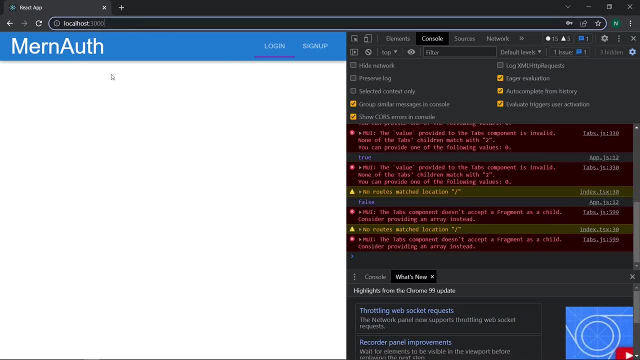 remaining, because if i will click on the log out, log out, log out- and if i will now just move on to the url, and if i will now just move on to the url, and if i will now just directly access the, and if i will now just directly access the, 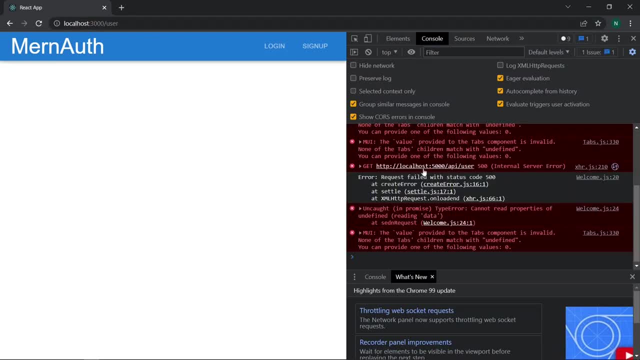 and if i will now just directly access the user, so now you will see we are now user. so now you will see we are now user. so now you will see we are now able to go to the user and it will throw. able to go to the user and it will throw. 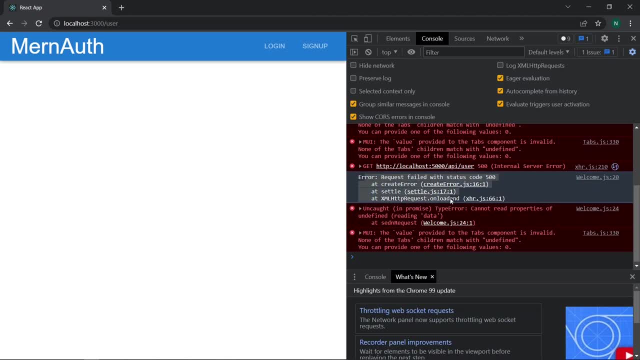 able to go to the user and it will throw us an error because it is showing us an us an error, because it is showing us an us an error, because it is showing us an error because we don't have any error, because we don't have any. 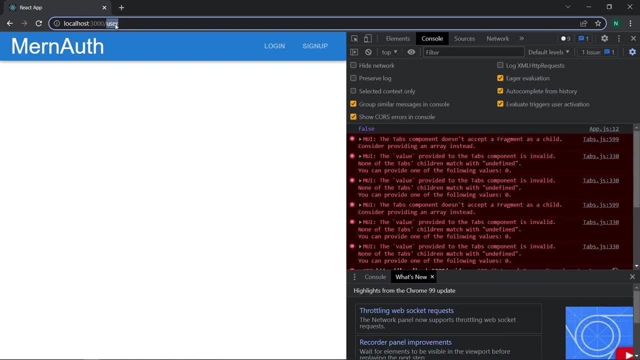 error because we don't have any credentials and we are still moving on credentials and we are still moving on credentials and we are still moving on to the user. so we need to fix that also to the user. so we need to fix that also to the user. so we need to fix that also. so for that we can just move on to the. 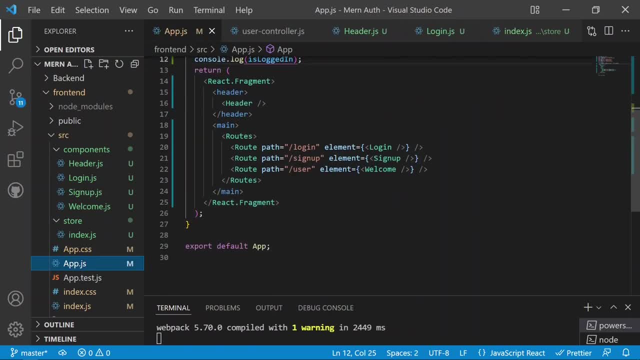 so for that, we can just move on to the, so for that, we can just move on to the appjs, appjs, appjs, and that we need to just create this and that we need to just create this, and that we need to just create this route as the protected route, so we can. 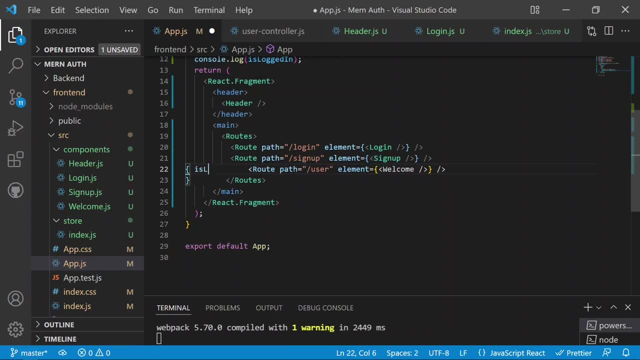 route as the protected route, so we can route as the protected route, so we can just create that, so we can just create. just create that, so we can just create, just create that, so we can just create. by the: by the is logged in, so once the by the by the is logged in, so once the. 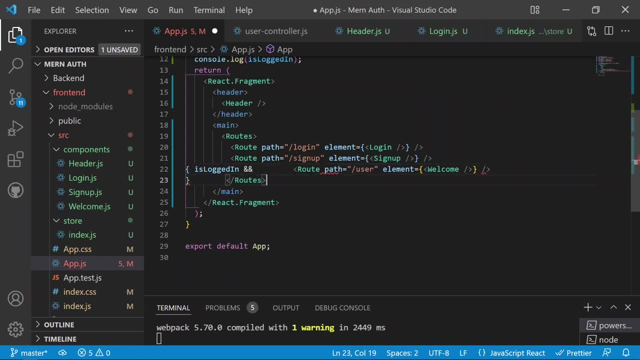 by the, by the is logged in. so once the is logged in, equals to the true, is logged in, equals to the true, is logged in, equals to the true, and then only this route will work, and then only this route will work, and then only this route will work. so this is the new condition: that if the 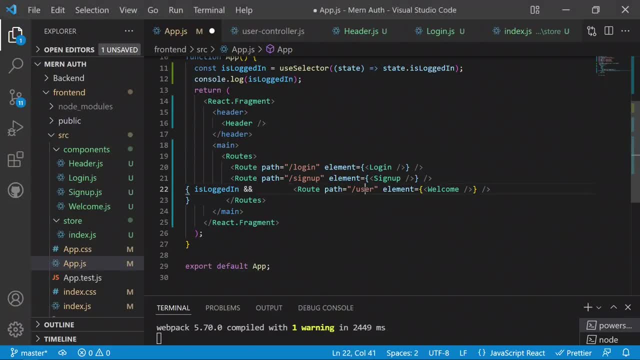 so this is the new condition, that if the so this is the new condition, that if the is logged in property is true, and then is logged in property is true, and then is logged in property is true, and then only we are able to render this route, only we are able to render this route. 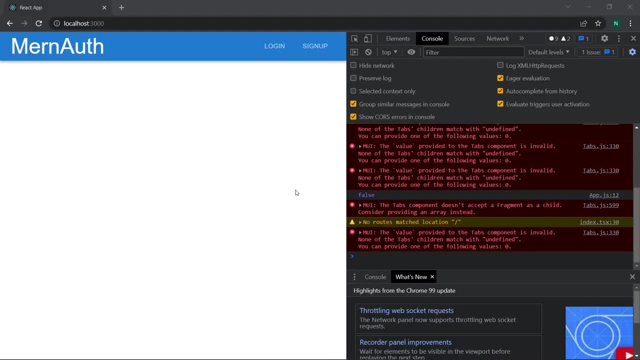 only we are able to render this route. if i will now save, so now we should see. if i will now save, so now we should see. if i will now save, so now we should see if everything would work fine now you. if everything would work fine now you. 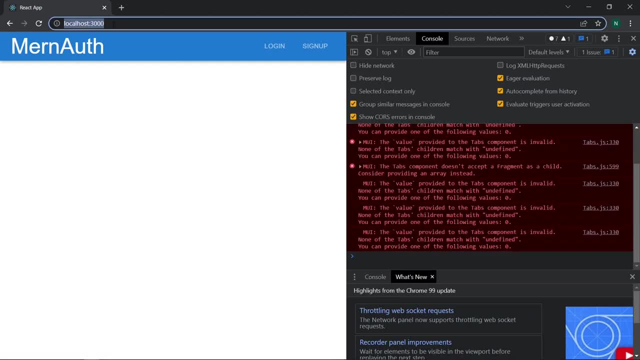 if everything would work fine. now you can see if i will now refresh the page, can see if i will now refresh the page, can see if i will now refresh the page again, again, again, if i will now just enter the user route, if i will now just enter the user route, 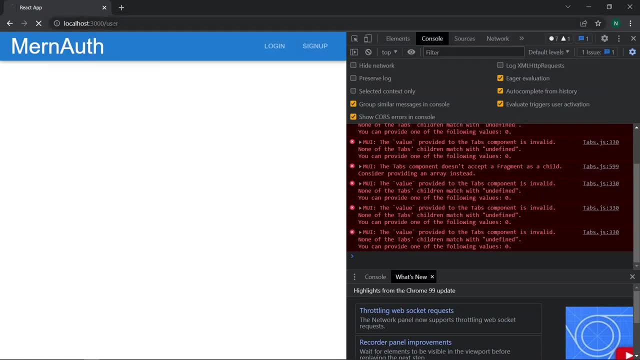 if i will now just enter the user route without the login, without the login, without the login. thoughtful the slash user. thoughtful, the slash user. thoughtful, the slash user. so now you can see the error is now gone. so now you can see the error is now gone. so now you can see the error is now gone, because it was sending the http request. 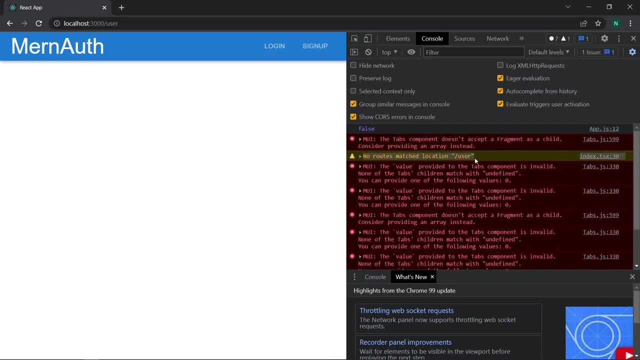 because it was sending the http request. because it was sending the http request. and then you can see now the no routes. and then you can see now the no routes. and then you can see now the no routes. match for the location user. match for the location user. 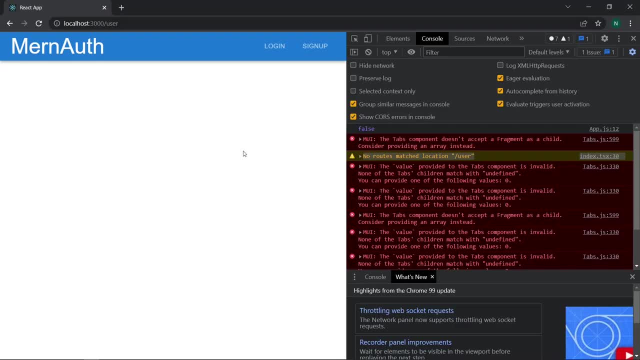 match for the location user. because now we are currently not, is because now we are currently not, is because now we are currently not is logged in. logged in, logged in. now we are logged out and once i will. now we are logged out and once i will. now we are logged out and once i will click on the login, if i will click on. 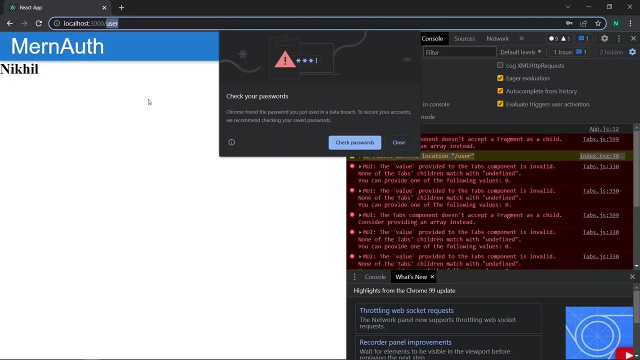 click on the login. if i will click on click on the login. if i will click on the login, now you can see we are now the login. now you can see we are now the login. now you can see we are now moving ahead to the user and once i will